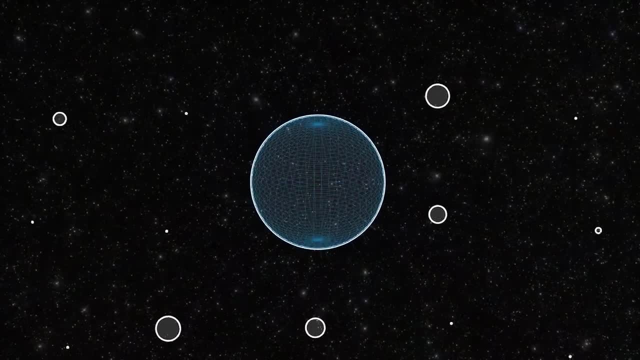 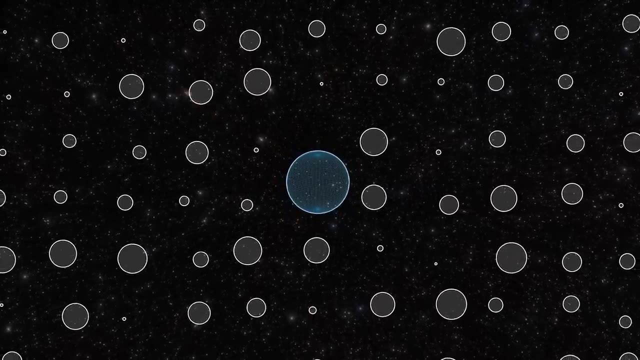 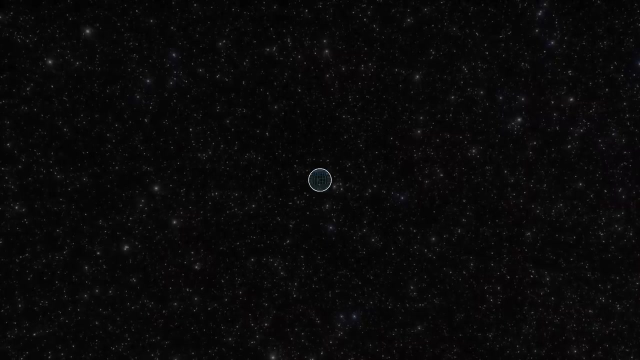 that put Bang in Big Bangpangan and which set the stage of everything that anyways should happen. Enormous prices, prices・ would continue elsewhere, eternally producing bubble universes distributed through a potent, everlasting multiverse. Or perhaps our current universe is merely the latest in a long and 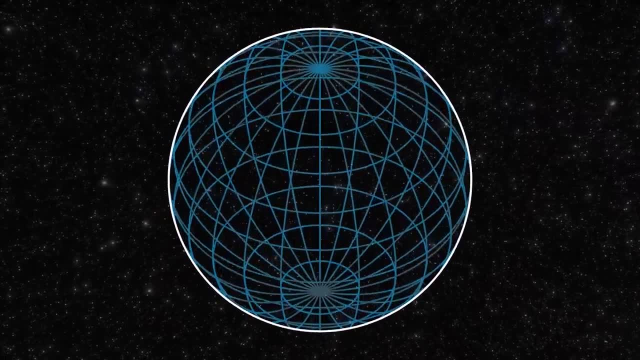 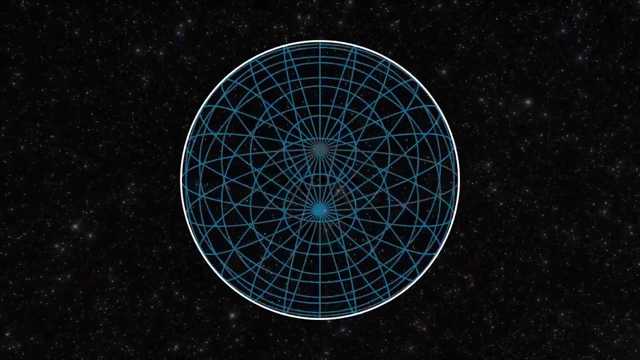 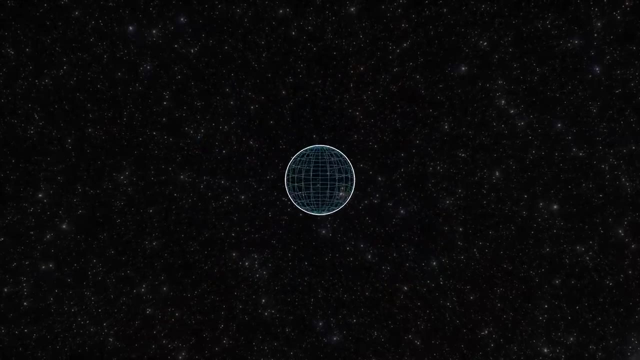 potentially infinite series of expanding and contracting cosmos, a theory known as the big bounce. In this, instead of starting from nothing and inflating exponentially to produce the structure we see today, contemporary physicists like Paul Steinhardt suggest a cyclical growth and contraction of everything within the universe. Or perhaps our understanding of scale is 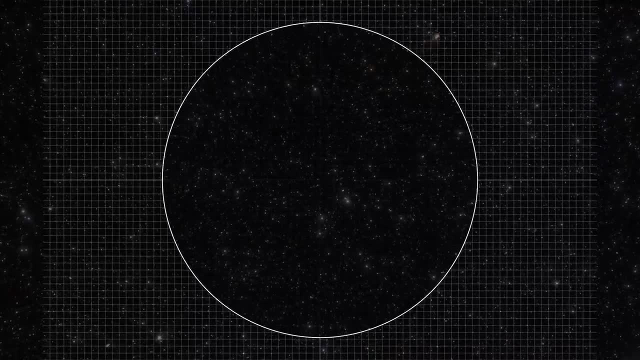 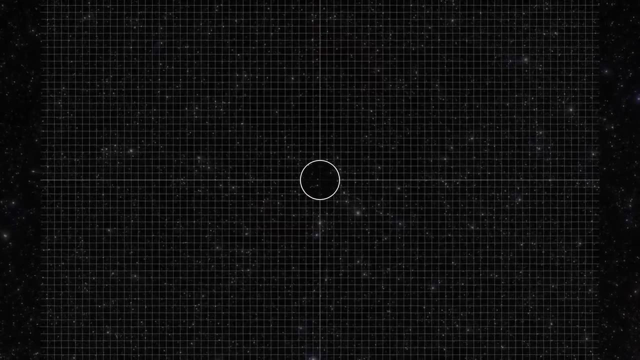 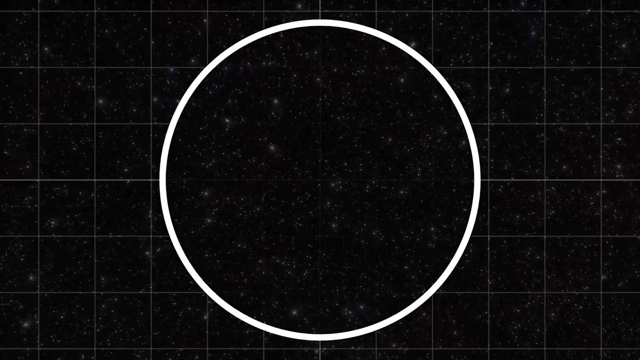 fundamentally incomplete. Physicist Roger Penrose considered the properties of shapes regardless of their size and believes we can do the same with the cosmos. In this idea, the universe loses a sense of time and scale at the infinitely small and the infinitely big and becomes to all intents 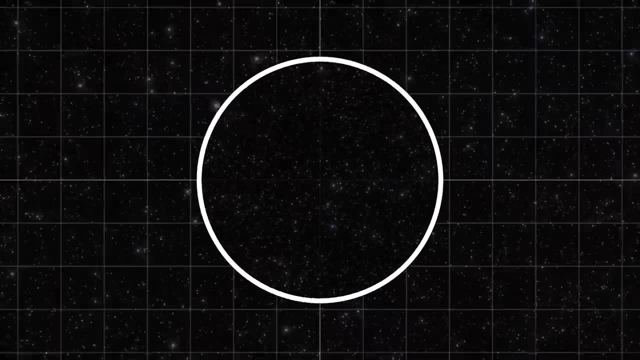 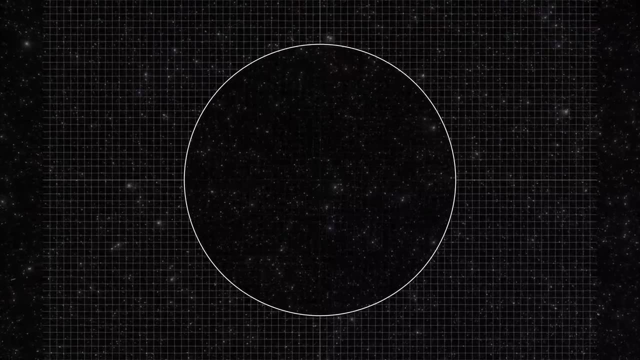 and purposes equivalent. The game of chess played the same whether on a board that fits in your pocket or on a board that fits in your pocket. The game of chess played the same whether on a board that fits in your pocket or spans an entire courtyard. Or perhaps our cosmos came about as a 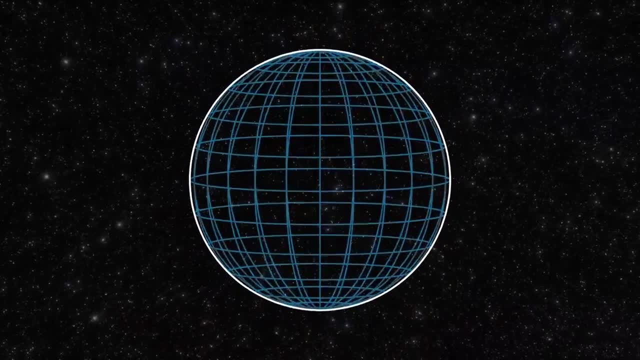 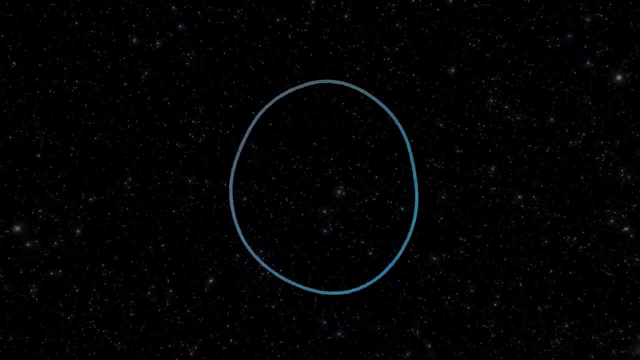 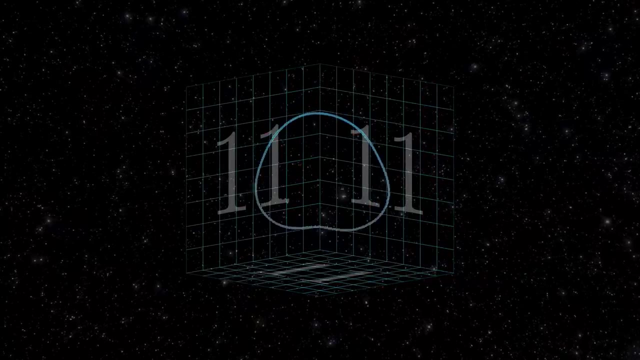 transient collision of dimensions. String theory attempts to explain the fundamentals of reality as tiny vibrating strings within an 11-dimensional reality of hyperspace. The three dimensions of space and one dimension of time that we experience within our cosmos are merely a single brain in the 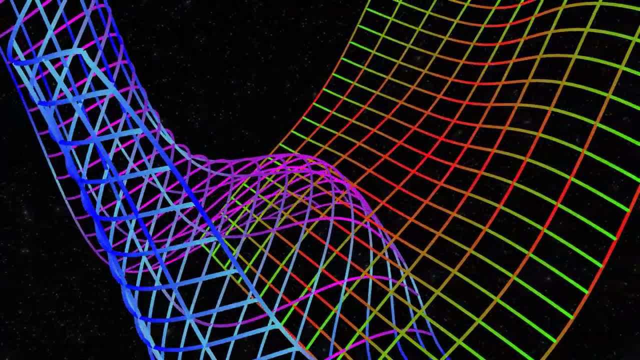 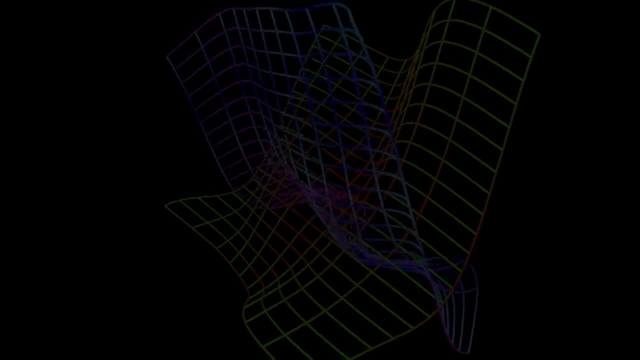 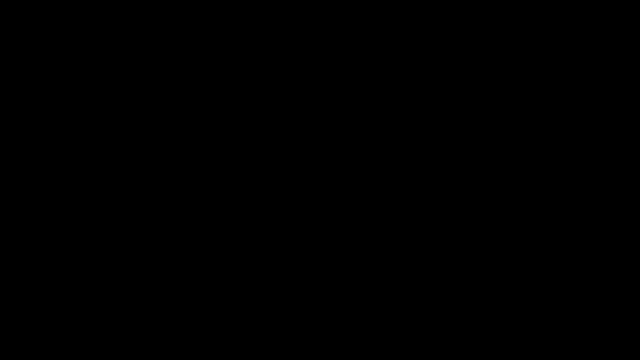 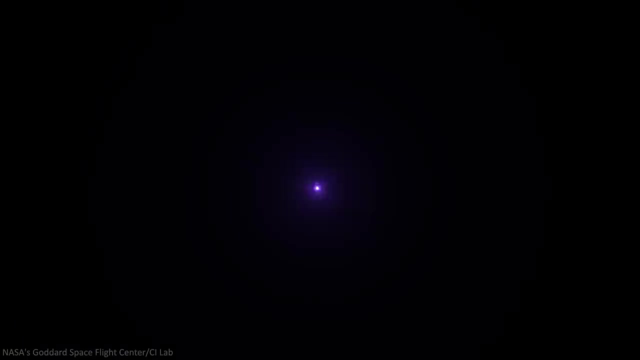 overall bulk, with the beginning and growth of our universe coming about as higher-order brains. Or perhaps there is something else, some corner of mathematics or physics that we have yet to shine a light into and which, for the time being, eludes our understanding. For now, our universe's origin. 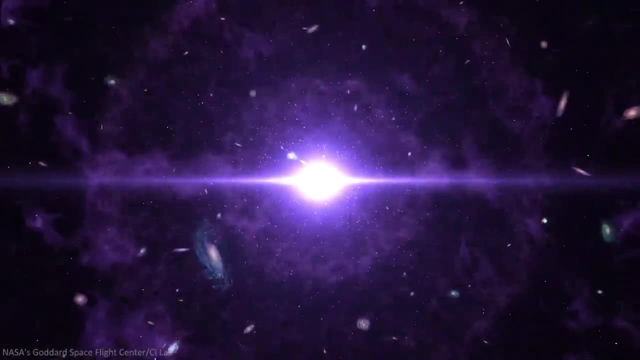 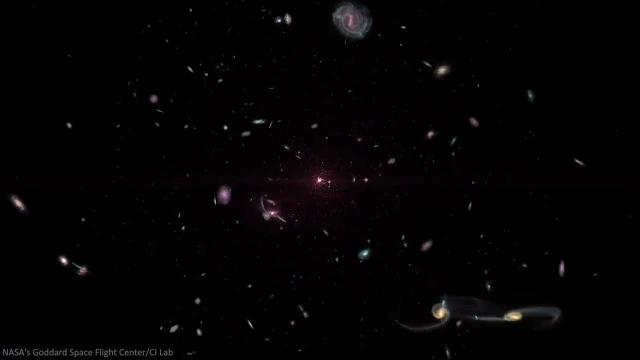 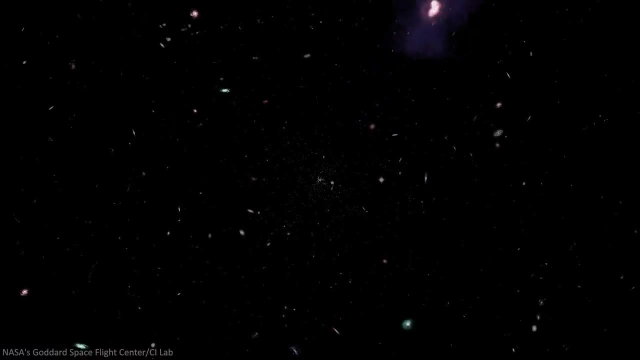 story remains a mystery, a multiple-choice choose-your-own-adventure. Nevertheless, 13.8 billion years ago, the universe was a universe of the universe. The universe was a universe of the universe. So the universe did begin, And this is the story of what happened next. 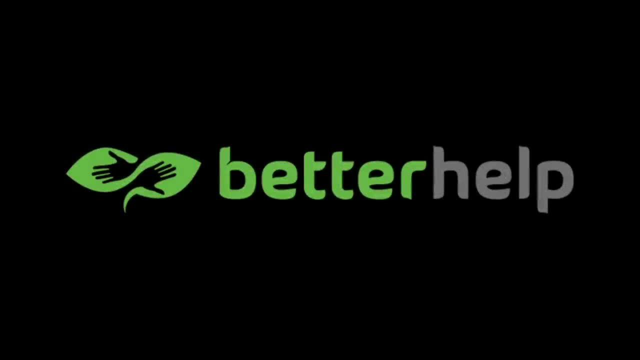 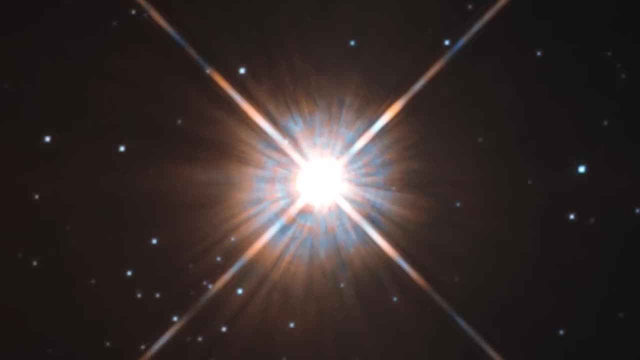 Thank you to BetterHelp for sponsoring this video. This is Proxima Centauri. If we had travelled at more than 50,000 kilometres an hour, it would still take us more than 80,000 years to arrive there. And it is our closest star. It's estimated there are 100,000 million more. 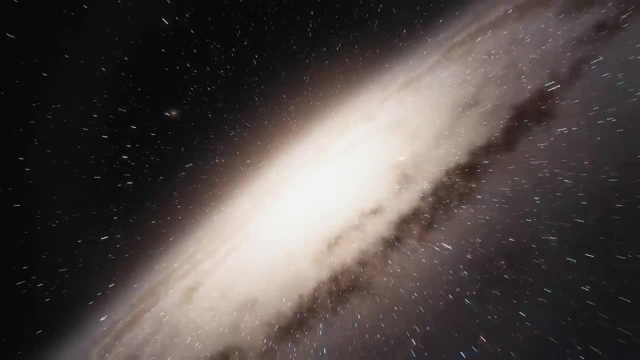 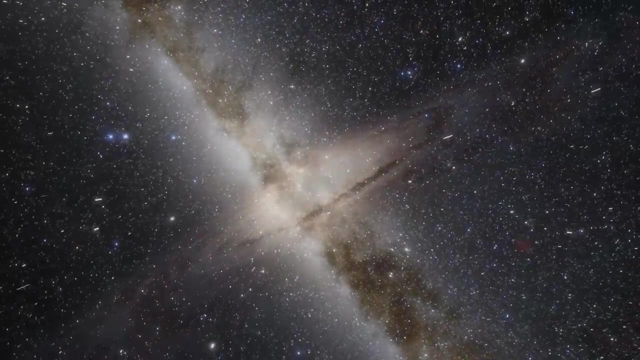 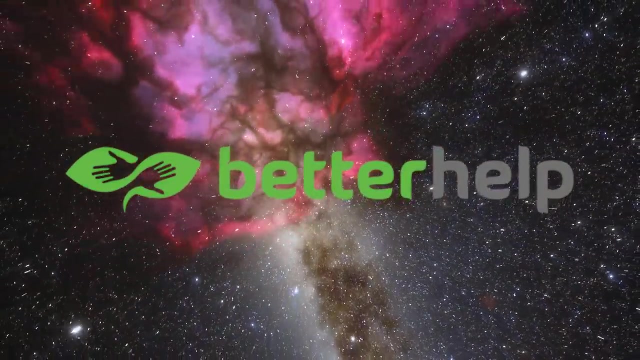 distant stars in the Milky Way, And so sometimes it can be overwhelming to square our own lives with the vastness of everything else And to work these things through it's nice to have some help. BetterHelp is the world's largest therapy service and it's 100% online With BetterHelp. 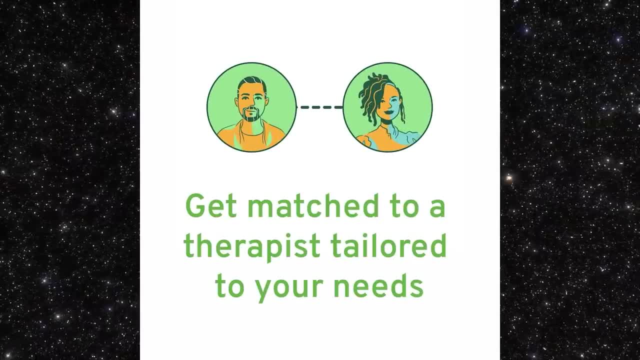 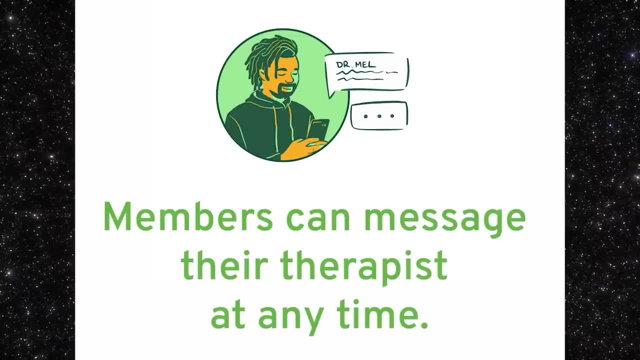 you can tap into a network of over 30,000 licensed and experienced therapists who can help you with a wide range of issues. You can talk to your therapist however you feel comfortable, whether it's via text chat or video call. You can also message your therapist. 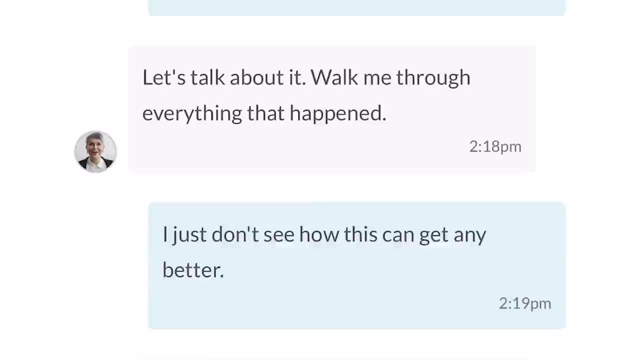 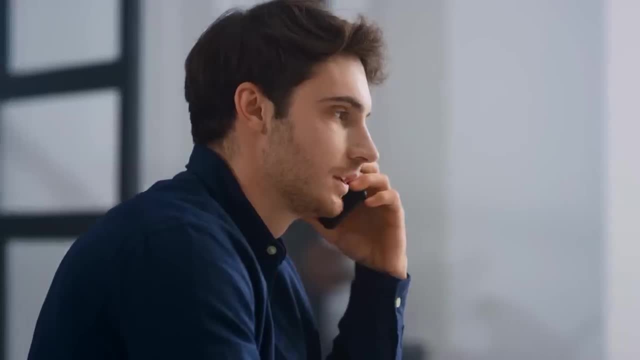 at any time and schedule live sessions when it's convenient for you, And if your therapist isn't the right fit for any reason, you can switch to a new one at no additional charge. With BetterHelp, you get the same professionalism and quality you expect from in-office therapy. 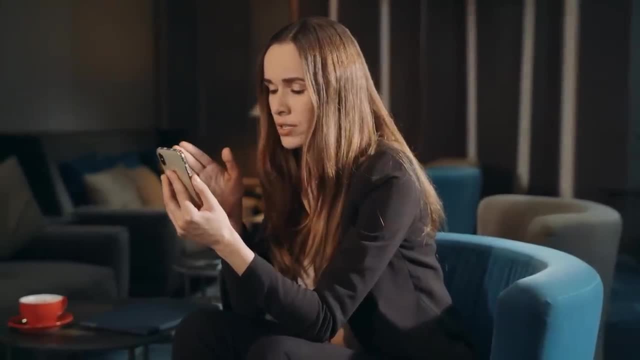 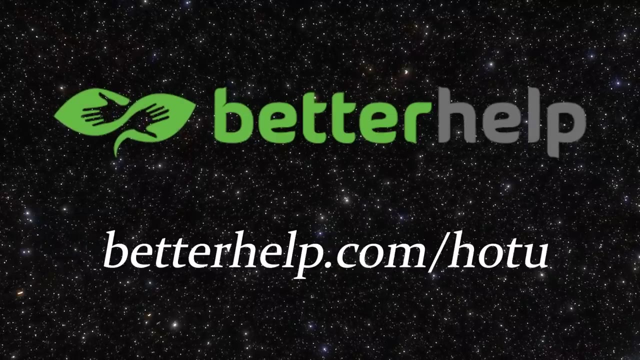 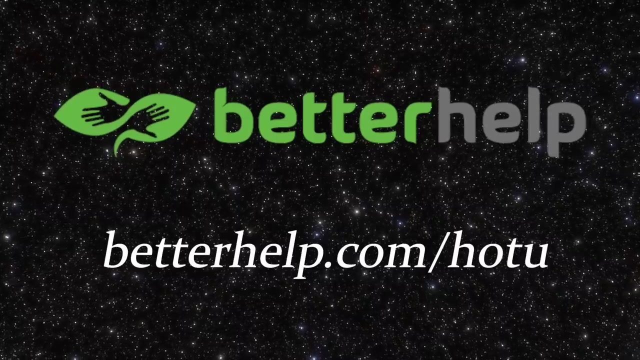 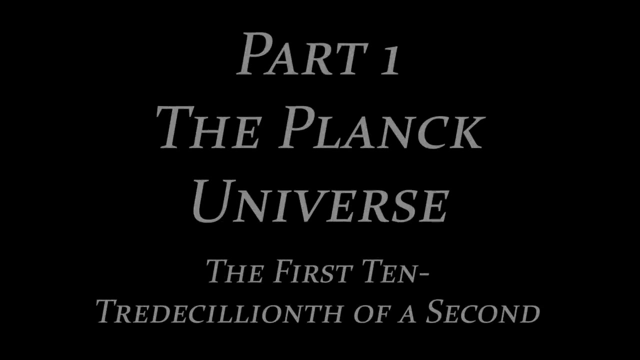 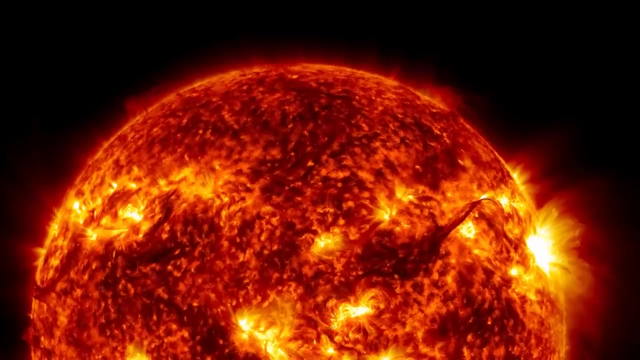 but with a therapist who is custom-picked for you, with more scheduling flexibility and a more affordable price. Thanks to BetterHelp for supporting educational content on YouTube. Where is the hottest place in the universe Universe? You might expect to find it in the natural fusion reactor at the center of a star, but 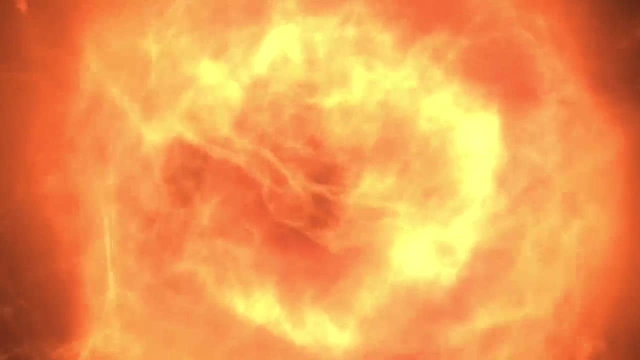 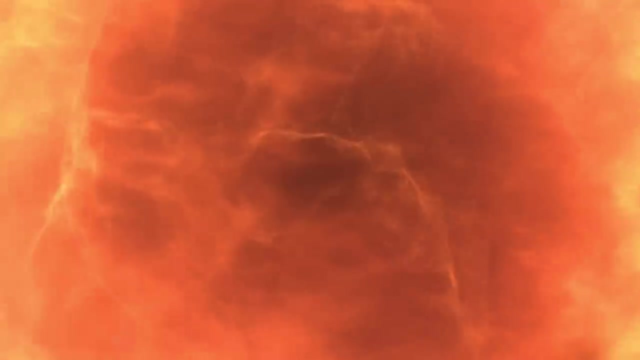 even as you incinerate in the plunge through its fiery depths, your journey would be in vain. Temperatures at the core reach a mere 15 million degrees Celsius. You may look to even more violent phenomena in the cosmos, like explosive supernovae. 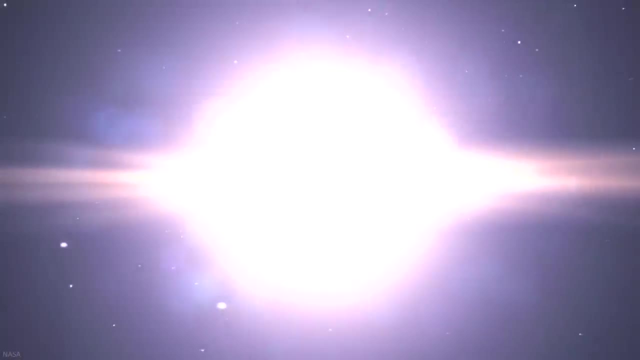 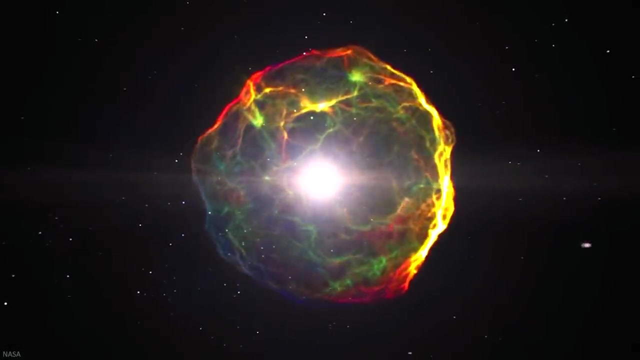 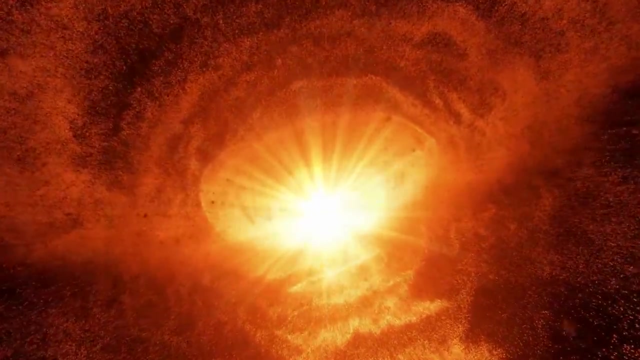 Here, during the dramatic death of a star, superheated shells of gas are ejected many light years in every direction, leaving a gravitationally compactified neutron star at their center. Temperatures here far exceed normal stellar furnaces, reaching 100 billion degrees Celsius. 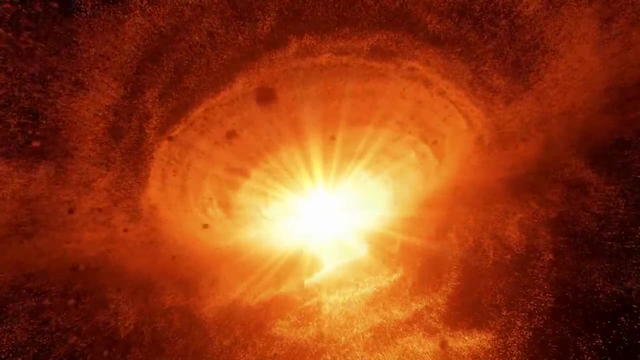 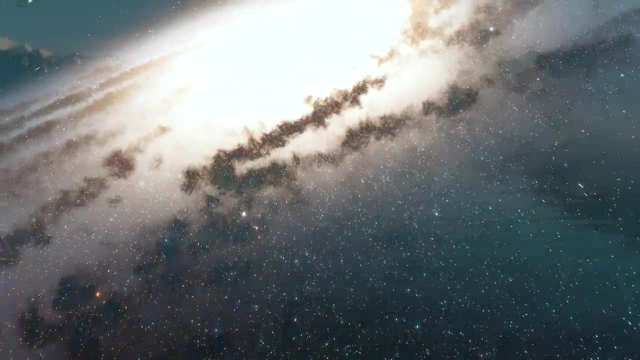 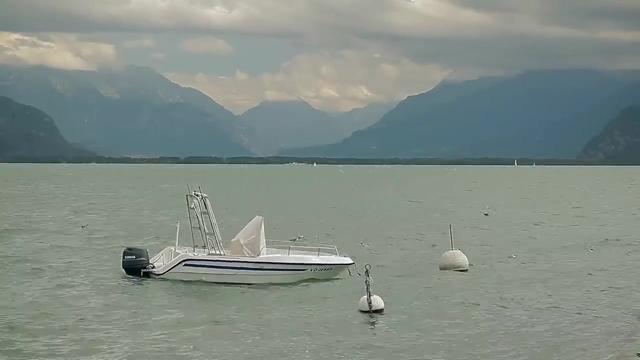 But this still isn't the hottest temperature to be found. In fact, the highest temperature that has ever been recorded anywhere in our vast cosmos was 100 meters beneath the snow-covered ground near the shores of Lake Lamont in Switzerland. And it didn't come about from a natural process, but rather the concerted efforts. 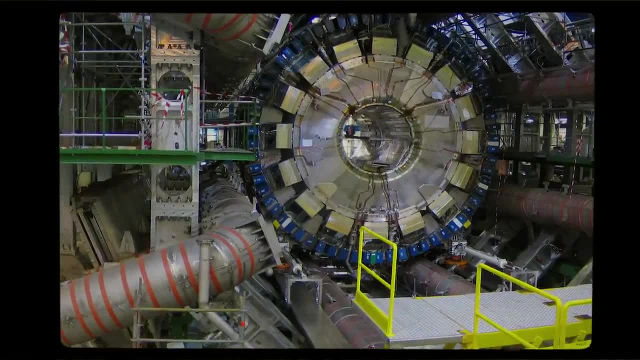 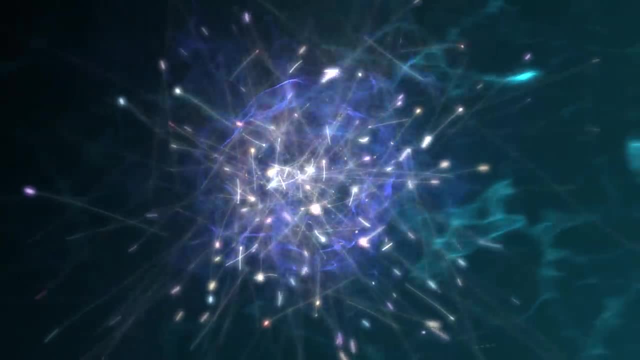 of hundreds of scientists and billions of euros' worth of research and development In CERN's Large Hadron Collider, where individual particles are routinely smashed into one another at velocities approaching the speed of light. the collision of two lead atoms in 2012. briefly, 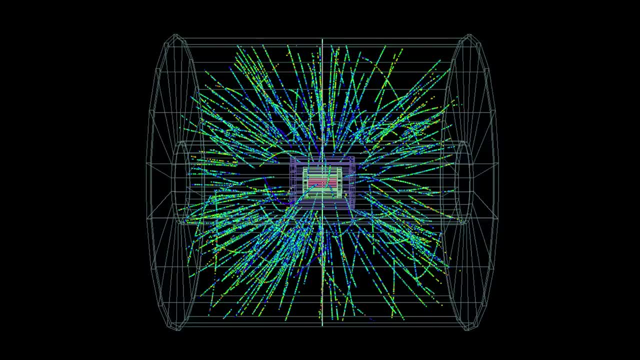 produced a temperature of around 5.5 trillion degrees Celsius. And that's not all. In fact, there's a lot more than that. In fact, there's a lot more than that. In fact, there's a lot more than that. 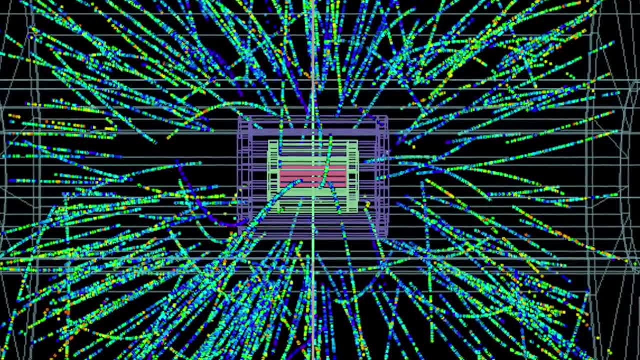 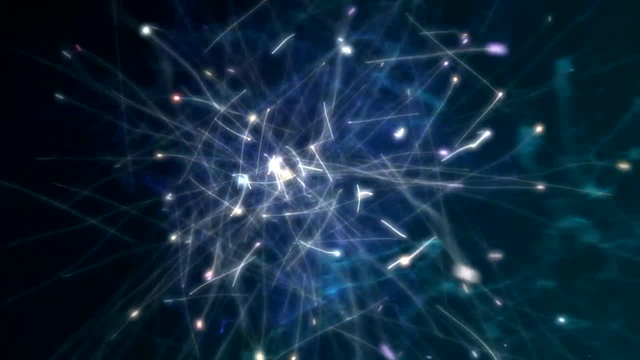 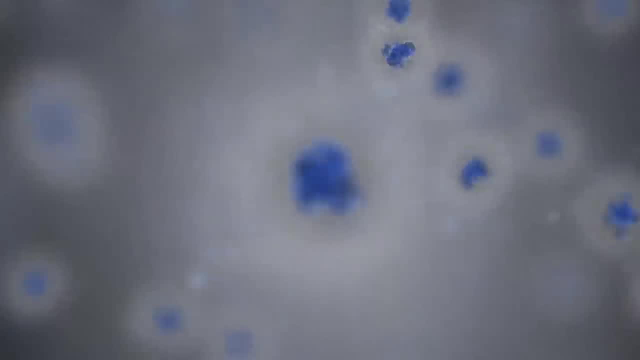 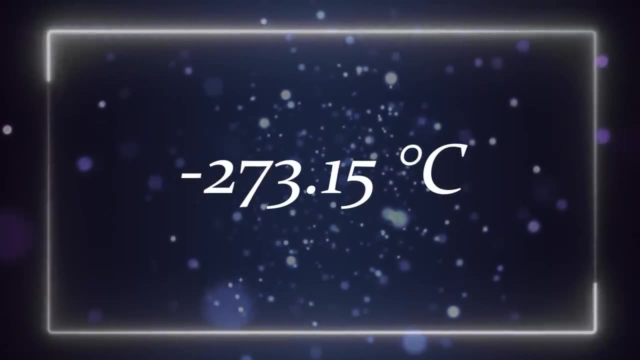 50 times hotter than a supernova, But this still isn't even close to the highest possible temperature. Temperature is little more than a manifestation of a particle's energy, its motion or how fast it's vibrating. Absolute zero, marking zero kelvin is the lowermost limit where particles hypothetically 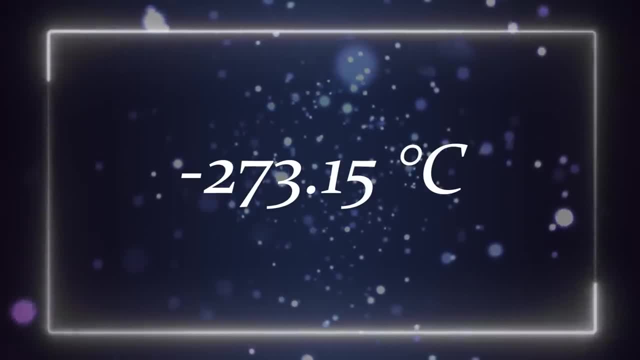 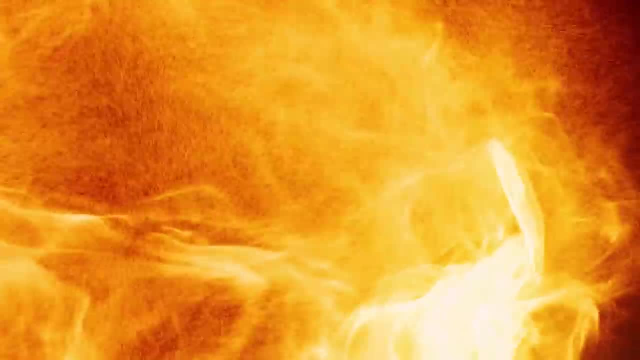 would come to a complete shuddering stop, Whereas, no matter how high the temperature was, 0 would alert the particle to its high it possible to reach. But there is also an upper limit too, an absolute hot that marks the highest temperature before the particles themselves are torn apart by their own energy. 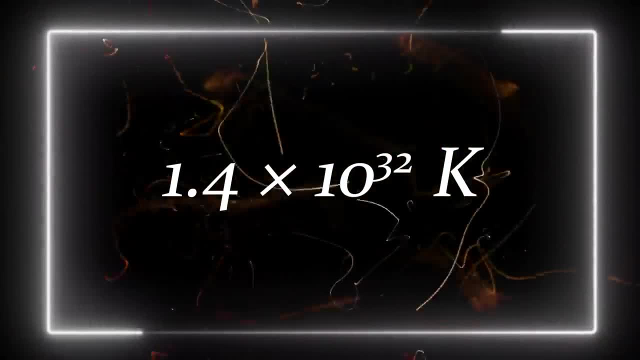 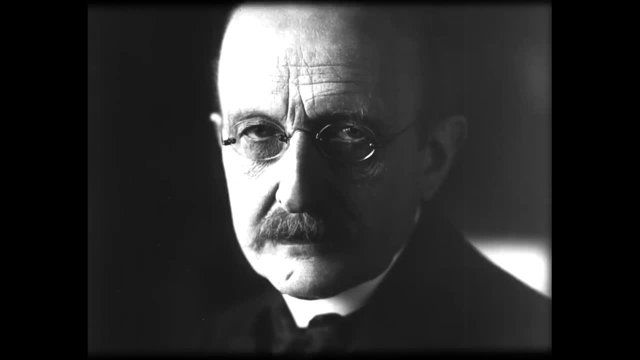 It's known as the Planck temperature, and it is around 1.4 times 10 to the 32 Kelvin. Max Planck, who gave his name to this impossibly blistering temperature, was a German theoretical physicist who found his academic stride around the beginning of the 20th century. His ideas 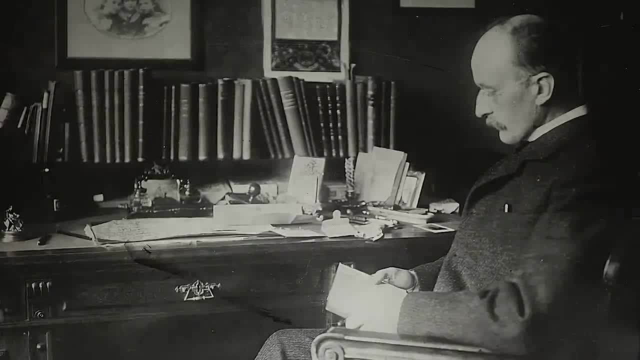 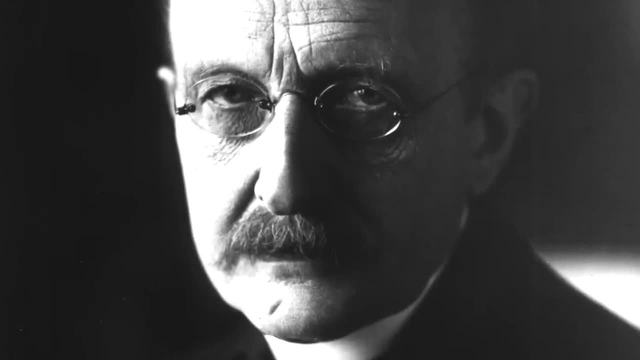 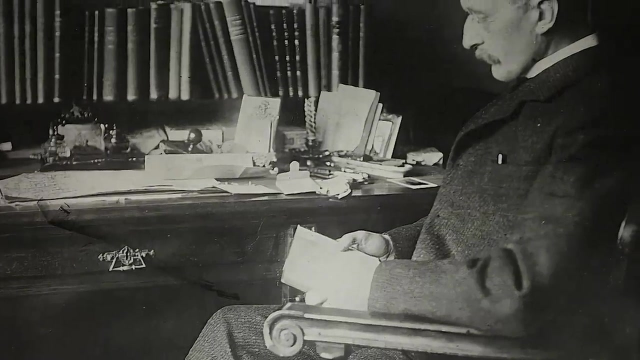 are seen as the founding blocks of quantum physics and led to the quantization of light into discrete chunks of energy called photons, but they also led him to consider the fundamental quanta of other natural phenomena, Using such universal qualities as the speed of light and the force of gravity. in combination with his eponymous Planck constant, he defined 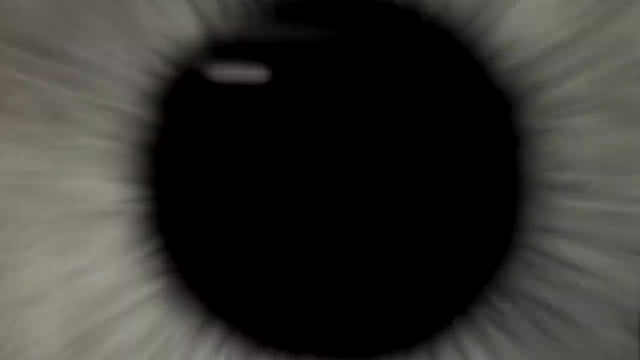 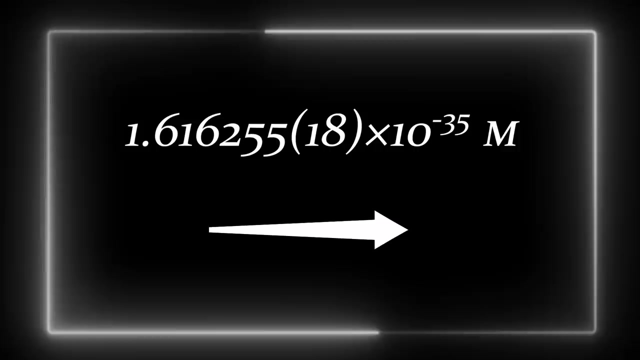 the Planck length, the smallest quantum of distance, as around 1.6 times 10 to the maximum. The Planck length, the smallest quantum of distance, is around 1.6 times 10 to the minus 35 meters, about 100 quintillion times smaller than a proton. 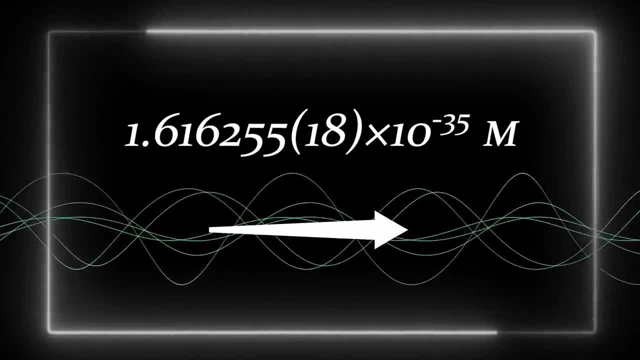 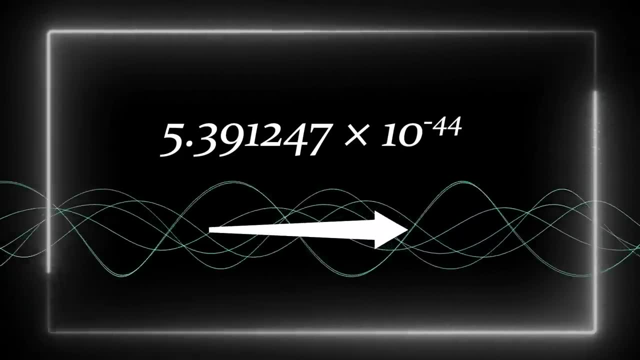 The time it takes for light to travel through this minuscule distance, through a vacuum, is the Planck time, amounting to 5.39 times 10, to the minus 44 seconds, And the Planck temperature, that practical measure of absolute heat, is the temperature. 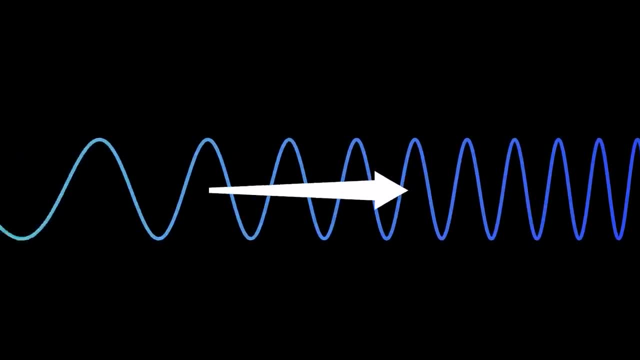 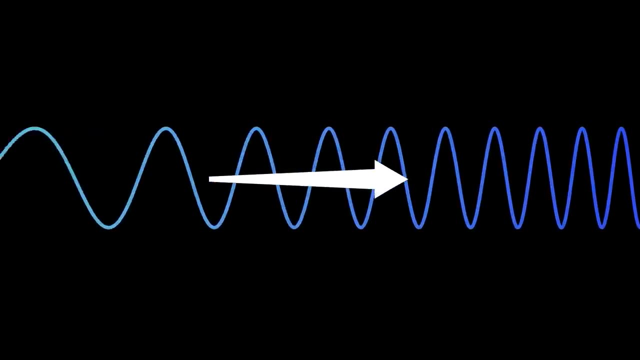 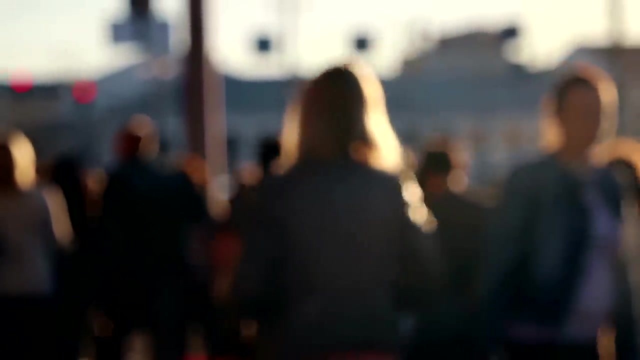 at which the wavelength of thermal radiation reaches the Planck diameter. It can go no smaller. It is no fair reflection on the human brain to say that these numbers are beyond our true comprehension. We are evolutionarily attuned to scales that are relevant to us, and so it may seem that 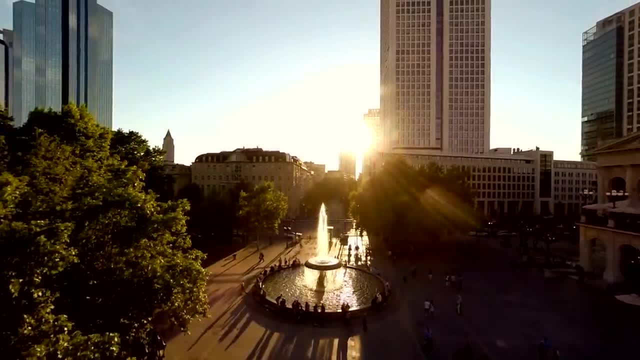 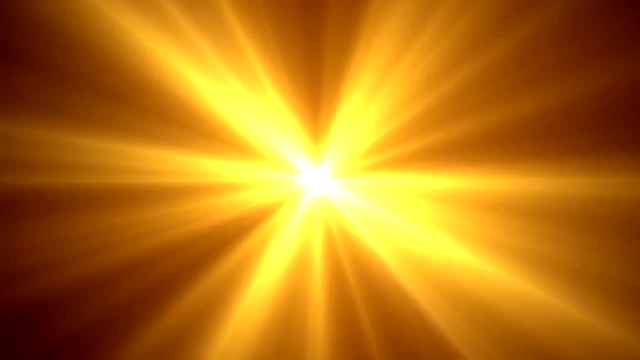 these Planck units are too small or, in the case of temperature, too large to be of any practical use. But it is when contemplating the immeasurably tiny moment at the beginning of our immeasurably vast cosmos that these units really come into their own. 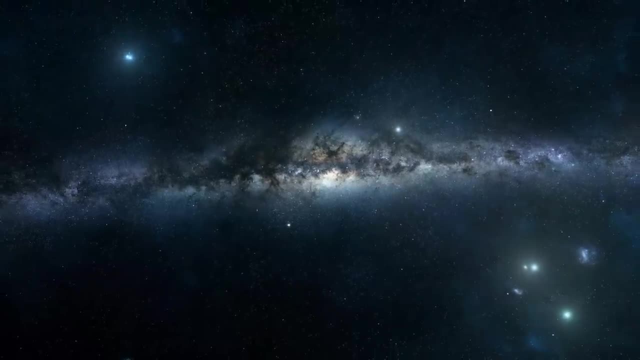 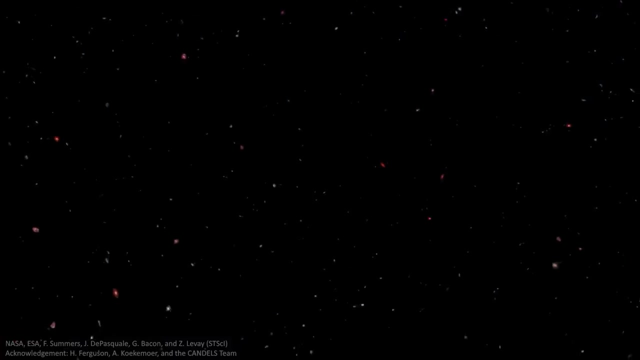 Because our universe is expanding, becoming less dense, and it has been for all its history. Scientists don't know if our universe is infinite or not, but if it is, then it always has been So. rather than starting as a single point, it would have also begun infinitely large. And rather than grow over time, it would simply have become less dense. Our observable universe, the only part of the universe we could ever see or interact with, or could ever see and interact with us, is limited by the speed of light and 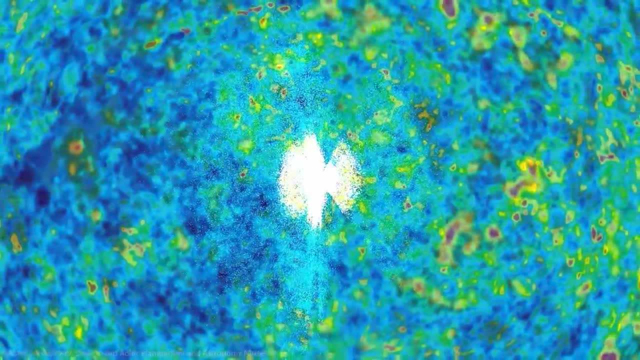 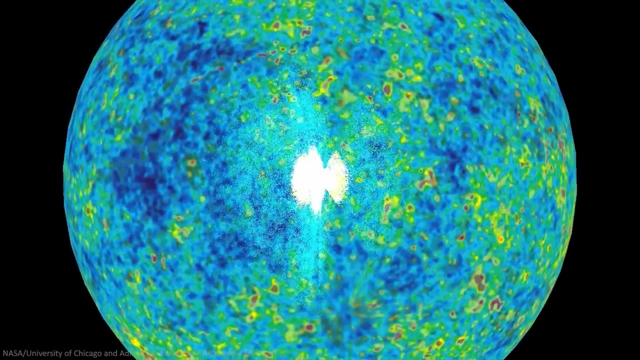 the distance it has been able to travel since the universe's birth 13.8 billion years ago. But as we travel back in time, the observable part of the universe shrinks and becomes more compact, Until, eventually, we get to a time when everything within it was only a single Planck unit of 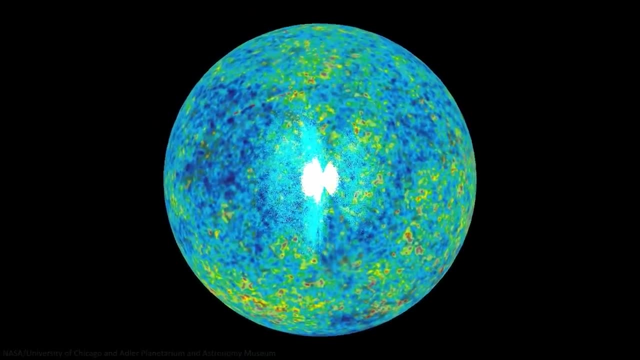 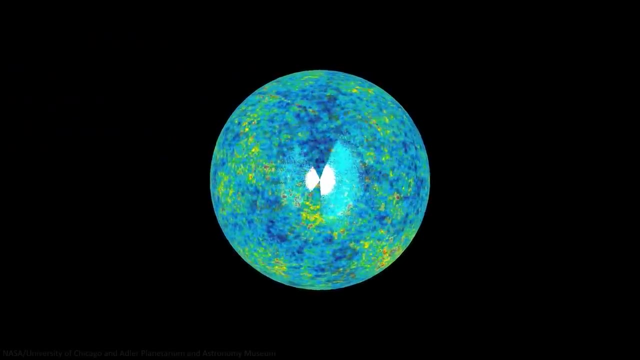 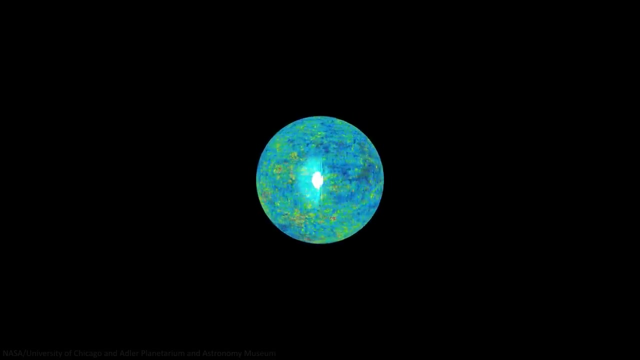 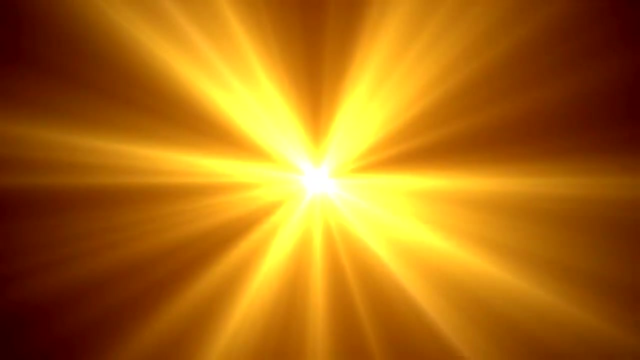 time old, A single Planck length in diameter, and with all of our observable universe compacted into such a tiny space, the temperature of the whole cosmos sat squarely at Planck temperatures. It may come as little surprise to learn that this moment, 100 million trillion trillion- 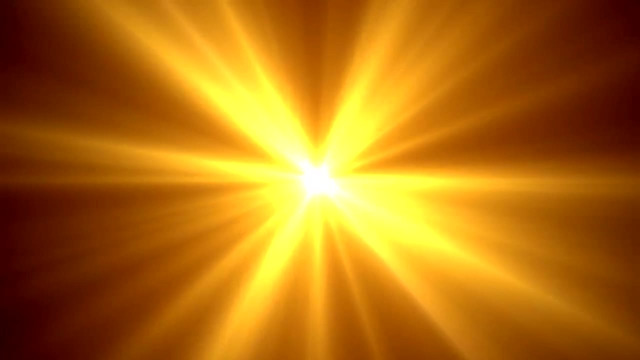 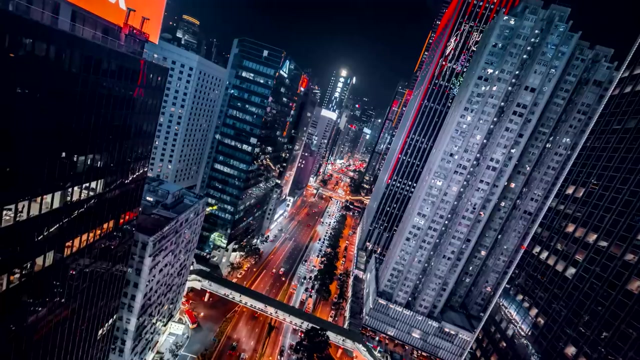 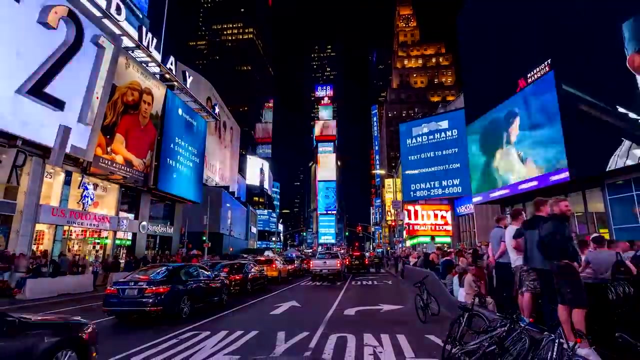 trillionths of a second after the beginning of time and space is therefore known as the Planck error, And it is a very strange time. In the cosmos today, everything we experience is governed by certain immutable laws of nature, which are ultimately controlled by the interaction of four major forces. 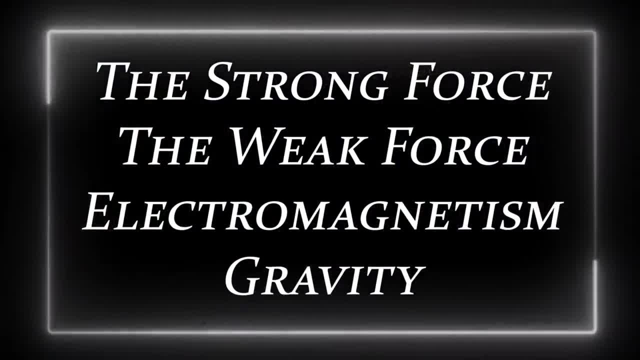 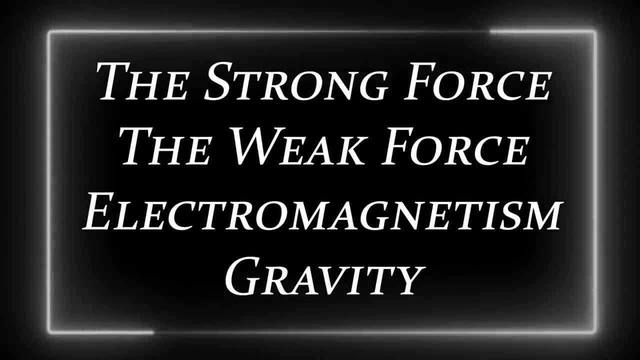 The strong force holding atoms together. the weak force governing certain types of radioactivity. the electromagnetic force distributing energy over great distances and gravity, As Max Planck predicted at the end of the 19th century. the strong, weak and electromagnetic. 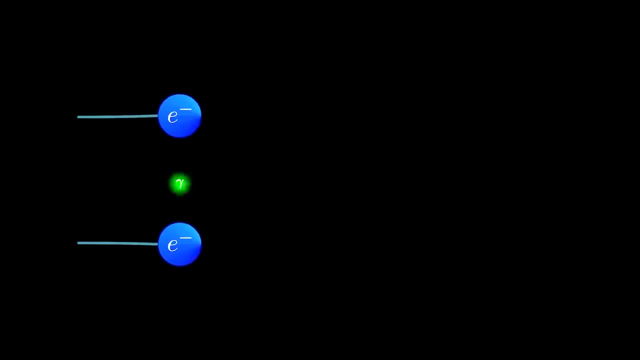 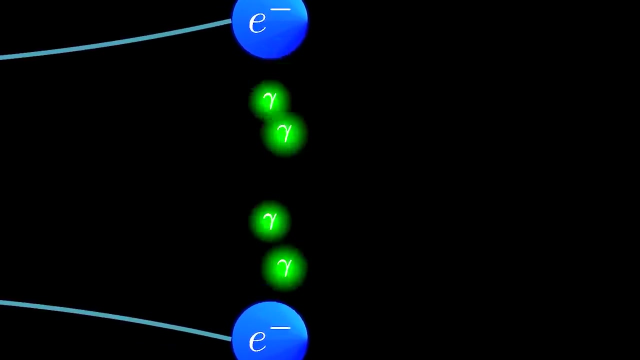 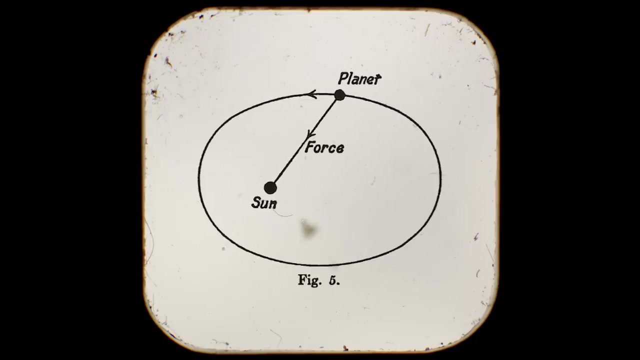 forces can be quantized, represented and thought of as tiny, individual parcels of interaction similar to particles of matter. These so-called messenger particles are known respectively as gluons, W and Z, bosons and photons, But gravity is different. 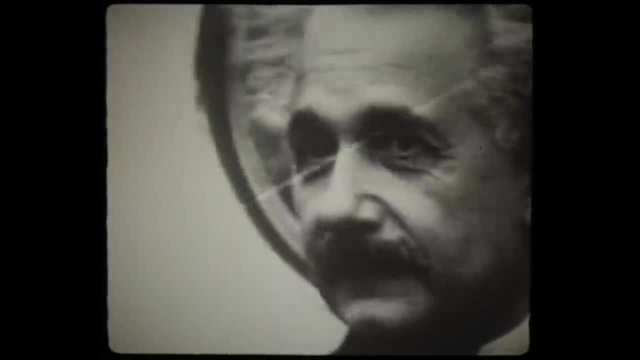 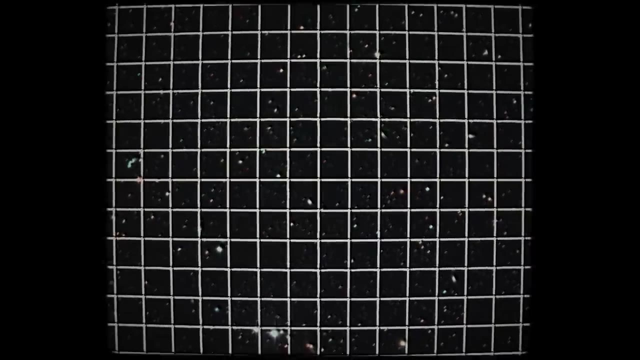 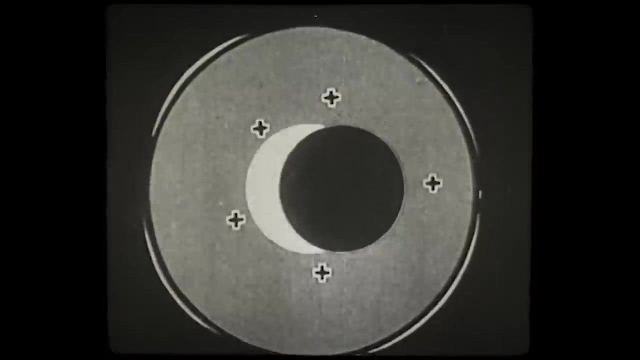 With his general theory of relativity, Albert Einstein was responsible for overthrowing the classical mechanical definition of gravity. He conceptualized it as the curvature of spacetime, a warping in the very fabric of reality. Through various large-scale experiments, general relativity has been verified time and time. 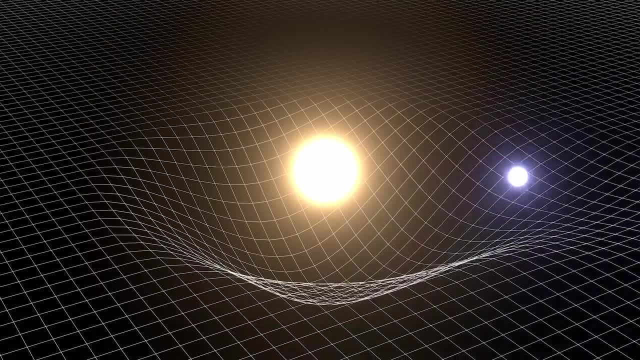 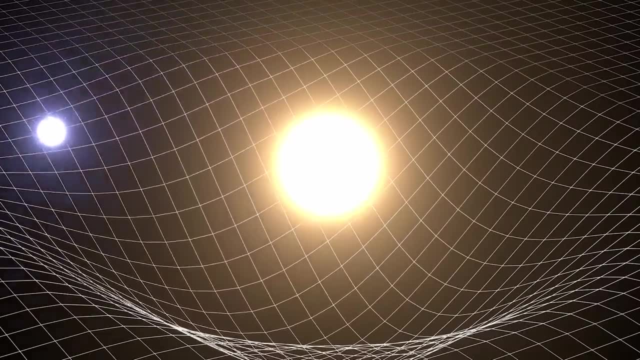 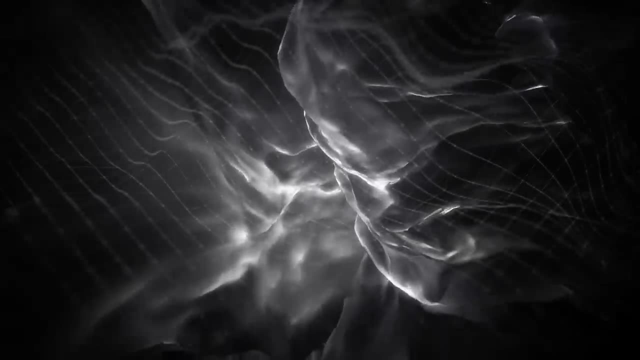 again, and the gravity-induced curvature of spacetime is now recognized as a property inherent to the universe, which affects all matter and energy within it. Therefore, during the Planck error, long before any of the conventional laws of nature held sway, it was gravity that was the first. 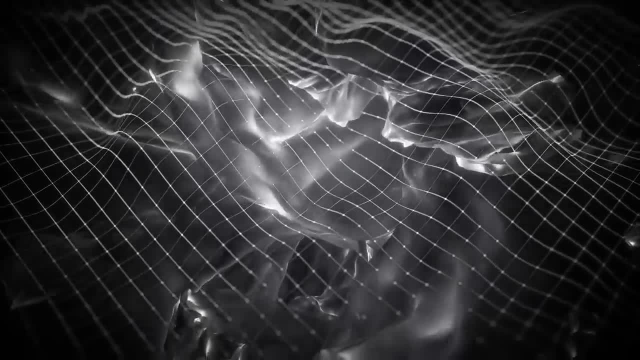 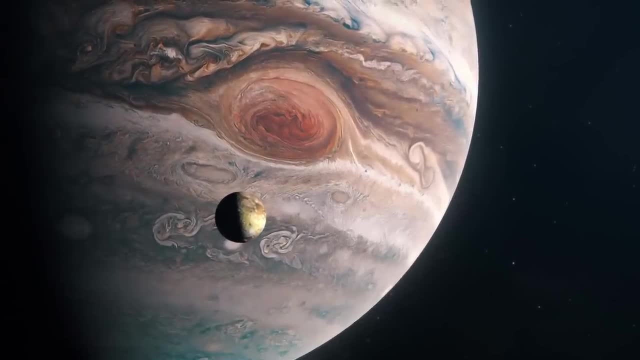 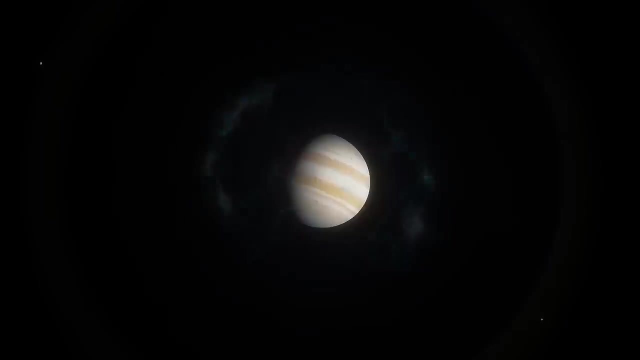 But there is a problem. Everything we know about the workings of gravity today is based on Einstein's successful theory, But that theory is only really tested and verified on larger scales. During the Planck error, however, our entire observable universe was condensed into an 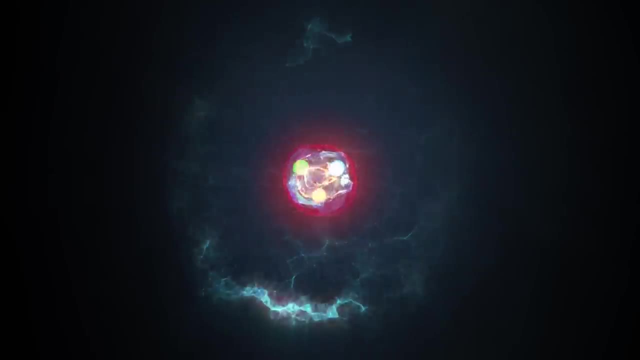 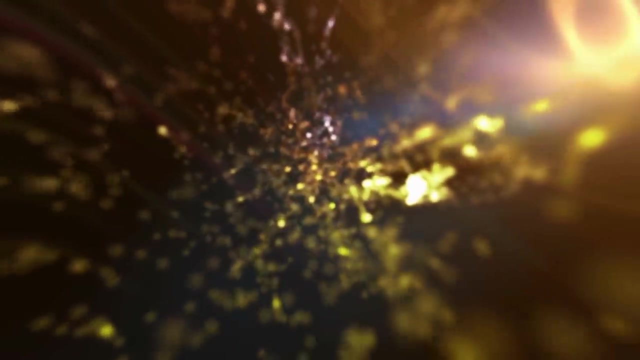 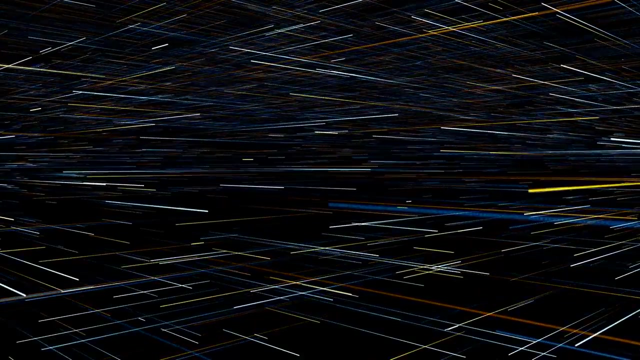 area many trillion times smaller than a proton, and so general relativity doesn't really help. Instead, the dynamics of the extremely tiny are governed by quantum mechanics At scales small enough that we can consider the individual subatomic particles of matter or the quantized messenger particles of force and energy- an entirely different set of rules. 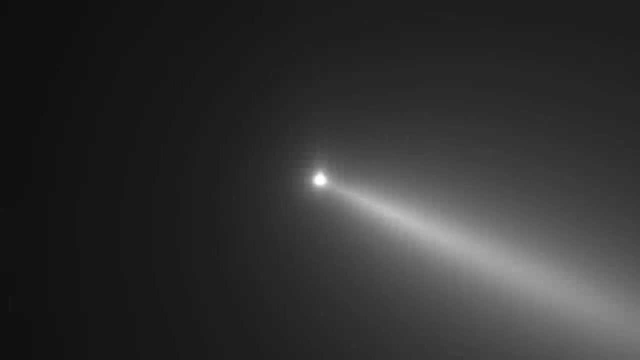 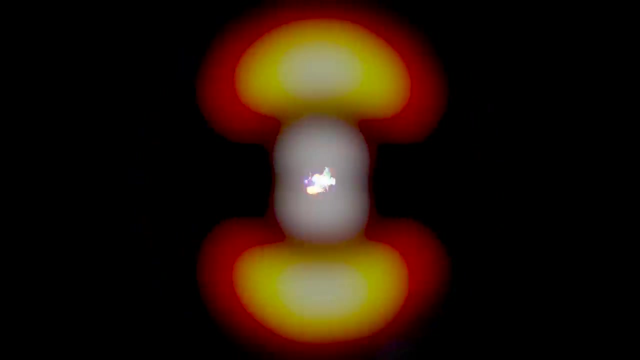 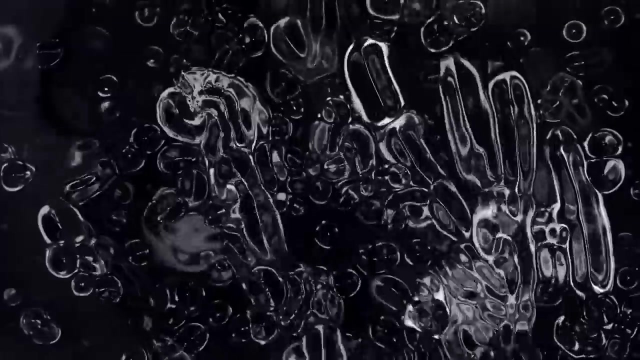 holds sway, where nothing is ever where you expect it to be and the very act of observing changes the outcome. Instead of dealing in absolutes, quantum physicists, consider probabilities, and nothing ever stays the same for long. Fortunately for us, this lawless quantum world only reigns on nanoscopic scales and 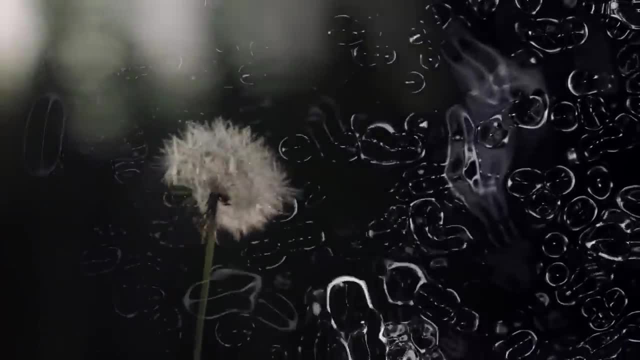 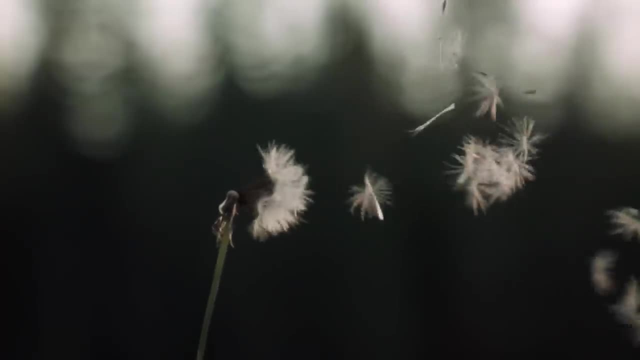 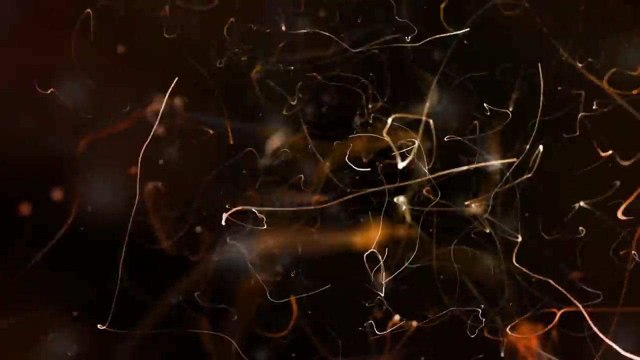 by the time we reach magnitudes that we're more familiar with, the probabilistic weirdness averages out, But during the universally nanoscopic Planck error, there is no escaping… the quantum. And herein lies the problem for understanding how things actually worked in that moment. 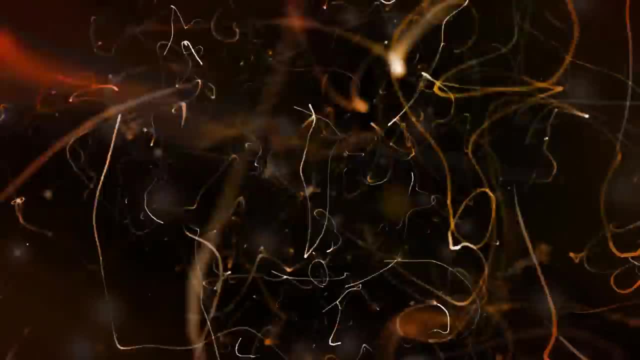 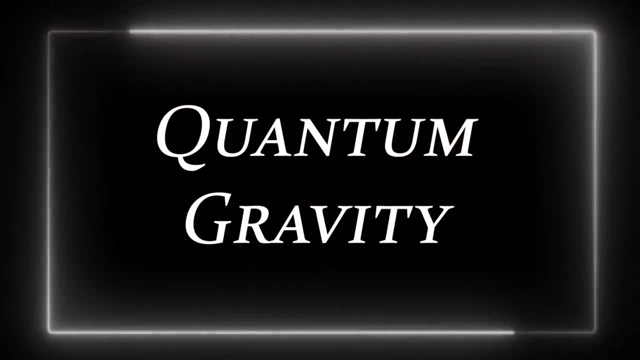 General relativity and quantum mechanics are fundamentally different than they are in the real world. They are fundamentally incompatible with one another. So researchers are still searching for a solution, a so-called quantum gravity, that is able to reconcile two of the most important theories in modern physics and properly describe how. 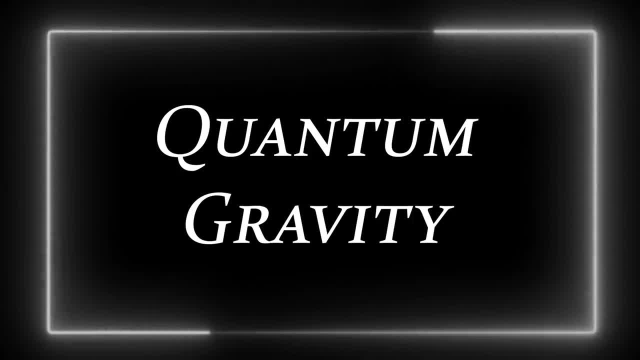 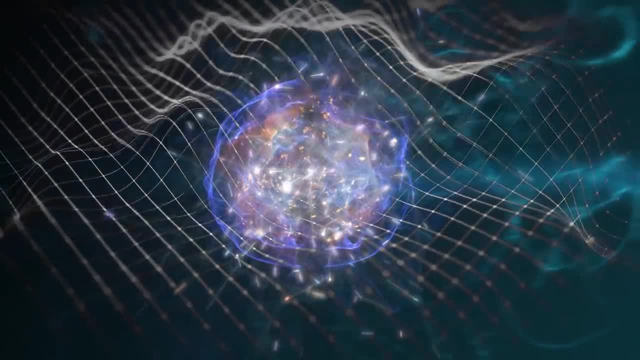 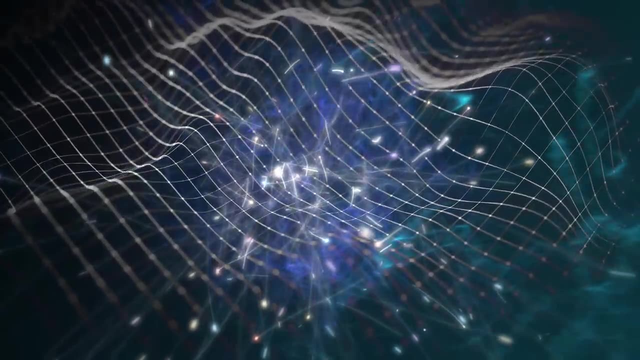 the Planck error universe behaved. Unfortunately, it is a question that cannot reasonably be tackled by experimental means. Considering the vast energies needed to produce and study the other force, messenger particles inside collider facilities And the elevated plane that gravity occupies in defining all of space-time, it would take 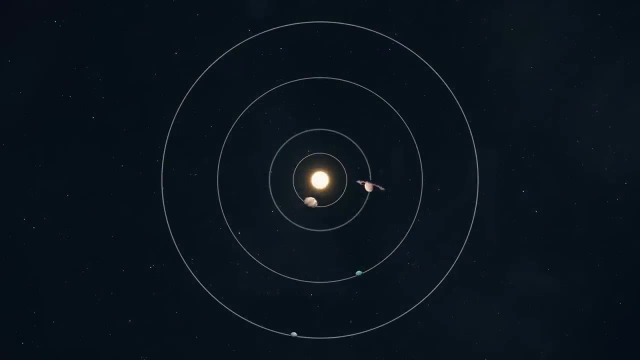 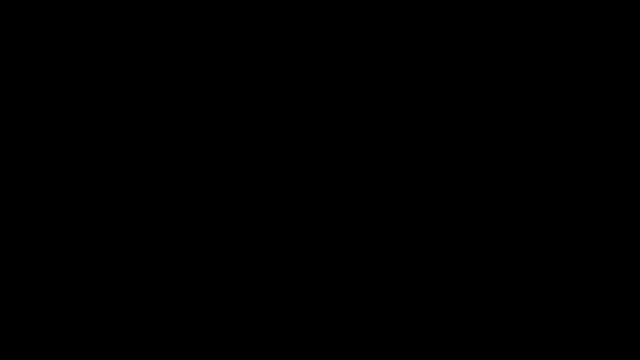 a particle accelerator roughly the diameter of our entire solar system to generate enough power to truly probe gravity during the extremes of the Planck error. But this doesn't stand in the way of theoretical speculation and extrapolation. One idea suggests that, like the other fundamental forces of nature, gravity is also a form of. 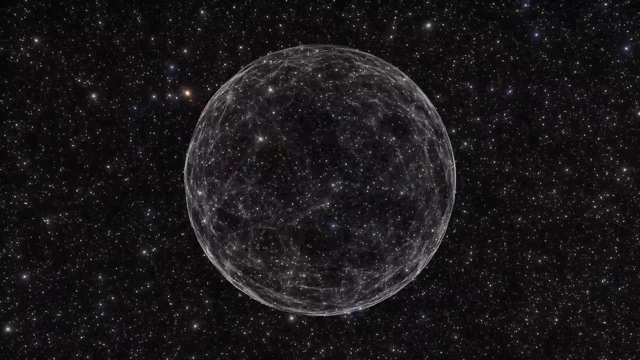 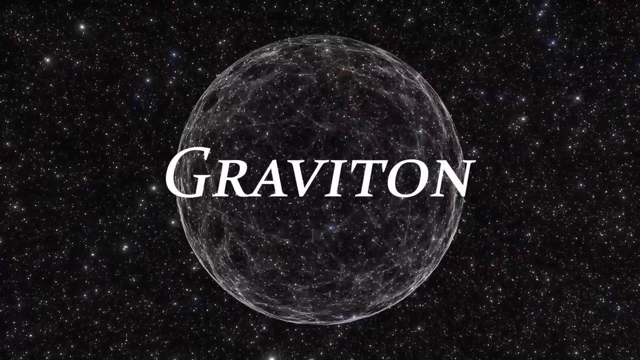 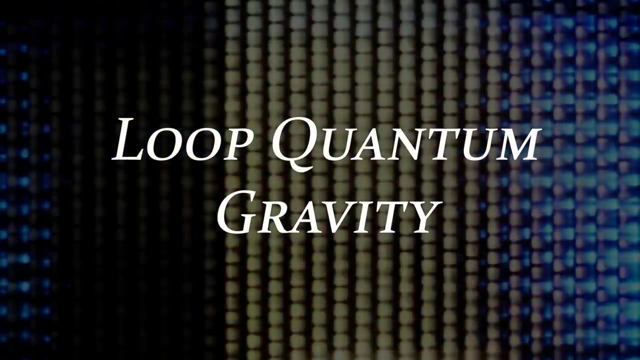 gravity that is communicated by a messenger, particle, a quantum unit of gravity that has come to be known as a graviton. But gravity as a force is so much weaker than the others that its meagre messenger would be practically impossible to detect. Another theory, known as loop quantum gravity is very different. 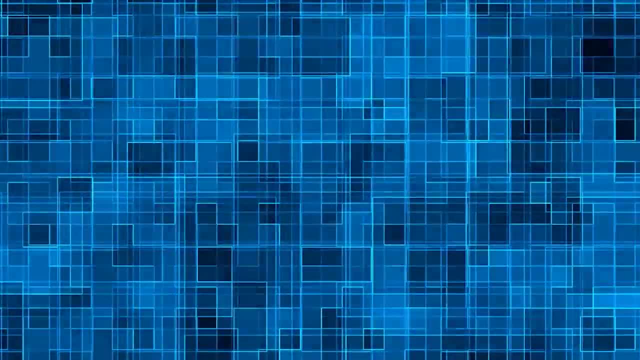 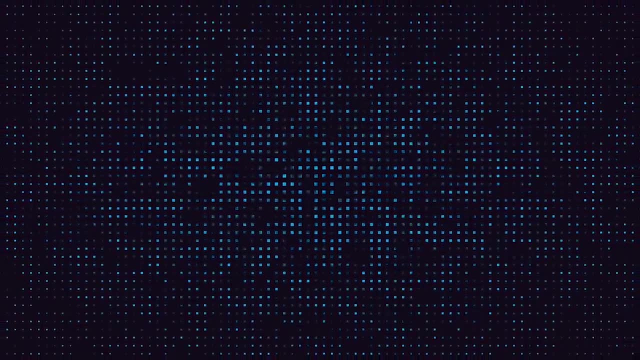 In this, physicists imagine the smooth and ever-changing geometry of space-time, to be ultimately pixelated on the very smallest scales, And, by rewriting Einstein's equations of general relativity, they can now be used to calculate the length of the gravity of a particle. 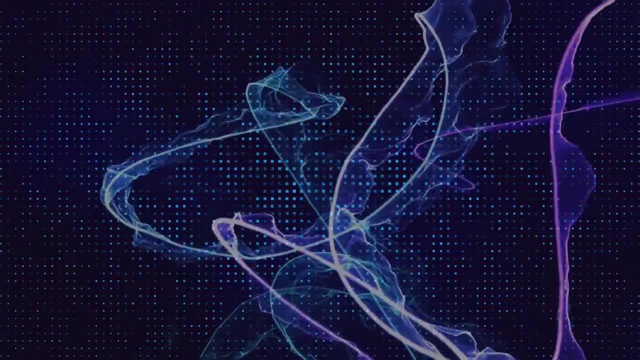 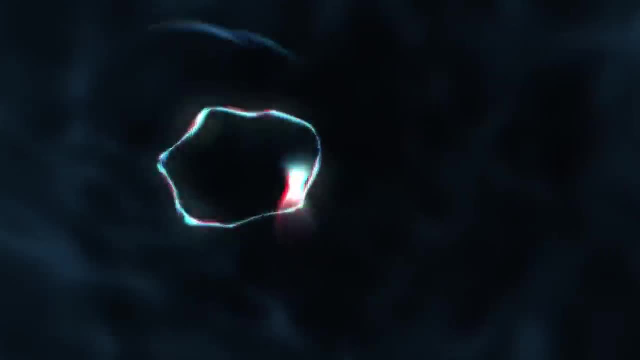 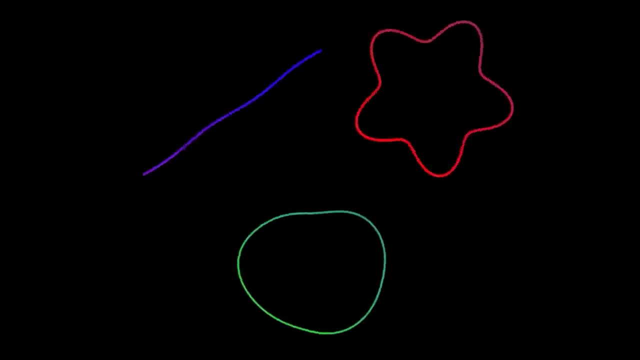 By using equations of general relativity in terms of lines or loops instead of points, the calculations for gravity on a quantum scale become much more manageable, And perhaps the leading possible quantum gravity solution continues to rumble away in the background of theoretical physics. String theory imagines the point-like particles of traditional physics as one-dimensional. 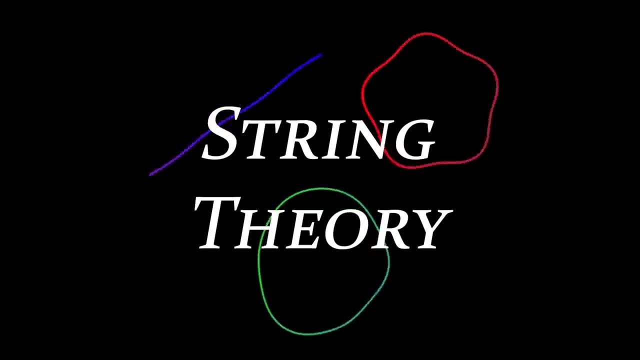 vibrating strings, And it is the vibrational state of the strings that defines what a particle does, What a particle is, As well as the elusive force of gravity. And yet, in order to make the mathematics of string theory work, it becomes necessary. 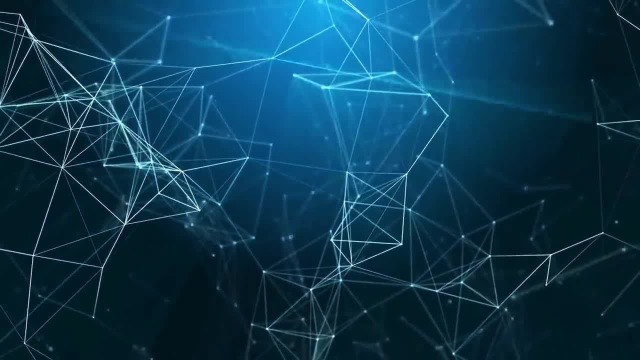 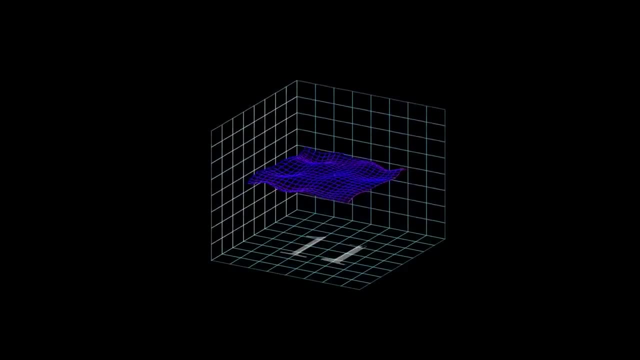 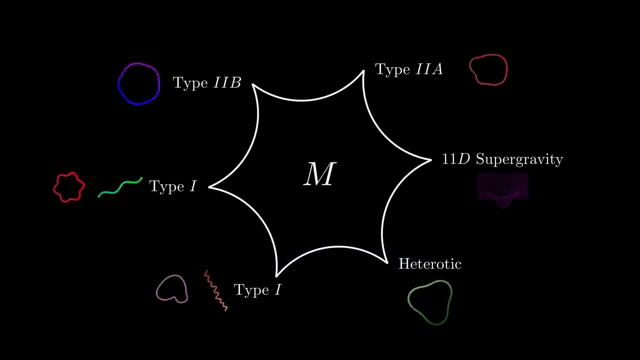 to involve no fewer than ten or eleven dimensions, Many of which would be folded in on themselves or partitioned into two or five-dimensional structures known as brains, The fundamental objects of an even more elusive overarching theory with the simple moniker M, And that's it. 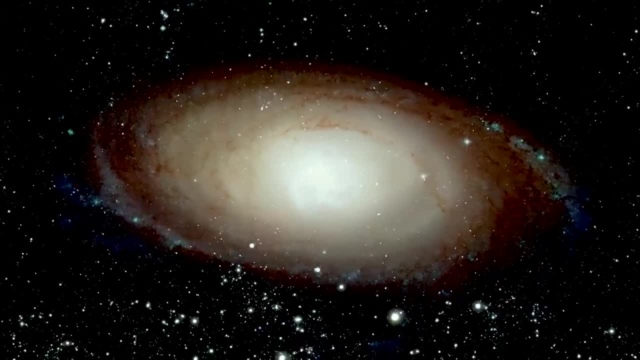 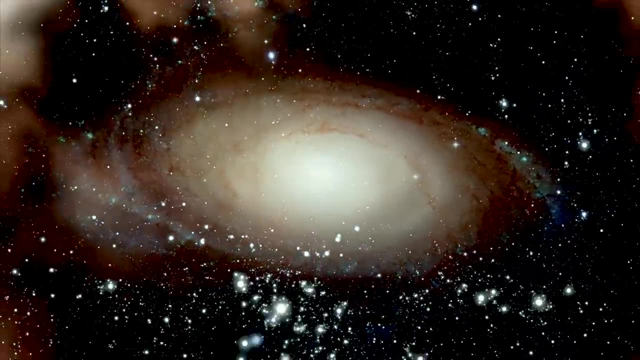 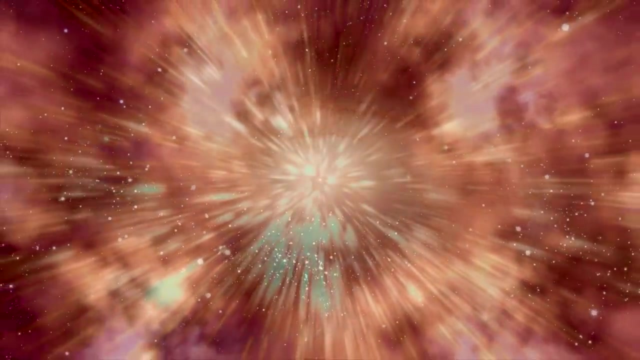 Thanks for watching. And so each of these hypotheses for how quantum gravity may actually work is more mind-bending than the last, rooted in the abstractions of mathematics and almost impossible to visualise. And yet that is what we are trying to do when we cast our minds back to imagine the 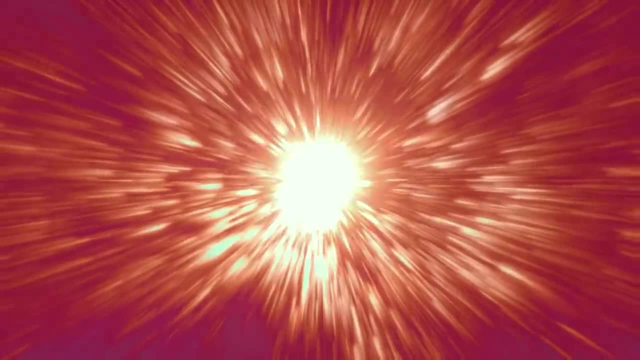 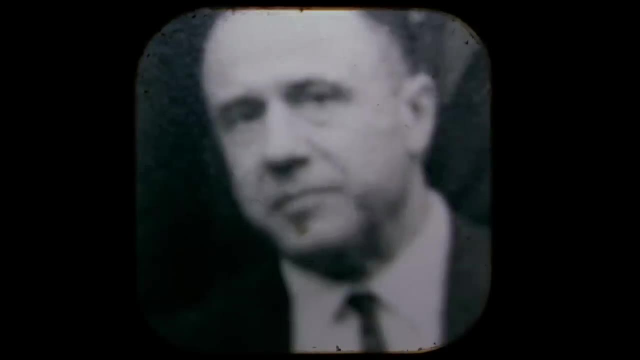 first fraction of a second of our universe during the Planck era. Ironically, it was in the 1950s when the science of quantum mechanics was first introduced. It was then that quantum mechanics was first introduced. It was then that quantum mechanics was still in its infancy. that American theoretical physicist 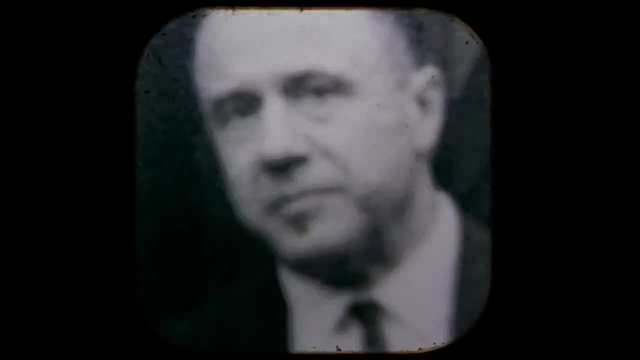 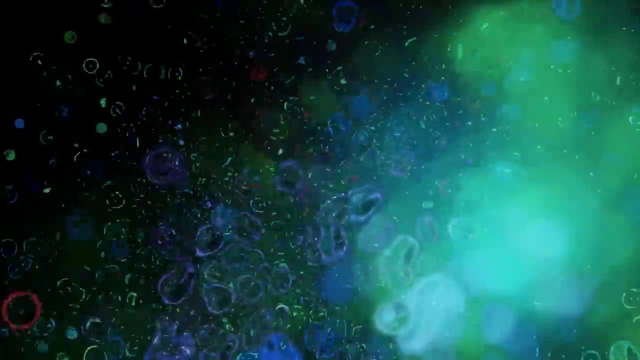 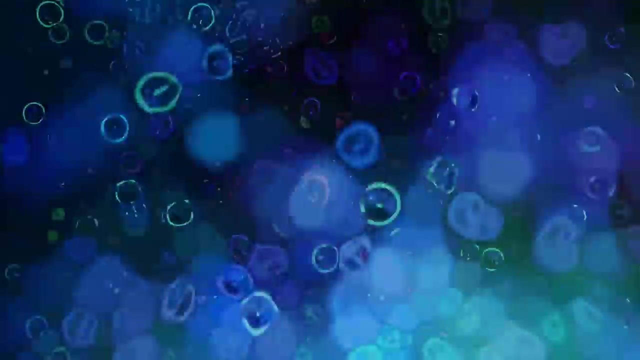 The quantum foam is a form of interaction between the two. Heisenberg's uncertainty principle seriously compromises our ability to define length, time or energy at any one point within the Planck-sized universe, And so the continuous and coherent spacetime that we are familiar with today is replaced. 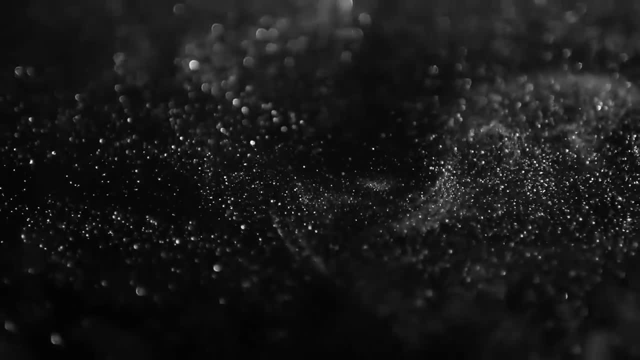 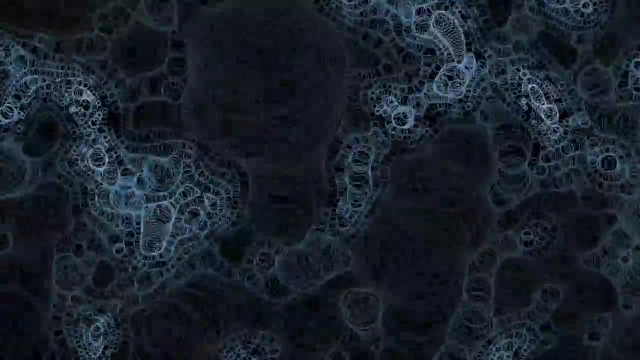 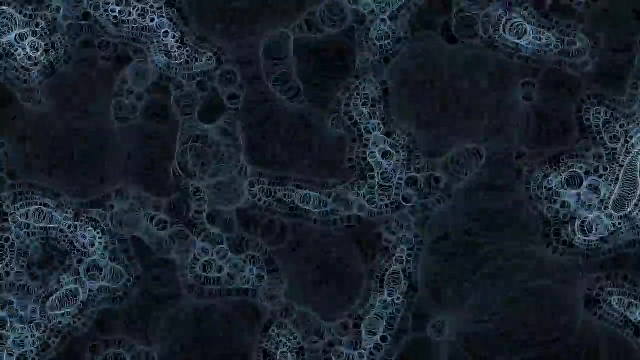 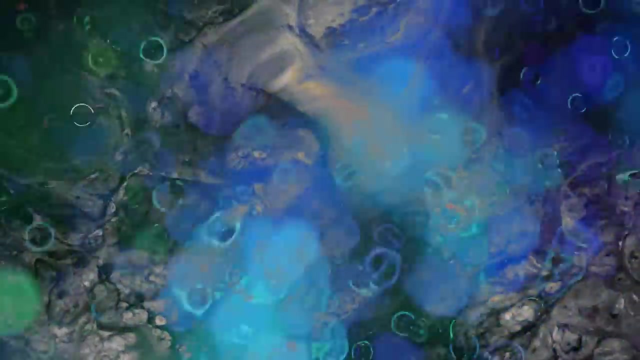 by an inherently unpredictable and varying foam-like texture that shifts and changes randomly, Quantum, micro-black holes and wormholes spring spontaneously into existence and then disappear without a trace. Without a trace, without any apparent cause and effect, In this highly energetic, super-compact and miniaturized cosmos, for the briefest of moments. 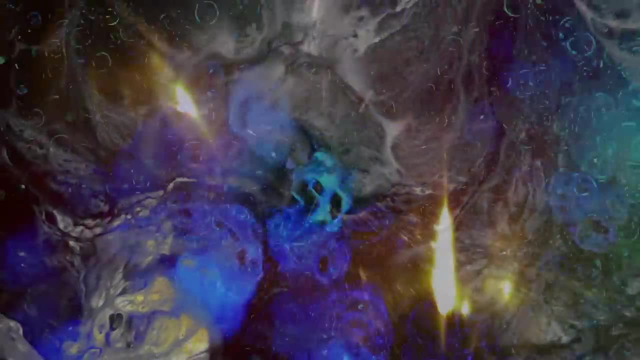 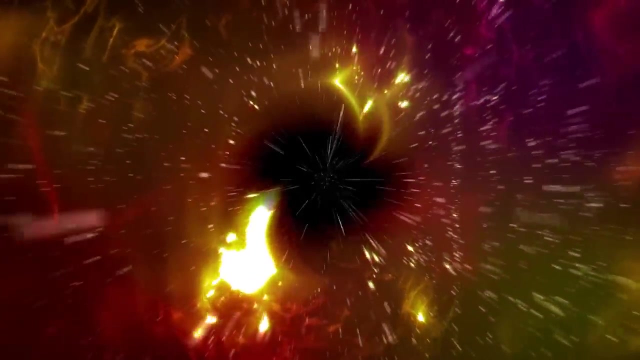 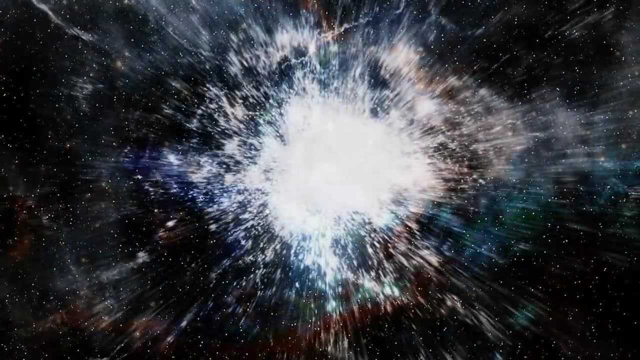 anything goes, But after only one hundred million, trillion, trillion trillionths of a second, the widespread unpredictability of the Planck era comes to an end. as the minuscule growth and cooling of the universe heralds a new epoch, The universe won't look ordinary. 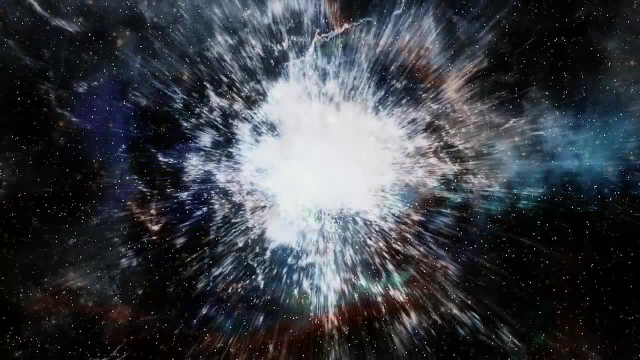 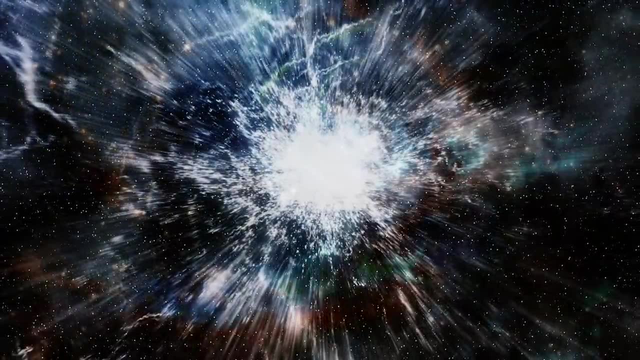 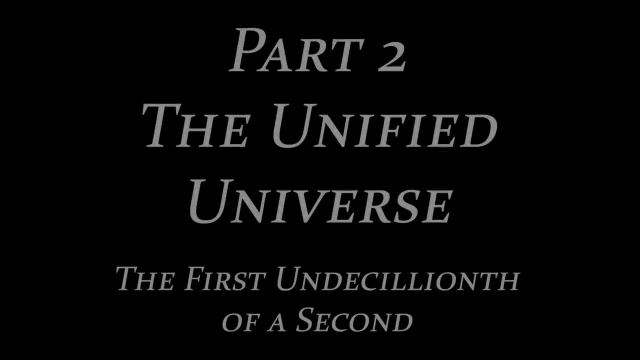 It won't look or behave anything like it does today for a while, But from here on out, our current theories do at least stand a chance of describing just what is going on. Everything in our universe is controlled and defined by the four fundamental forces of. 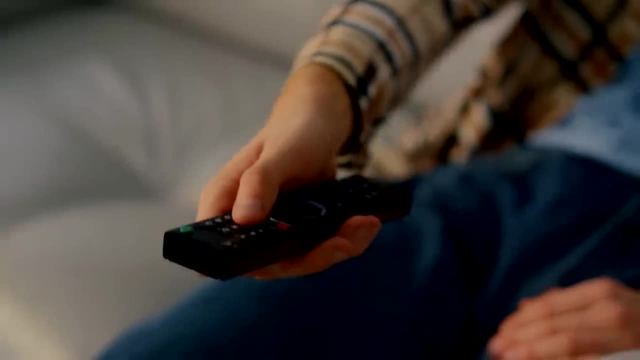 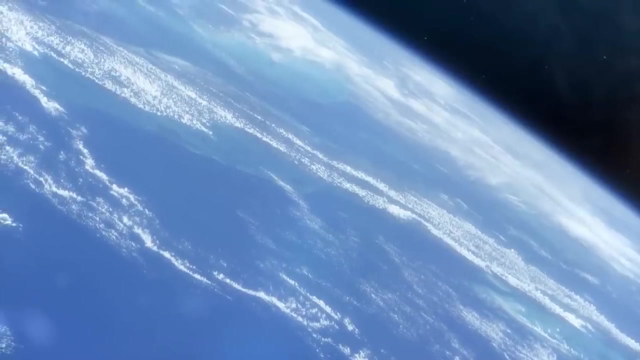 nature. Imagine turning on your television. Gravity keeps you pinned firmly to the seat of your chair, holds the Earth's atmosphere close to the surface and holds the Earth in orbit around our nearest star, providing a habitable environment for your continued existence. 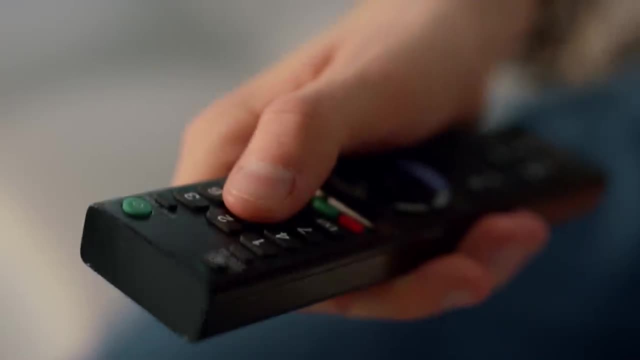 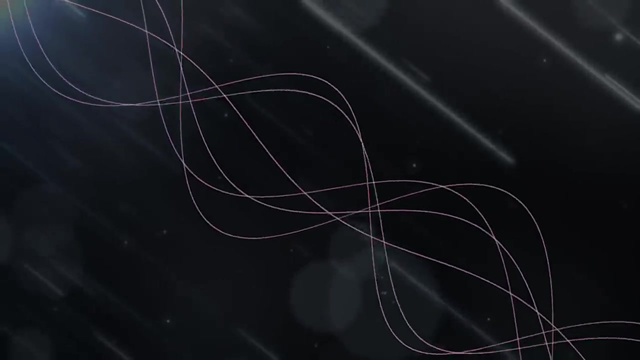 Yet, despite this, gravity is relatively weak and you can overcome it with the muscles of a single arm. to lift the remote In response to your button press. invisible infrared light, electromagnetic radiation beams across the living room from the front of the remote. 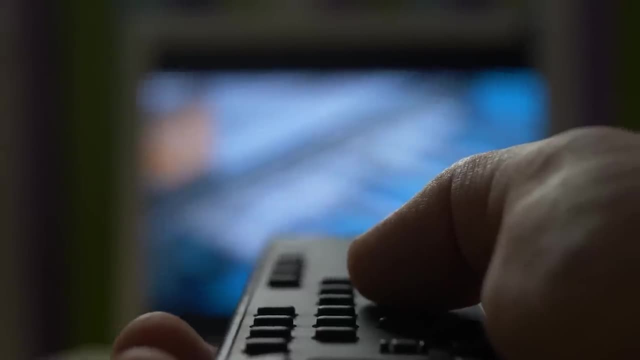 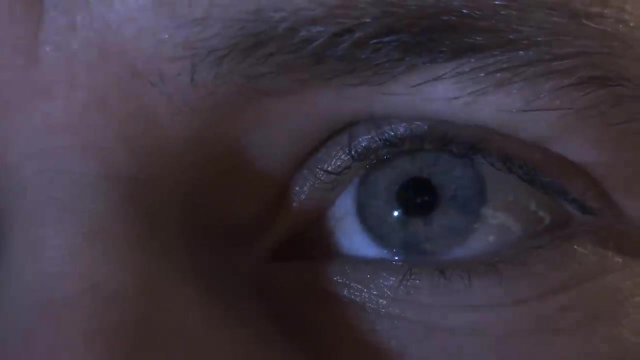 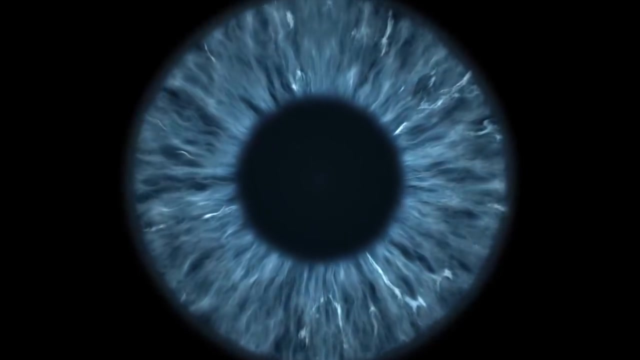 The picture comes to life in front of you through millions of tiny pixels emitting visible light, another form of electromagnetic radiation which travels back across the room and into your eyes. Your eyeballs themselves are marvels of evolutionary innovation, but they ultimately rely on the properties and behaviors of the atoms within Electrons and nuclei held together by the 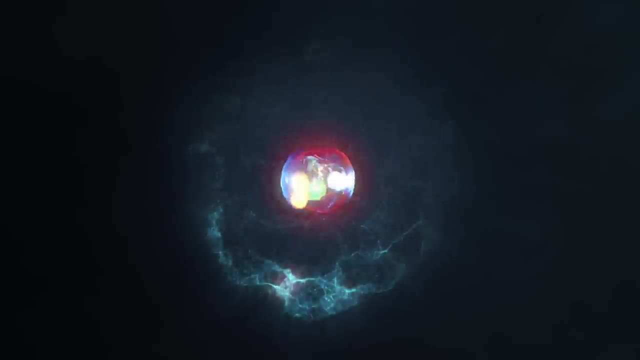 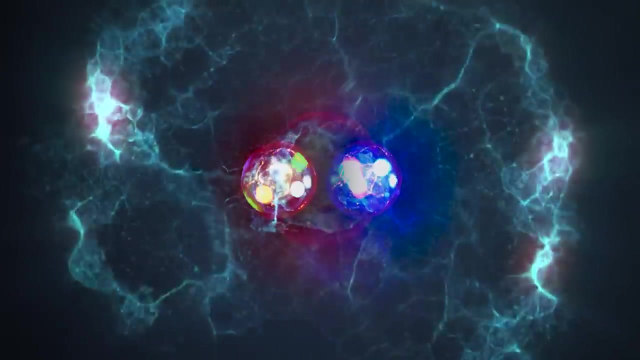 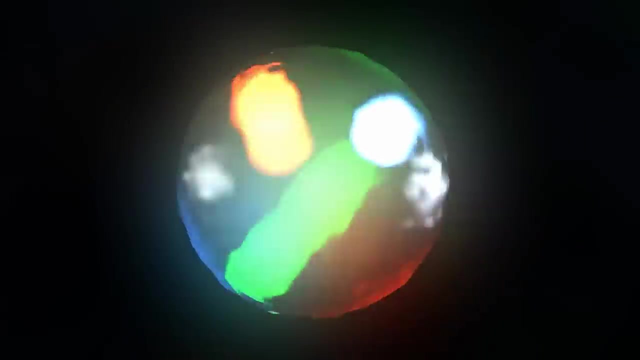 electromagnetic force. The atomic nuclei themselves are held together by the strong nuclear force: protons and neutrons forced together in the center of the atom. Not only that, these protons and neutrons are really a combination of three smaller subatomic particles called quarks, which are also bonded by the same pull. 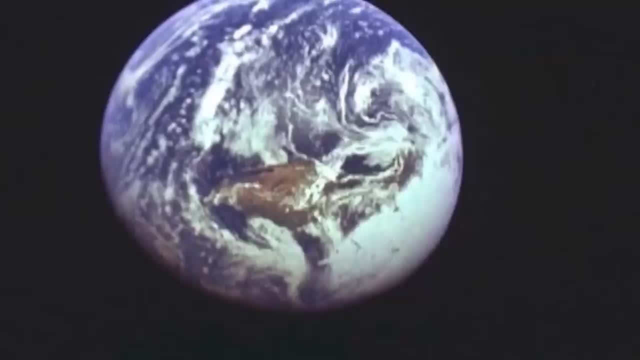 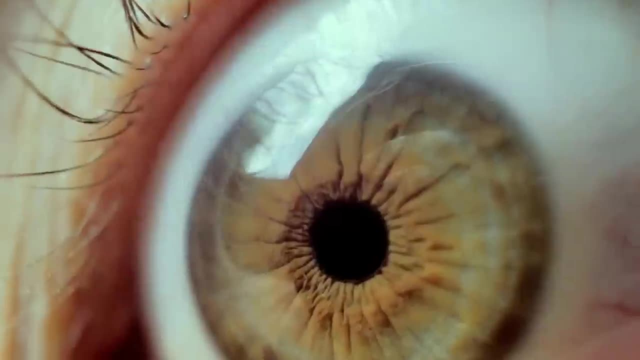 Every atom in your body, in the television, in existence itself, relies upon this force. As your eyes focus and you engage with the pictures moving on the screen in front of you, each of the nerves inside your brain fire at up to 200%. 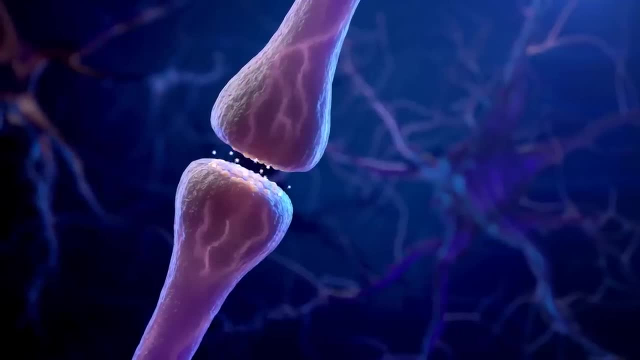 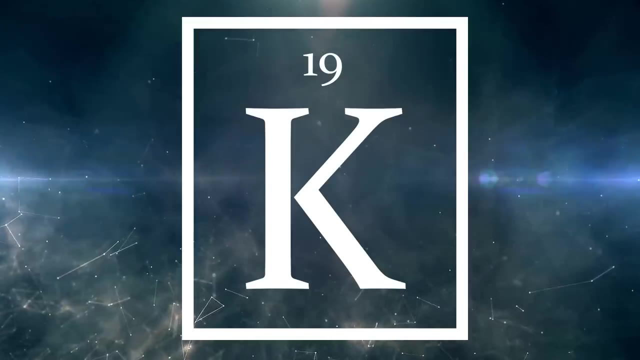 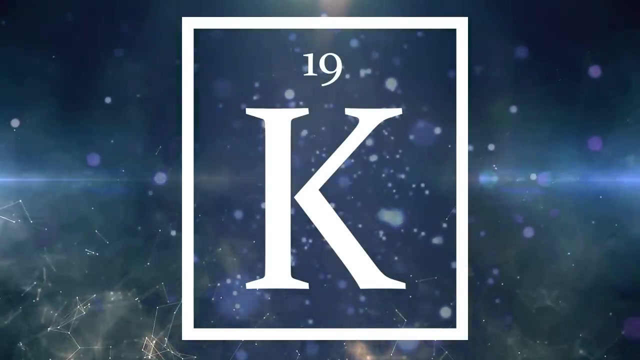 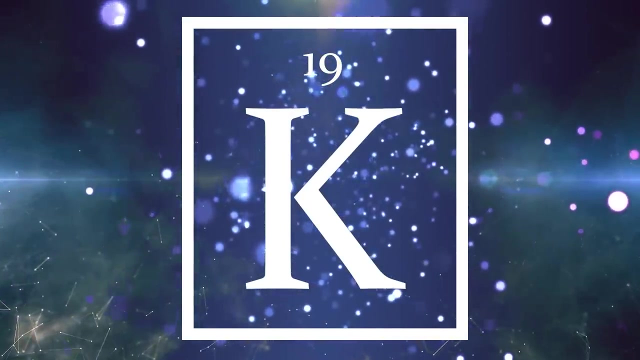 All of that coordinated electrical potential relies on a proper balance of potassium in the body. Like the other elements, potassium is held together by the strong nuclear force. but there is something else at play as well, because potassium is very slightly radioactive And around 5,000 potassium atoms radioactively decay every second, A decay driven by the weak. 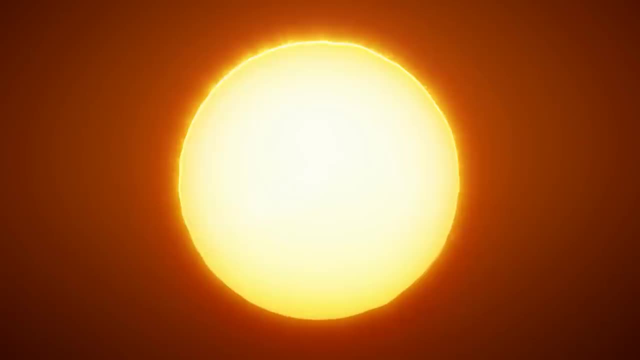 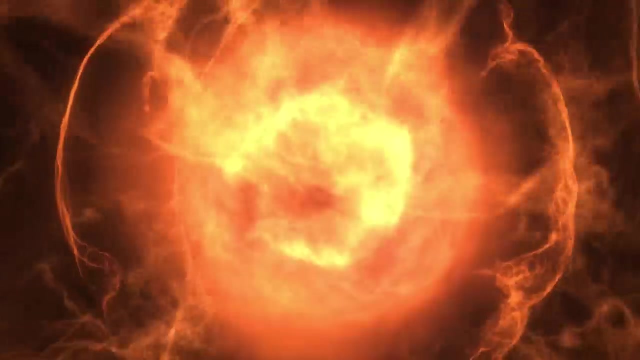 nuclear force, And so one could imagine the next generation of the nuclear force to be the same as the last. 150 million kilometres away, the core of our sun burns with the heat of a stellar furnace powered by the fusion of hydrogen into helium. This incredibly powerful reaction is responsible. 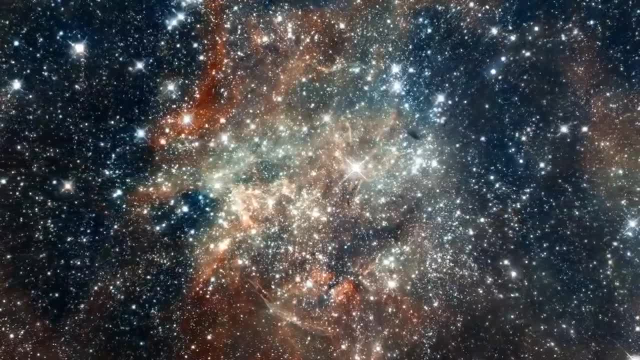 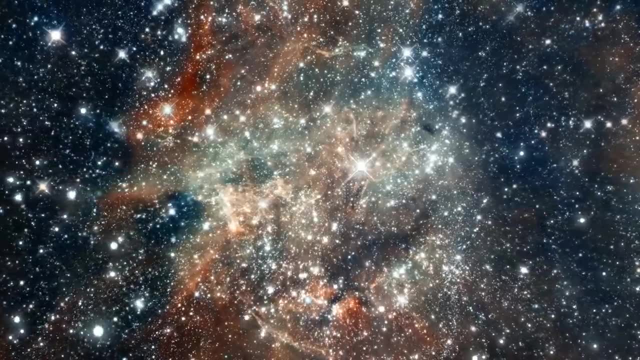 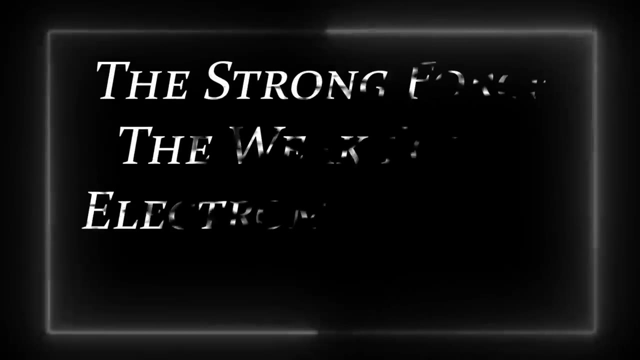 for the heat that keeps the earth habitable, and on a galactic scale, the very elements that make up the planet, the television and you. And all of this is also reliant on the weak nuclear force, Cosmos, Each of these four fundamental forces- gravity, electromagnetism, and the strong and weak 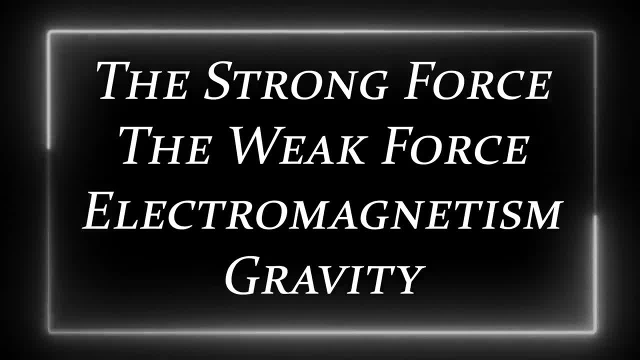 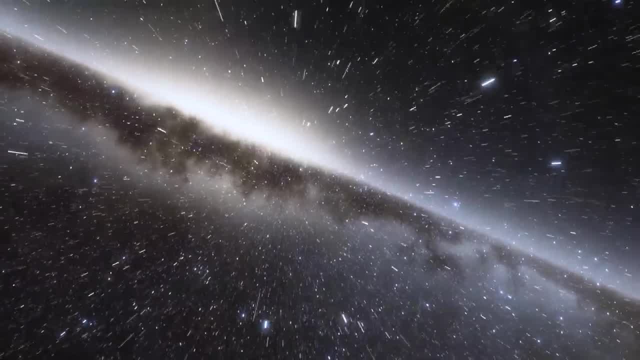 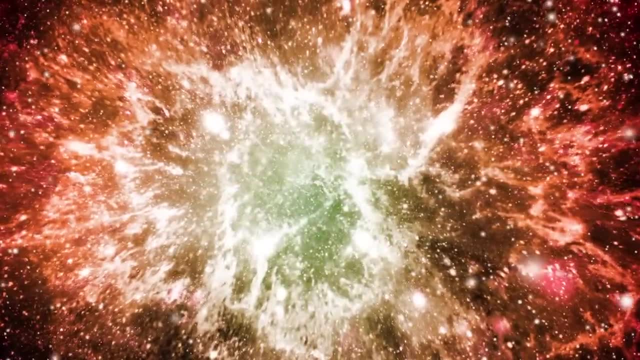 nuclear forces act together to shape our experience of the universe, and so it has been for the majority of our cosmos' multi-billion year history. But in the very first moments of time, conditions conspired to craft a very different set of rules. During the Grand Unification Epoch. 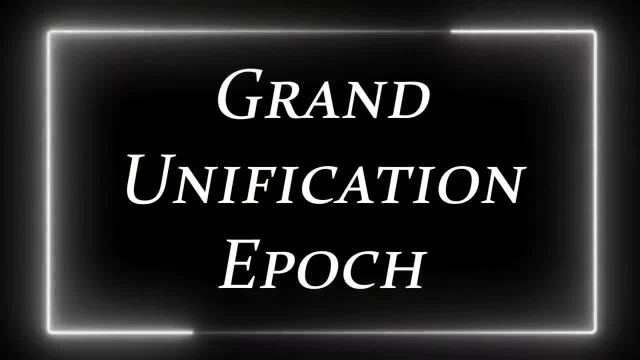 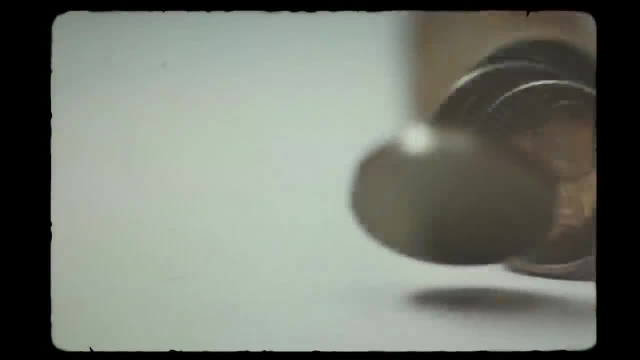 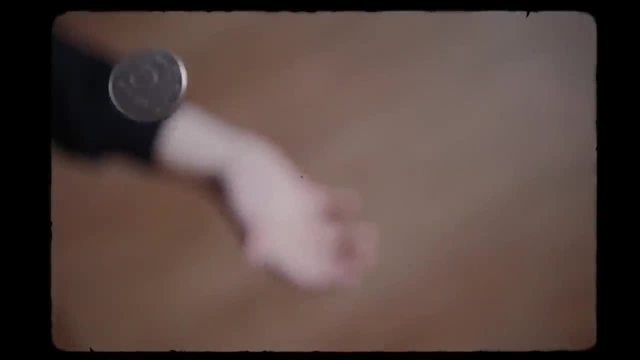 which followed the Planck Era, there were only two forces. But how could this be the case? The key to visualising this lies in a coin toss. Flip a coin to decide between two equally weighted choices: Heads for one team, tails for the other. 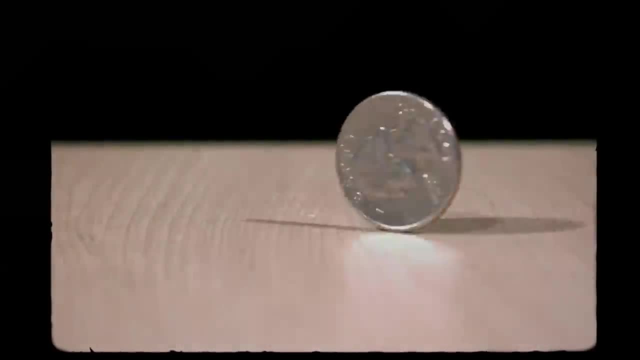 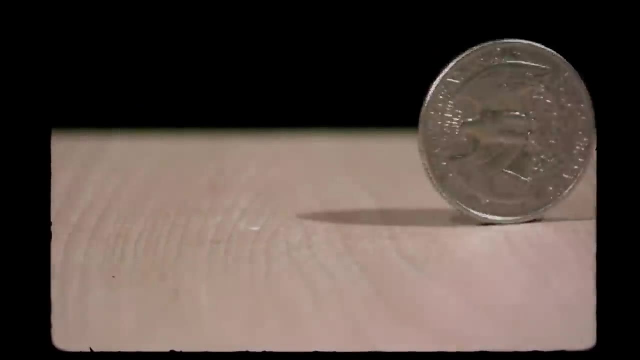 The decision is only reached when the coin settles after the flip, when the energy provided by the flexing of thumb and forefinger is completely spent and the disc comes to rest Before that point, when the coin is still imbued with energy. 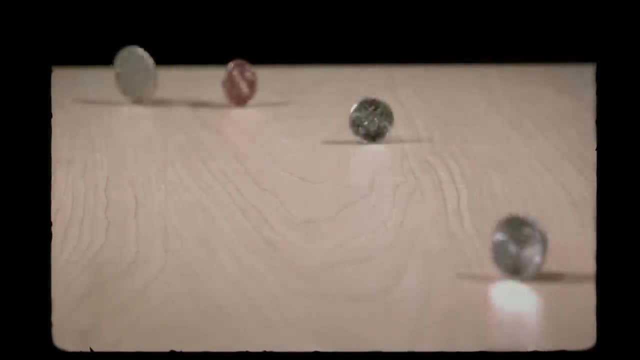 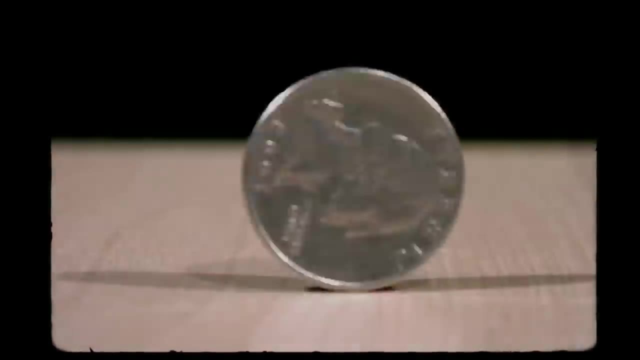 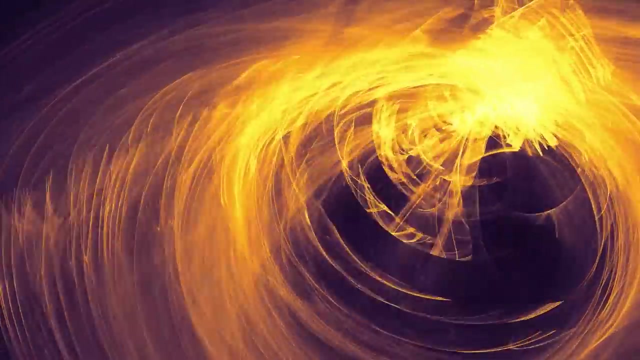 and it is spinning through the air or across the table. it is nigh on impossible to even distinguish the two faces, the two choices available to you. There is just a single spinning orb with characteristics all of its own, And this is what we encounter when we examine the behaviours of the fundamental forces. 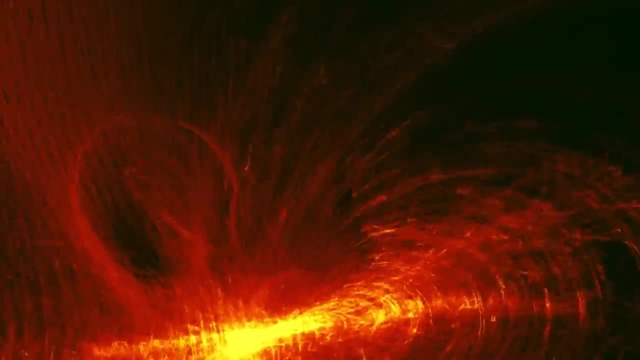 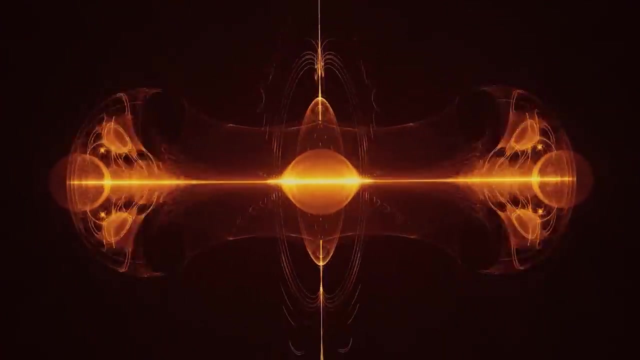 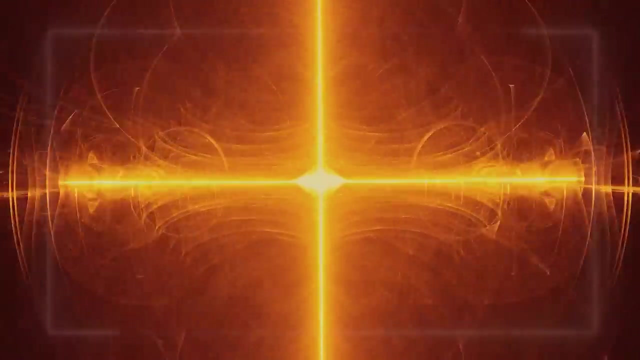 at higher energies. the energies that were present in the nascent universe Increase the temperature dramatically and the individual properties of the weak nuclear force and the electromagnetic force begin to weaken and blur into one another. We no longer see the distinct heads of electromagnetism. 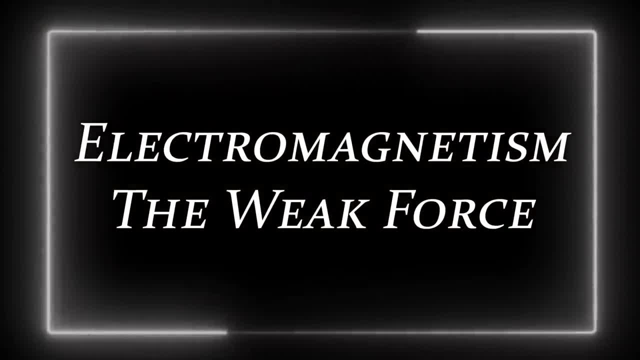 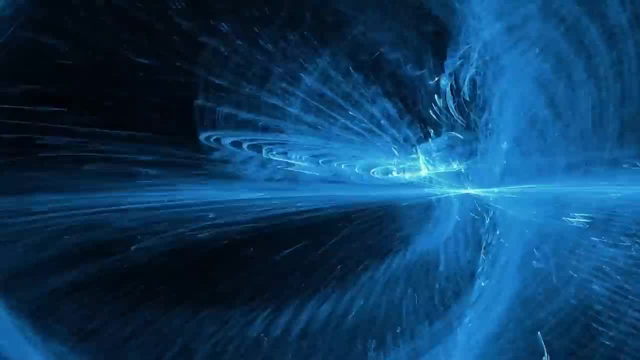 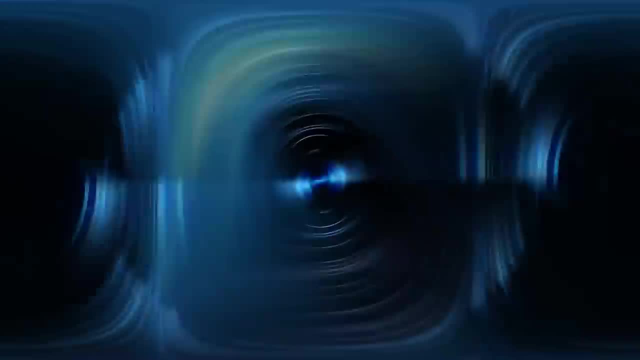 and the tails of the weak force, but rather the spinning faceless force of the two united, The so-called electro-weak force, Increase that energy even further and the spinning coin concept again applies to the strong force and the electro-weak. With high enough temperatures, these 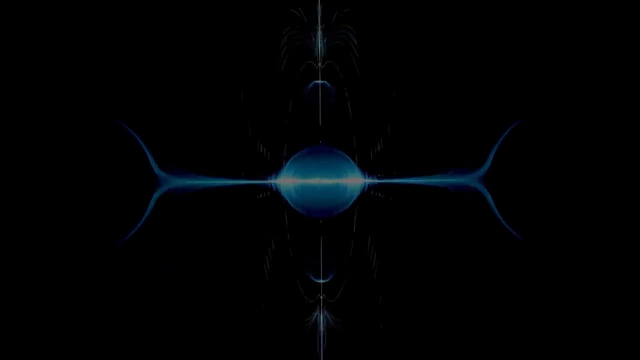 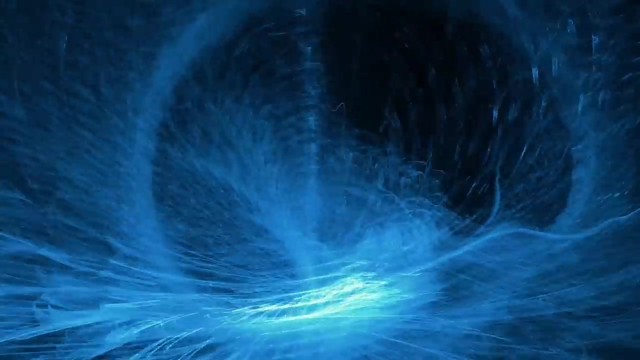 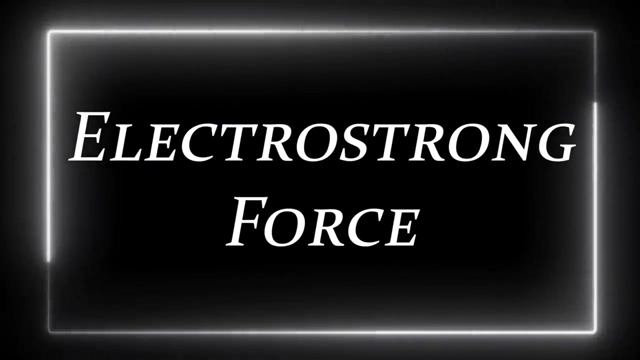 in turn blur into a single unified whole in a process known as grand unification. This ultimate unification of three of the major fundamental forces gives rise to what is known as the electro-strong force, though this tidy spinning coin theory of grand unification has 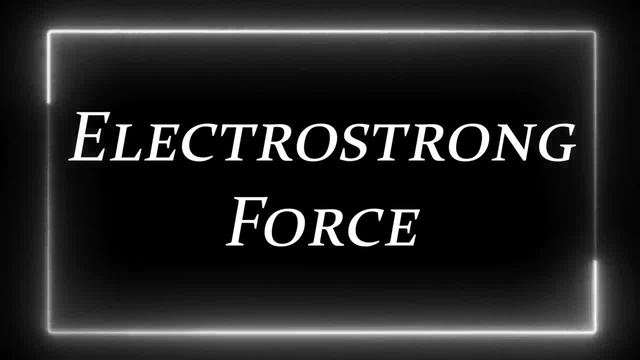 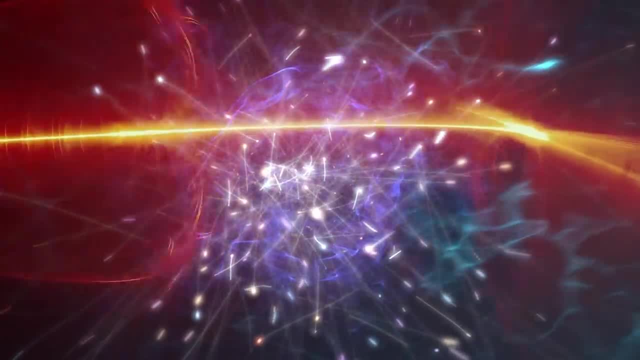 yet to be definitively proven experimentally. Even though the energetic collisions inside particle accelerators can point us towards the joining of electromagnetism and the weak force, it takes energies some million million times greater for the strong force to lose its identity in the 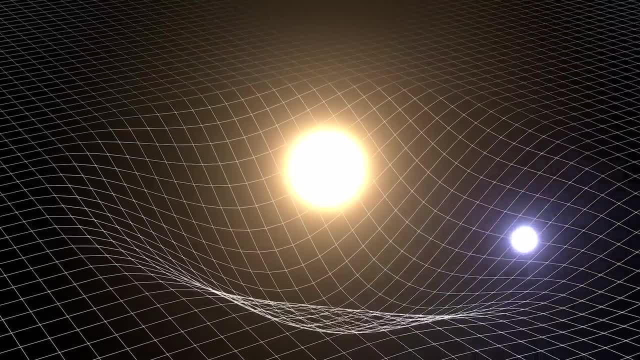 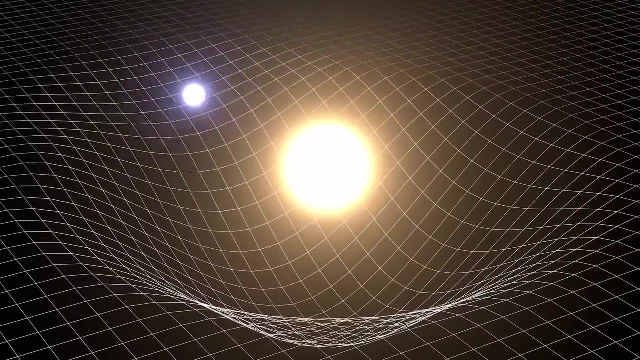 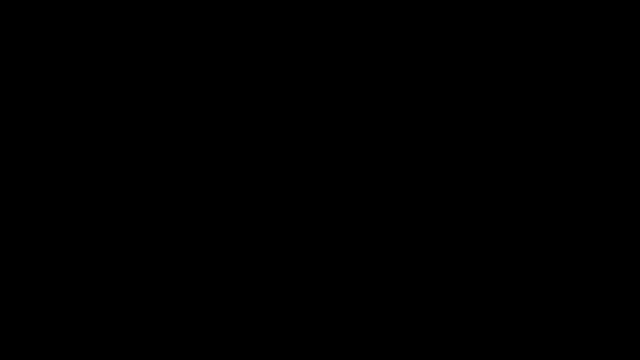 same way As for whether gravity, the fourth fundamental force, is ever accepted into the unified fold. that is a question for the mysterious and unpredictable Planck error and yet another problem for contending theories of quantum gravity. Still, the grand unification theory, as it is known, is a strong contender for. 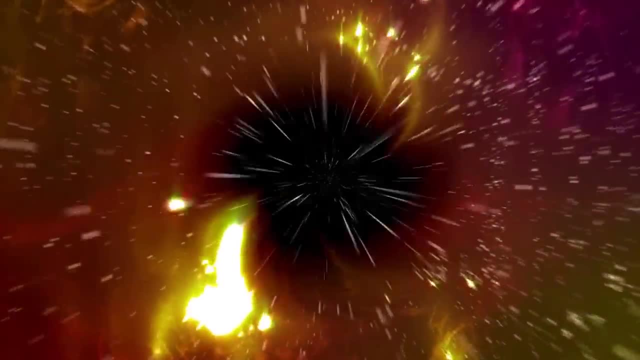 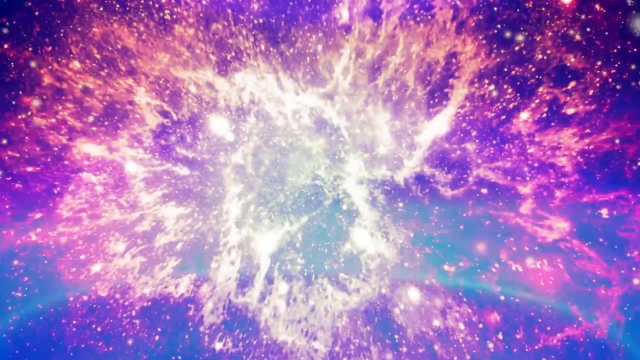 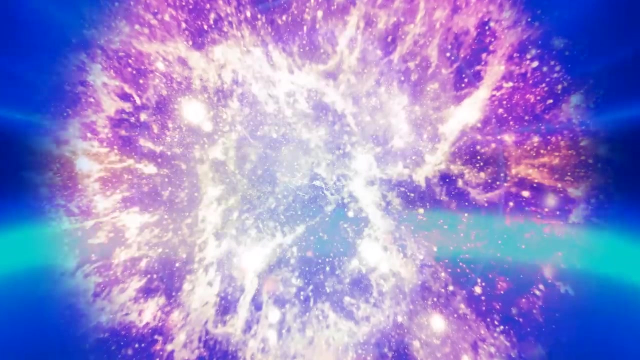 the unification of the universe and the universe itself. For a period of time some ten million times longer than the entire Planck error. the universe expanded and cooled, But it is testament to just how dense everything started out that even by the end of this time, 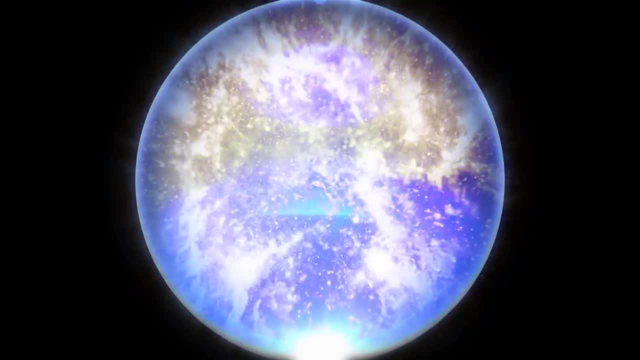 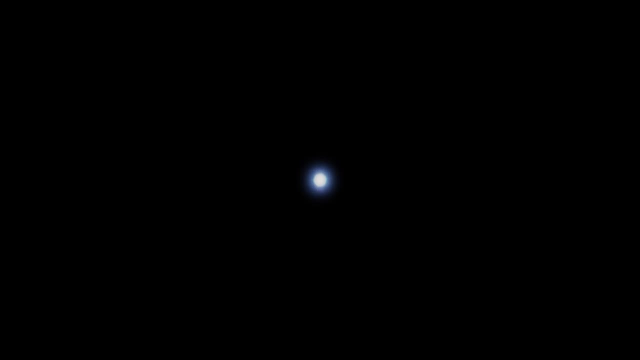 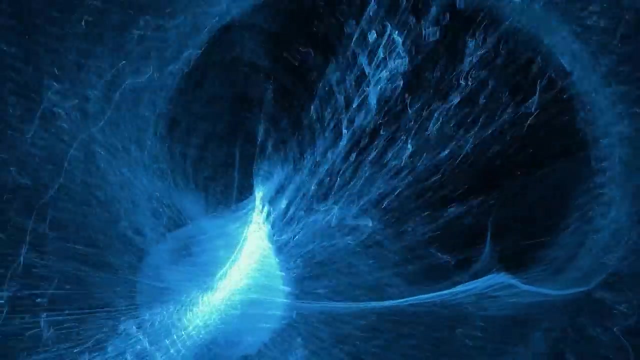 the entire observable cosmos was still smaller than a single quark. With the latent energy of that cosmos compressed into such a tiny space, the temperature reached one hundred thousand trillion trillion kelvin, some trillion times higher than the large hadron collider has ever managed. These were the conditions for the grand unification epoch ruled by the chimeric. 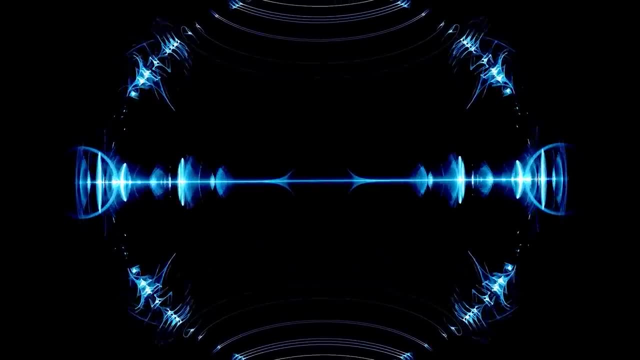 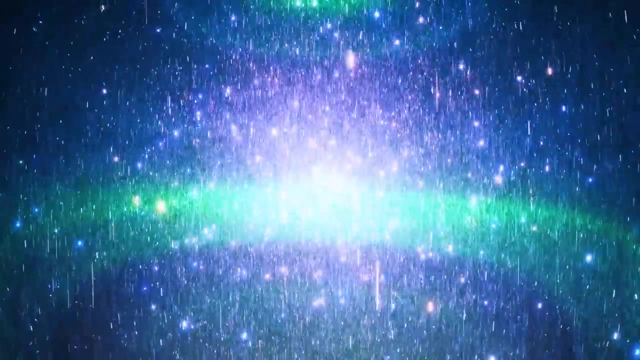 electrostrong force and the bizarre interactions that it brought about. The minuscule cosmos is filled with particles undergoing an extreme identity crisis. Photons transform spontaneously into matter-antimatter pairs, creating quarks. The universe is filled with particles undergoing an extreme identity crisis. Photons transform spontaneously into matter-antimatter pairs, creating quarks. 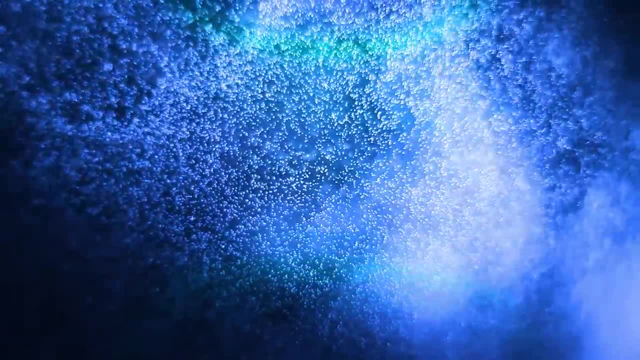 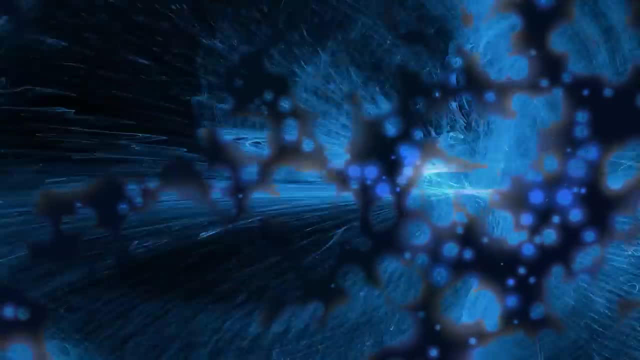 But these nascent particles are desperately short-lived, decaying rapidly back into photons scarcely as soon as they have formed Electrostrong messenger bosons only serve to complicate the picture, helping quarks to transform into leptons, leptons into quarks. 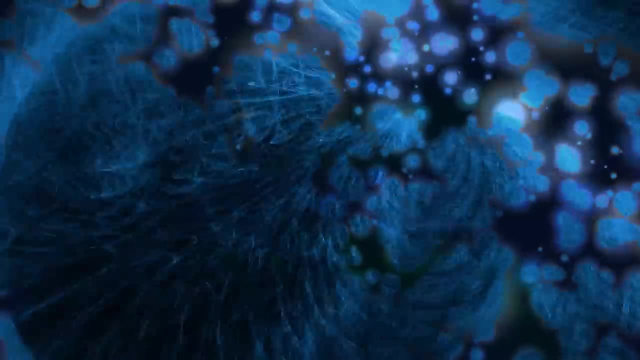 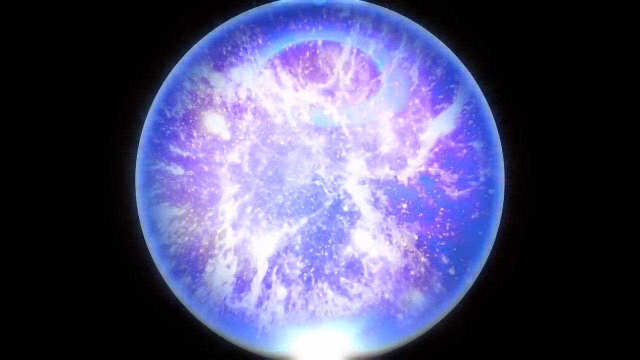 matter into antimatter and vice versa. Under the chaotic rule of grand unification, it is a free-for-all of energy and matter Of particles both virtual and real, Of particles both virtual and real, Of particles both virtual and real. 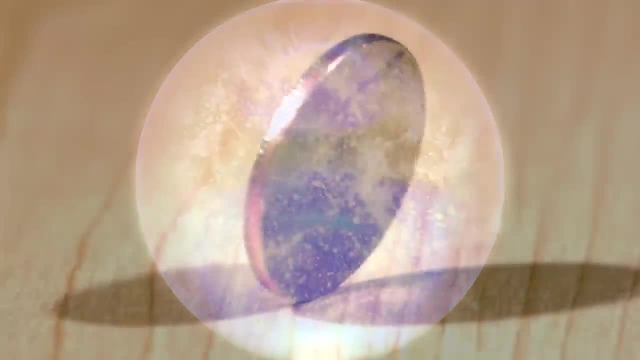 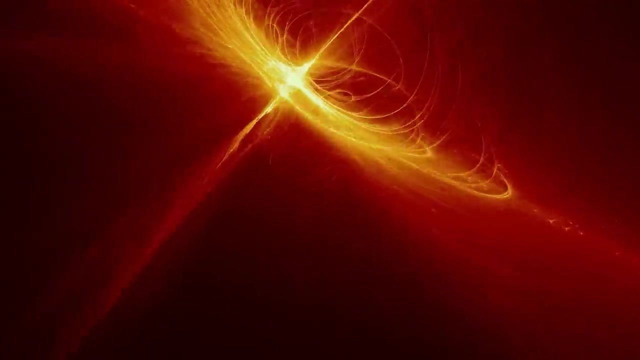 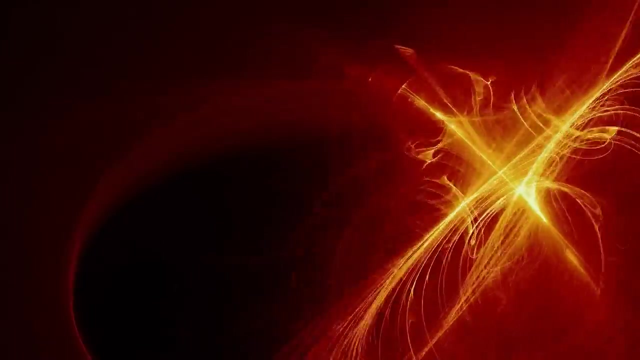 Until a trillion, trillion trillionth of a second after it began, the penny drops. Temperatures drop to a mere thousand trillion trillion degrees, rendering it cool enough for the strong force to break free, for two forces to become three and everything to change once again. 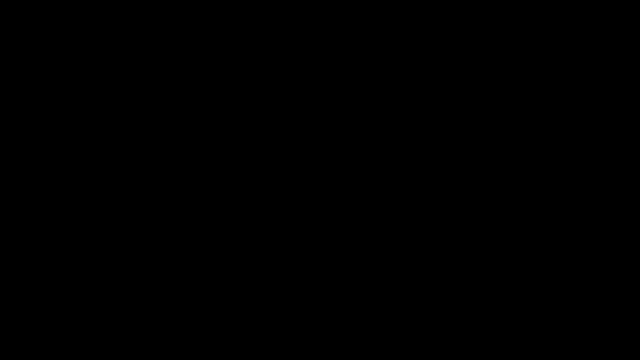 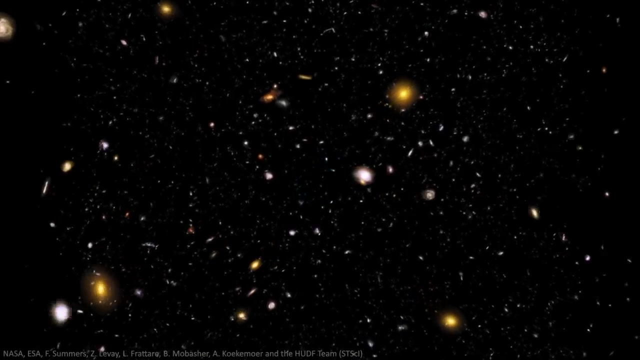 And yet there is a problem with this picture. While these theories may adequately describe the behaviour of particles within the earliest moments after the Big Bang, they fall short of explaining the large-scale cosmos that will eventually come to exist. Indeed, when comparing the starting conditions with the universal end result, 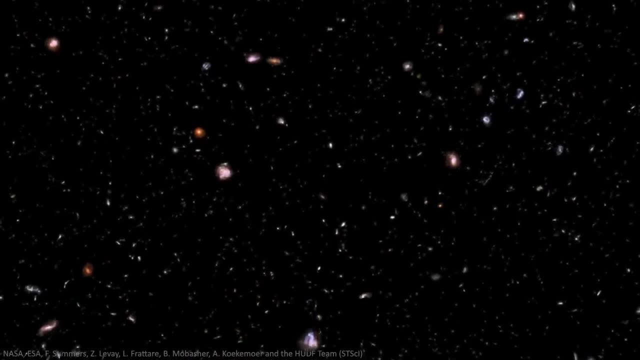 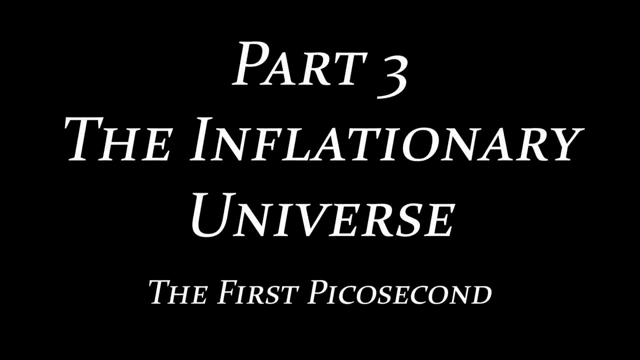 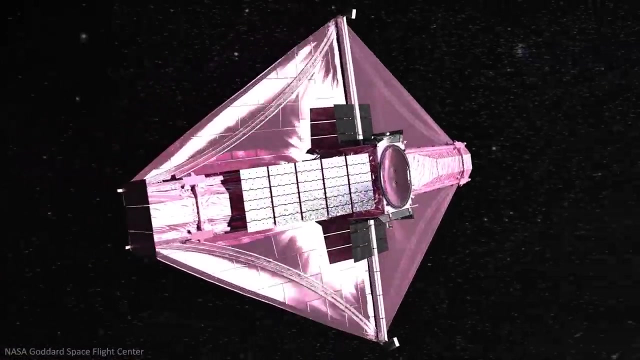 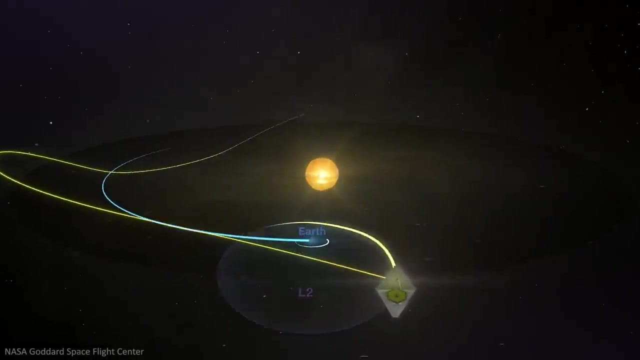 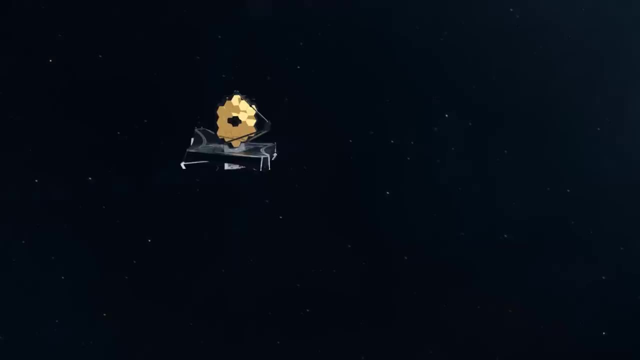 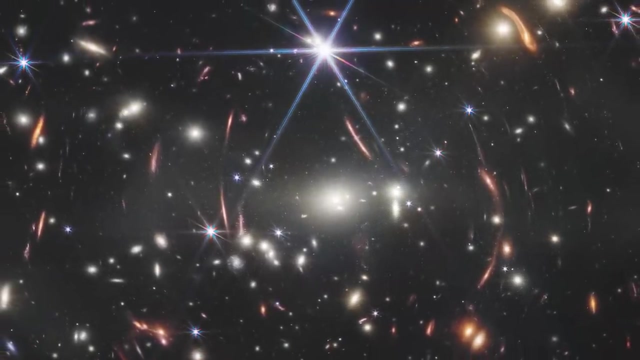 operations in earnest, But when it focused its 18 golden mirrors into some of the deepest reaches of the observable universe, scientists were shocked After seeing the images returned from the revolutionary telescope. American astrophysicist Alison Kirkwood said Kirkpatrick wrote in the scientific journal Nature that she found herself lying awake at 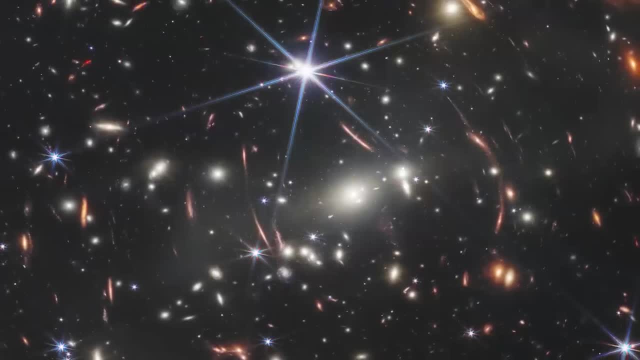 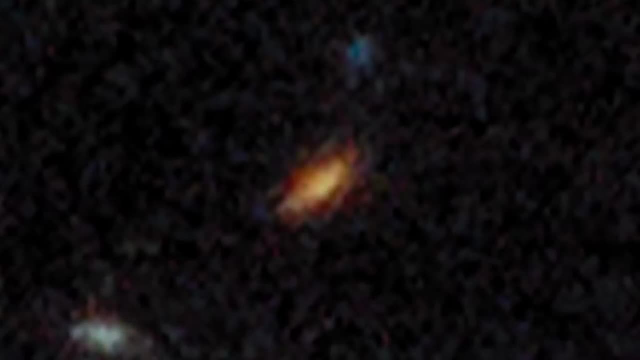 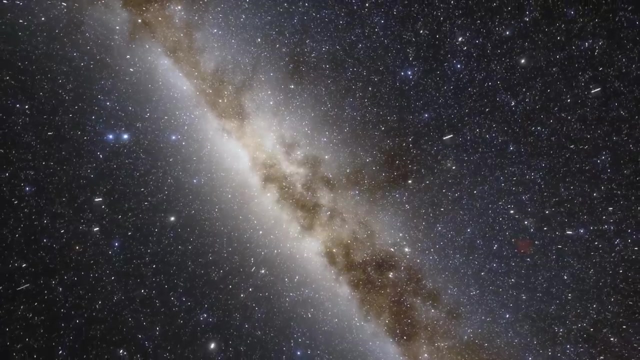 three in the morning, wondering if everything she had ever done was wrong. And within a month, these images and Kirkpatrick's comments had grown a life of their own. The Big Bang, The fixed speed of light, means that the deeper we peer into space, 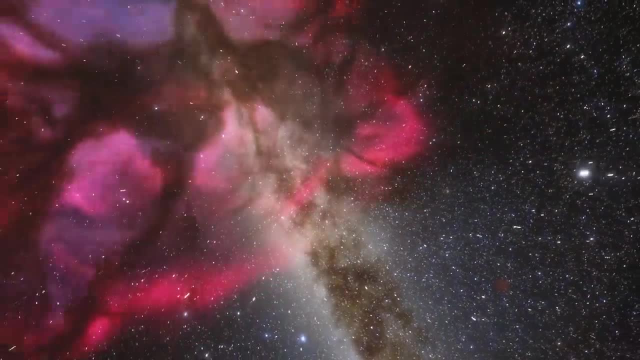 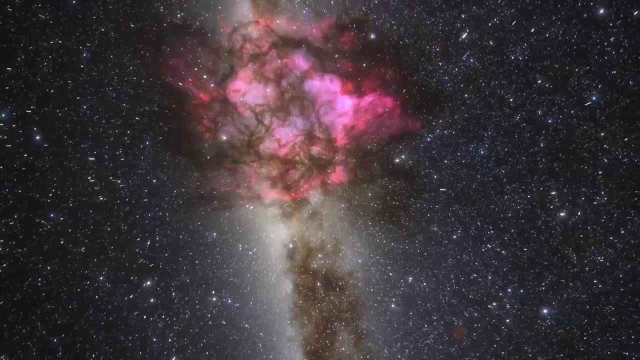 the further back in time we are looking, and at distances corresponding to just 200 million years, we will soon be able to see the stars. In the first few months after the beginning of everything, the James Webb Space Telescope had seengalaxies. 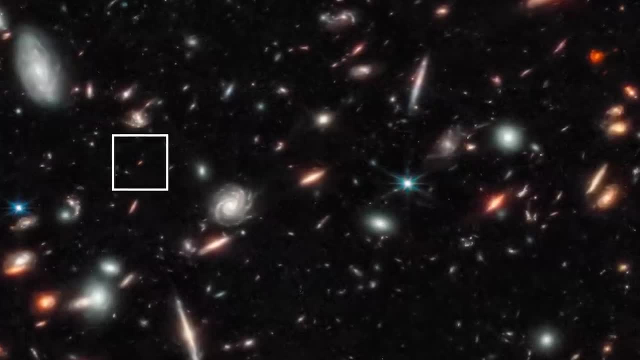 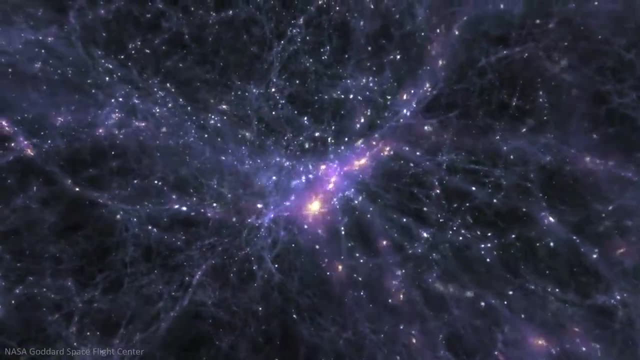 Not only that, but these galaxies were ordered with much more structure than anyone had thought possible. Theories of star and galaxy formation had no way to explain it, and it was this that Kirkpatrick had been so concerned about. Unfortunately, soon her concerns had been. 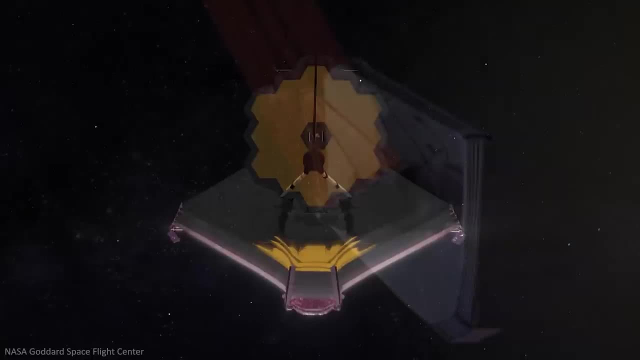 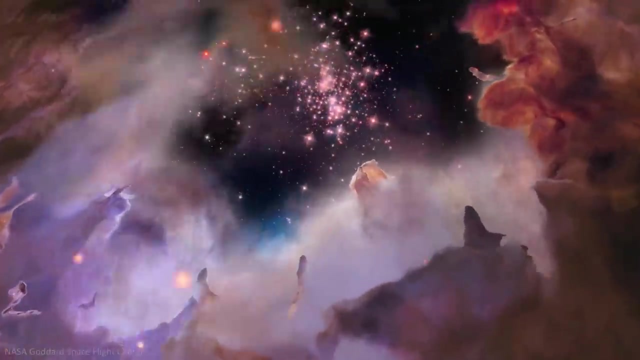 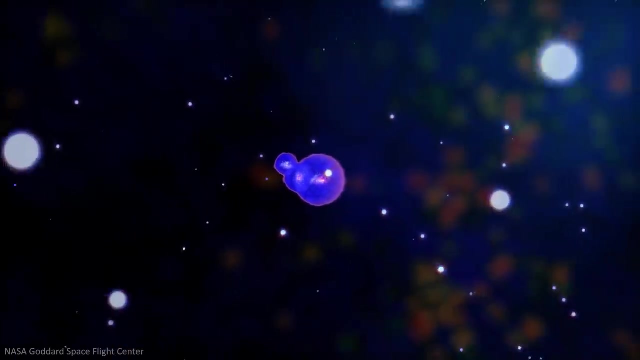 extrapolated to cast doubt on the Big Bang itself, with some media outlets claiming that the next generation telescope had disproved the landmark theory with its very first images. Thankfully, those concerns were misplaced. Kirkpatrick had only been concerned about existing theories on galaxy formation, not entire cosmos creation, The inexplicable structuring of early galaxies. 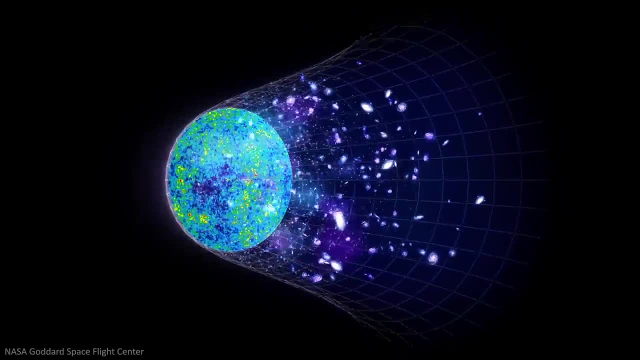 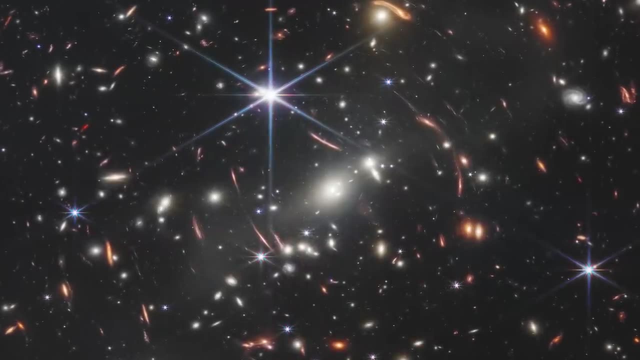 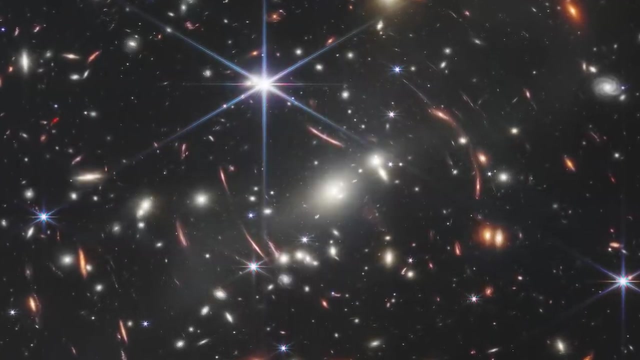 meant that there was a piece missing from our understanding, not that everything we knew was wrong, little more than a storm in a cosmic teacup, And so the Big Bang is safe from that quarter, for now at least, But as a complete explanation of how our modern universe came to be. 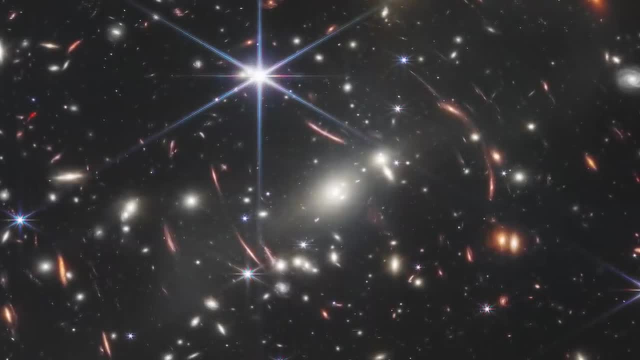 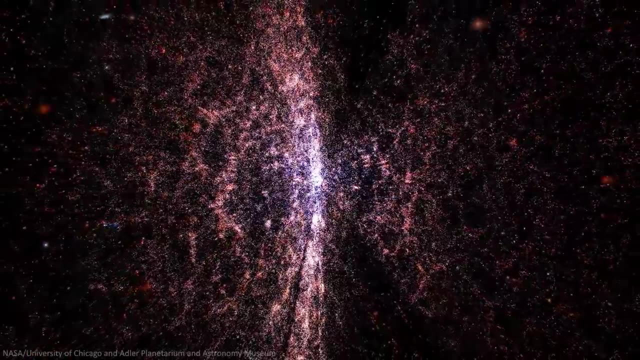 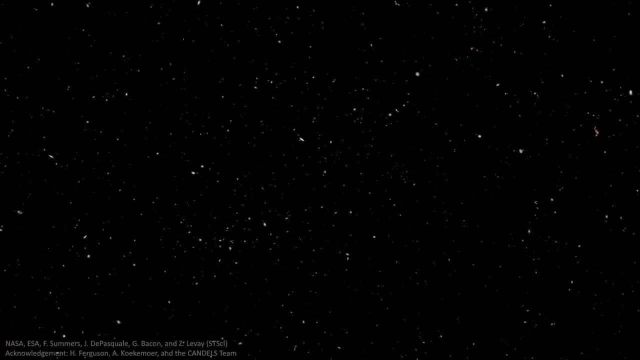 it has been under far more severe threat for much longer. When we look at the large-scale structure of the universe as it is today, there are a number of phenomena that don't quite add up. To begin with, the average temperature, Even though stars burn at several million degrees. 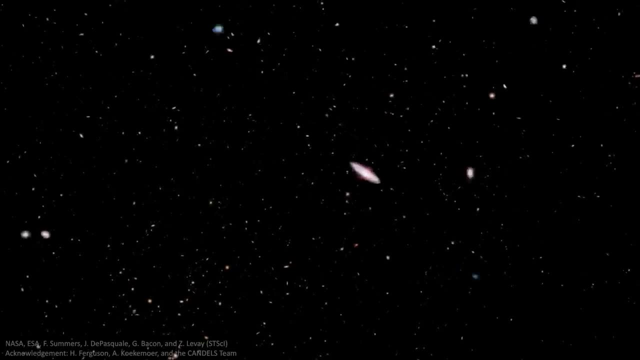 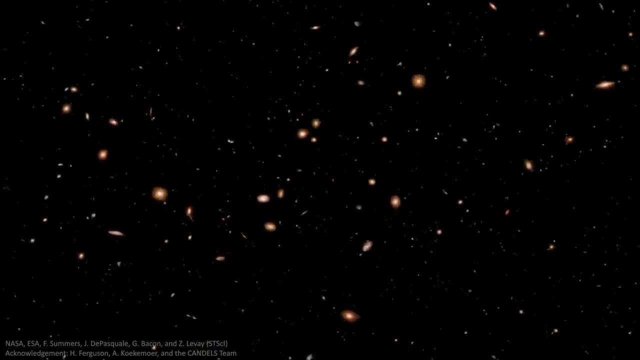 Celsius and empty space shivers at just a few degrees above absolute zero. the average temperature that we observe in one direction is remarkably similar to any other: 2.7 Kelvin everywhere in the universe, all 93 billion light-years in diameter of it. 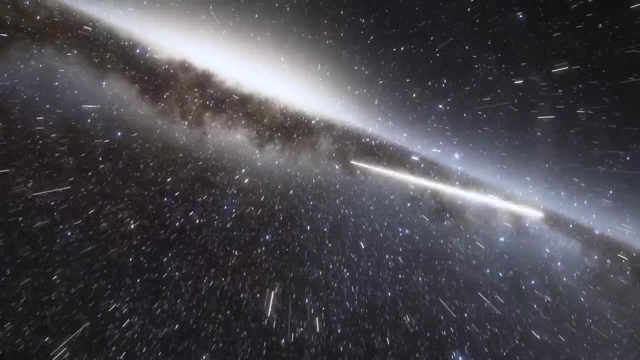 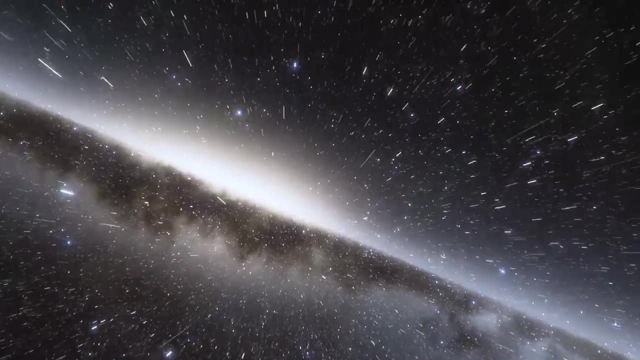 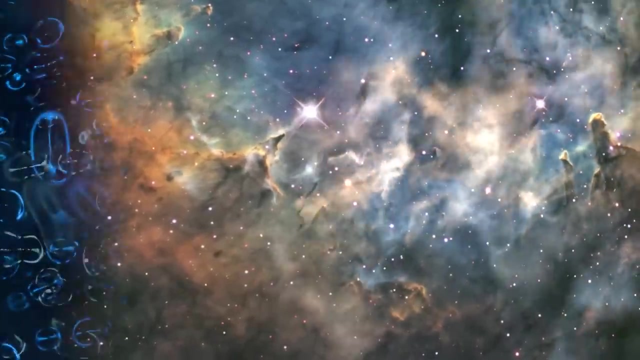 But how? If the universe has been gradually expanding for nearly 14 billion years, then how can two points further? The fact that we see such thermal homogeneity now implies that there was thermal homogeneity back in the universe's earliest moments, a fact that seems wildly improbable given the nature. 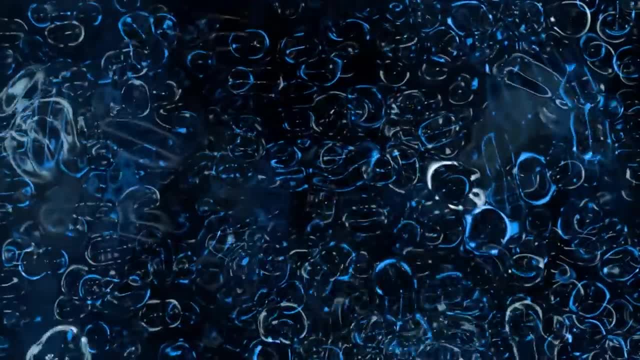 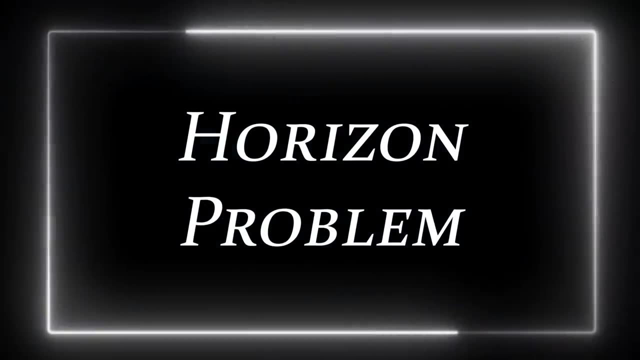 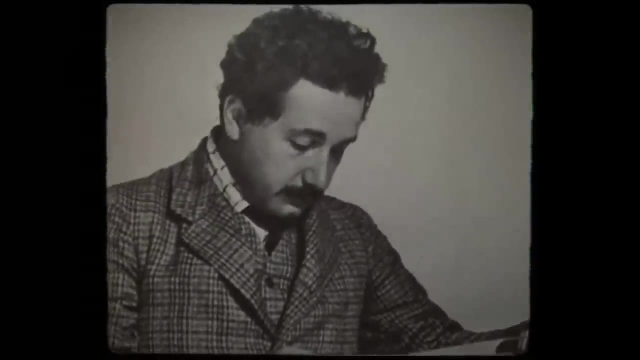 of quantum fluctuations in the compactified early cosmos. This is known as the homogeneity problem or the horizon problem. But there is more. General theory of relativity describes how massive objects create curves in space-time which then govern the movement and evolution of matter within that space-time. Stars 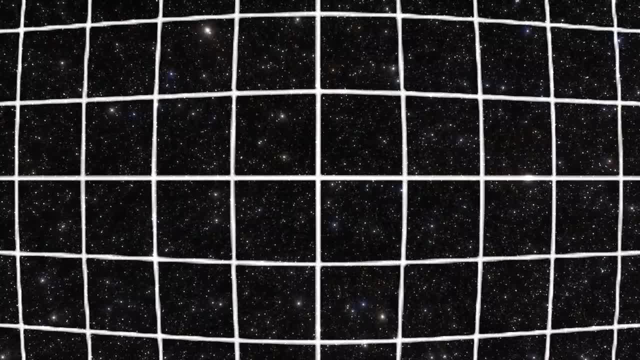 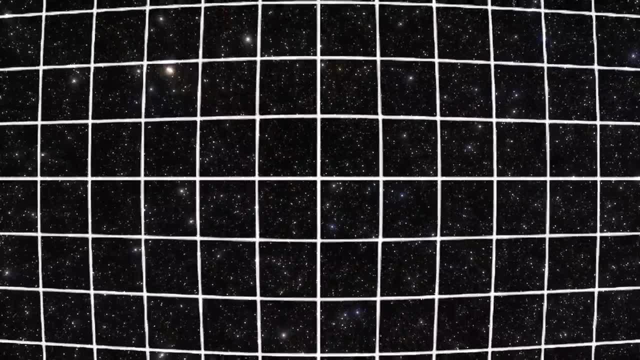 galaxies and black holes leave pinches and pockmarks in the local-scale structure of space-time, but when we zoom out to a larger scale, these imperfections even out to leave a smoother structure which, like the average temperature of the cosmos, seems to vary very little. 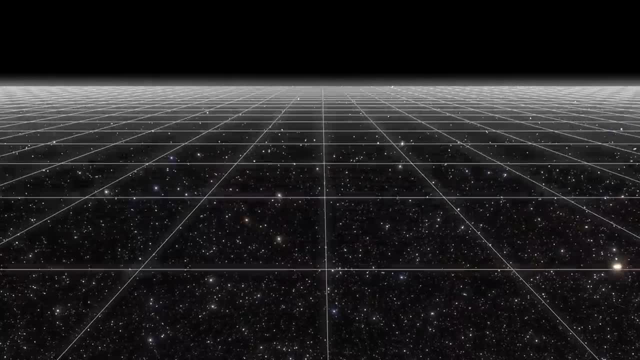 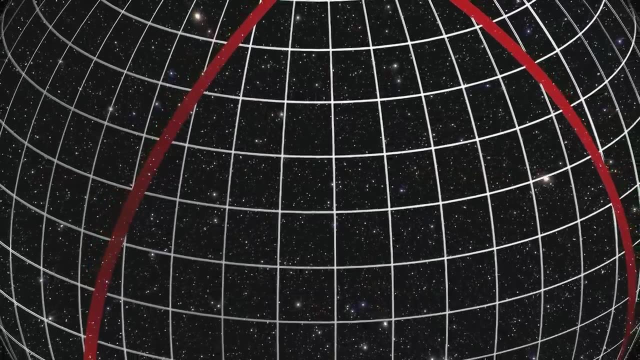 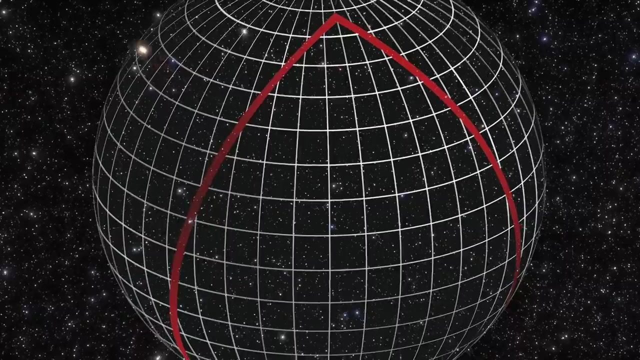 The universe on the largest scale seems flat. If the overall density of matter in the universe is sufficiently great, space-time will be what's known as positively curved, bending back on itself like the surface of a sphere. This means that eventually, the gravity exerted by all the matter in the universe will be enough to slow down and eventually reverse the trend. 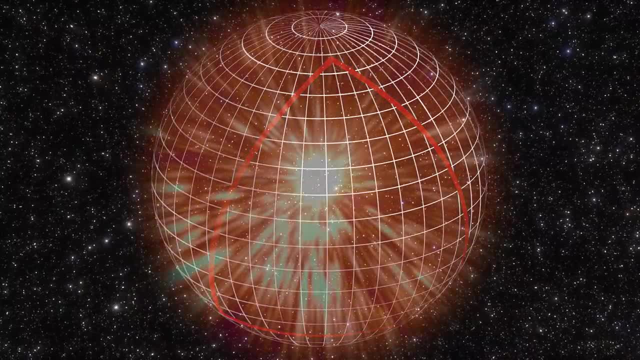 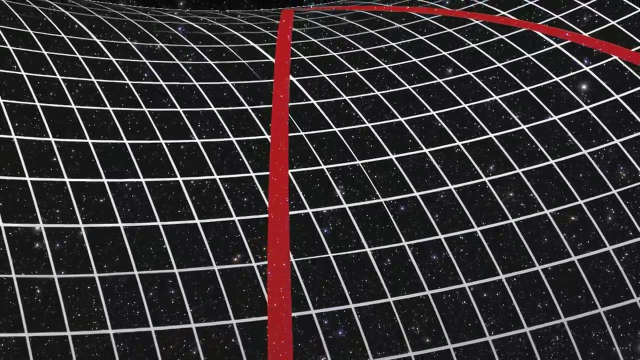 of expansion, collapsing the universe back in on itself in a so-called big crunch. In contrast, if the overall density is much less, it results in a negative curvature of space-time bending out in an open fashion like the surface of a saddle. 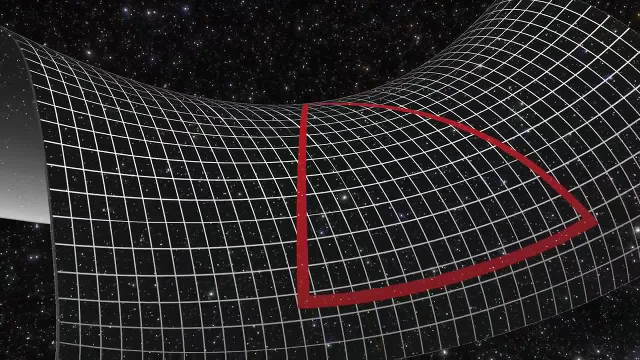 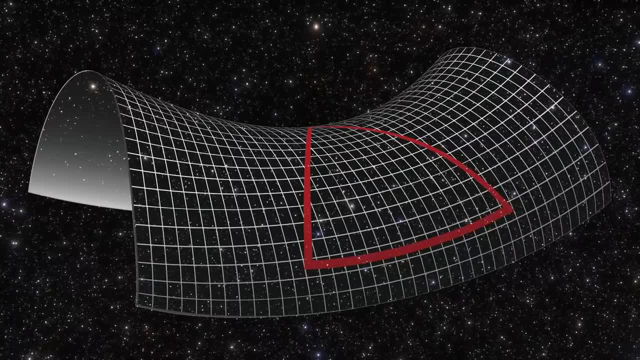 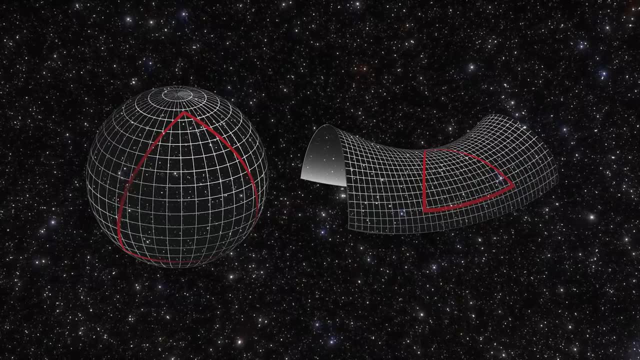 With this geometry, gravity never overcomes expansion and the cosmos continues to grow for eternity. Which of these overall geometries holds true has big implications for the future evolution of our universe, and so it has been the preoccupation of astronomers to try to measure the overall curvature of the cosmos we can see, And counterintuitively. 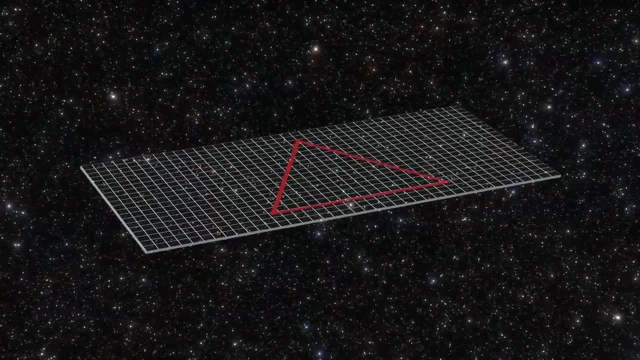 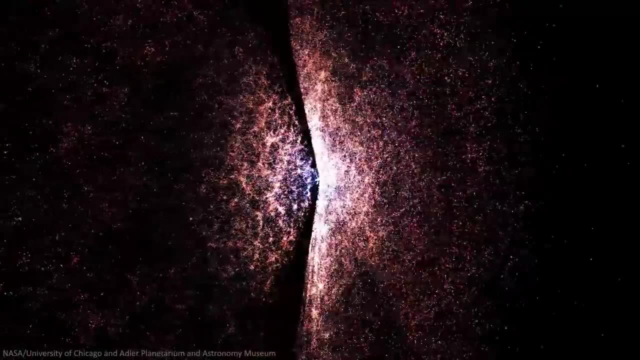 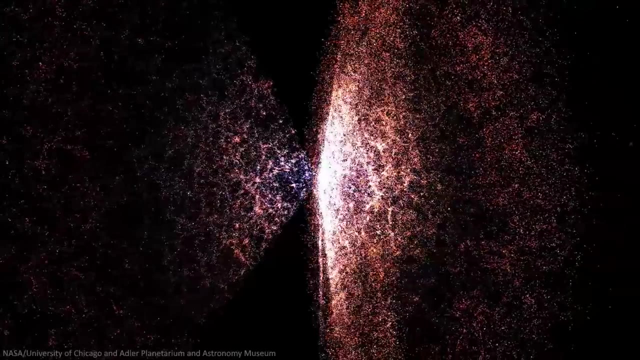 It appears to be completely flat, Just like the horizon problem. the likelihood of this being the case is incredibly small, tantamount to tossing a coin and having it land perfectly on its edge. For obvious reasons, this has become known as the flatness problem. 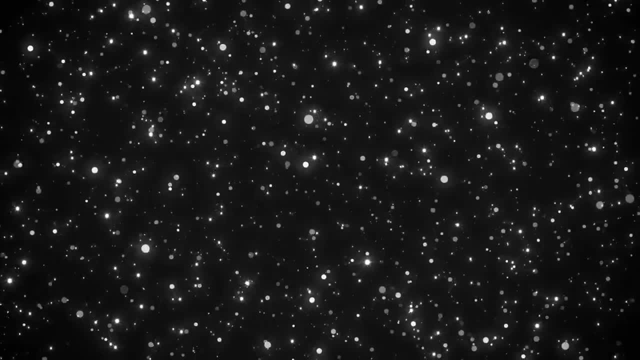 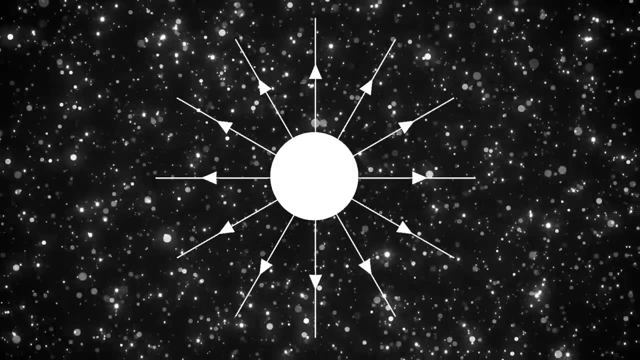 And there is one additional problem that blights our theories of the cosmos in the first trillionth of a second. And there is one additional problem that blights our theories of the cosmos in the first trillionth of a second: They are seen seem to be no magnetic monopoles at all. All through the universe, electrical charges exist. 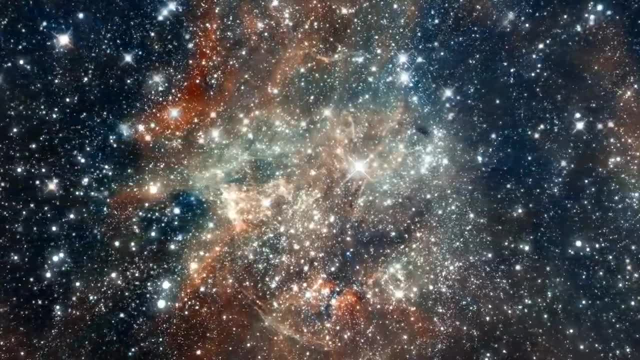 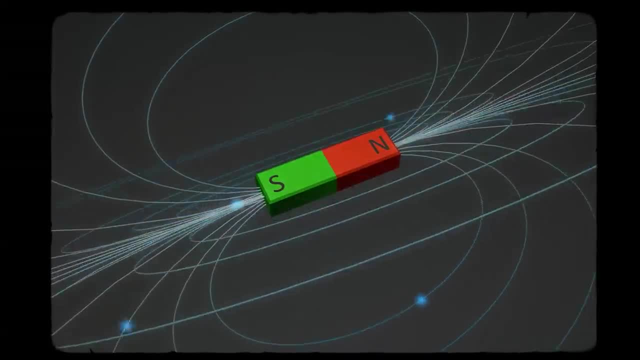 in positive and negative pairs cancelling one another out to result in a stable, neutrally charged hole. In a similar way, magnets are found with both north and south poles with magnetic field lines flowing between them to produce a stable and balanced hole. 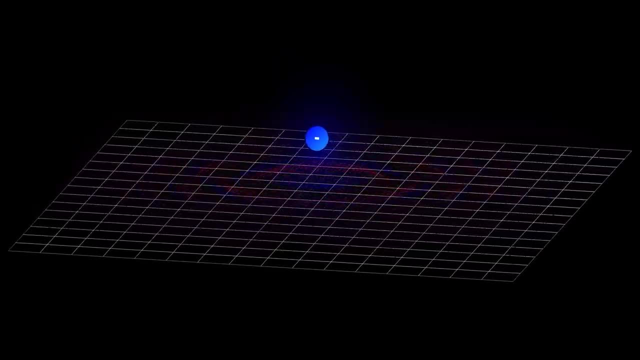 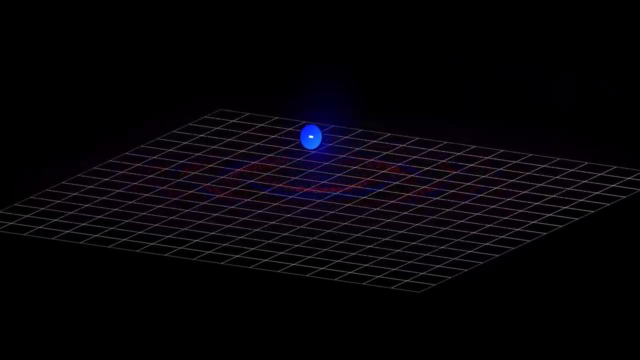 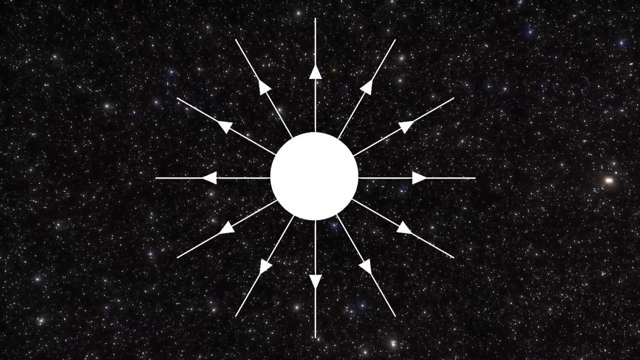 However, while it is possible for both positive and negative charges to be found alone, like in isolated protons or electrons respectively, no such isolated poles exist for magnets. No matter where we look in the cosmos, we have yet to find a lone monopole without its. 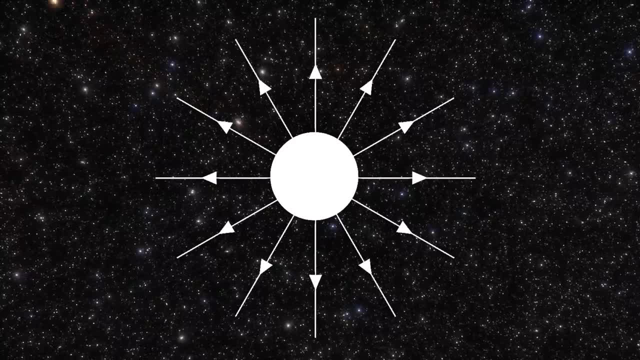 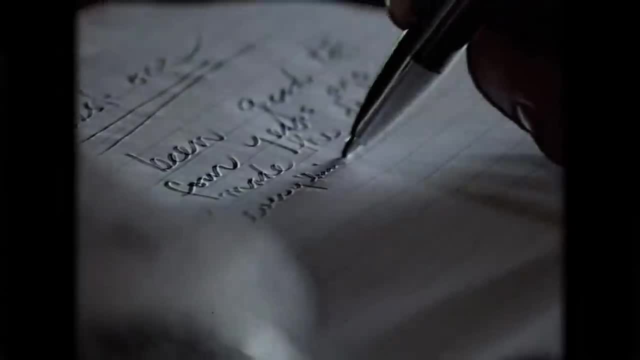 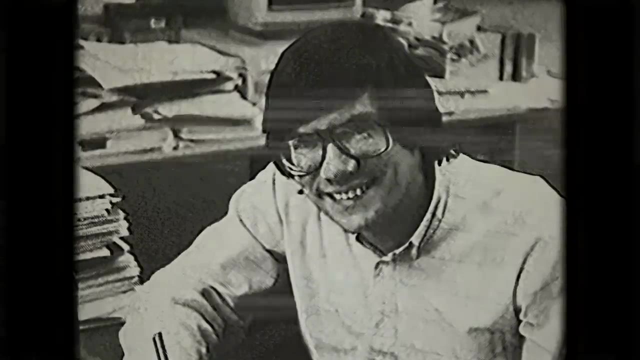 opposite pairing. And so it was on a December night in 1979, while puzzling over the mystery of the missing monopoles, that theoretical physicist Alan Guth struck on a remarkable solution, One that not only addressed his own problem but also tackled the horizon and flatness problems, as well, Instead of expanding gradually over billions of years to the vastness we see today, Guth found a mechanism by which the universe could have suddenly and almost instantaneously inflated to many, many times its original size, before slowing down and continuing in a more linear. 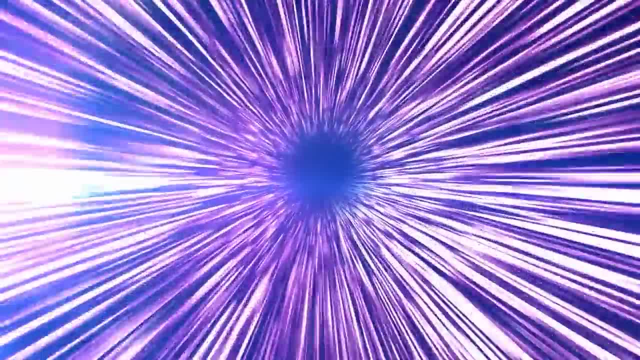 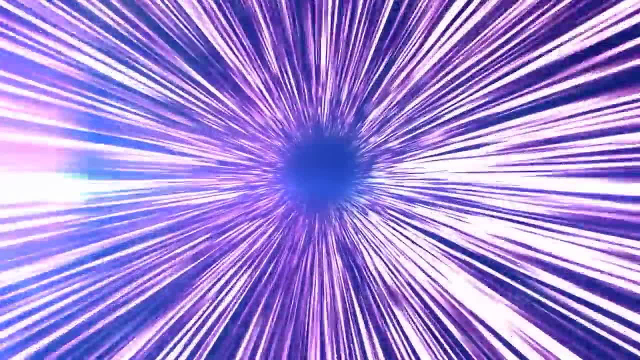 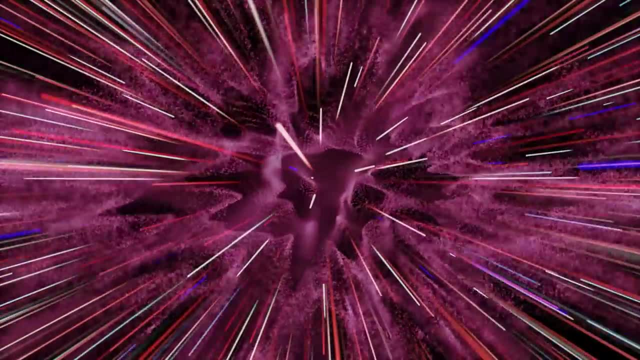 expansion. This inflationary period that Guth proposed would see the universe double in size around 90 times in less than a trillionth of a second, resulting in an exponential expansion that would fundamentally change the face of the cosmos. Because when exponential expansion is at play, things get very large very quickly. 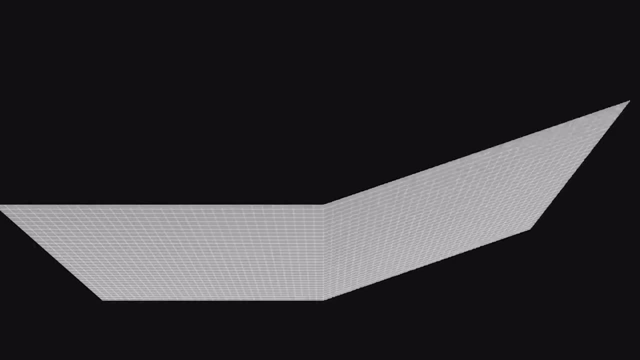 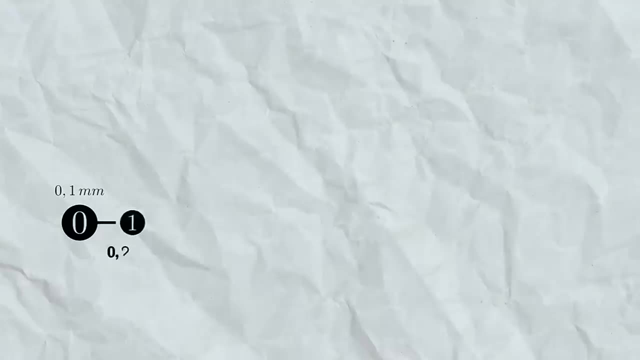 Consider folding a gigantic piece of paper in half time and time again. If it starts out one tenth of a millimetre in thickness, it will be a giant piece of paper in half. If it starts out one tenth of a millimetre in thickness, it will be a giant piece of paper in half. Then the first fold. 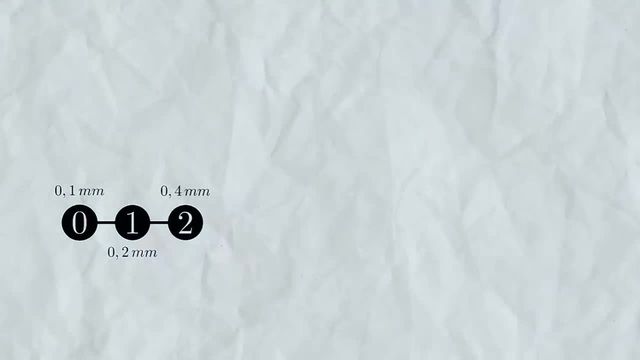 will double that to two tenths, and the next brings it to just under half a millimetre. The third fold doubles it again, and now it is about the thickness of a finger nail. So far, so unremarkable, But by the time you reach 7 folds, the single sheet has now reached the thickness of 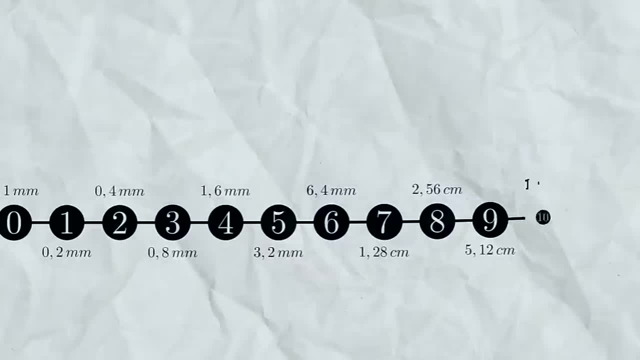 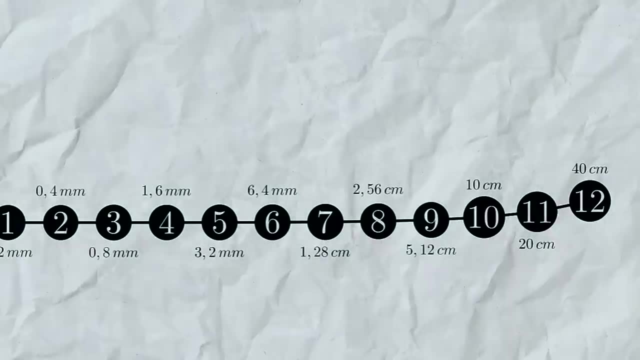 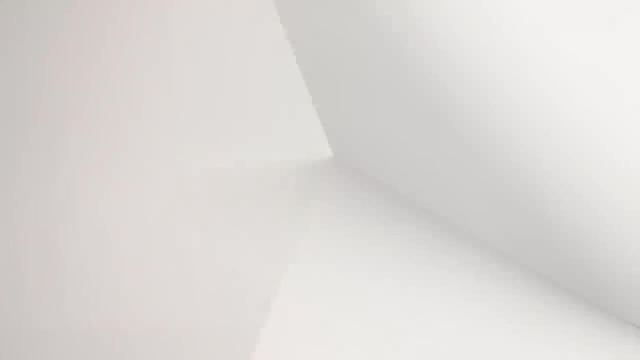 an entire notebook- 10 folds, and it will be as thick as your hand is wide, And the world record for actually doing this experiment sits at just 12 folds when, in 2002, an American schoolgirl folded a piece of tissue paper more than 1.2 kilometers in length into a 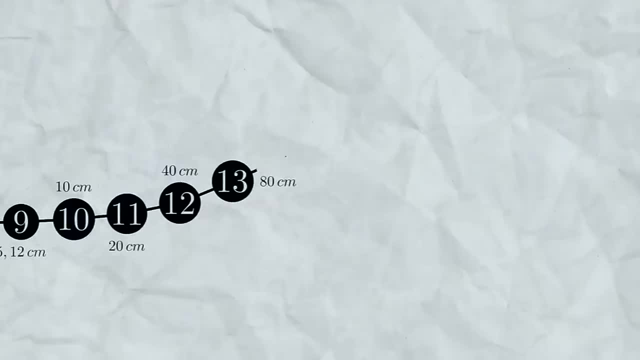 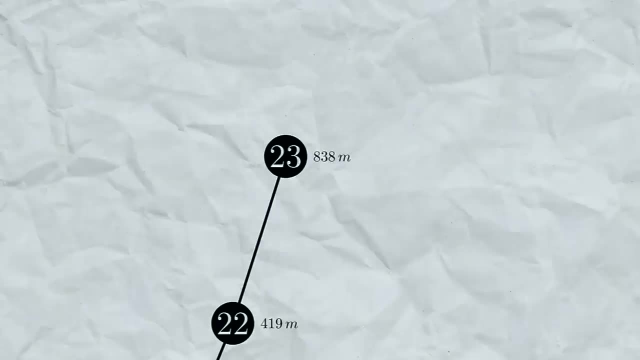 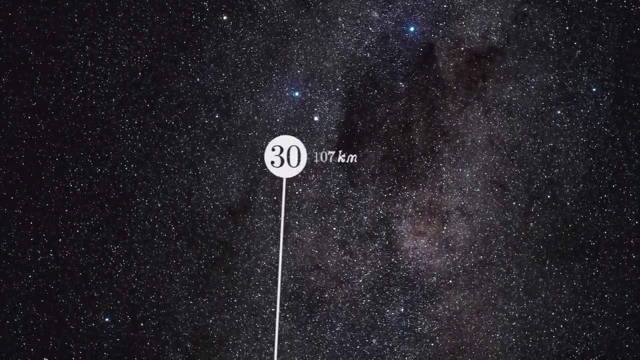 bundle over half a meter thick. But if it were possible to make and handle an even bigger sheet, further folds would increase the thickness astronomically. 23 folds will make the paper around one kilometer thick and 30 folds will be enough to get you to space rising 100 kilometers. 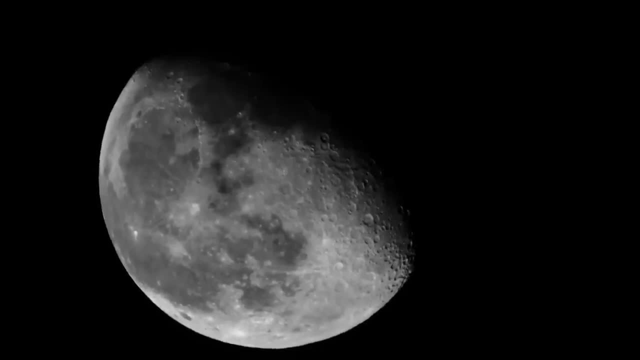 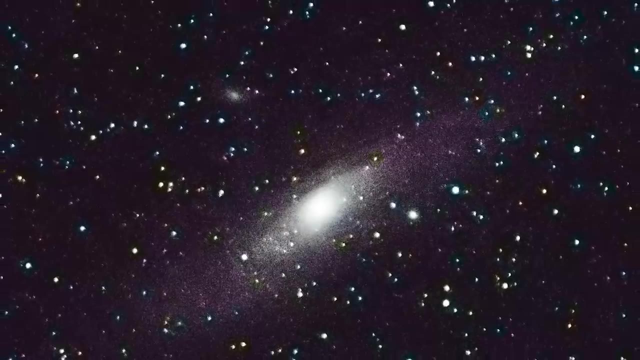 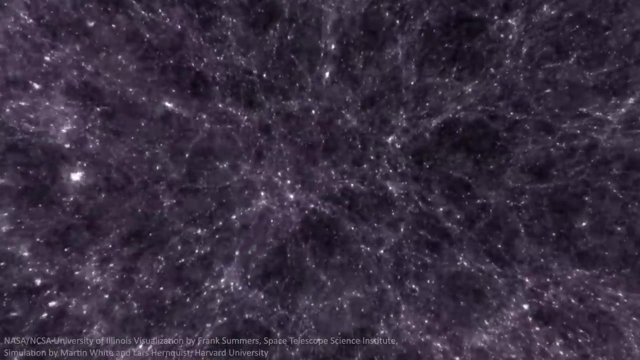 from the surface of the Earth. 42 folds will get you to the Moon and 51 will make it to the Sun. 81 folds will make the paper as wide as the Andromeda Galaxy, at around 141,000 light-years across, And 90 folds equivalent to the 90 doublings that Guth proposed for the inflationary. 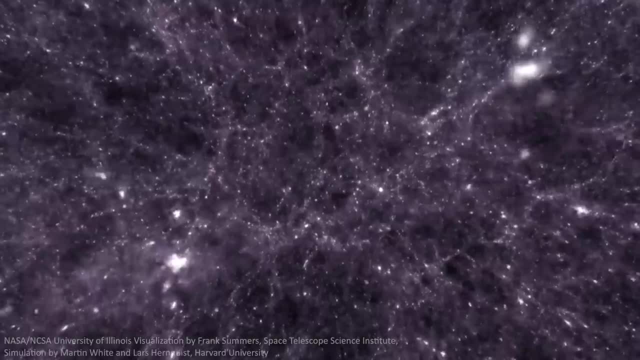 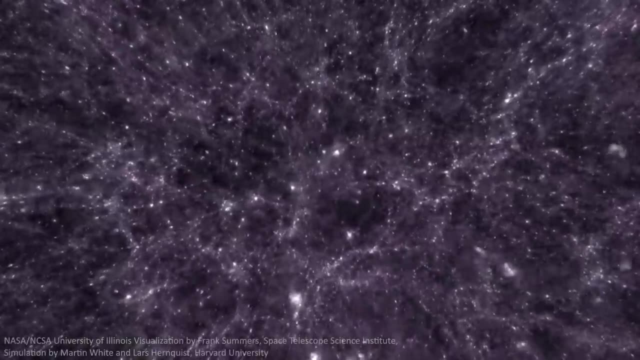 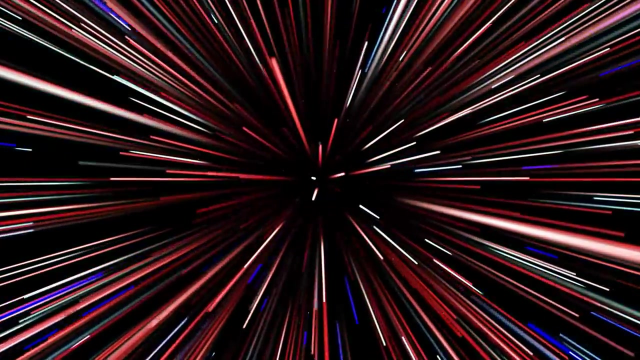 period will transform that single colossal piece of paper to a folded pile bigger than the entire Virgo supercluster, 130 million light-years across. This incredible inflation is what Alan Guth proposed for the entire universe In less than a trillionth of a second. after the confusing turbulence of the Planck era and the Grand 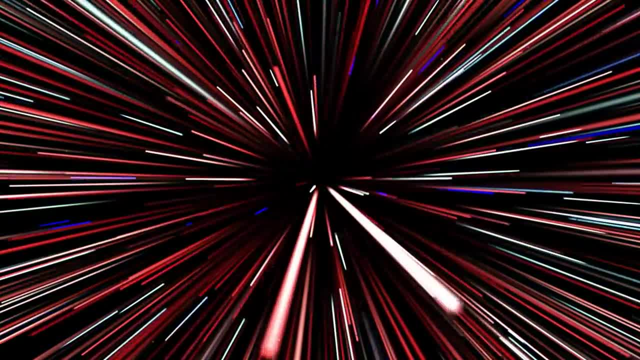 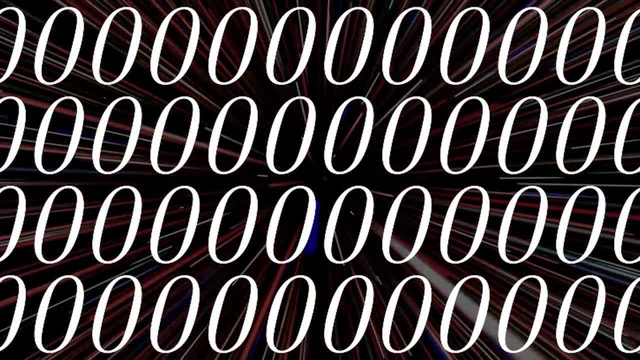 Unification era, the hot, hyper-dense cosmos blew up to more than an octillion times its original size. It was this, if anything, that put the bang in the Big Bang. The universe, which one moment had seemed so hot, energetic and hot, was now a big bang. And it was this, if anything, that put 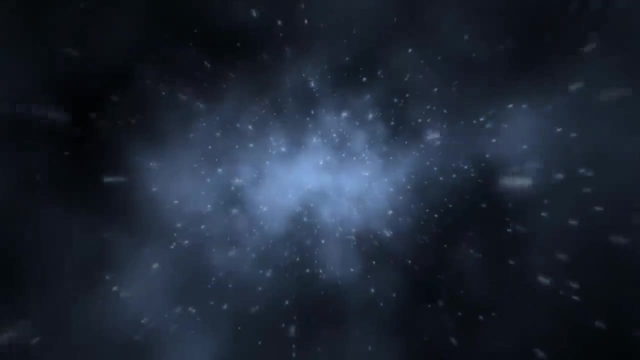 the whole universe back together…. 214 And full is now left vast, vacuous, cold Обс дней vary в то как в How вкусно, холодно и moldно пquet و покинутый. 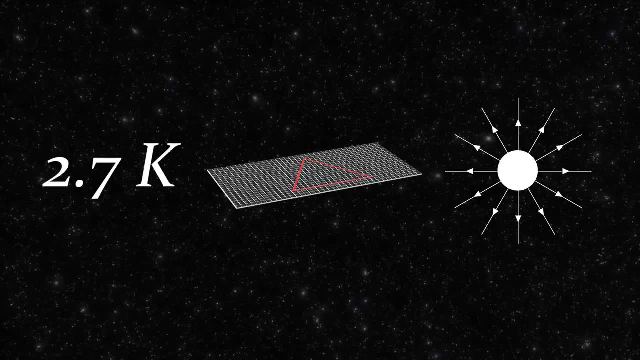 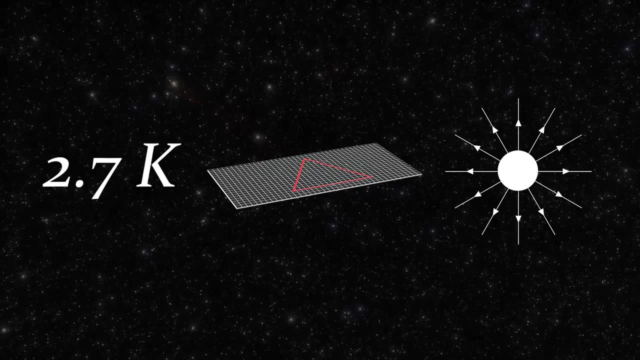 Я лучше, Though it seems drastic…It IS indeed an elegant solution for the three problems vexing the Big Bang Theory, because Inflation allows us to entertain the possibility that the immense universe we see isn't actually all there is. It is merely a bubble. 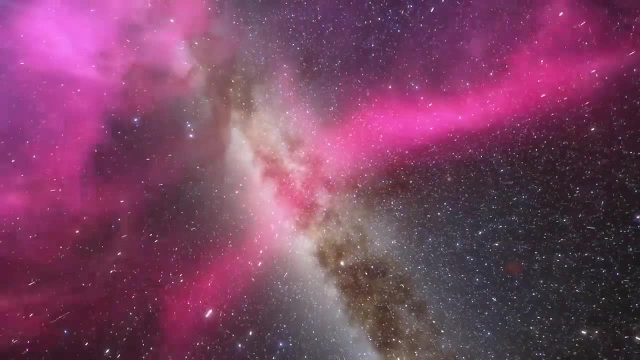 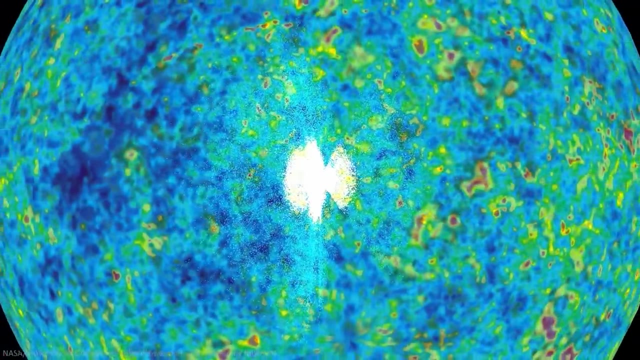 of observable universe, whose size is defined by the speed of light, the amount of time that has passed and the expansion that has taken place since then. 283 taken place since the beginning of time. Thanks to inflation and subsequent expansion, our observable bubble is some 93 billion light. 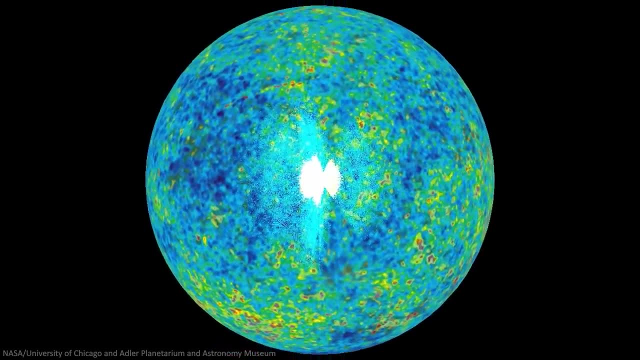 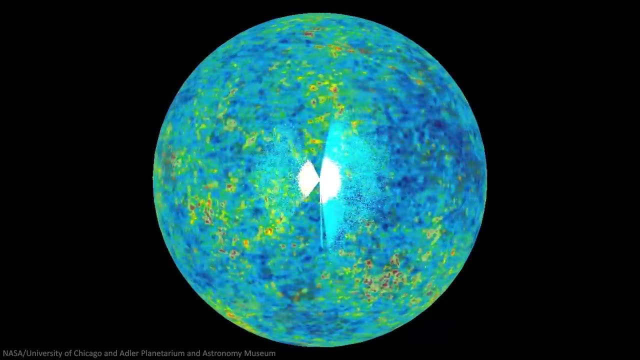 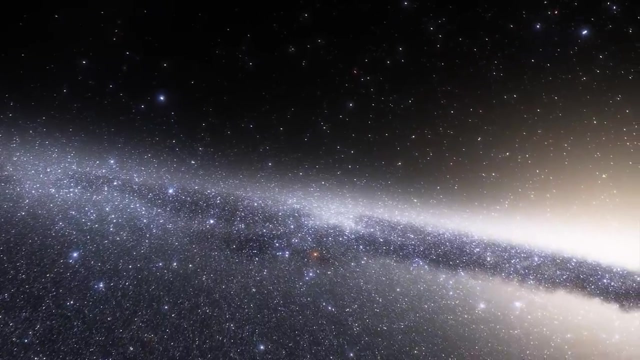 years in diameter, but it is still merely a fraction of the universe as a whole, and it is in this unseeable extent that the answers to our problems can be found. The horizon problem of thermal homogeneity is only a problem if the homogeneity we see. 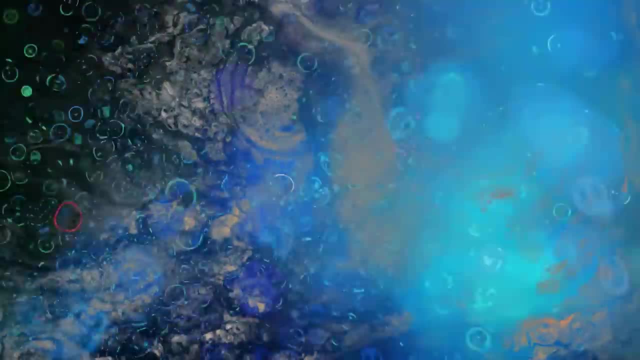 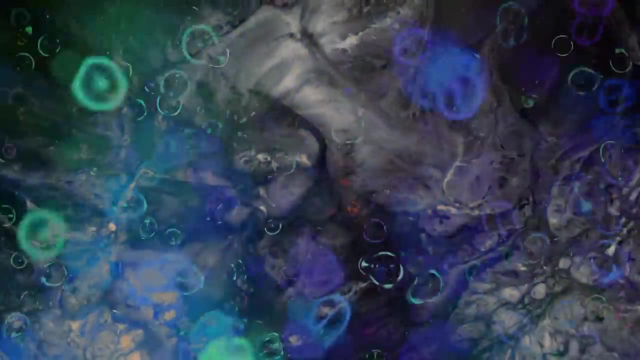 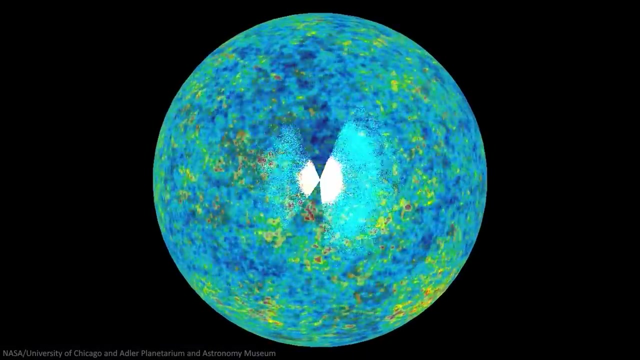 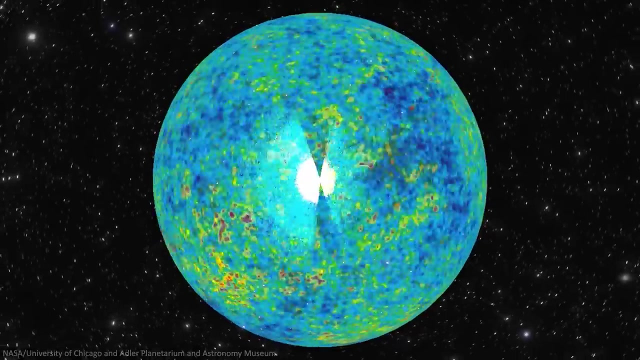 applies to the entire universe, But inflation allows the compact early universe to contain extreme thermal variations which are then flung far apart from one another during exponential expansion. Our local patch of observable universe merely represents one small part of the whole, which was in thermal equilibrium with itself before inflation happened and may be wildly different. 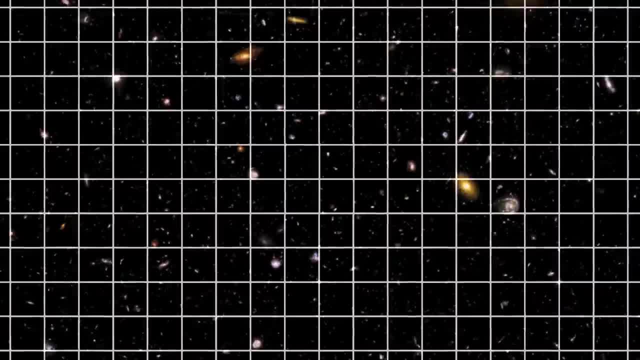 from other parts that we cannot see. Similarly, the flatness problem of the universe is only a fraction of the universe as a whole, and it is in this unseeable extent that the answers to our problems can be found. The problem of space-time curvature is only a puzzling coincidence. if the flatness we 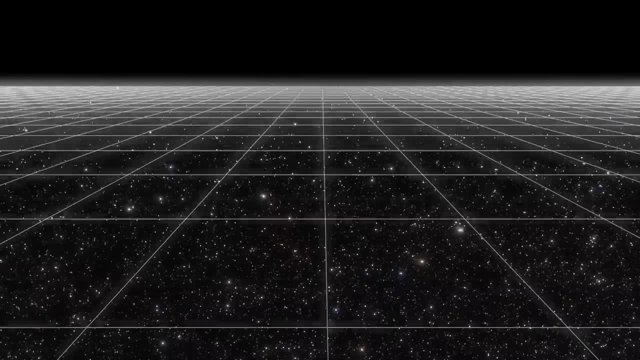 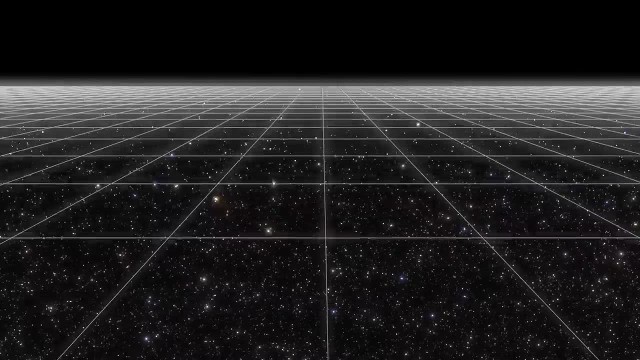 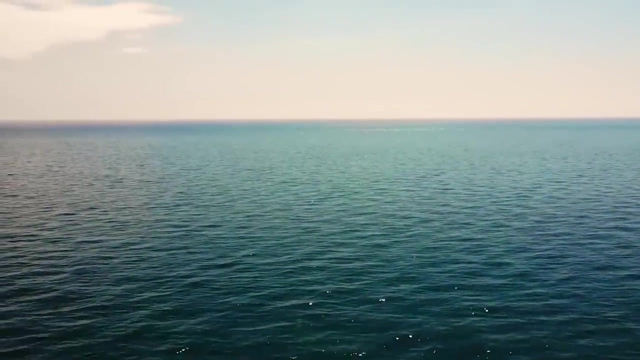 see applies to the entire universe, but if we are only seeing a tiny fraction of the whole, then it is impossible to say whether it does or not. It could be a matter of perspective. From the seashore, an ocean horizon appears flat, but it is only when we fly far above. 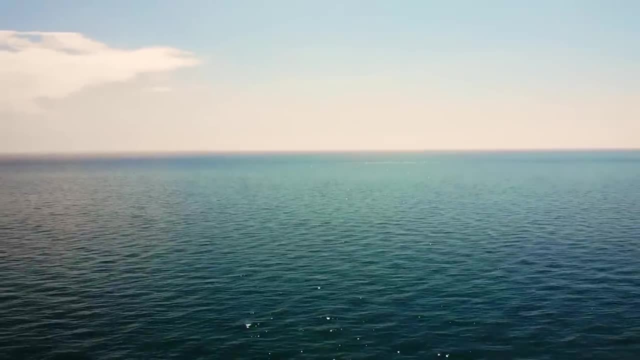 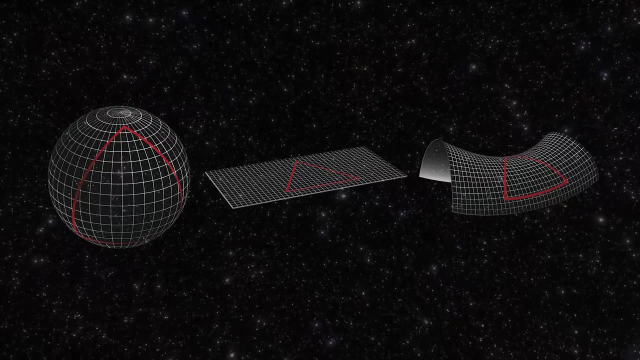 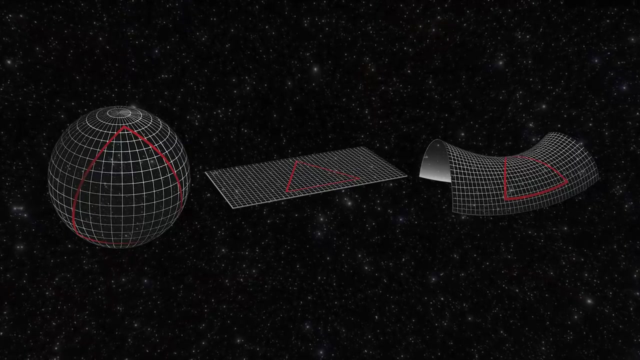 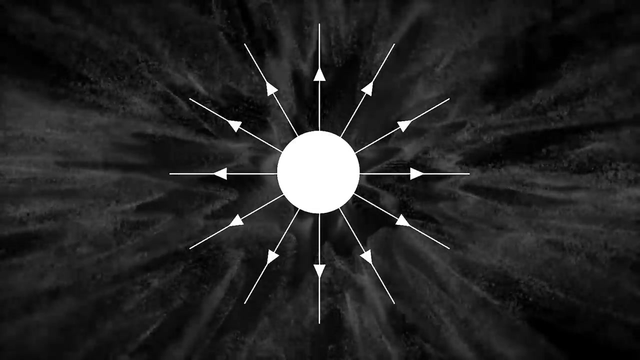 the surface, perceiving more of the earth that we see it is in fact curved. The wider cosmos may be positively curved, negatively curved or a twisted combination of both, but we are unable to see past our own cosmic shore. And finally, the absence of magnetic monopoles is only a problem if we assume they are missing. 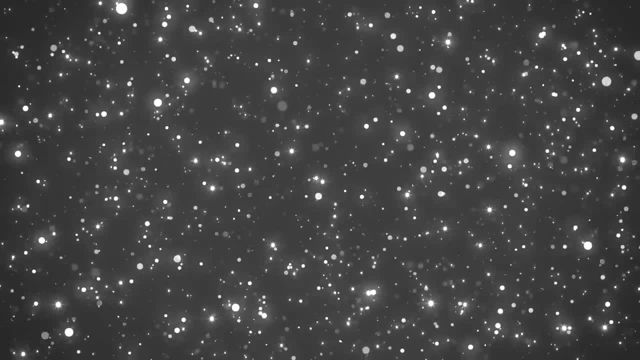 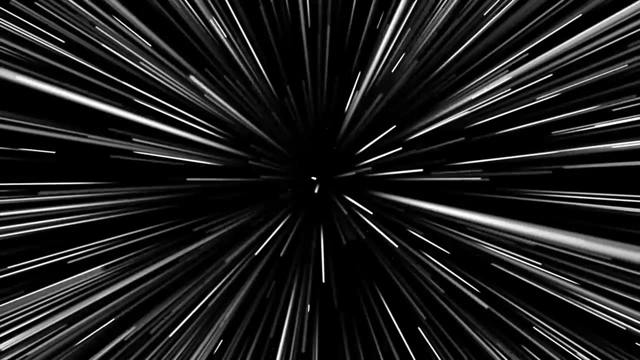 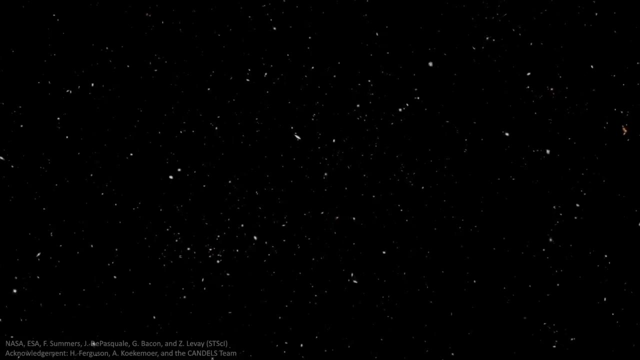 from the universe as a whole. but if they existed in the early universe in the quantity predicted by our current models, then exponential inflation would have seen them spread apart from one another Until they were distributed to roughly one per observable universe. And when we are looking for a singular monopole within a sphere 93 billion light-years across. 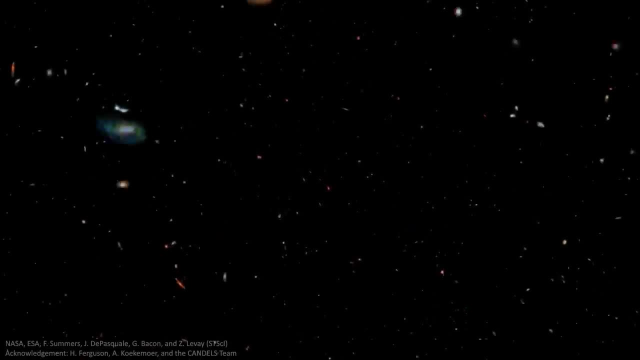 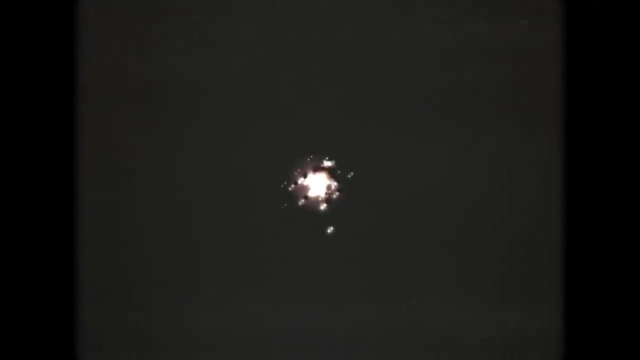 it's little wonder we haven't found it yet. Inflation is now securely part of our understanding of the earliest moments of the universe, and cosmologists have spent the 40 years since Alan Guth's revelation figuring out the mechanism by which a universe can so suddenly and so dramatically change. 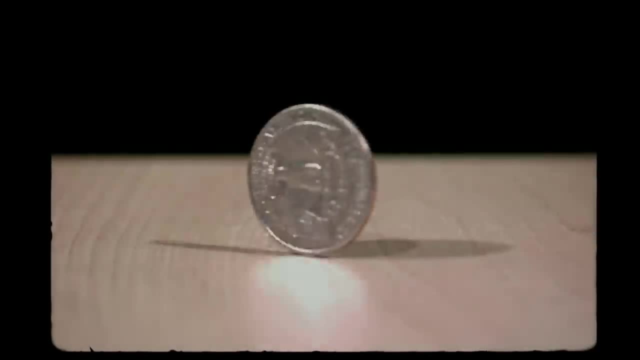 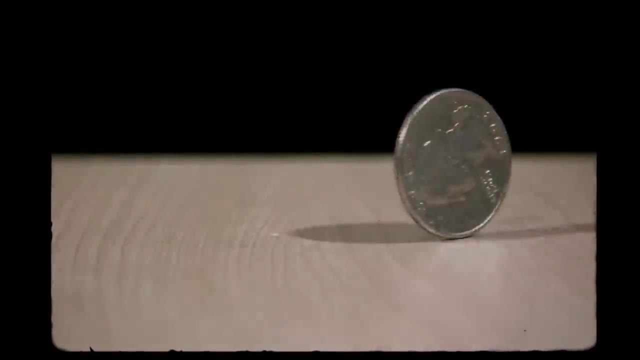 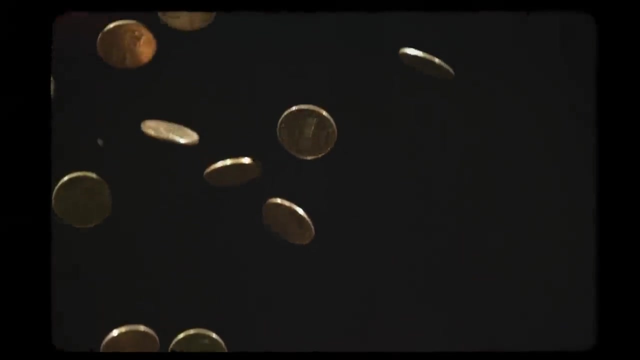 The timing of this dramatic phase coincides with the energy drop and cooling that saw the end of the grand unification of fundamental forces and the emergence of the strong nuclear force. It is theorised by some scientists that the decay of the X-Boson messenger particles that 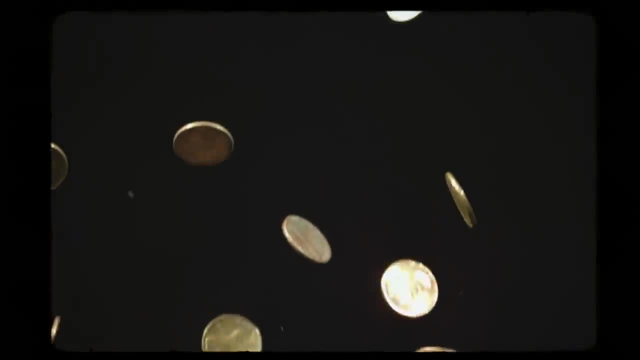 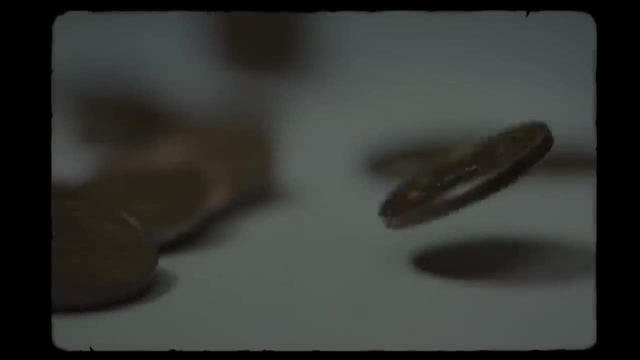 carried the electrostrong force, created a strong inflation field carried by a new messenger called the inflaton. This overwhelming new inflation energy transformed the entire universe into a new form of energy, and this new form of energy was called the inflaton. This overwhelming new inflation energy transformed the entire universe into a new form of energy. 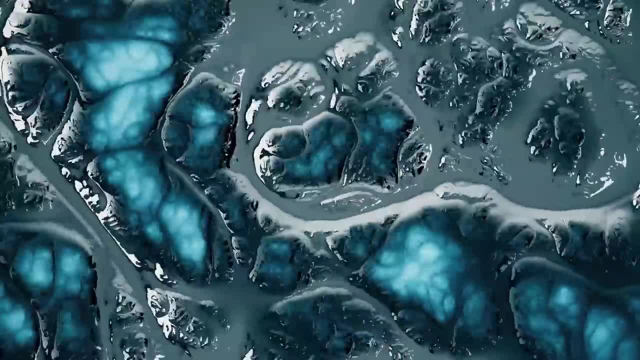 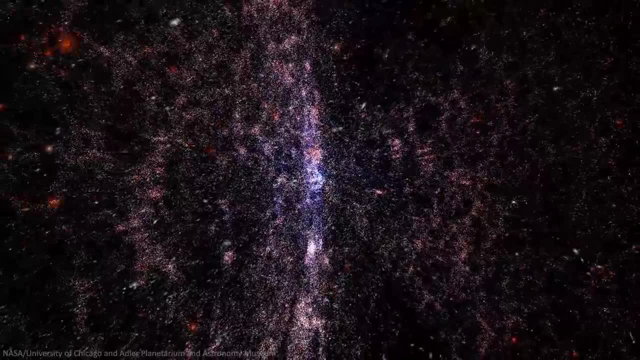 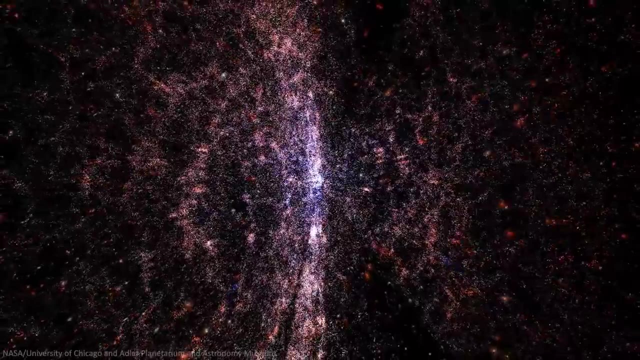 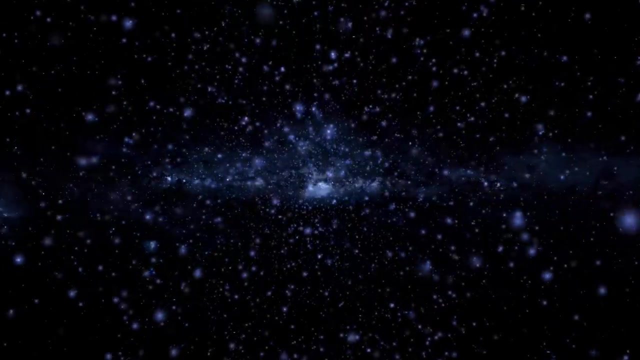 and drove universal exponential expansion, which saw quantum-scale irregularities almost instantly scaled up to large-scale structure, transient quantum fluctuations becoming huge regions of overdensity and energy that would provide the seeds for galactic clusters and superclusters in the modern universe. All of this expansion inevitably cooled and emptied the cosmos, leading to a 100,000-fold drop in average energy levels. The expansion of the universe was the result of the expansion of the universe and the expansion of the universe was the result of the expansion of the universe. and the expansion of the universe was the result of the expansion of the universe. 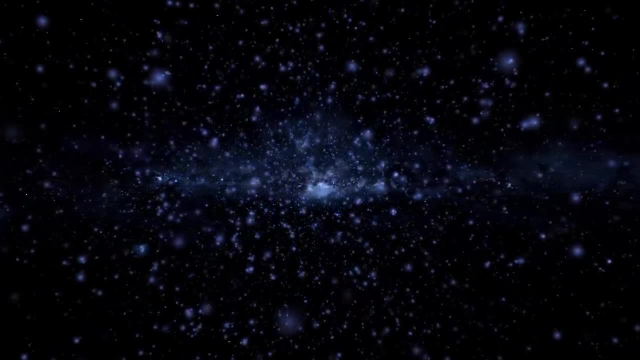 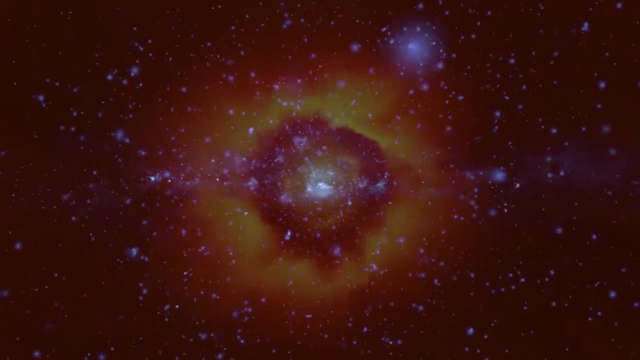 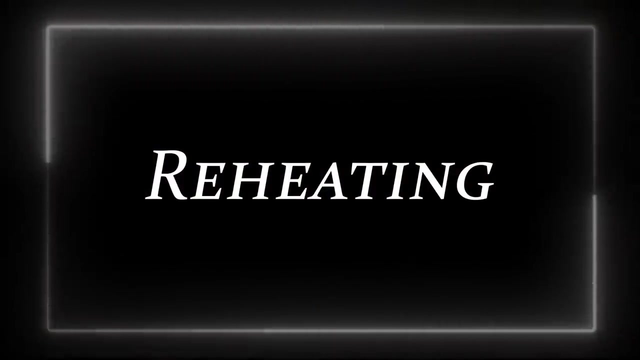 Scientists are as yet unsure of why exactly inflation stopped, but when it did, the inflaton field and particle decayed away, pouring much of that energy back into the universe in a phase known as reheating, And it's this that allows for the decisive creation of matter. 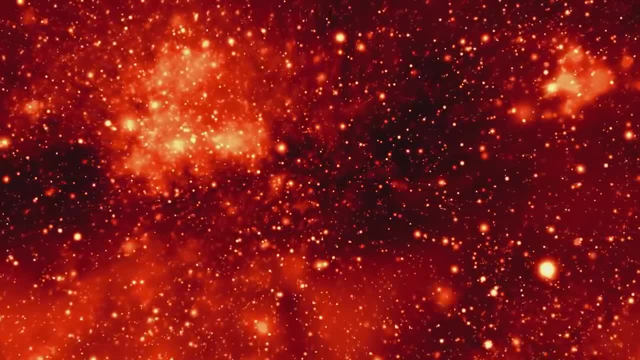 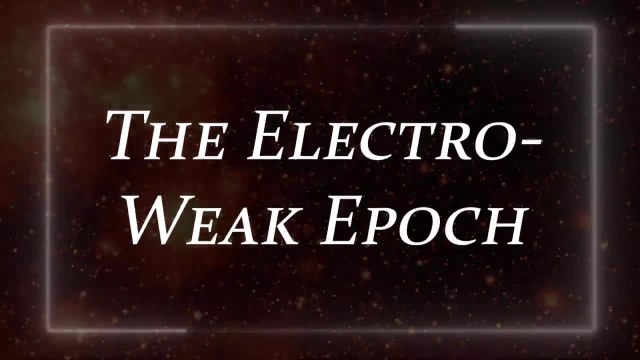 And now in a larger and roomier cosmos, the laws of nature are approaching something that we can finally understand and model. This is called the Electro-Weak Epoch, and it lasts until about a trillionth of a second. after the Big Bang. 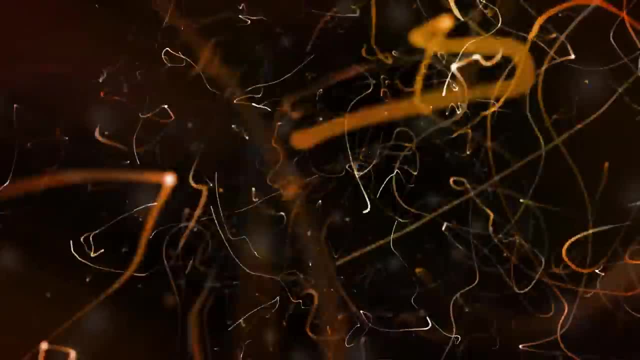 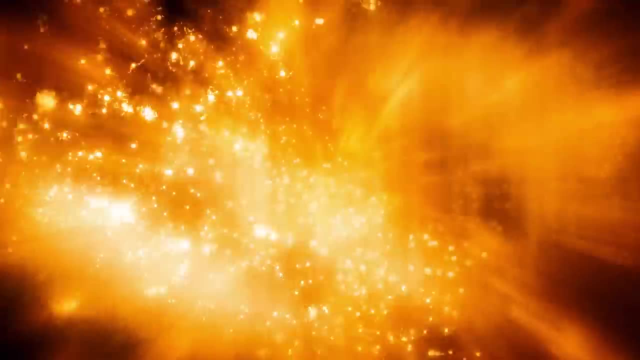 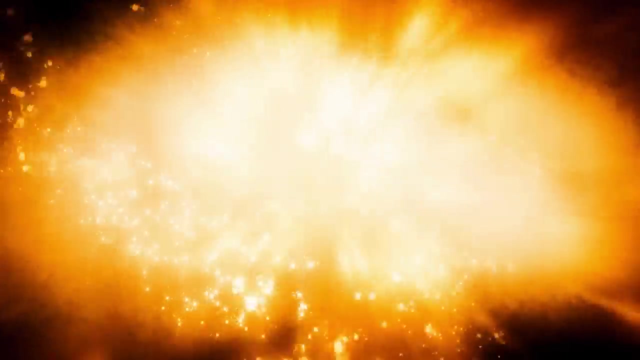 There are quarks and leptons, matter and antimatter, all ruled by gravity, the strong nuclear force and the chimeric electro-weak force. But temperatures and energies are still far too high for the strong force to have any real effect on the supercharged particles in this post-inflationary maelstrom. 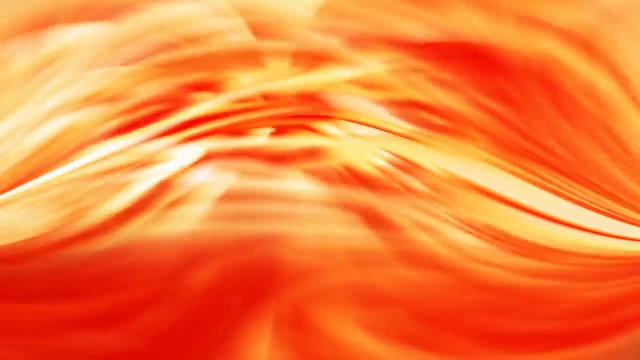 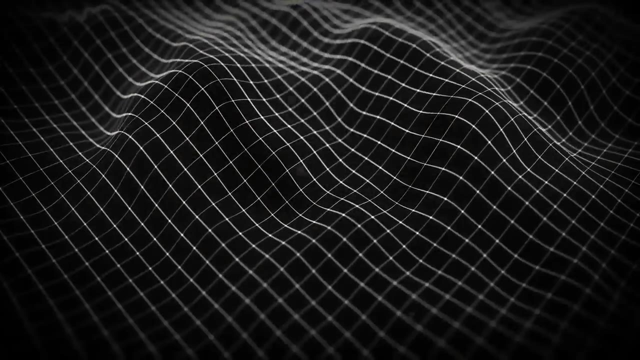 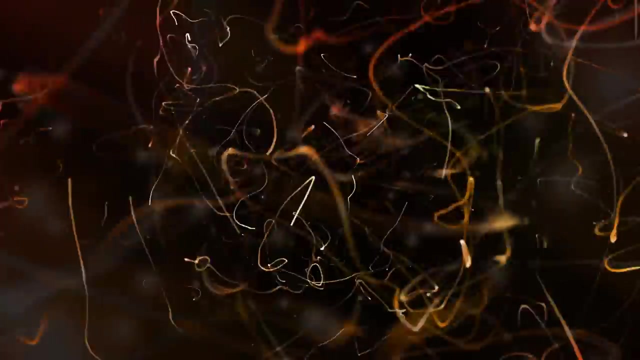 Similarly, the electro-weak force has little hold on the matter-energy balance and the matter-energy interactions. And while gravity may have pervaded the universe since its beginning, there is one major component still missing, which renders it all but powerless. Until these newly formed particles are granted mass, they remain unruly and ungoverned. 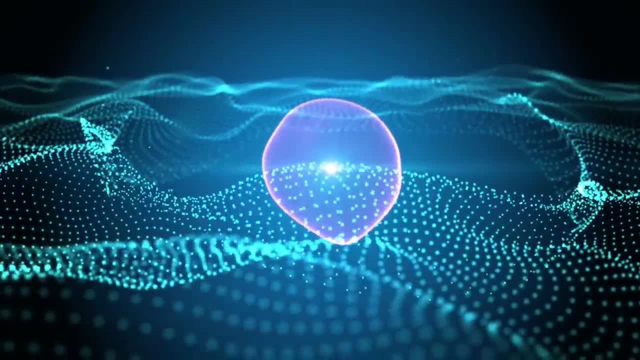 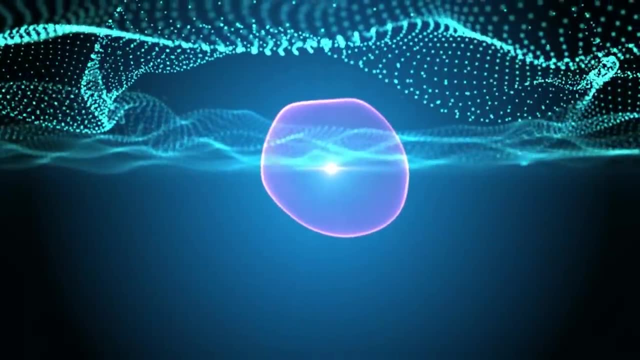 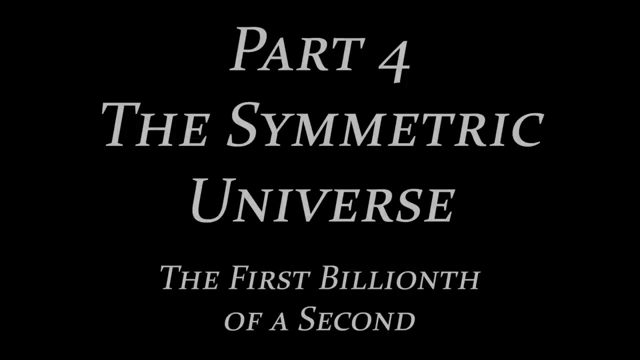 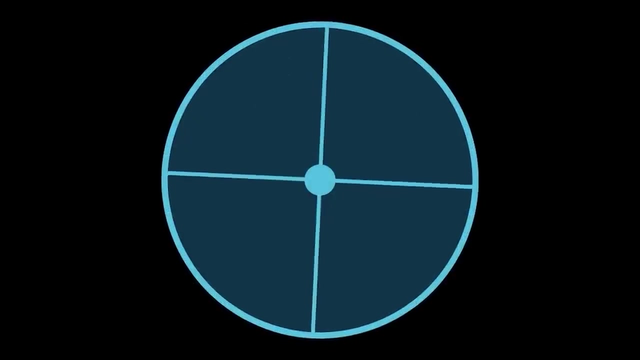 It will take another energy drop and another cosmological transformation before we reach a universe we begin to recognize as our own, And that's why we're here. Thanks for watching. Symmetry is everywhere. Anywhere we look in nature, we find balance, regularity and geometric harmony, be it in 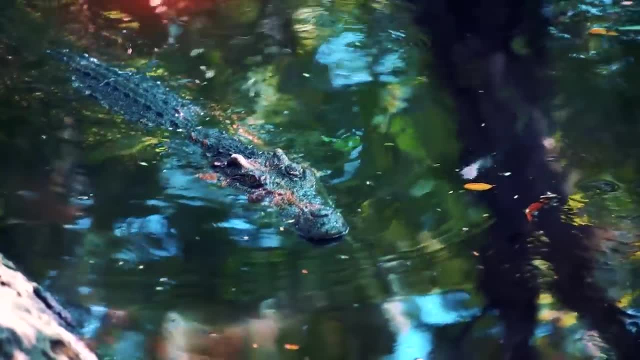 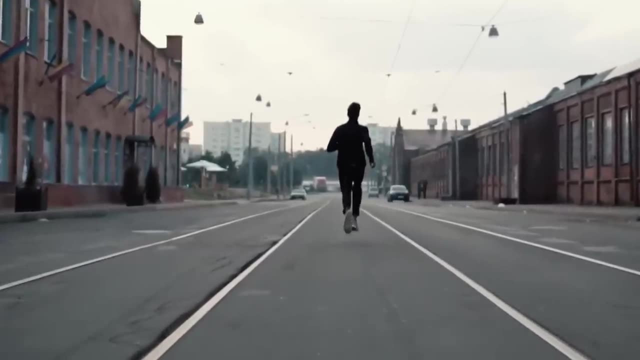 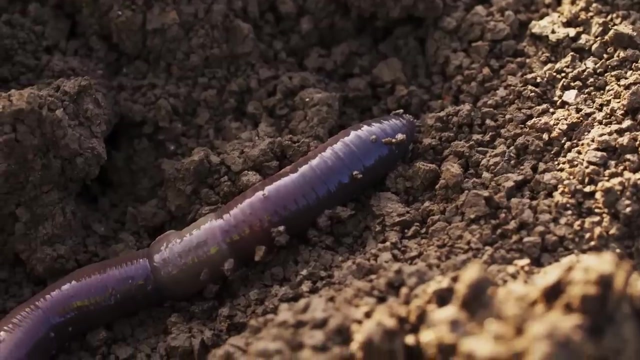 our own bodies, or the bodies of all animals, great and small. We are bilaterally symmetric, mirrored down the center, and perceive the greatest beauty in those whose symmetry is the most perfect. Many creatures share our bilateral symmetry too, from the greatest whale to the lowliest. 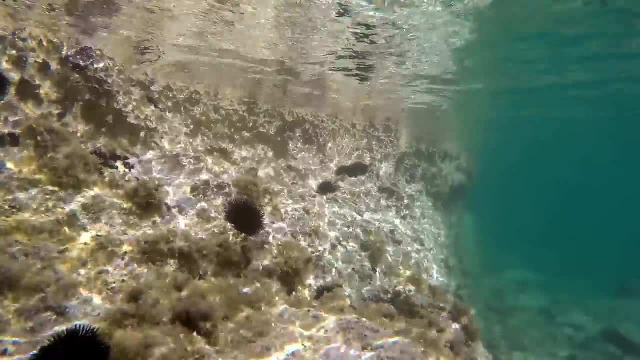 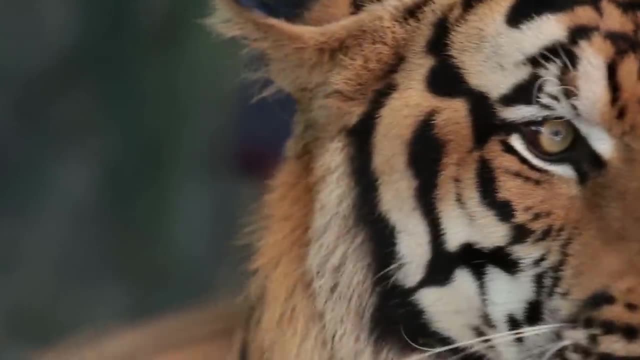 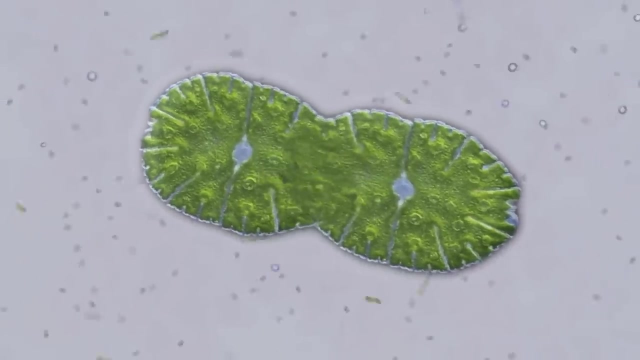 worm And, if not mirrored twofold, other animals like starfish and sea urchins, favor five spokes of radial symmetry. Scientists have found that evolution has a clear preference for these balanced, symmetric forms, not least because they are constructed from much more simplistic instructions than 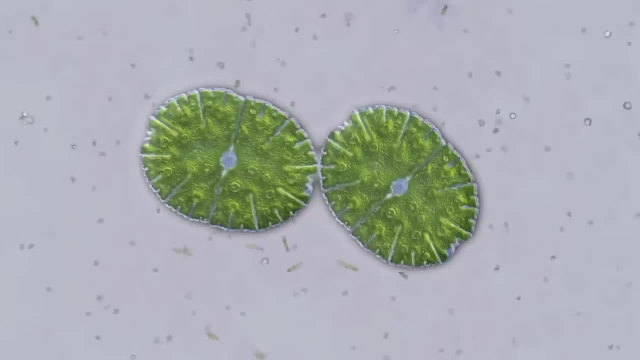 other more complex and non-repeating geometries, And it is mathematical, algorithmic simplicity that we are here to learn about. Make sure to subscribe to our channel and click on the bell. so very soon, and won't you be never-too-distant? 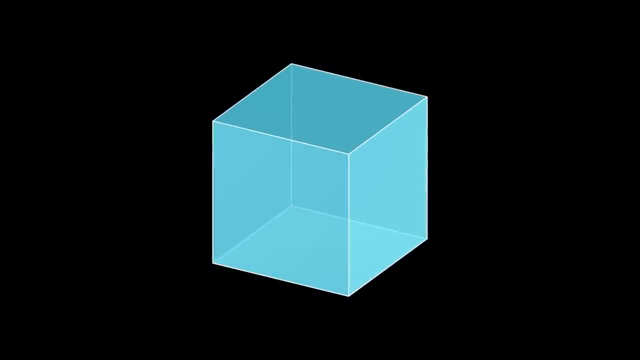 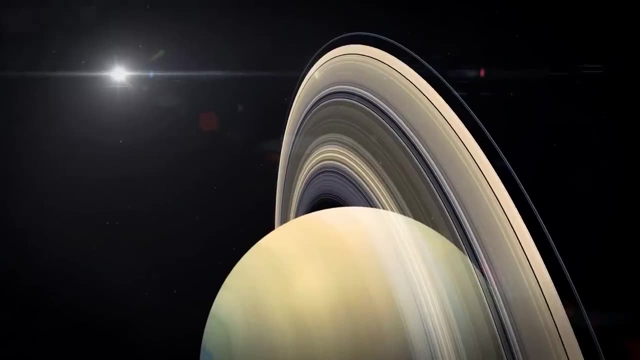 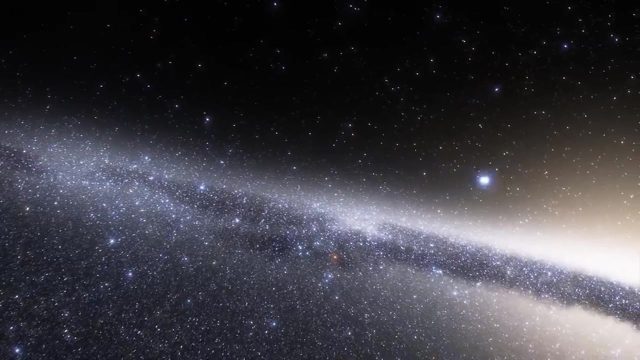 that underlies the symmetries found throughout the natural, non-living world. In science, symmetry has a much wider meaning than its day-to-day use. It indicates that something is the same, something that does not change whatever happens, From the laws of physics to the conservation of energy and momentum. 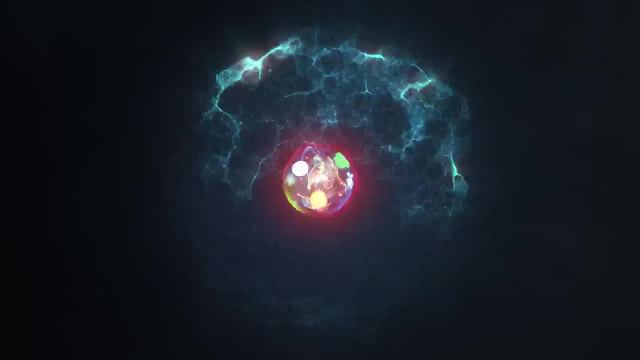 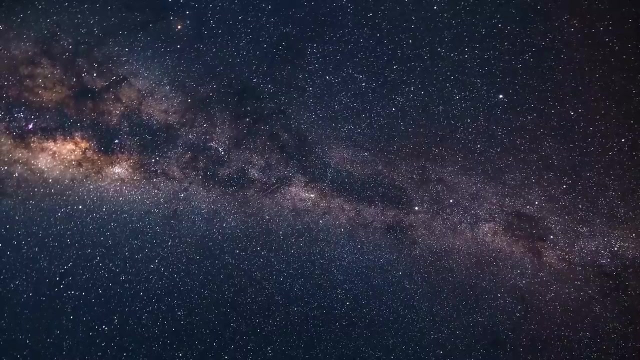 the universe is inherently symmetrical. Positive charges are balanced with negative ones. Some particles spin clockwise, others spin counterclockwise, And if you measure the strength of gravity on Alpha Centauri, you will get the same result as in our own solar system. 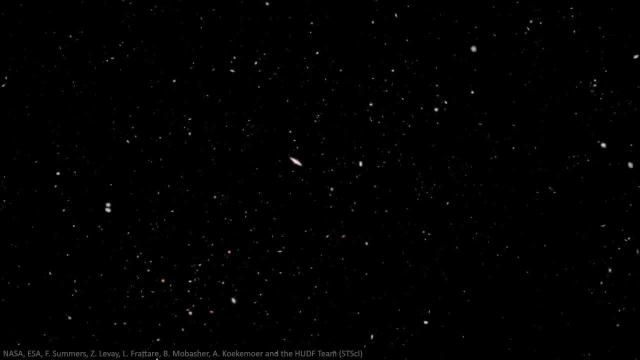 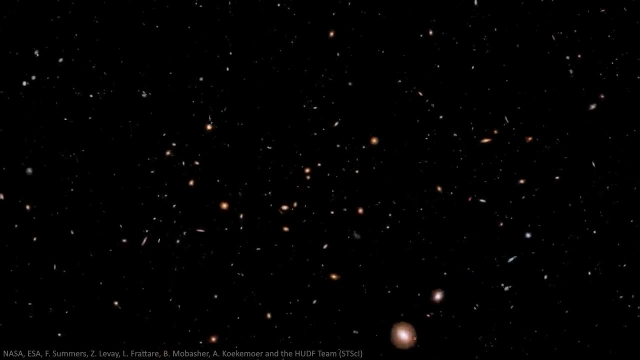 And yet the universe is not perfectly symmetrical. Just like the human body, when examined more closely, has the heart shifted to one side, there are also flaws in the perfect balance of the cosmos. There are some particles that never spin clockwise. 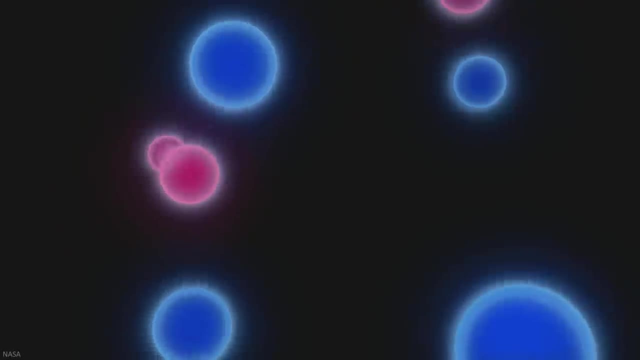 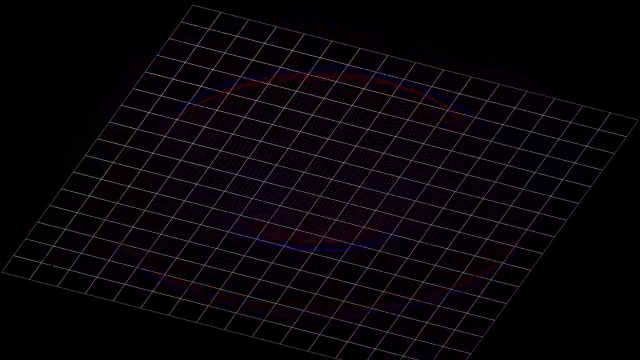 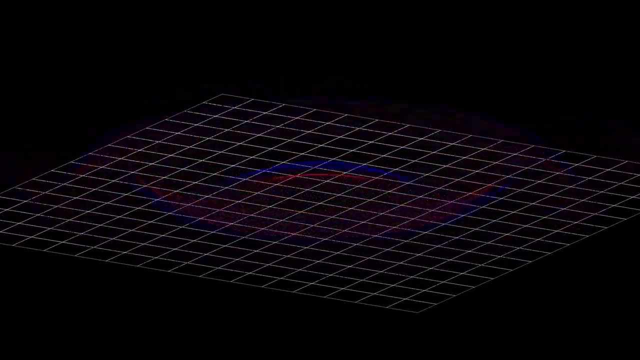 and others that never spin counterclockwise. There is an imbalance in the amount of matter and antimatter. There are things that electric fields can do that magnetic fields cannot, despite the two being notionally equivalent, And many of these imbalances are key to the functioning of reality. 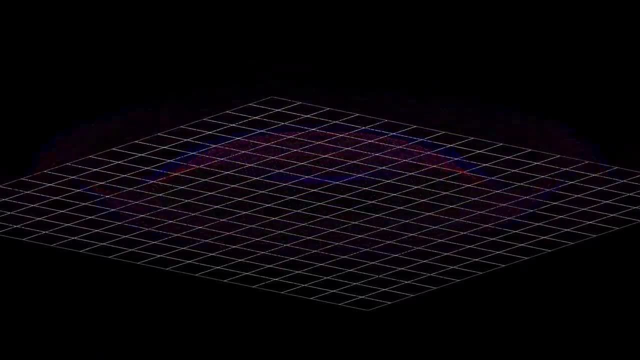 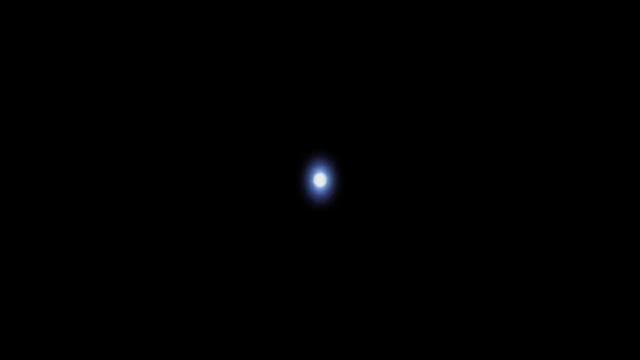 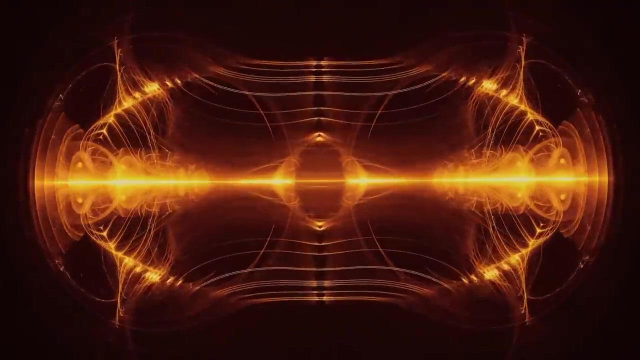 But it did not start this way. Indeed, for the first trillionth of a second or so, cosmologists believed that everything was perfectly symmetric, There was balance, But that all changed with the final separation of the force and the emergence of something that would come to influence much of existence. 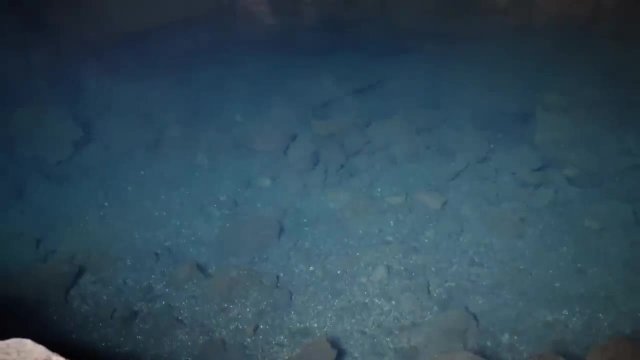 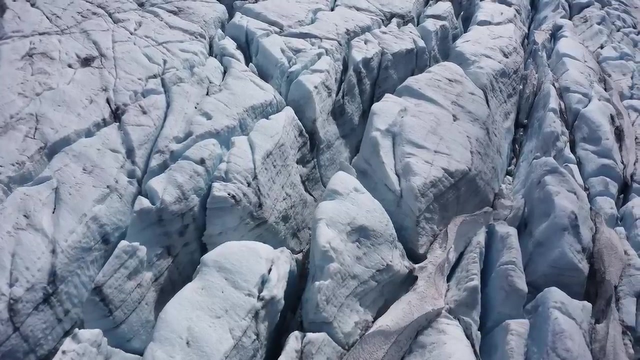 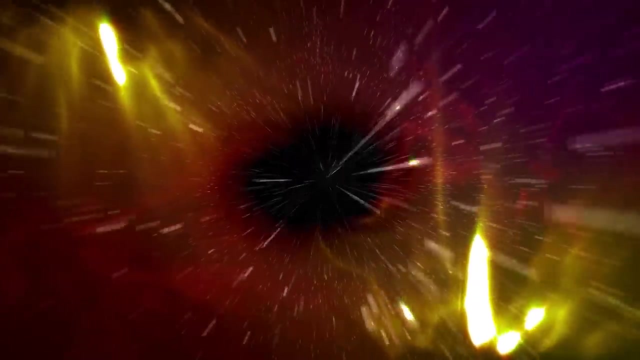 Mass. Just as dropping temperatures herald phase changes in water, from vapour to liquid to solid ice, fundamentally changing its properties at each transition and reducing its symmetry, so the dropping temperatures in the young cosmos brought about phase changes in the energy and matter that filled it. 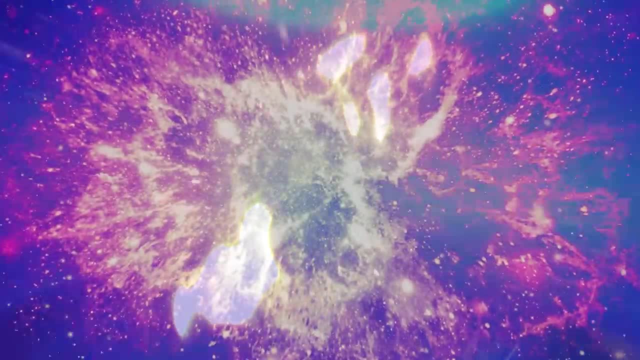 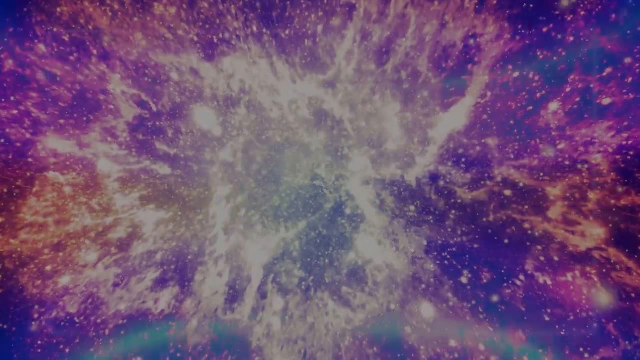 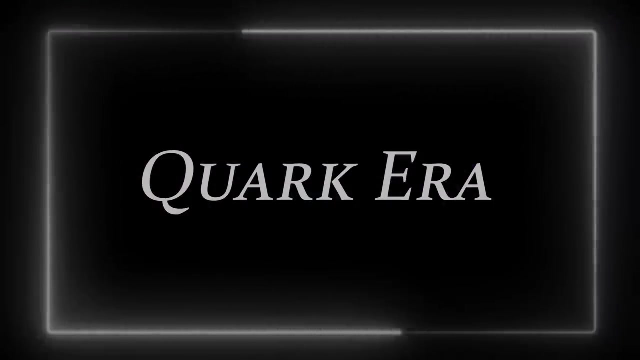 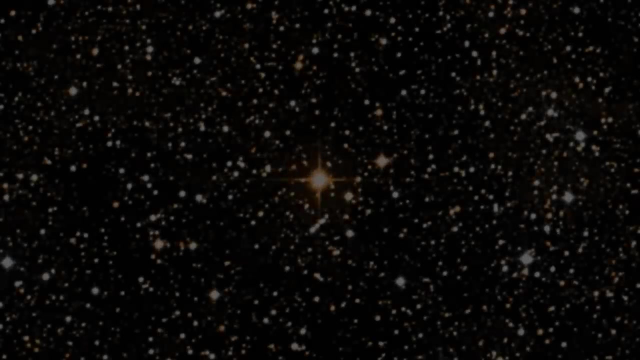 As the four fundamental forces finally fully split and crystallized as separate entities, a new era dawned, The quark era, defined for the first time by the interactions of matter. The biggest single object yet discovered in our universe is probably the hypergiant star. 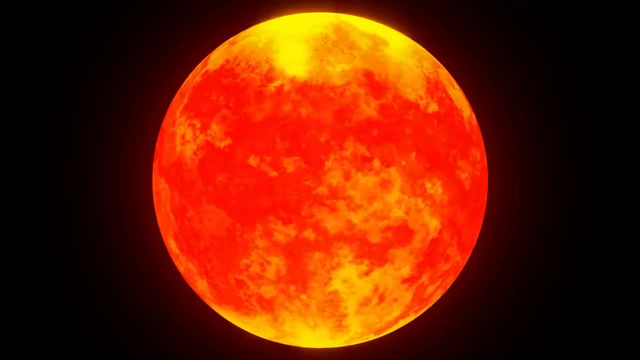 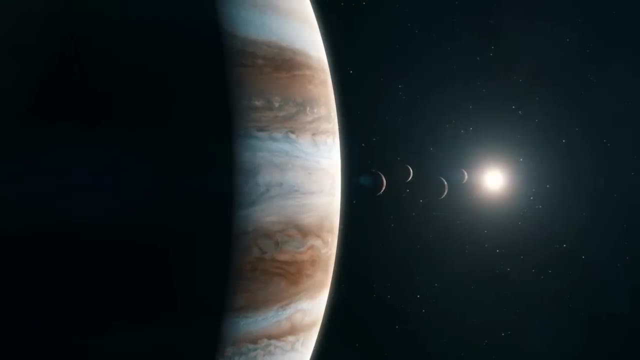 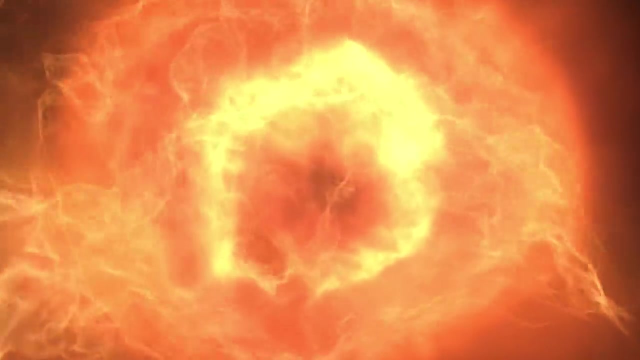 UY Scuti, With a diameter some 1700 times larger than our sun. if it sat at the center of the universe, its outer edge would sit just beyond the orbit of Jupiter. And yet it, like all stars, is composed almost entirely of some of the smallest things to be found in the universe. 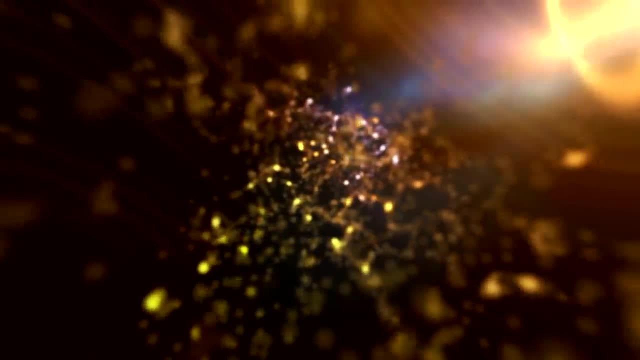 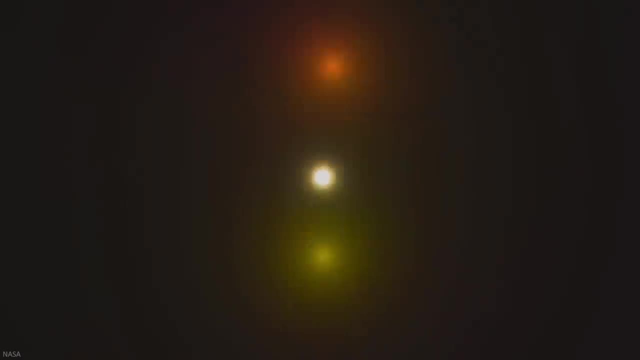 Individual atoms of the lightweight elements hydrogen and helium. Hydrogen is the smallest of the atoms, which themselves were once considered the smallest thing possible. Their very name derives from the Greek word for unsplittable, But we now know thanks to revolutions. 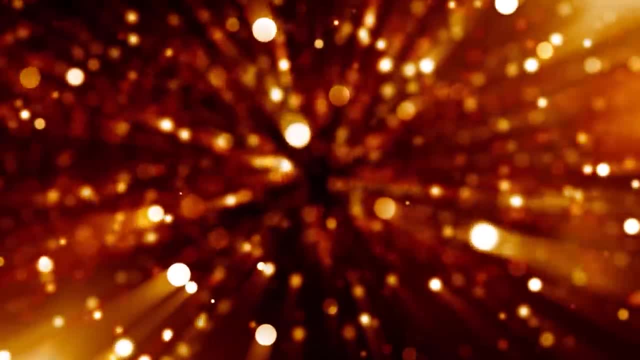 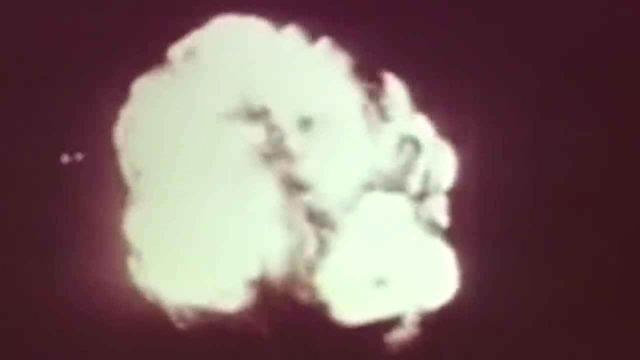 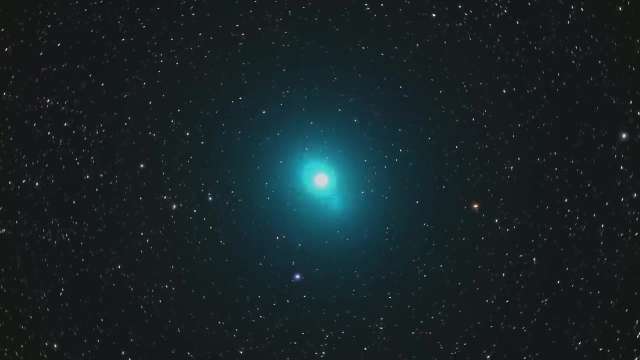 and atomic theory throughout the early 20th century that atoms are eminently splittable, a fact which has given rise to some of the most devastating weapons in human history. Hydrogen and helium, for all their simplicity, are composite particles of protons, neutrons and electrons. 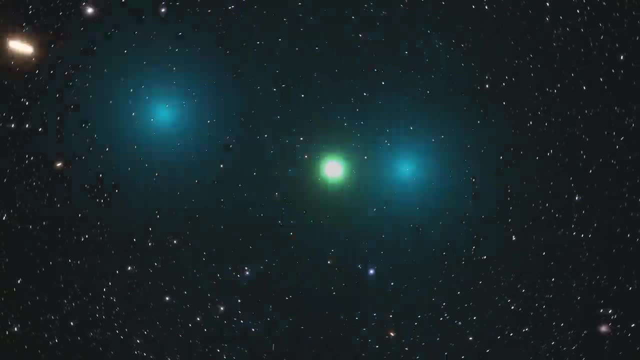 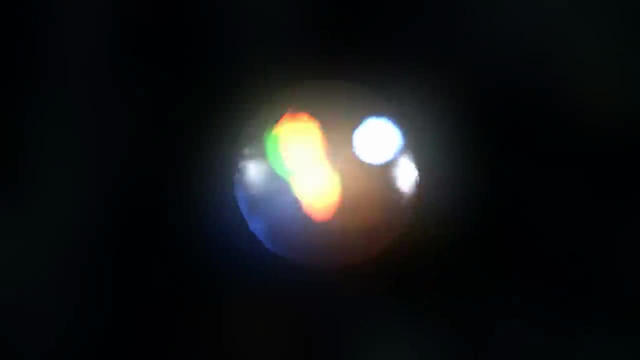 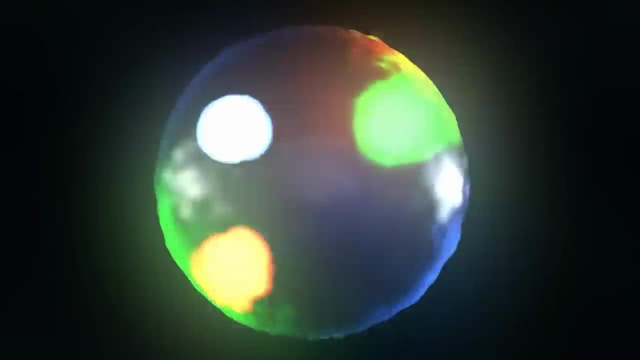 which can be isolated and manipulated with relative ease. But even these are not the smallest fundamental particles. there are Protons, and neutrons are themselves composites of even smaller units called quarks, whose various properties, alongside those of electrons, ultimately govern the characteristics and behavior of everything, including 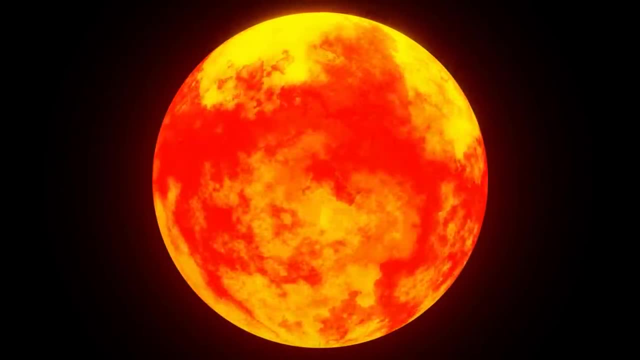 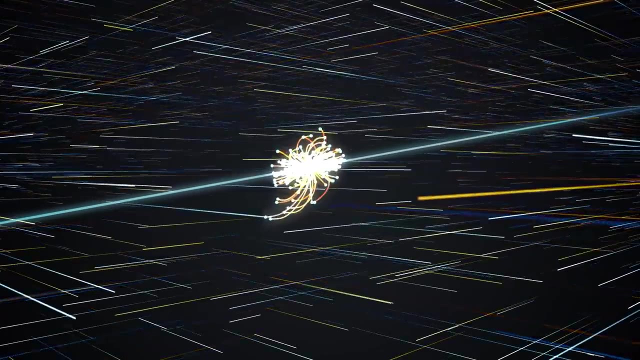 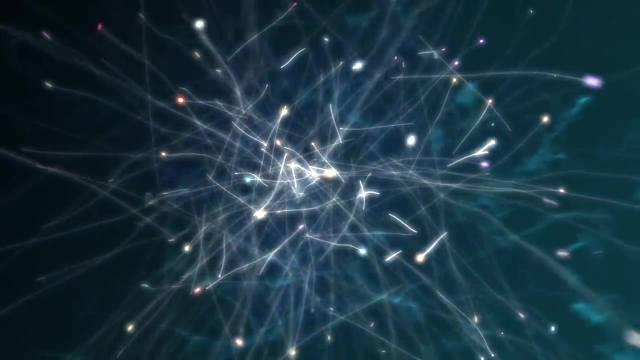 UY Scuti. The search for the fundamental particles of matter has been a guiding quest for physicists for some 200 years. Experiments to crack open smaller and smaller particles, to reveal what lies inside, require vast amounts of energy, which can only be obtained by accelerating those particles. 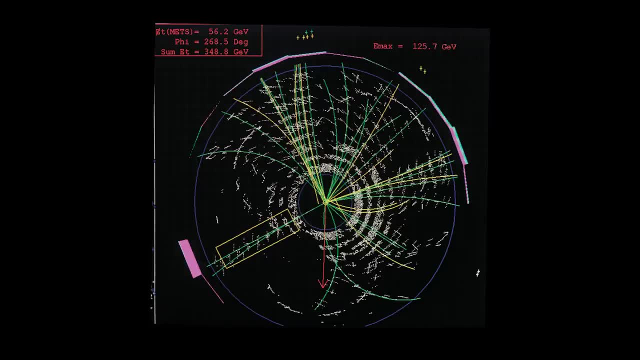 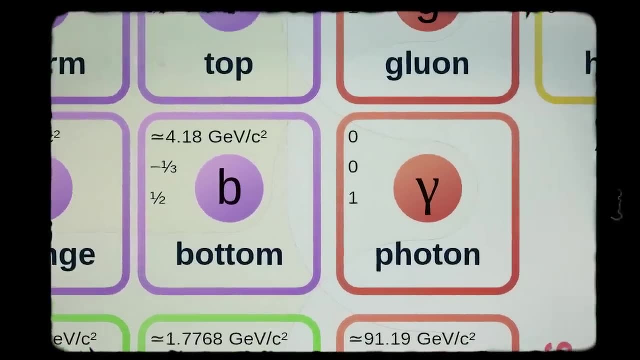 to blinding speeds and then smashing them into one another in particle colliders. Examining the wreckage of such collisions, we can piece together a full picture of the building blocks of our universe, This picture, which has come to be known as the standard model of particle physics. 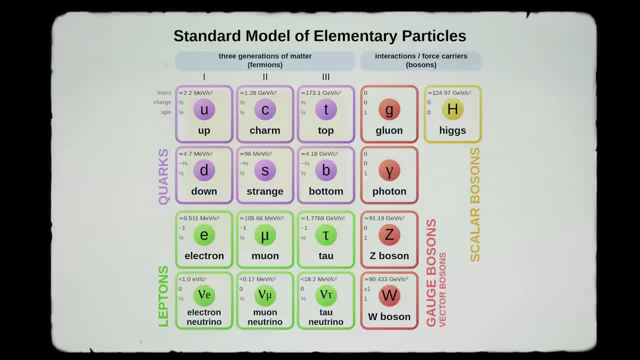 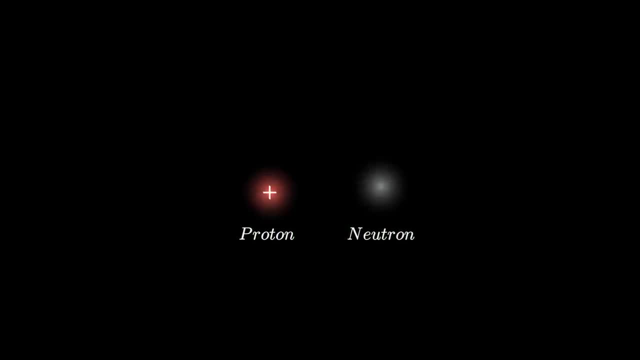 is theoretically all we need to explain why everything looks the way it does in the cosmos today. Normal matter, as we have seen, is composed of protons and neutrons, which are collectively known as hadrons, But they are themselves composed of a combination of quarks, each with distinct 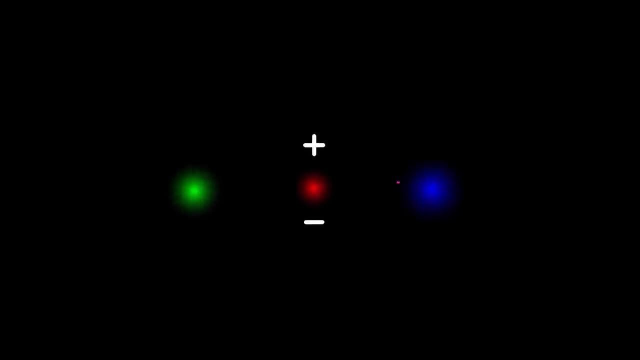 characteristics such as mass charge, spin, as well as another property called colour, an arbitrary name which has no relation to colour but helps to explain how they bind together in groups. A positively charged proton is made from two up quarks and one down quark. 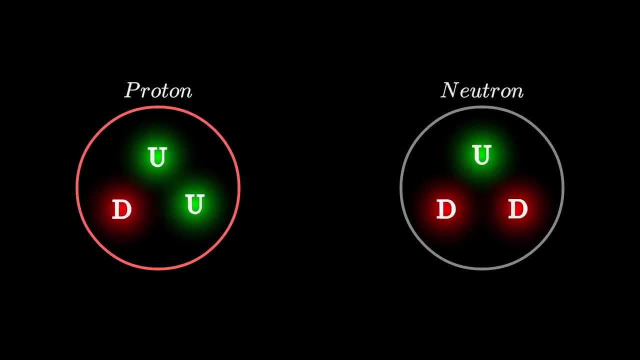 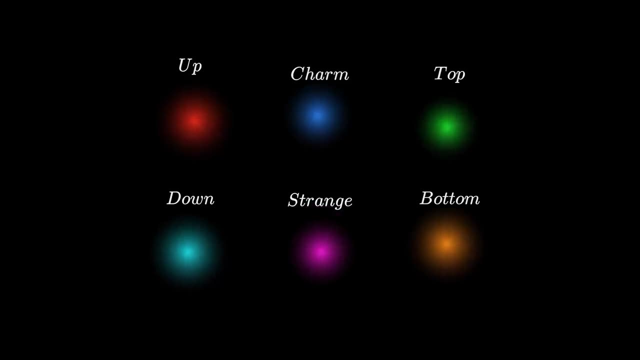 while an uncharged neutron is made from two downs and an up. But there are other flavours of quark out there with esoteric names like Strange Charm, Top and Bottom which combine to form more exotic composite hadron particles which are scarcely ever seen outside of physics experiments. 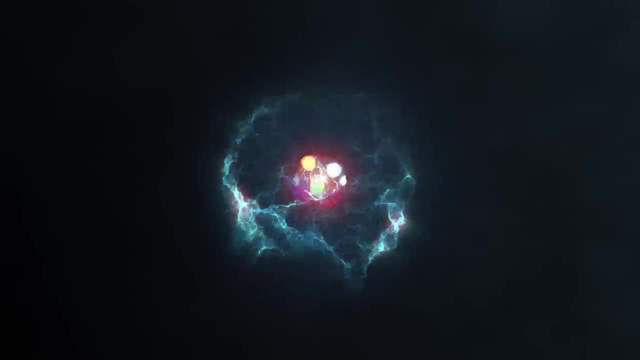 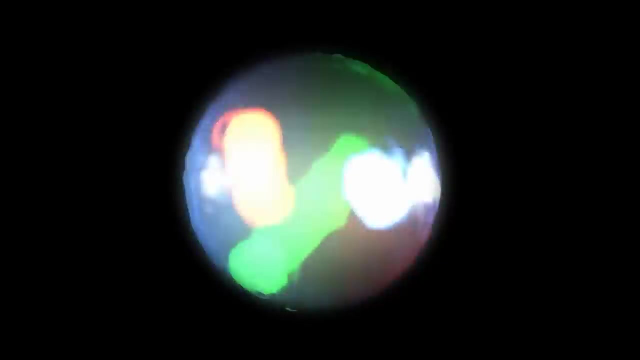 And so, despite smashing hadrons together in these experiments with ever increasing force, physicists have found no hint that quarks are made of anything smaller. They truly seem to be the bottom of the rabbit hole. Meanwhile, the electrons that orbit atomic nuclei appear similarly indivisible. 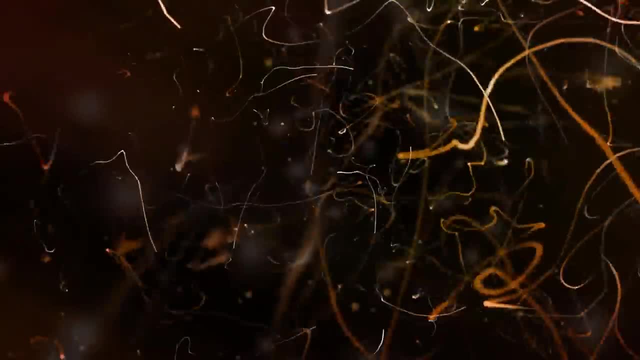 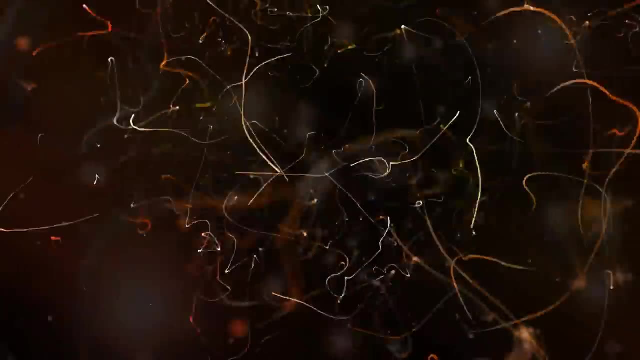 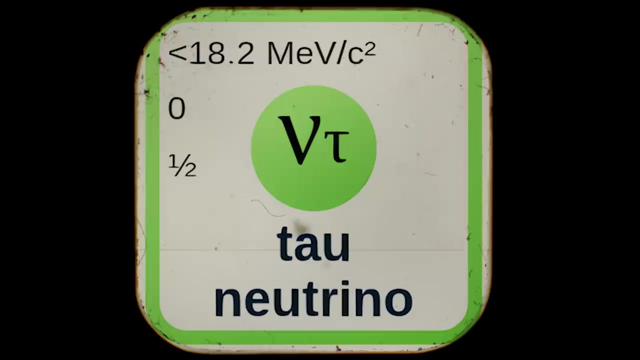 They are a kind of particle known as a lepton, And while all normal matter makes do with the negatively charged electron, there are exotic varieties to be found inside our colliders. Muons, tau, leptons and several varieties of neutrino can all be found in the wreckage of particle collision. 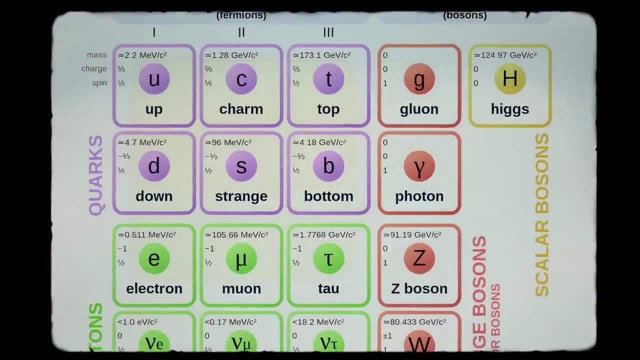 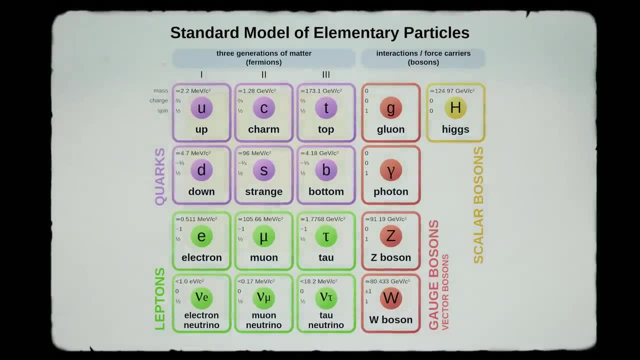 And so our standard model consists of 12 fundamental unsplittable particles of matter, six types of quark and six types of lepton, in addition to antimatter counterparts of each of these and the messenger particles of the fundamental forces: Photons for the electromagnetic force, gluons for the strong nuclear force. 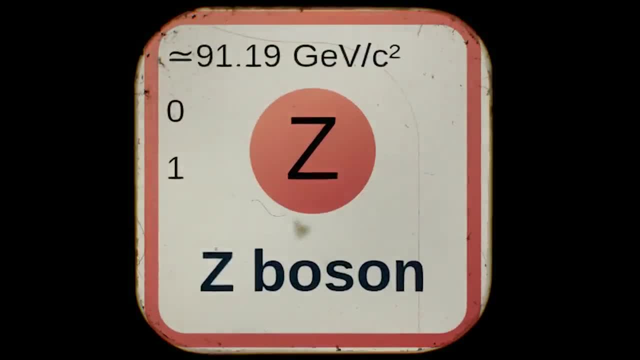 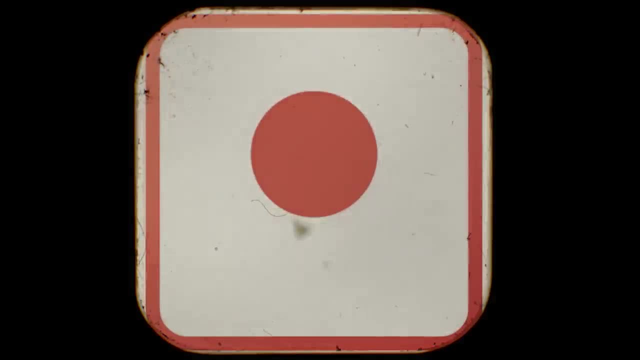 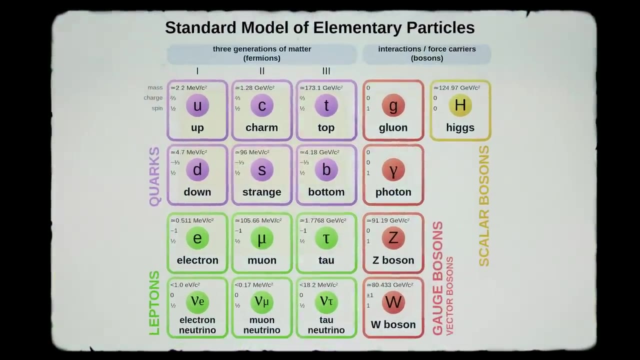 and W and Z bosons for the weak nuclear force. If a virtual particle exists to communicate gravity through spacetime, then it still evades detection. So for now only four gauge bosons join the particles of matter to describe everything within the universe today. 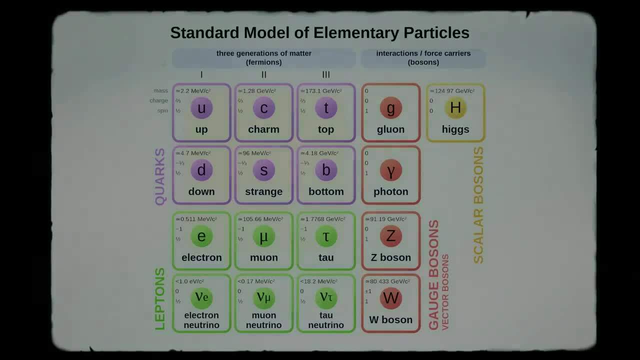 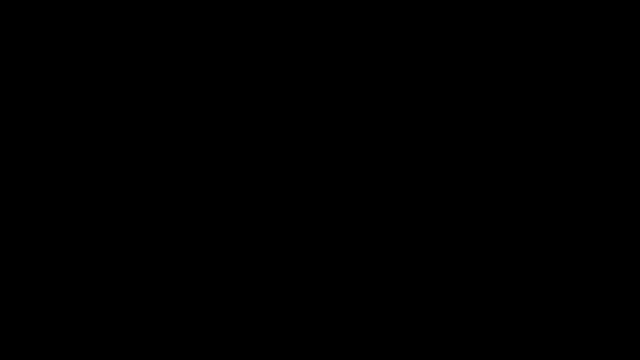 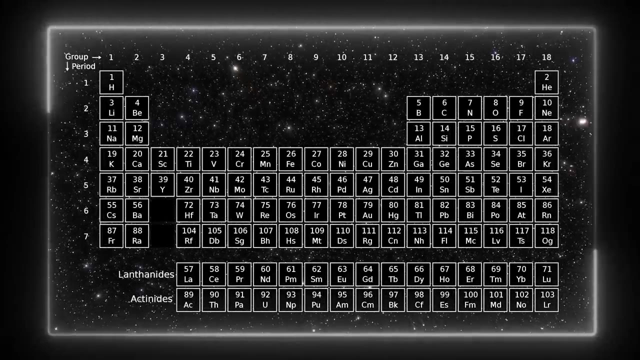 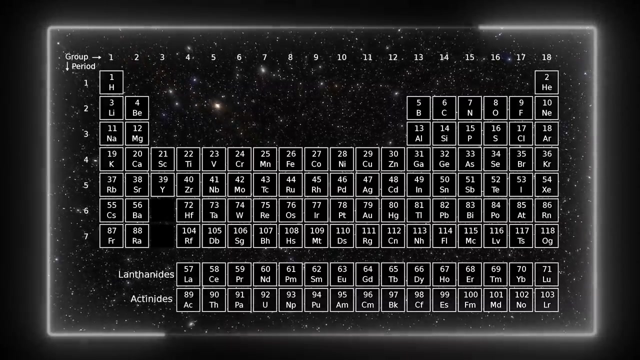 At least almost everything. There is one crucial missing piece to our model so far, and that is mass. Every element in the universe, from hydrogen to plutonium, has its own characteristic mass, corresponding mainly to the number of protons and neutrons within its nucleus. 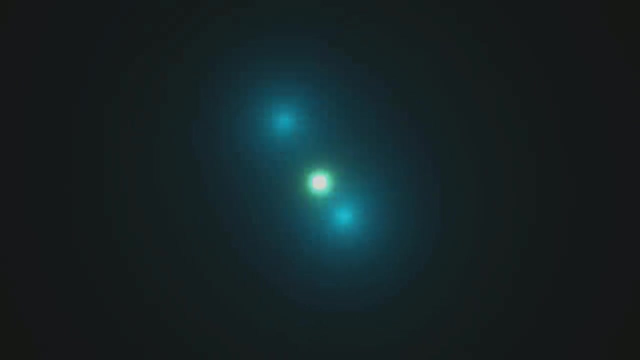 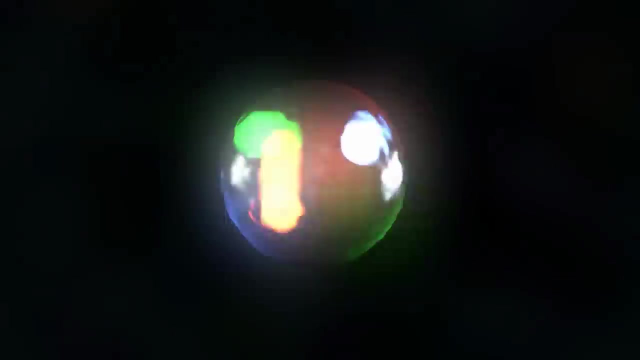 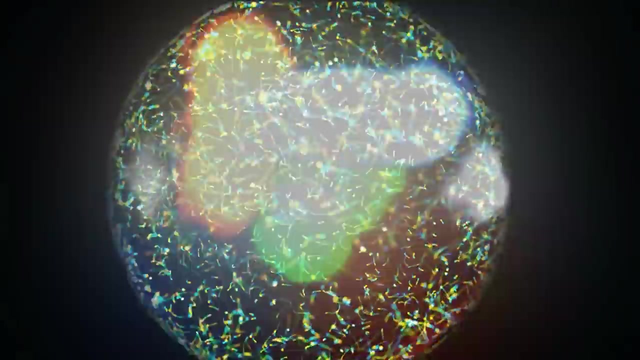 So it follows that the majority of an atom's mass comes from those protons and neutrons. But when we peer down smaller and smaller to find the ultimate source of that mass, that is not what we see, For it turns out that a proton weighs in at considerably more than the sum of its parts. 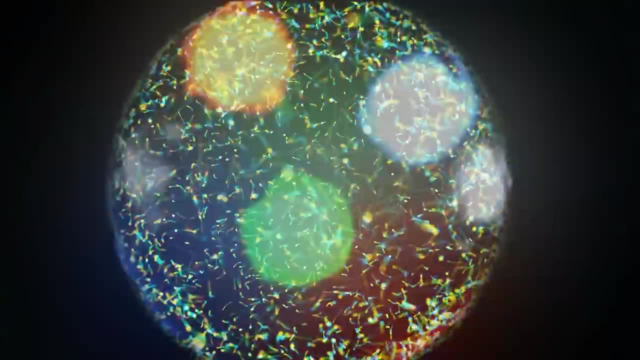 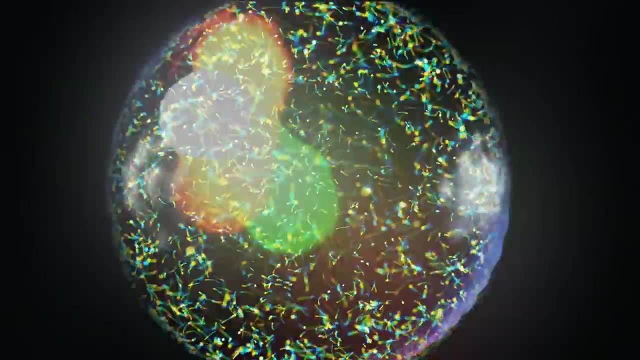 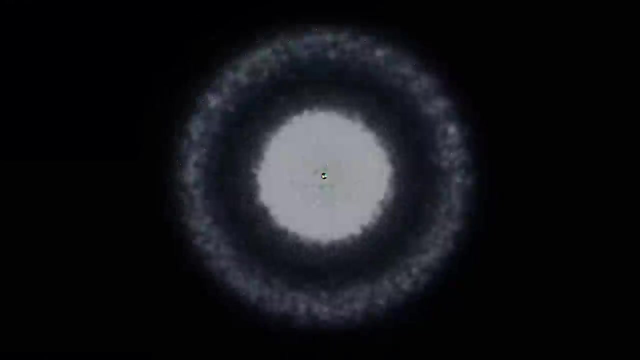 The fundamental particles at the heart of a proton are the three quarks, But the masses of these amount to just nine percent of the proton's overall mass. The rest comes from energy stored up inside that nucleus, from the intrinsic relationship between energy and mass that Einstein identified. 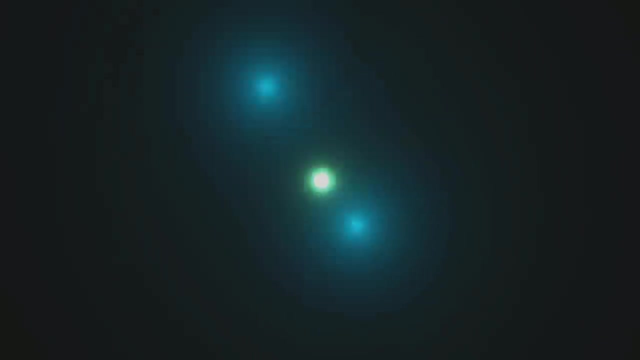 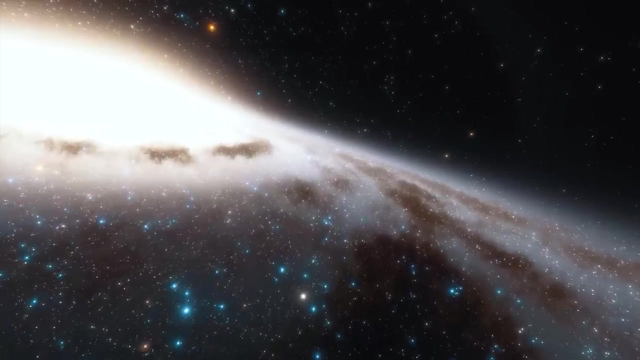 with his famed E equals MC squared equation, and from the bizarre quantum interactions of gluons, the mediators of the strong nuclear force. So when we reconsider the masses of every piece of normal matter in the universe, more than 90 percent of it doesn't actually. 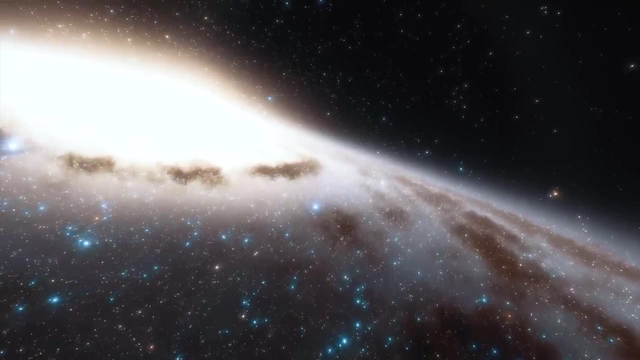 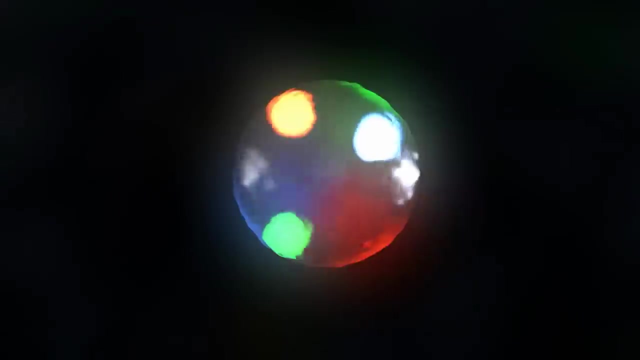 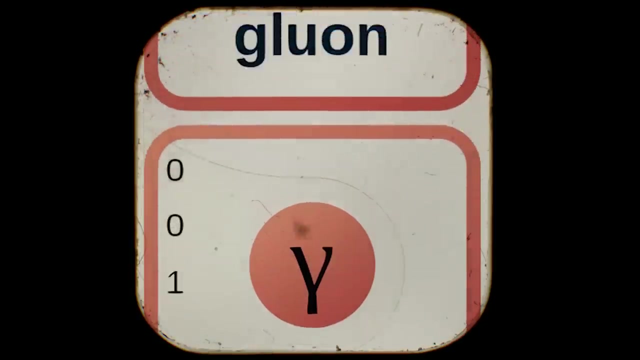 come from the stuff of matter at all, but from the latent energy and empty space within. But quarks do still have mass, something separate, something different to this energy, and the reason for this was a mystery for a long time. Photons and gluons get by just fine without mass at all. 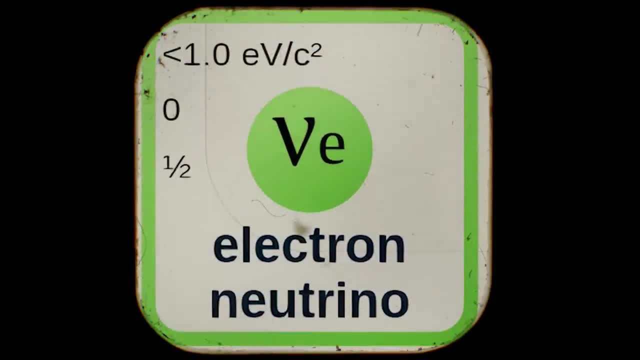 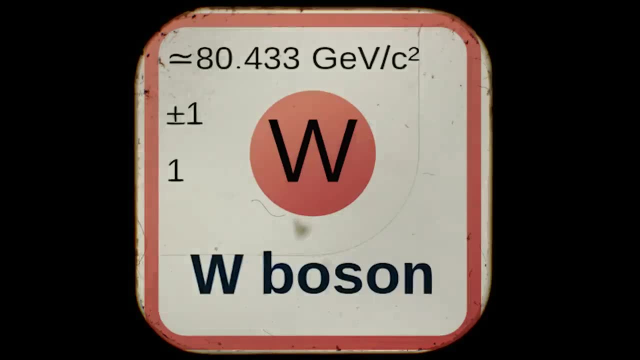 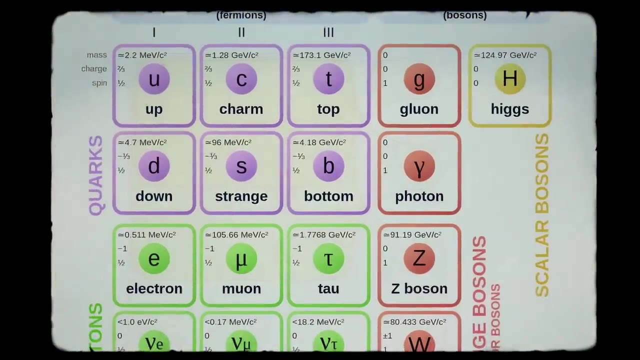 Electrons and neutrinos have even less than the smallest quark, while the W boson carrier force weighs in at some forty thousand times heavier than an up quark, heavier even than an entire iron atom. So what causes this incredible disparity in mass? 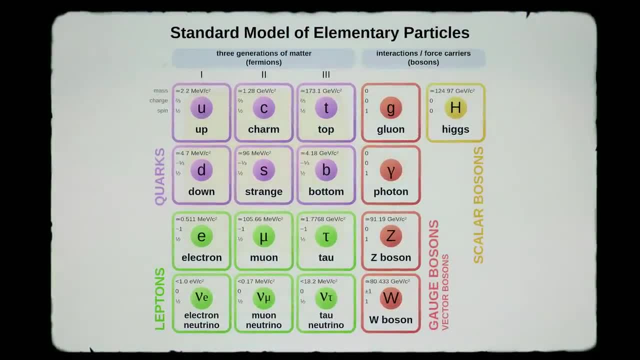 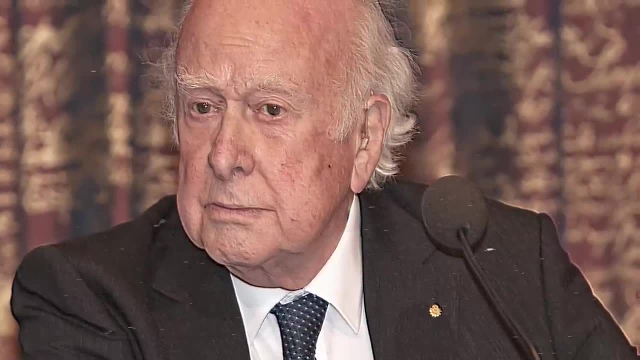 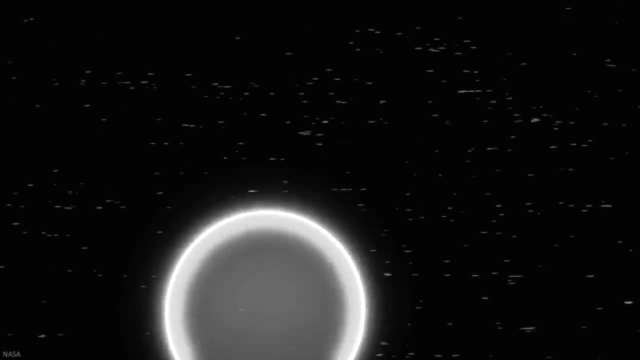 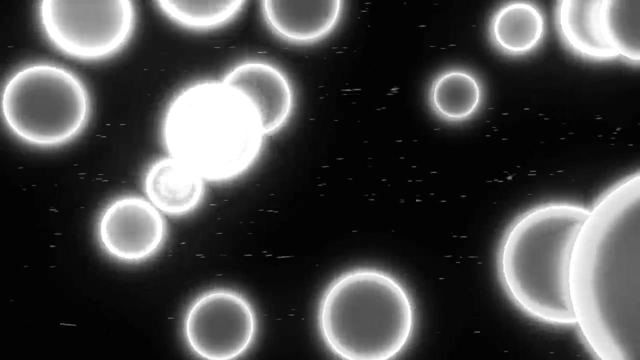 And why do particles have mass at all? This was the question that plagued British theoretical physicist Peter Higgs in the 1960s, while teaching and researching at the University of Edinburgh. as a solution to the problem, he suggested that all particles first came to existence in the universe without any mass at all. 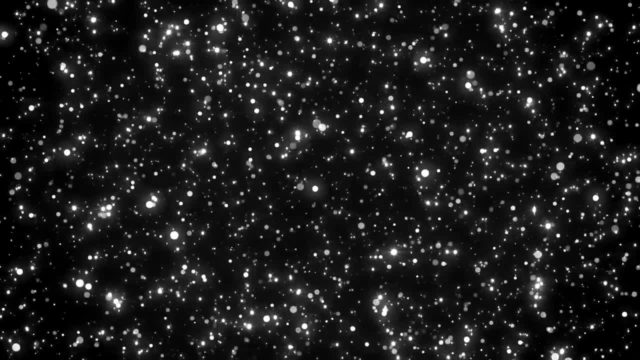 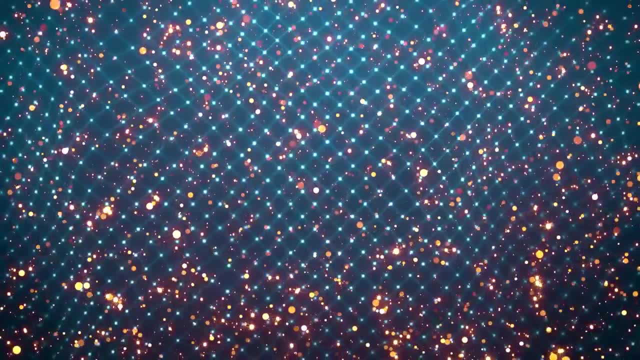 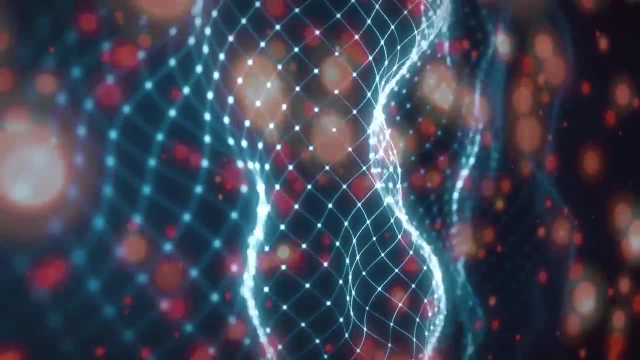 and that, at some point within the first split second, a new kind of energy field emerged and permeated all of spacetime, giving the various particles the property of mass. This Higgs field, as it became known, would be communicated by its own quantized messenger. 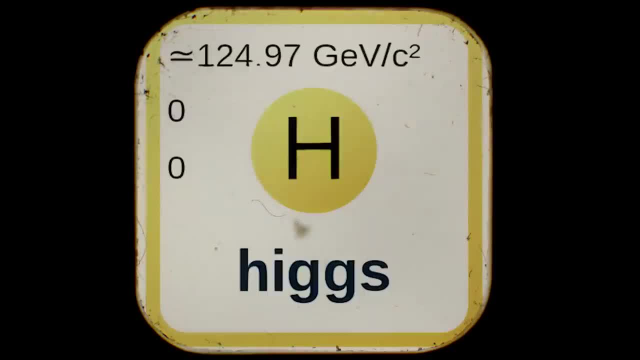 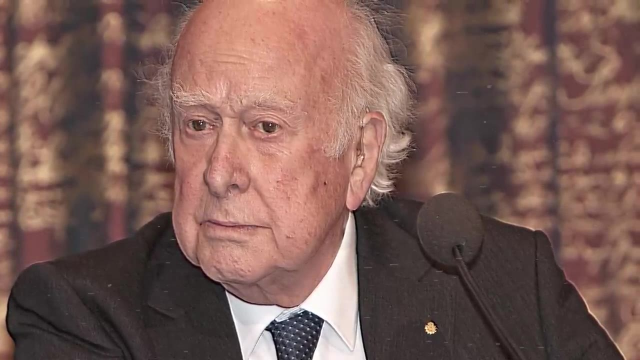 particle, the Higgs boson, which would sit alongside the other 16 particles of the standard model and play a major role in describing the behaviours and interactions of matter in the universe. And yet, even though Higgs theory was sound, it would take nearly 50 years to finally find the elusive Higgs boson. 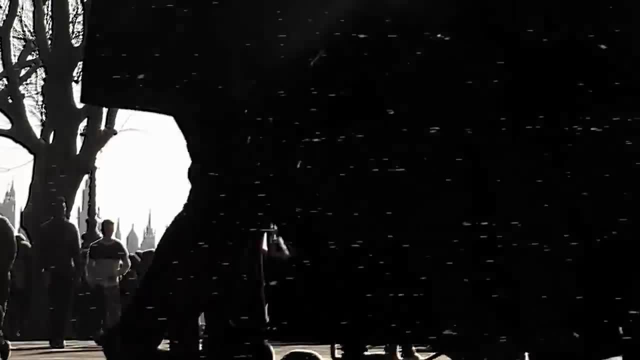 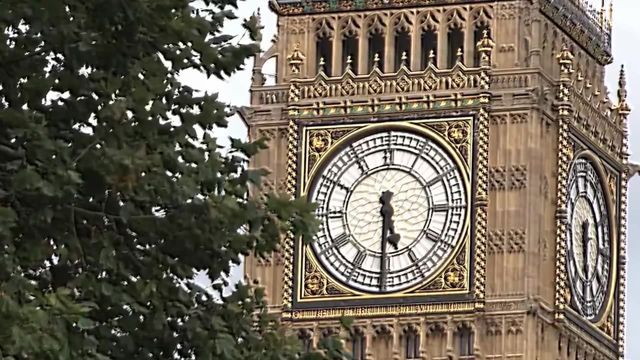 In the meantime, in order to bolster support for this expensive and seemingly esoteric search, the UK Minister for Science promised in 1993 to buy a bottle of champagne for the best analogy to explain the actions and importance of the Higgs field to the general public. 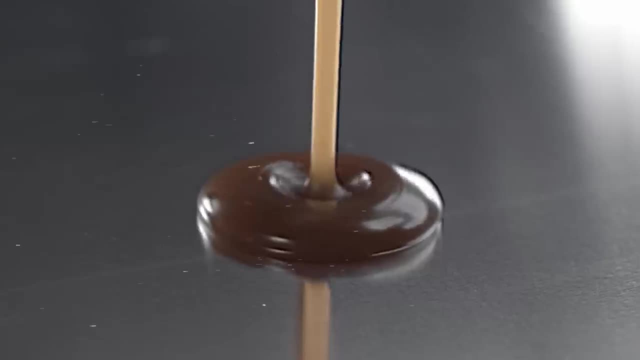 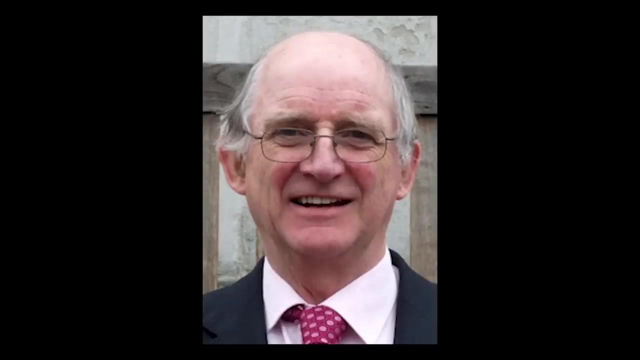 Despite various suggestions featuring pools of syrup, prisms and electric fields, it was physicist David Miller from University College London who ultimately claimed the prize with a description that focused on a busy cocktail party. At this party, he said, everyone is happily chatting among themselves. 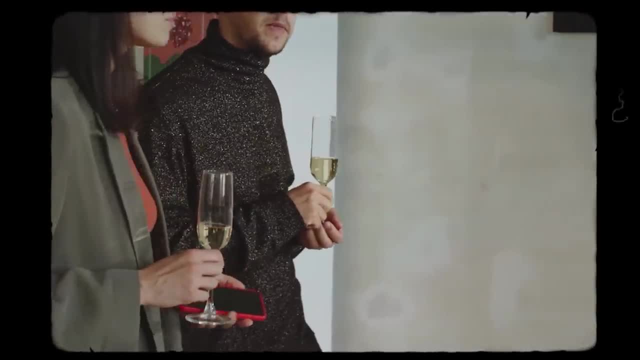 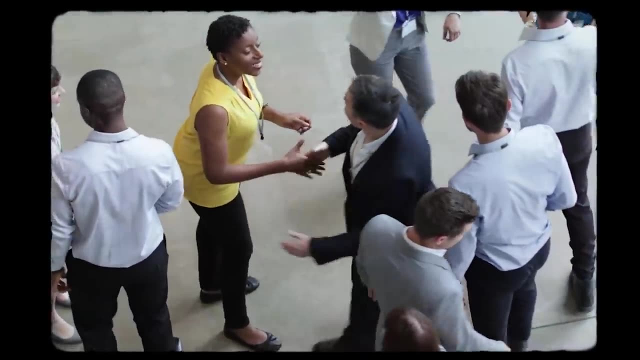 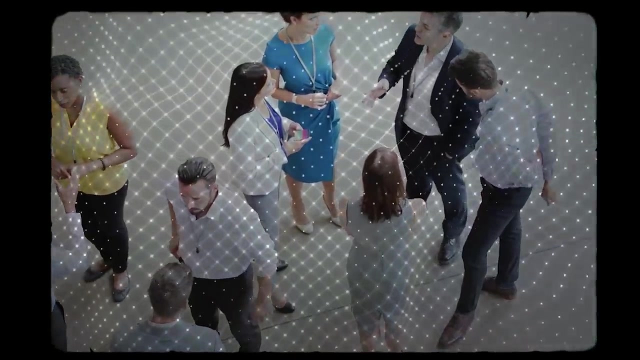 and a normal person is able to move through the room with relative ease. But when a more popular figure enters the room, they attract attention from the partygoers. Everyone wants to talk to them and their progress through the room is slowed In this way. the room full of partygoers represents the Higgs field. 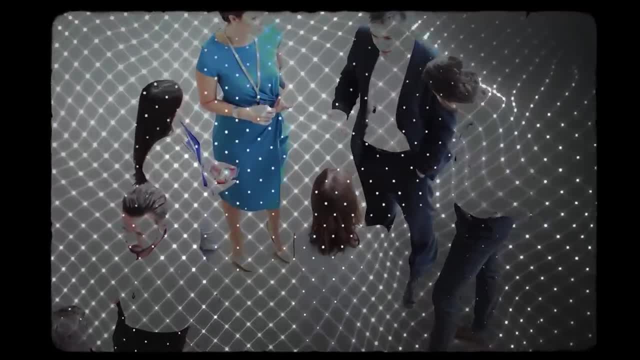 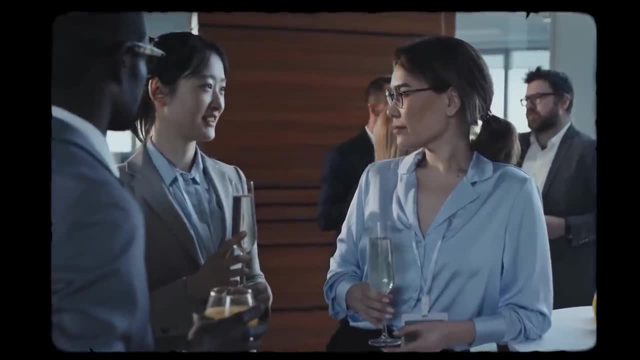 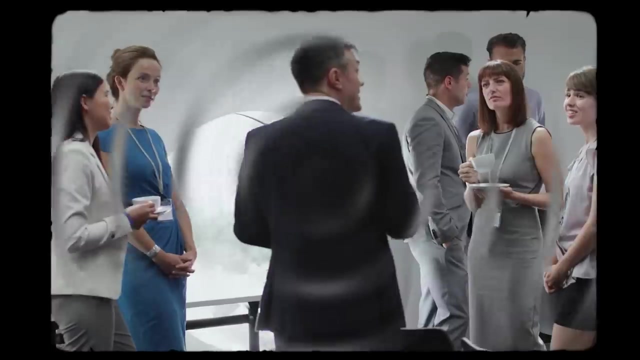 and the popular figure is a particle that has been imbued with mass. For those too far away to see the influential person, a rumour passes around the room as people come together to discuss their arrival. This physical rippling through the crowd can be thought of as the messenger Higgs boson. 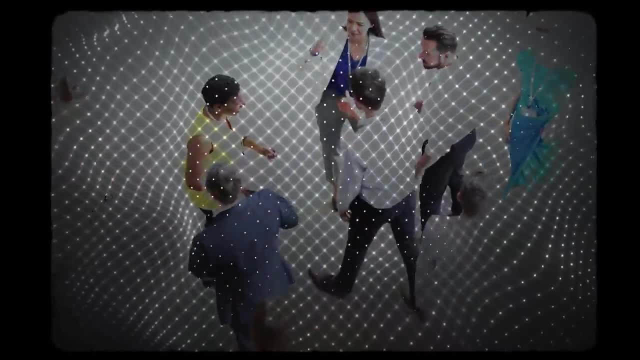 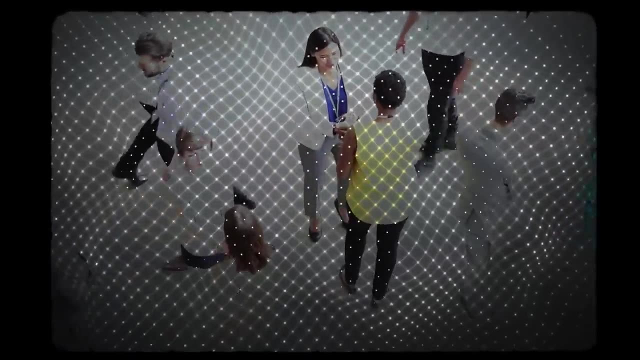 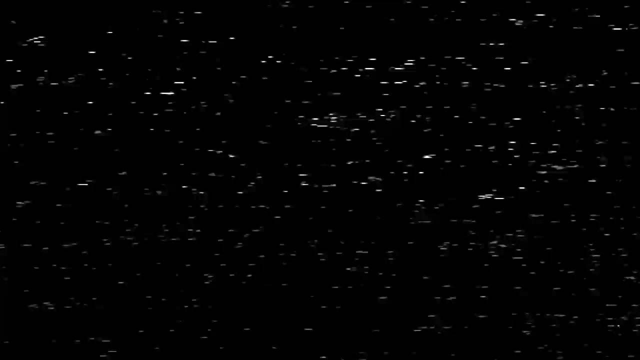 While the analogy isn't perfect, it has stood the test of time, And time was what was needed in what ultimately proved to be a frustrating search for something akin to a needle in a haystack. Two of the most powerful particle accelerators: the Tevatron at Fermilab in America and the Large Hadron Collider at CERN in Europe. 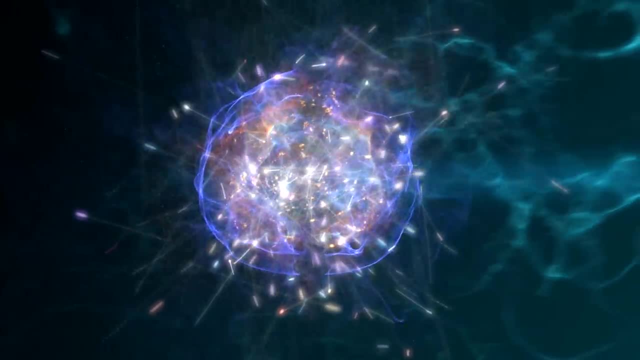 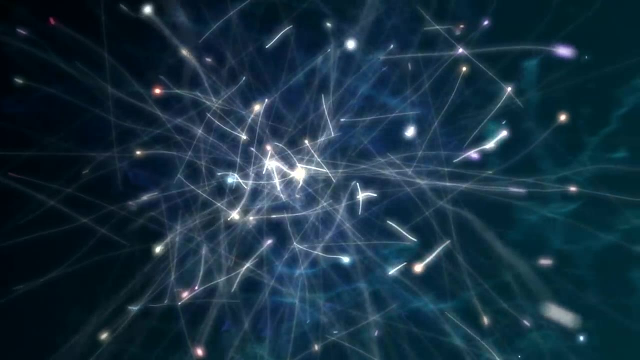 smashed particles that searched wreckage for years. The problem was, although Peter Higgs had theorised the field and boson existed, his theories said nothing about what energies would be needed to manifest them or the properties of the particles once they were found. 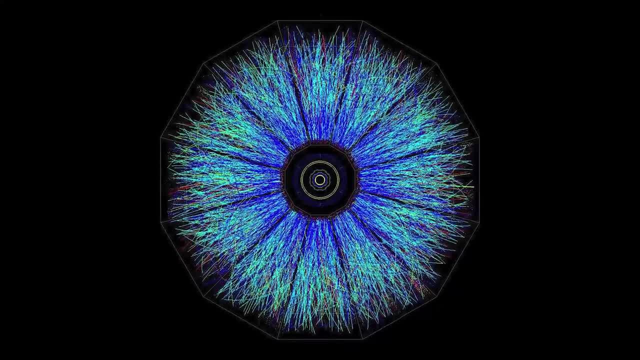 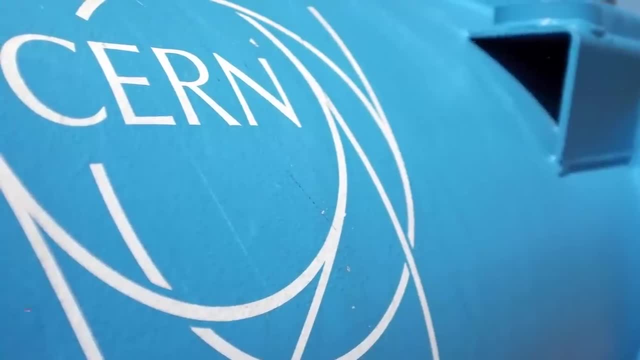 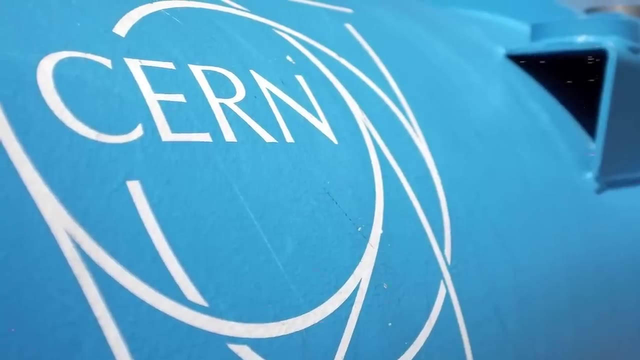 So like searching for a needle in a haystack when you had no idea what a needle even looked like. Eventually, though, in 2012,, experiments at the Large Hadron Collider achieved this seemingly impossible feat. Scientists confirmed they had in fact found the Higgs boson. 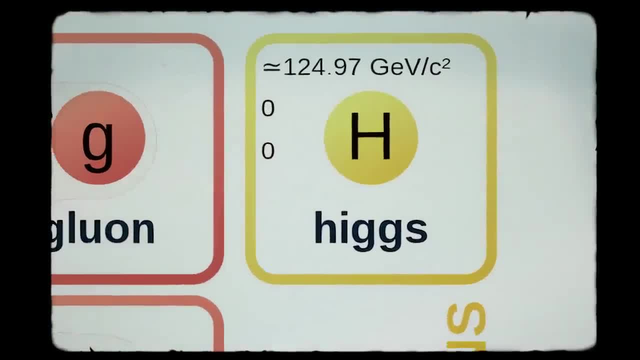 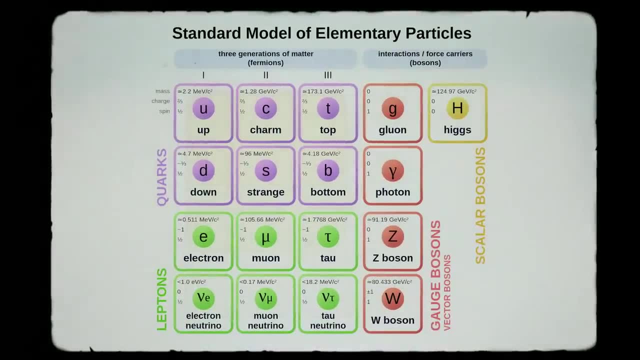 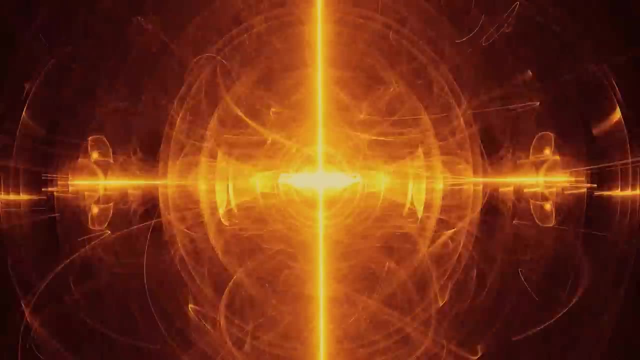 and in doing so proved the existence and action of the Higgs field once and for all. The particle had earned its place in the standard model and the field its role in the evolution of the early universe, A trillionth of a second after the Big Bang. 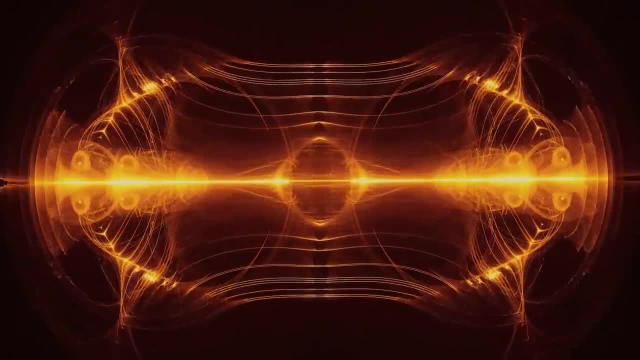 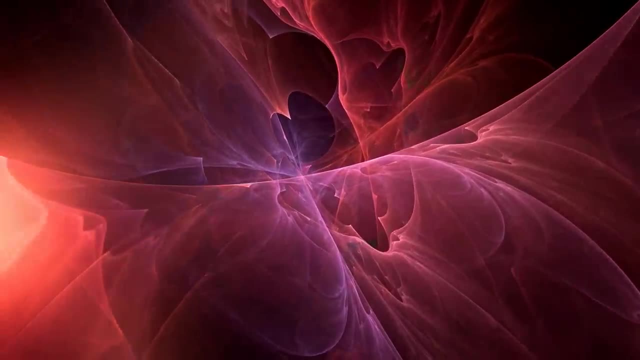 the electroweak force splits catastrophically in two, ending the perfect symmetry of the universe, as the W and B bosons that carry it decay into the photons of the electromagnetic force and the W and Z bosons of the weak nuclear force. 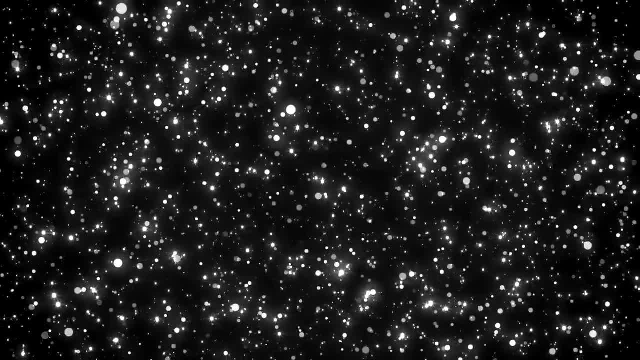 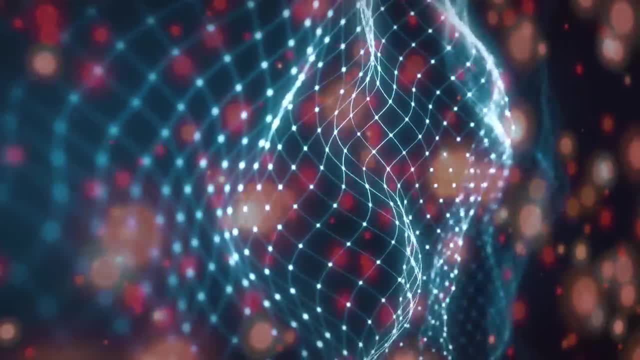 But this is only the beginning of the symmetry breaking. The emergence of the Higgs field around this time imbues the real and virtual particles that were created spontaneously during inflation and electroweak splitting. with mass, The W and Z bosons become heavyweights. 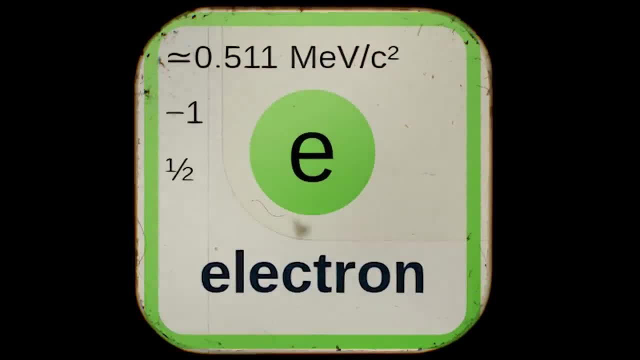 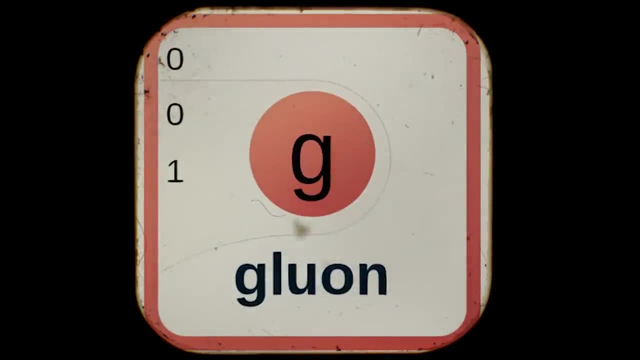 The quarks and leptons get their masses according to their flavour and type, While the photon and gluon continue as massless and unbounded by the Higgs, as they did before, As the quark era becomes fully realised by a billionth of a second after the Big Bang. 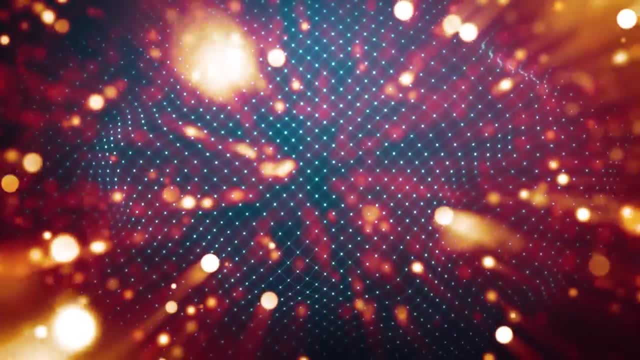 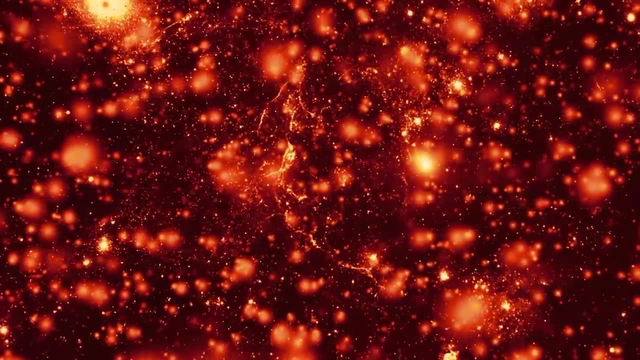 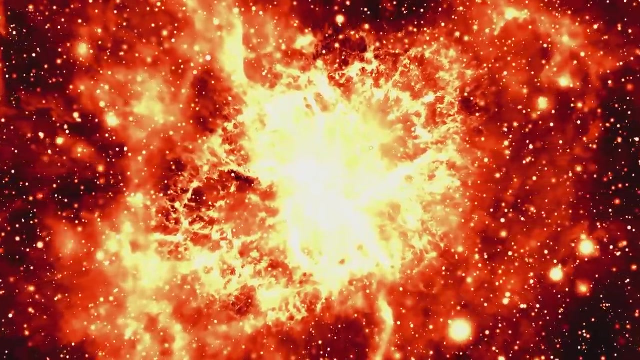 the universe is finally filled with all of the ingredients, the characteristic particles and the characteristic forces needed to make stars, planets and us. The quark gluon plasma that permeates the inflated cosmos is the primordial soup from which all structures in the universe will be made. 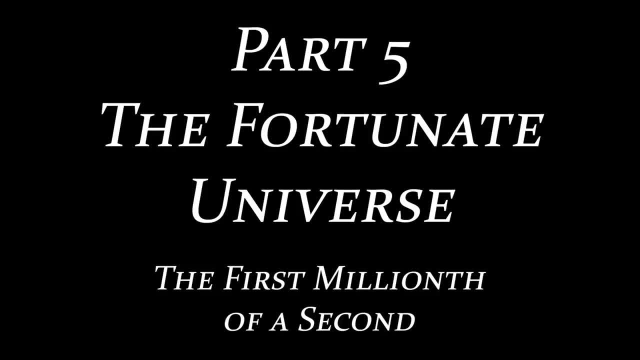 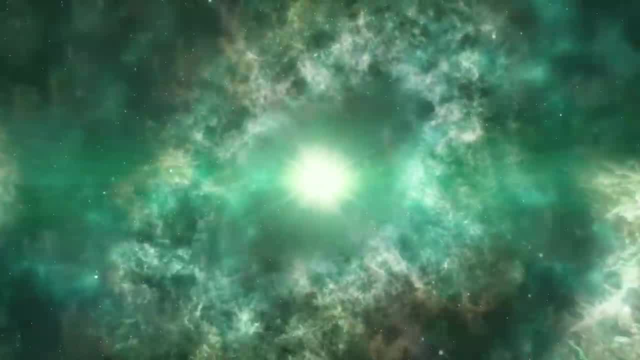 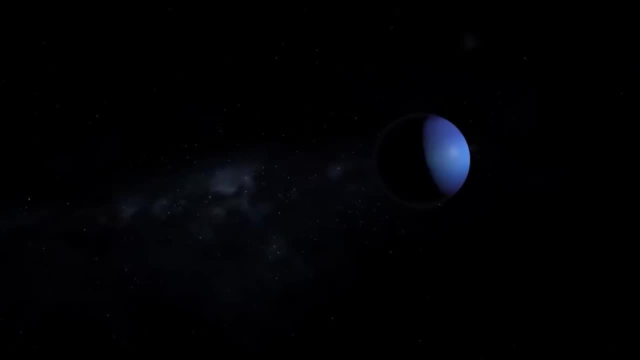 Our universe is full of incredible variety and diversity. There are stars that burn hot and fast, exploding catastrophically after scarcely a million years, and others that sizzle away slowly, unchanging for trillions of years. There are multitudes of planets. 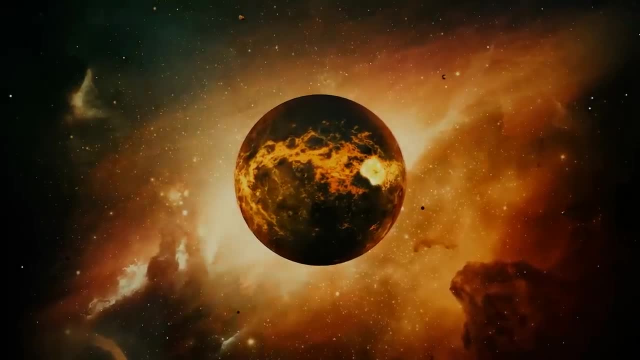 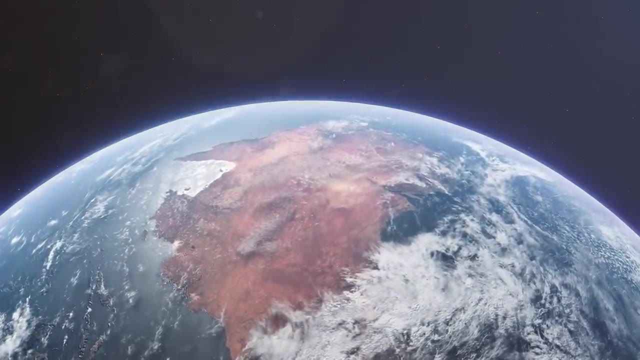 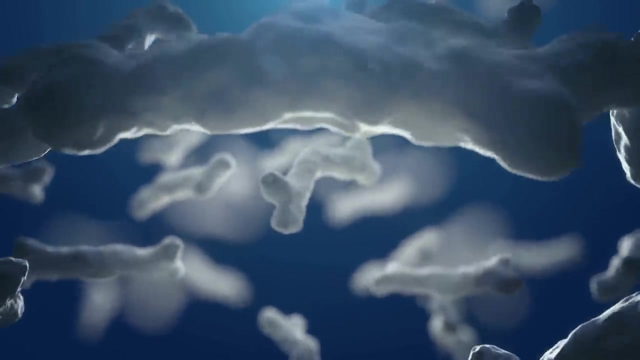 giant gas worlds, scorched and barren rocky worlds and occasionally green watery life ready worlds. And on those worlds that do host life, like Earth, there is every kind of life form you can imagine, from tiny bacteria who breathe sulphur or methane to self-aware and cognisant apes that build structures and telescopes. 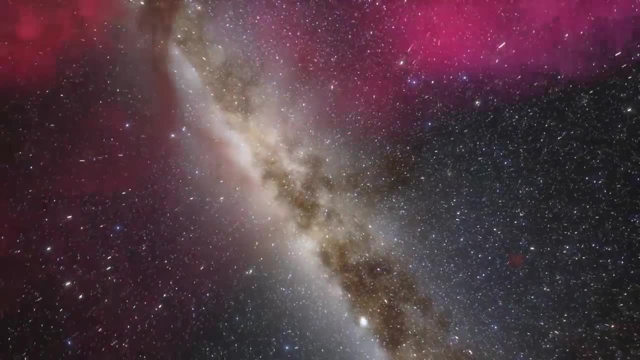 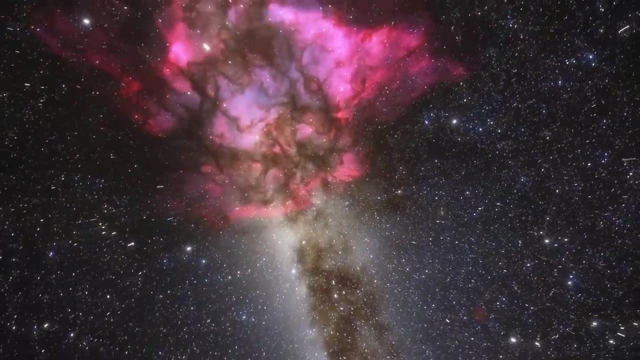 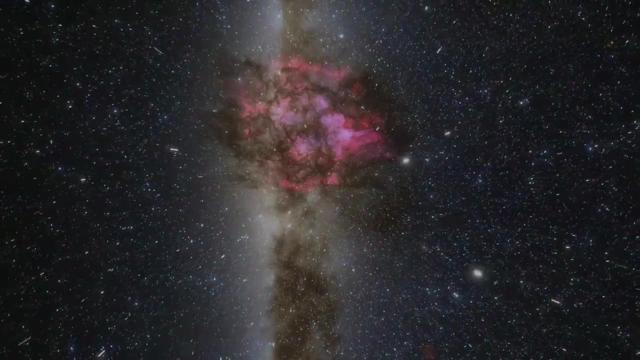 In the potentially infinite extent of the cosmos. there is almost infinite scope for variety, But there are also certain facets of reality that are immutable and constant, regardless of where you are in the cosmos or how you observe them. These so-called constants of nature have been revealed one by one as scientists. 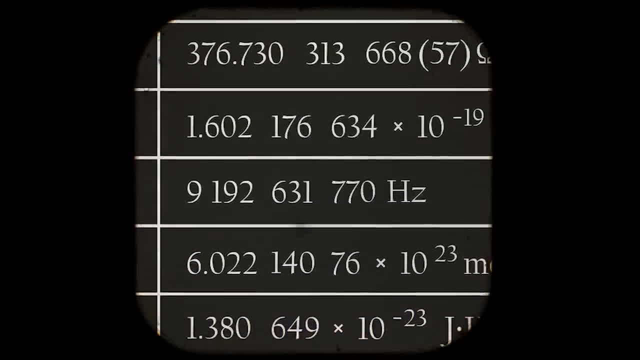 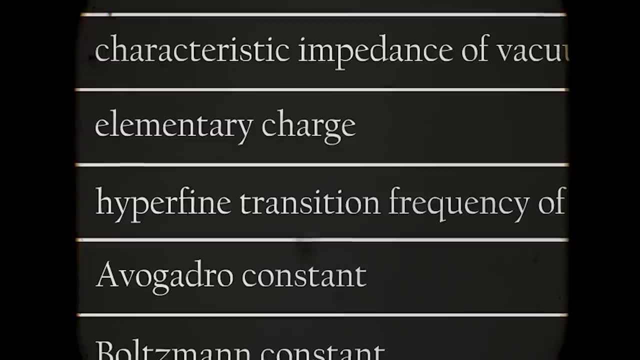 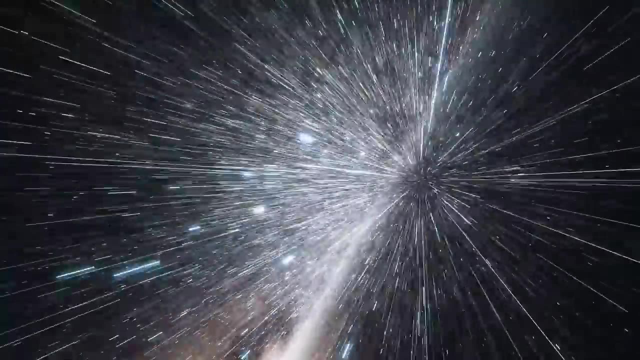 expand our understanding of how the universe behaves. Time and time again, we stumble across seemingly magical numbers unrelated to any other physical law or phenomena, Like the speed of light through a vacuum, often considered the absolute speed limit for anything travelling through the universe. 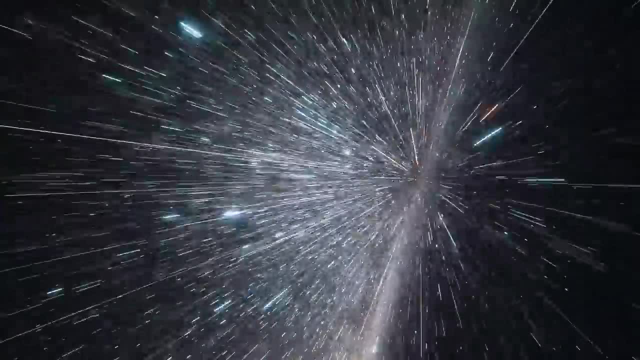 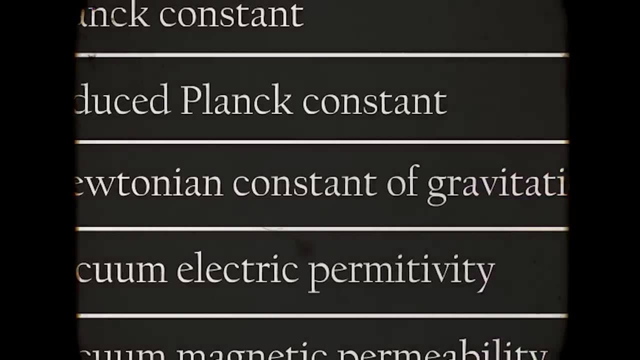 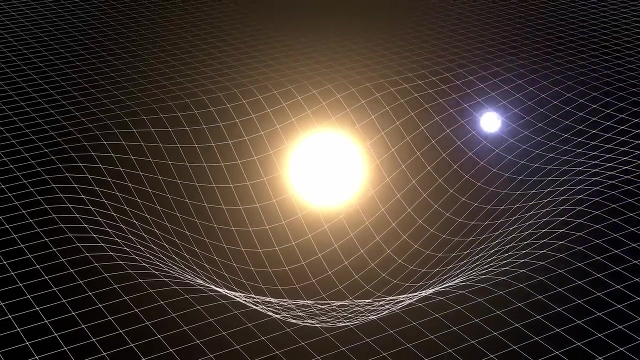 It is 2.99792 times 10 to the 8 metres per second, Or the universal constant of gravitation, which describes how strongly two objects will be attracted to one another due to gravity. It is 6.67384 times 10 to the minus 11 metres per second, squared per kilogram. 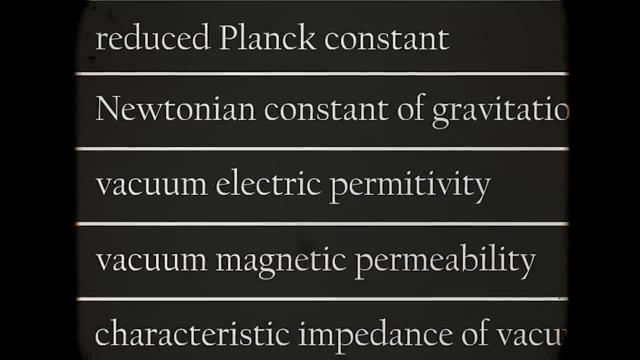 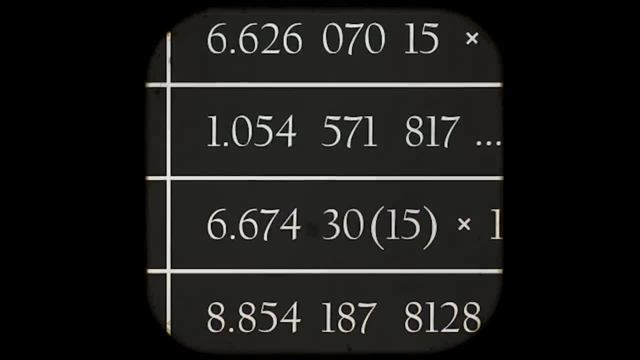 And the list goes on. There are precise and definable constraints relating the energy of particles to their temperature, for the strength of magnetic fields produced by electric currents and for the strength of an electric field that forms in response to electric charges. Less obviously, but still importantly. 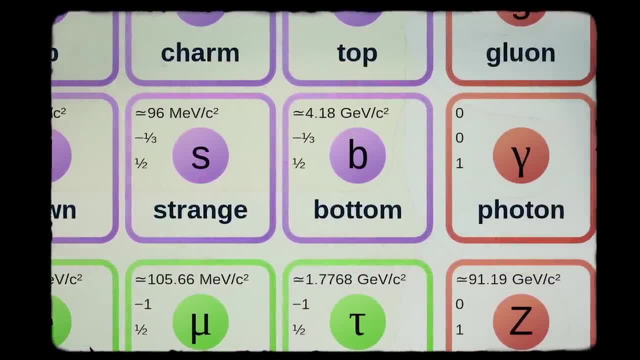 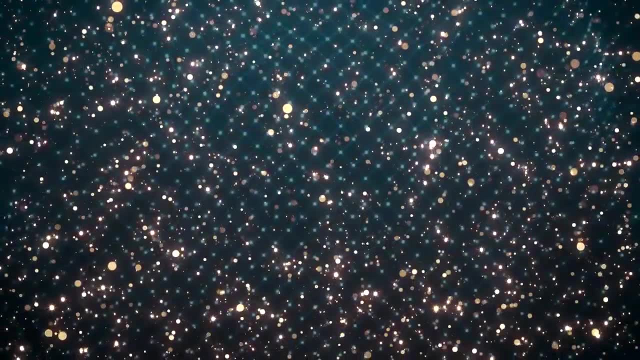 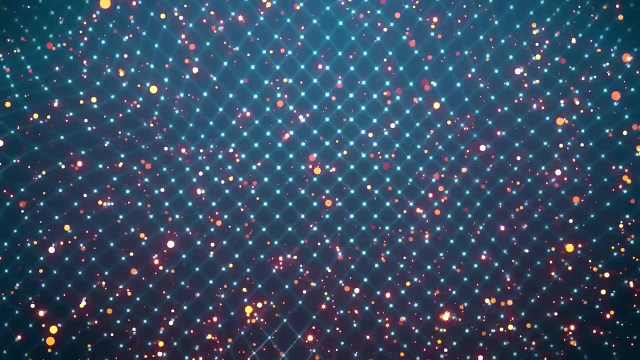 the masses of the fundamental particles are also set at constant but seemingly arbitrary amounts, a fact that even the Higgs mechanism is unable to account for. And so why should these natural relationships have these precise values? It is a problem that vexed even the great physicist Richard Feynman. 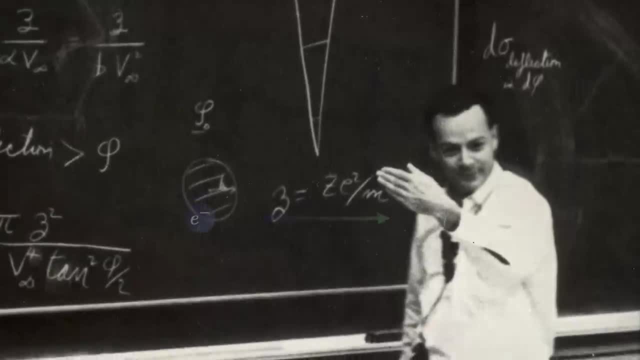 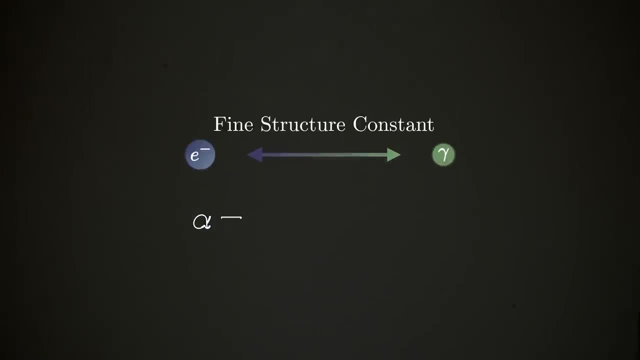 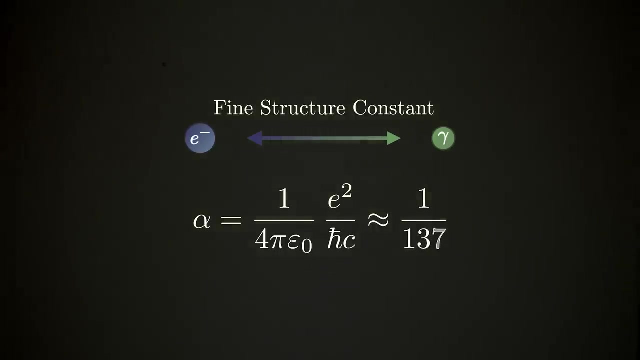 when he considered what is known as the fine structure constant. that essentially describes the strength of electromagnetic forces between particles, defining the chances that an electron will absorb a photon. Its value is a little over 137,, but there is no link between it and any other physical law. 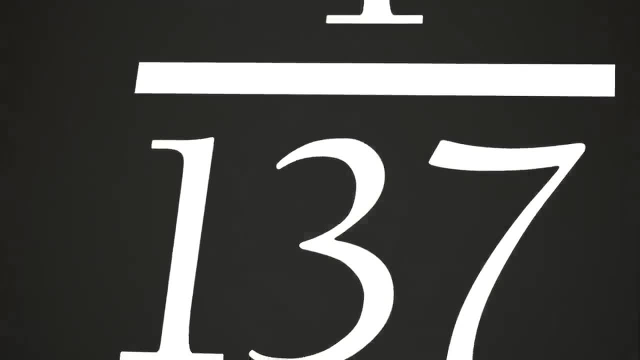 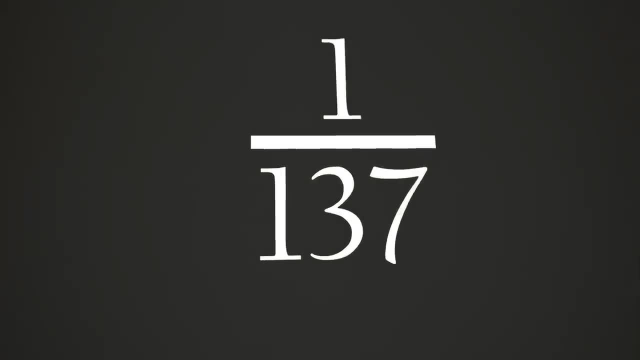 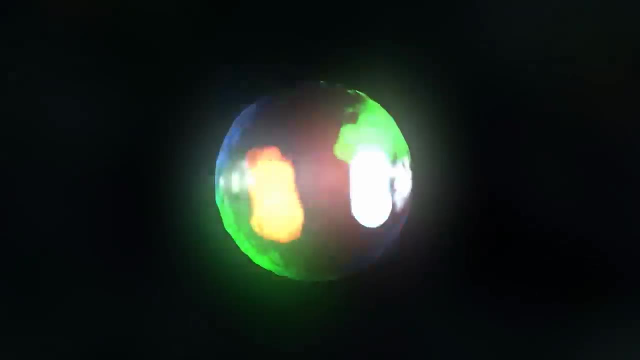 No reason for it not to be 12 or 135.. Or 3015.. The fact that it is 137 rather than any other number is crucially important for the overall state of the universe. If it were much larger or smaller, then it would seriously affect the stability of protons throughout the cosmos. 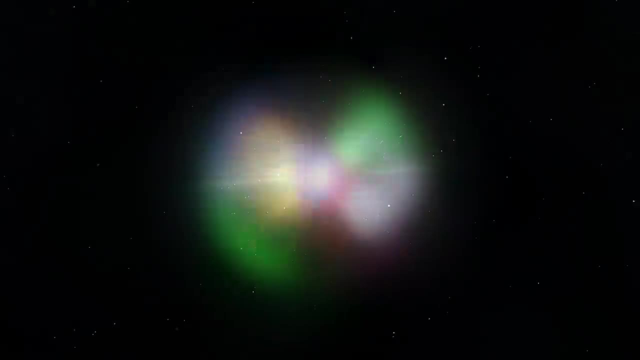 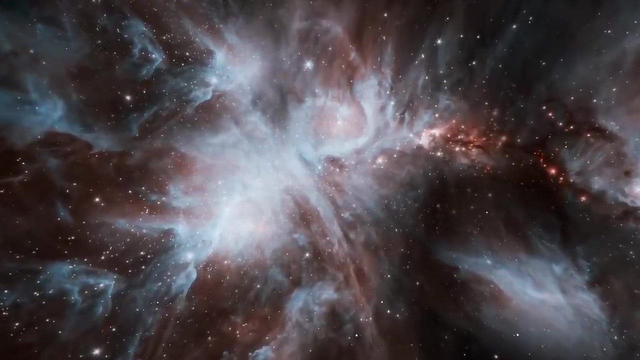 meaning that matter would have a hard time staying together, And the same goes for most of the other natural constants. If gravitation were weaker than it is, the universe would be filled with just an ever thinning soup of hydrogen gas. If it were stronger, then all matter would be drawn into black holes. 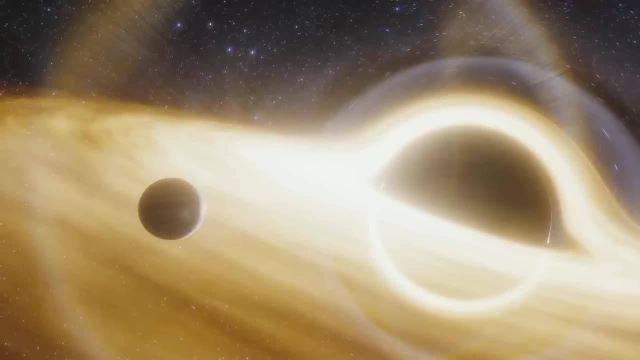 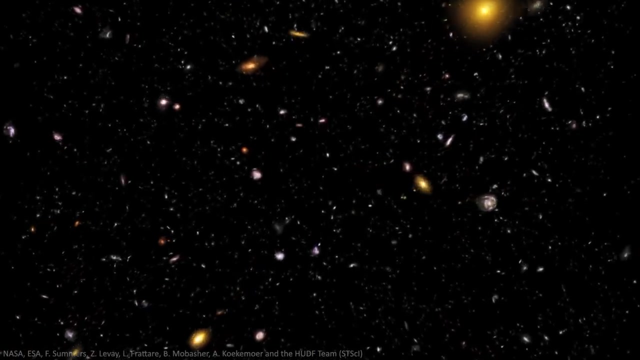 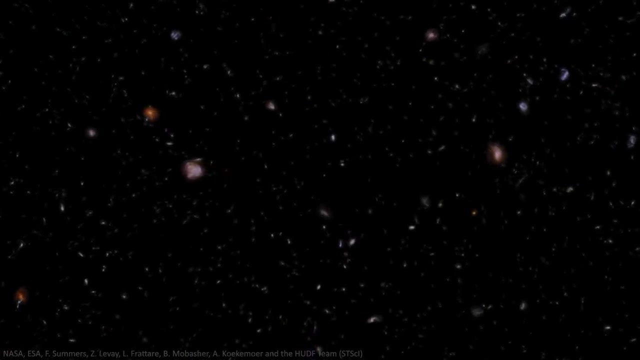 or violent, short lived stars, leaving no room for planets and life to form. The many constants of nature may seem arbitrary, but they are also finely tuned to allow for the varied and diverse universe we find ourselves within. But why, We still don't know. 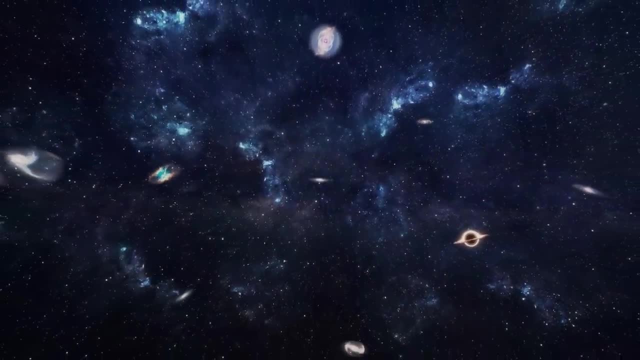 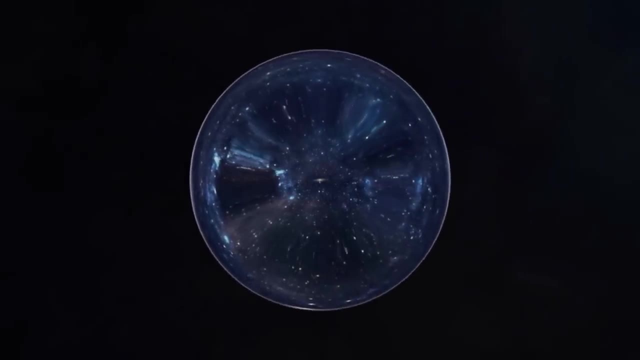 Is it just a lucky coincidence or the hallmark of a creator with their hands on the dials? Or, as many scientists suppose, is it that our universe is merely one of a multitude, all created with different starting conditions and different values for those fundamental constants? 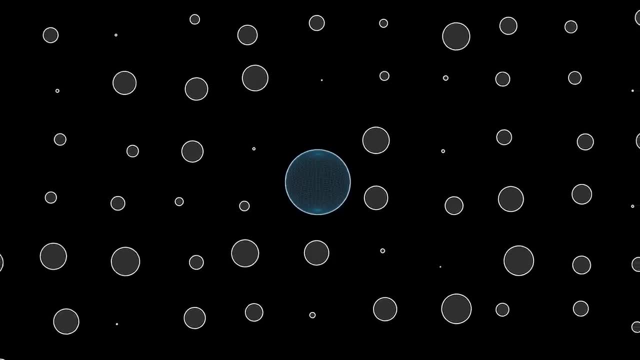 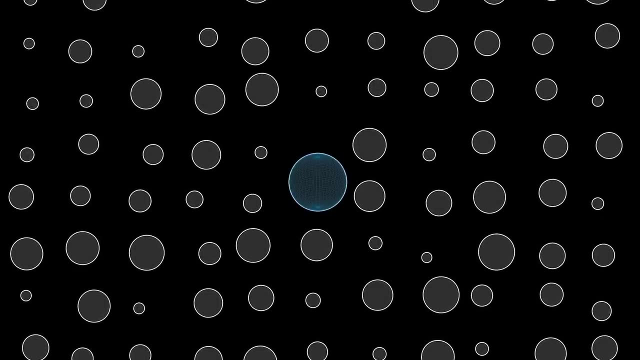 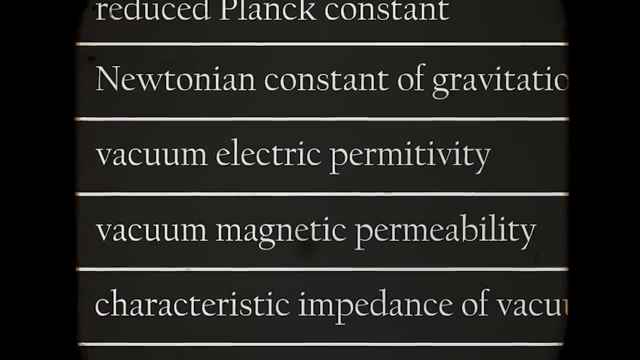 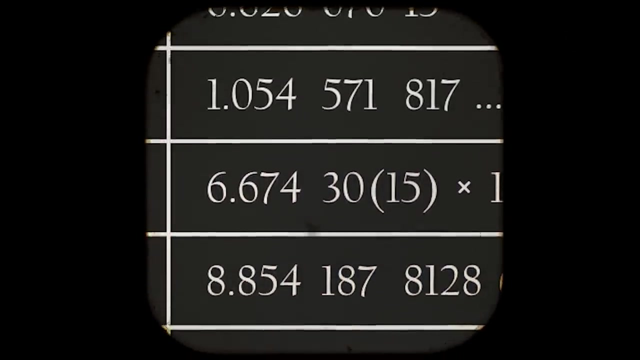 The vast majority having resulted in failed, barren universes and only those in which the values are just right able to culture cosmological variety, longevity and consequently us. Whatever the reason, this fine tuning is already hugely important in the opening seconds of existence. 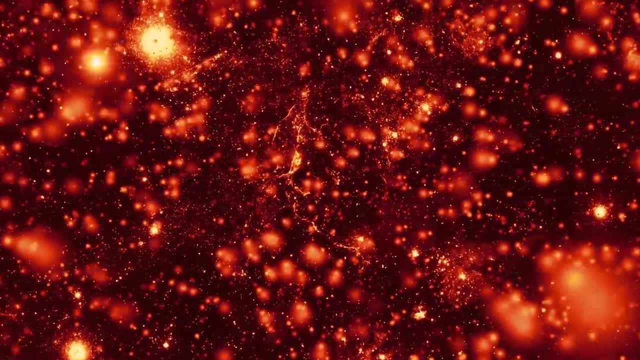 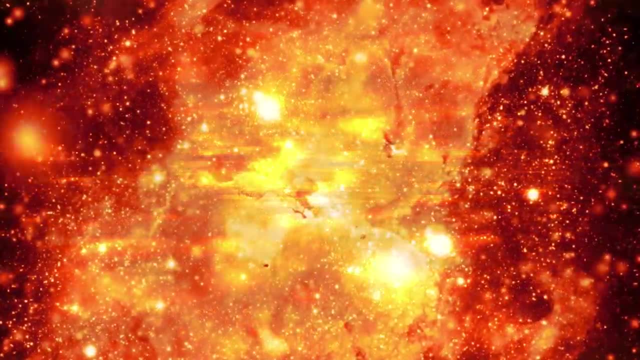 By the time, a billionth of a second has passed. since the Big Bang, the universe has been filled with an astonishing abundance of quarks, leptons and virtual particles, but temperatures and energies were still too high for any of these fundamental particles to interact meaningfully. 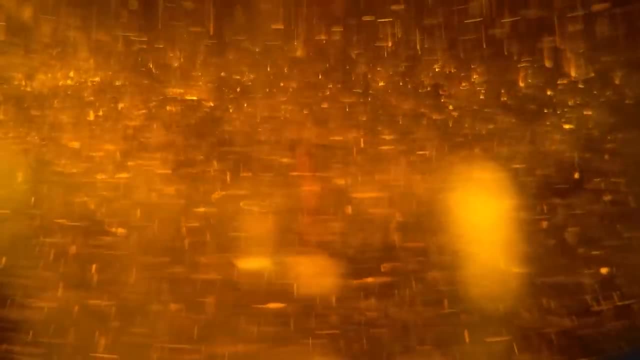 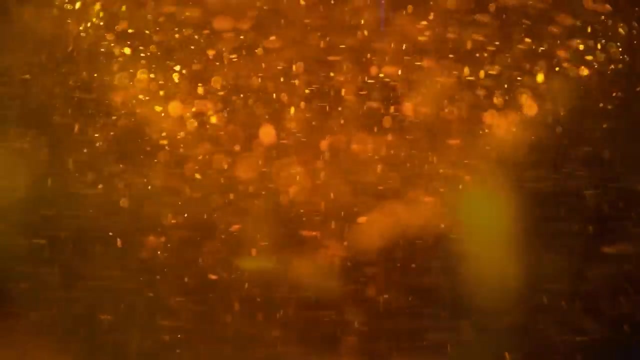 with one another. Temperatures drop, and by a millionth of a second after the Big Bang, the universe is a mere one trillion degrees Celsius. Gluons and quarks finally slow down their frantic vibration, allowing them to interact with one another for the very first time. 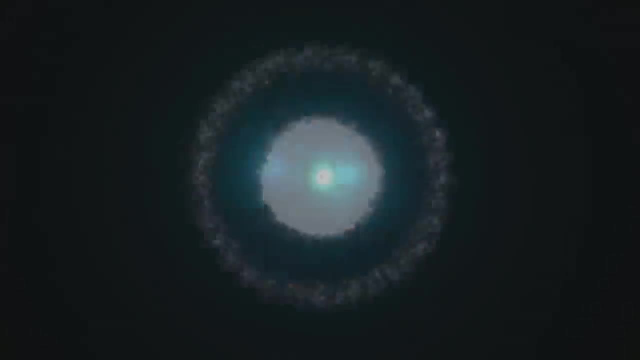 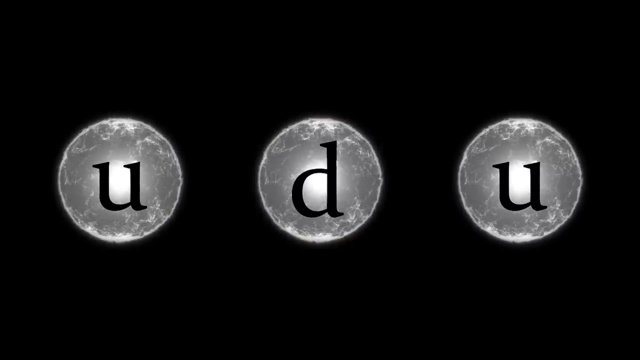 As we have seen, protons and neutrons are composite particles, each made from three quarks. but the component parts of a proton, two up quarks and a down quark are not natural bedfellows. The up quarks both have positive charge and, like charges, repel. 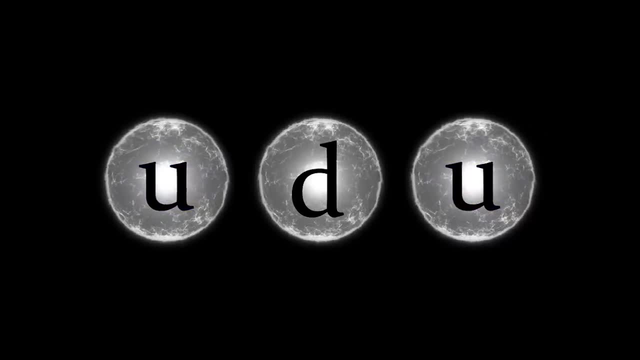 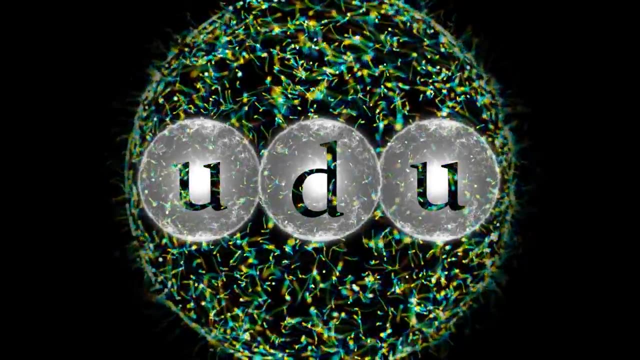 The closer the like charges get, the more strongly they reject one another. so it takes the assembled might of the strongest force of all, the strong nuclear force mediated by gluons, to hold them together into a stable hadron particle. But it turns out the internal anatomy. 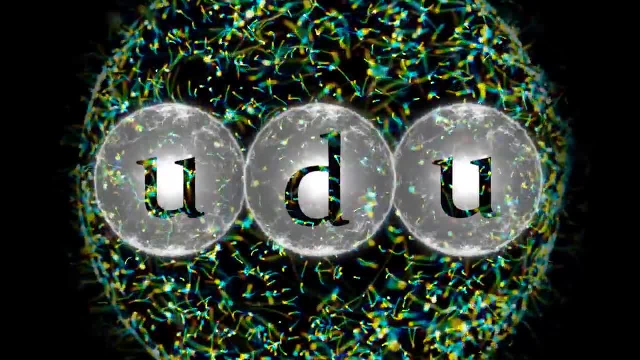 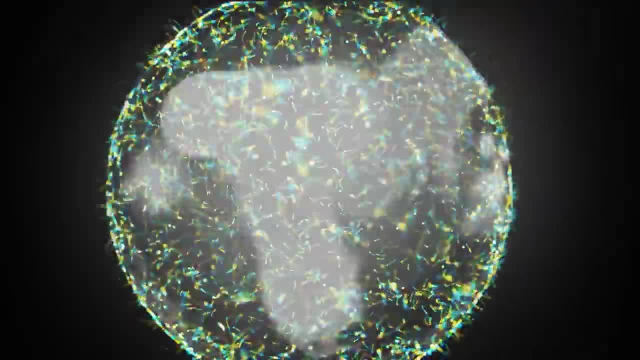 of a proton is even stranger than we might imagine. Not only is the majority of the mass made up of energy and quantum dynamics, but the composition of the matter isn't as constant as we might imagine. Sometimes one of the typical quarks inside a proton can spontaneously. 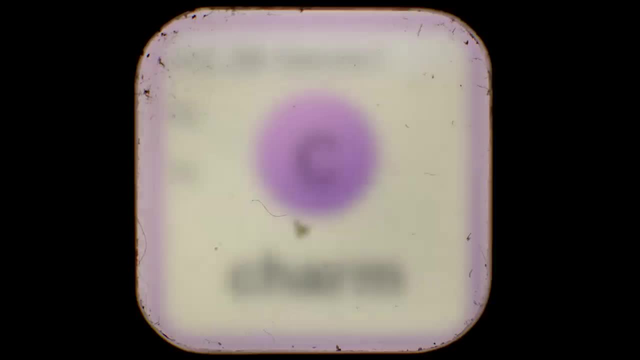 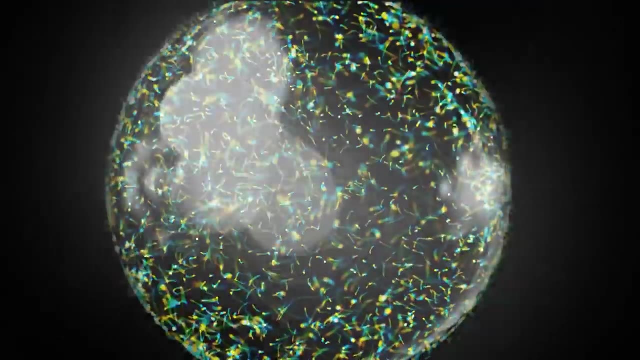 shapeshift into a charm quark And it's antimatter counterpart. The transformation is extremely short lived, however, and the charm quarks quickly recombine, But it means that protons are ultimately a constantly changing blur of the normal quarks, known as valence quarks. 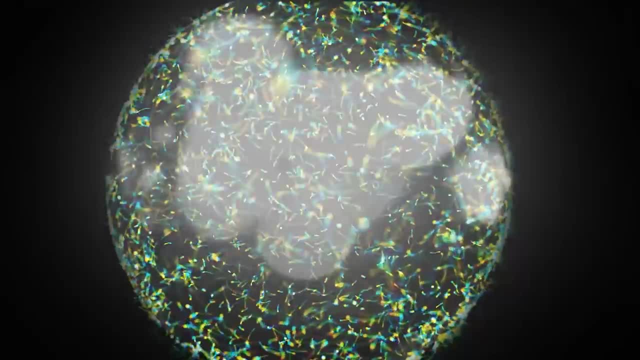 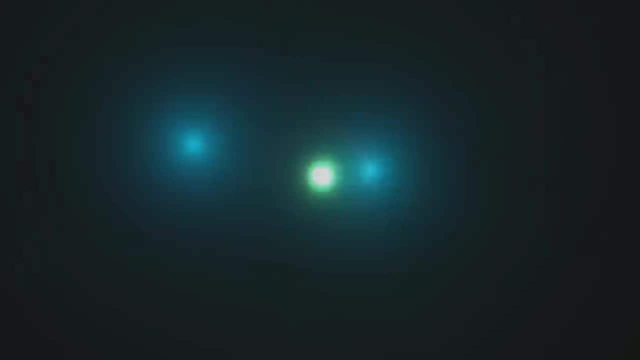 as well as gluons and charm quarks, Since both the gluons and the transient charms can be considered virtual particles. that means that the vast majority of a proton, as much as 99 percent, is actually made up of particles that don't. 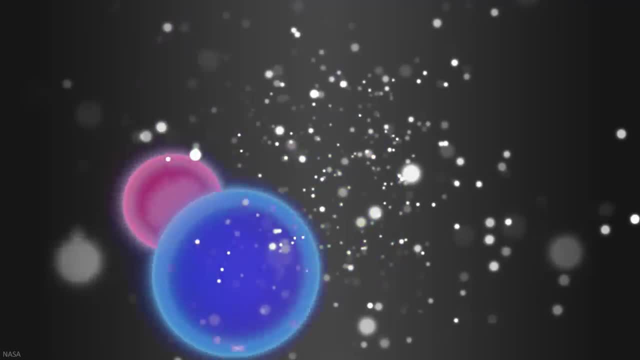 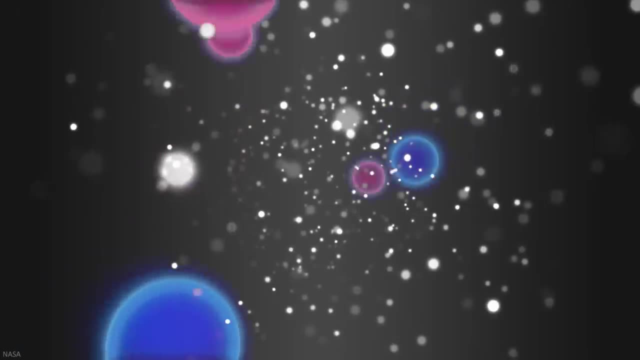 exist. The internal workings of protons and neutrons may be truly bizarre, but in the first millionth of a second of the universe, they are becoming an ever more prominent part of the universe's makeup. However, thanks to the effect of the weak force in this hot, dense plasma, newly formed protons can easily change identity to become neutrons and vice versa. It's only as the temperature drops even further, as the universe is approaching one second old, that this particular quark of the weak force becomes ineffective and the protons and neutrons eventually slow. 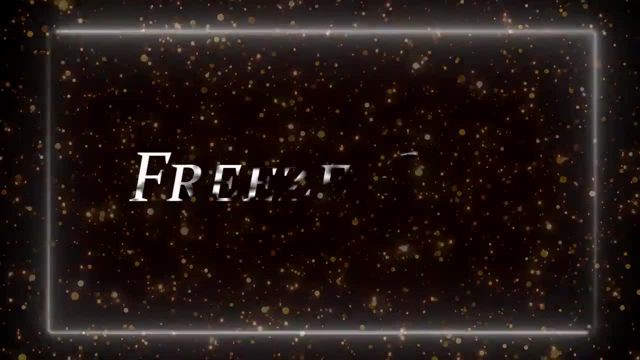 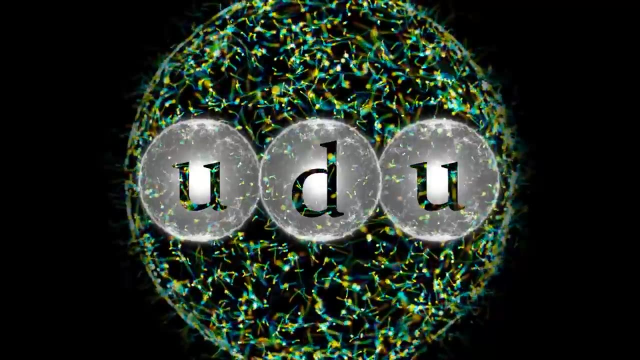 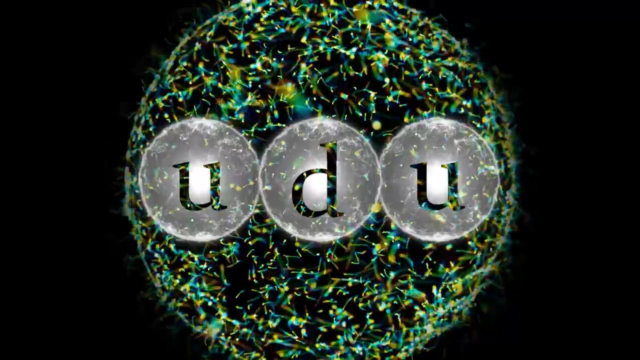 their switching. During this so-called freeze out, the hadrons choose an identity once and for all, And it is when this happens that the seemingly arbitrary, fine-tuned constants of nature, in this case the masses of the up and down quarks- 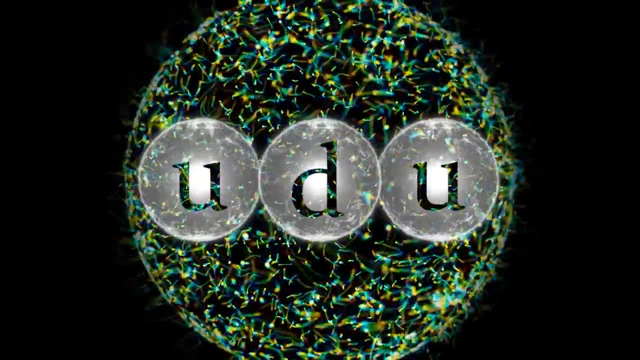 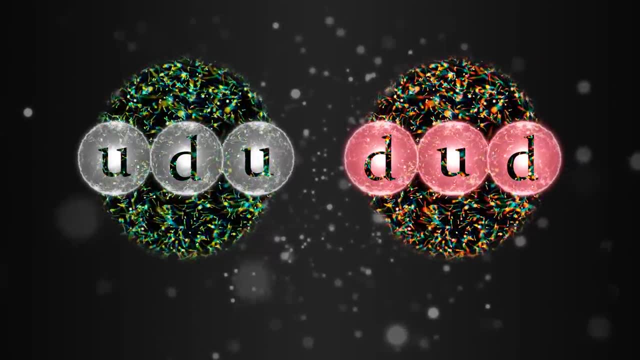 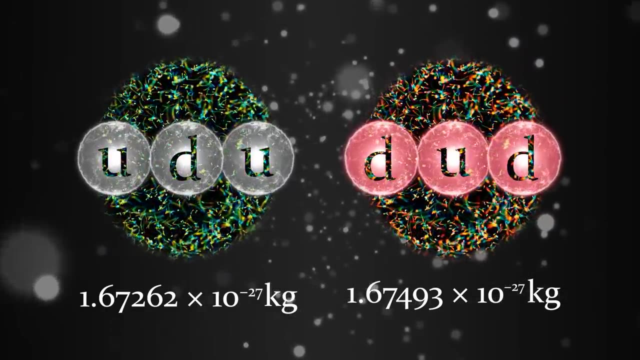 have their first real opportunity to shape the future of our cosmos, Because down quarks are heavier than their up cousins and neutrons contain two downs. the mass of a neutron is very slightly greater than the two up containing proton. So as the final identity switches take place in an ever cooling cosmos, 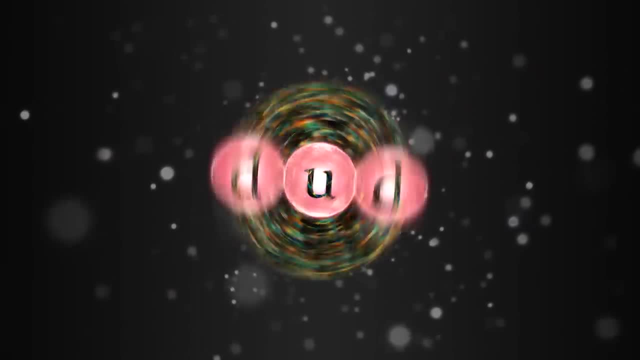 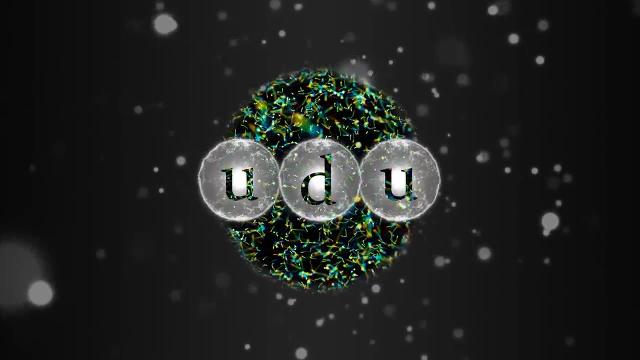 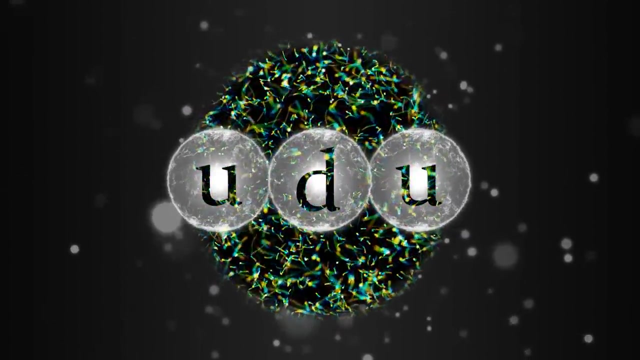 the downhill energy slope from heavy neutron to lighter proton is favoured over the energy intensive hole in the opposite direction. It is this very slight mass difference that ultimately results in an imbalance in the number of protons to neutrons in the universe from that point on, with roughly seven protons to every neutron. 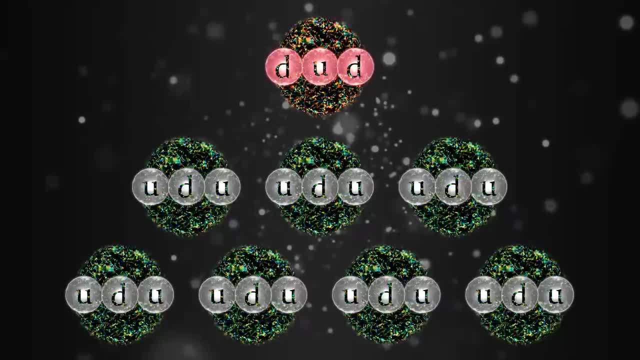 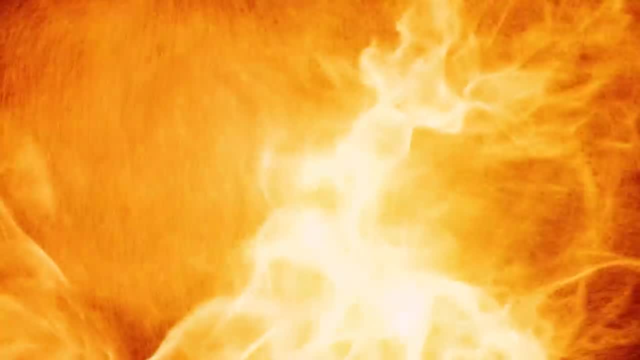 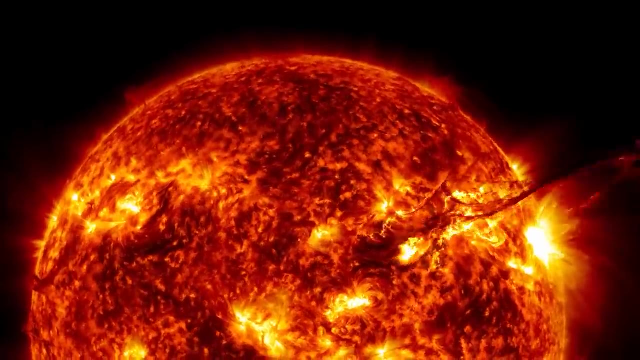 And this, it transpires, has been an important ratio for the formation of the universe as we know it. Protons are the basis for hydrogen and helium, the fuel for stars and the building blocks for all other heavier elements in the universe. The abundance of these charged particles over the uncharged neutrons is what allows. 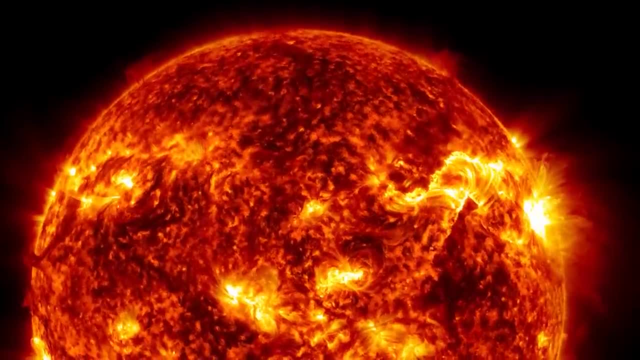 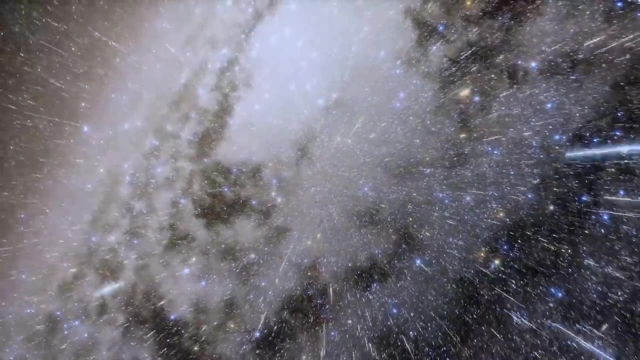 for elemental interactions leading to chemistry and biology. If things are started out differently, if the down quark had been allocated a slightly lower mass during the fine tuning of our reality, then the universe we see today would be very different. If neutrons weighed less than protons, then it would have been those that were favoured during freeze out. With more uncharged neutrons than protons, there is a limit to what chemistry could reasonably be accomplished. Hydrogen consisting of only a proton with no neutrons in attendance wouldn't be stable for long periods of time. 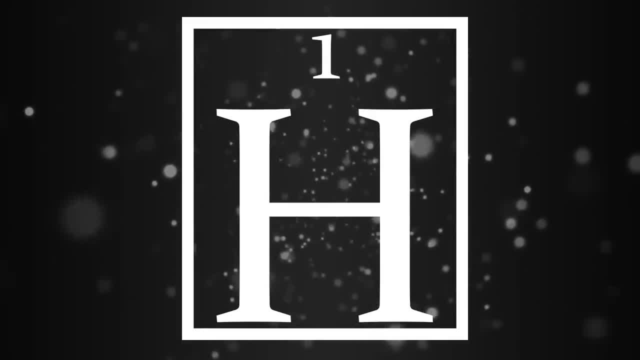 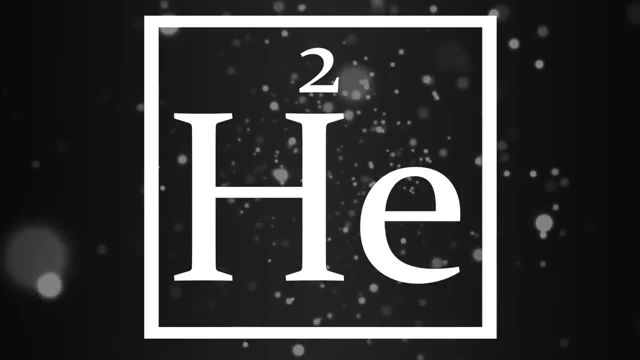 Some of the heavier protons could have been saved by binding to neutrons before decaying away, creating atoms of helium, But helium is often considered the most inert of all the elements. It is inherently stable, but unwilling to react. Between this and the overabundance of generally unreactive neutrons. 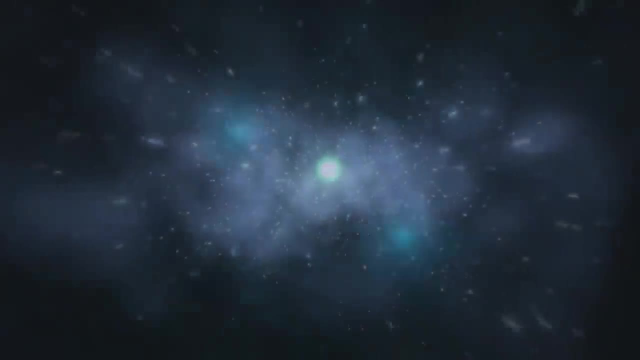 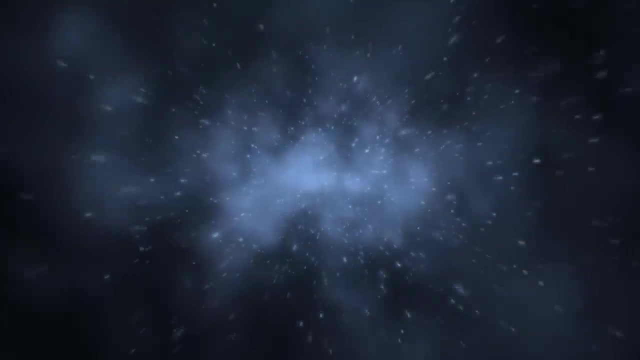 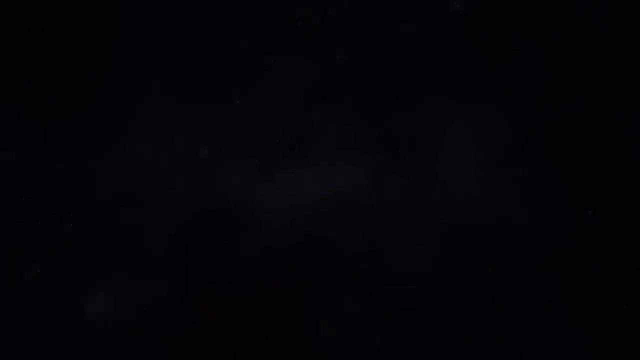 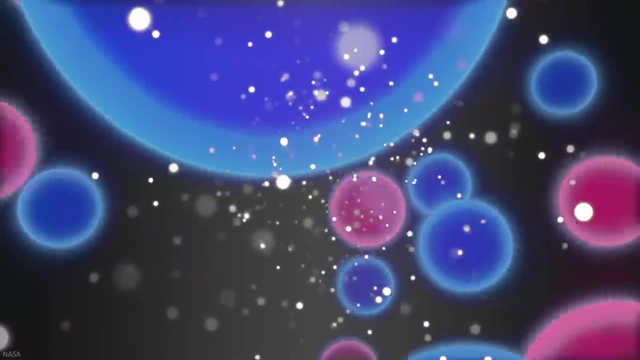 it would be hard to imagine how nuclear fusion could work. We would be left with a cold, dark universe with no stars, no galaxies, no planets and certainly no us. We can therefore be thankful for the universe's inexplicable leaning towards protons over neutrons. 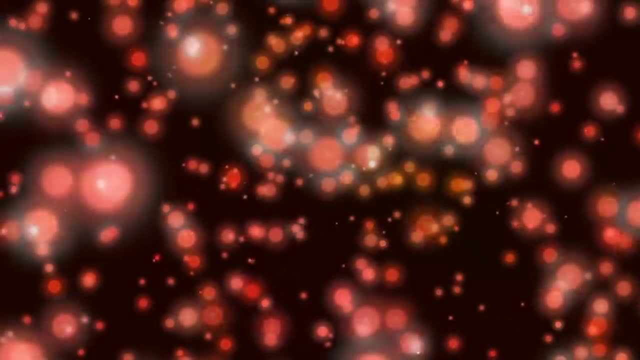 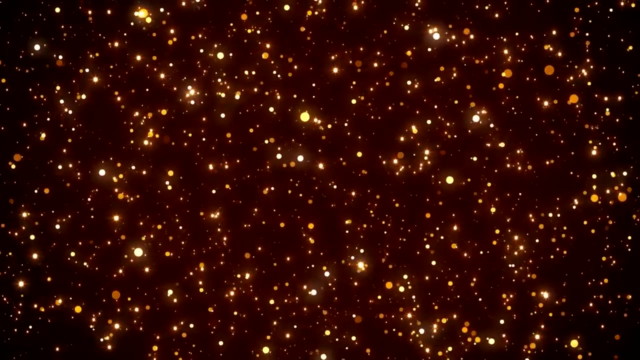 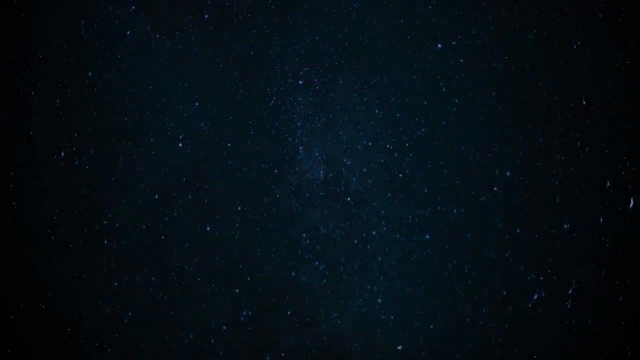 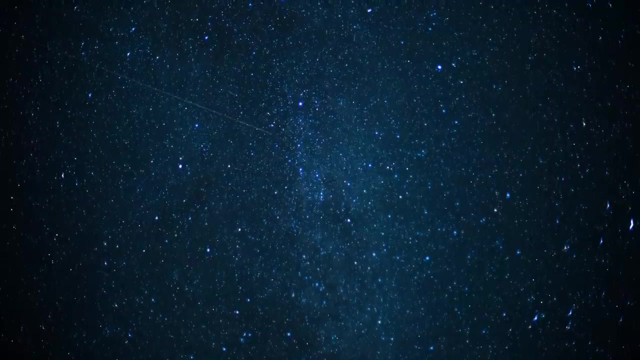 But this isn't the only imbalance that becomes baked into the cosmos around this point in its evolution. There is also a mysterious but fortuitous lack of antimatter. One day in the future, as we peer into the sky, we may be looking in the right corner at the right time to see an alien civilization. 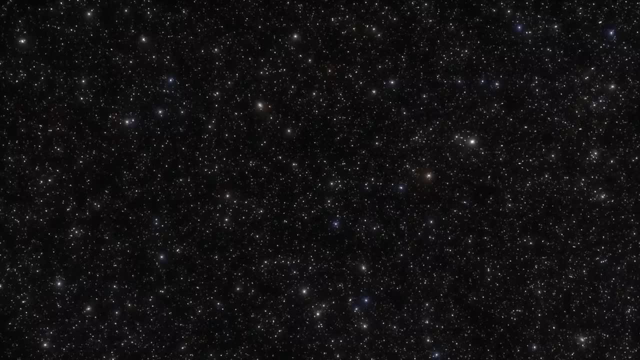 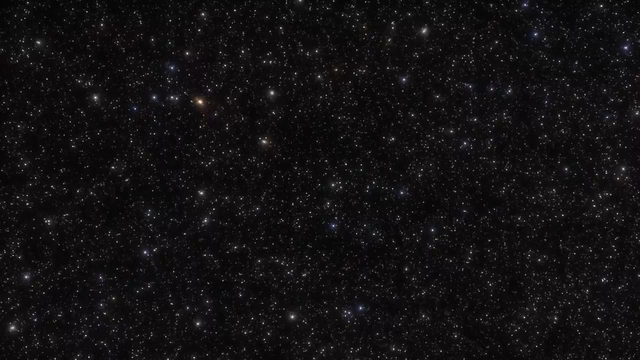 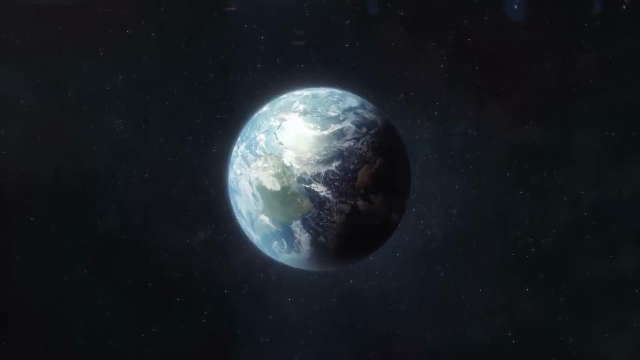 destroy itself. Scarcely more dramatic than the subtle brightening of one of the faintest stars in the black, but representing an energetic explosion from a weapon powerful enough to level an entire world. History tells us that disagreement and discord is a common theme among Earth. 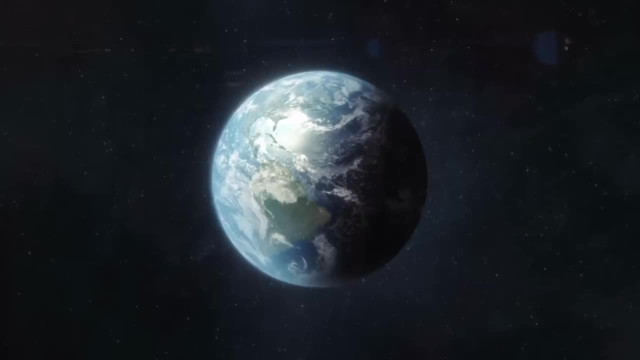 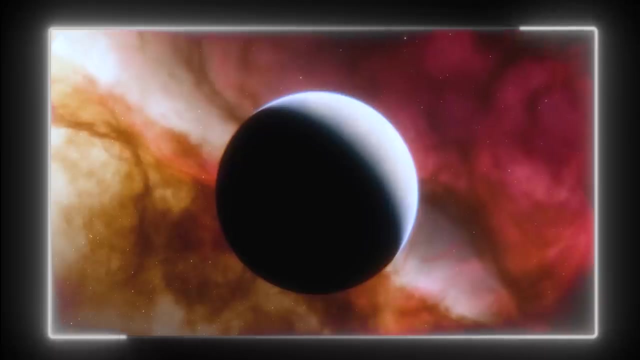 and there's no reason to believe this wouldn't be the case elsewhere in the galaxy And so on a warring alien world as on Earth, efforts to prevail over the enemy lead to an arms race, from sharpened points to explosive projectiles, nanomachinery to atomic bombs. 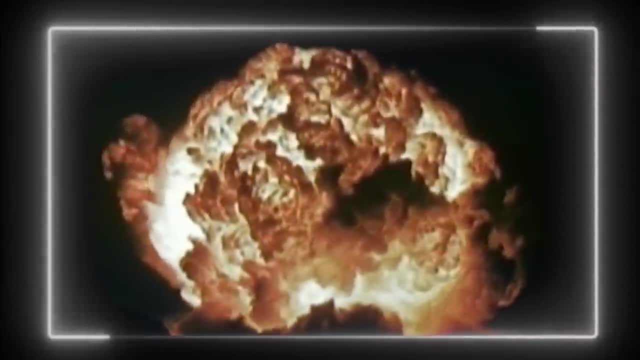 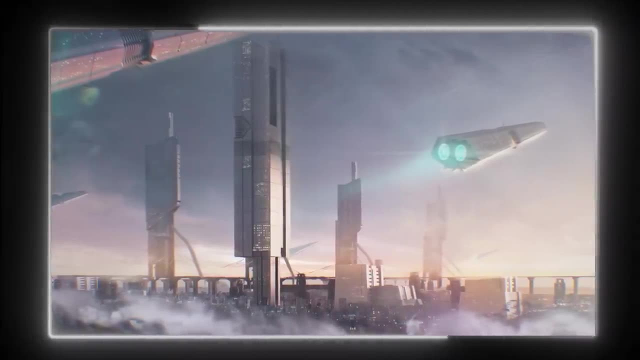 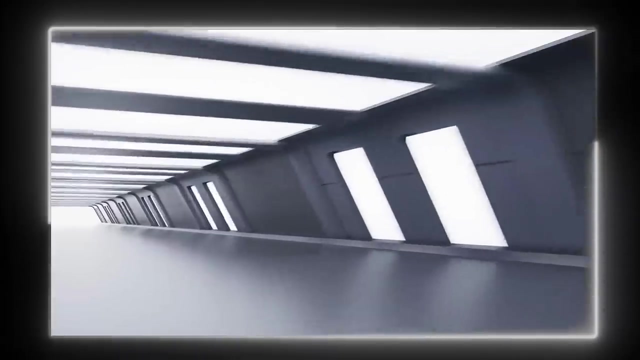 The struggle for the most destructive weaponry goes on, But these advanced extraterrestrials are still not satisfied and soon turn their attention to an even more powerful source of latent energy. With greater technological prowess than humanity, they have learned to produce and isolate particles of antimatter, holding them in a vacuum suspended. 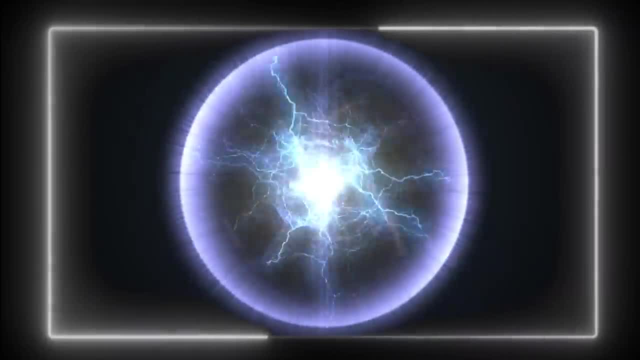 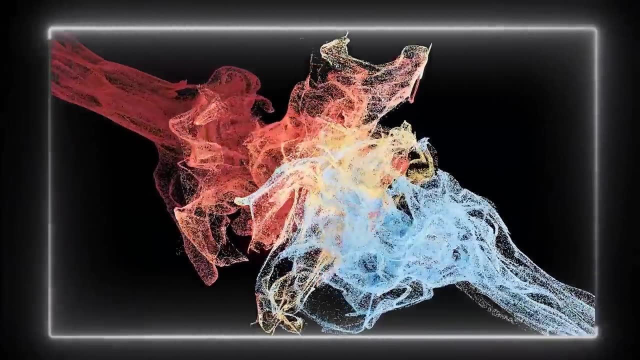 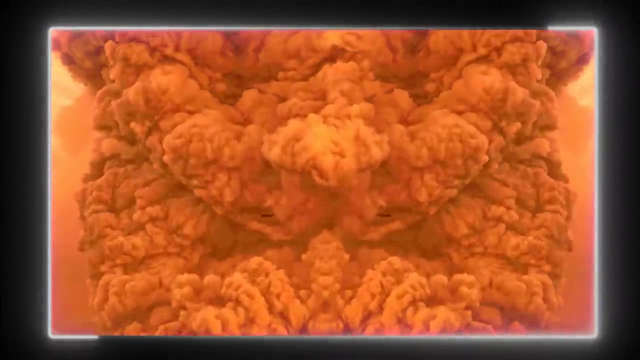 by electromagnetic forces until it is time for them to be deployed, But they do not need vast quantities of fuel or any sort of trigger, For the moment that antimatter comes into contact with the normal matter that prevails on their homeworld, the particles will annihilate together, destroying themselves and releasing vast 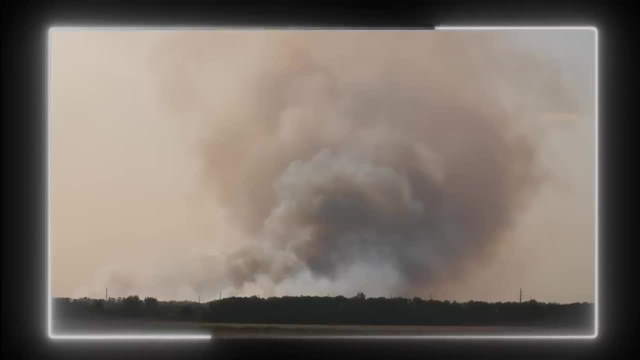 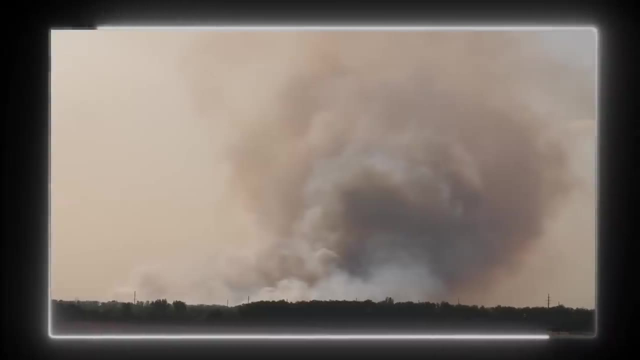 amounts of energy. Just one gram of antimatter releases as much energy as a traditional nuclear weapon with some 90 kilograms of fuel. And as the arms race goes on, the stockpiles grow, Whether it is used in anger, confusion or simply by accident. 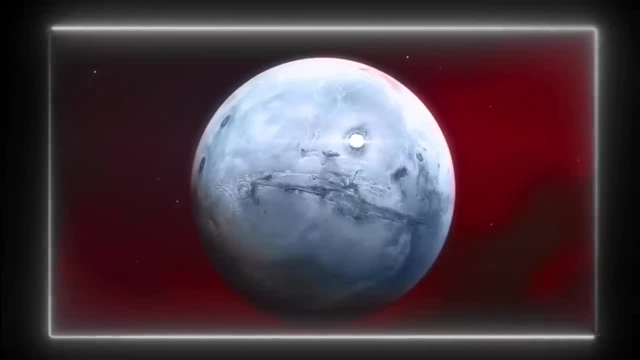 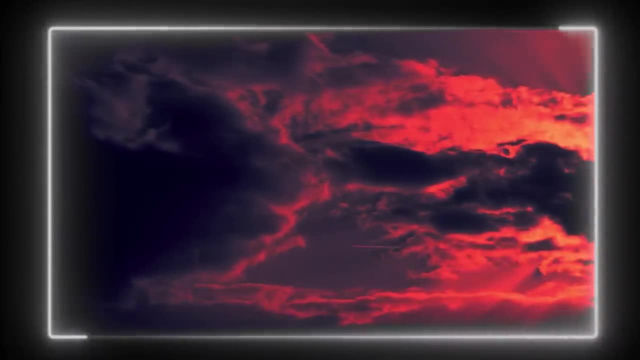 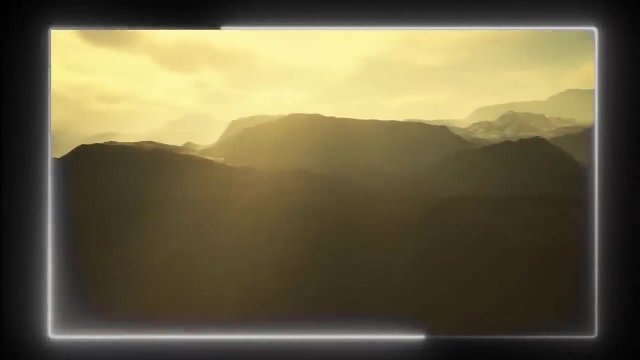 the detonation of this antimatter weaponry occurs. Night turns to day in an instant. Scorching winds raise entire cities, destroying both warring factions and all other life on the planet. The entire world is transformed for centuries to come. Such is the devastating possibility. 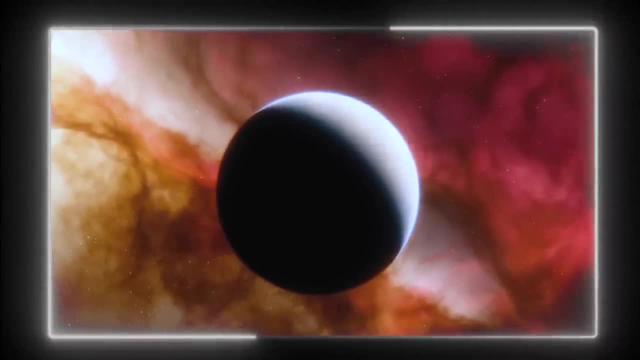 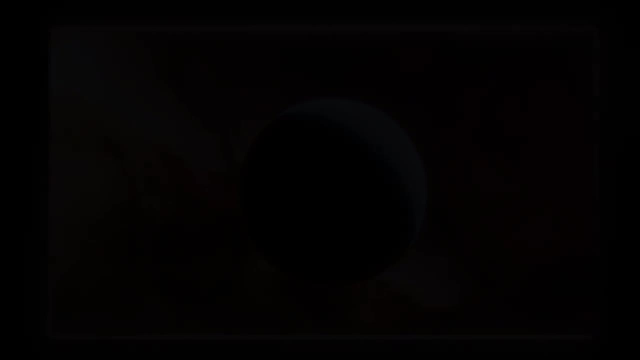 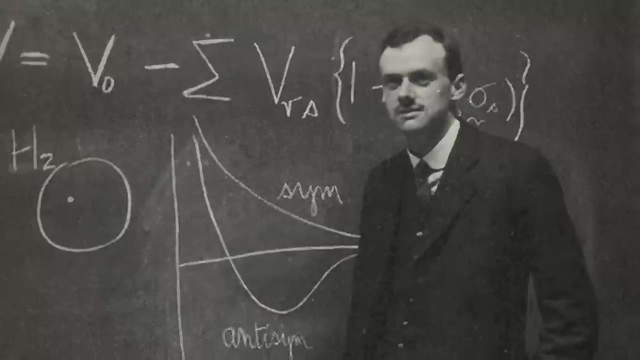 of antimatter coming into contact with matter, And yet we are surrounded by it every day. It was the English physicist Paul Dirac who, in 1928, first predicted the existence of antimatter working to integrate Einstein's theory of special relativity with the relatively 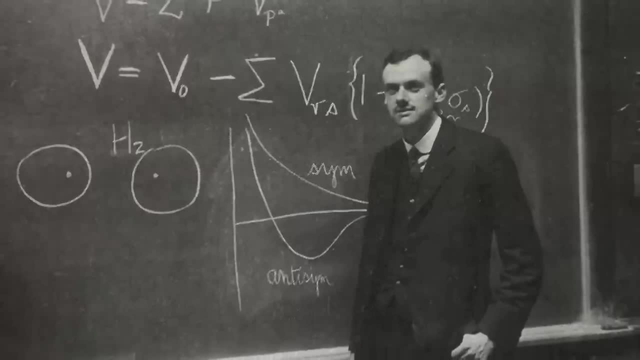 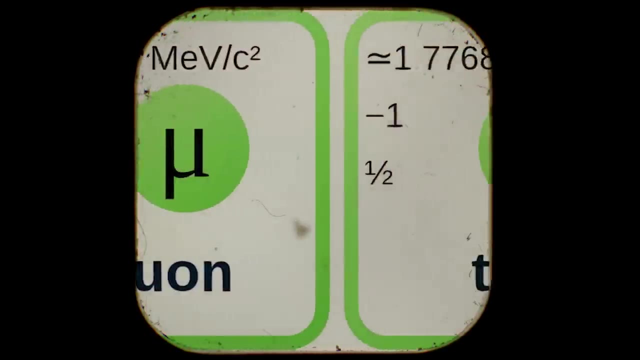 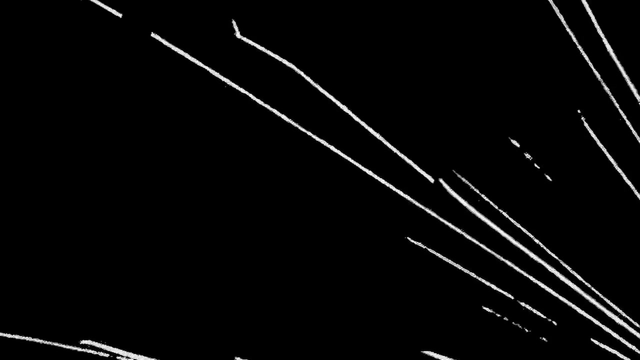 new quantum mechanics, He realized his equations applied not only to negatively charged electrons, but also to positively charged equivalents, thereby predicting a particle that was entirely new to science: an anti-electron or positron. Four years later, an independent American physicist. 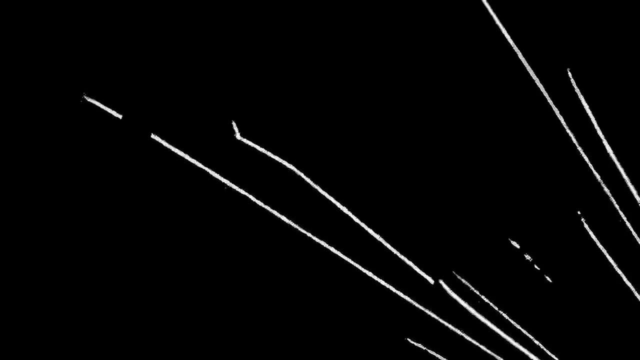 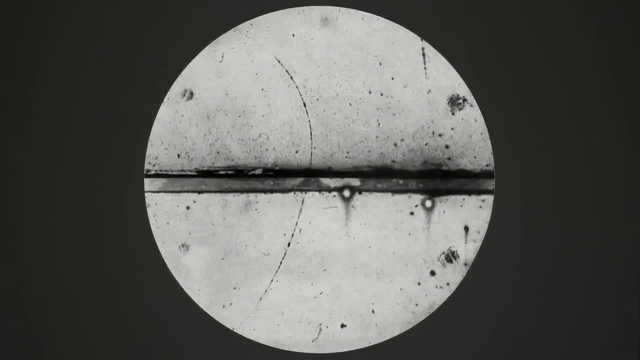 Carl Anderson actually detected this elusive particle in a rudimentary instrument called a cloud chamber. With the existence of antimatter now proven, physicists turned their attention to other antimatter particles. In the 1950s, the Bevatron accelerator in California succeeded. 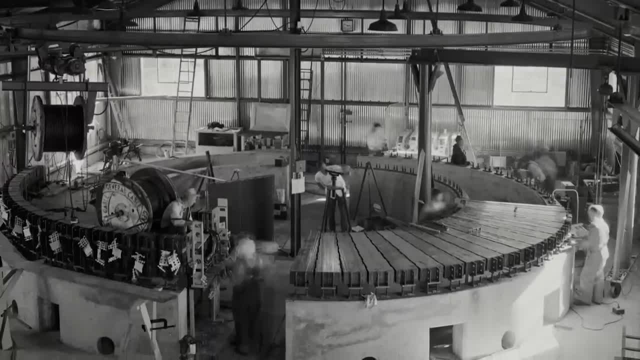 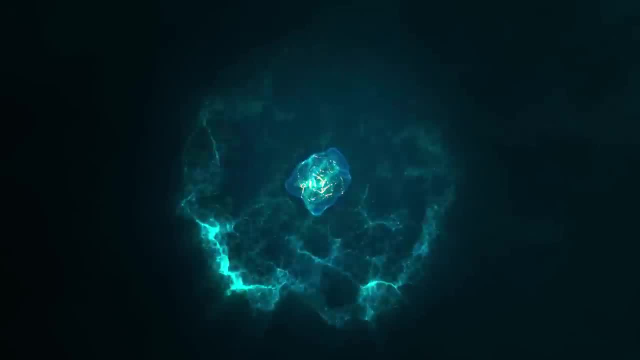 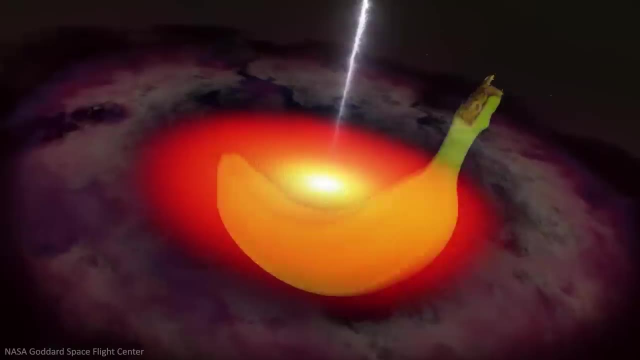 in detecting the first anti-proton and the first anti-neutron, And in 1995, scientists finally assembled an anti-hydrogen atom. Now we recognize antimatter in a wide variety of settings, from supernovae and black hole jets to the radioactive decay. 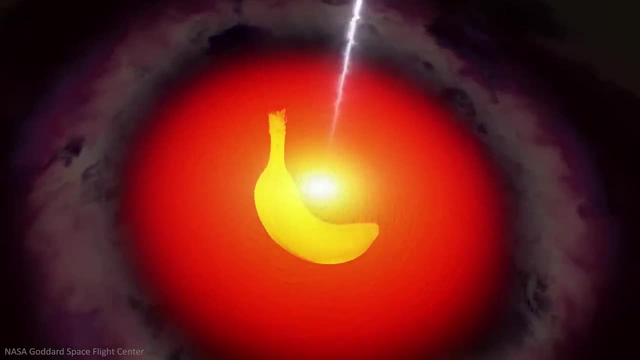 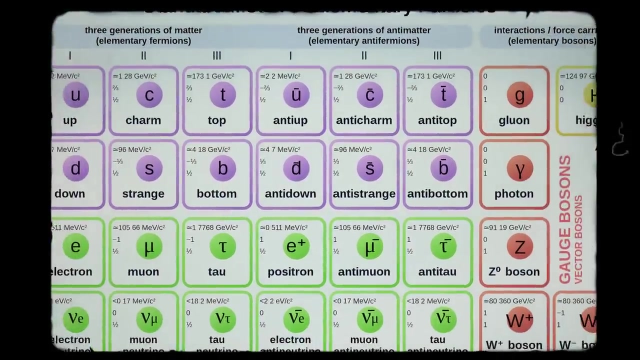 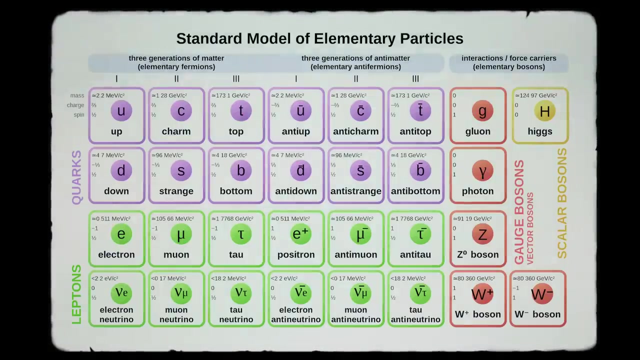 of potassium in a banana, producing a positron roughly every 75 minutes. So antimatter may not be confined to futuristic sci-fi settings, but it is still hugely outweighed by normal matter in the universe, Based on the notable absence of annihilation signatures. 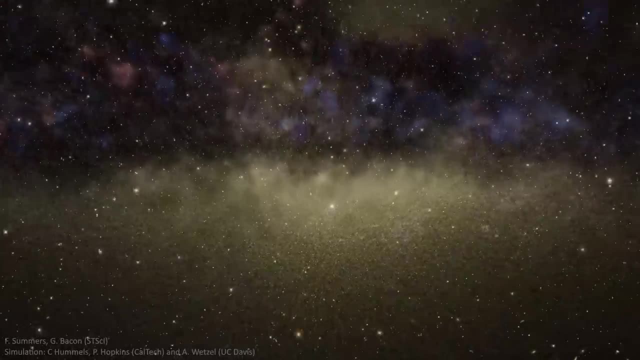 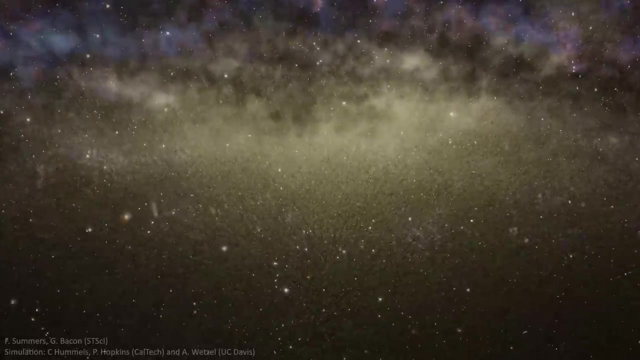 physicists believe that there can be no more than one antimatter particle for every quadrillion matter particles within the Milky Way. And this is just as well, because if there were equal quantities of both, then annihilation would have resulted in the ultimate destruction of all particles. 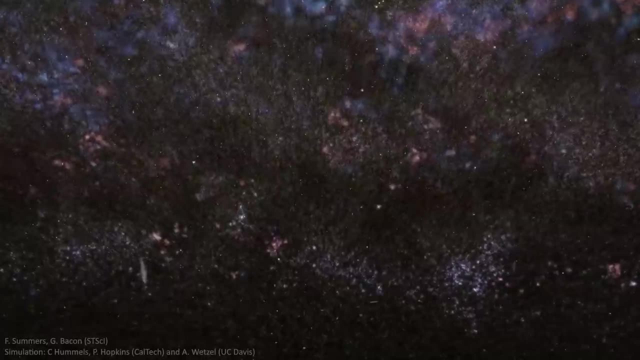 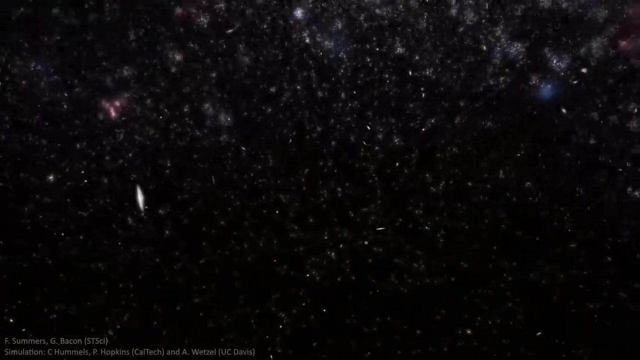 leaving nothing with which to build stars and planets. But the question of how this lucky imbalance came about is one that still troubles physicists. Could it be another quirk of fine tuning? In the beginning, antimatter would have been formed in tandem with matter. 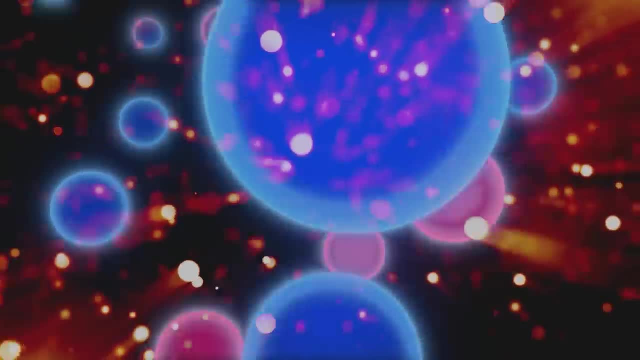 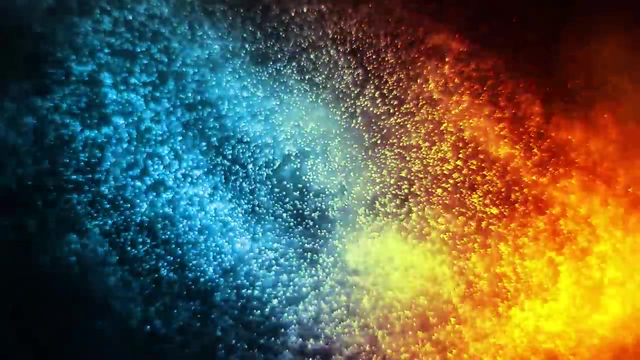 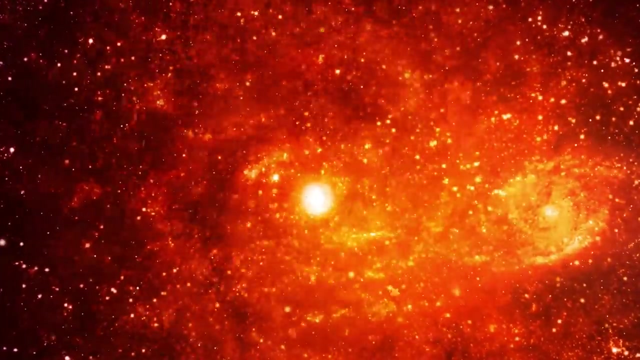 with pairs of particles forming from spontaneous energy transformations within the universe's first billionth of a second. But in such a dense environment they wouldn't have lasted long before encountering their opposite, annihilating together and transforming back into energy This process of spontaneous creation. 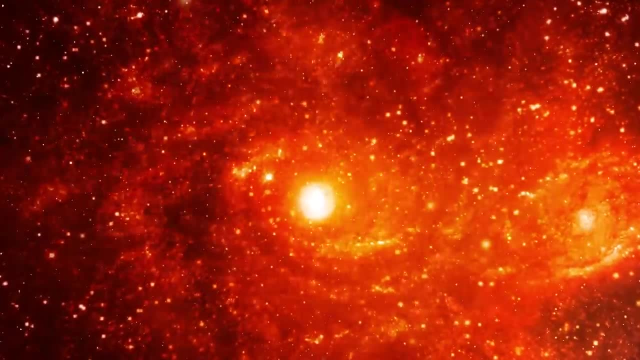 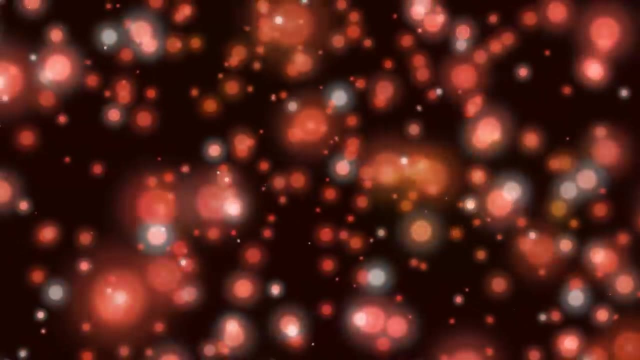 and destruction continues until the temperature of the universe drops And no new quark-antiquark or lepton-antilepton pairs are made. But gluons are not discerning on what kinds of matter they assemble, And as protons and neutrons are being made for the first time, 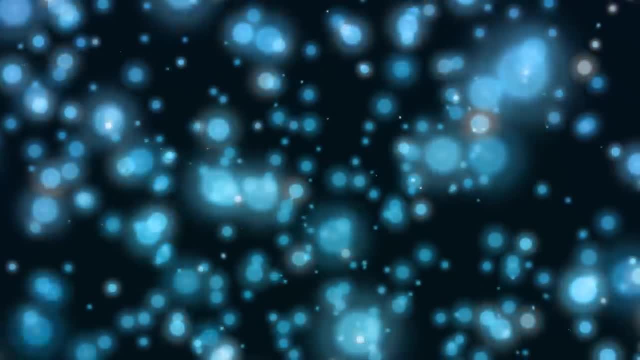 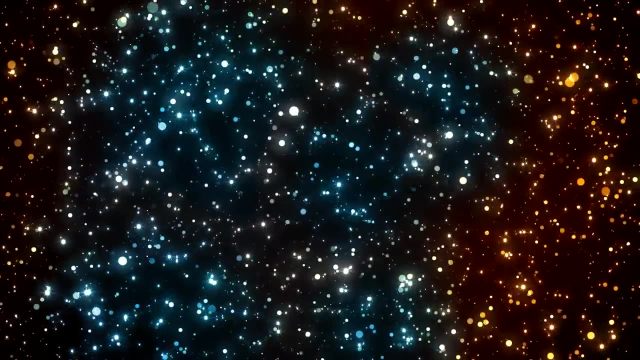 they are accompanied by an equal number of antiprotons And antineutrons. Everything should be in balance. At this point. there should be no difference in the quantity of matter and antimatter and, since the two kinds of particles behave identically and are only destroyed in pairs as well. 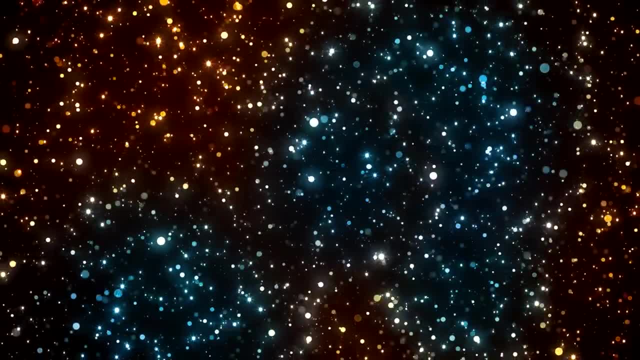 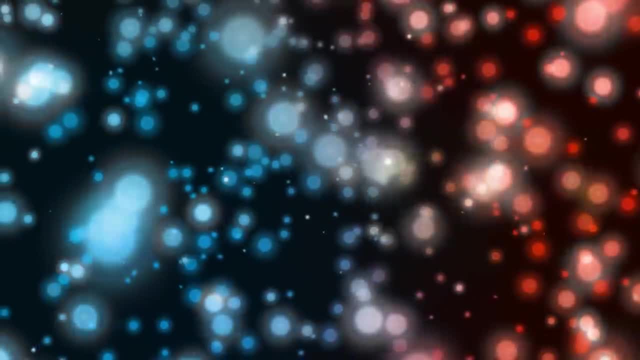 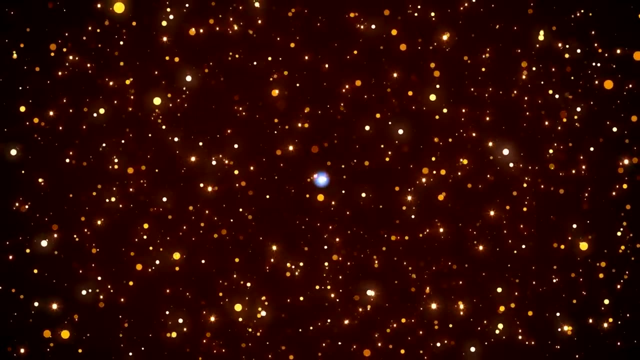 there should continue to be equal amounts of each, But this isn't what we see. At some point between a millionth of a second and two minutes into the universe's timeline, the balance of antimatter and matter changes until only one antimatter particle in a billion remains. 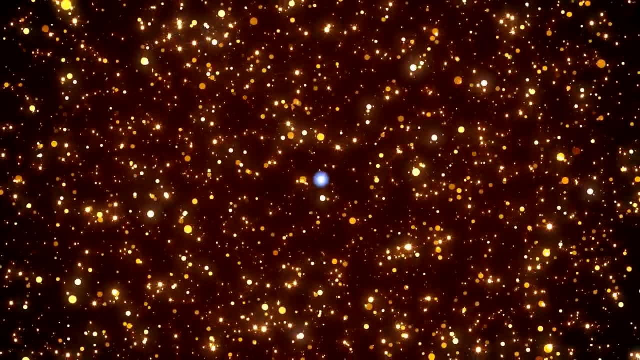 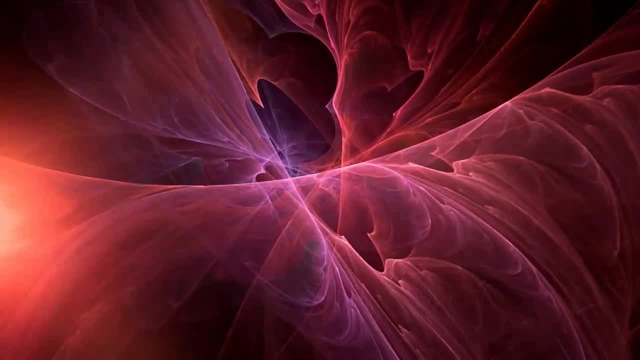 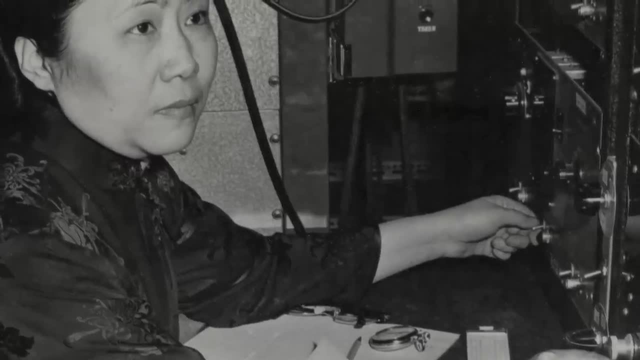 And to this day, physicists still aren't certain why. It could be partly as a result of the broken symmetry that came about with the emergence of the weak force. Experiments by Chen Xiangwu in the 1950s showed that quarks and antiquarks are. 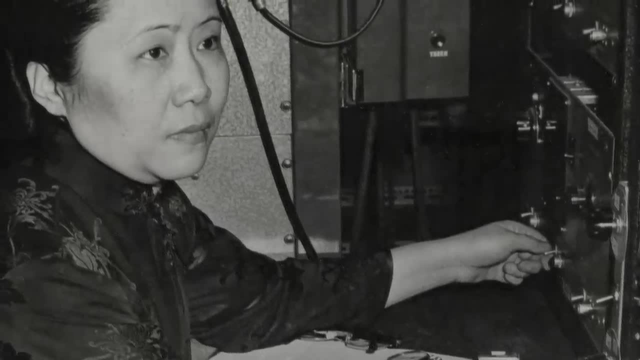 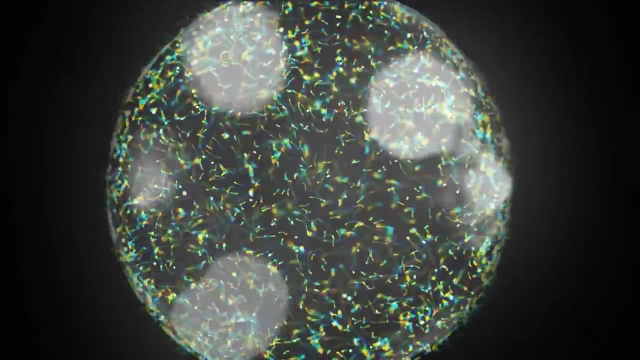 in fact treated slightly differently by the laws of nature. The difference is very small, but it is significant enough for us to see. Even so, scientists don't think it is enough to explain the overwhelming triumph of matter over antimatter in the early universe. 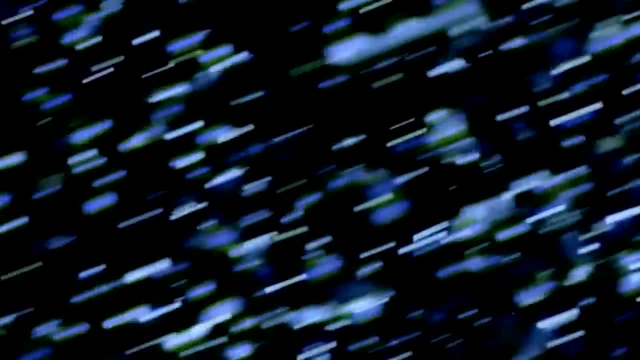 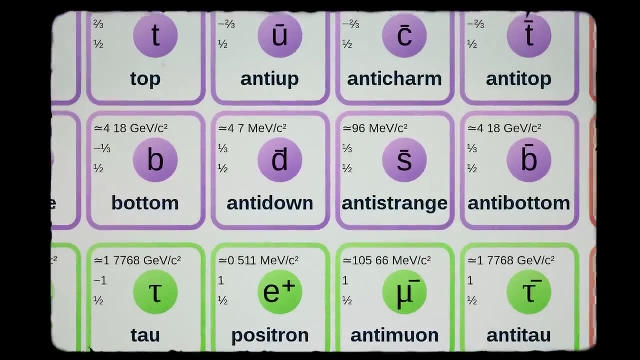 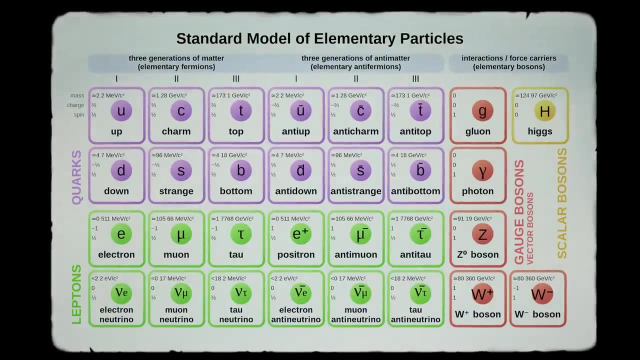 Instead, they entertain the possibility that another, as yet undetected and potentially extinct particle has a role to play. The idea comes from another kind of asymmetry that has been found within the standard model. Every particle and antiparticle we have found exists in both right handed and left handed forms, representing a kind 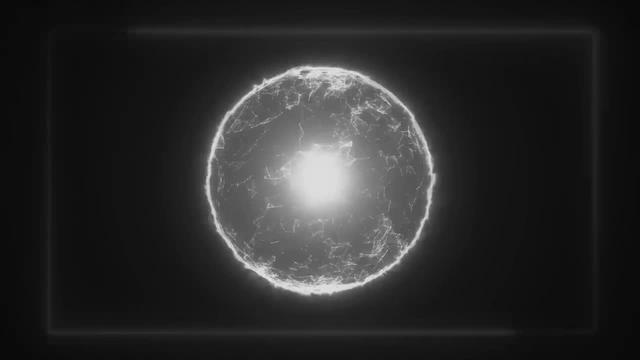 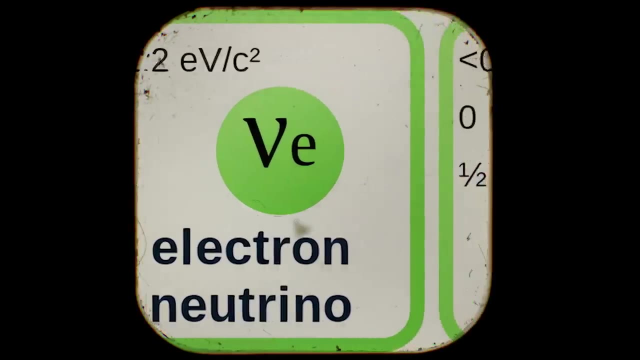 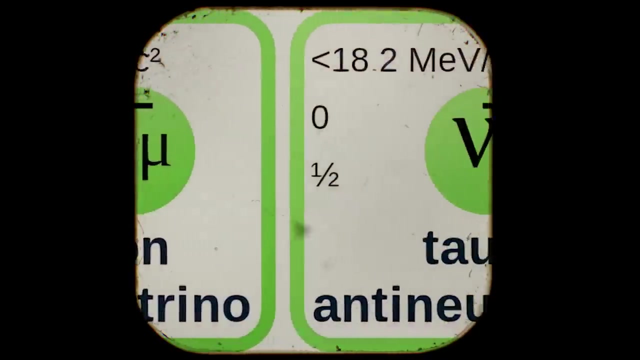 of symmetry in handedness that physicists call parity, But there is an exception where parity symmetry appears to be broken. Experimental physicists have only been able to find left handed neutrinos, whereas all the anti neutrinos are right handed. And so where are the right handed neutrinos and left handed anti neutrinos? 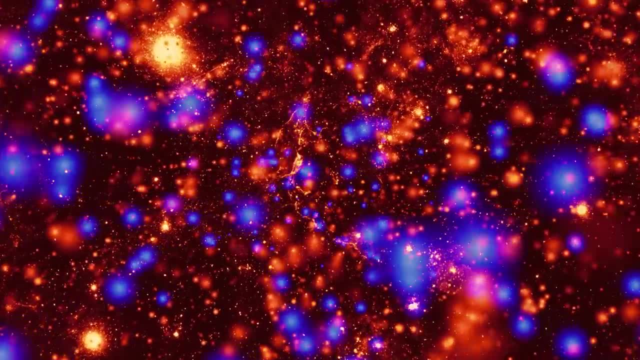 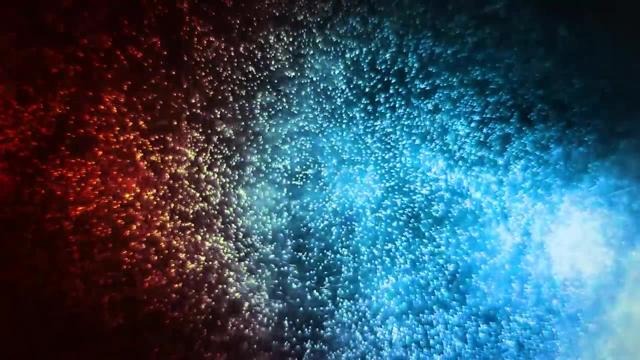 Scientists speculate that they may have existed early on, within the universe's first millionth of a second, but were still and decayed away. if they decayed preferentially into matter rather than antimatter, then this could have laid the foundation for matter's ultimate triumph. 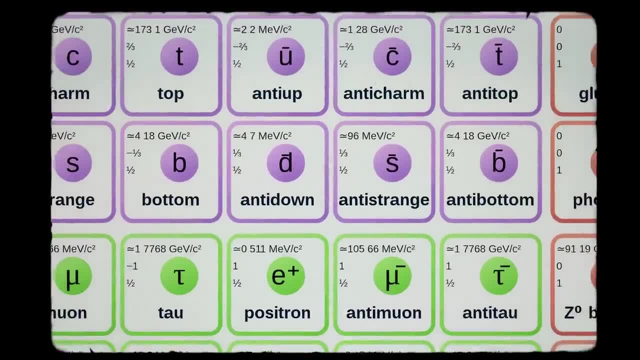 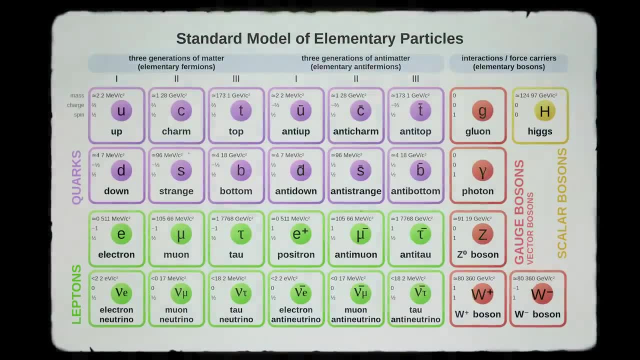 The theory is a tantalising one, but unfortunately there is not much that can be done to prove it. until we know more about these mysterious missing neutrinos- And it won't be until the universe is one second old- that neutrinos will have anything to tell us at all- 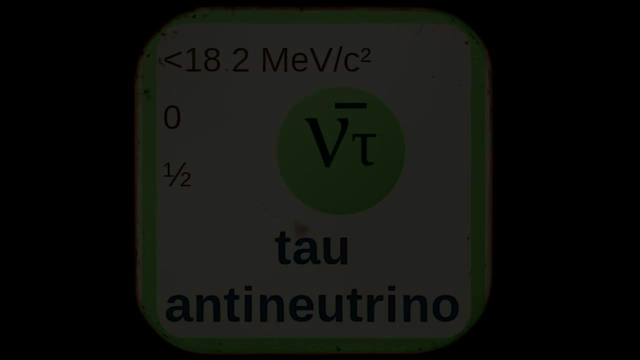 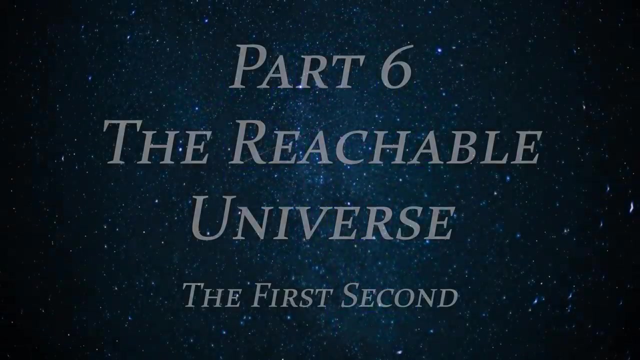 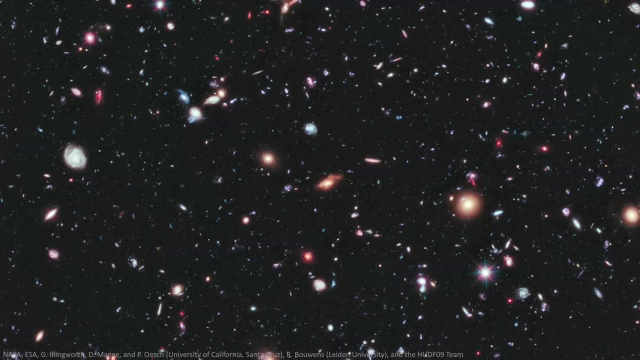 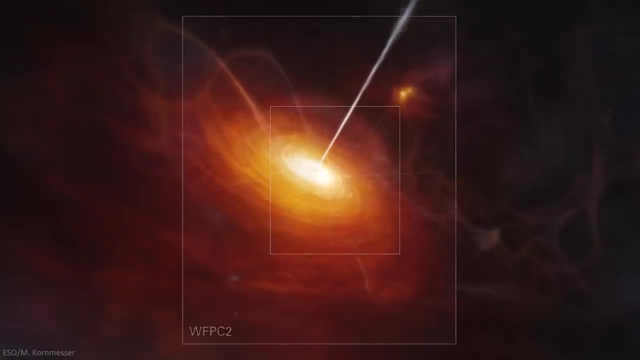 When we peer into the deepest reaches of the night sky, we are greeted with wonders. in almost every wavelength There are delicately curled galaxies, colourful nebulae and piercing points of light known as quasars. far distant, supermassive black holes swallowing matter and light at the centres of galaxies. 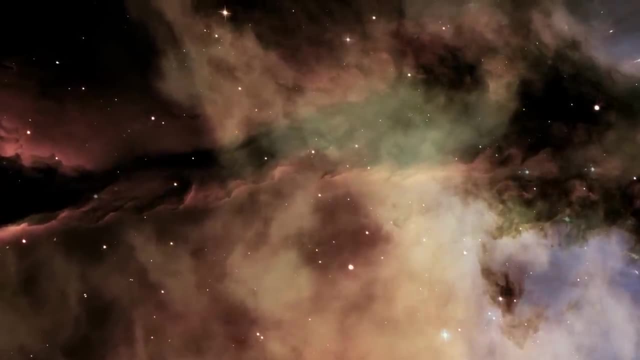 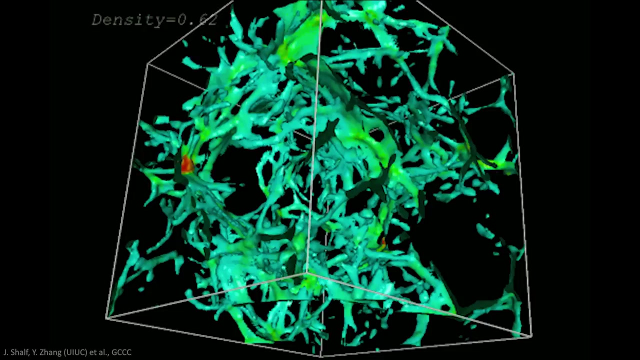 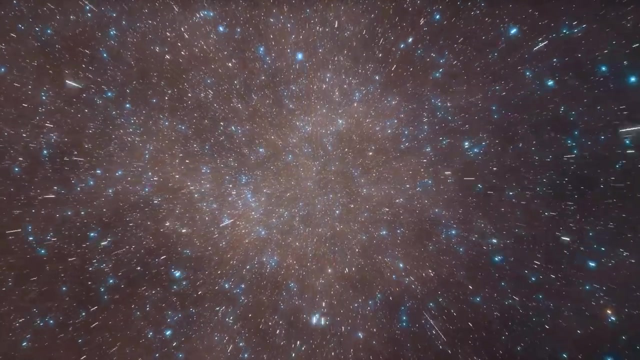 But these quasars also illuminate another curious feature that permeates deep space, known as the Lyman Alpha Forest. The constant speed of light through the expanding vacuum of space means that the more distant an object is, the older it is as well. So when we see quasars at great distances, 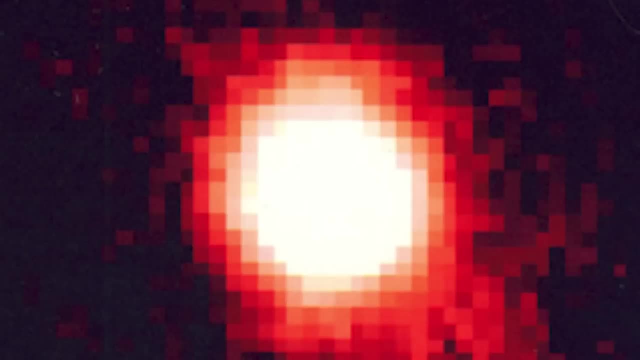 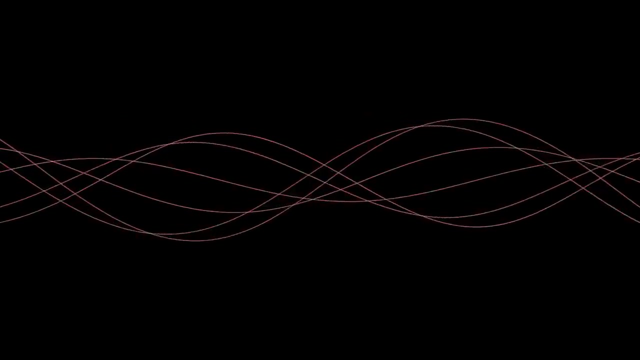 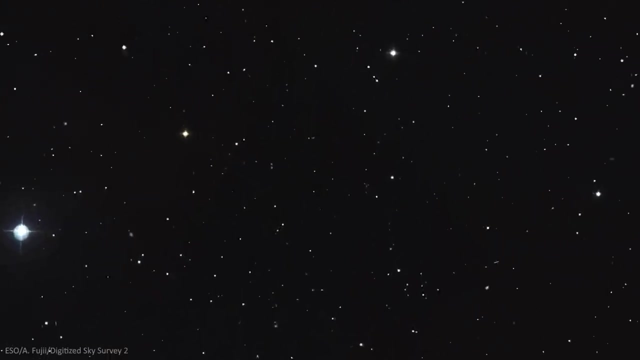 we are seeing them as they appeared billions of years ago and the light they emit is redshifted, stretched into the red parts of the electromagnetic spectrum compared to how they would normally appear. But when we examine the spectral signatures of such distant and ancient quasars, there is more to see than just 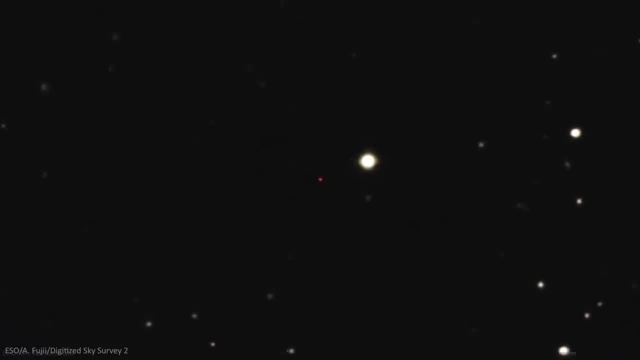 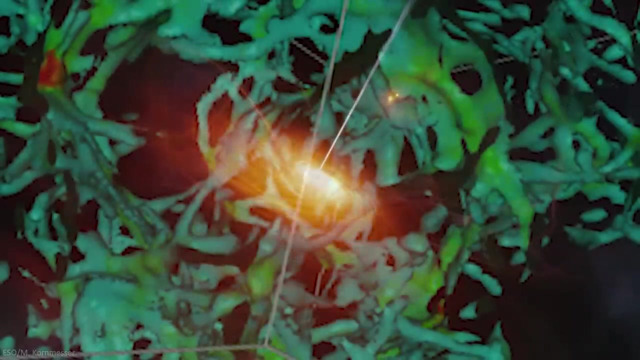 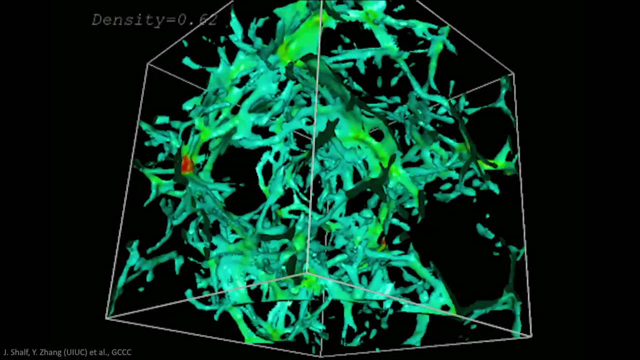 the redshifted light they give off At shorter wavelengths. there are also sharp dips in the light we see, and sometimes so many that they cluster thickly like a dense thicket of tall pine trees on an alpine mountainside. This is the Lyman Alpha Forest and it's created not by trees but by low density. 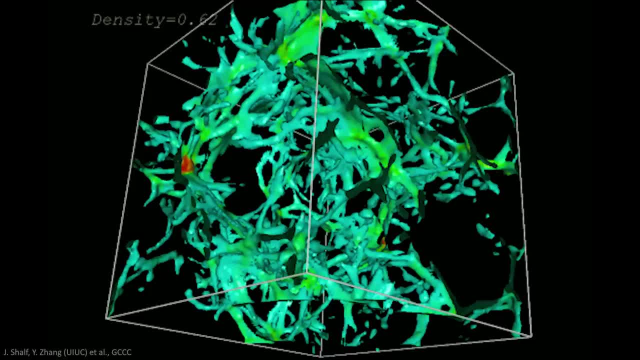 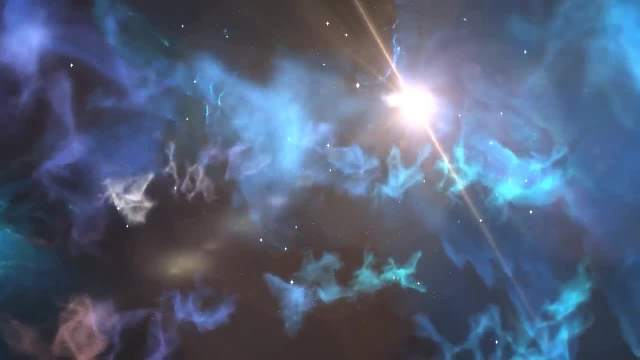 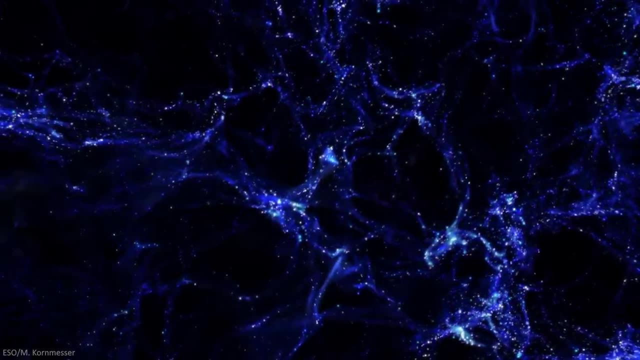 clouds of hydrogen gas lurking in intergalactic space, Because when light passes through a cloud of hydrogen, some of it is absorbed, leading to a dip in the spectrum that we eventually intercept here on Earth. And this is what is happening with the light from distant, ancient quasars. 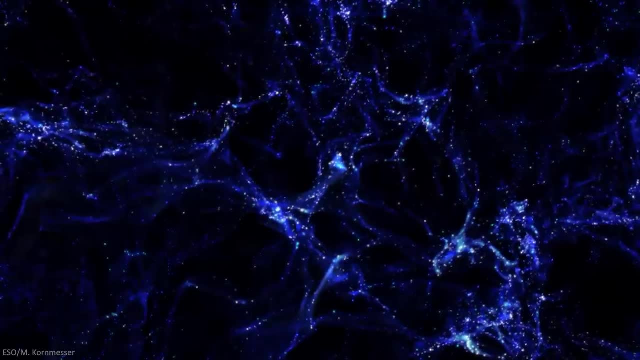 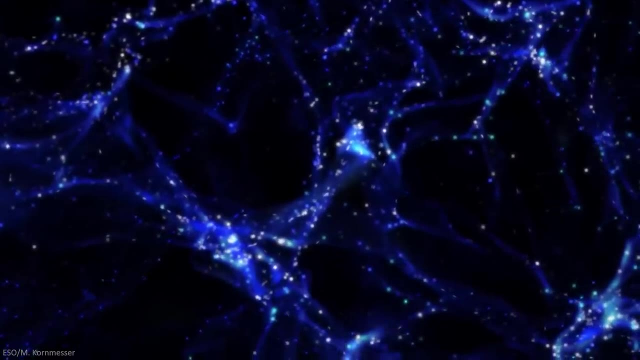 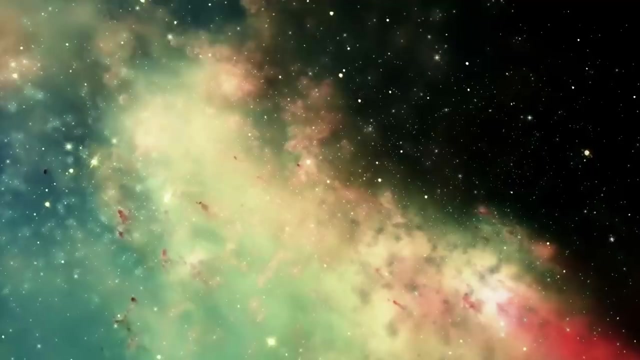 with every dip in the spectrum corresponding to an otherwise invisible hydrogen cloud. Visualizing these tenuous structures is remarkable enough in itself, but there is more we can tell from the structure of this spectral forest. Astronomers have noticed that the absorption dips cluster most thickly at high redshifts. 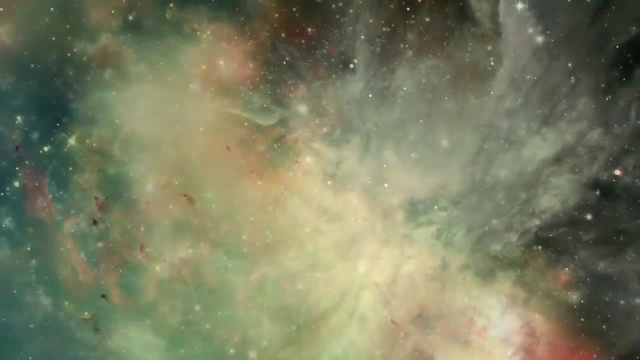 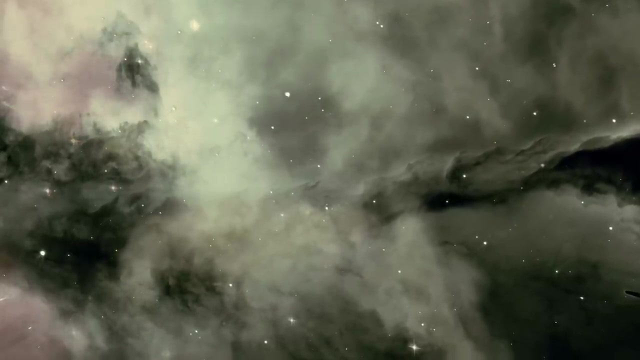 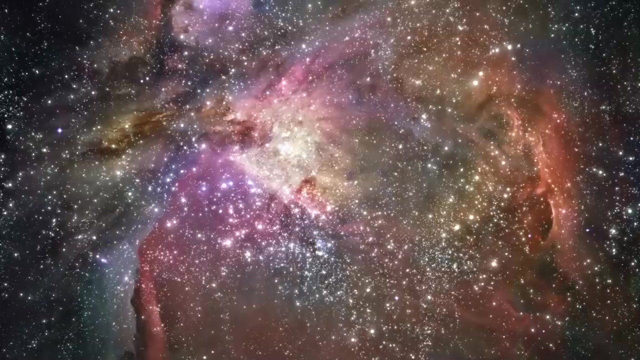 which correspond to great age, giving us an insight into the chemistry and composition of the earliest universe Compared to today. early space was full of these low density hydrogen clouds, such that it became impossible for the quasars light to avoid them. And it was that hydrogen. 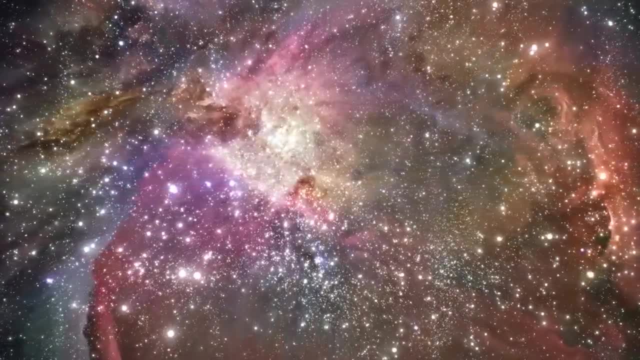 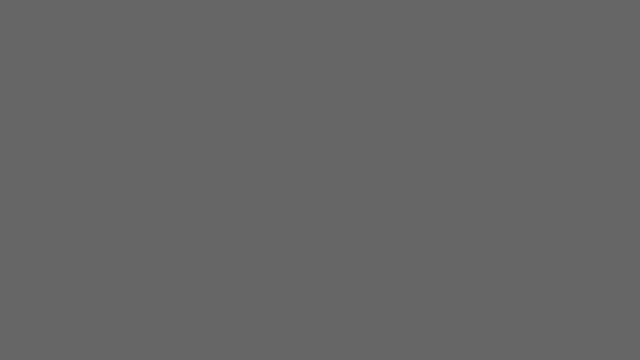 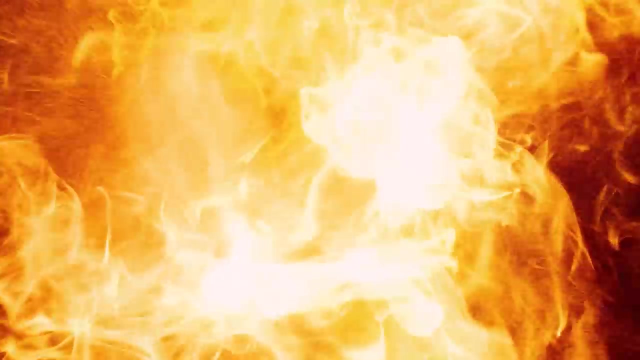 that became the nursery for stars and galaxies and was itself seeded in the first moments of the universe's existence. By the time a single second has passed in the history of the universe, a great deal has happened. It is now a mere 10 billion degrees Celsius. 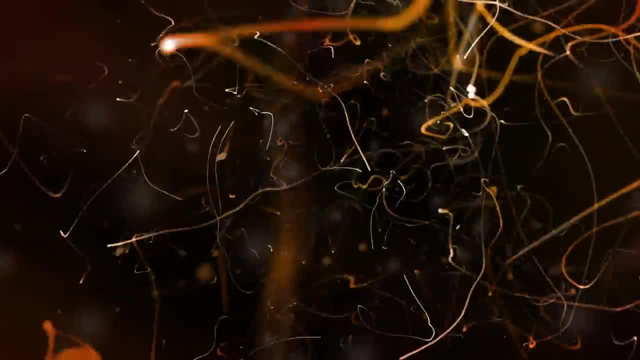 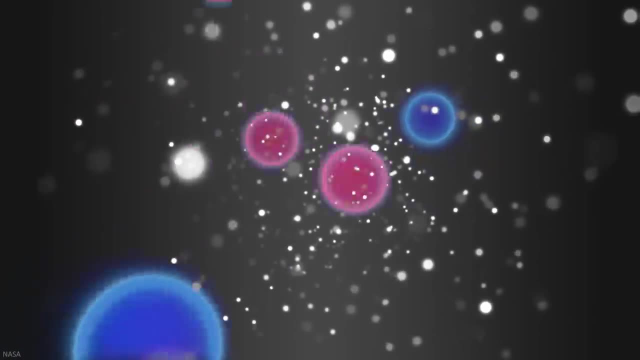 It is filled with the victors of ruthless particulate battles, along with the energetic photon shrapnel of countless mutually destructive encounters. Through quirks in the properties of the remaining particles, the balance between protons and neutrons is set as the era of spontaneous. 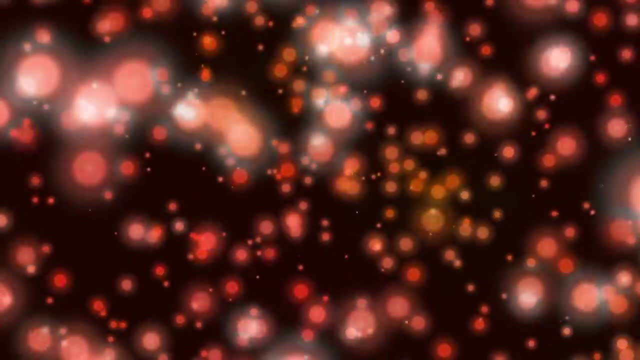 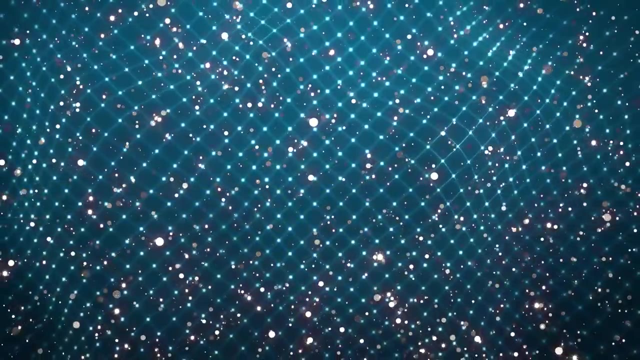 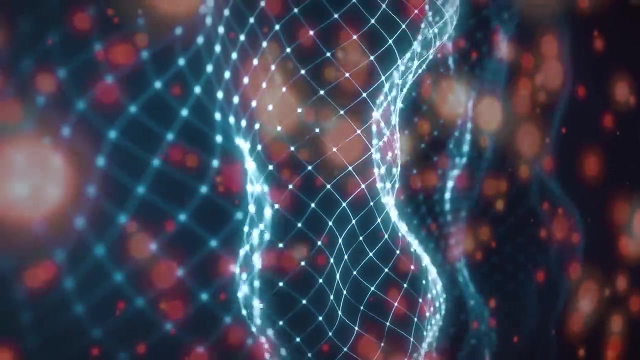 particle births and swaps is finally brought to a close. Those particles that possess mass today are already endowed with it, thanks to the Higgs field and the four forces that rule our lives today- The strong nuclear force, electromagnetism, the weak nuclear force and gravity- are now in full and comprehensible operation. 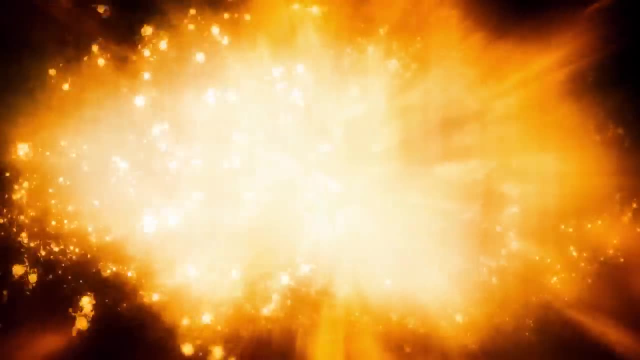 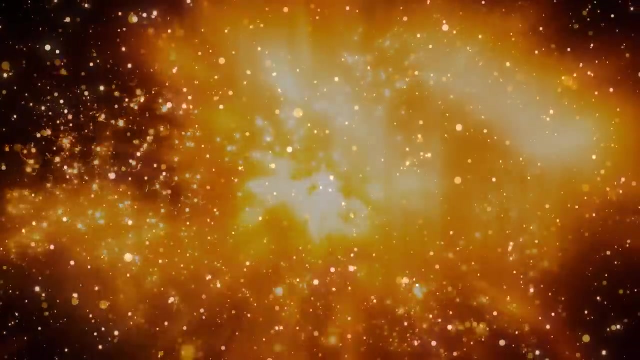 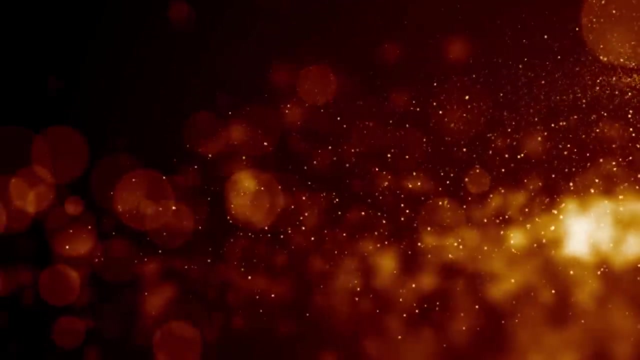 So far, the workings of the one second old universe has lain primarily within the realm of theoretical physics, with our most powerful instruments still struggling to generate the kinds of energies that prevailed within those first moments. But we are now entering an era of the universe that can be studied more. 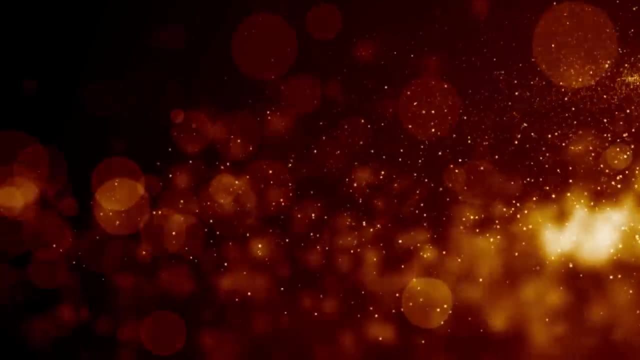 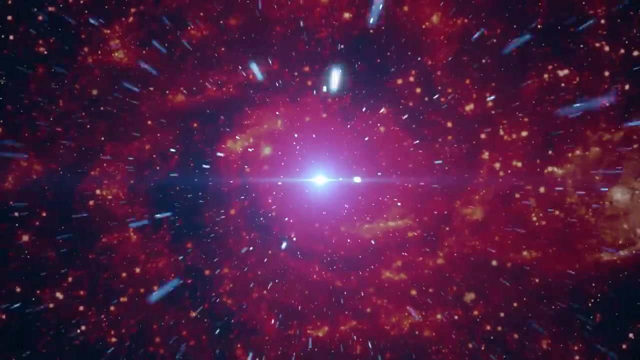 meaningfully by experimental physicists and even astronomers, We are finally reaching a part of our cosmological history that we can hope to observe, And it is only then that we can finally reach a point in our cosmological history that we can hope to observe. 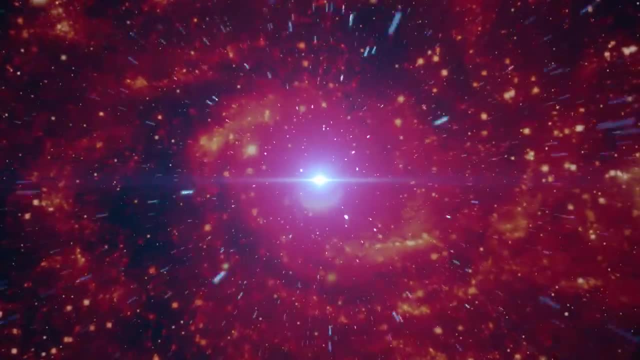 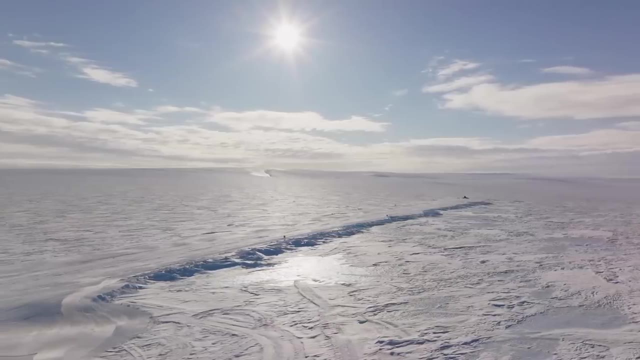 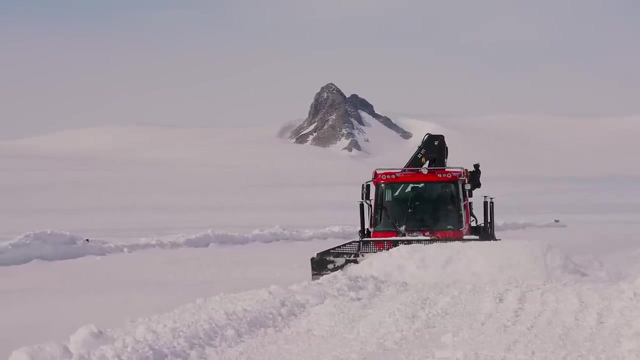 And it is only then that we can finally reach a point in our cosmological history that we can hope to observe, and even map In, the icy wastes of Antarctica. for a couple of weeks a year, the sun does not set, And this is where the work started. 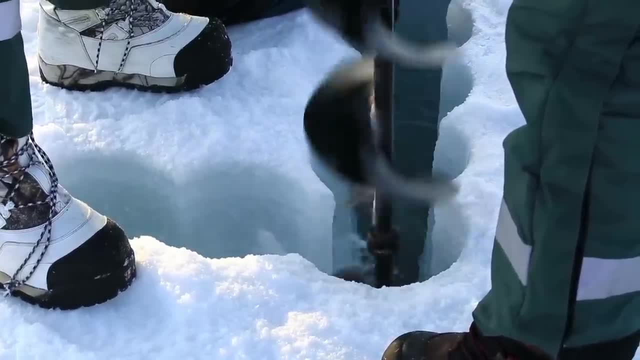 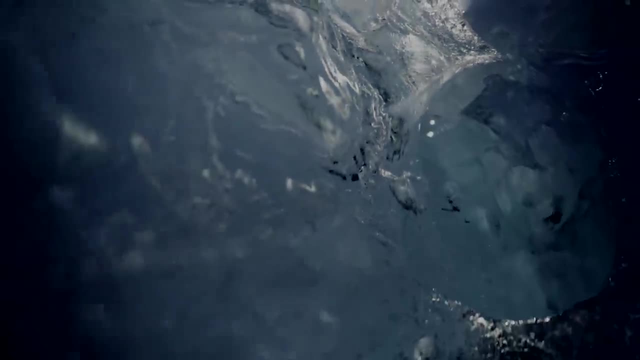 Spraying hot water directly downwards into the ice. in January 2005,, scientists working on the cutting edge IceCube neutrino observatory began the arduous, 58 hour long process of creating the first 2.5 kilometer hole needed. 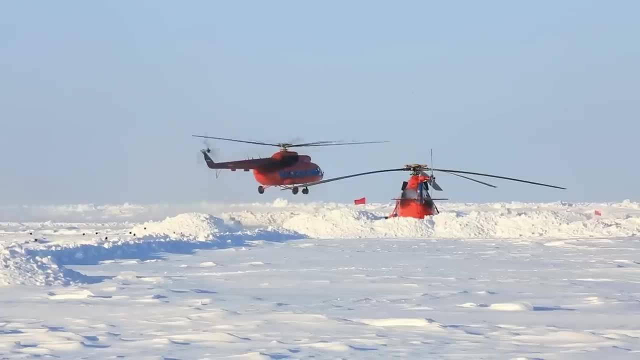 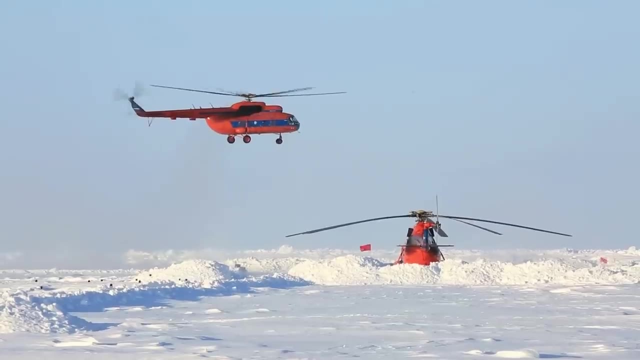 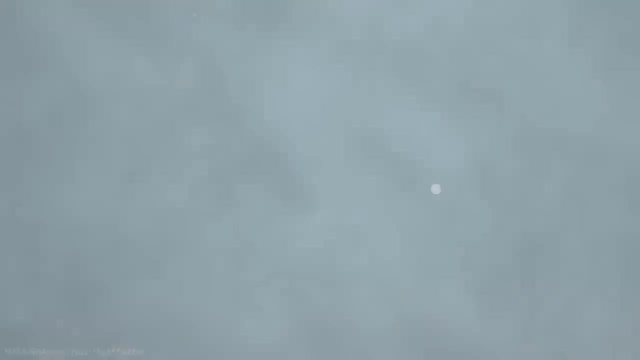 the first of 80.. Now the IceCube array's various holes occupy a square kilometer of Antarctic ice. But this immense size and improbable location aren't the only surprising features of this next generation telescope. For instead of pointing up into the night sky, 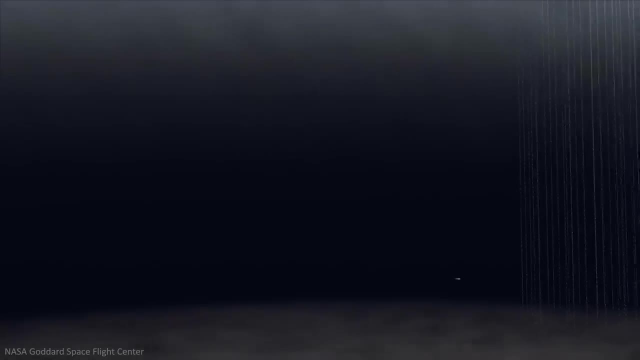 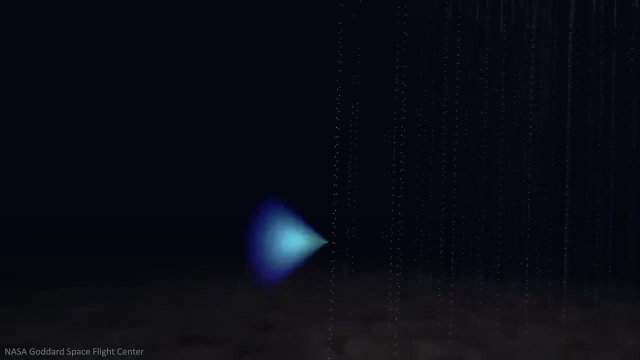 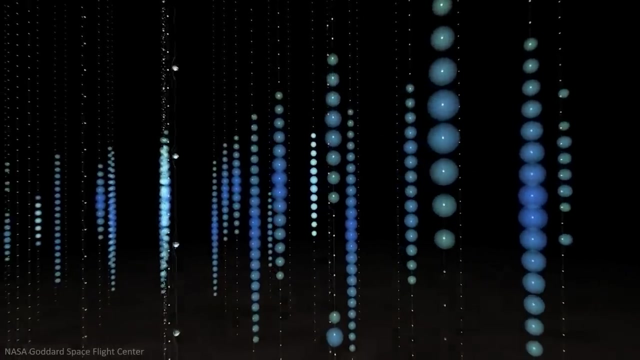 it stares down into and through the bowels of the Earth. It has no lenses, mirrors or radio dishes, but instead is made up of over 4,000 modules dangled on over 80 strings deep in holes in the ice, hanging like pearls in the cold, dark Antarctic depths. 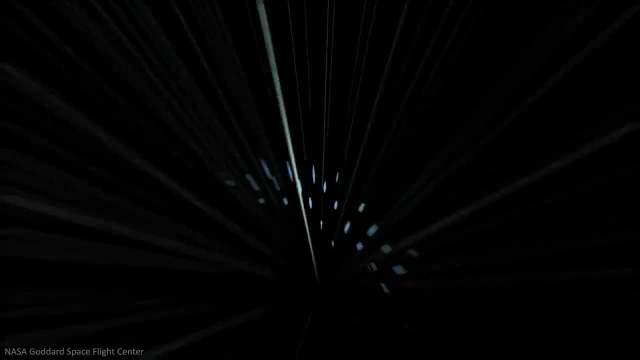 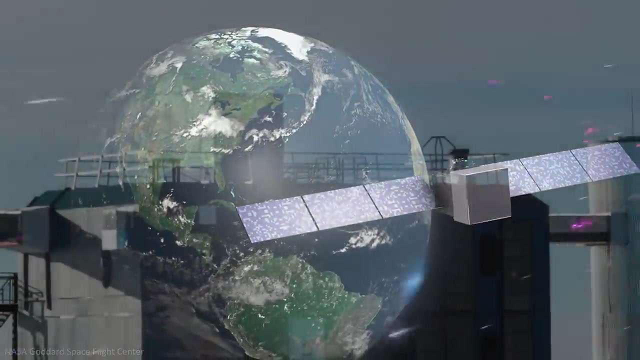 As counterproductive as this may sound, it is in fact the ideal kind of construction for observing one of the most elusive particles in the entire universe, And the IceCube Neutrino Observatory is joined by similar projects at the bottom of the ice cube. 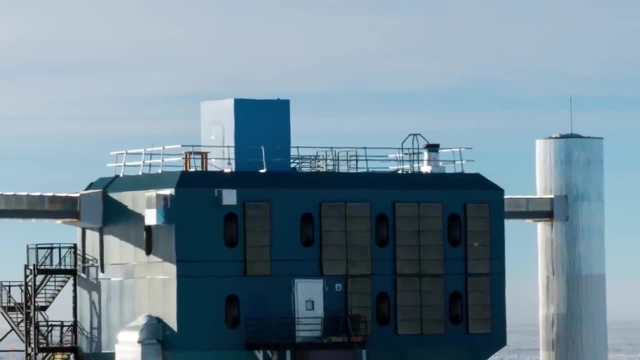 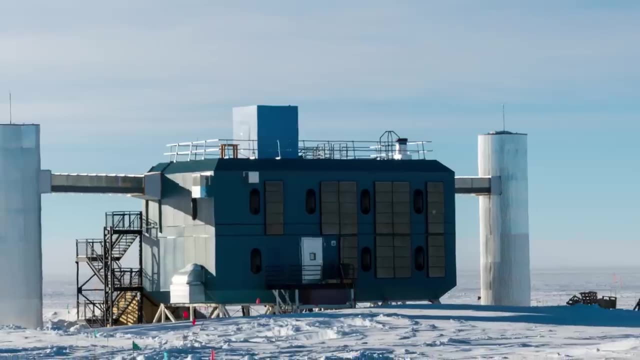 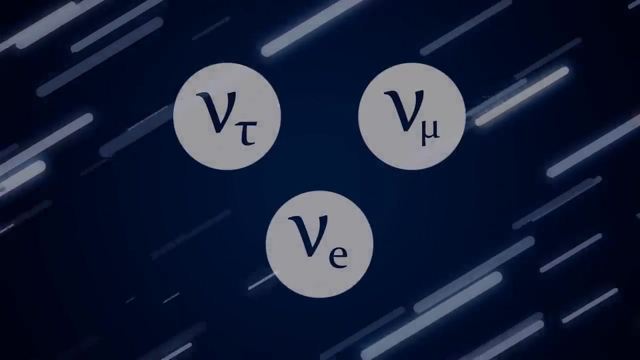 in the middle of gold mines, deep beneath the world's largest lake and in the hearts of Japanese mountains, all dedicated to the search for the mysterious neutrino. As a particle, the neutrino was first proposed in the 1930s, when particle physicists were balancing 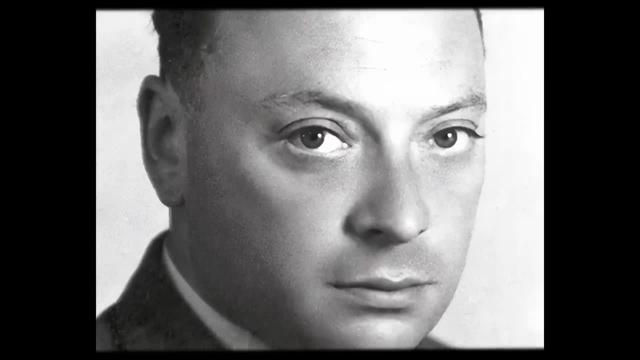 the equations of nuclear decay. Observing how a neutron would sometimes spontaneously decay into a proton and an electron, Wolfgang Pauli noticed that a tiny amount of energy was missing, which he hypothesized was another kind of particle, too small, lightweight and ghostly for us. 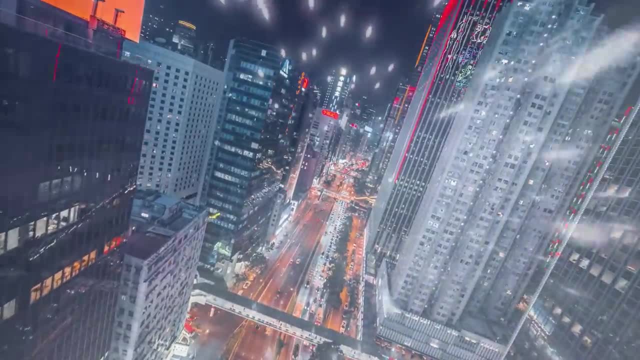 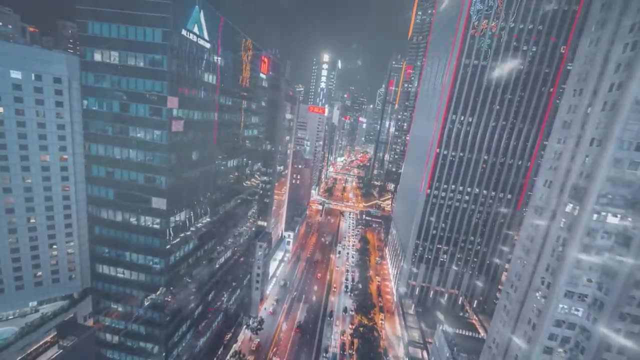 to have any hope of detecting it. Indeed, with the frequency of this kind of nuclear decay, 100 trillion of these ghostly particles must be streaming through our bodies every second, without us having any notion of their passage. But scientists do not accept defeat that easily. 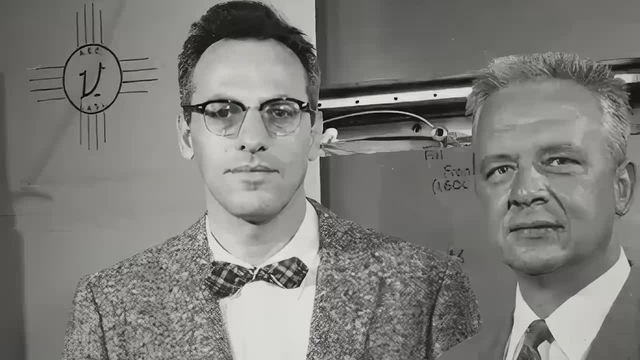 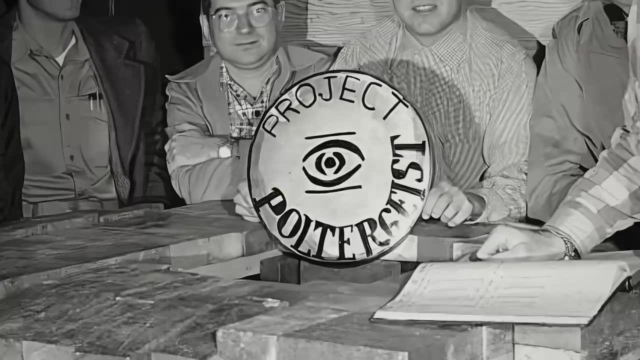 And in 1951, a pair of American physicists, Clyde Cohen and Frederick Raines, began to search for it And in what became known as Project Poltergeist, they turned to powerful nuclear fission reactions to provide the vast quantities of energy needed. 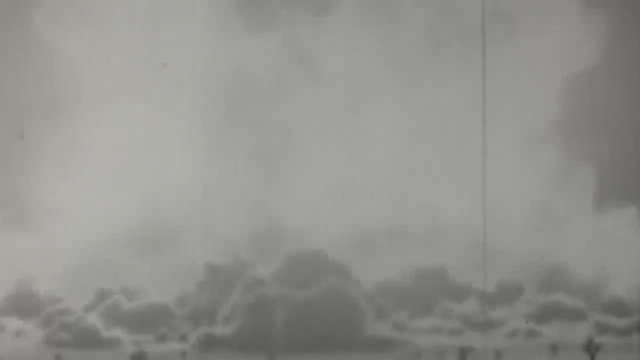 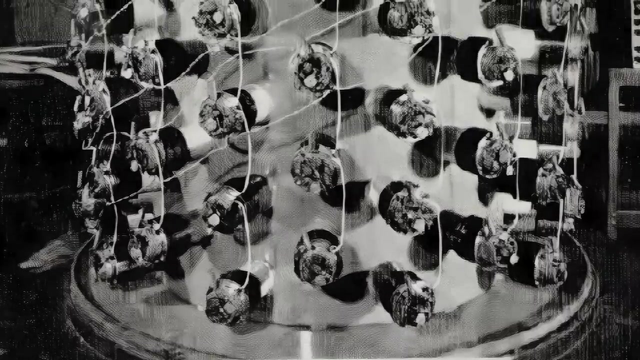 to detect neutrinos. Cohen and Raines first proposed detonating a 20 kiloton nuclear payload and installing an immense detector just 50 meters away from the blast. This detector, nicknamed El Monstro, was designed to pick up a flash of light. 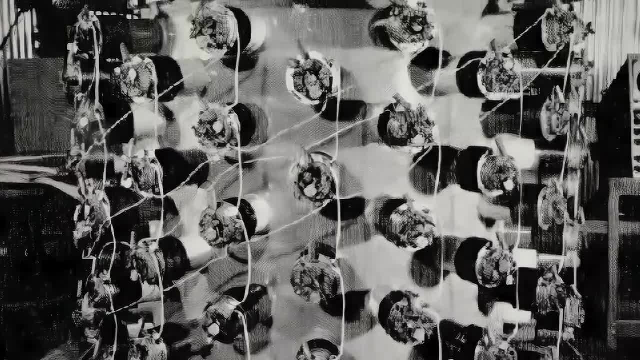 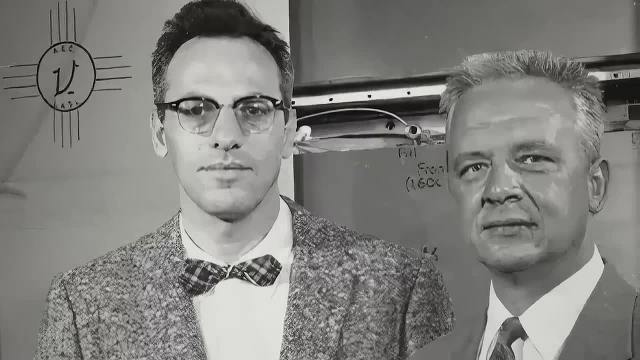 after a neutrino collision, And if it had been built with a single shot, it would have been almost a thousand times larger than any previous detector. In the end, however, this experiment proved too challenging and the scientists turned to the somewhat more controlled 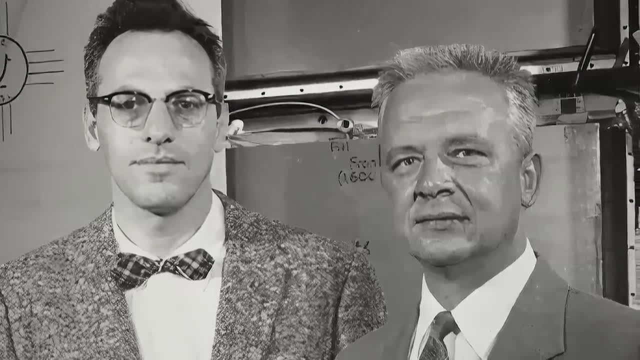 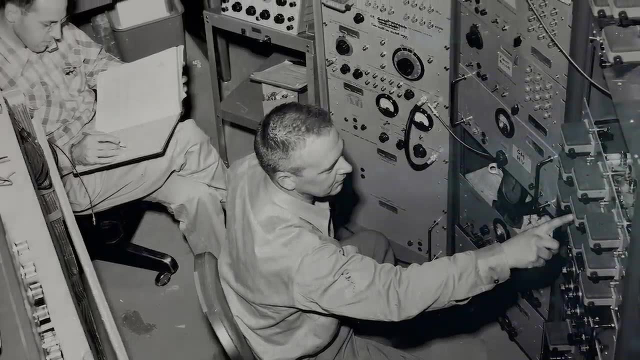 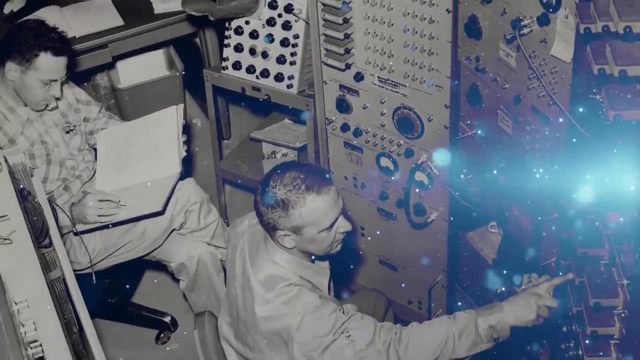 energy release to be found in nuclear reactors. And so, in 1956, Cohen and Raines' experiment succeeded, finally achieving the seemingly impossible: detecting the ghost particle that had been haunting physics for more than 20 years. These days, the production and study of neutrinos has advanced greatly. 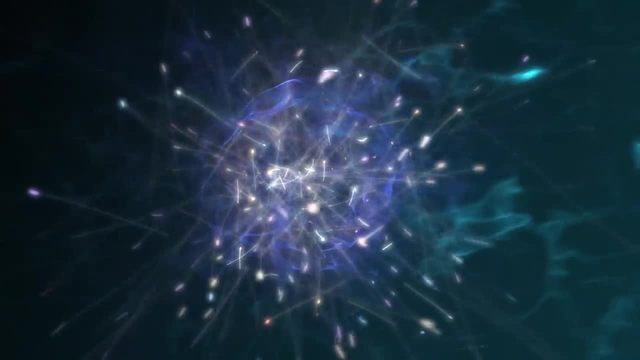 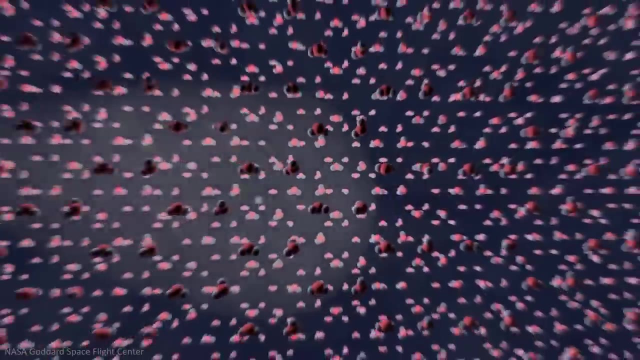 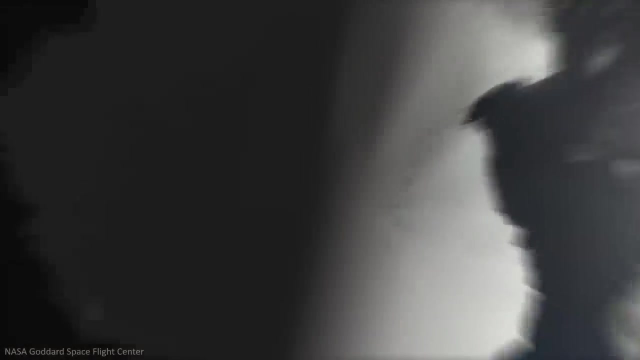 and scientists are now able to produce and study them in powerful particle accelerators, although there is still a place for monstrous detectors like the one in Lake Baikal, For neutrinos can be used to answer not only questions about our universe today, but also its very first moments. 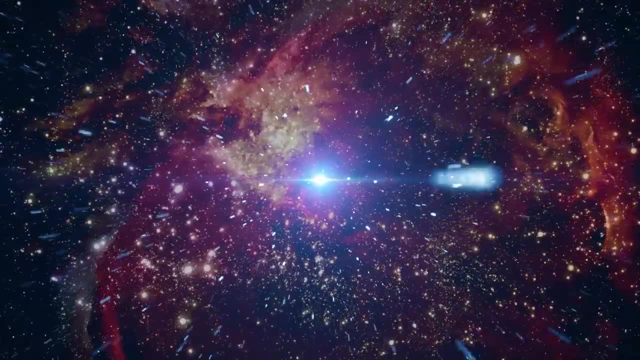 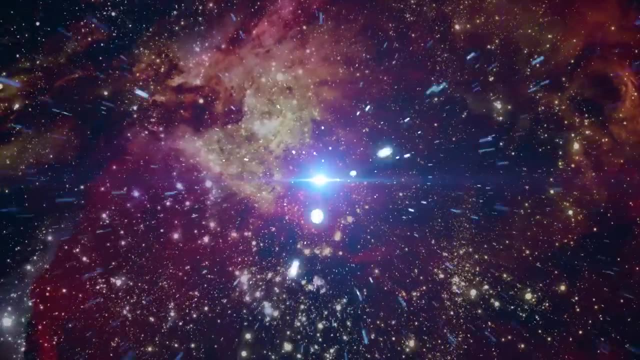 Neutrinos are produced in such quantity by such a variety of electromagnetic sources that scientists can't even imagine how many of them there are. Scientists are trying to use them to study some of the most extreme events in the modern universe One hundred and sixty-eight thousand years ago. 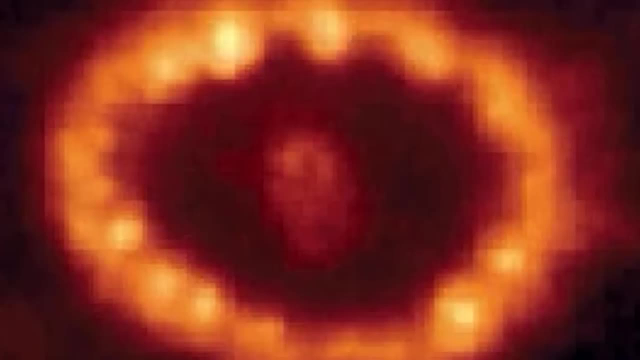 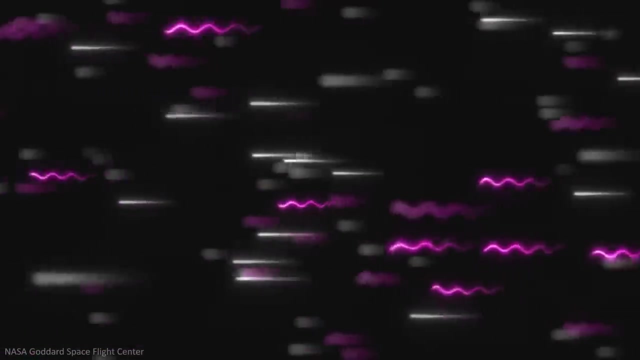 a star within the Large Magellanic Cloud went supernova. The explosion sent atomic shrapnel reeling across intergalactic space at nearly the speed of light. This shrapnel including the countless neutrinos that were emitted in the blast. 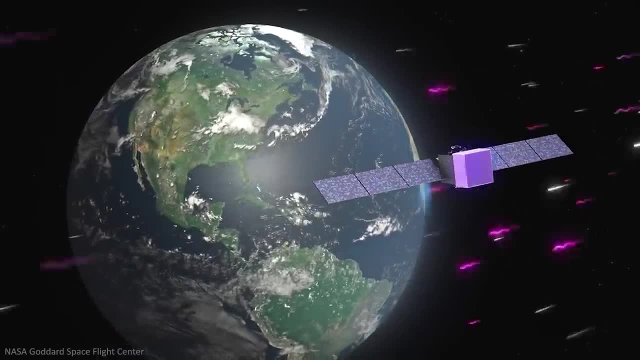 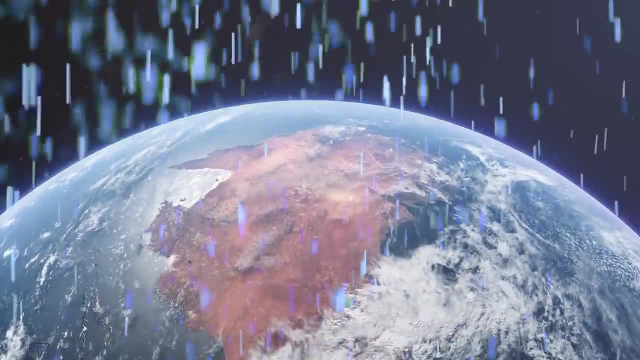 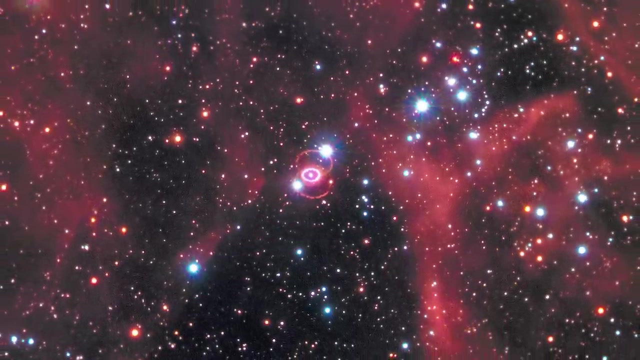 struck the Earth in 1987, and scientists in Japan considered themselves extremely fortunate to be able to detect eleven of these neutrinos. As insubstantial as this may seem, the fact that astronomers could see the supernova through this neutrino lens helped to usher in. 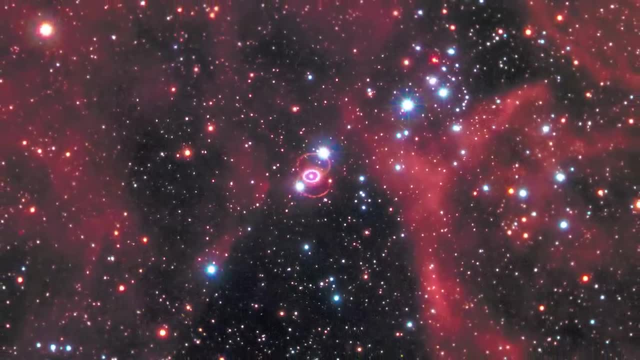 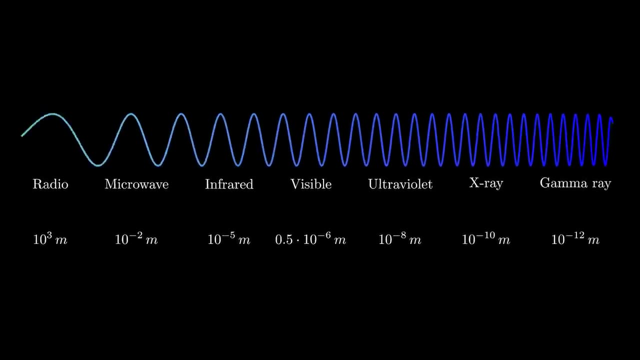 a new era of multi-messenger astronomy. Gravitational waves, telescopes tuned to a variety of electromagnetic frequencies and neutrinos could all be deployed together to study and understand the most extreme events in the world. to study and understand the most extreme events in the world. 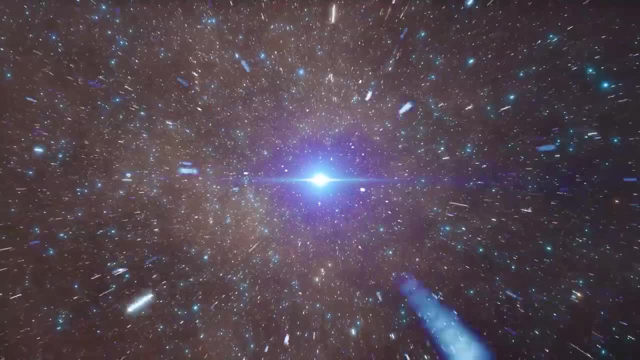 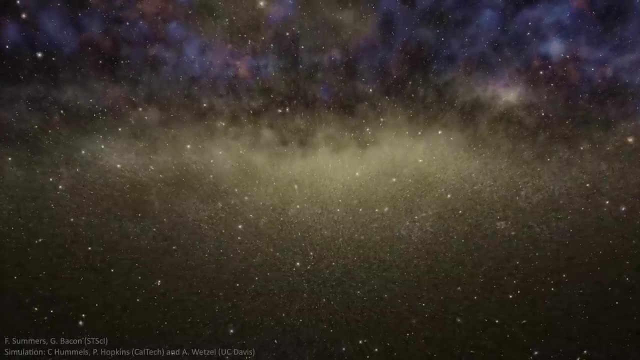 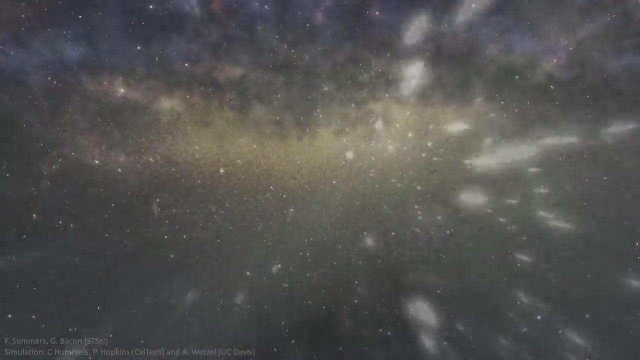 But not only that. neutrinos give us the opportunity to probe objects that are too opaque for light to penetrate, since their extreme unwillingness to interact with any matter at all sees them stream through everything from nebulae to stars and even entire planets. 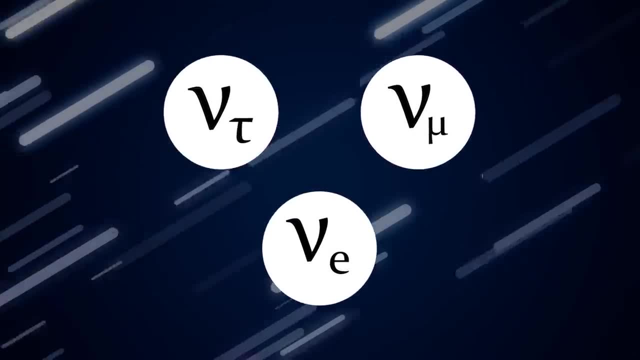 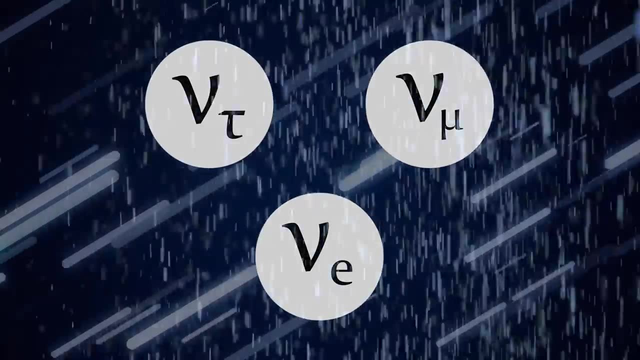 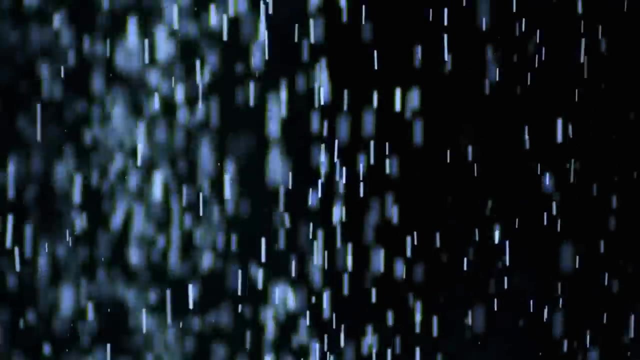 And this is because they only interact with two of the fundamental forces: the weak force and gravity, This remarkable penetrative ability, which can be called gravity penetrative ability, making them powerful tools in probing some of the earliest moments of the universe. 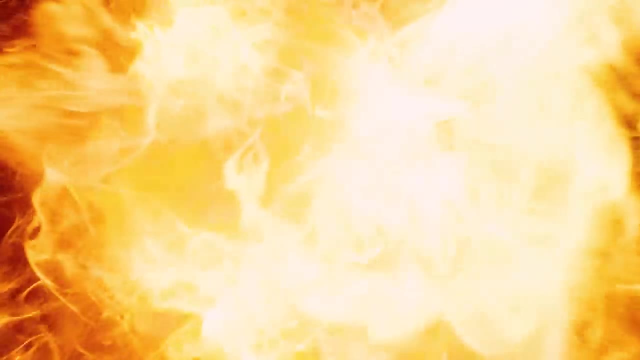 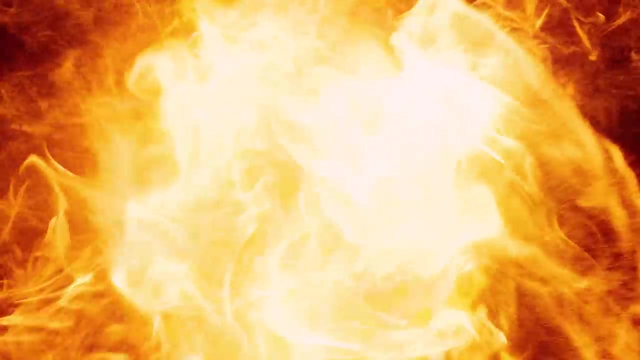 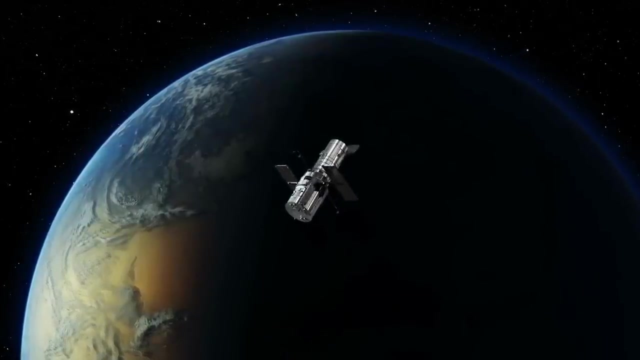 After the decisive formation of matter around one second after the Big Bang, the sheer density of hot energetic particles and photons rendered the early universe completely opaque for hundreds of thousands of years Now. telescopes which rely on the passage of photons through empty space cannot probe. 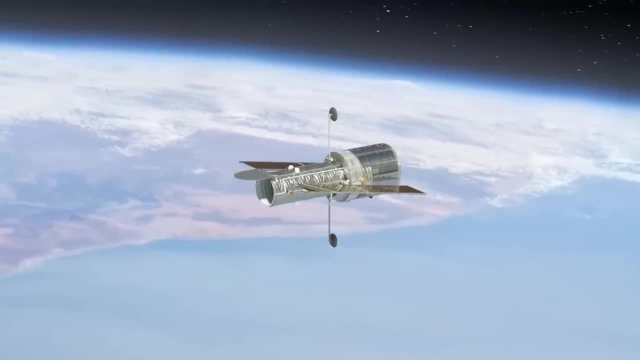 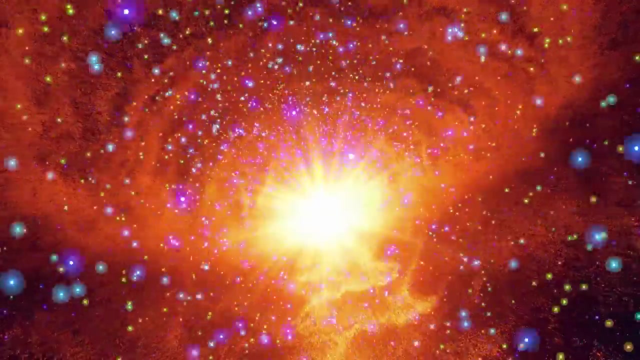 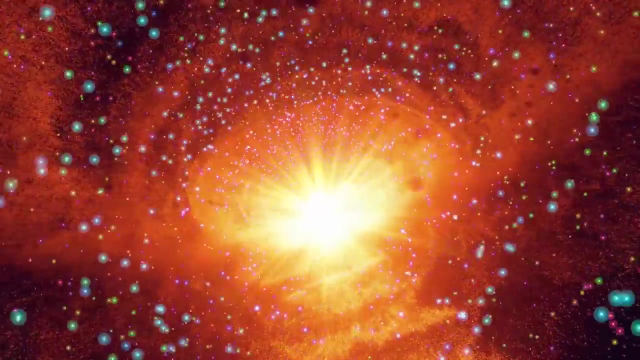 this opaque plasma, and so, to see further back in time, scientists need a different approach, And that's where the neutrino comes in. Less than a second after the Big Bang, neutrinos and anti-neutrinos were just another part of the hot cosmic soup. 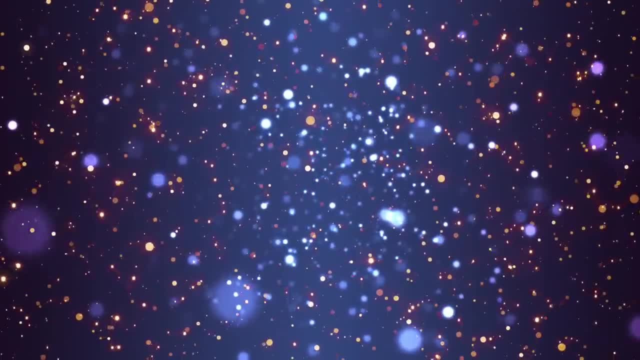 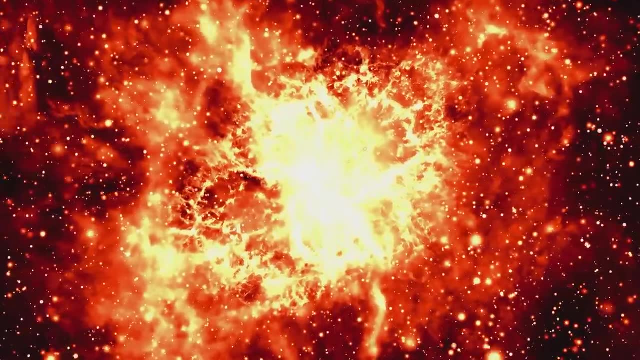 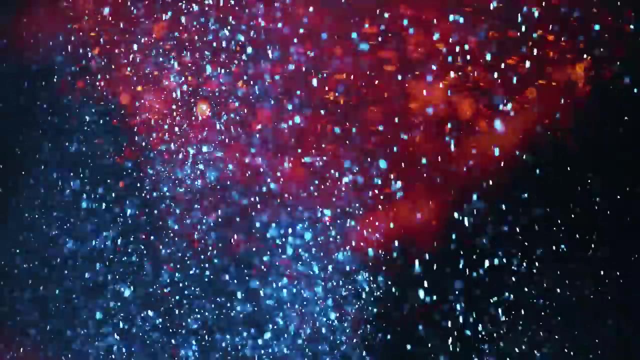 They collided and scattered, interacting with other matter because everything in the still dense universe was so energetic. But around the one second mark, temperatures in the universe dropped to 10 billion degrees Celsius and the particles correspondingly slowed. Eventually they were moving slowly enough for neutrinos to escape and find a way through. 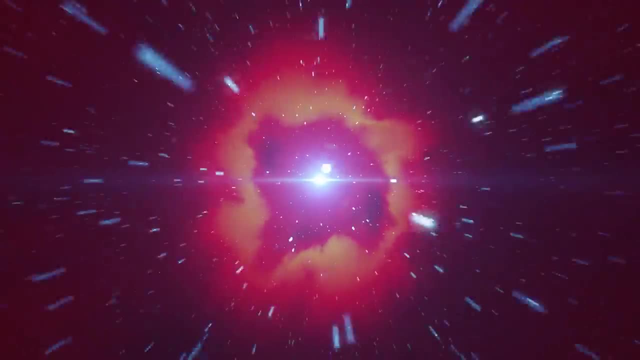 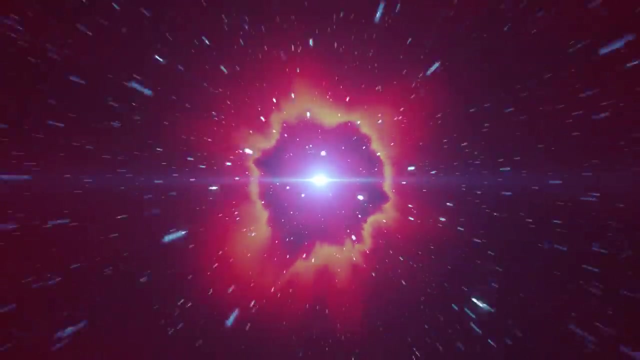 the snarl of other particles, They no longer collided with matter or light and could therefore break free to leave an imprint of their passage on the universe. And so if we could find that imprint, known to scientists as the Cosmic Neutrino, it would. 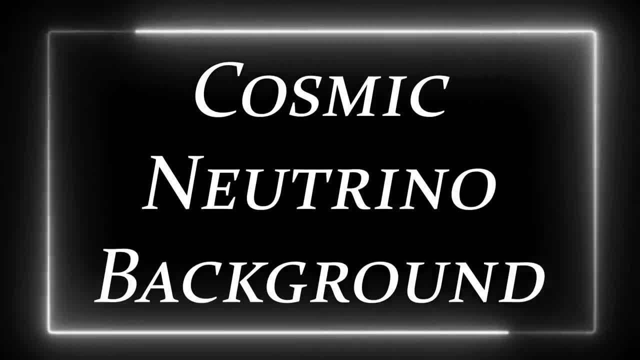 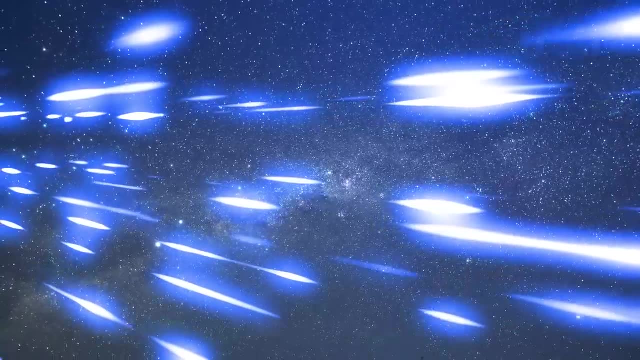 represent an image of the universe at just one second old, extending our astronomical reach back in time by some 380,000 years. But if these relic neutrinos from the first second of the universe are out there, they are even more elusive than their high energy counterparts. 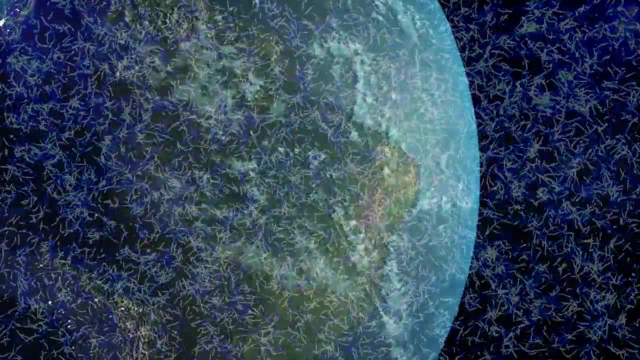 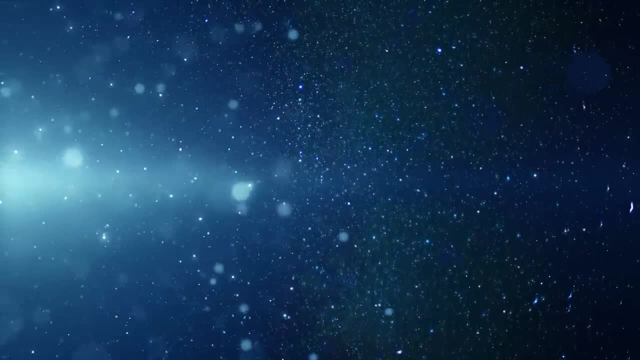 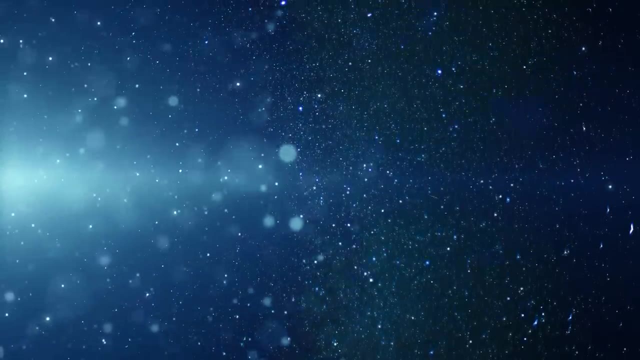 Compared to the 100 billion high energy neutrinos per cubic centimetre of space. there are thought to be just 300 from that earliest time. To detect them directly we would need to build our instruments with some billion times the current precision or somehow detect the effect they had on the cosmos when they broke. 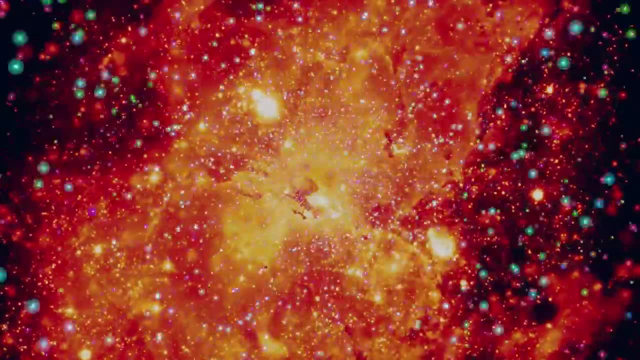 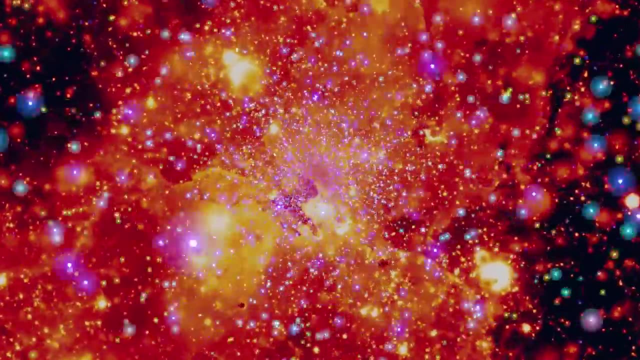 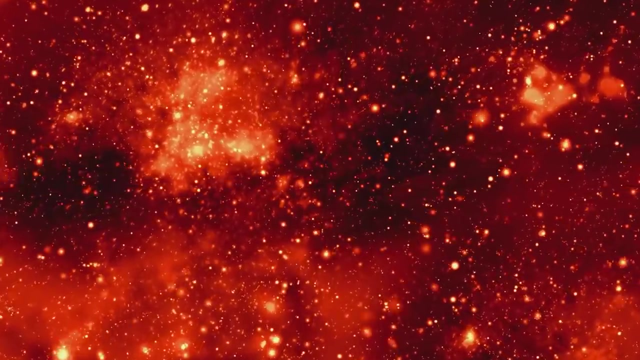 free For, as the first things to stream through the otherwise opaque cosmos, these tiny particles are expected to have left miniature sonic booms in their wake, fundamentally altering the distribution of matter and energy. Some parts of space would have become slightly hotter And some parts slightly cooler thanks to this disruption. 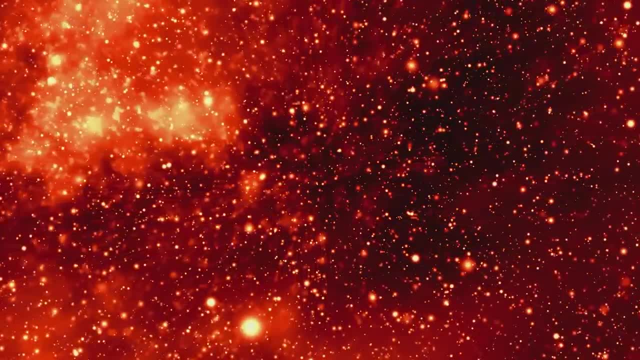 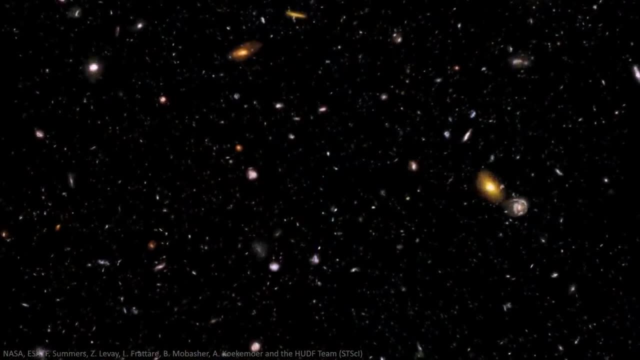 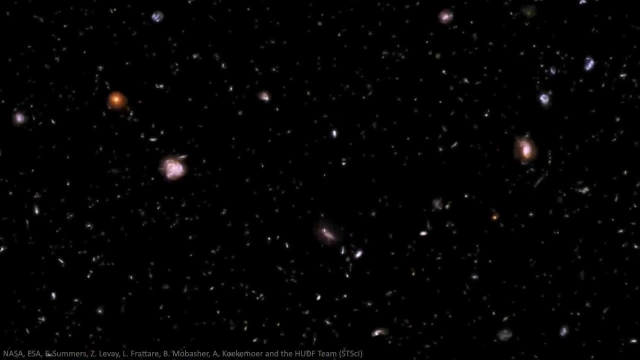 And in the intervening 13.8 billion years space has expanded, magnifying these patches into a larger scale structure in the universe. If we could decode some of that large scale structure written into the distribution of galaxies today, then we may just be able to tune into the echoes of a universe one second. 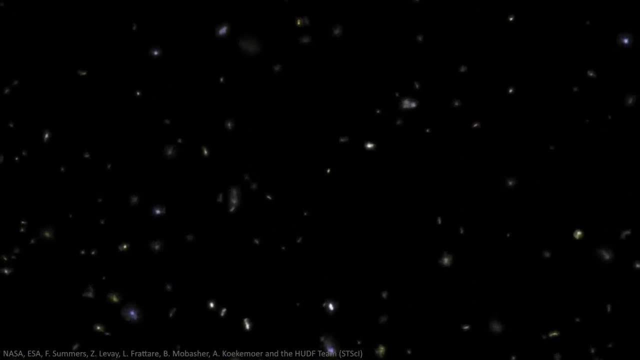 old, And this is not the only modern mystery that could happen. It could happen in the future. It could happen in the future. It could happen in the past. It could happen in the future. It could happen in the future as well. 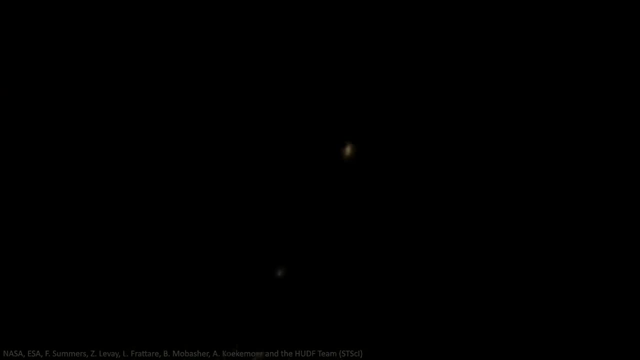 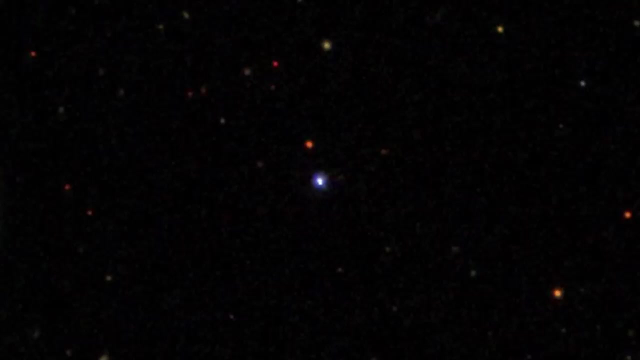 It was a mysterious discovery that could have its origins in the one second old cosmos. This is TON 618.. At some 18.2 billion light years away from us, it burns some 140 trillion times brighter than the Sun, making it one of the brightest objects in the known universe. 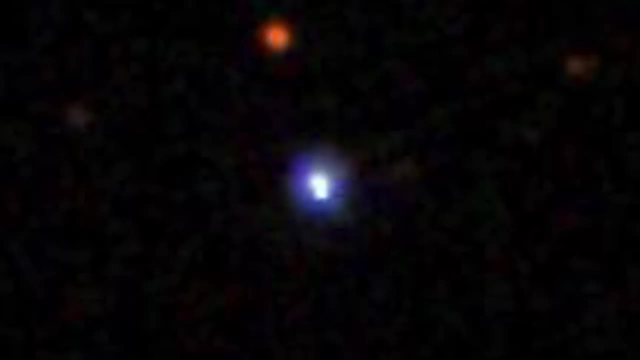 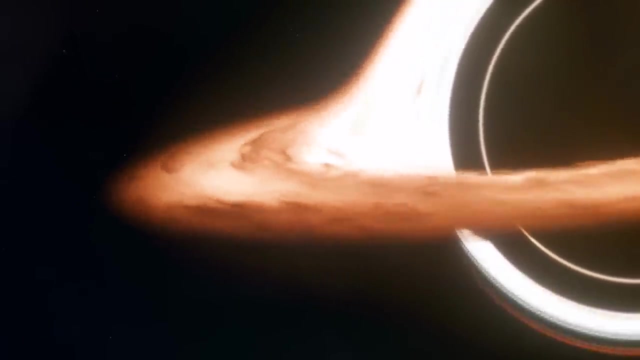 OOOH. nearly 11 billion years old. despite its incredible luminosity, it is actually one of the cosmos' biggest black holes. Understood to be a hypermassive black hole at the centre of a galaxy whose trillions of stars it far outshines, ton 618 has a mass that is some 66 billion times that of our. 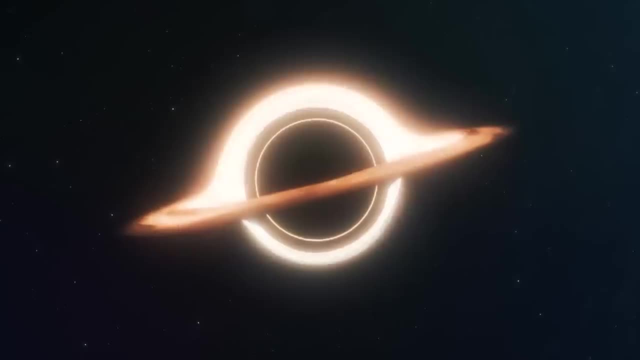 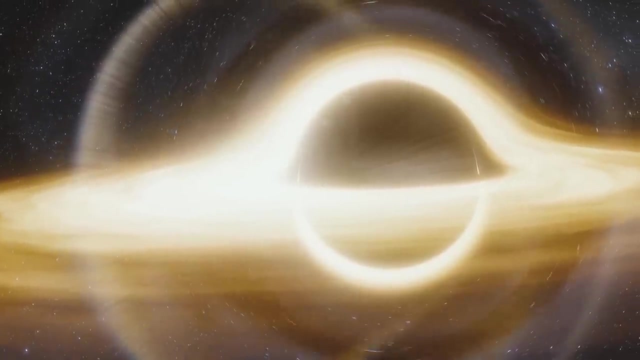 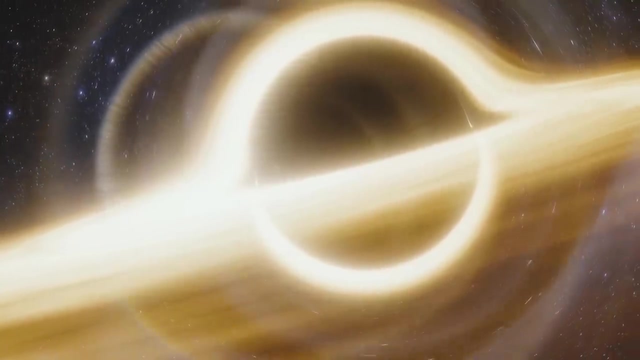 sun and is more than 15,000 times more massive than Sagittarius, A star, the black hole at the centre of the Milky Way. In fact, this single black hole is heavier than all the stars in the Milky Way put together. Matter is falling into it at speeds of more than 10,000 kilometers per second, causing 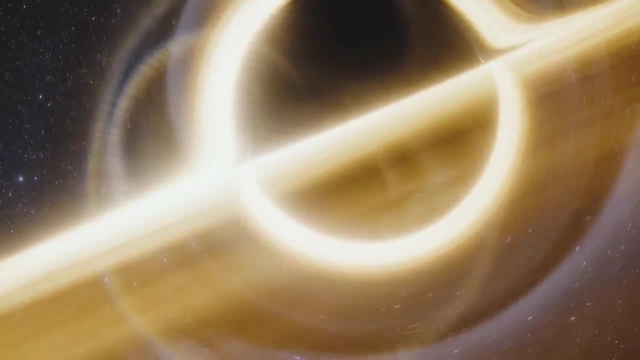 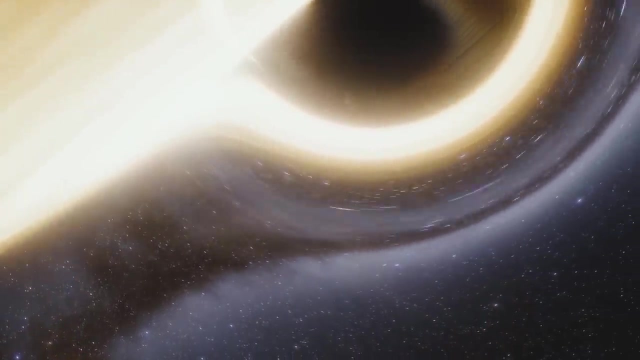 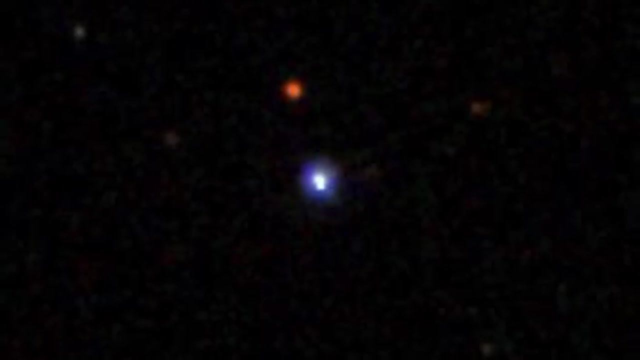 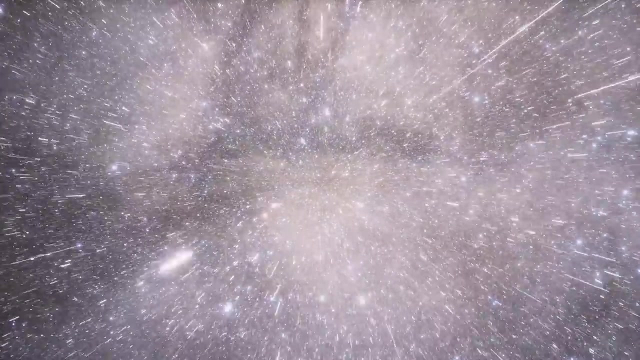 intense heating so that the doomed material in its accretion disk glows brightly, despite the light swallowing dark heart at its centre. Ton 618 may be the largest we have found, but it is by no means the only such Titan lurking. It is one of the largest galaxies in the galaxy, with a mass of more than 100,000 times that. 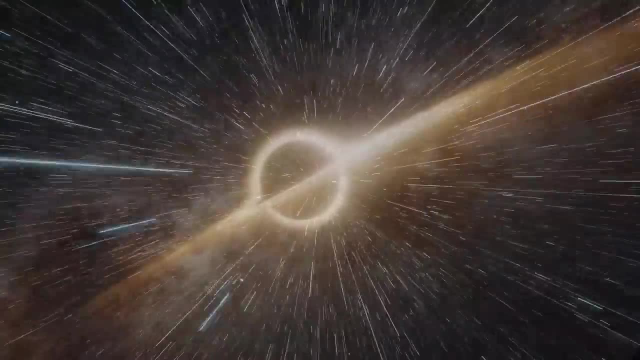 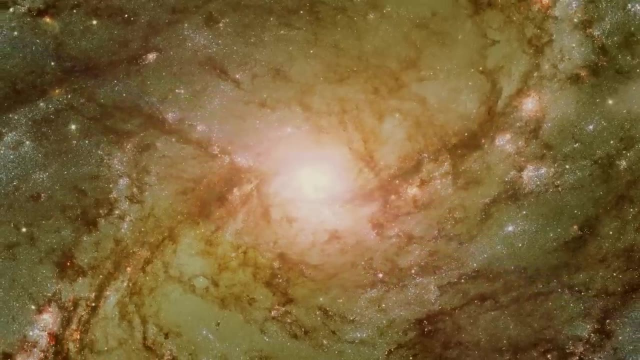 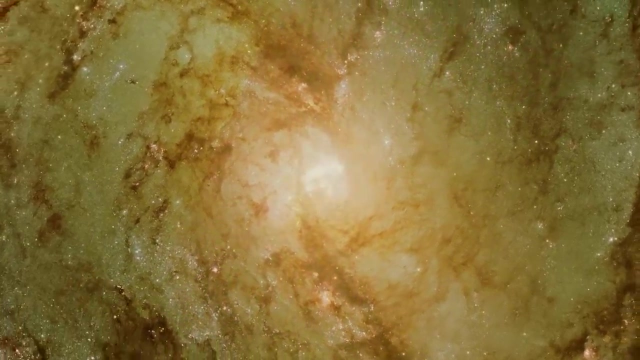 of our sun and is thought to be a major influence on how those galaxies have formed and evolved over billions of years. These hot, massive hearts themselves are thought to grow by swallowing stellar matter from their galactic entourage. But there is something about the timing of these supermassives that doesn't quite add. 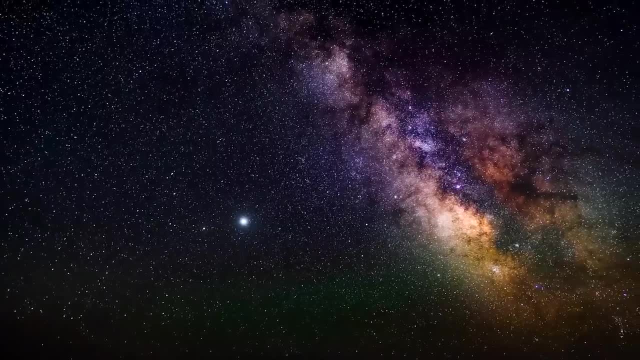 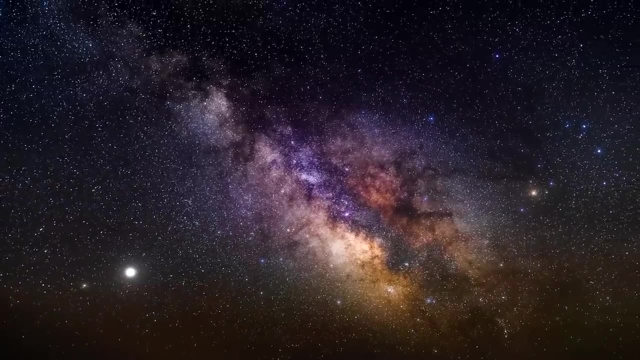 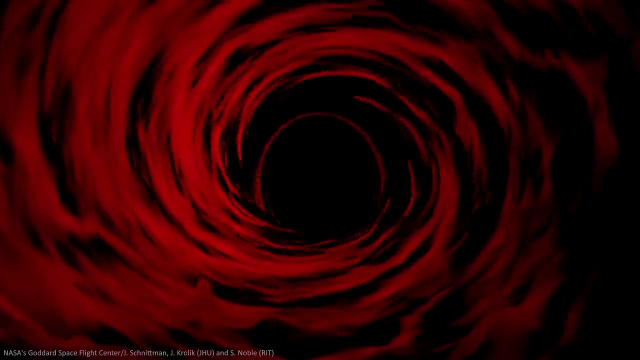 up. If we look at the sky, they find these gigantic black holes dating to just a few million years after the Big Bang. despite the fact our models do not allow for the birth and death of enough stars to feed such early giants, Some of the supermassive black holes we have found grew to a billion times the mass of 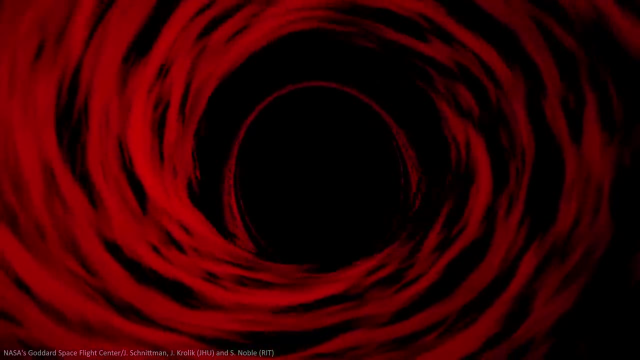 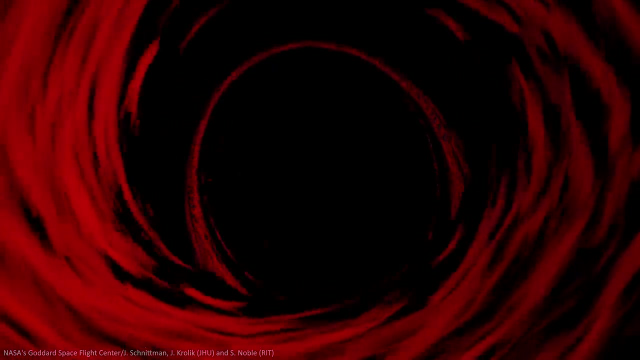 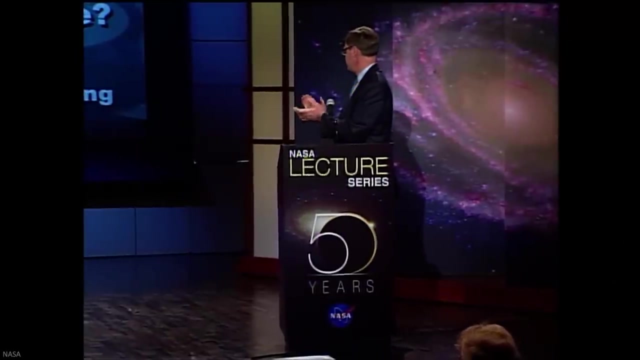 our sun by less than a billion years after universe formation, when, according to models of star formation, only around 100,000 solar masses should have been possible. A potential solution to this conundrum may be found in a theory that was developed many 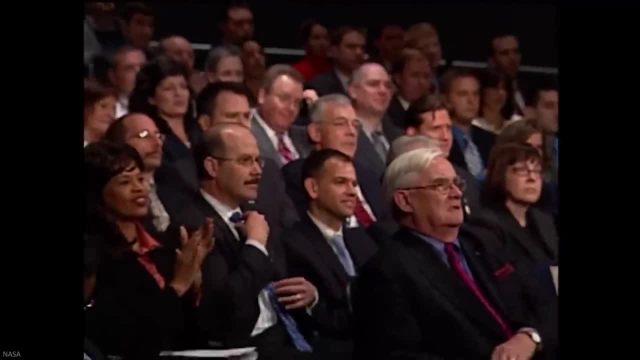 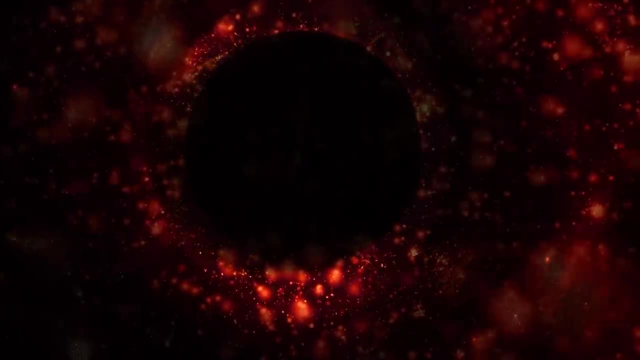 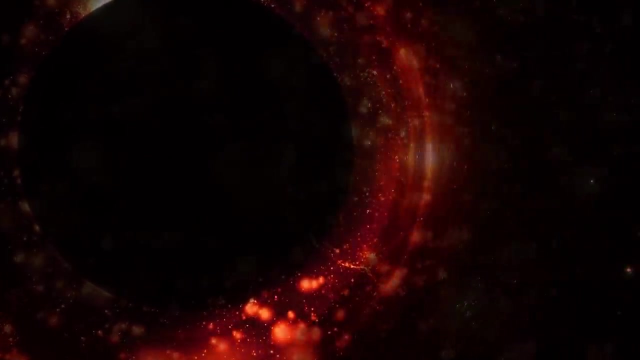 years before we were even aware of the oversized early supermassives. In 1971, Stephen Hawking proposed that there was another way that black holes could be formed without any precursor stars at all, but rather from density fluctuations in the very early universe. 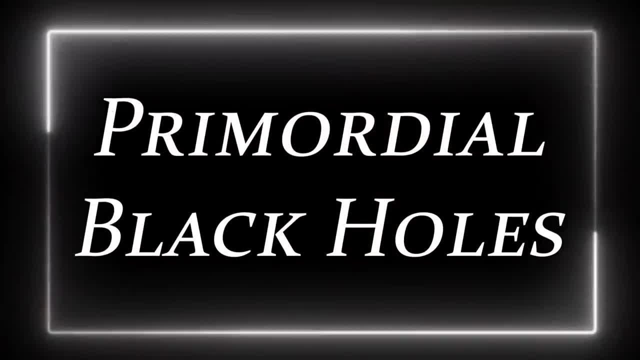 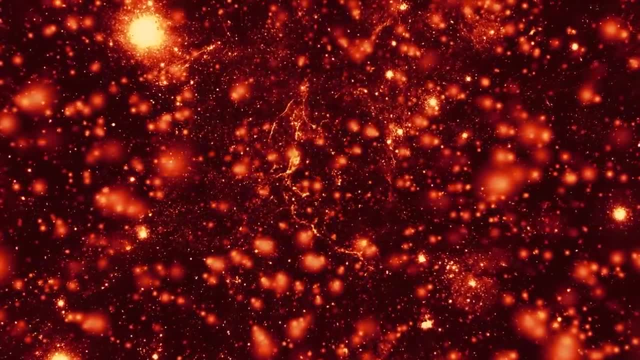 This is the theory that was developed many years before we were even aware of the oversized supermassives. He called them primordial black holes. During the radiation dominated era, when the universe was still an energetic plasma of photons and matter, major inhomogeneities- essentially lumps of matter- would have resulted. 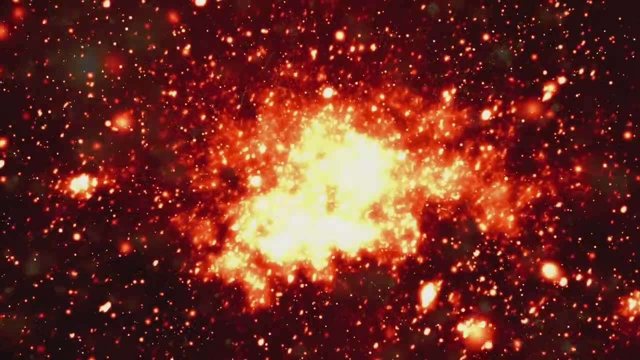 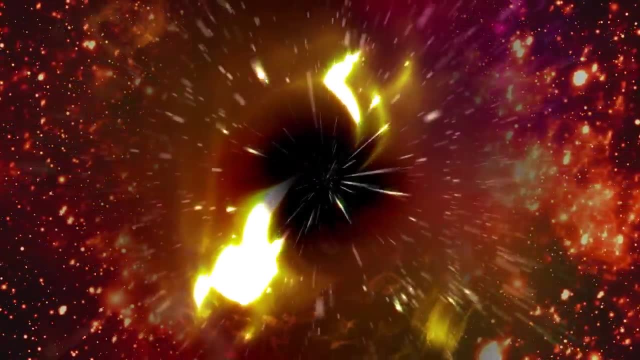 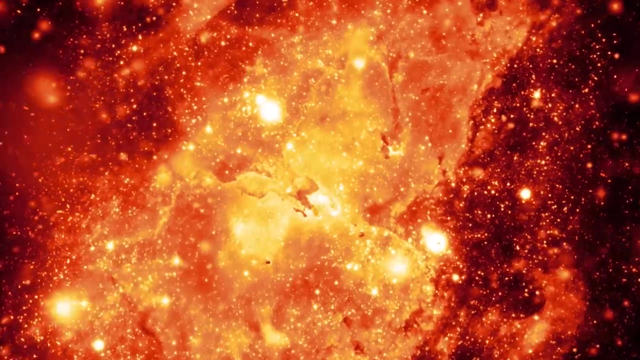 from the inflation and subsequent reheating of quantum irregularities in the nascent universe. Gravity already inherent to the universe would have acted on these density contrasts, collapsing vast areas of gas down on itself. However, there was only around a one second window after the big bang when this could 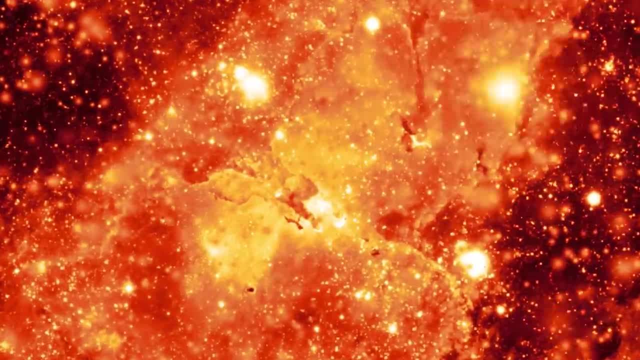 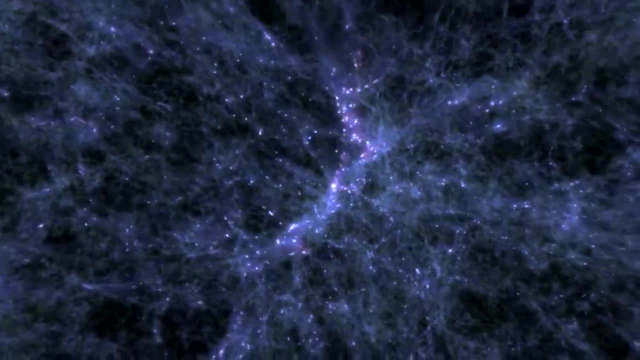 have happened before. the universe expanded and cooled to such a size that gravity was no longer effective at pulling together matter into these black hole prisons. After that, the universe would have to wait many millions of years before a new black hole would form through the death of stars. 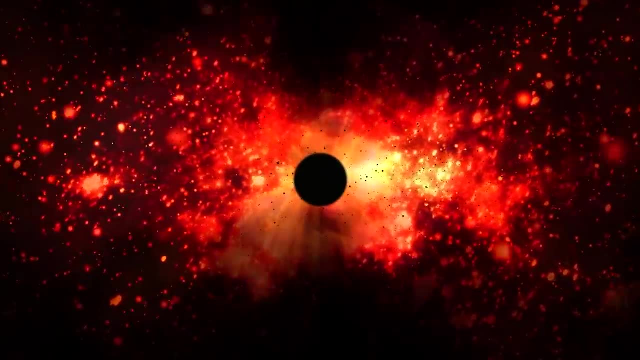 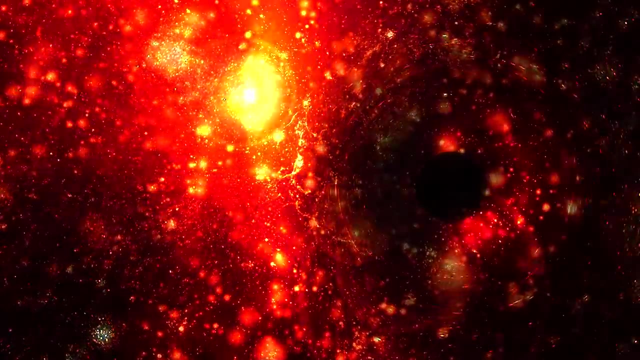 But these primordial black holes could be the seeds for the otherwise unexplainable black holes we are detecting today. The problem is, although this theory seems consistent with our understanding of how matter behaved in the early universe, we have very little information on when exactly they did. 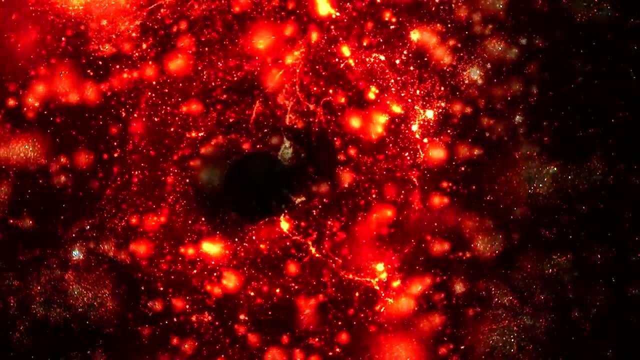 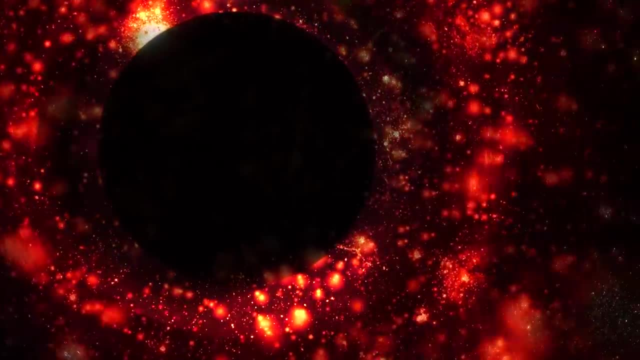 so, and how large they could have grown in that one second window. Mathematically, the later a primordial black hole forms, the larger it would be, and so estimates for their size vary spectacularly, ranging from minuscule specks weighing a hundred. 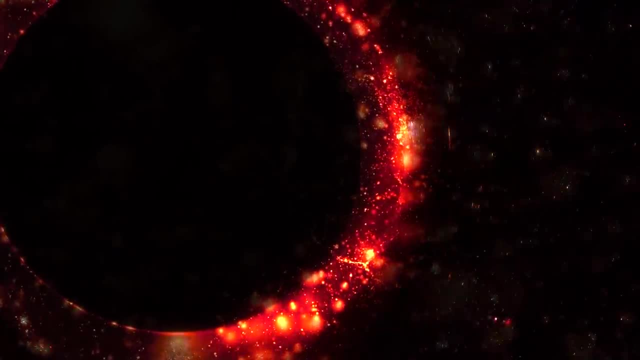 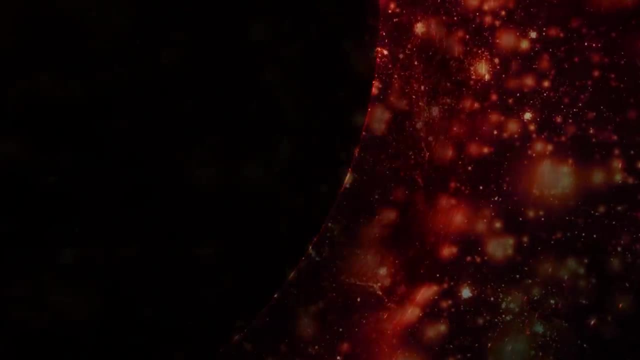 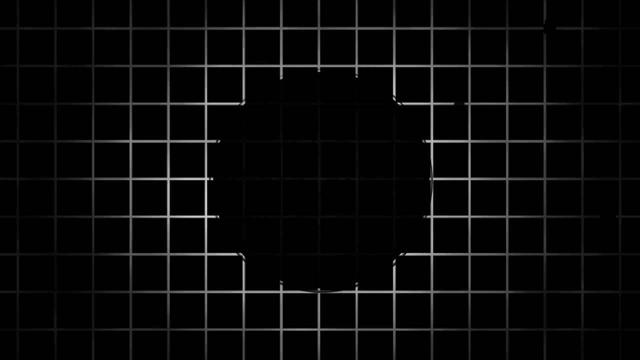 thousandth the mass of a paperclip to mammoths, a hundred thousand times heavier than the sun. And so how do we find and identify them, if they do exist? In the 1970s, Stephen Hawking also theorised that black holes do more than just swallow. 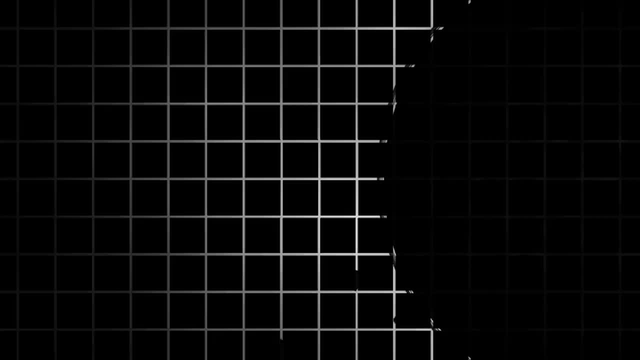 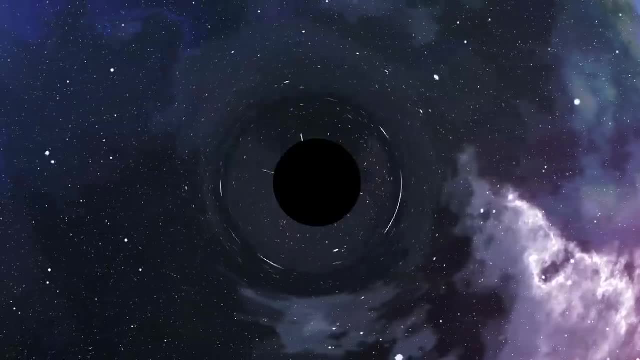 matter and grow ever larger. He suggested they could lose some of their weight through what became known as Hawking radiation. This weight loss is faster the smaller a black hole is, and the runaway acceleration of radiation would ultimately lead to the appearance of a black hole. 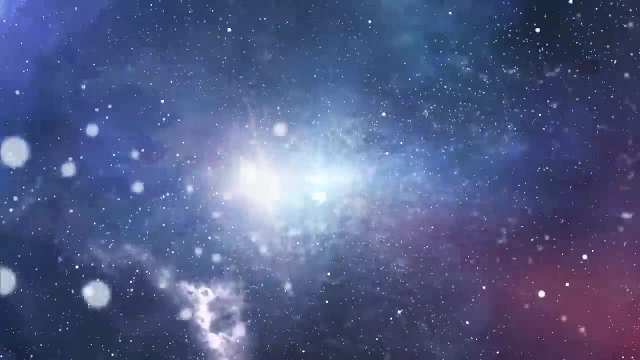 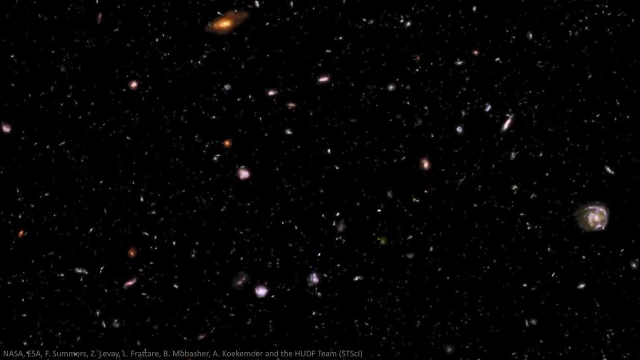 The black hole is the smallest black hole in the universe. It has an acceleration of a black hole in an explosion equivalent to one million megaton hydrogen bombs. Any black hole that was less than 100 billion kilograms in mass could be expected to decay away within the age of the universe. so scientists have begun searching for these characteristic. 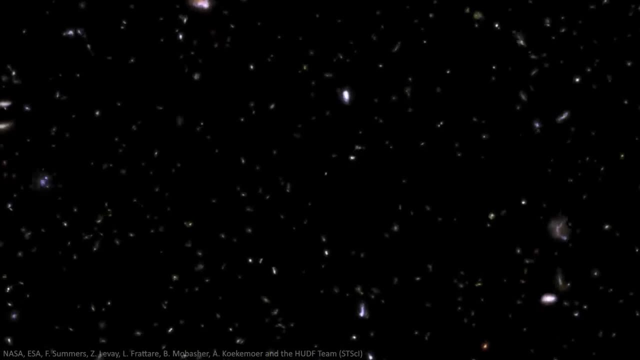 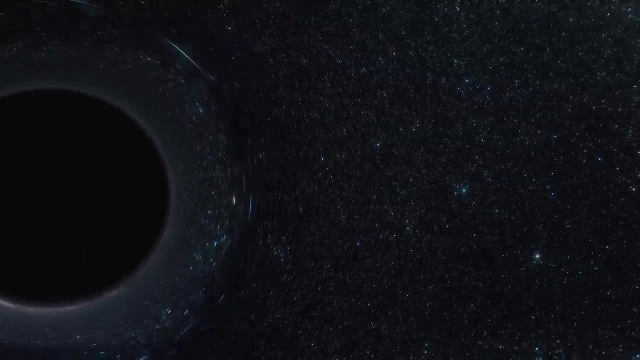 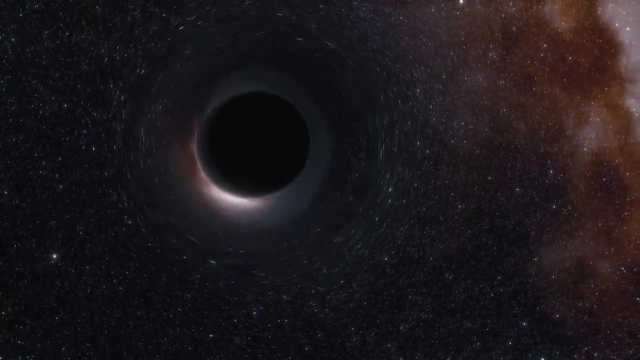 explosive death throes. with instruments like the space-based Fermi gamma ray telescope, Other potential methods for searching for these elusive primordial seeds involve looking for microlensing and magnification of stars in the universe of stars and galaxies as the black holes pass in front, or trying to detect the destruction. 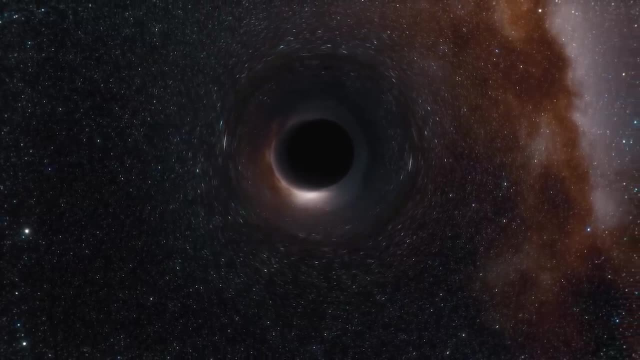 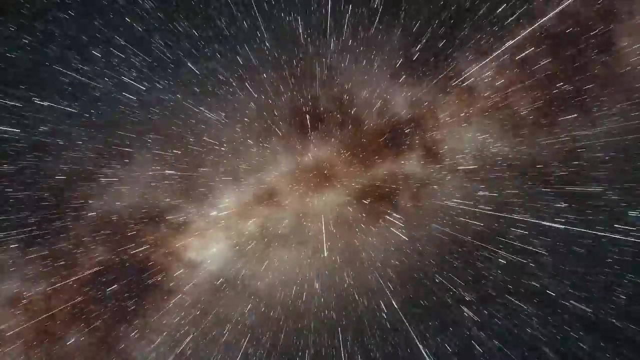 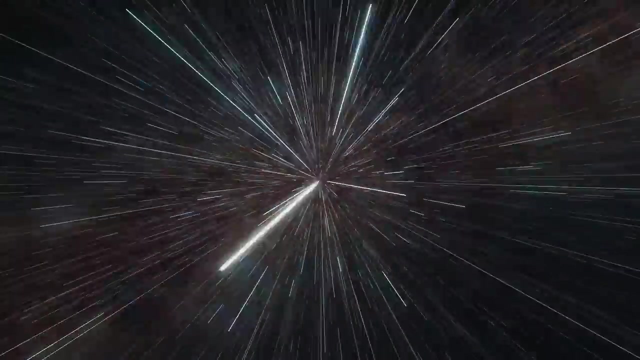 of dense stars caught in the primordial's gravitational wells. But all these studies have accomplished so far is to rule out certain size ranges, leaving an ever-shrinking envelope of possibility for how big primordial black holes can be and when they formed. 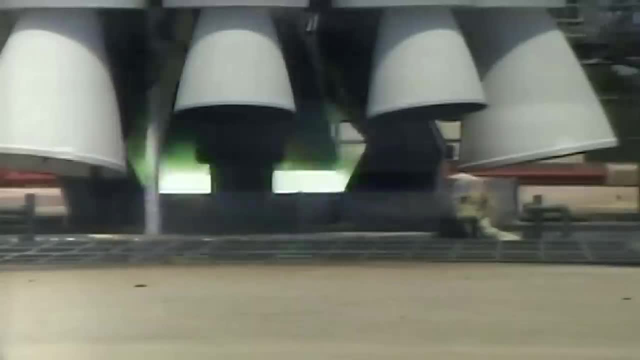 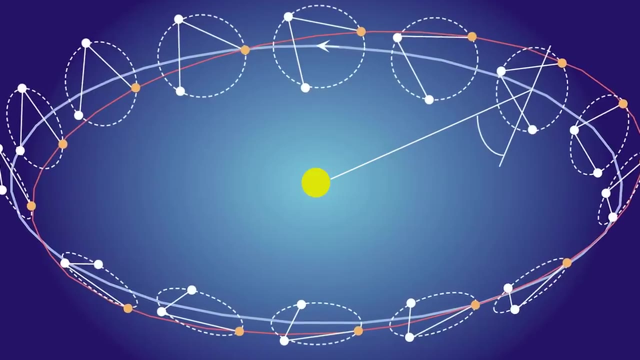 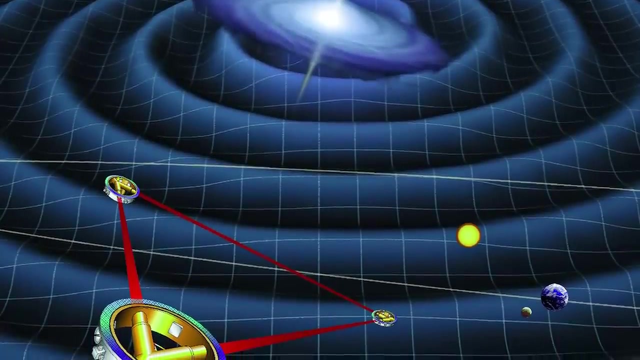 Although astronomers have not yet given up hope, the next generation of high-tech telescopes will continue the search with better reach and precision than ever before. The Laser Interferometer Space Antenna, or LISA, will launch next decade to continue spanning space for gravitational waves, some of which may come directly from primordial 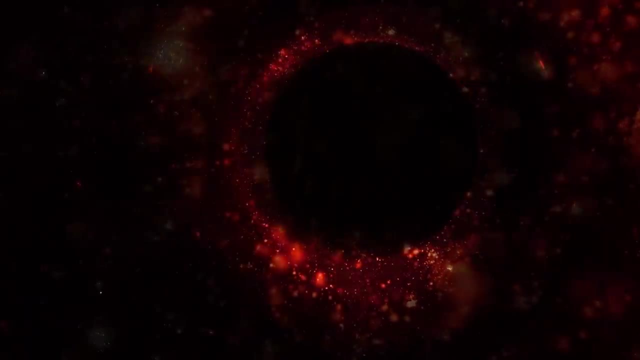 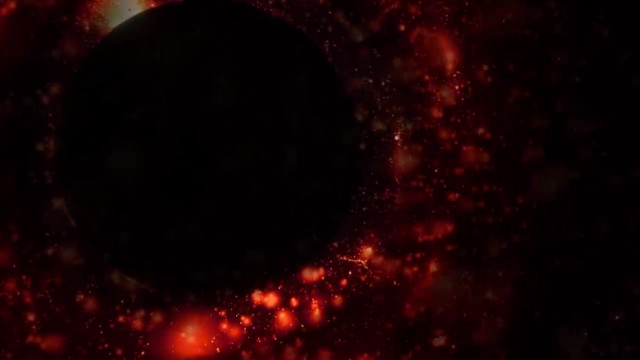 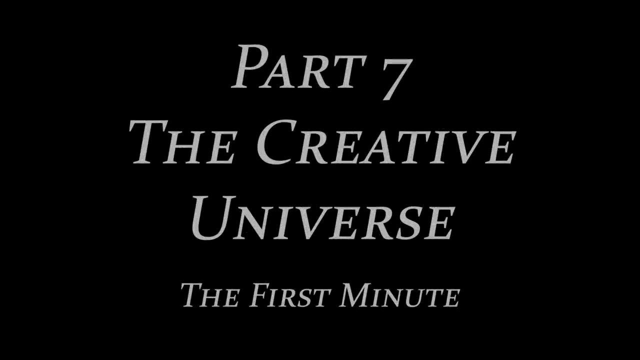 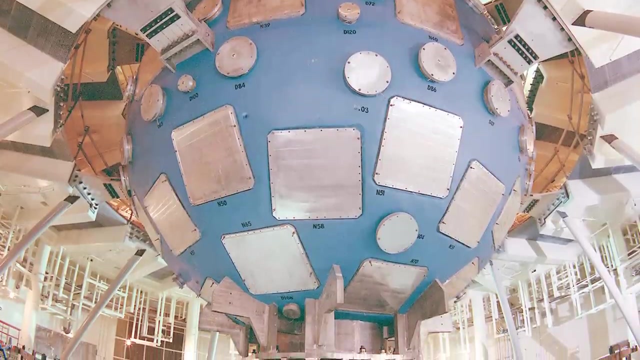 black holes that have been roaming the universe since they first formed barely one second after the beginning of time. SAGES OF LIroscopy On the 5th of December 2022, in the bowels of the National Ignition Facility at Lawrence. 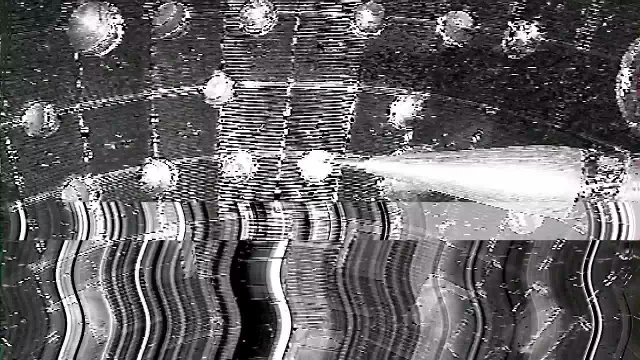 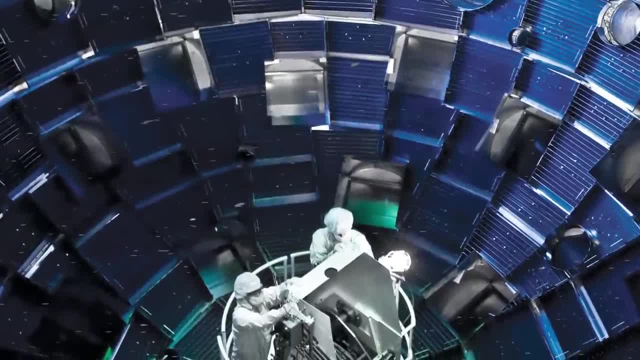 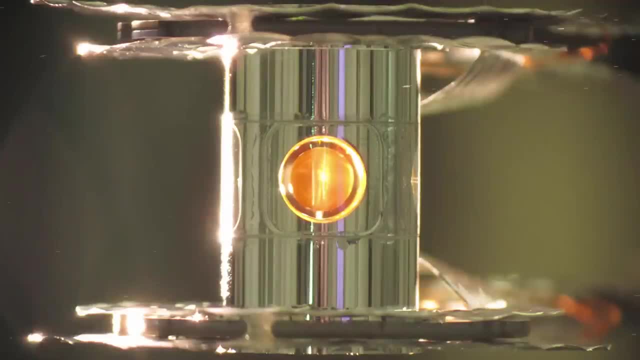 Livermore National Laboratory in California, humanity achieved something remarkable. Scientists at the lab focused 192 lasers inside a one-centimetre-long gold cylinder containing a single fuel pellet the size of a peppercorn. It held one conventional fuel pellet falling from the prze discutń, itself containing two. 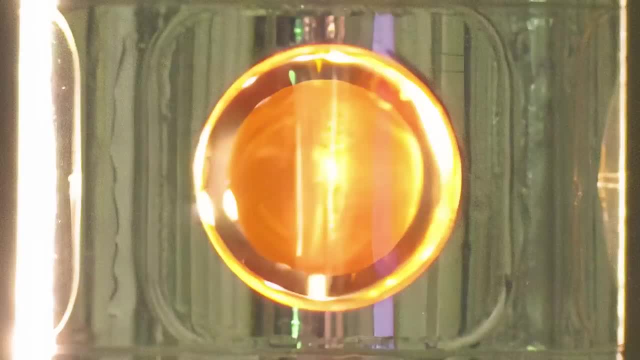 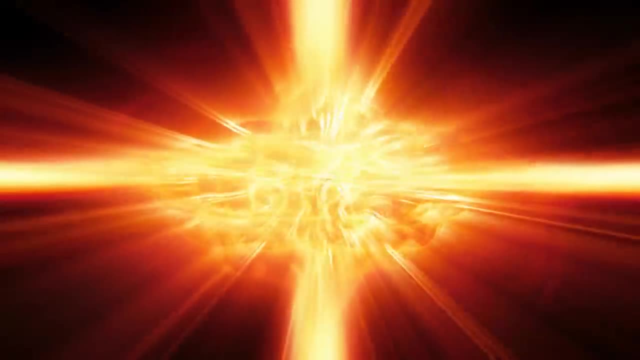 two isotopes of hydrogen, deuterium and tritium. When the laser energy struck the walls of the capsule, it heated them up to around three million degrees Celsius, a temperature hotter than the surface of the sun, causing them to emit X-rays inside the cylinder. 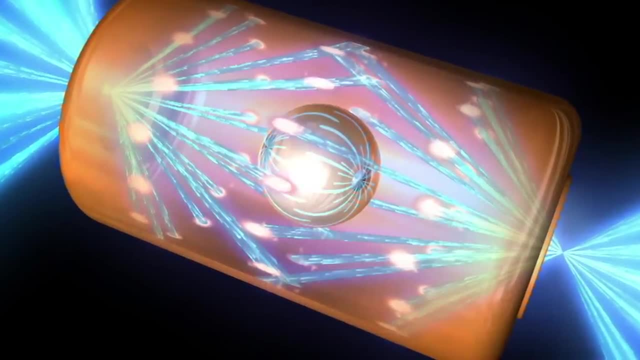 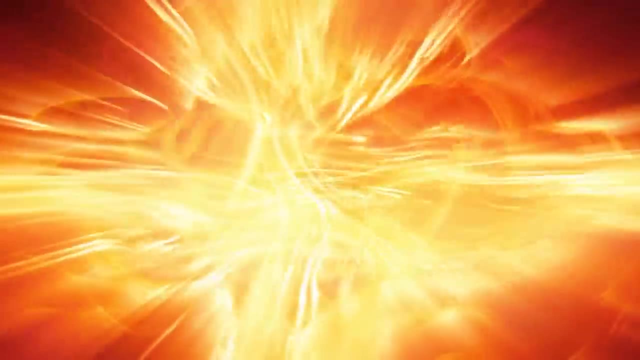 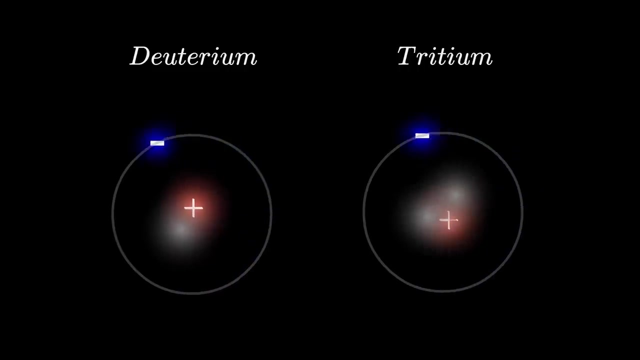 These powerful X-rays then blasted the surface of the pellet and compressed the fuel at some 400 kilometers per second. The fuel imploded, reaching a hundred billion times atmospheric pressure in less than ten billionths of a second. The atoms of deuterium and tritium fused together, transforming them into helium, while also giving 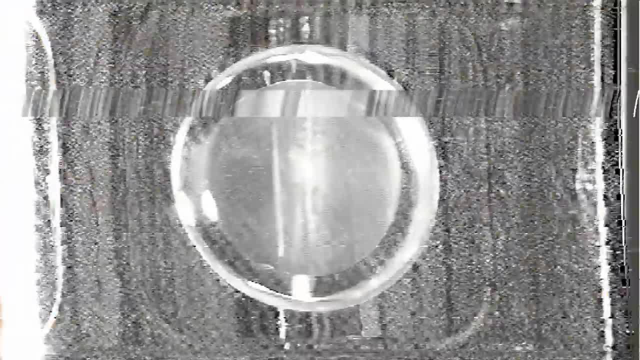 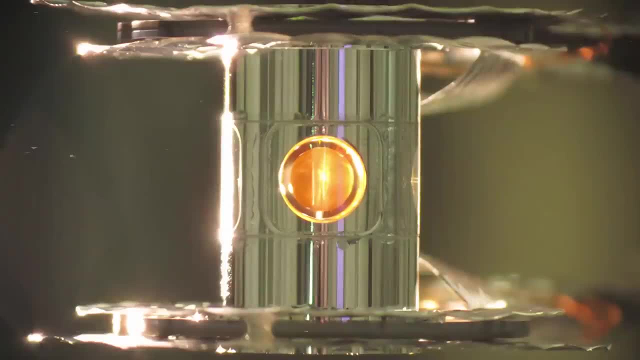 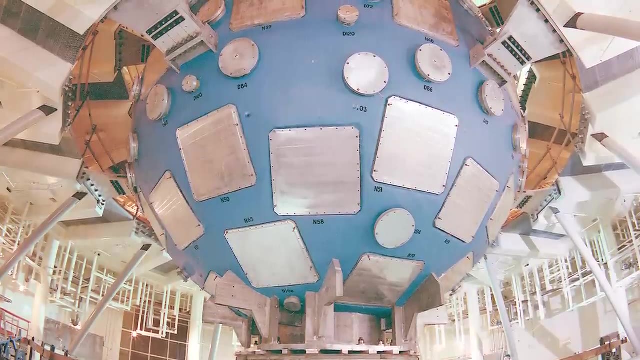 off a high-energy neutrino and other energy. In total, 2.05 megajoules of energy entered the cylinder and 3.15 megajoules were produced by the fusion reaction. In this way, for the first time in nearly 70 years of trying, scientists managed to. 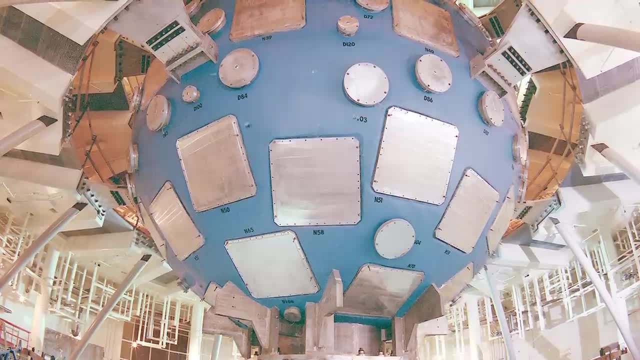 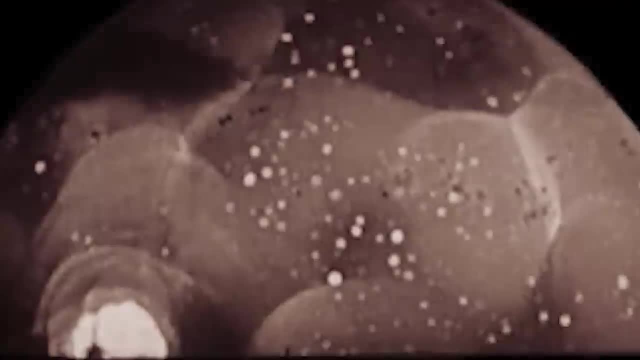 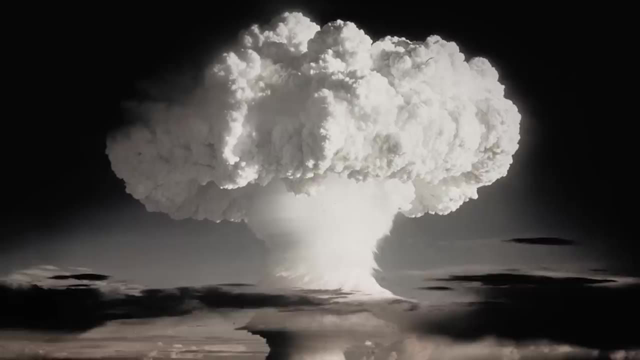 initiate a productive nuclear fusion process Reaction. The fusion itself was nothing new. Humans have been making deadly fusion weapons since the 1950s, But this reaction in 2022 was the first time we've created fusion that was able to release more energy than was put in to get it started. 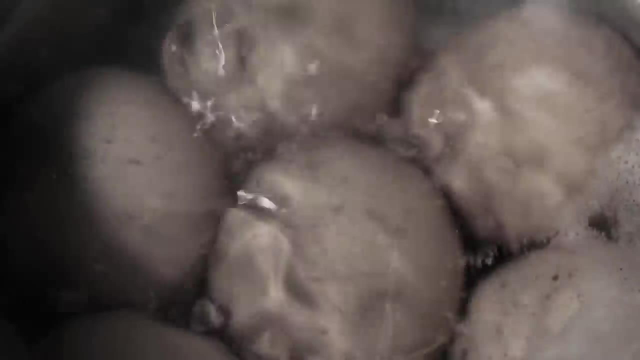 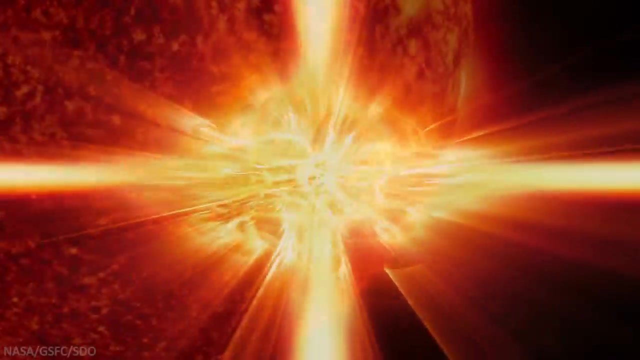 The roughly 50% energy gain would have been enough to boil around 20 kettles Still. the breakthrough is a major one for nuclear physics And yet this is a process that has been going on, naturally in the hearts of everyone. 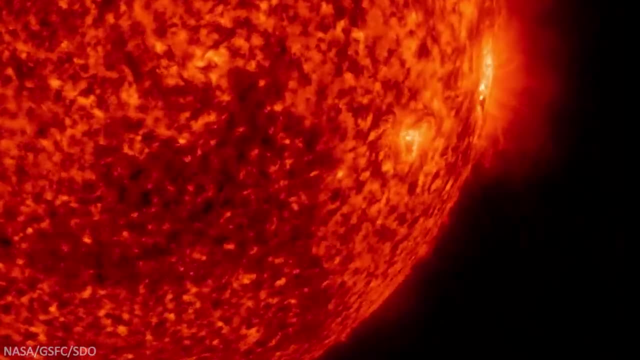 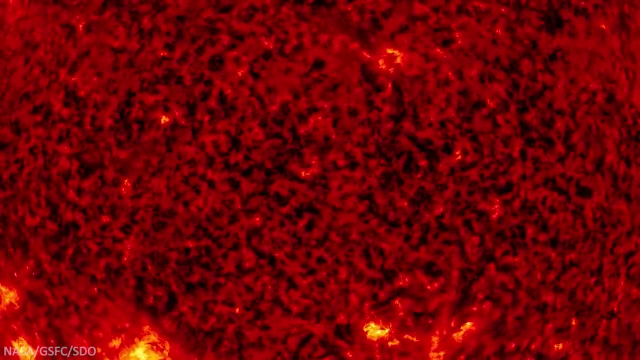 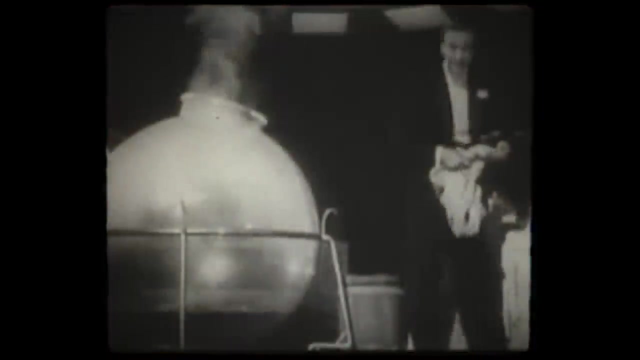 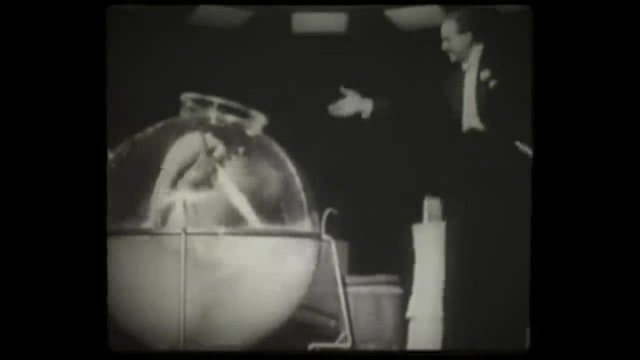 Every single star in the universe for billions of years. Not only that, but the physics of the universe had this fusion figured out within its very first minute. Humans have long been preoccupied with the seemingly magical act of turning one thing into another, Whether it is producing a bunch of flowers from thin air or alchemically transmuting. 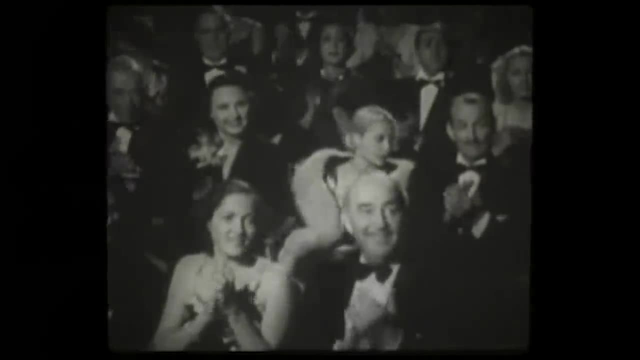 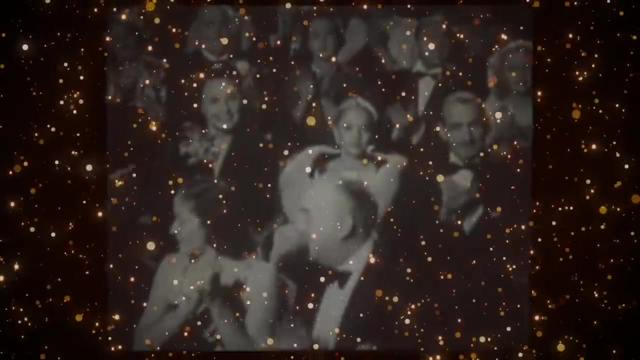 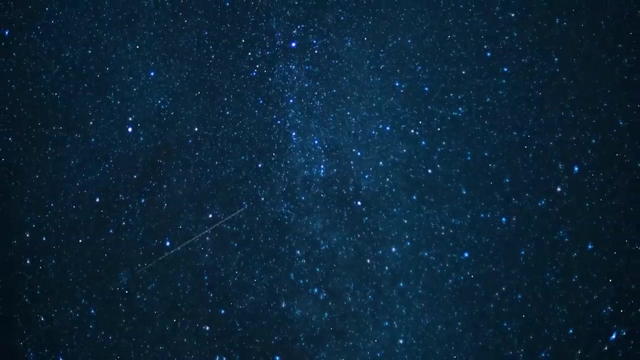 base metals into valuable gold. Nothing fascinates us more than the idea of getting something novel from something mundane, And the very early cosmos was rife with such transformations, while the unsettled fundamental forces drove chaotic identity swaps. But such transformations continue all around us, even in the modern universe. 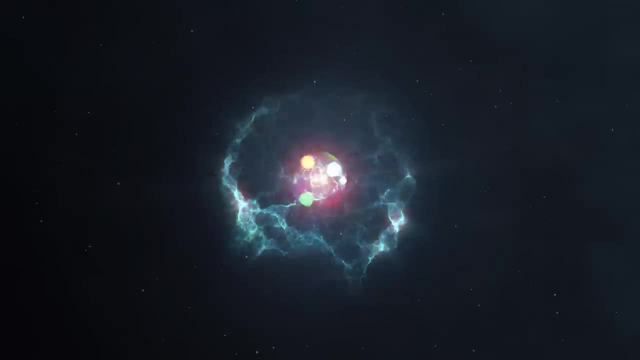 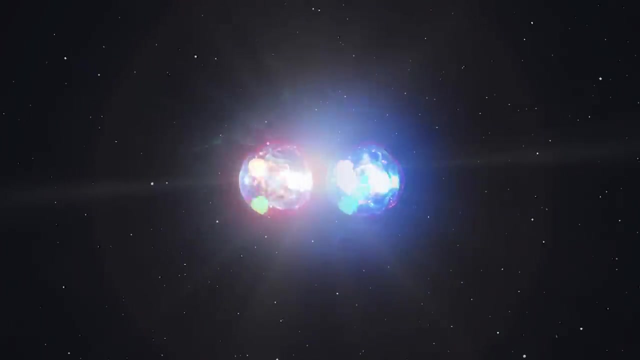 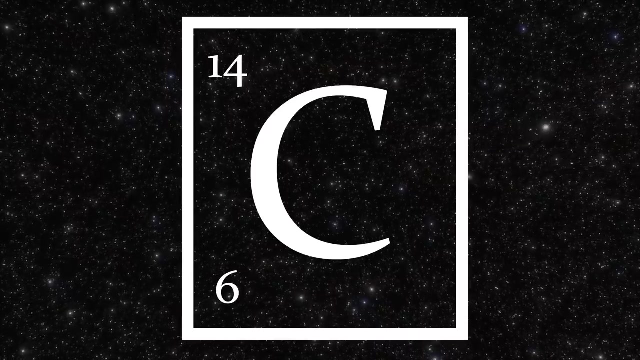 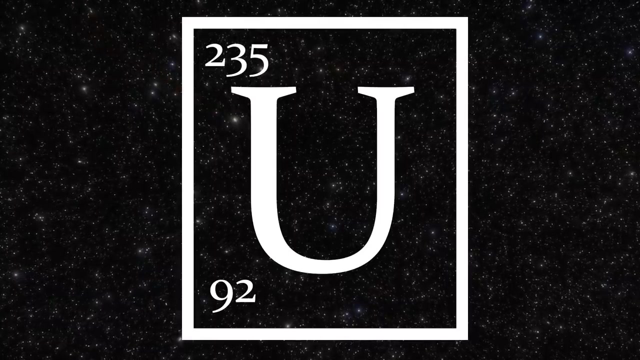 Radioactive decay, mediated by the weak force, sees atomic nuclei fracture and break, transforming elements into their less massive cousins on regular and predictable timescales. This nuclear fission occurs in a wide variety of elements, from carbon-14, used for carbon dating, to technetium-99, used for medical imaging, and uranium-235, used as fuel for nuclear reactors. 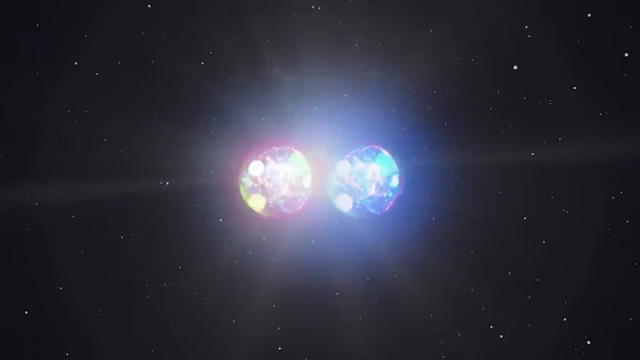 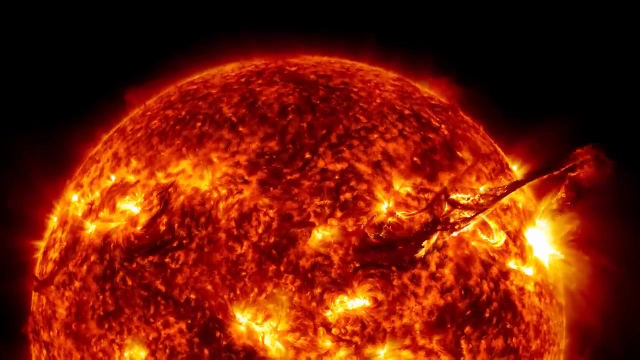 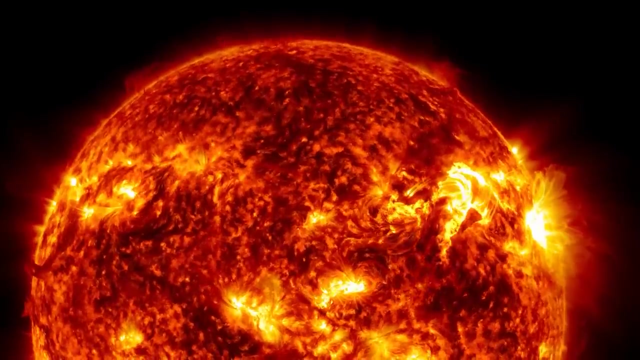 Such radioactive decay occurs as a consequence of unstable atomic nuclei and will typically happen spontaneously under the most ambient conditions. But as the other kind of nuclear transformation, nuclear fusion sees atomic nuclei increase their mass and move up the periodic table, it is much harder to achieve. 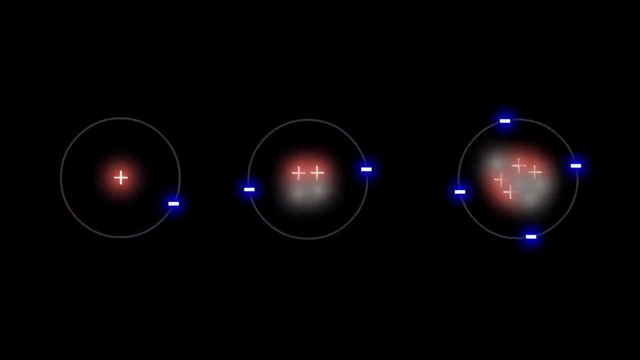 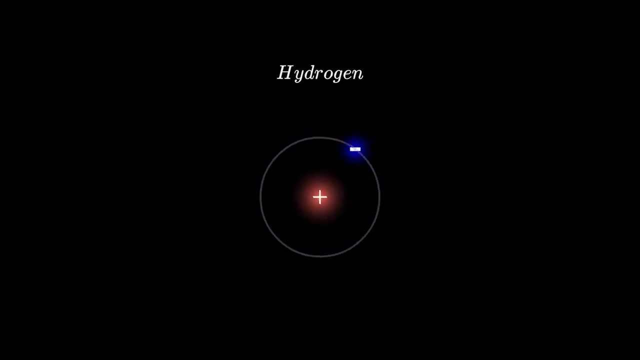 The identities of all atoms are determined by the numbers of protons and neutrons within their nuclei. Hydrogen has one proton, with different varieties of isotopes with different masses possessing different numbers of neutrons. Protium has only one proton. deuterium has one additional neutron, doubling the relative. 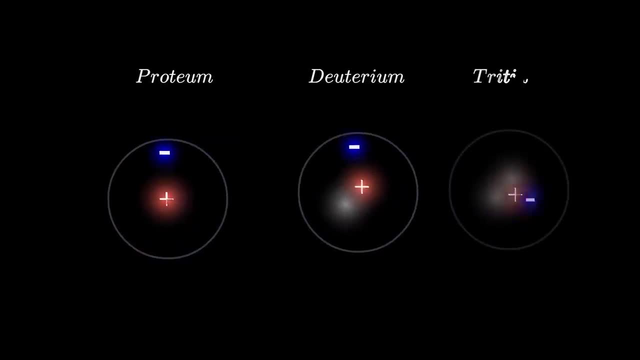 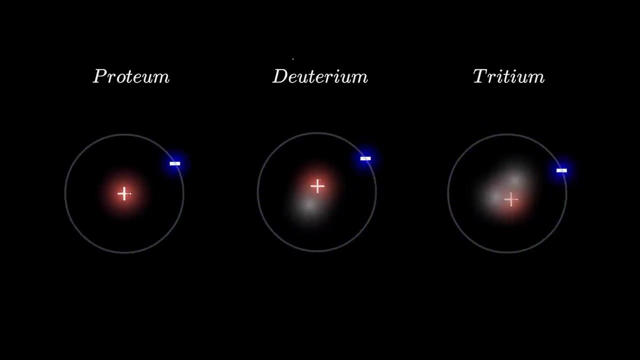 mass of the atom and tritium has two. Tritium has two neutrons, bringing the total relative mass to three. Only when another proton is added does the identity of the element change. Two protons make a helium nucleus, with helium-3 possessing one neutron and the most stable. 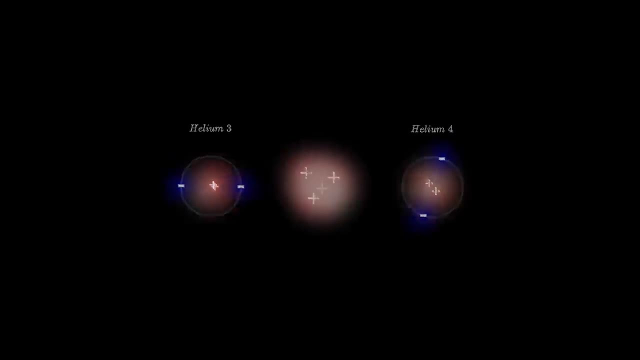 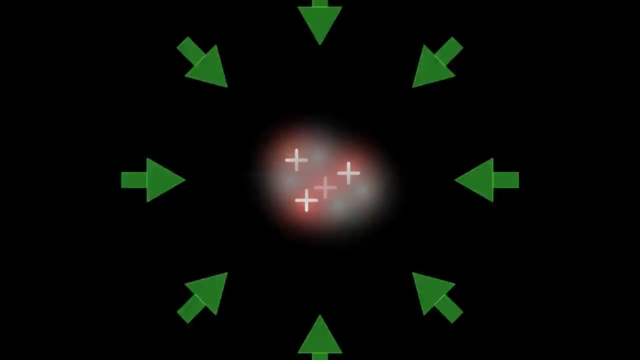 helium-4 having two neutrons. The strong nuclear force is the agent responsible for binding all of the hadrons together into stable atomic nuclei, But with protons sharing a light positive charge, they are pushed apart by another of the four fundamental forces. 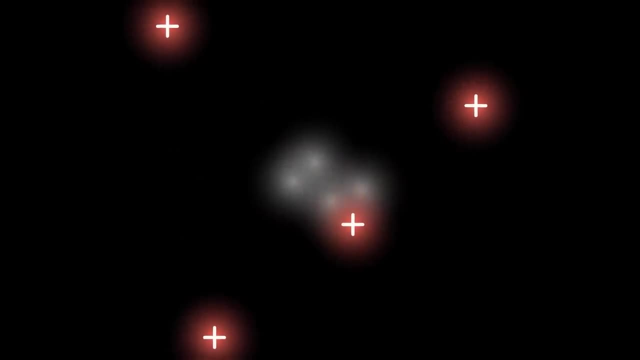 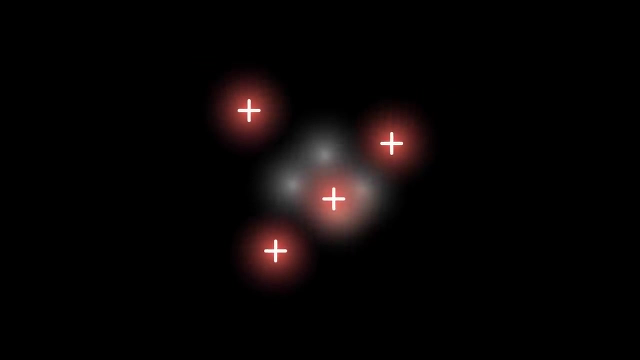 The electromagnetic long before the gluons can hold them together. So it takes intense heat and physical pressure, such as that found at the heart of stars or inside in a radiated golden capsule, to push the protons close enough for the strong nuclear. 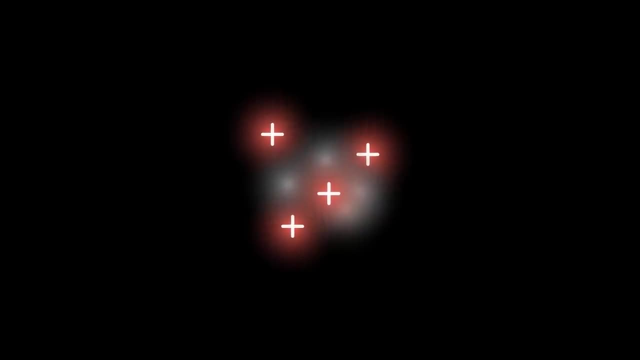 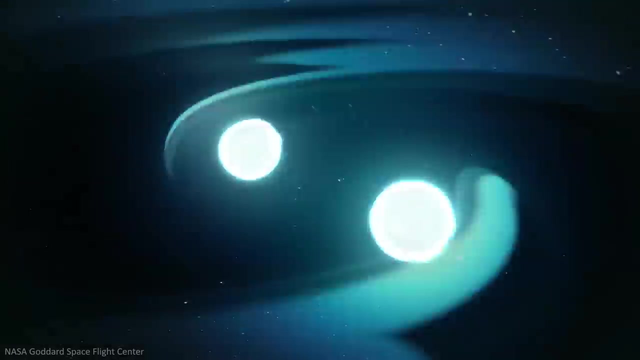 force to overcome its force, kin, and for the elements to fuse into something new, To make even heavier elements combining many tens of protons together. it takes even more extreme cosmic events like supernovae or mergings of stars. The supernovae are also known as the supernovae. 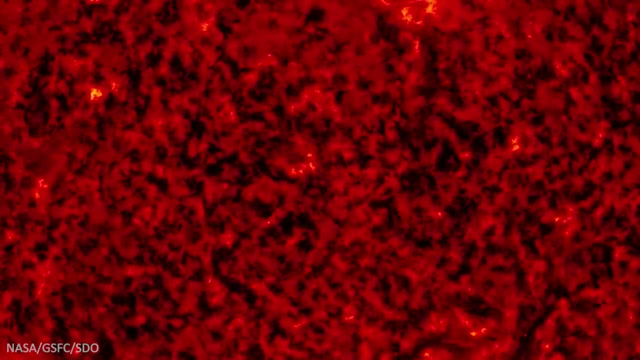 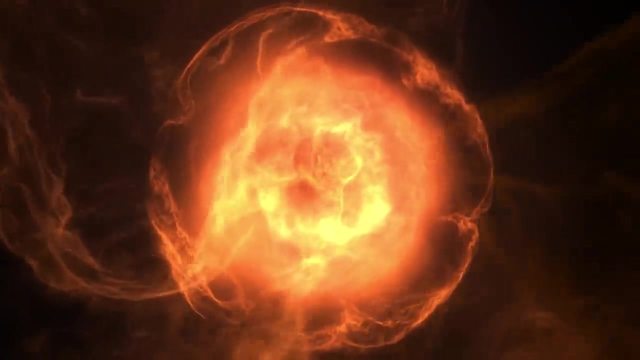 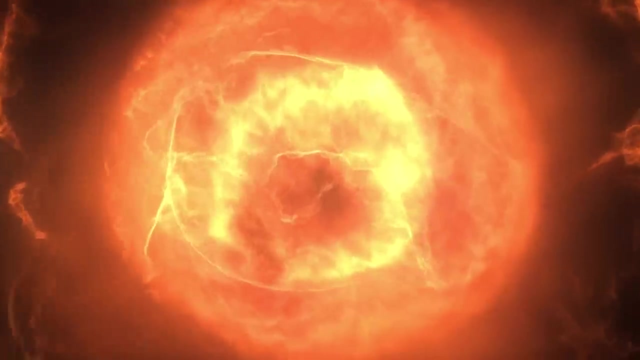 Despite their struggles to replicate it in the lab. scientists have a good understanding of how nuclear fusion works inside stellar furnaces to create new elements from simple hydrogen and helium. They have even witnessed and understood the very beginnings of that process inside so-called failed stars. 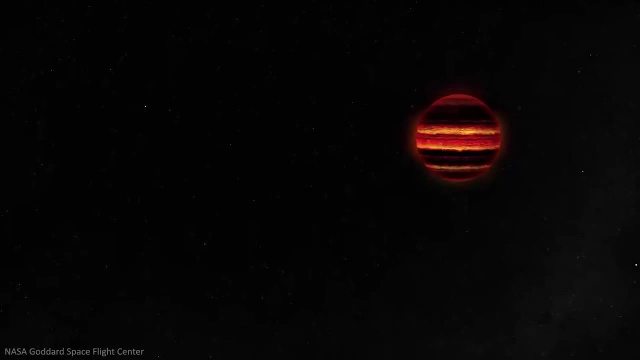 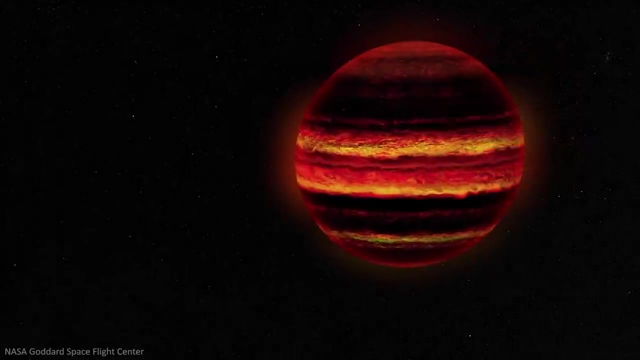 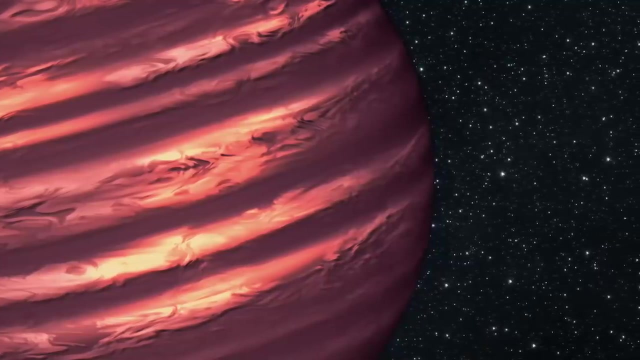 Brown dwarfs are massive orbs of gas, larger than the Jupiter-like gas giants, but smaller than an active star. Inside them there simply is nothing. There simply isn't enough heat and pressure for lightweight protium hydrogen to fuse into helium. The process is accomplished by using heavier deuterium as an intermediate. 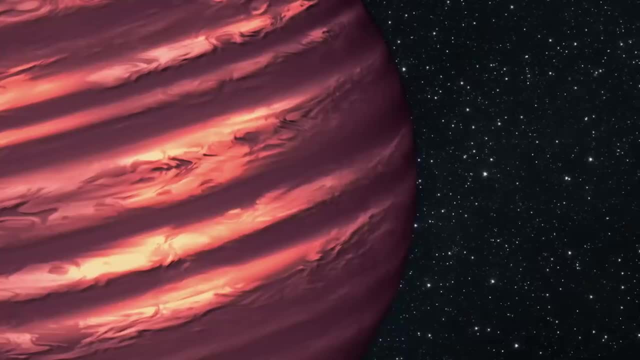 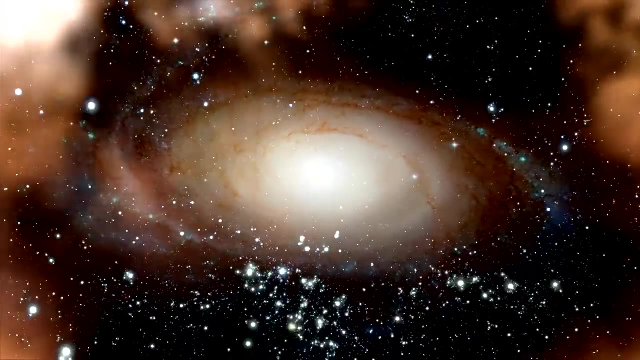 However, none of these processes help to explain where the larger atoms of deuterium and helium came from in the first place, And so for that we need to look back to an age before stars, before stellar fusion, to the universe's very first minute. 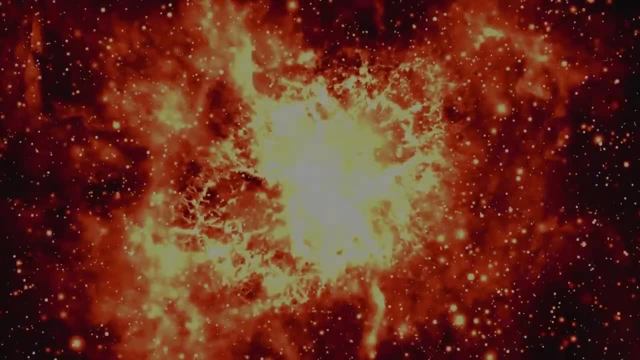 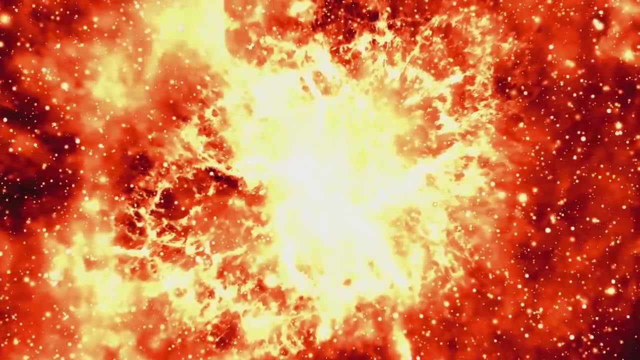 When the average temperature of the universe dropped to around 10 million degrees celsius- about a microsecond after the big bang- it was finally cool enough for quarks to bind into protons and neutrons, making the building blocks for all elements to come. 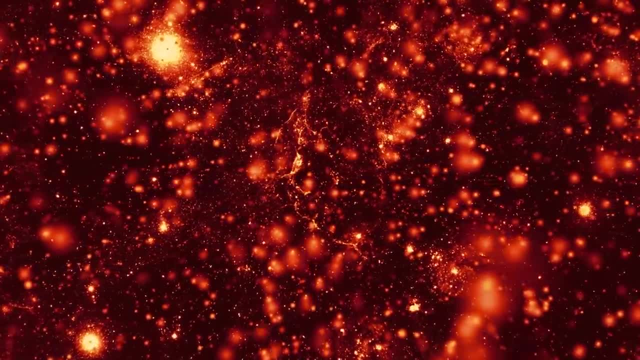 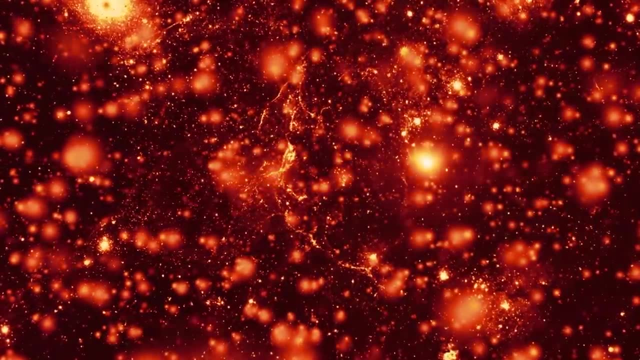 But there is a hundred million year gulf of time before we see the first stars begin to shine, powered by the nuclear fusion of atomic nuclei at their cores. So when and how did these nuclei come together? It took a long time to find out. 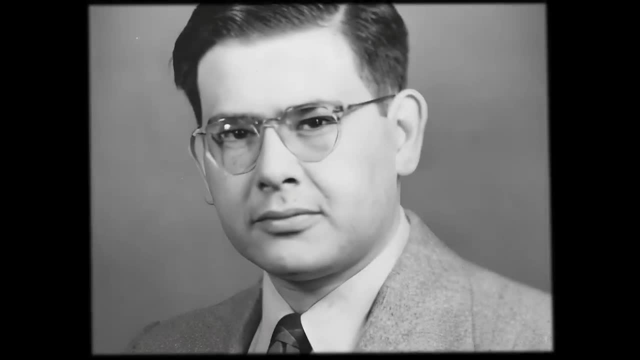 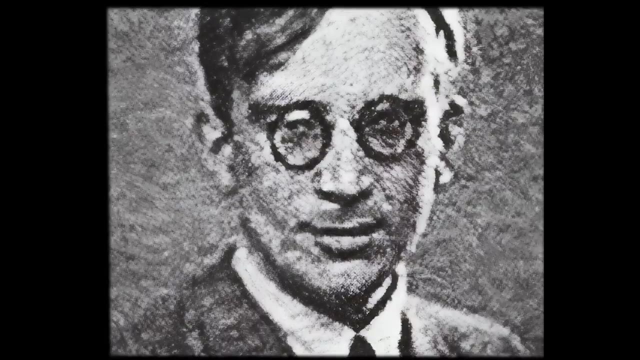 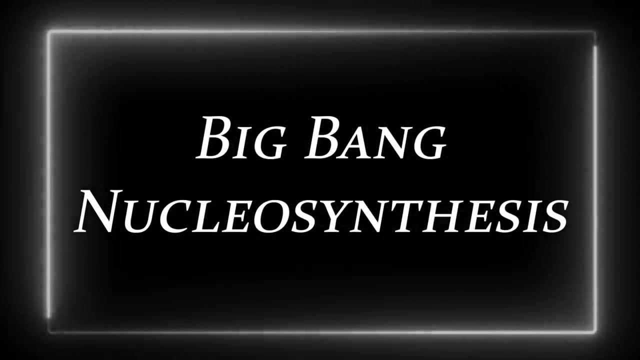 It was in 1948 that the prodigious American PhD student, Ralph Alpher, working with his supervisor, George Gamow, proposed a mechanism that would later become known as Big Bang Nucleosynthesis. It was a bold and inspired theory, but the brilliance of Alpher's work was somewhat 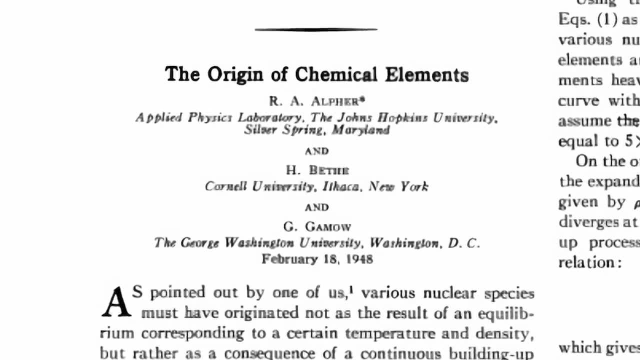 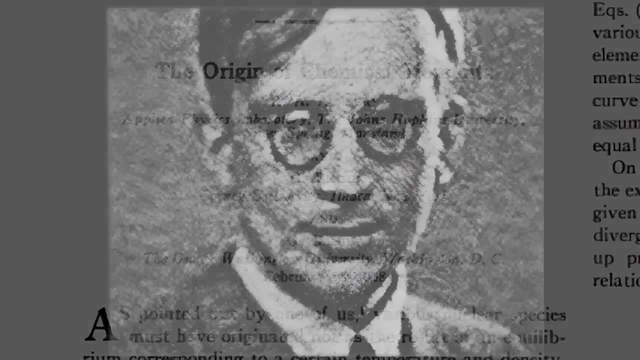 overshadowed by Gamow's insistence on including another author in their seminal paper who had no part in its development. In his words, it seemed unfit to the Greek alphabet to have the article signed by Alpha and Gamow only, and so the name of Dr Hans A Beta was inserted. 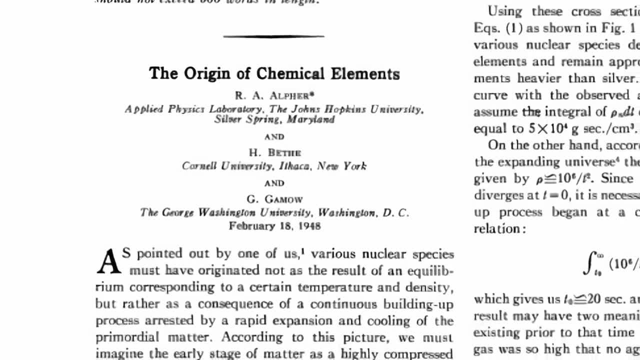 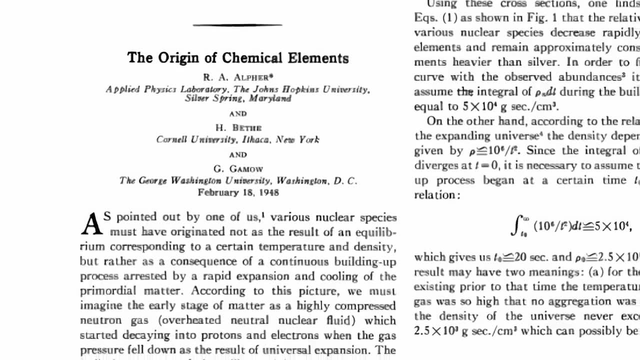 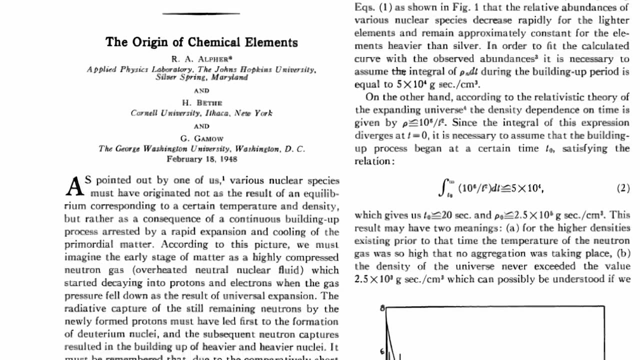 in preparing the manuscript for print, And so the Alpha-Beta-Gamma paper became the authority on pre-stellar fusion and to this day provides the foundation for understanding how the high temperatures at the beginning of the universe could turn hydrogen into helium via deuterium intermediates. 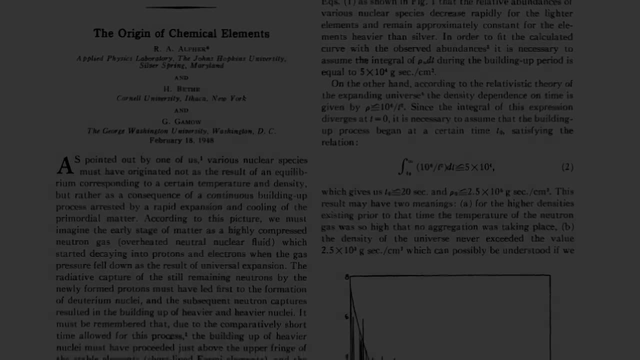 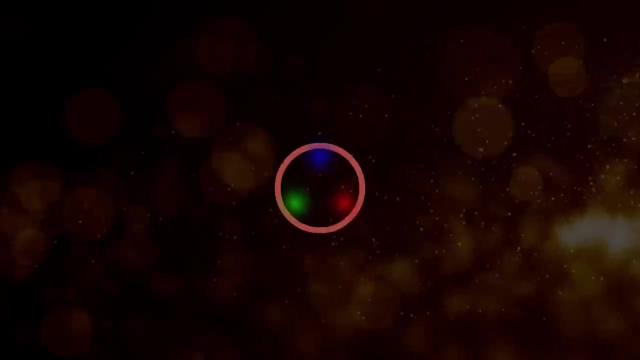 What is Protium? Protium is the lightest variety of hydrogen. It is the lightest in the universe. It consists of a single proton, So as soon as quarks bound into protons, these hydrogen nuclei existed. although it's important. 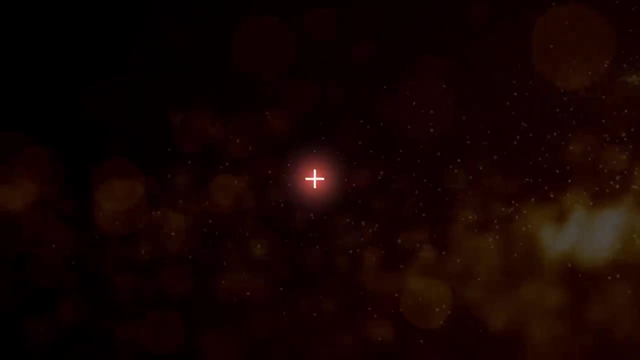 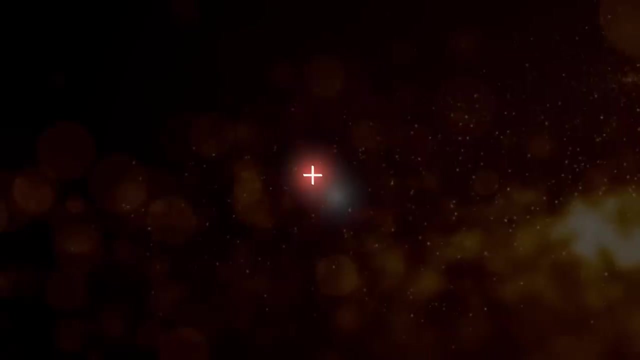 to note that it will be some time before neutrally charged hydrogen atoms with both protons and electrons will form. Around 10 seconds after the Big Bang, it was cool enough for some deuterium nuclei with one proton and one neutron to form. 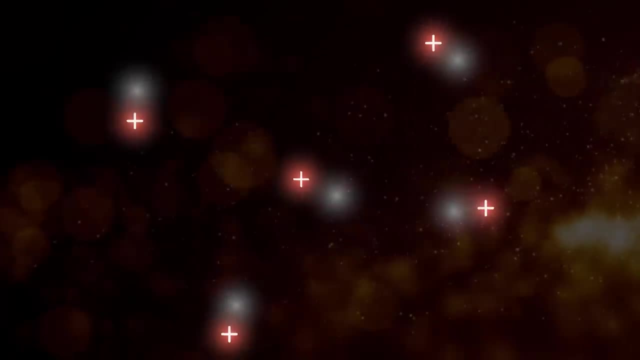 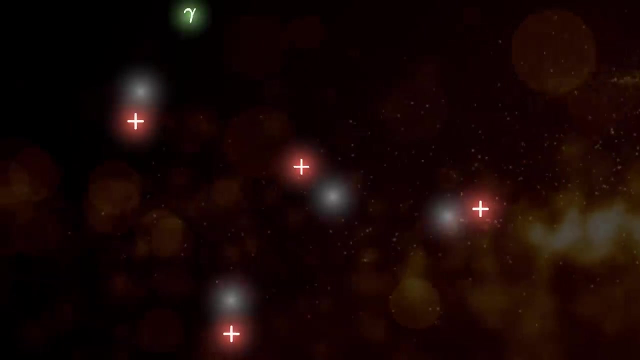 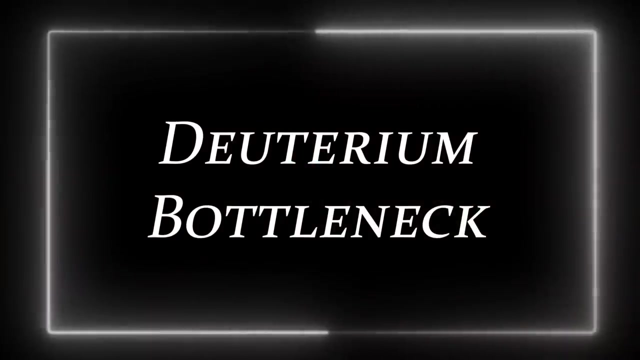 But in this hot cosmic soup, temperature and particle energies were still so high that the deuterium nuclei were unstable. If they were struck by a photon, as was inevitable under such densities, these first composite nuclei would break apart again. This is known to physicists as the deuterium bottleneck, and, until it was overcome, nucleosynthesis. 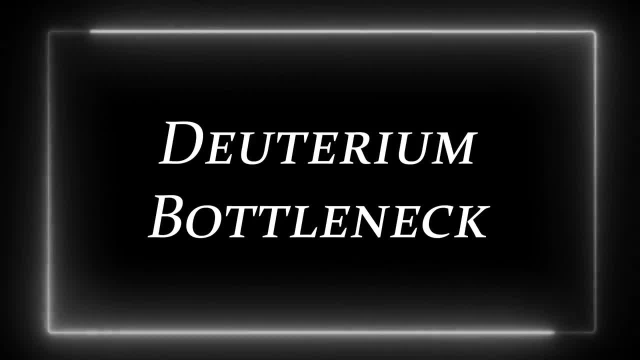 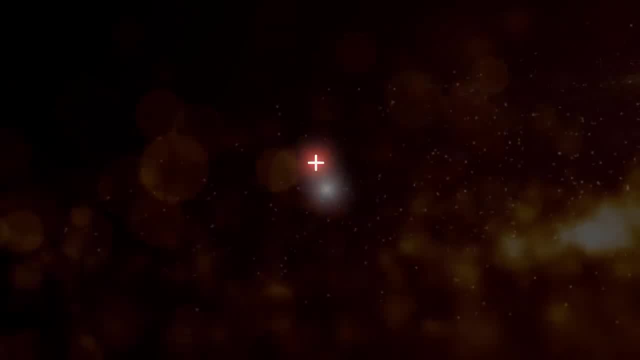 simply couldn't progress past the fusing of one proton and one neutron. Only after another 300 seconds did temperatures drop sufficiently for deuterium to become more stable and additional elements to form. But the deuterium was still there. It was still there. 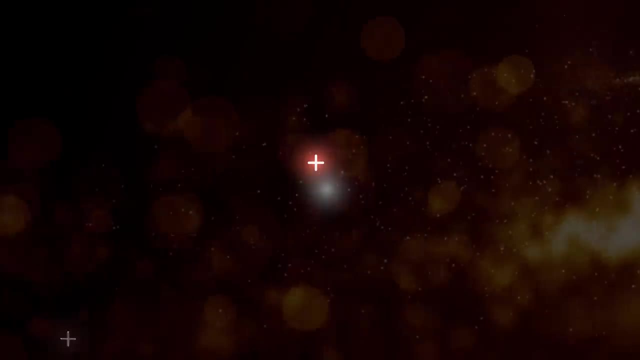 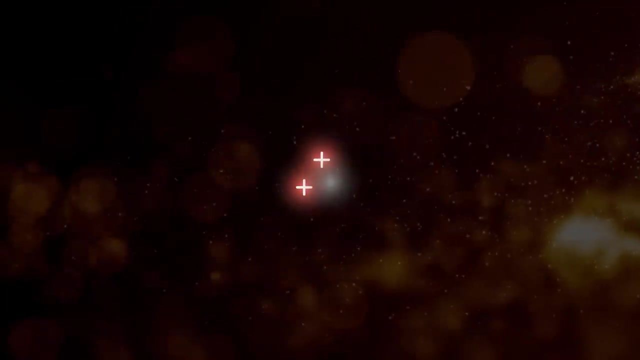 First deuterium, with its one proton and one neutron, is able to fuse with individual protons under the intense compressive force of the entire universe. The result is, for the first time, an entirely new stable element. 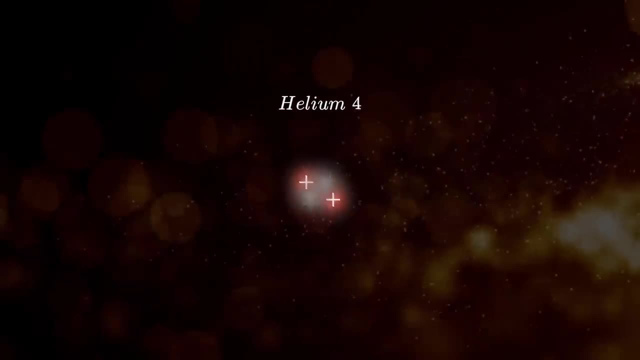 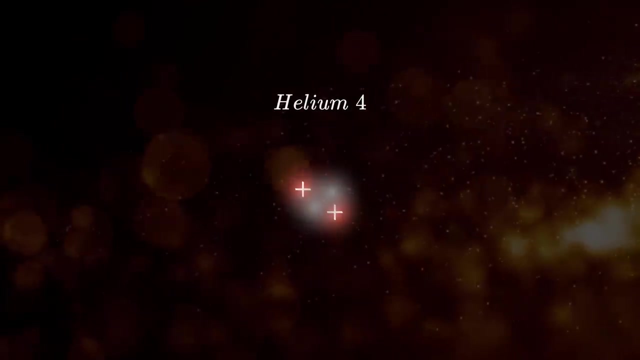 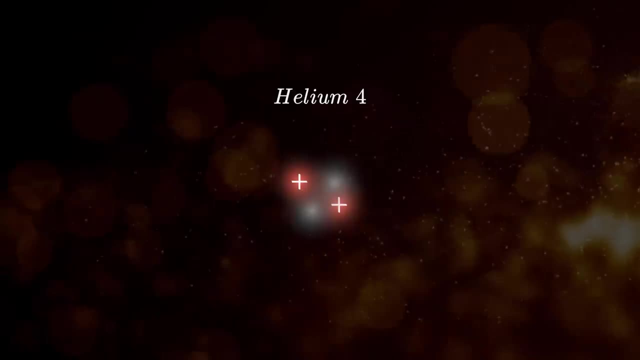 Helium-1 and Helium-2 are the most stable atomic nuclei in existence. Helium-1 and Helium-2 are the most stable atomic nuclei in existence Because of this and the conditions that prevailed within those first few hundred seconds. most 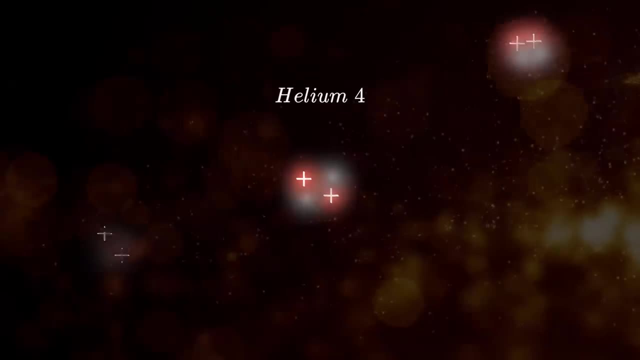 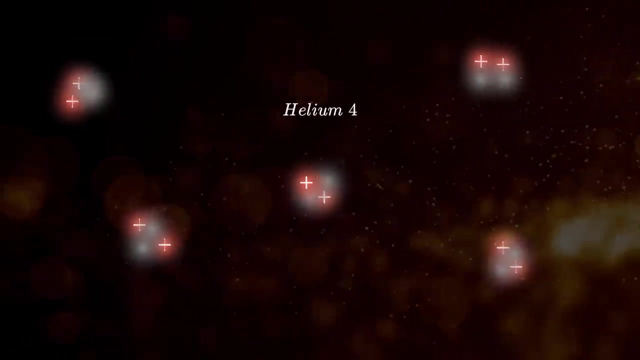 of the free protons in the early universe become swallowed up into helium and go no further. Calculations based on the initial balance of protons and neutrons and the available energy at this time predict that this would result in a universe that is around 25% helium. 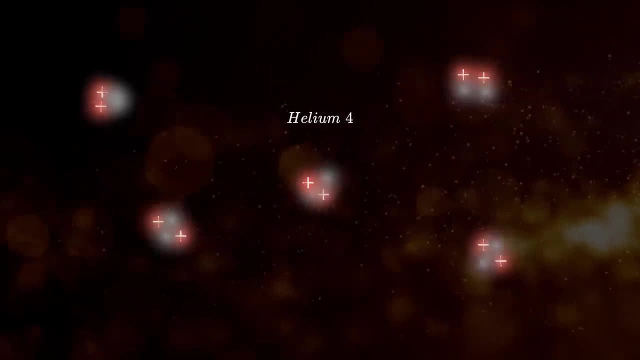 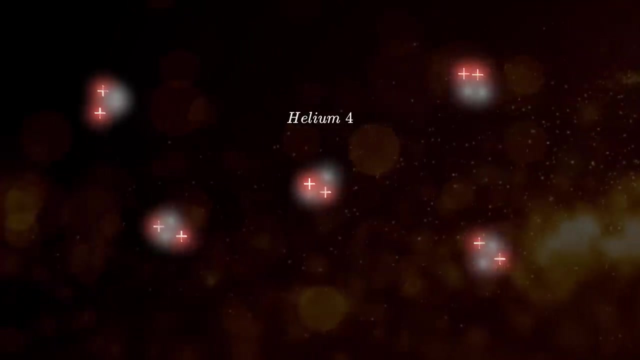 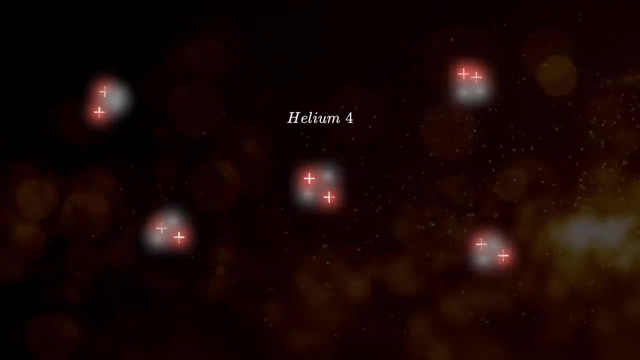 by mass. And this is indeed what we find: Helium-3.. 3.. 1. Even years after this energetic burst of helium creation, even after the lives and deaths of countless stars, the universe is still around 23% helium. 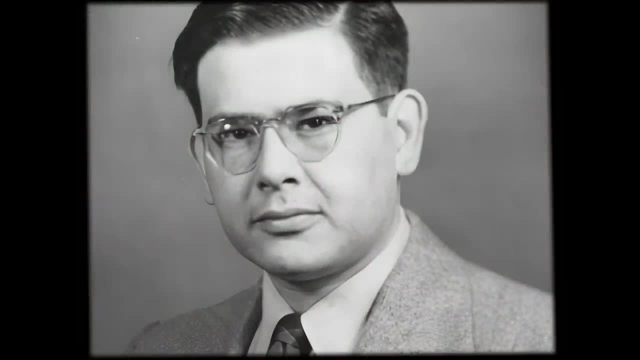 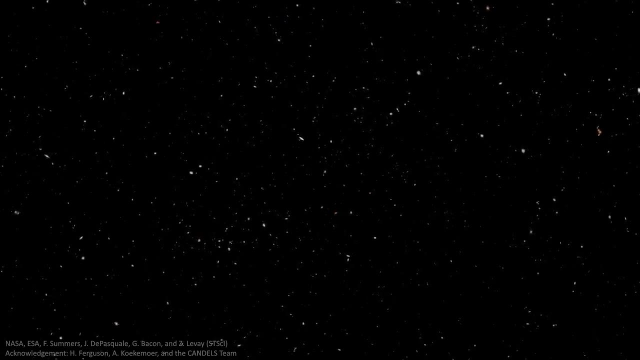 This observation alone is a striking confirmation of Alpha's theory, And it is here that we see another example of the fortuitous fine-tuning of the universe's initial conditions. We already know that if the proton to neutron ratio had been different than much of the 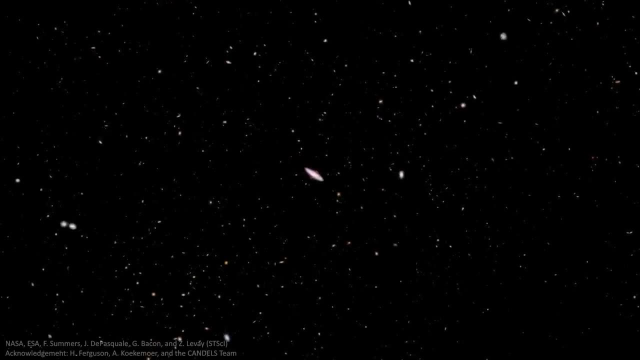 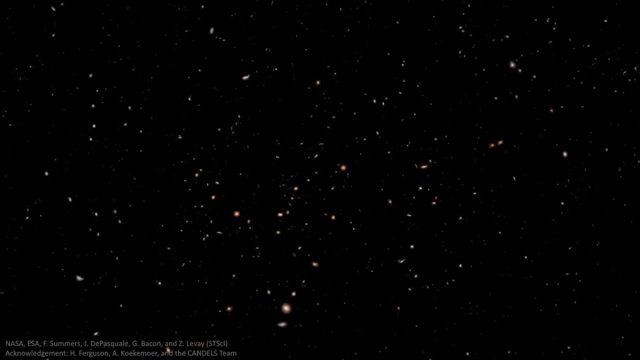 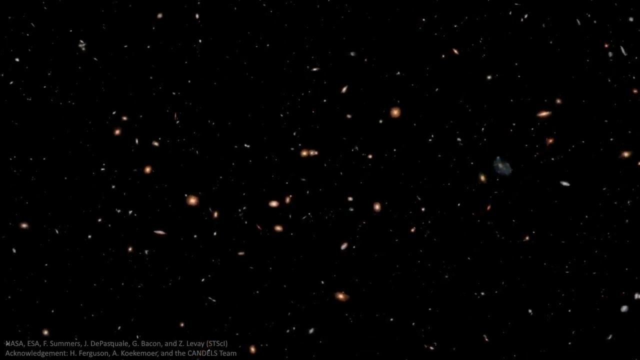 universe's ordinary matter. it would have decayed away into uncharged and unreactive neutrons and helium. But similarly, even with the proton-neutron ratio we were dealt. if the matter in the cosmos had been any more compact at the time of Big Bang, nucleosynthesis, then even more. 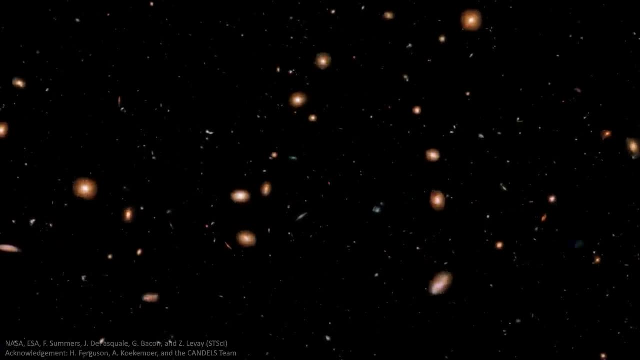 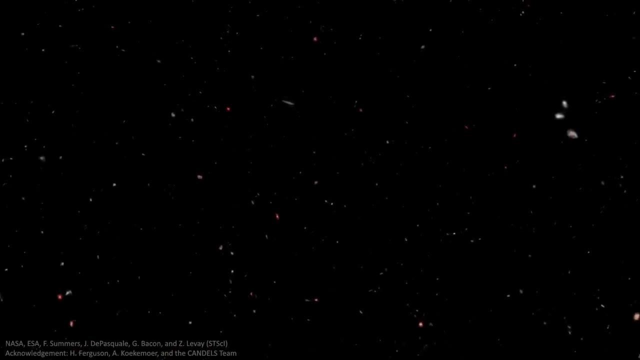 helium would have formed. The unreactivity of a universe made predominantly of helium would have meant little to no chemistry would have been possible thereafter, Again, leading to the bleak prospect of a universe that would have been made of helium. And if the matter in the cosmos had been any more compact at the time of Big Bang? nucleosynthesis. then even more helium would have formed A universe with no stars, no galaxies and no us. Thankfully, however, this was not the case. Even as so many hadrons settled into their stable helium nuclei, the universe is still full of latent energy – which could be used for further fusion. 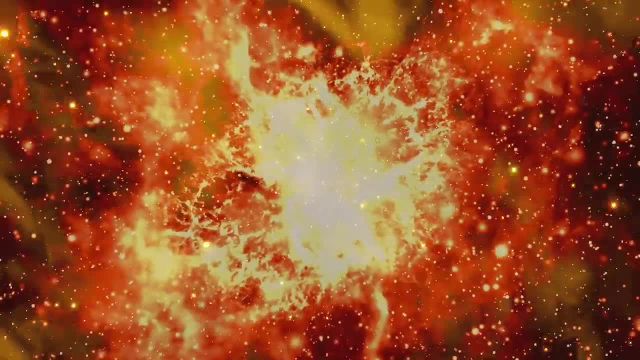 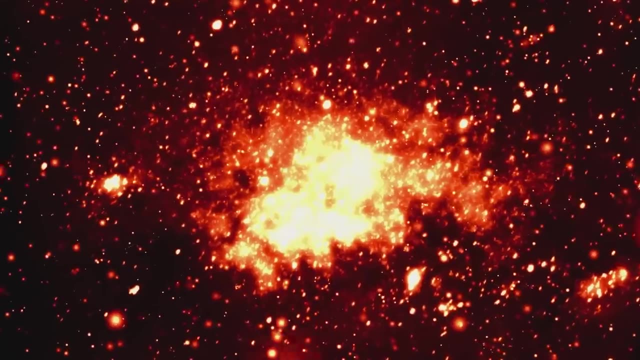 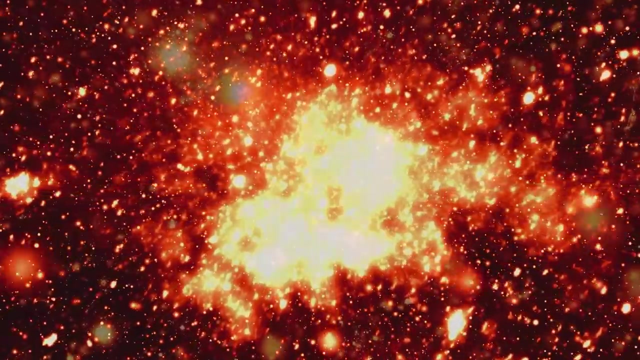 And now the race is on to see how many novel elements can be created before the ambient energy of the universe drops too far. Eventually, after around 1200 seconds of furious cosmic nucleosynthesis, amounting to little more than 20 minutes of universal existence, the nuclear furnace finally sputters and dies. 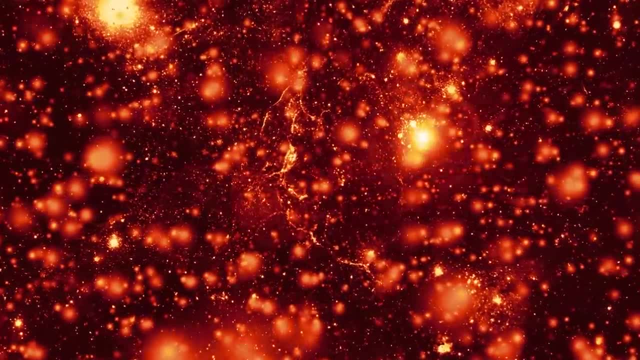 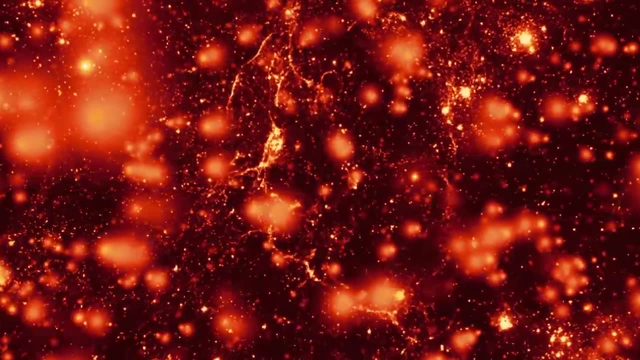 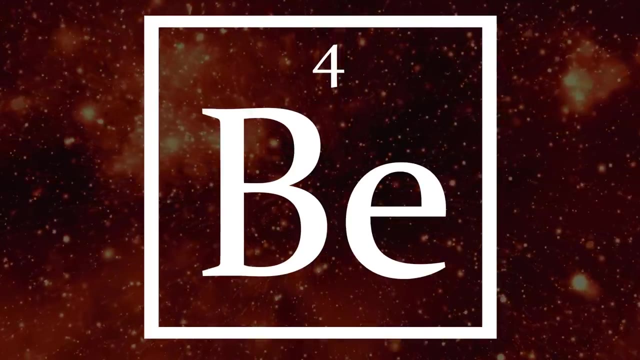 It is still blisteringly hot by human standards, but it is simply too cold for any further nuclei to form, and so at this point, only four elements exist: Hydrogen, Helium, Lithium and Beryllium, And, because of the short-lived stability of those beryllium nuclei, only the first. 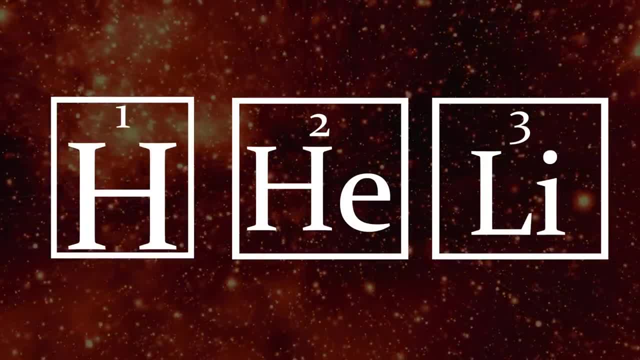 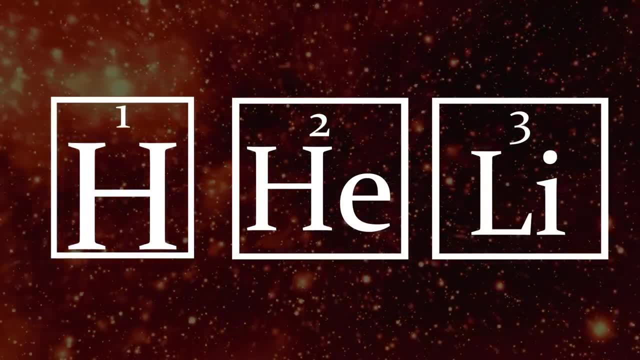 three will survive long enough to see the first stars and to become the ultimate fuel for creating the other 98 elements that could be found naturally within the modern universe. At this stage, there are 12 hydrogen nuclei for every helium nucleus and a billion photons. 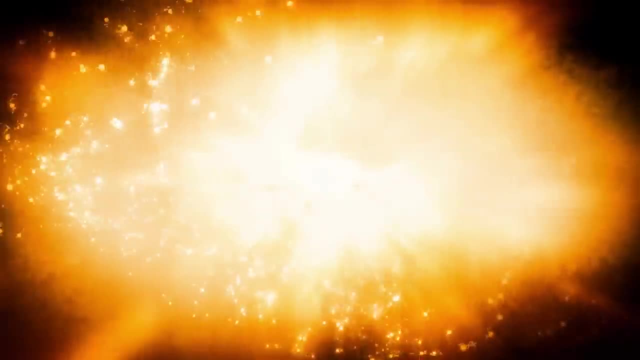 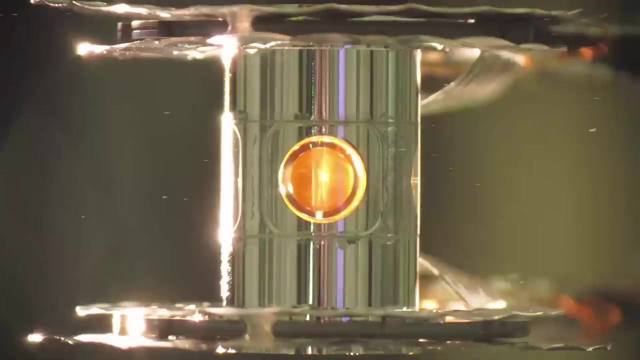 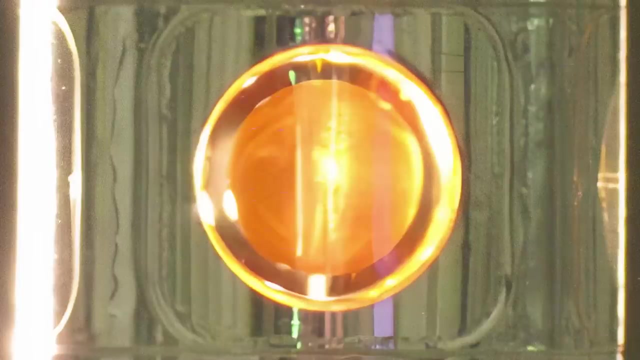 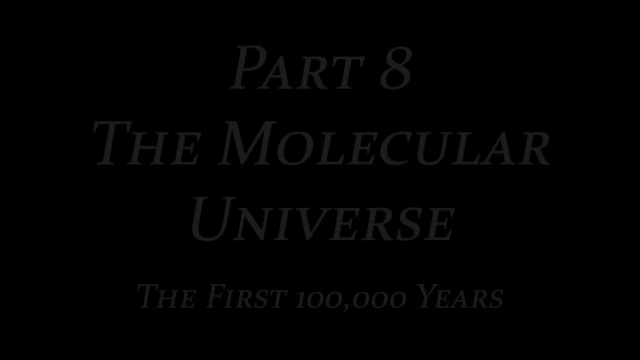 for every composite matter particle, but with these basic ingredients the stage is truly set for the formation of everything else. Even the deuterium and tritium that scientists fused together in California in 2022 was itself first formed in the heat of a newborn universe 13.8 billion years ago. 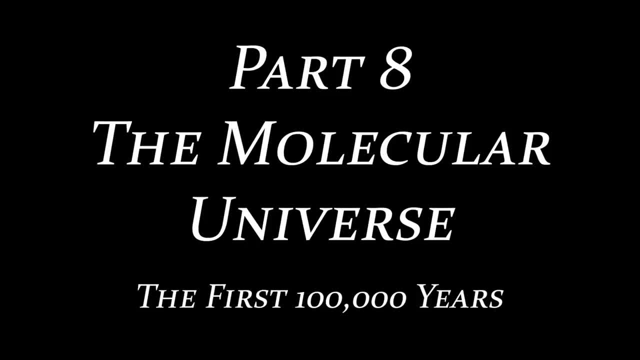 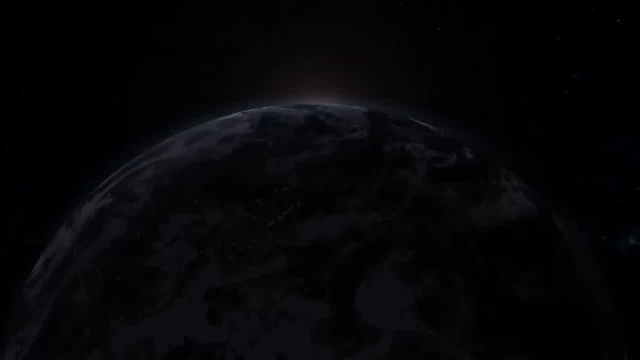 Life in the Universe is a Miracle of Chemistry. Life in the Universe is a Miracle of Chemistry. Life in the Universe is a Miracle of Chemistry And, as far as we know, that chemical miracle has only arisen in one place: On a nondescript, wet, rocky planet around an average yellow star sitting on the inner. 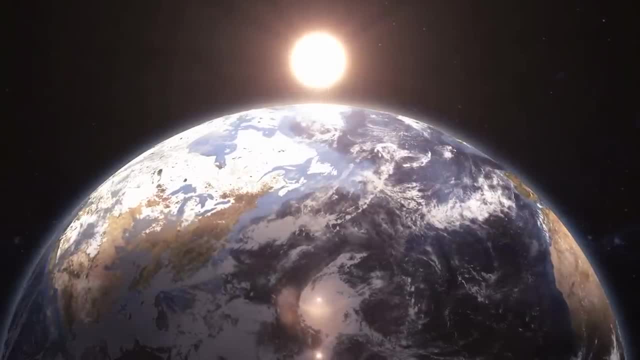 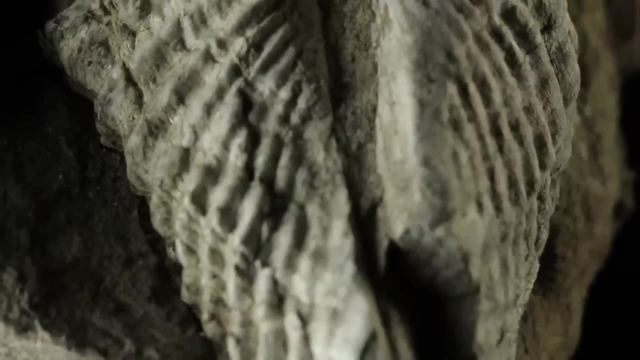 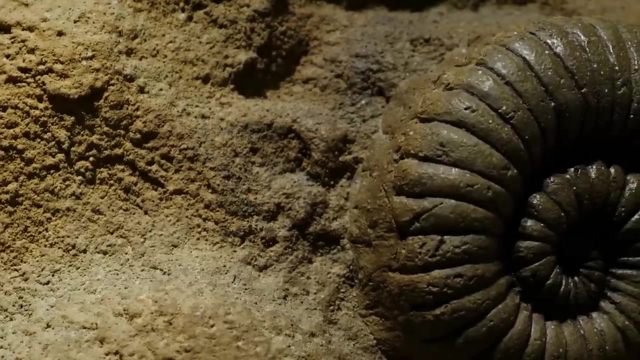 edge of one of the Milky Way's smaller spiral arms. But how did living things come to grace…the Earth, Despite a healthy fossil record that extends back through some 3 billion years of the planet's history, This moment of biological genesis, The spark of life? 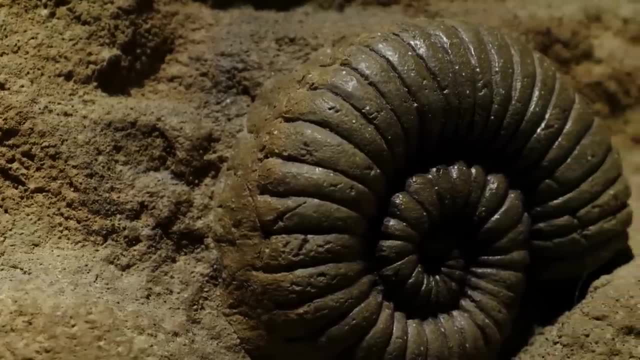 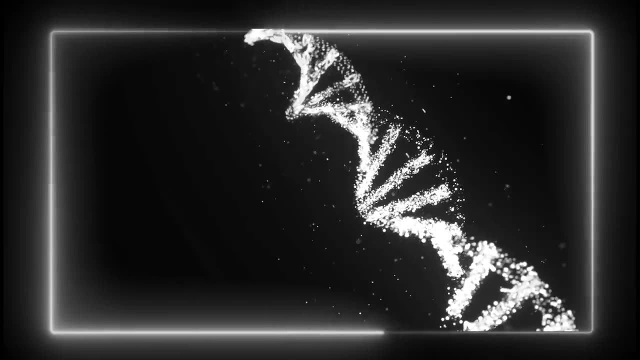 life is lost to the mists of time. Biologists agree that living things are composed of organic molecules made from carbon, oxygen and hydrogen. Added to that, they have discovered that all living things share a common chemical instruction manual in the form of DNA and. 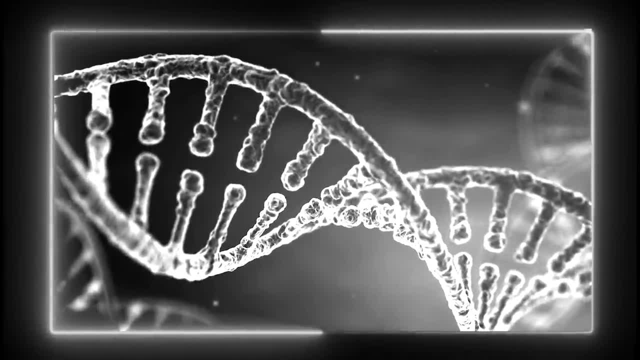 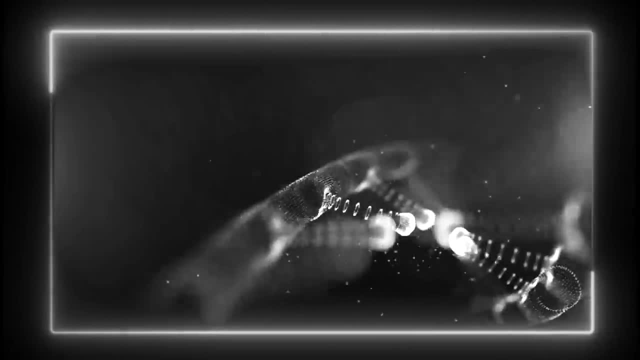 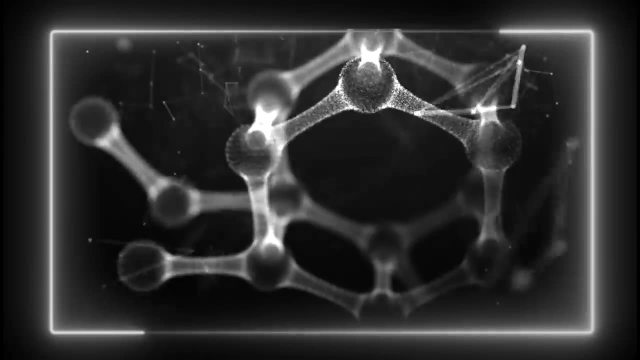 RNA, which are themselves composed of repeating units called nucleobases. Cytosine, guanine, adenine, thymine and uracil provide a universal language with which to encode information on how to grow a leaf, a flipper or a hair follicle. But where did these molecules come? 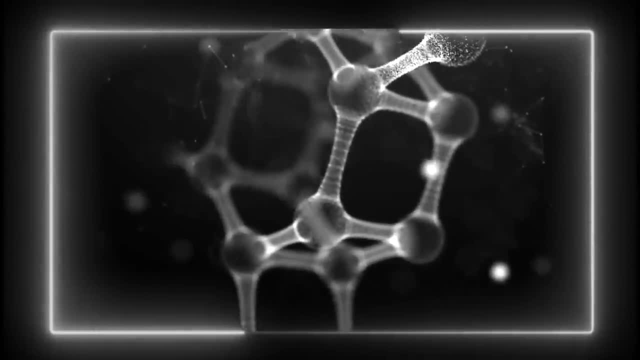 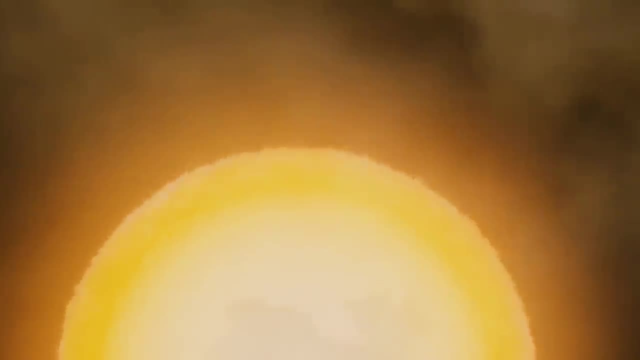 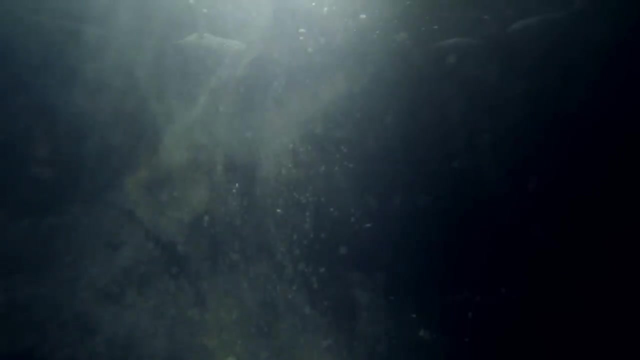 from in the first place. Some imagine that the warm and potent chemical environment on the newly formed Earth provided the perfect conditions for assembling organic molecules and nucleobases from scratch. But there is an alternative theory: that the ingredients for life were not created on Earth, But a 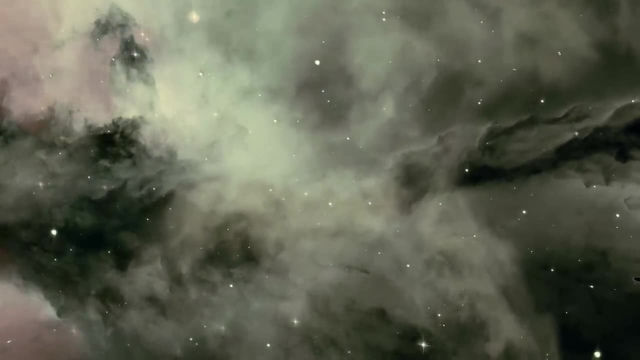 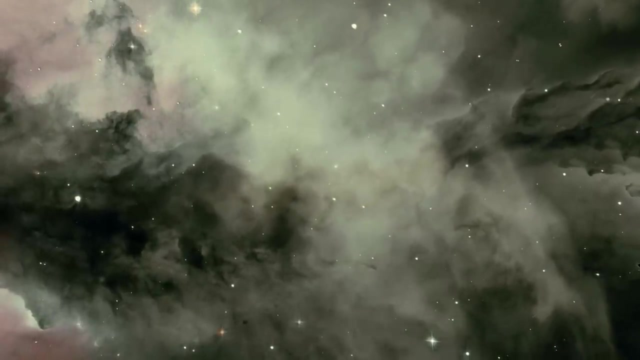 method of growing a leaf, a flipper or a hair follicle is a very simple one, and it's not the stars in the depths of space, And indeed we are finding compelling evidence for the stuff of life far out in the cosmos. 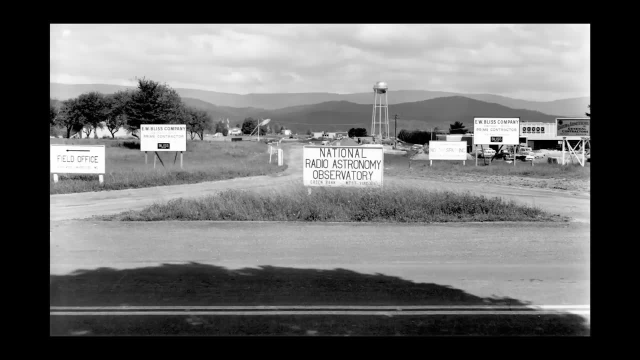 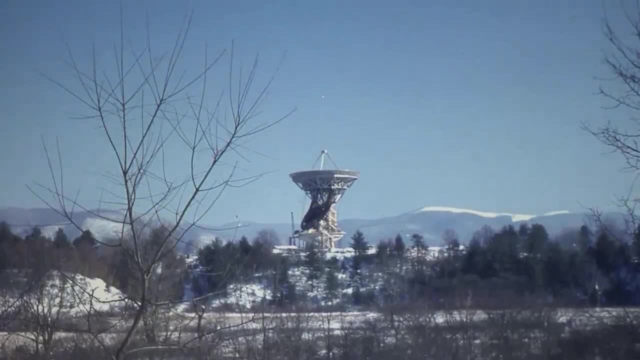 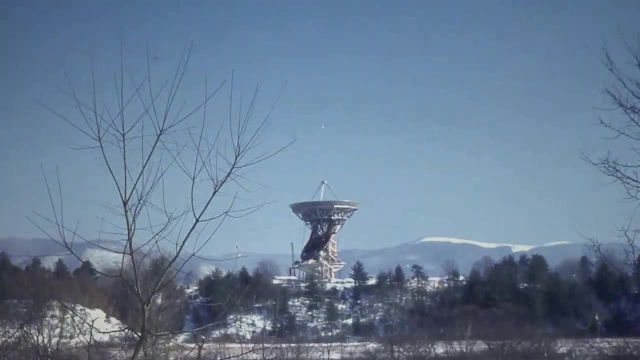 In 1969, American astronomers working out of the National Radio Astronomy Observatory in Greenbank, West Virginia, detected the characteristic vibration of formaldehyde molecules containing carbon hydrogen and oxygen deep in interstellar space, And many other complex molecules have followed. 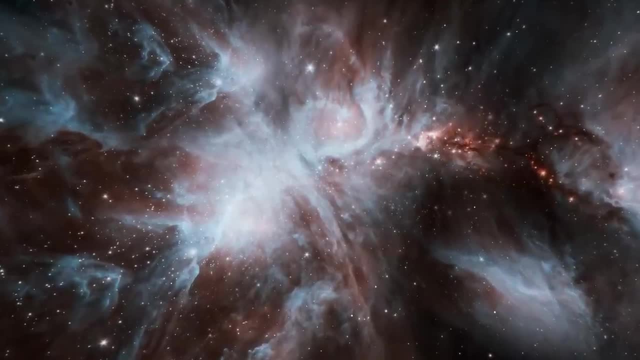 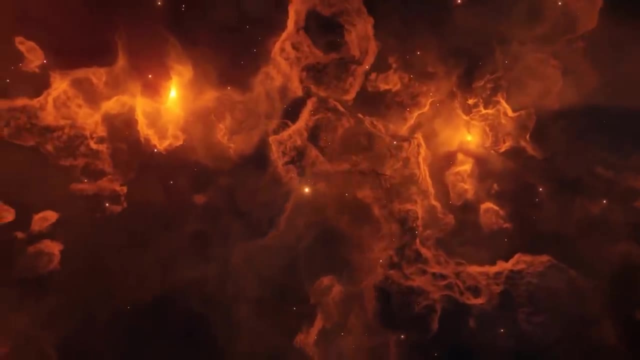 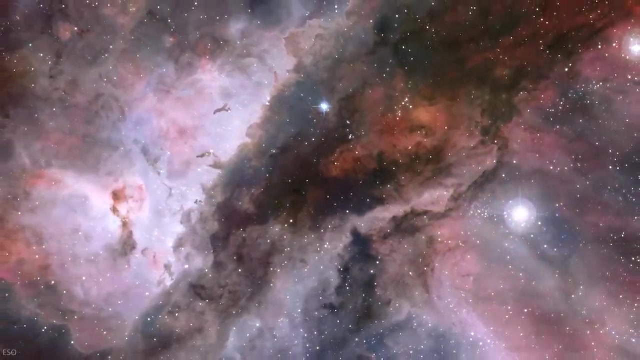 Scientists have now identified over 250 organic molecules inside interstellar clouds and in the shells of materials surrounding stars: Aldehydes, alcohols, acids and amines- all fundamental building blocks of the larger molecules of life lurking out there in the 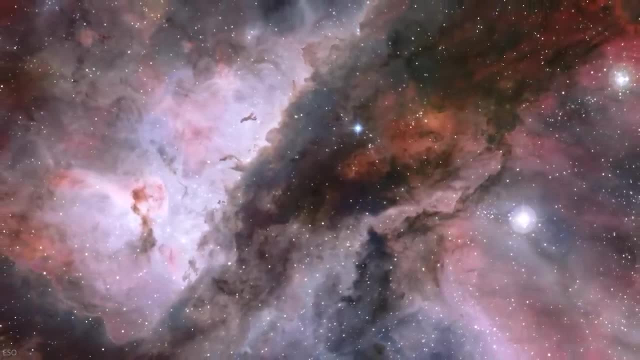 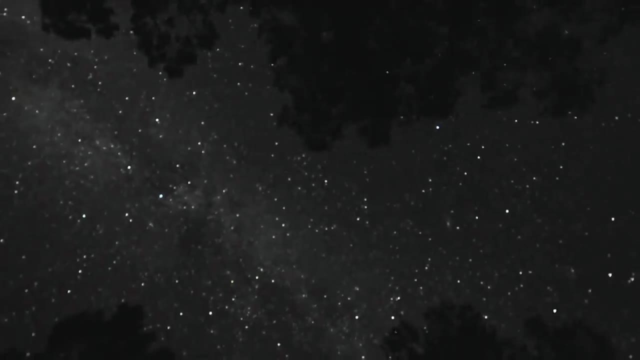 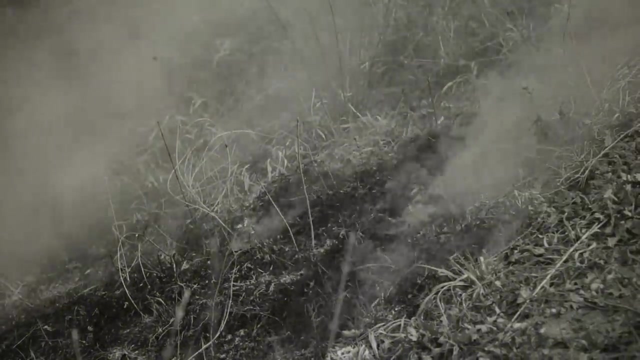 lifeless reaches of the atmosphere. Another, even more compelling clue to the life-bringing potential of outer space arrived on Earth as far back as 1864.. Just after 8pm on the 14th of May, a meteorite fell to Earth in around 20 pieces. 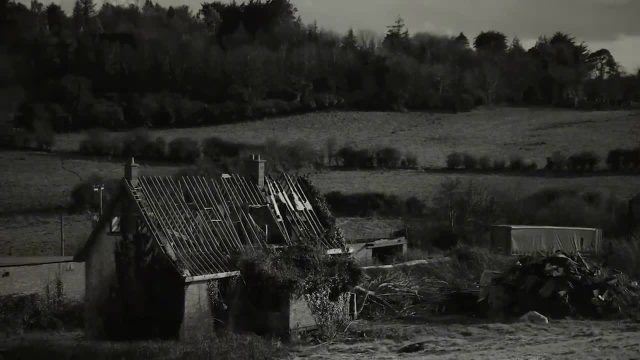 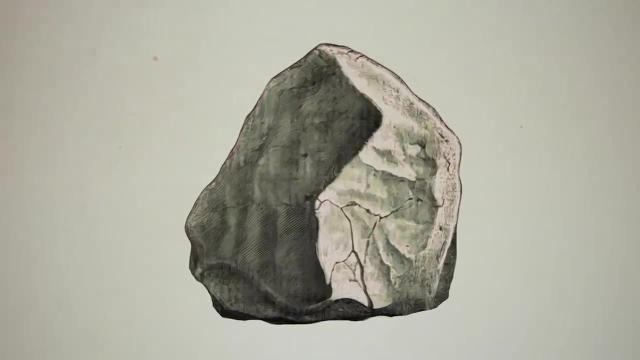 landing near the town of Augaille in southern France. The scientists who recovered and analysed the Augaille meteorite reported a composition very similar to peat, sparking intense debate over whether this or not was a meteorite. The meteorite was a meteorite that was found in the middle of the 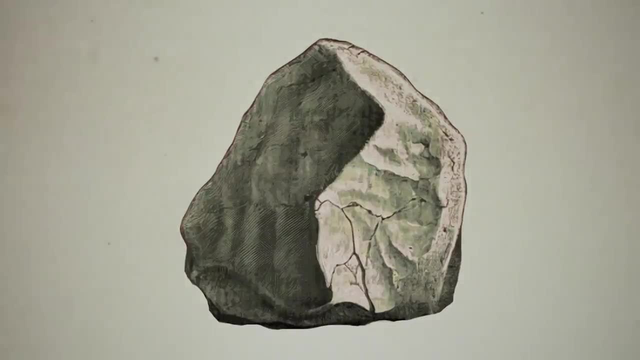 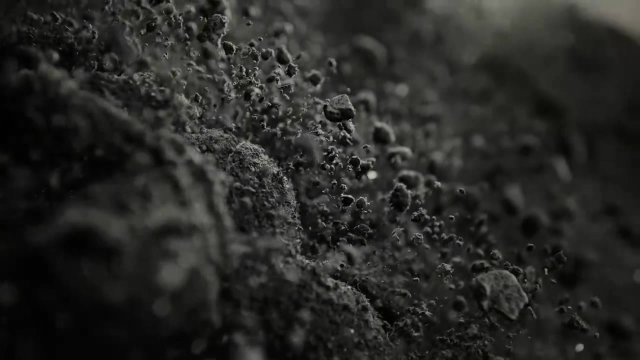 Atlantic Ocean. The meteorite was found in the middle of the Atlantic Ocean. This organic matter could have biological origin, But the lack of any identifiable biological structures made such a conclusion unlikely, Though, when the meteorite was re-analysed, almost 100 years later. 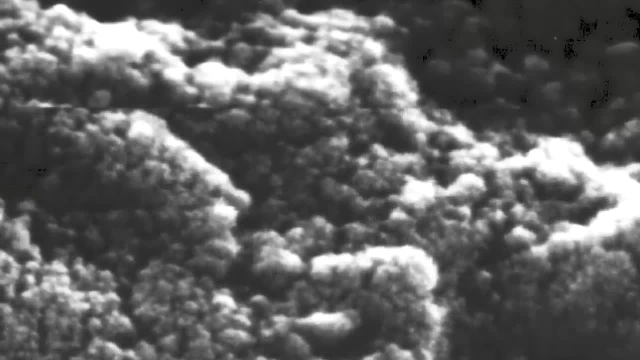 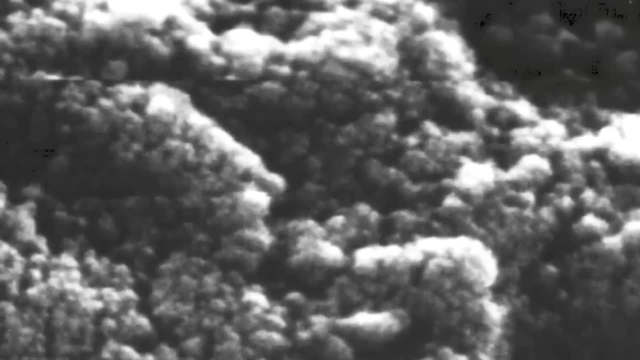 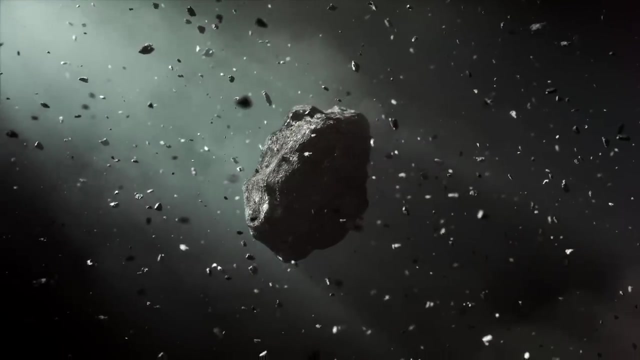 using more modern instruments and techniques, chemists were amazed to discover nucleobase molecules of adenine and guanine, identical to those we find in DNA and RNA today. Subsequent studies of other organic rich meteorites that have fallen all over the world have found the rest of Earth, life's nucleobases, as well as several others that 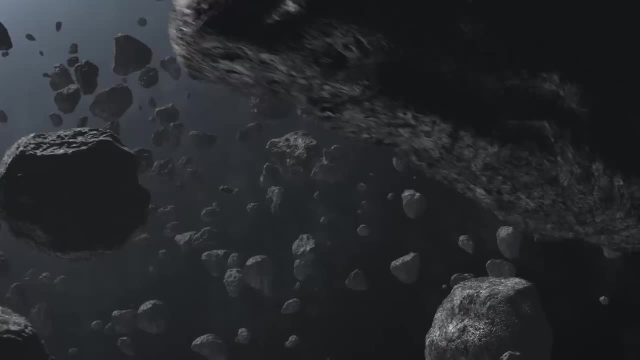 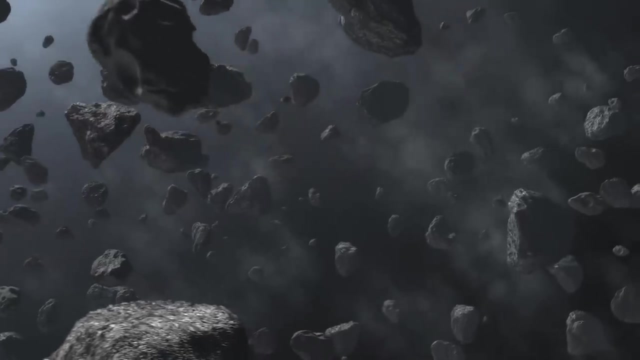 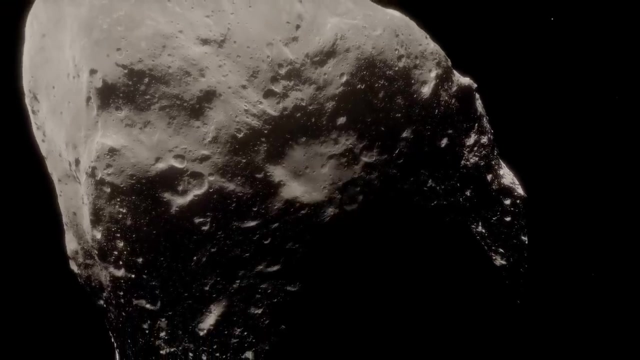 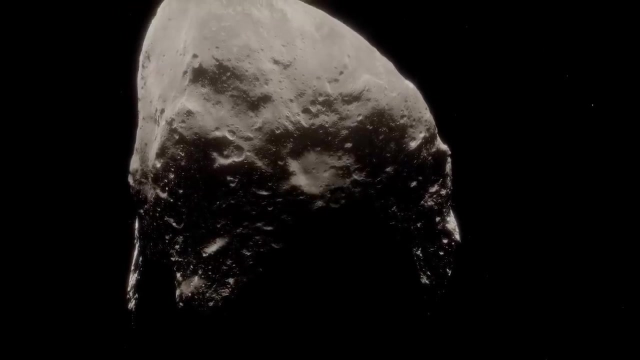 aren't found in our biological make-up. A definitive answer to this question has yet to be revealed, but the observations so far do at least point to one certainty, a surprising truth about the cosmos. Without any special provocation or encouragement, the universe itself has the capacity to build molecules and perform remarkable acts of chemistry. 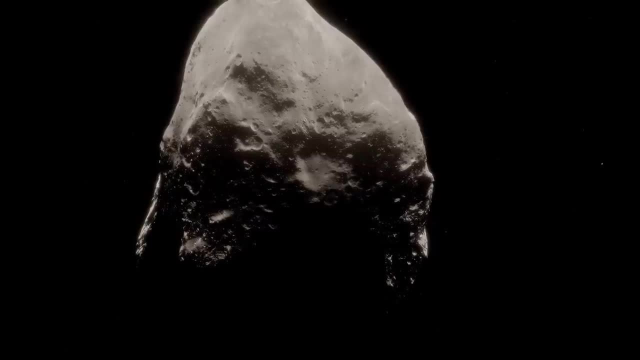 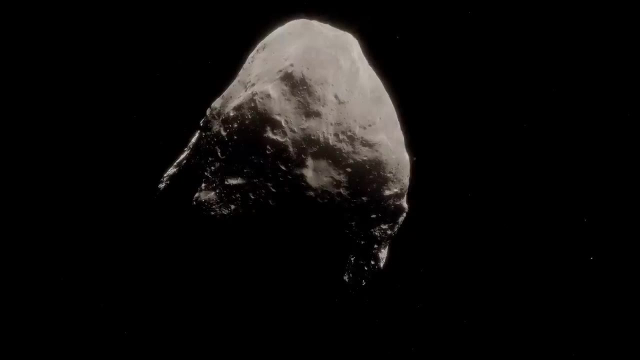 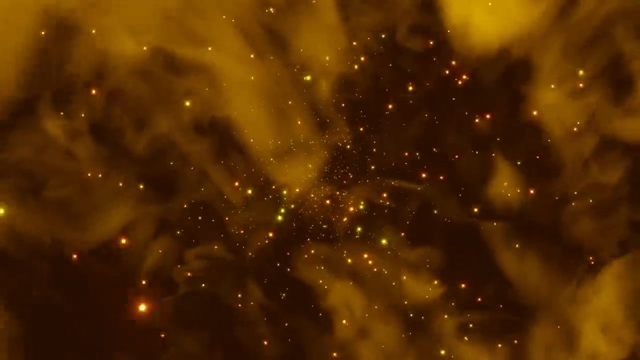 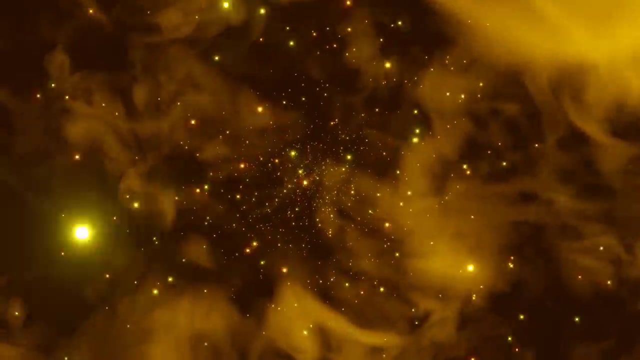 And this space chemistry had its beginnings right back in the infant universe, less than 100,000 years after the beginning of time. The furious act of elemental creation during Big Bang, nucleosynthesis had ground to a halt after just 20 minutes of universal existence, as the cosmos expanded and cooled The ambient. 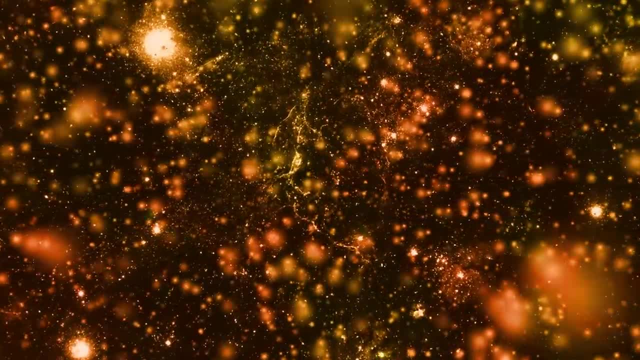 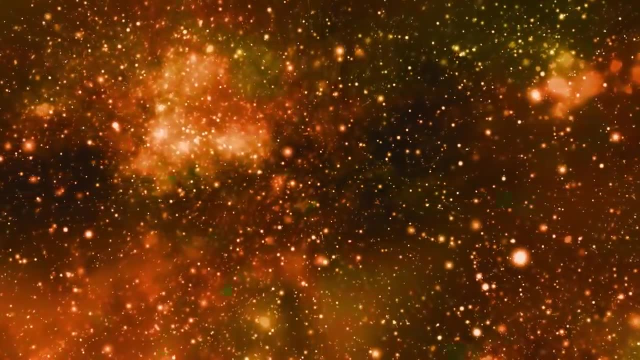 energy was no longer high enough to fuel nuclear fusion, but conditions like the ones in the universe were still extreme. The entire cosmos was still denser than the air we breathe and temperatures still too high for lightweight electrons to slow down enough to 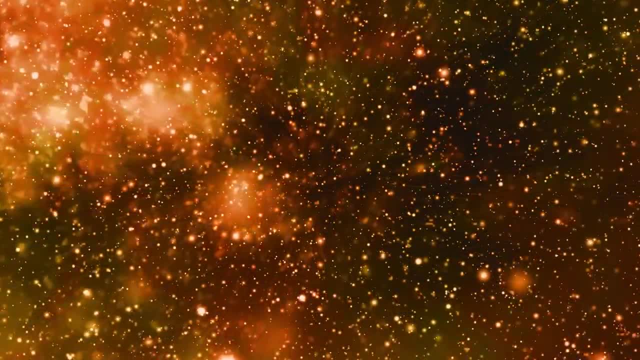 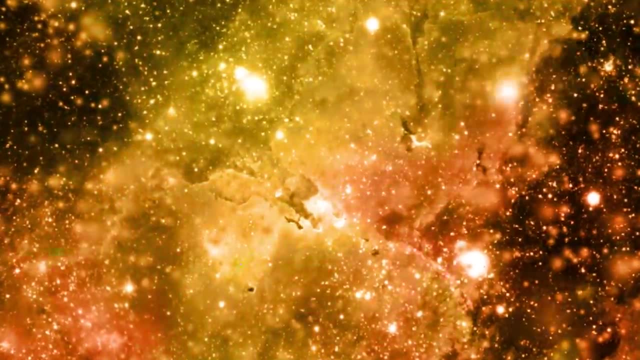 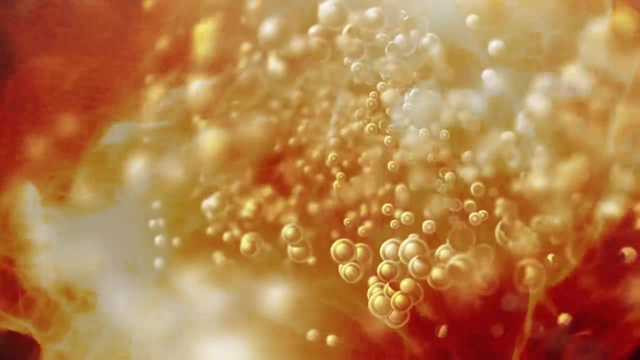 be captured by the newly formed elemental nuclei. There was also still more energy than matter in the universe, which exists as a hot, disassociated plasma, and it will still be tens of thousands of years before further cooling allows anything to begin to change. And yet something is happening. 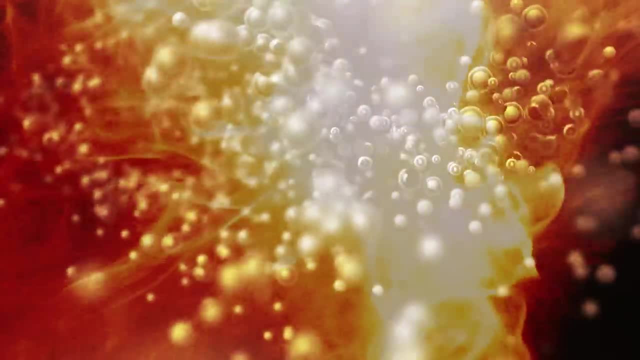 in the chaos. The universe is still hot, disassociated plasma, and it will still be tens of thousands of years before further cooling allows anything to begin to change. And yet something is happening in the chaos. First created in labs in 1925,. 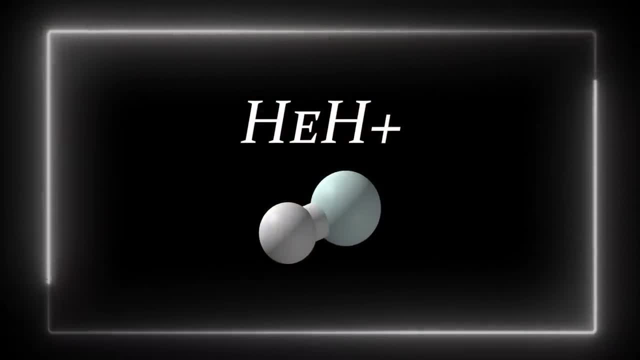 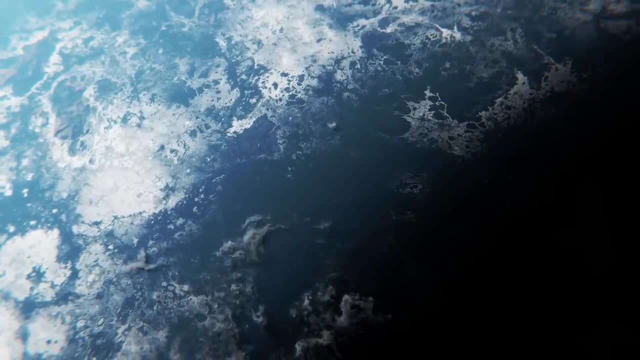 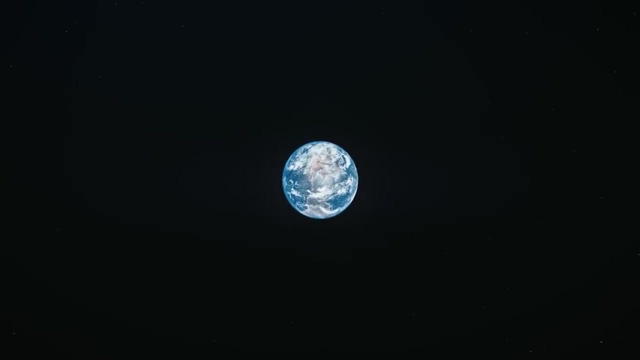 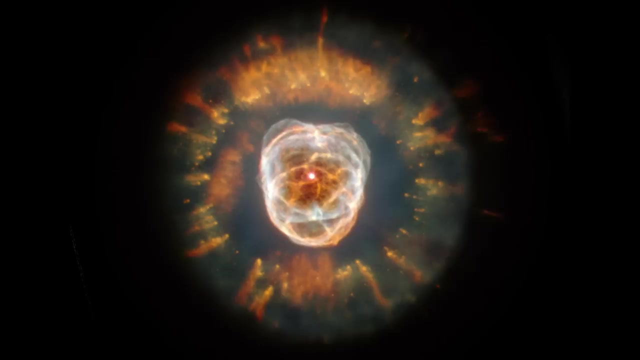 helium hydride is an unstable ion of helium bonded with hydrogen very rarely found in nature, And in 1978, astrochemist John H Black at the University of Minnesota suggested that it could be found in abundance in space, Specifically in planetary nebulae which form from the energetic 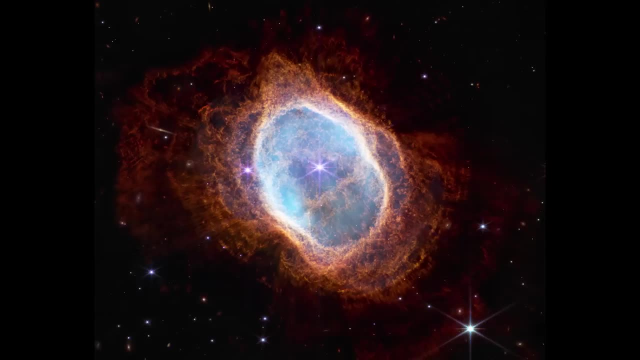 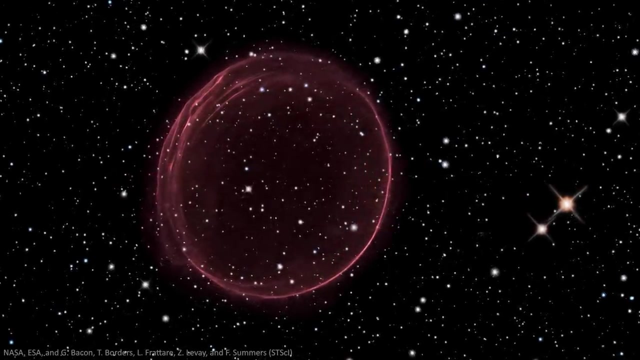 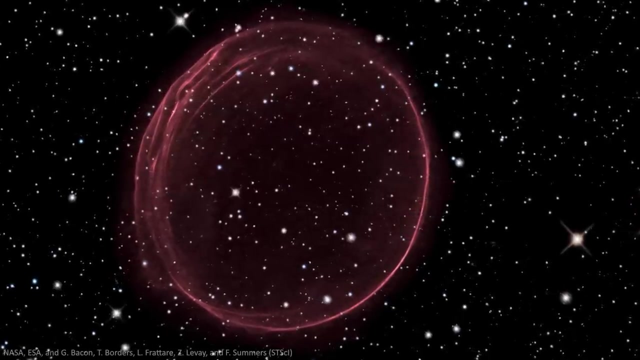 industry of the solar system, of the universe. it is said that the helium ions – the strong need for electrons to neutralize their charge – could drive them to steal one from the only other source around: the hydrogen: The association between these two in the superheated nebula. 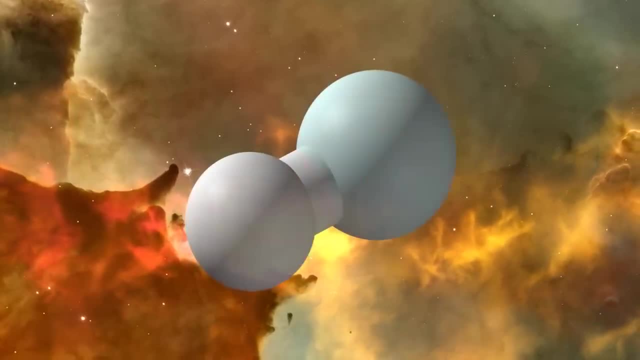 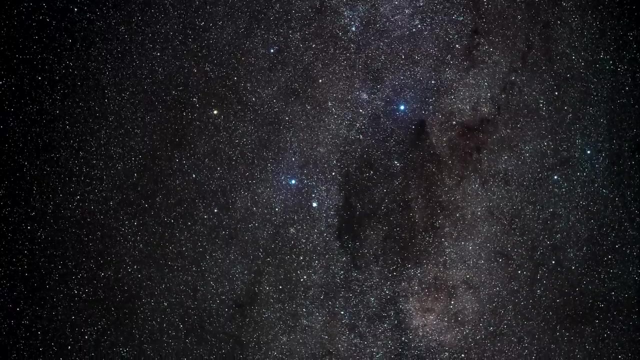 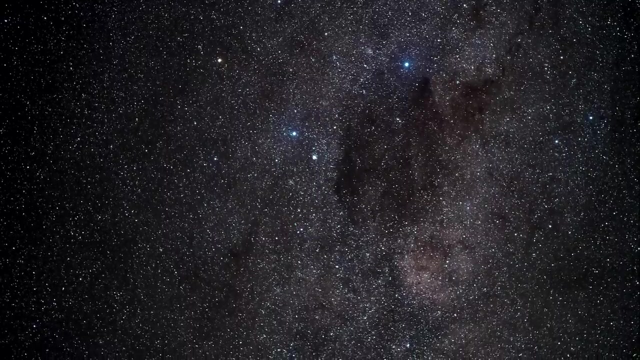 would ultimately lead to the formation of helium hydride ions, And yet the molecule continued to prove elusive. A long search ensued, with frustratingly little success. That was until 2019, when an innovative telescope managed to achieve the seemingly impossible. 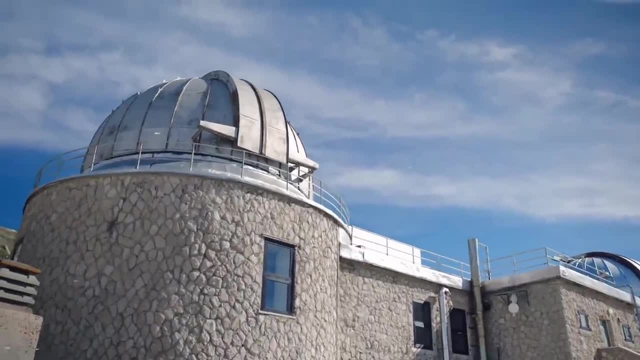 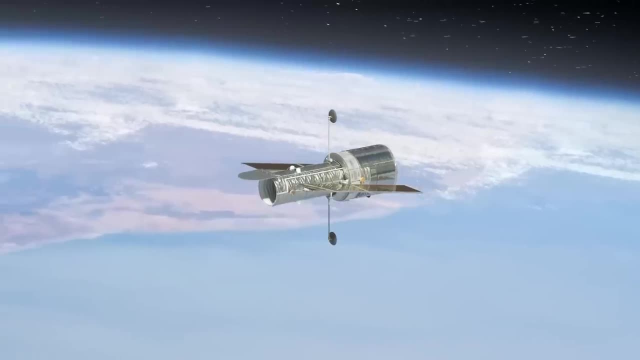 These days, most telescopes are either based on the ground, situated high on mountaintops, to avoid the worst of light pollution, weather and atmospheric distortion, or they're launched into space to get rid of those problems altogether, as they orbit the Earth or the Sun. 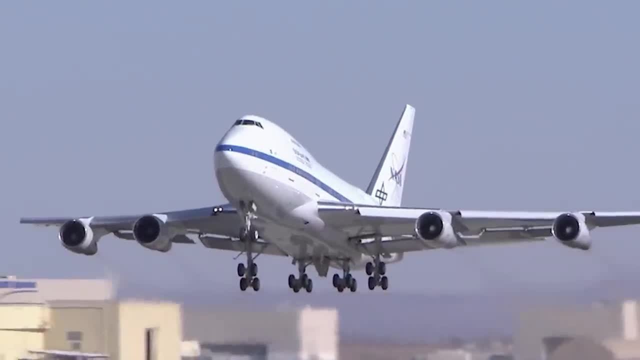 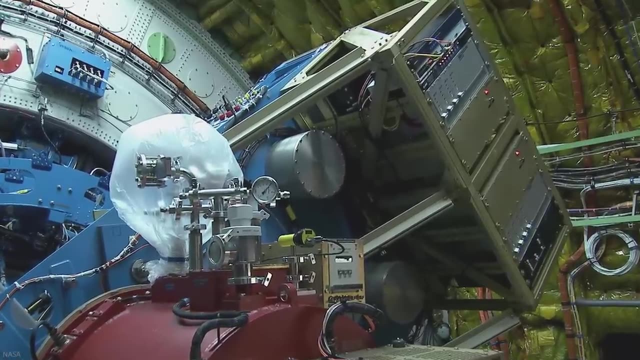 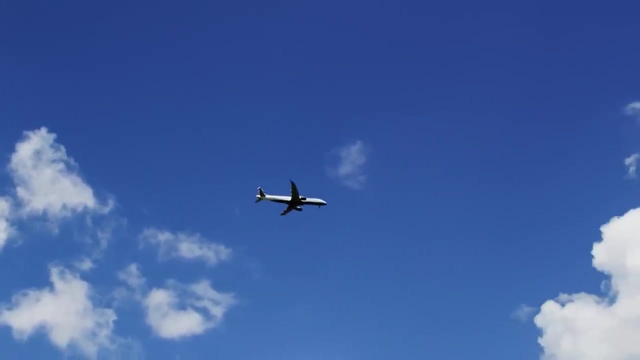 But the SOFIA observatory did something different. It consisted of a 2.7-metre-wide mirrored telescope that was pointed out the back door of a specially adapted Boeing 747, flying at over 43,000 feet. At this height, the instruments connected to the telescope could 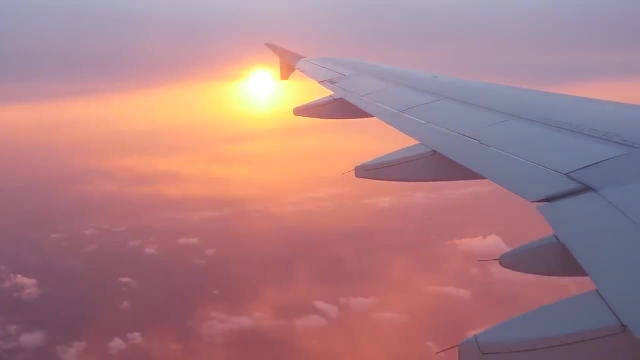 enjoy many of the benefits of a space telescope, since they would be lifted above the majority of the world. But the telescope was not the only one. The instruments connected to the telescope could also be used to probe water in the Earth's atmosphere, allowing them to probe wavelengths of 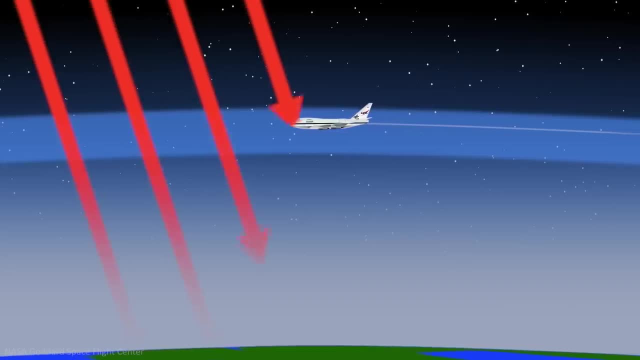 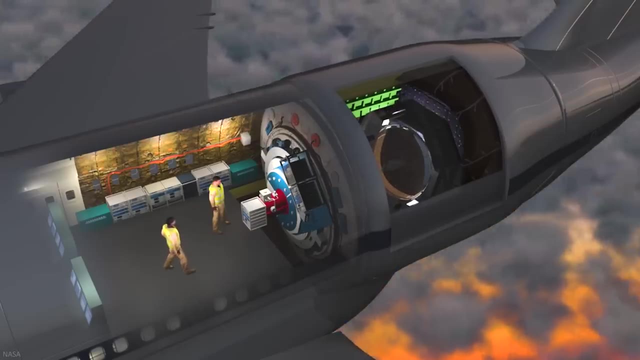 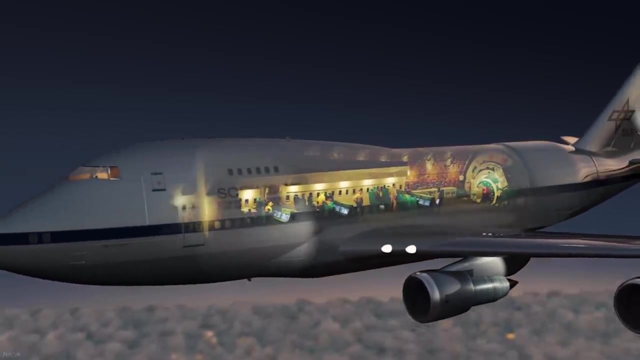 light that water vapour usually absorbs And, critically, the telescope connected to the Far Infrared Receiver, known fittingly by its acronym GREAT, which had sufficient resolution to finally pick out the faint overlapping signature of helium hydride ions in deep space. 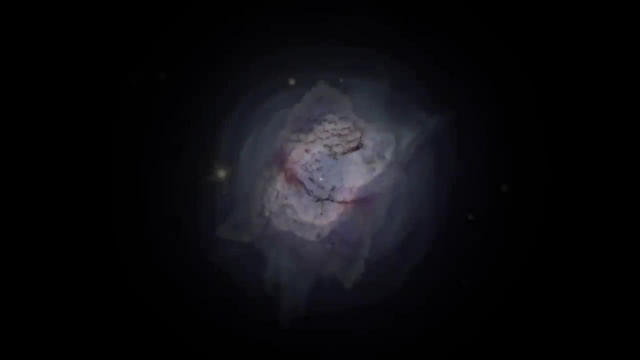 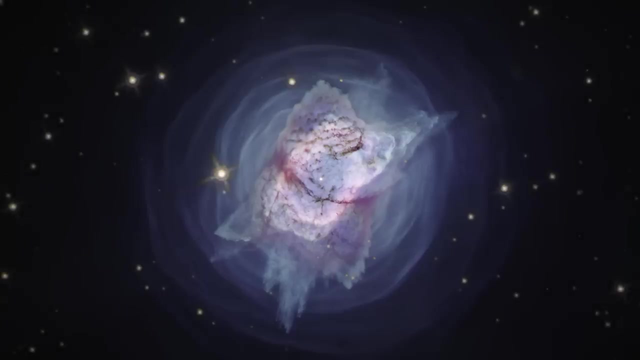 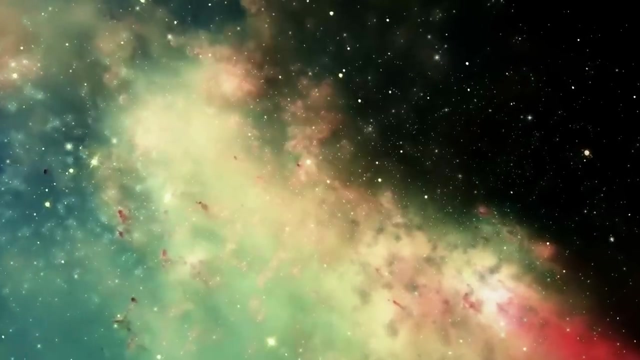 In the end. the detection came from three days of observation on a planetary nebula designated NGC 7027, which sits about 3,000 light-years away from Earth in the direction of the Cygnus constellation. In this hot and energetic interstellar environment, 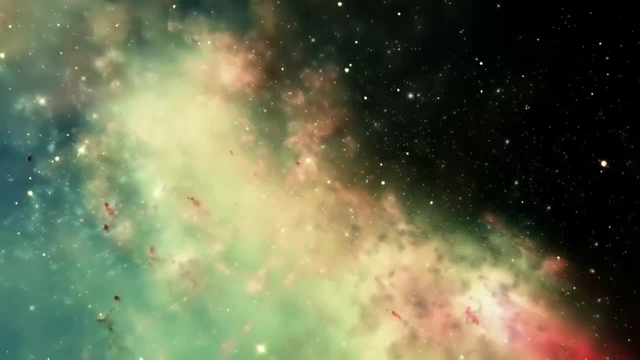 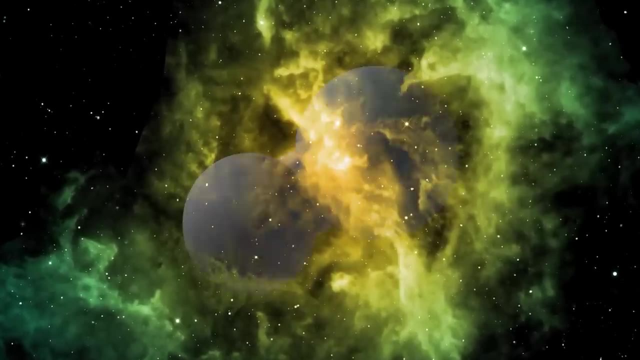 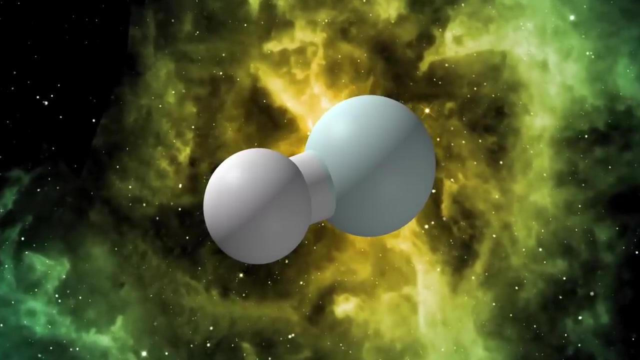 just as John Black predicted 40 years earlier, helium hydride is able to form and leave its signature on the nebulous spectrum. Detecting this signal is a triumph for nearly 100 years of experimental and theoretical chemistry, But the implication, however, of its discovery here is even greater For the conditions inside this distant nebula. 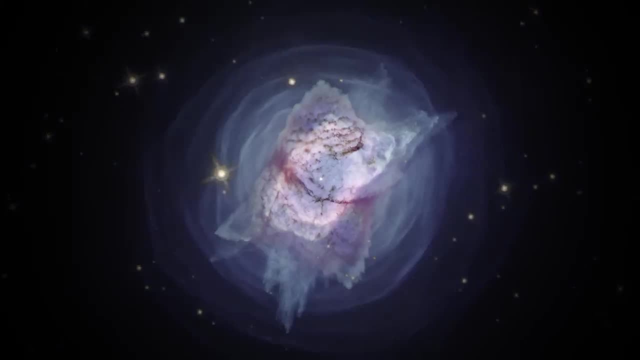 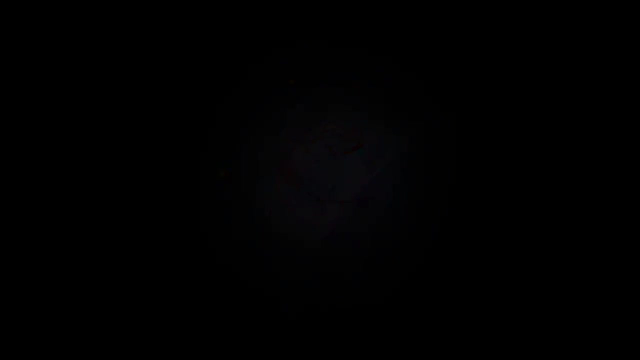 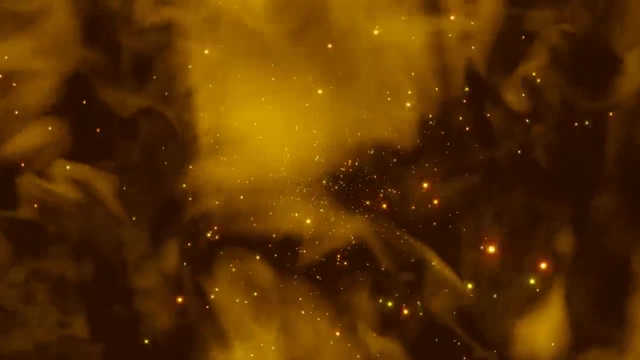 are very similar to those that prevailed throughout the whole universe. within its first few tens of thousands of years, Big Bang Nucleosynthesis was very efficient at creating atomic nuclei, But for hundreds of thousands of years afterwards, cosmic energies remained too high for hydrogen deuterium and 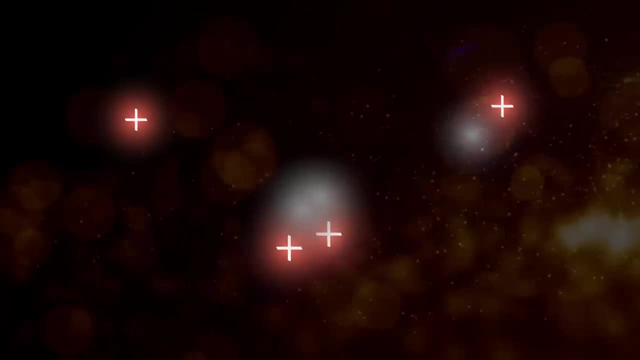 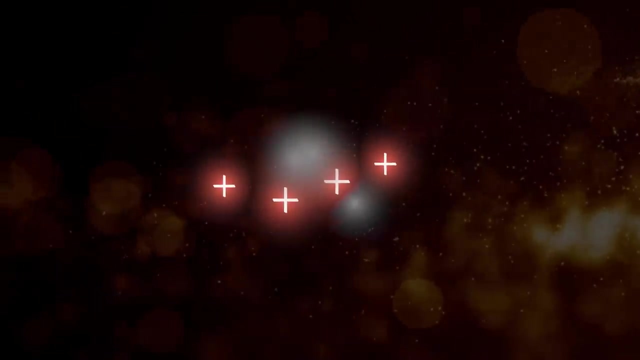 helium to combine with electric energy. So with the advent of the NGC 7027, the NGC 7027 was able to create electrons to make uncharged atoms. However, when ambient temperatures dropped to around 4,000 Kelvin, those wayward nuclei were able to combine with each other in a specific order governed by what's known as their ionisation potential, And it is because of this that helium is today considered the most noble of all the noble gases. It is the most inert and the least likely to react because of the huge amount of energy it takes to strip away one of its electrons. and transform it into a nuclear. This is the reason why the NGC 7027 is so important to us. It is the most likely to react because of the huge amount of energy it takes to strip away one of its electrons and transform it into a nuclear. 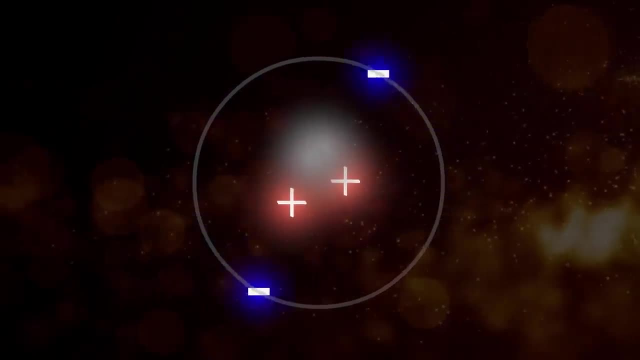 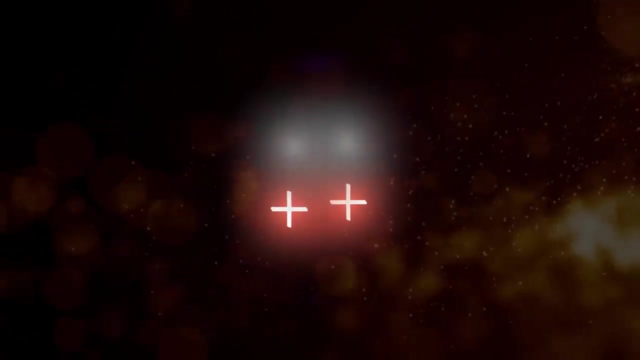 It is the most likely to react because of the huge amount of energy it takes to strip away one of its electrons and transform it into an ion. But in the early universe, when all that existed were ions, particles with net charge, this supreme grabbing power means that helium was the first element to attract. 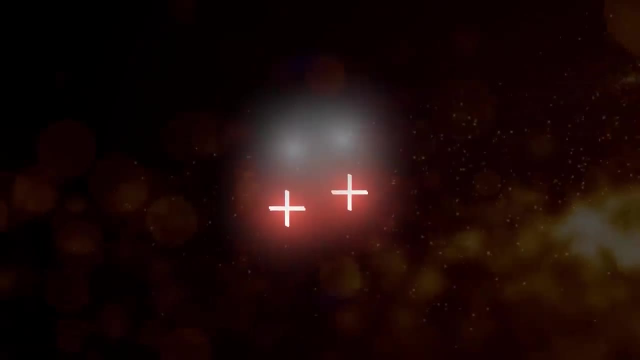 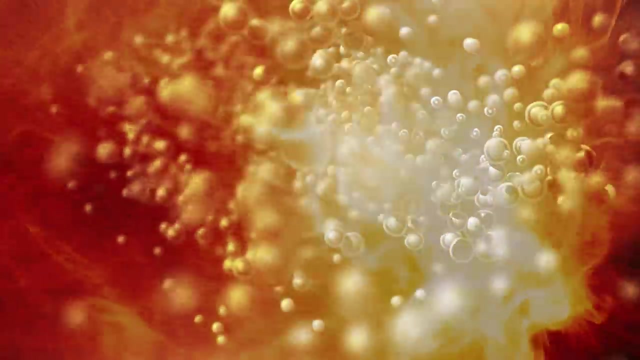 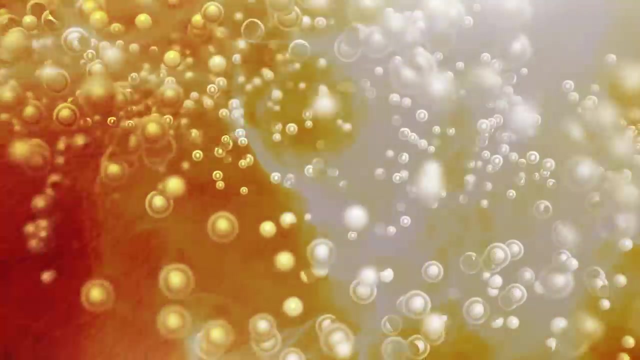 electrons and hold onto them, forming the very first uncharged atoms. However, this stability for helium was sadly short-lived. It was still too hot for lone protons to capture electrons to make hydrogen atoms. so the protons turned to the helium and its balancing complement of electrons, seeking an arrangement where they 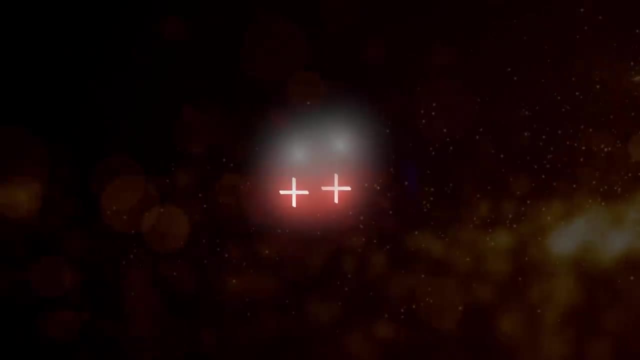 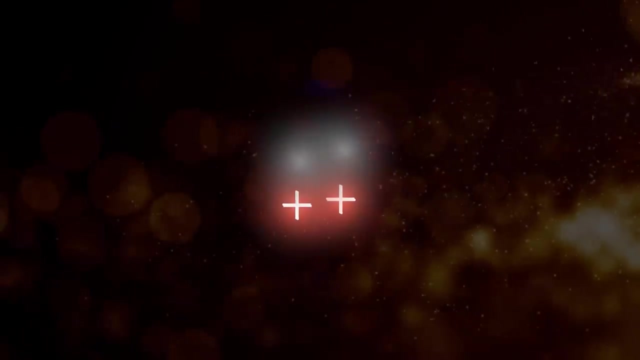 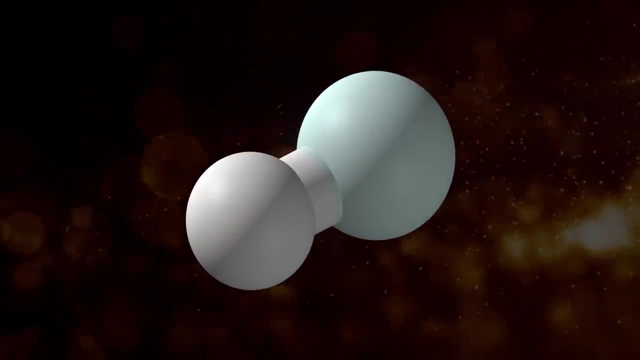 could share. And so eventually, under the crushing burden of these clingy protons, helium relented, forming the very first chemical bonds and the first molecule in the universe creating very unstable helium hydride ions in the process. And despite this instability, 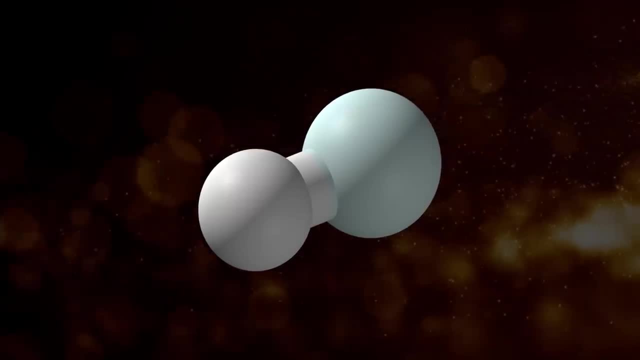 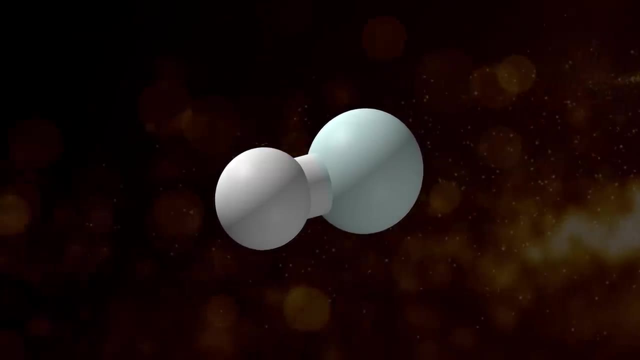 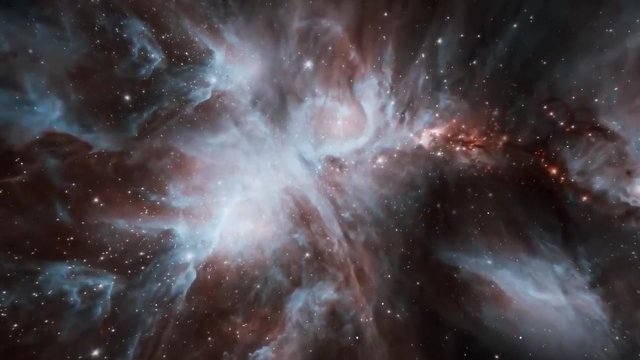 these short-lived molecules paved the way for the creation of other molecules and the beginning of space chemistry, Around 100,000 years having passed since the big bang. Today, the field of astrochemistry is well developed as the study of what molecules 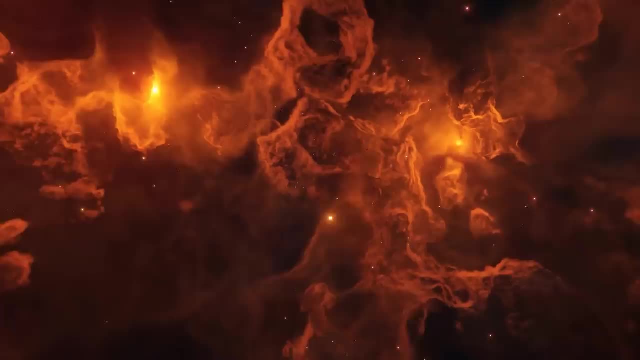 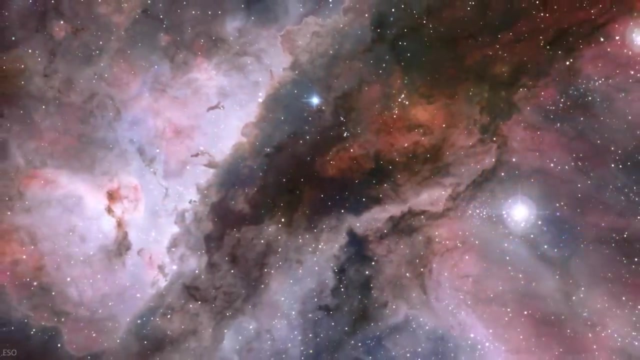 we can expect to find in space and how they form. Many atomic structures that are found on Earth are also common throughout the cosmos, including water and ammonia, But others are much more exotic, like dihydron, monochloride cations or hydroperoxides. 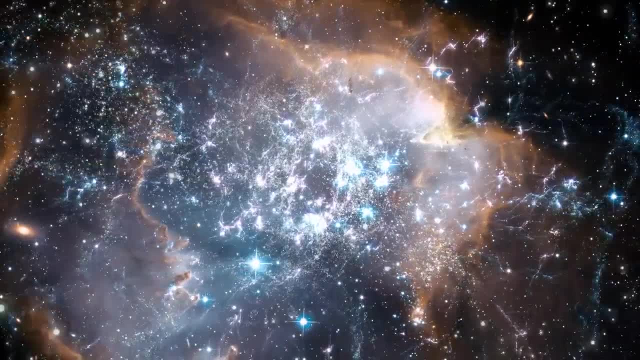 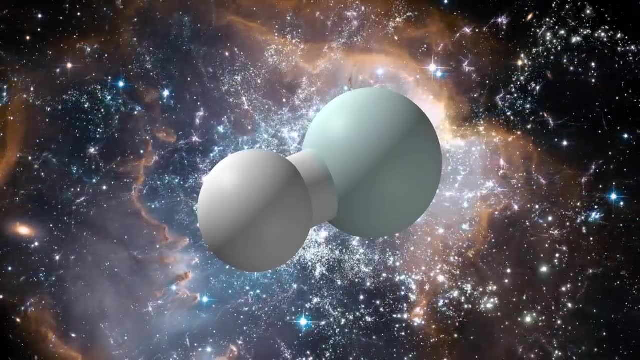 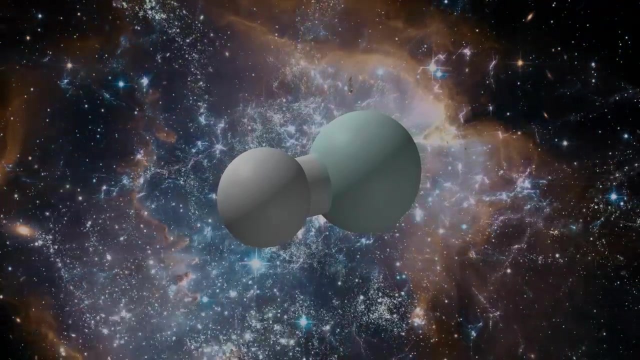 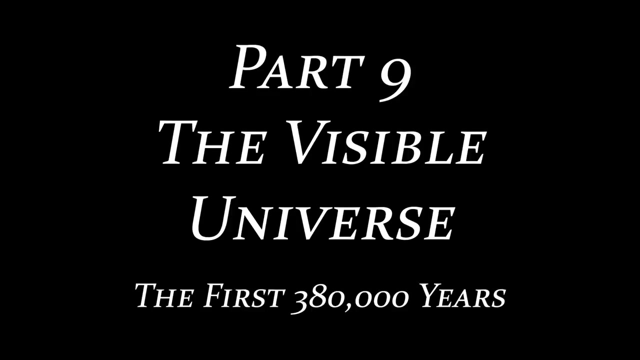 Though many are yet to be discovered. whatever they turn out to be, they ultimately owe their existence to helium hydride ions, made and unmade, in the first 100,000 years of the universe. You may think that you have a good grasp of the world that surrounds you. 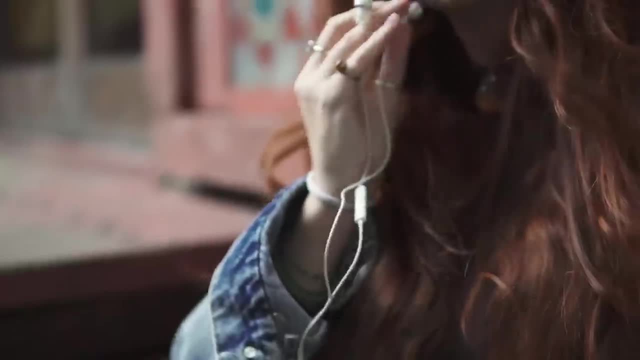 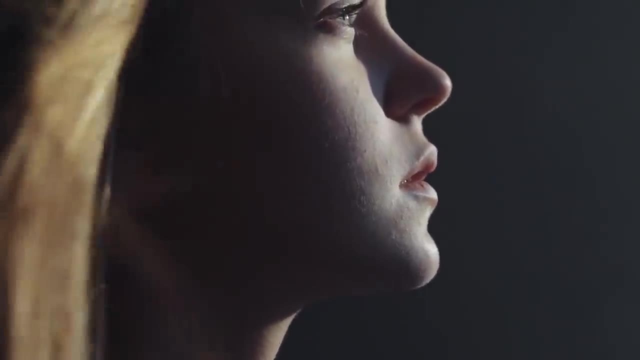 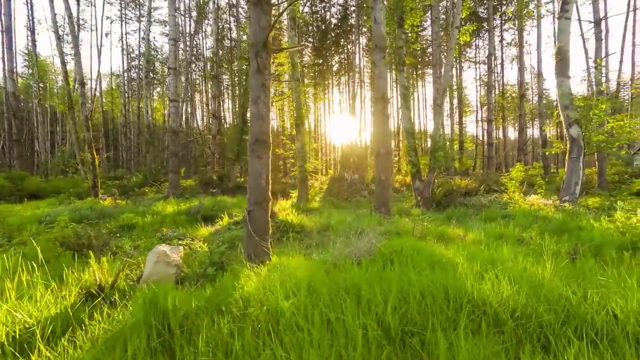 With specialised organs dedicated to sensing light, sound, the solid touch of matter and the chemical nuances of molecules, our brains seem well-fitted to perceive all the possible stimuli the universe can provide, But this simply isn't true. There is much. 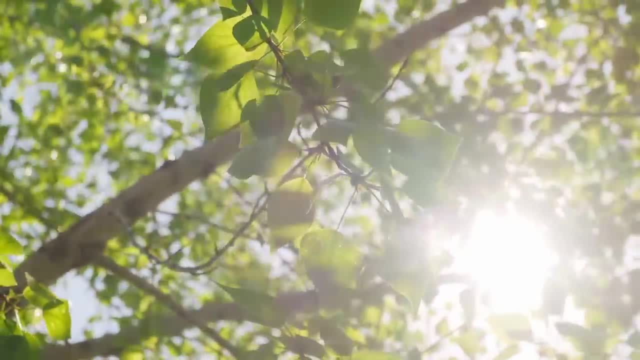 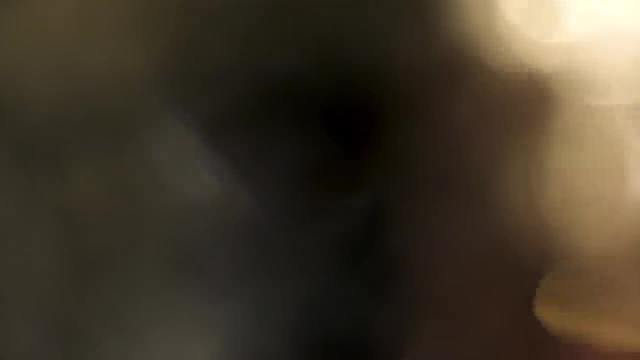 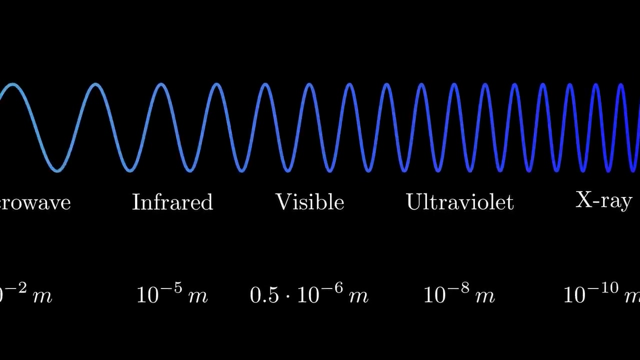 much more to reality than meets the eye, ear or fingertip. Take light: Most of us are able to see the world in glorious, sharp-focused technicolour. But visible light is just a tiny fraction of a wider electromagnetic spectrum. 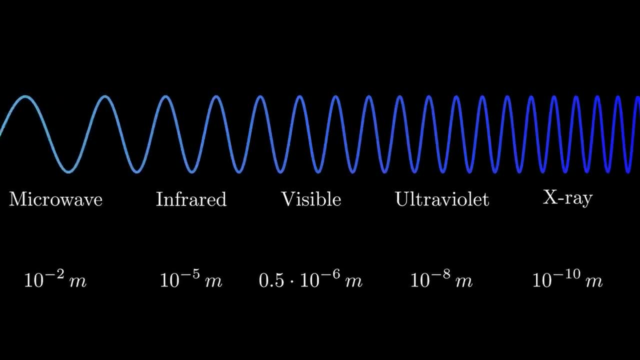 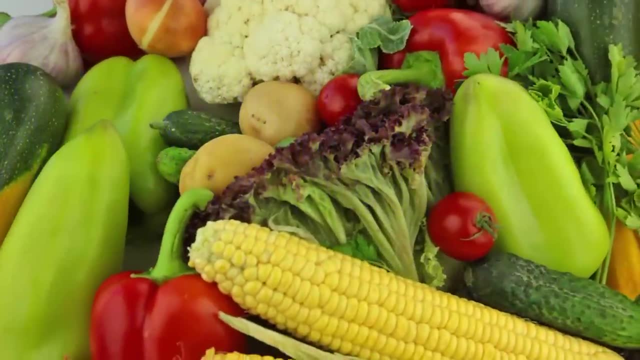 whose waves are constantly and imperceptibly washing over us every moment of our lives. High-energy gamma and x-rays are emitted by the food we eat, the bricks that make up our homes and even our own bodies. The radiative energy from the sun which we may think we can perceive. 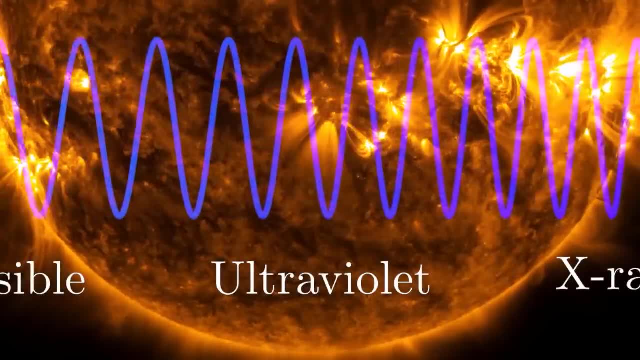 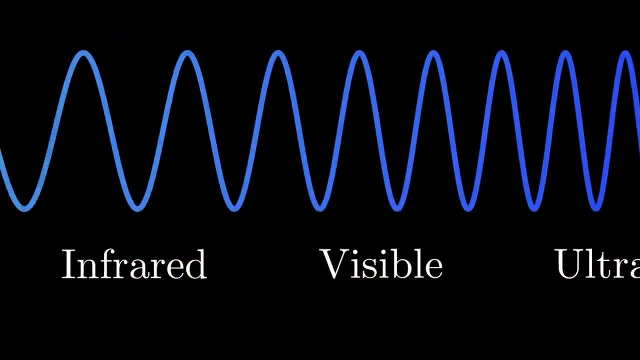 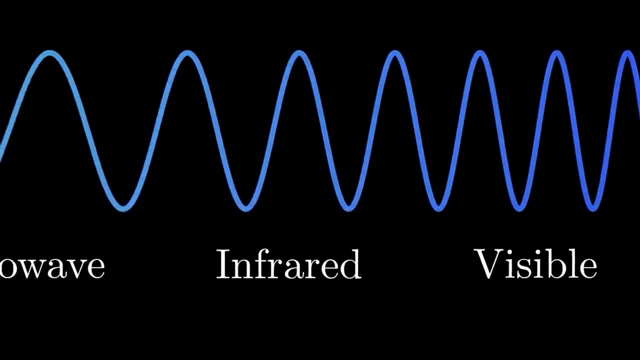 contains around 10% ultraviolet light, with the capacity to penetrate and damage our skin and eyes, And at energies lower than visible light. sunlight is composed of around 50% infrared radiation, some of which we experience as heat, But even at lower energies, infrared technologies like motion sensors and television remotes. 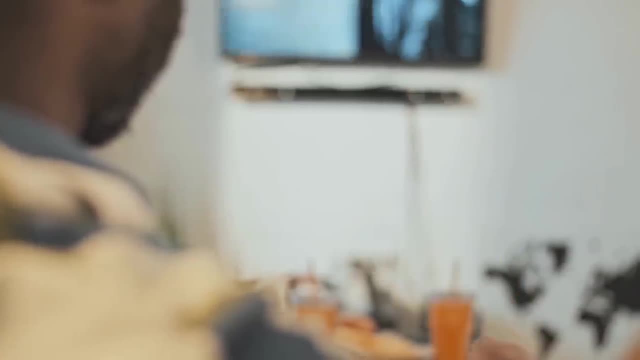 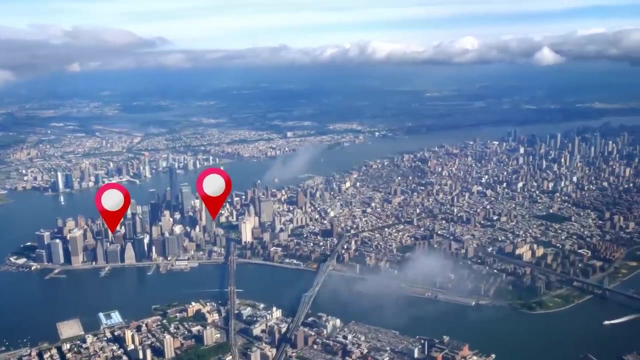 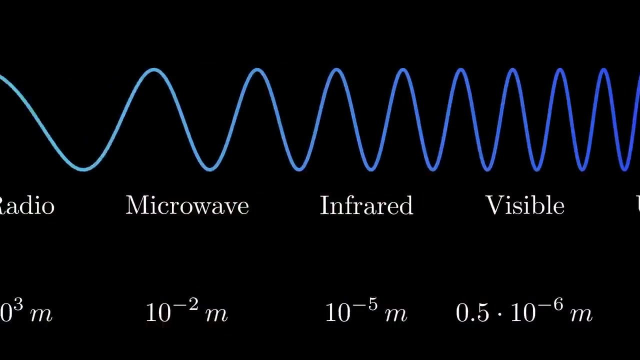 send and receive their signals entirely undetected. Bluetooth, Wi-Fi, cellular, mobile and GPS all work by exchanging information through the air via microwave frequencies of radiation. Meanwhile, our analog radios and televisions use the longest wavelength of EM radiation – radio waves. 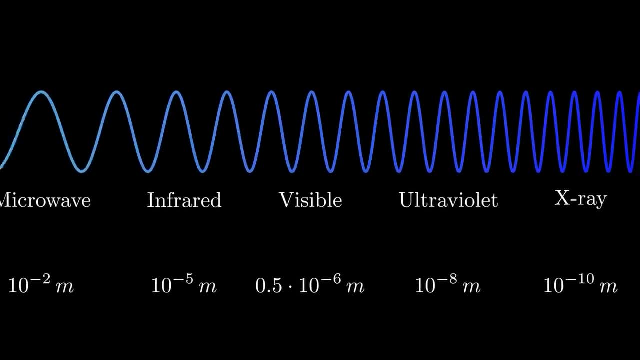 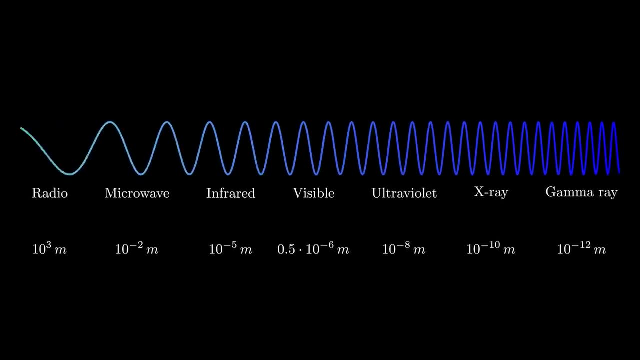 If we could see all of them, we would be blinded, All told. for all our apparent sentience, we are unaware of at least 99% of what is occurring within the universe. Perhaps this is just as well, as it is hard to imagine how our brains could adapt to cope. 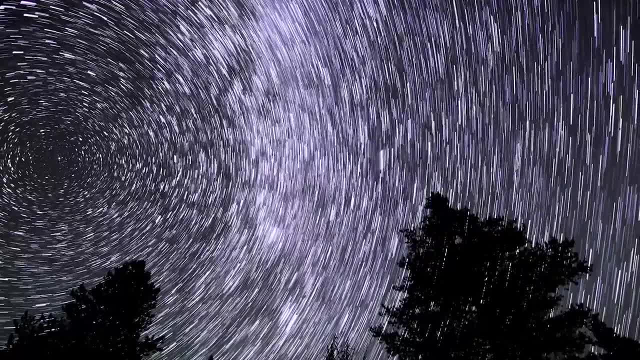 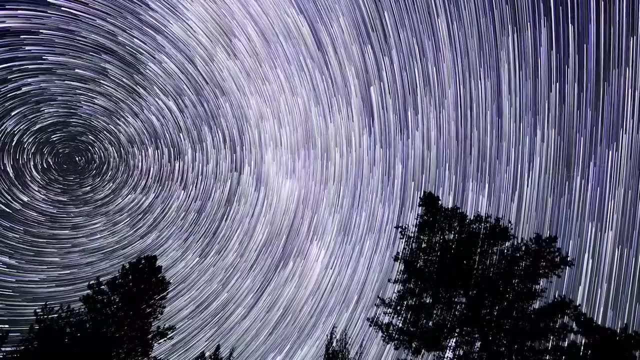 with all the possible stimuli, The relative calm of a night sky. It would be a blaze of colour and a riot of sound, with sharp points of light and song from a multitude of sources, And behind it all, everywhere, a faint backlit glow. 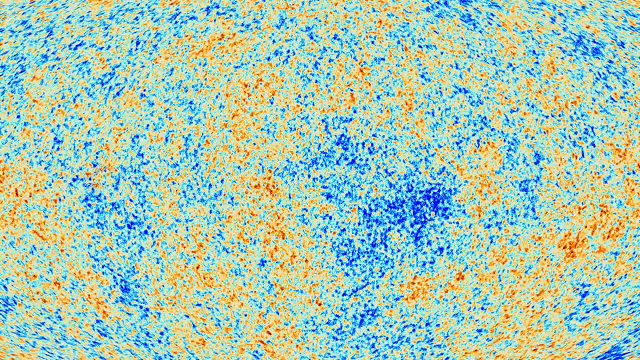 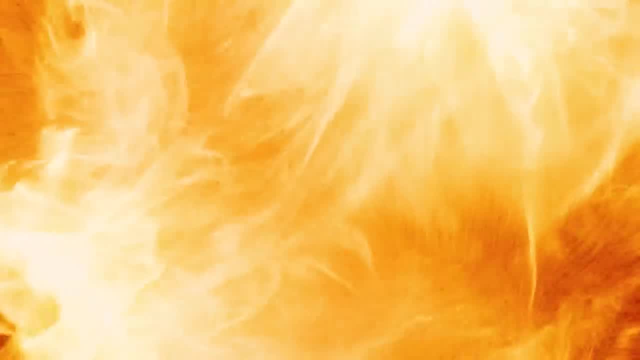 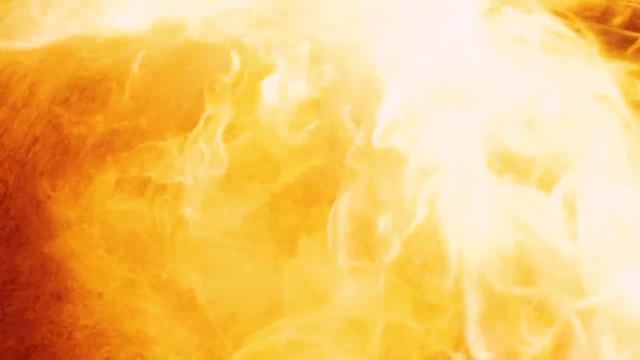 The lingering radiation of the first light in the cosmos. For the first few hundred thousand years of the universe's existence, it was utterly opaque. despite being full of light, It was completely opaque. This concept is hard for us to imagine today, but since a trillionth of a second after the, 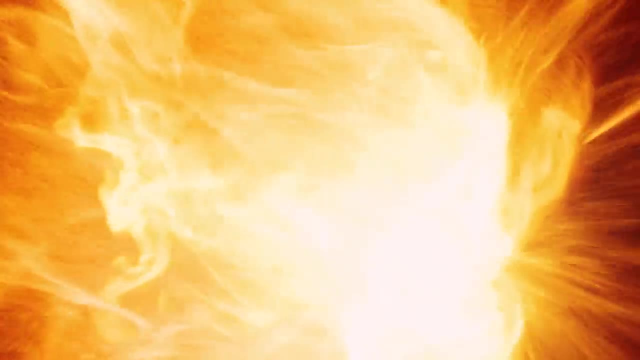 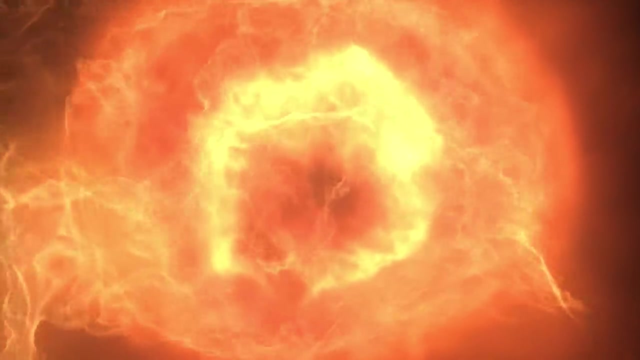 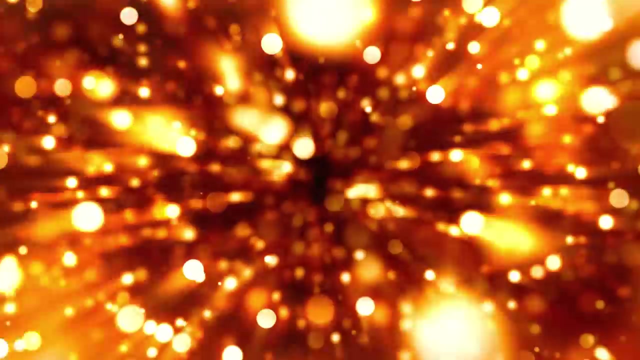 big bang, the photons that carried much of the energy in the universe had become trapped in a maze of their own making, With matter and energy occupying opposite sides of the same coin. the cooling of the newborn cosmos saw pure energy transformed into matter, flooding the universe with subatomic 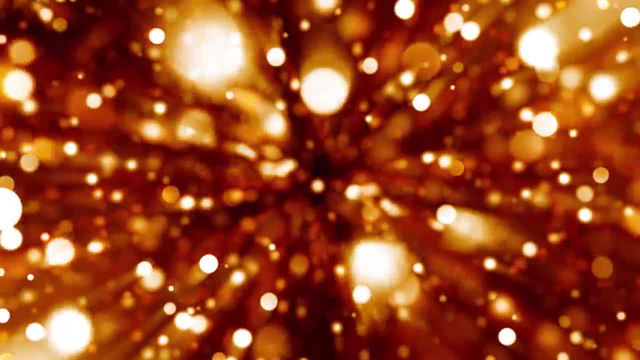 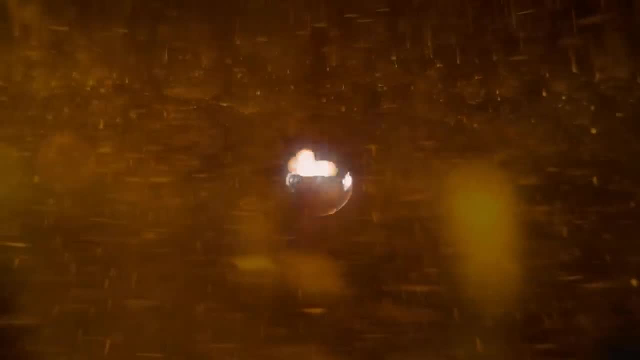 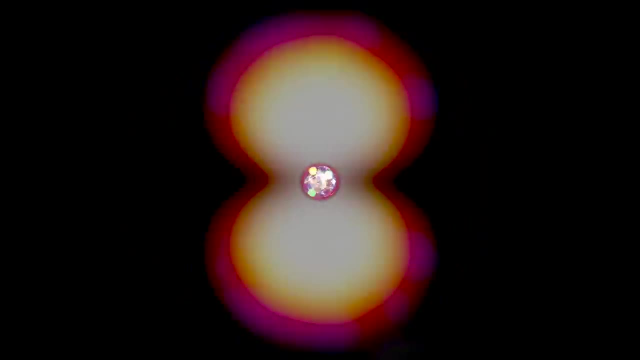 particles, The density and intense vibrational energy of these such that photons simply could not penetrate the swarm. It wouldn't be until the ultimate formation of atoms that anything would change. In the modern universe, it is uncharged atoms, rather than charged ions that are the building. 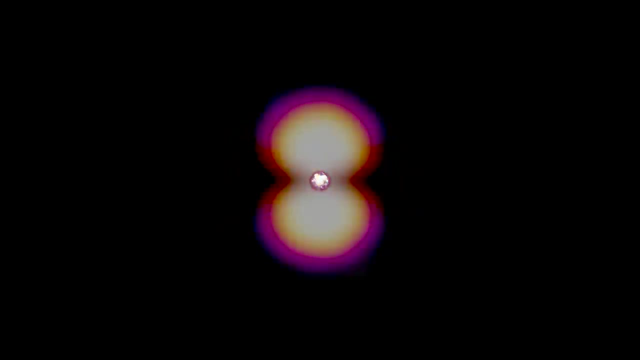 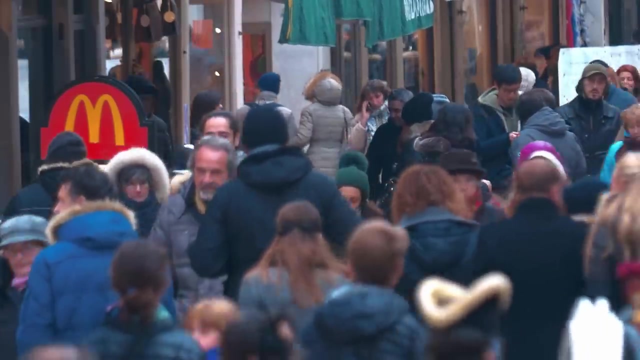 blocks for everything around us. Due to their small size, it takes a staggering number of these atoms to build anything. There are around seven octillion atoms in each human body. That's a seven, followed by twenty-seven zeroes. Scale this up to the number of humans. 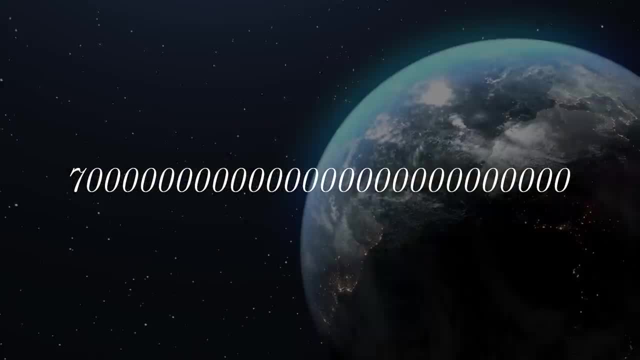 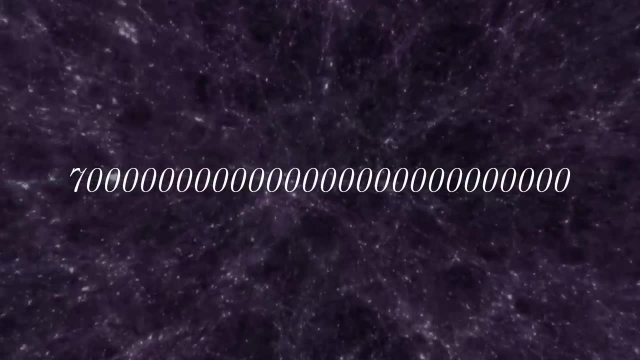 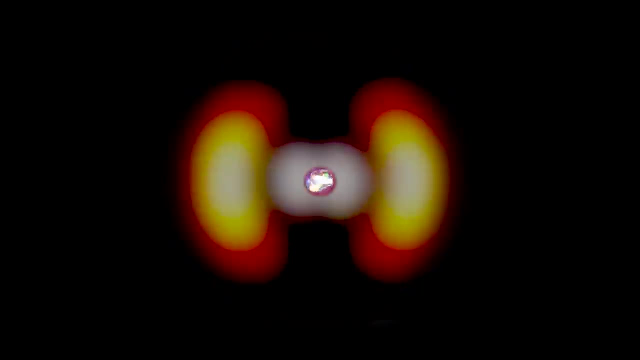 And all of them are zeroes. All other living things on earth factor in the earth itself and multiply by all the planets and stars in the cosmos and the number of atoms in the entire universe is ungraspable. But the real key to making an atom lies in the capture of electrons. 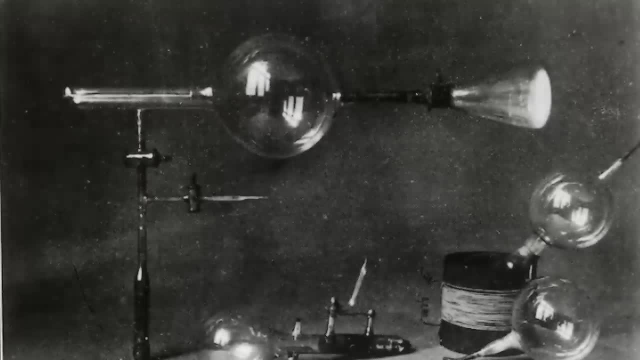 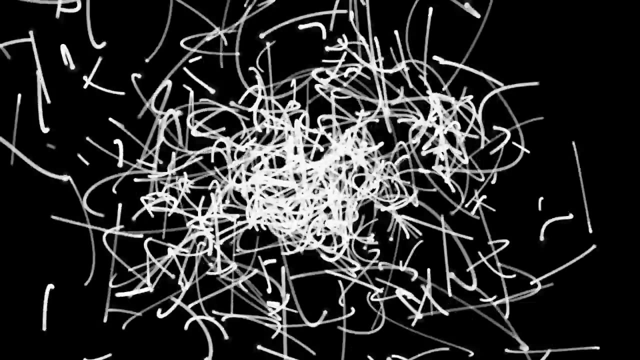 First discovered towards the end of the nineteenth century. these negatively charged leptons are two thousand times lighter than a proton and can be thought of as a singular point with no shape or internal structure. At such minute scales, quantum mechanics can be used to measure the size of an atom and 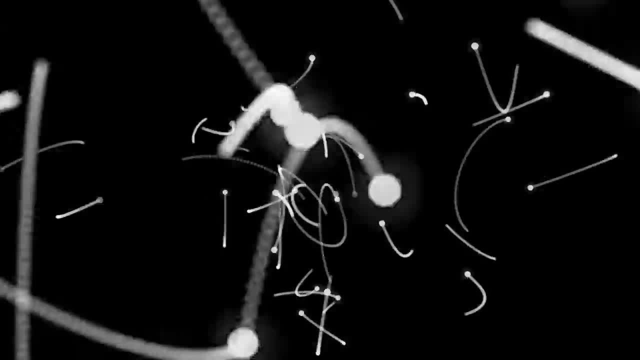 even the size of an atom can be used to measure the size of an atom. In fact, it is impossible to measure the size of an atom in the universe. Quantum physics governs their behaviour and quantum uncertainty dictates that we cannot know their speed and position. 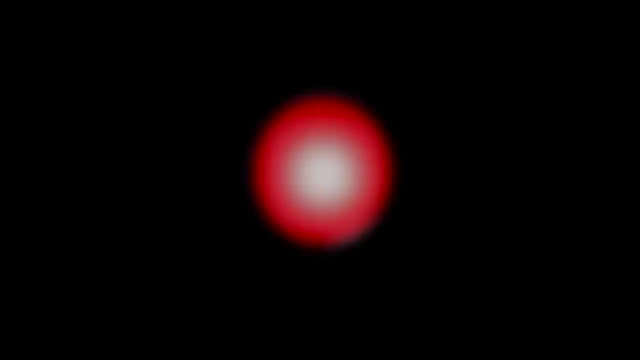 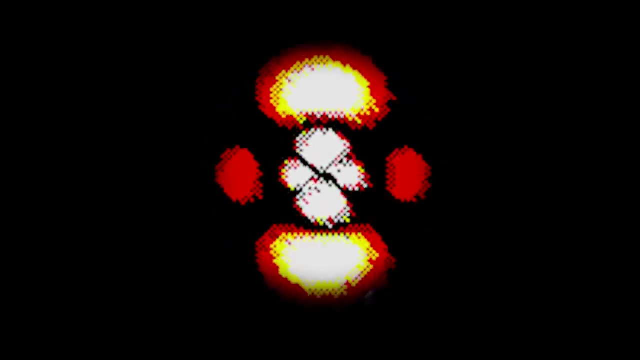 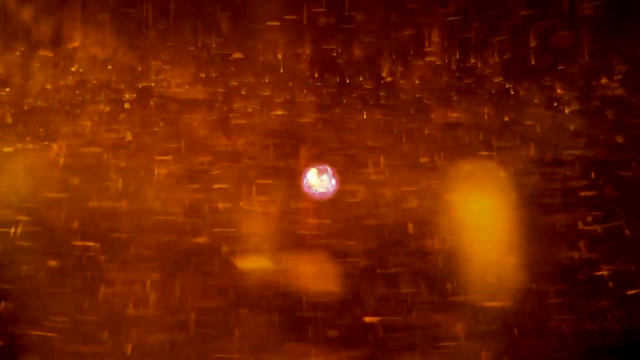 We would never be able to pinpoint a single electron. Instead, they can be thought of as simultaneously occupying every possible spot that they can, as far as the laws of physics allow. Once positively charged atomic nuclei have been created during Big Bang, nucleosynthesis. 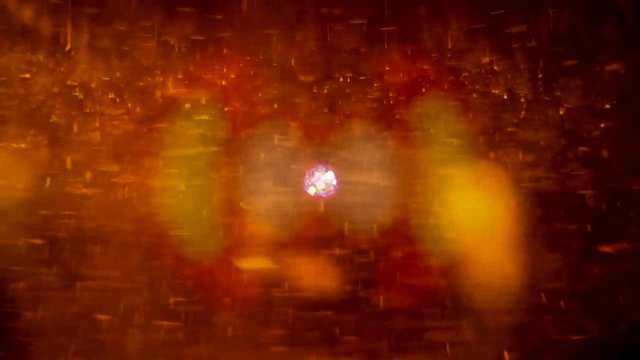 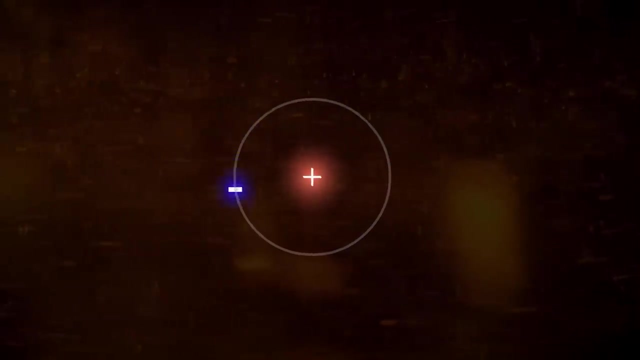 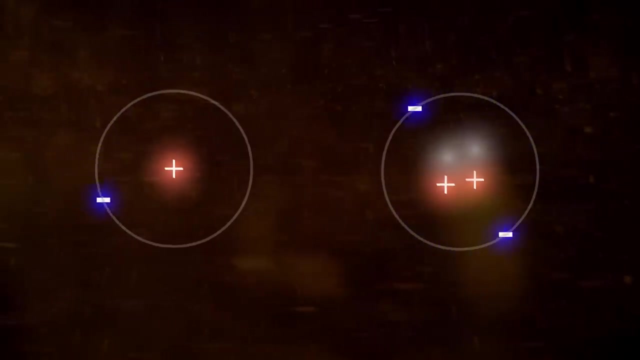 the electromagnetic force helps to ensnare negatively charged electrons to create the neutrally charged atom. Hydrogen nuclei capture a single electron and helium nuclei capture two. But simple as this may sound, it is not a quick process. The electromagnetic force is some one hundred times weaker than the strong force that holds. 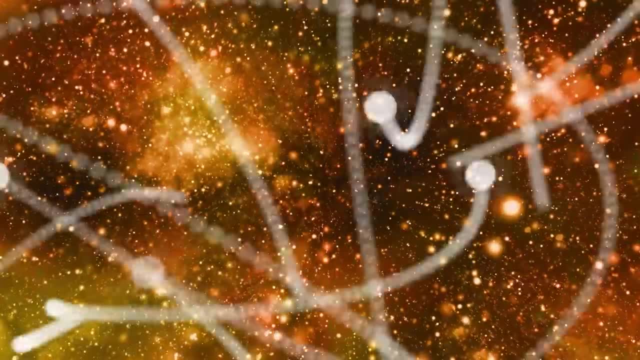 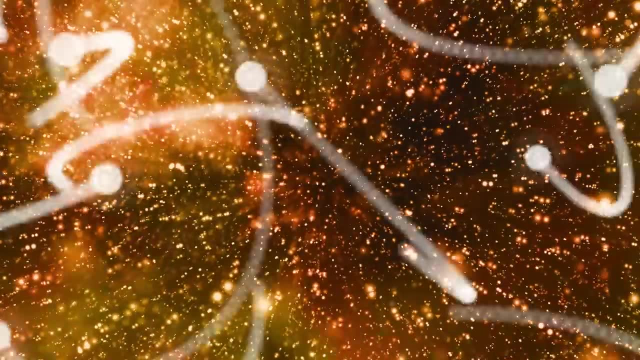 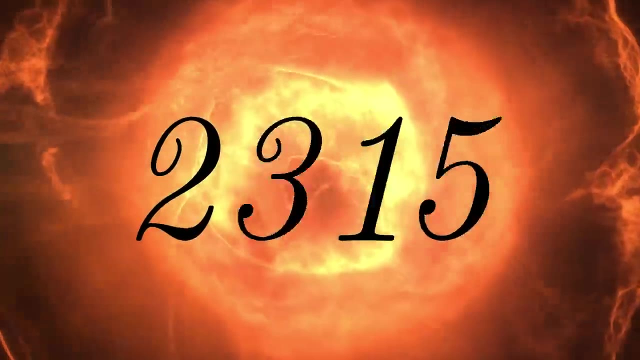 hadrons and nuclei together, and so the ambient conditions of the universe must be that much less energetic if electromagnetism hopes to lasso the supercharged electrons and bring them into the corral. In the end, it takes three hundred and eighty thousand years of cosmic expansion for temperatures. 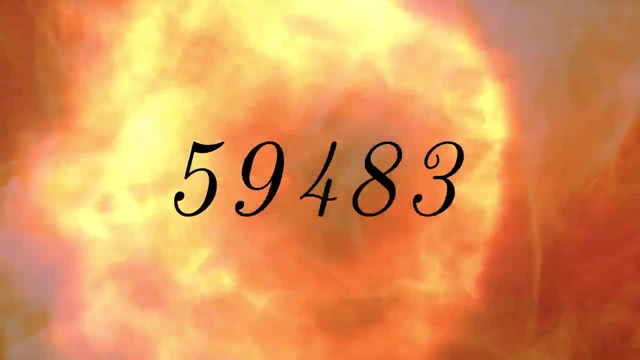 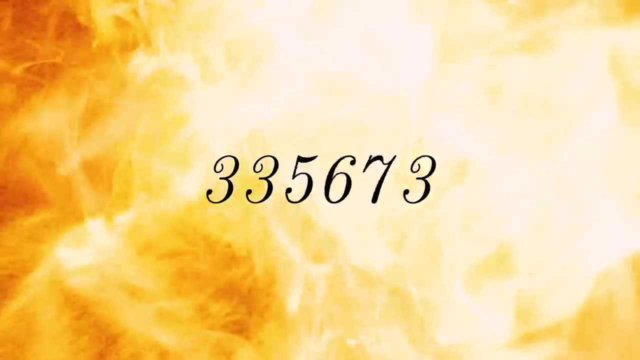 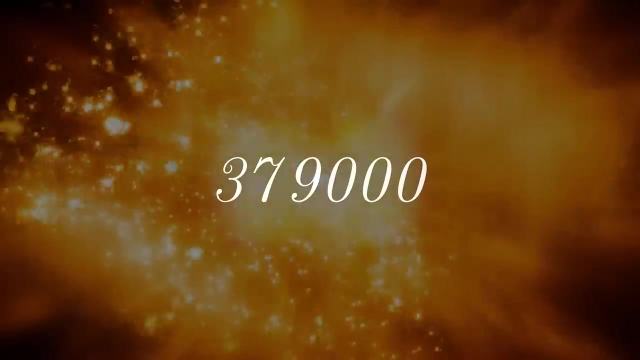 to drop far enough, to around three thousand kelvin- for electrons to finally join the herd and make the first stable atoms. And when they do, the entire universe transforms. Electromagnetic attraction sucks electrons into stable orbits around atomic nuclei, where they once roamed freely through the universe. 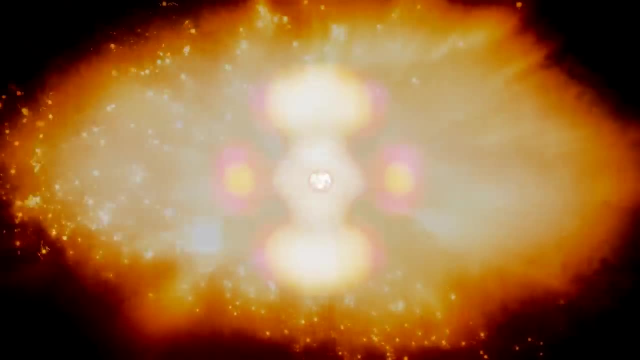 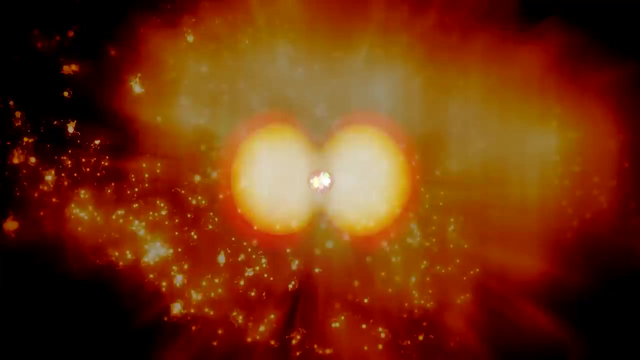 This is the first time in the history of the universe that an atomic nucleus has ever been created. The electrons are now tightly bound to their positively charged counterparts, opening up empty space for the first time since the creation of matter, The photons that have been trapped in a labyrinth for hundreds of thousands of years. suddenly, 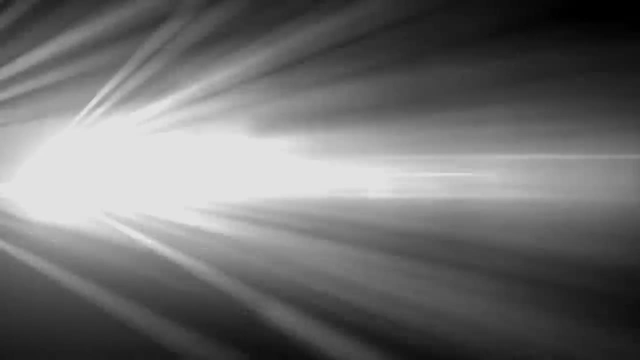 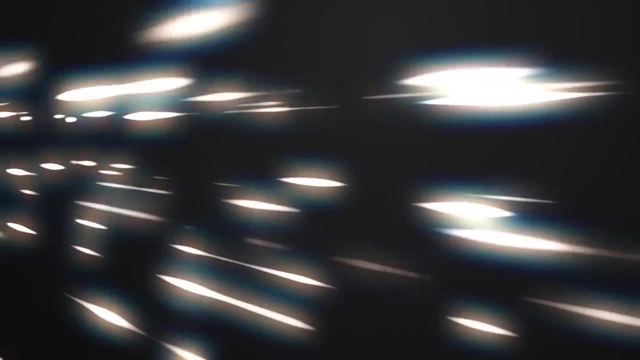 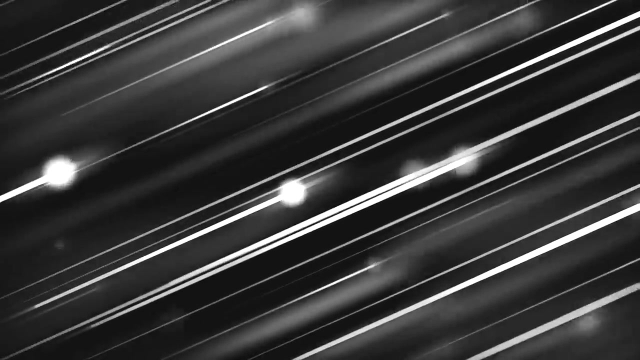 find their paths clear. They can escape travelling in straight lines without instantly striking another particle. They are the first light that truly penetrates the universe. What was one moment opaque now becomes transparent. What was once opaque now becomes transparent. What was one moment plasma now becomes gas. 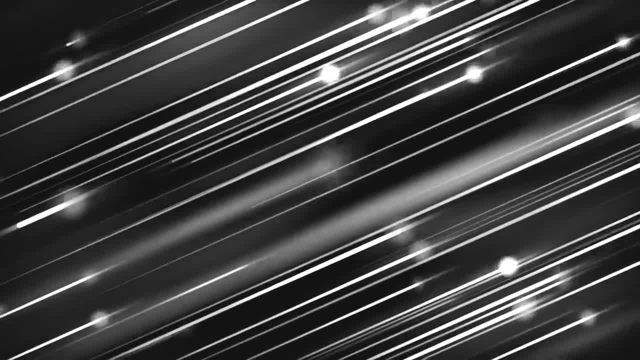 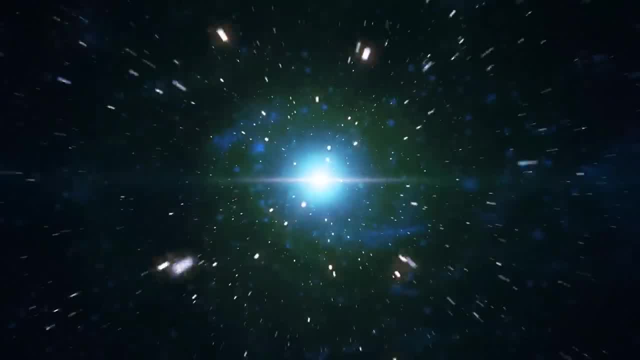 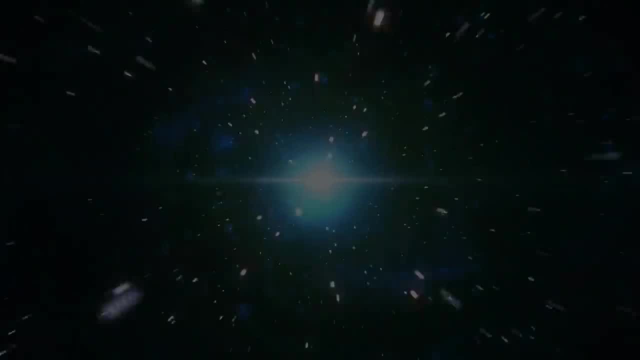 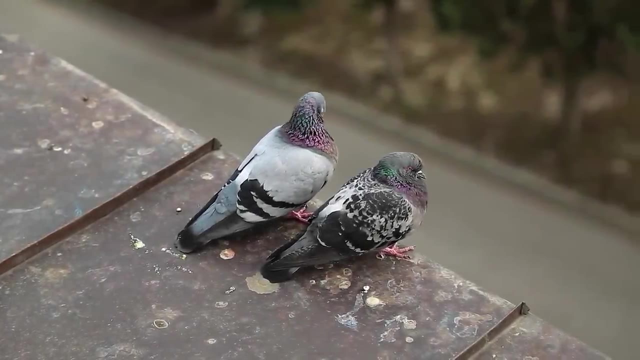 And what was one moment shattered now becomes whole. For the first time in the entire history of the universe, we finally have a chance of seeing what was going on. INTRO: VERY FEW DISCOVERIES IN SCIENCE ARE MADE BY ACCIDENT. 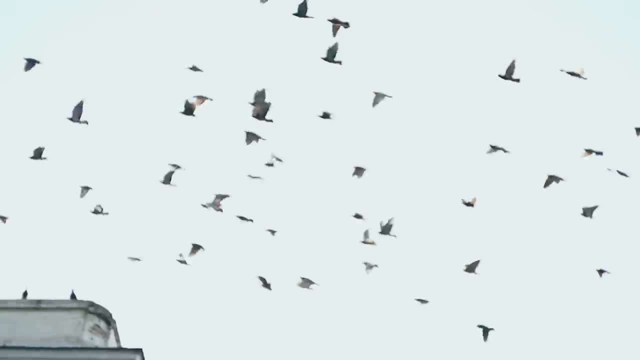 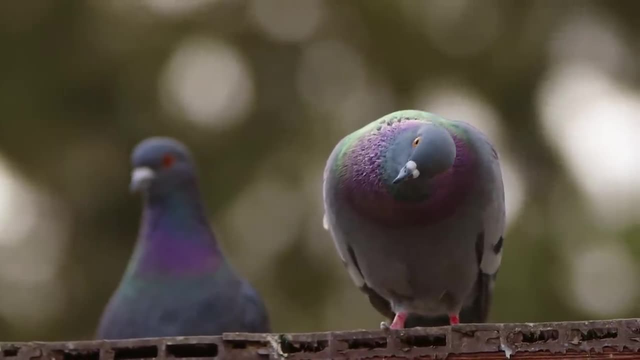 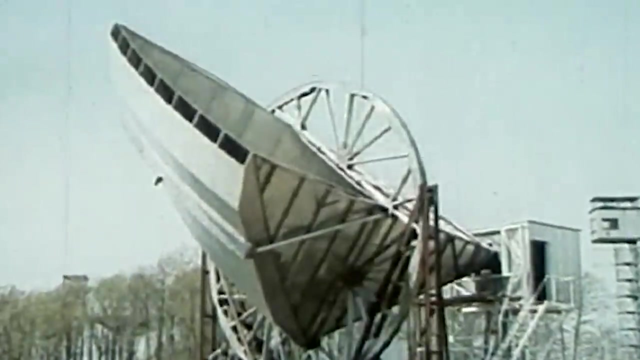 NOT IN THE PAST, Much less the kinds of discoveries that lead to Nobel Prizes. Instead, scientific progress is typically hard won through years of commitment, incremental research and investment. But in 1978, the Nobel Committee flew in the face of convention and awarded that year's 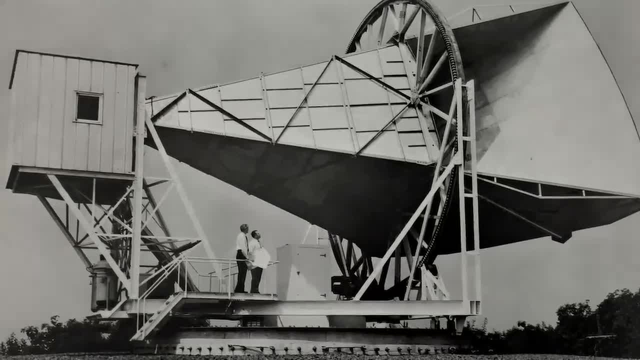 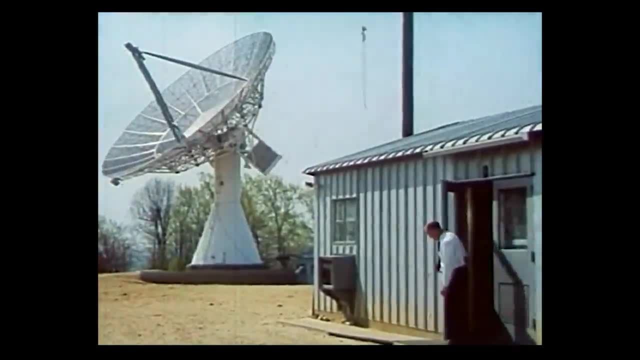 prize in physics to two men whose groundbreaking discovery was something of a fluke. The Nobel Prize in Physics was a success. The Nobel Prize in Physics was a success. It was in the early 1960s. It was in the 60s, in the small town of Holmdel, New Jersey, that the stage was set for the. 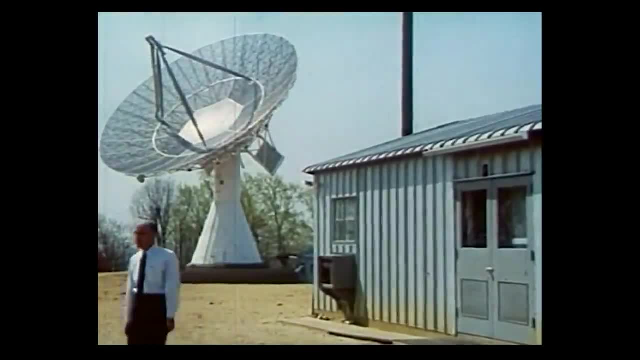 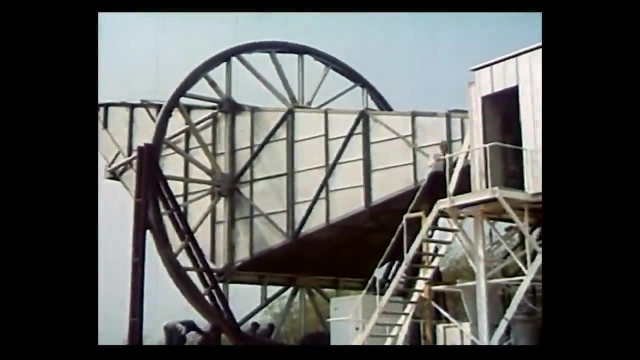 most fortuitous of discoveries, for it was there that the company Bell Labs had constructed a 20-foot horn-shaped antenna. Just a few years after the Great Horn was built, a new satellite system usurped the original, rendering the instrument obsolete. 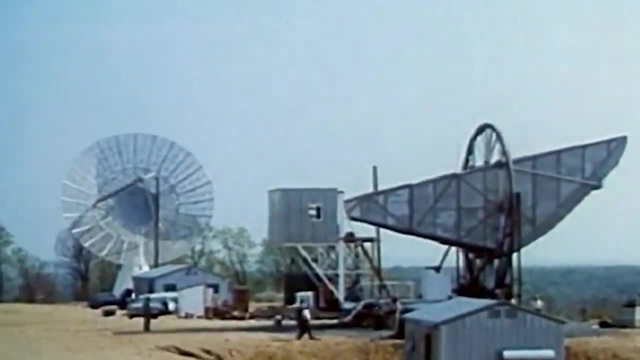 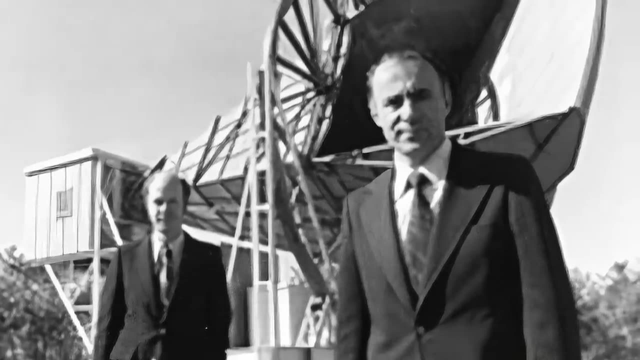 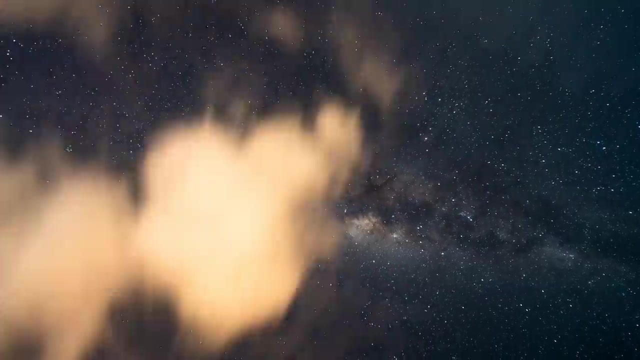 But Bell Labs didn't let their gigantic hearing aid go to waste. instead, they opened it up to researchers Arno Penzias and Robert Wilson, who planned to tune into and analyse the radio signals coming from the space between galaxies. However, when they began their observations, the two astronomers struggled to make out. 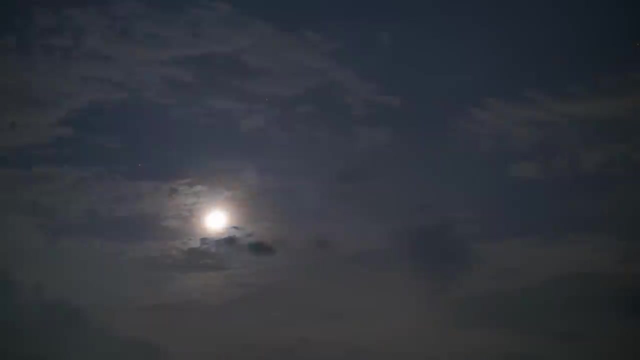 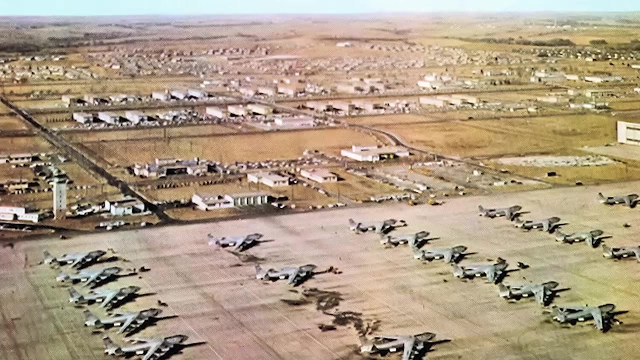 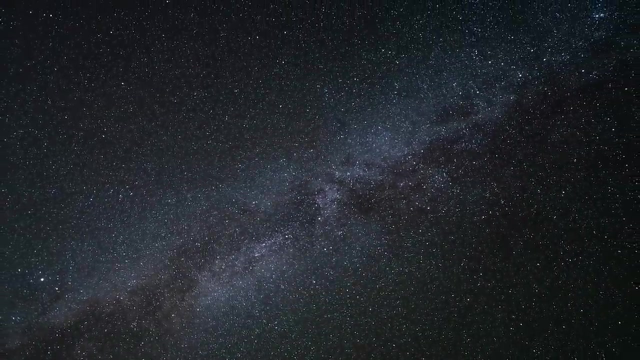 the signal above a low but persistent radio hiss. They checked it wasn't coming from nearby New York City or from local military installations. They confirmed it wasn't coming from any particular part of the Milky Way or outer space, but rather it seemed to be coming from the entire sky. 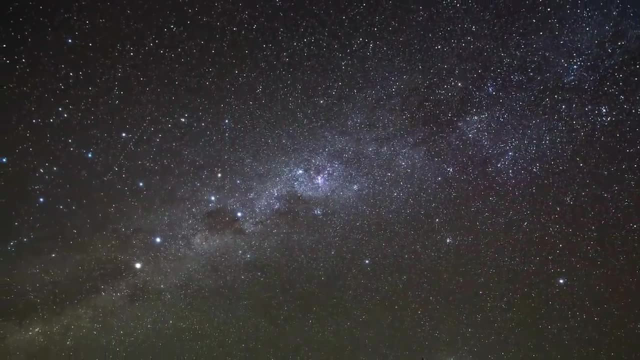 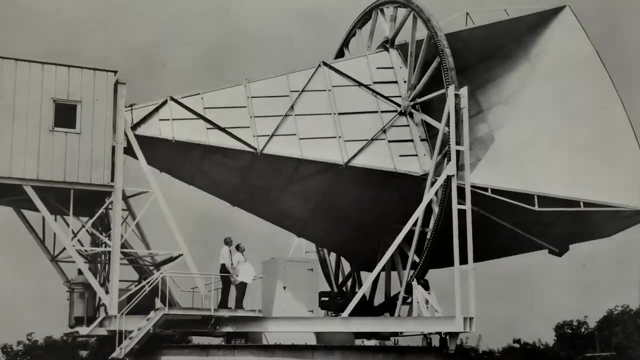 And so for this noise to appear so consistent and omnidirectional, the researchers concluded it must be due to some error within the instrument, And indeed, when they inspected the antenna, they found it to be home to a number of roosting. 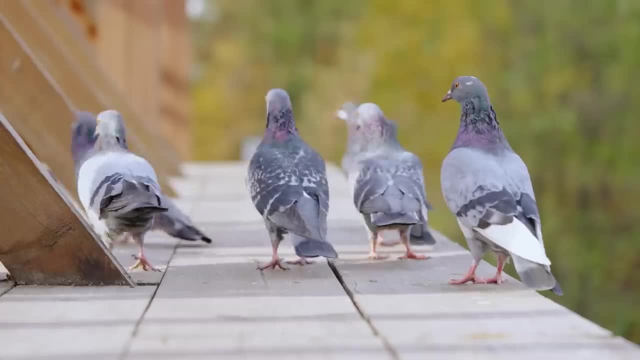 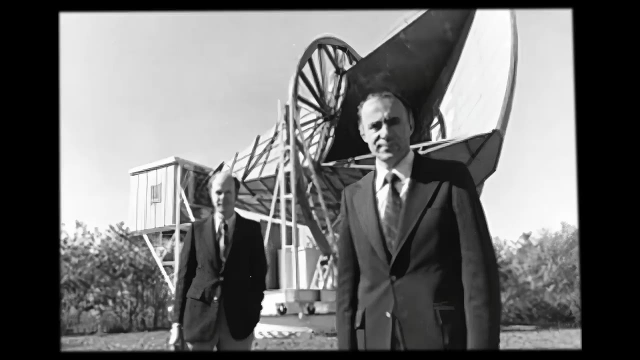 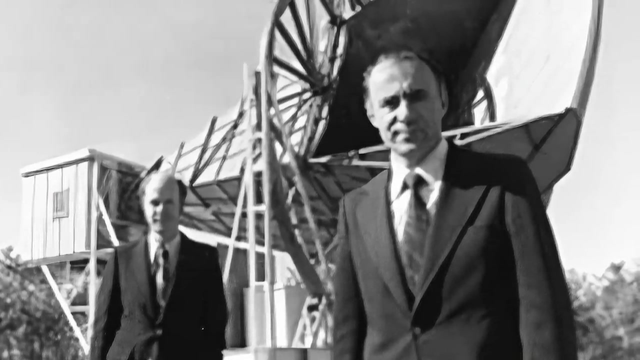 pigeons. Perhaps their droppings, what they described as a white dielectric material, was giving off heat that was creating the noise. After several failed attempts to humanely rehome the birds, the researchers resorted to more drastic measures and eventually cleared the horn of both pigeon and droppings. 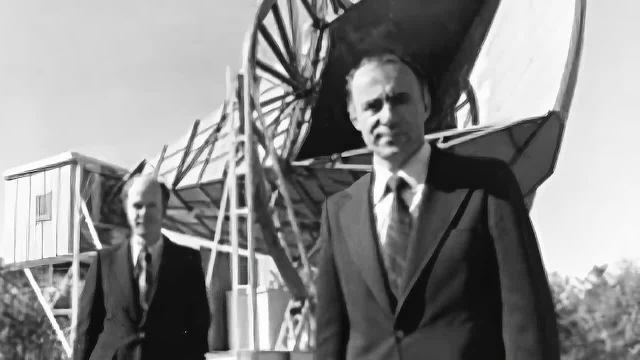 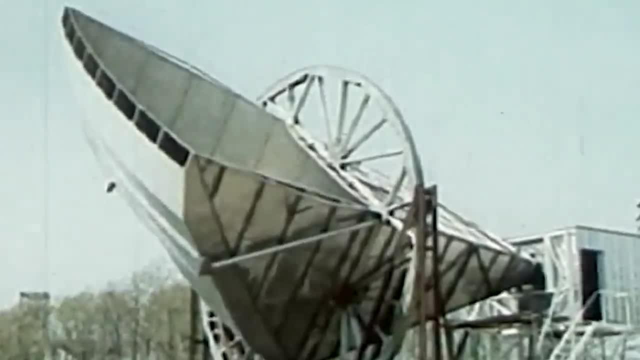 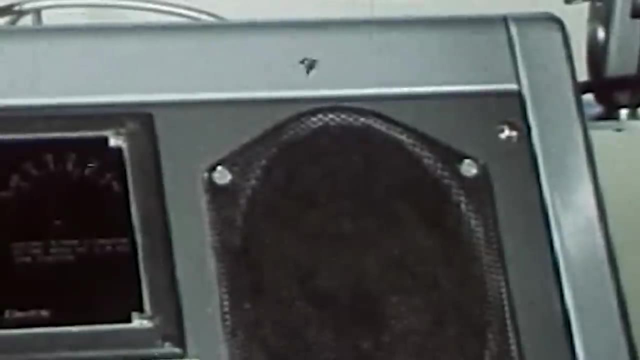 And yet the hissing still remained. Penzias and Wilson had eliminated all possible sources of error in their instrument and so, as a last resort, began to entertain the notion that this radio noise could in fact be coming from the entire sky. 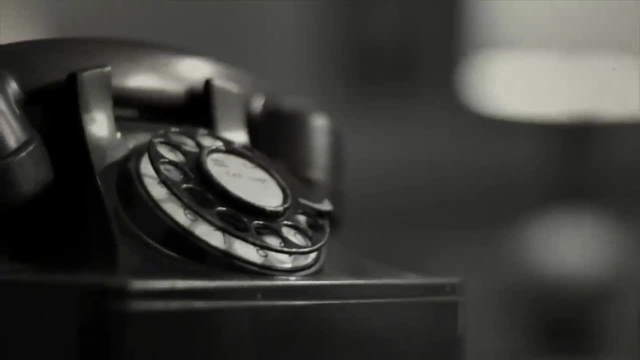 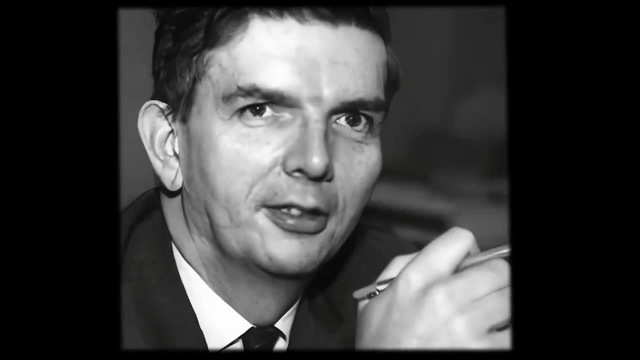 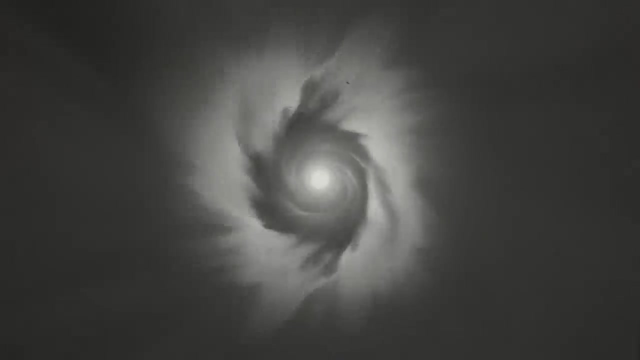 They reached out to a fellow astronomer at Princeton University, Robert Dickey, for advice, And it was Dickey who solved the mystery in the biggest way possible. He had been developing a theory of atom formation in the early universe, believing the Big Bang. 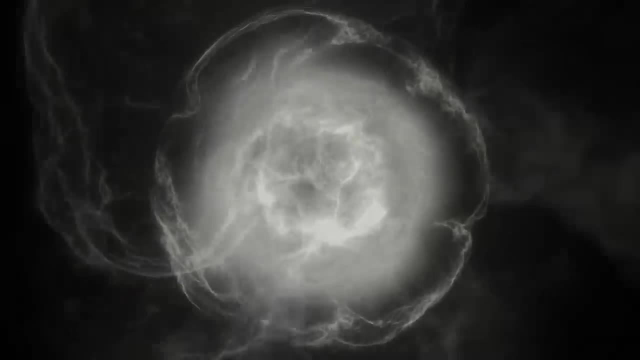 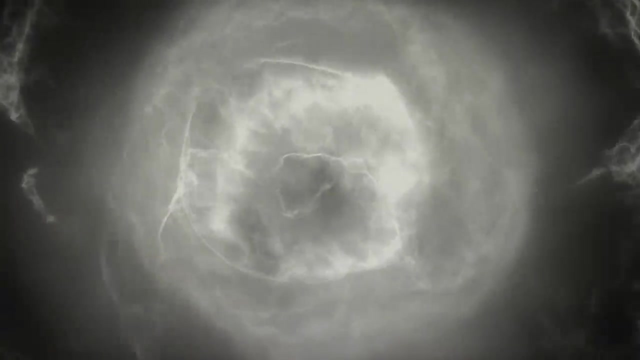 to be cyclical, all the atoms of a previous universe being ripped apart in a scorching fireball of compression and reassembled when the universe expanded and cooled again. This so-called recombination was an important part of the theory. 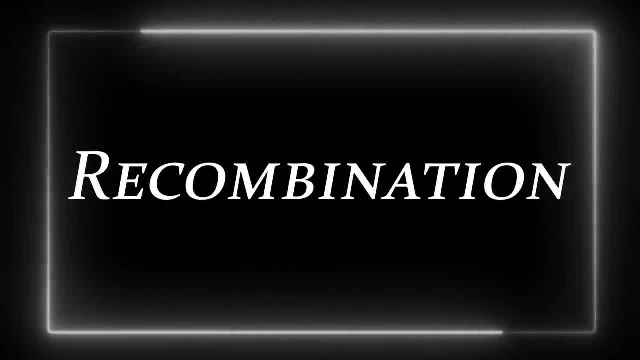 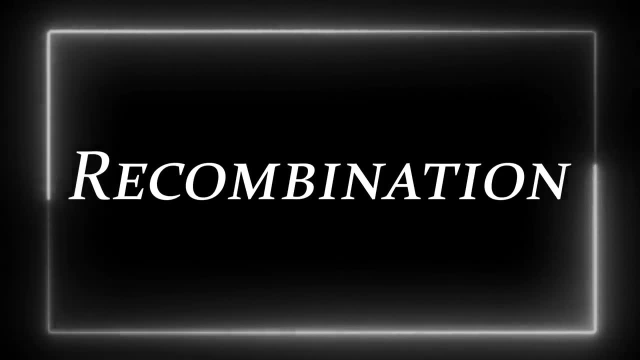 It was an important part of the theory. Dickey's theory of atom formation would turn the cosmos transparent and allow light to be released for the very first time in this universe's chronology. His theories predicted that such light originally in the visible part of the spectrum as a yellow-orange. 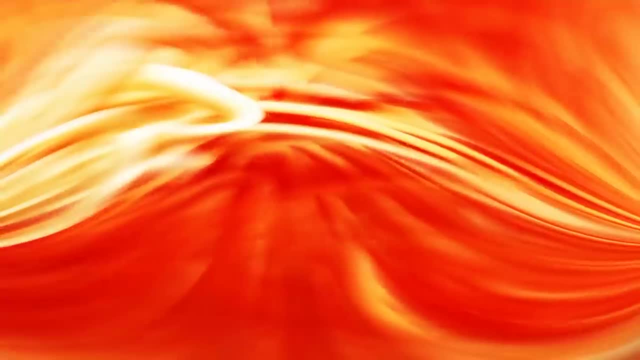 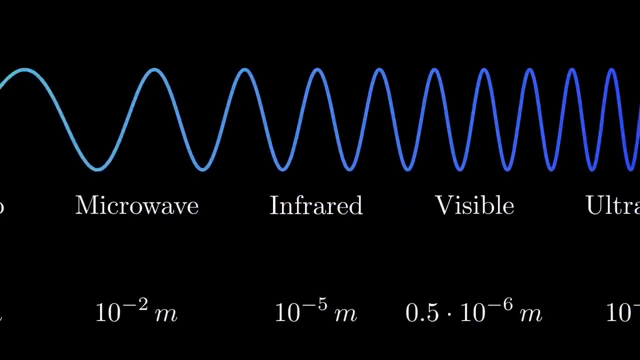 glow could still be detected at great distances within the universe. Subsequent expansion of the cosmos would stretch that early spacetime until the glow became redshifted beyond the perception of our eyes and into microwave wavelengths. Dickey's theory of atom formation. 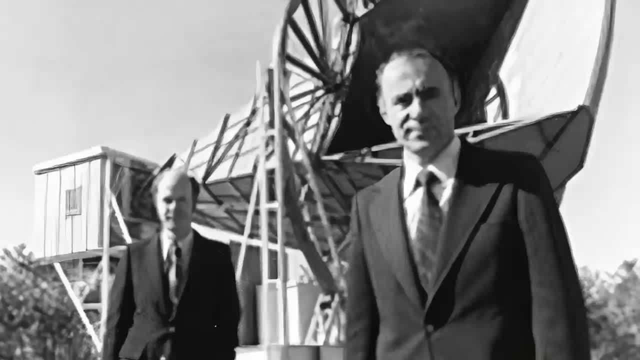 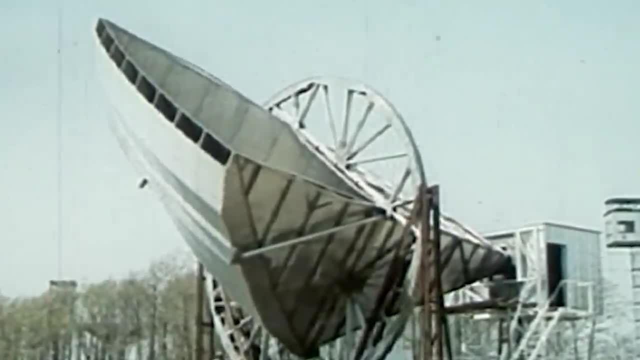 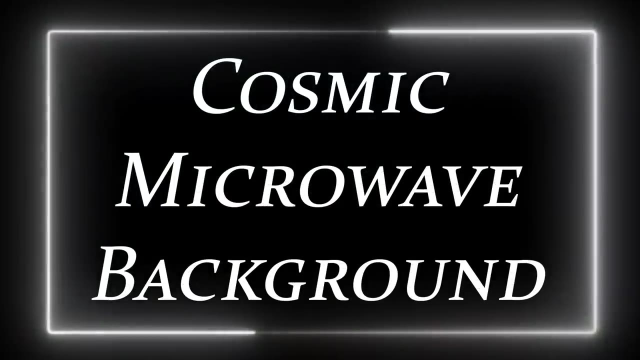 Dickey's theory of atom formation. Dickey had planned to search for it himself, but Penzias and Wilson had unwittingly beaten him to it, And so, a decade later, it was the two Bell Lab researchers who were awarded the Nobel Prize for the discovery of the so-called Cosmic Microwave Background. 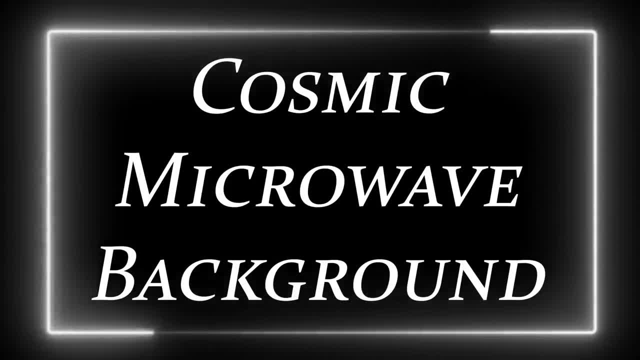 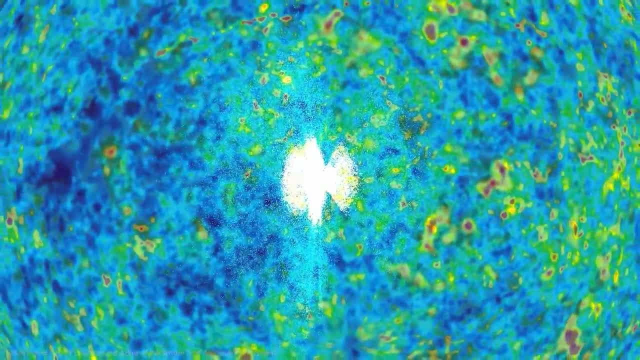 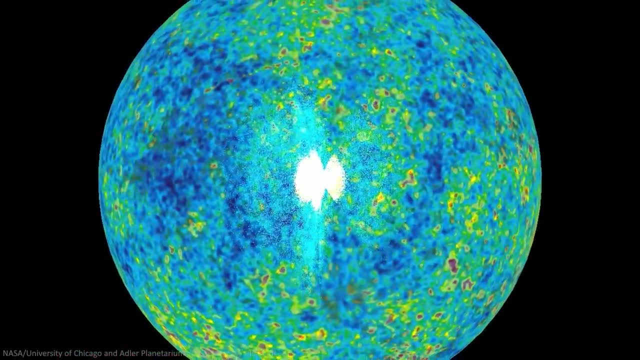 And not Robert Dickey. Regardless of who was credited for finding or figuring out the Cosmic Microwave Background, and despite Dickey's cyclical fireball model being later ruled out, its detection represented a major turning point for our understanding of the Big Bang. 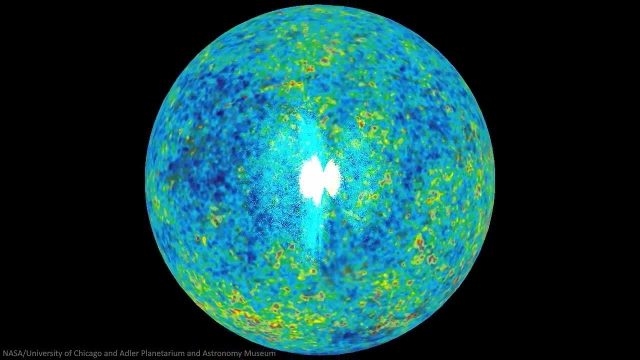 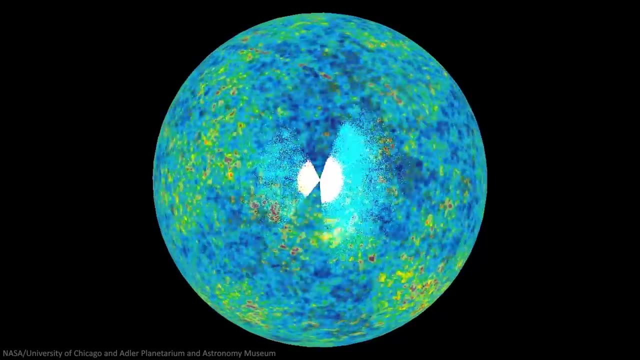 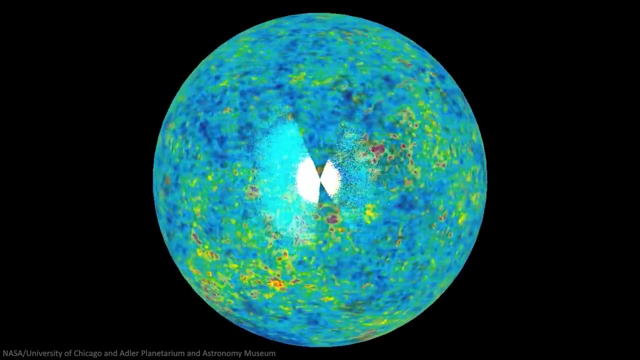 The discovery of this redshifted fireball glow, now stretched out to be just 2.7 degrees above absolute zero, is conclusive evidence that the universe did in fact start-out in a hot, dense state, Even though it dates to a moment some 380,000 years before the universe was even created. 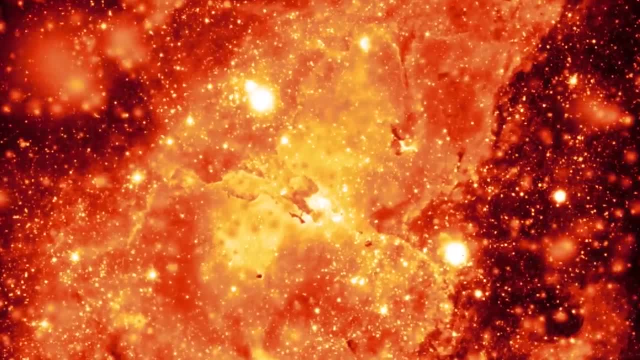 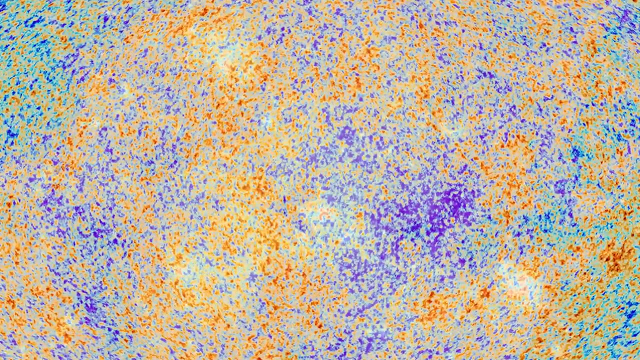 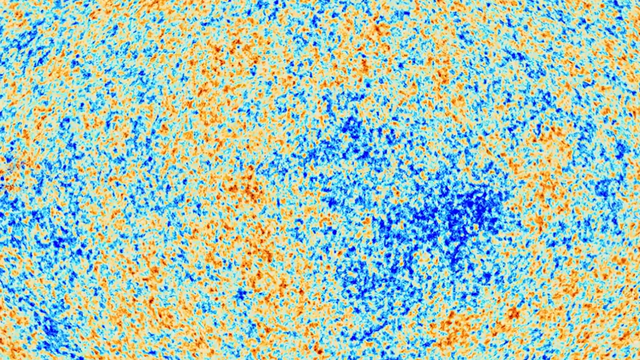 the universe remains a dark, dense state. The universe is a state that has been there for thousands of years, Years after that moment of cosmological creation. it is vindication for our theories of how things unfolded in the intervening period, The earliest observational evidence we have of a hot, energetic and compact early universe. 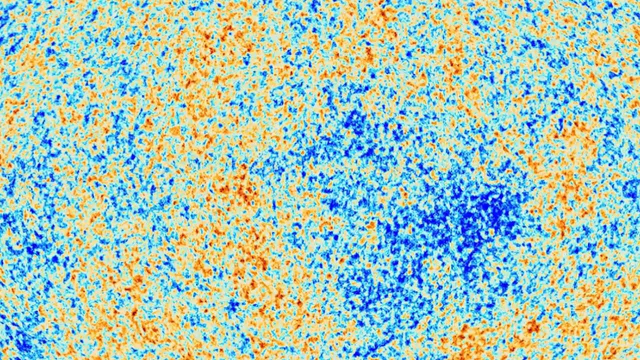 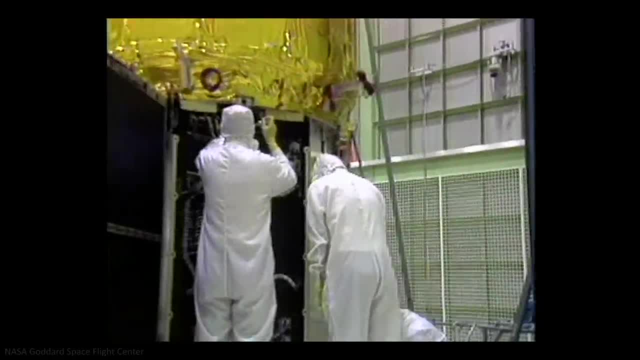 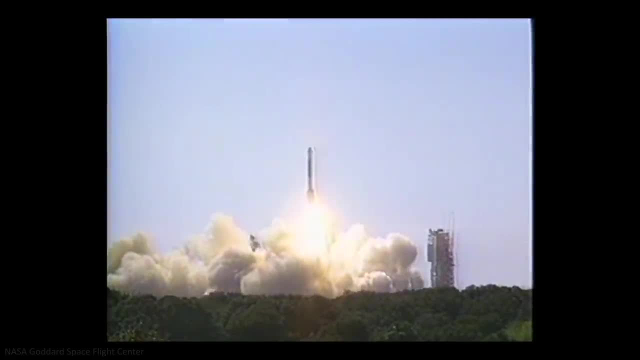 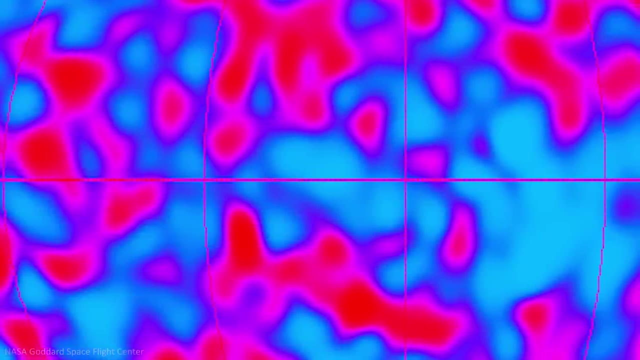 even containing within it clues as to how the universe will unfold, Because, while Penzias and Wilson found the microwave hum to be remarkably consistent across the night sky, later instruments designed to study the CMB discovered very slight variations – places where it was slightly hotter or cooler by a few hundred thousandths of a degree. 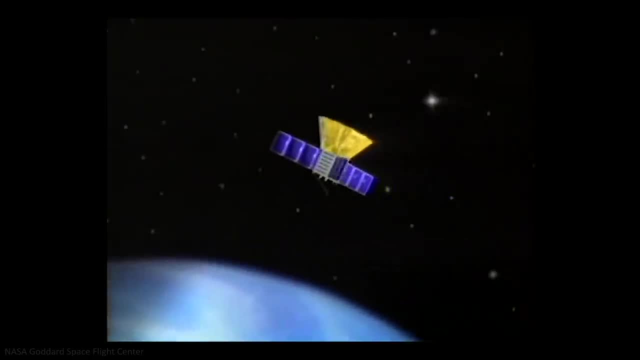 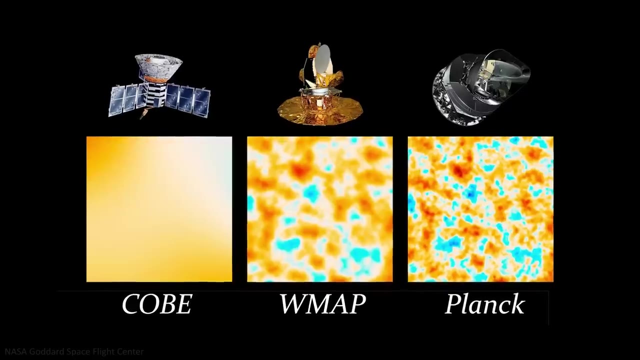 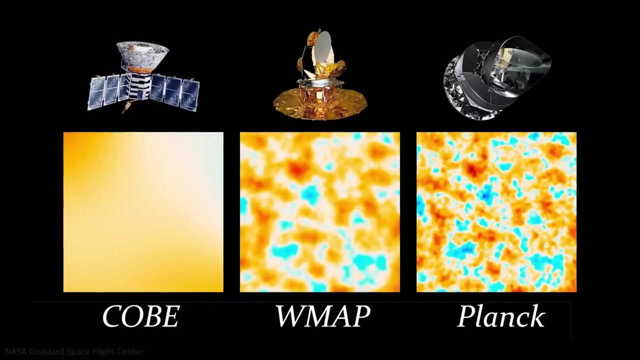 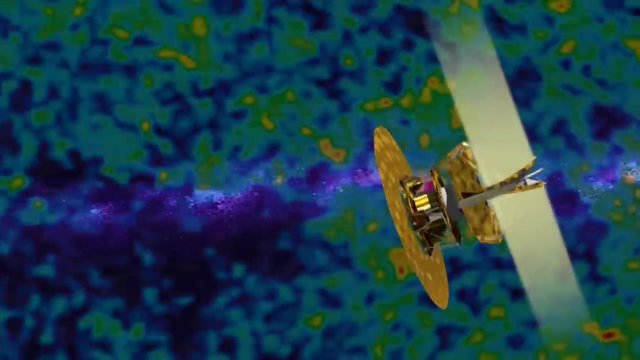 Mapping. the CMB became a priority for projects like the Cosmic Background Explorer, the Wilkinson Microwave Anisotropy Probe and the Planck Telescope, giving rise to incredibly detailed images of energy and density variations in the 380,000 year old universe. And it was those density variations that provided the seeds for large scale structure today. 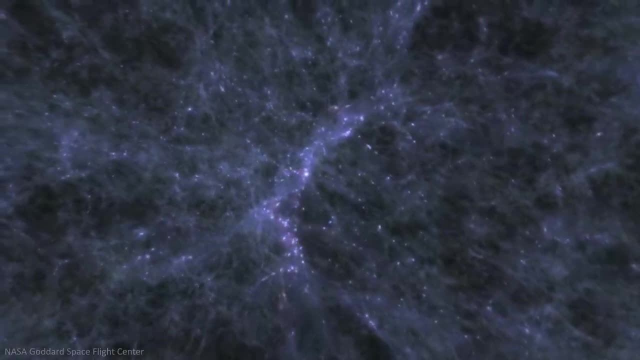 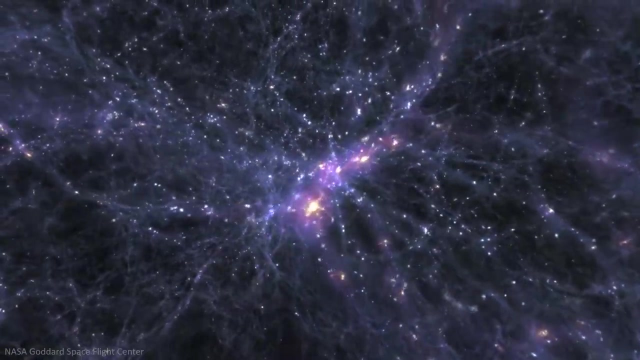 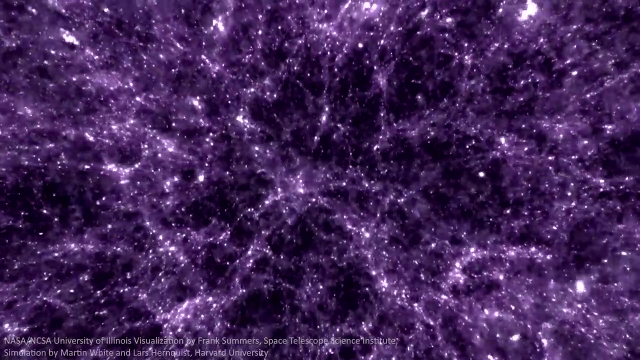 since they contained more matter, which then attracted more matter, becoming denser and pulling in even more, And within a hundred million years, these overdensities had grown massive enough to trigger the formation of the first stars and galaxies. These variations seemed to be largely random. 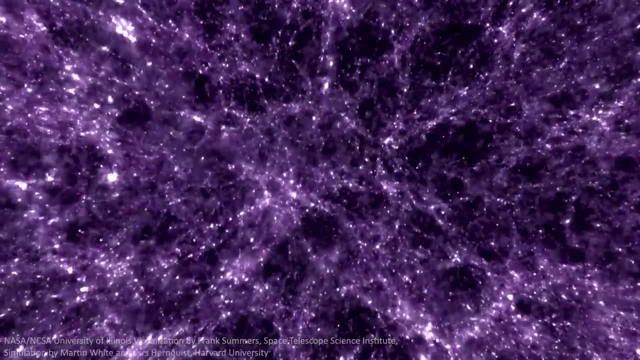 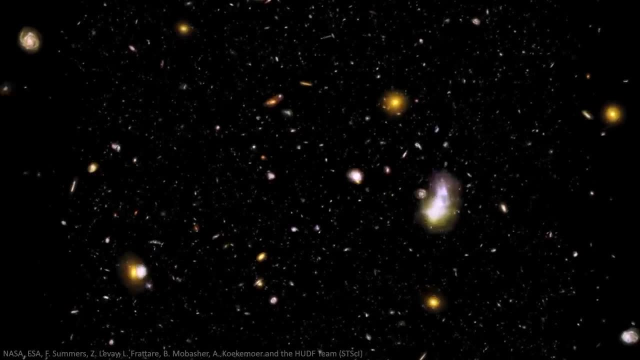 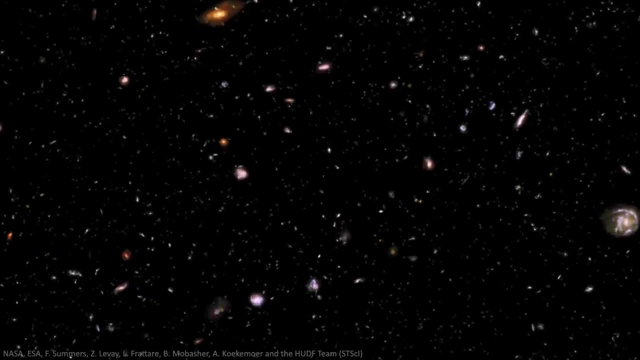 As would be expected, the result of subatomic quantum fluctuations inflated to massive scale through inflation in the first fraction of a second after the big bang. But closer analysis also reveals another curious pattern hidden within the CMB, and one that is also mirrored in the large scale structure of the universe today. 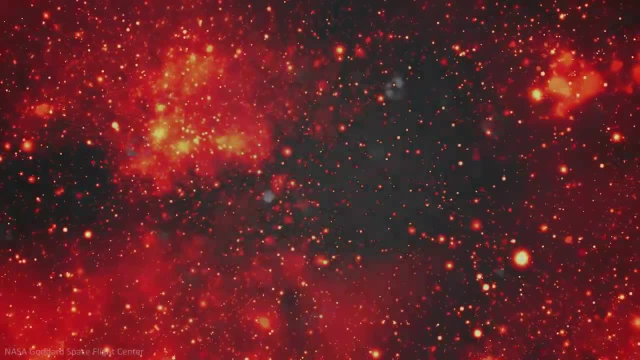 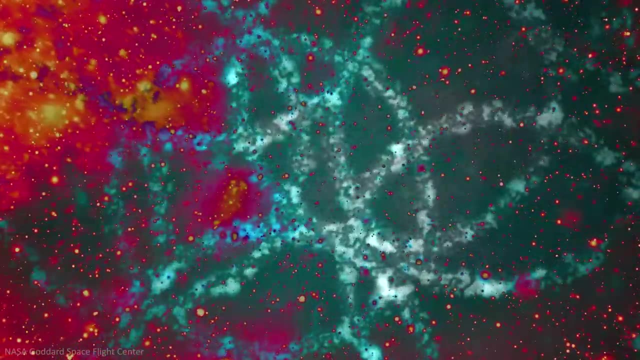 Prior to the formation of atoms, when the universe was still filled with opaque plasma, it was dense enough for sound waves to pass through it, just as sound travels through the air today. These waves had their origin in conflicting forces of attraction and repulsion within. 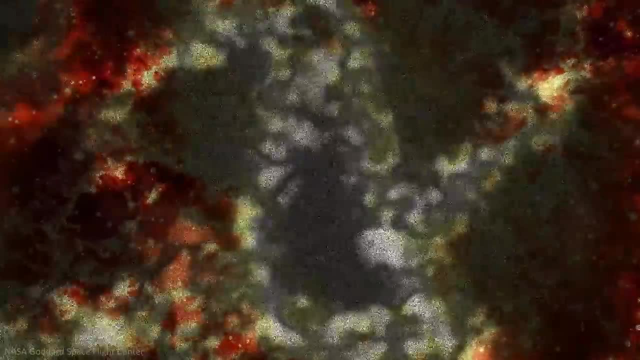 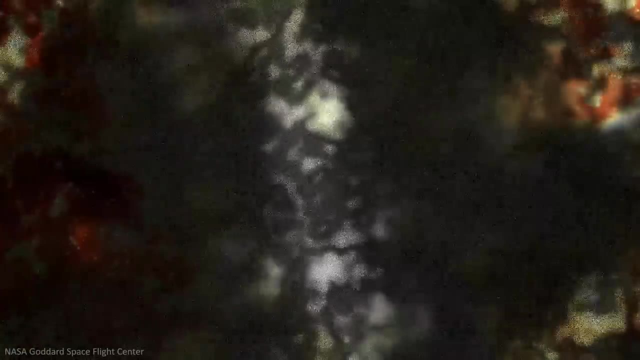 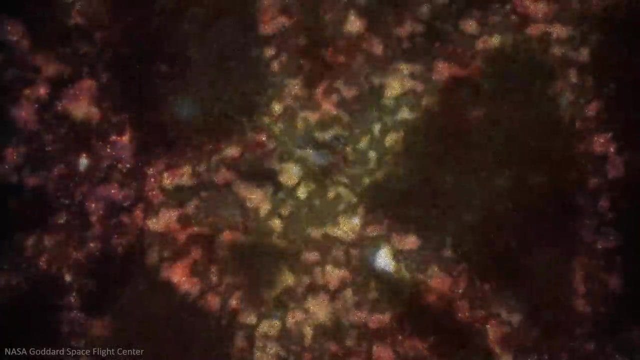 the roiling energetic soup as gravity pulled matter in towards the centre of denser patches. but photons trapped within that collapsing maze rebelled and exerted an outward pressure upon being packed too tightly, And so these photons pushed back out, taking some of the matter with them, spreading out. 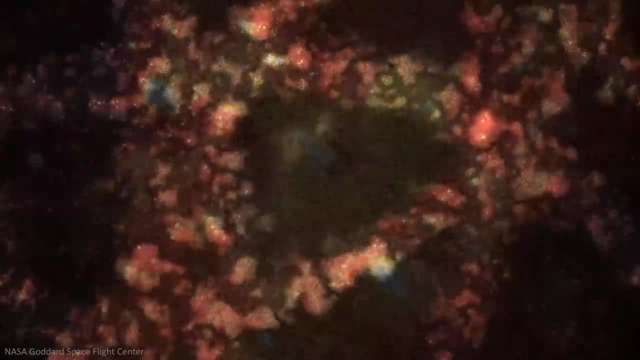 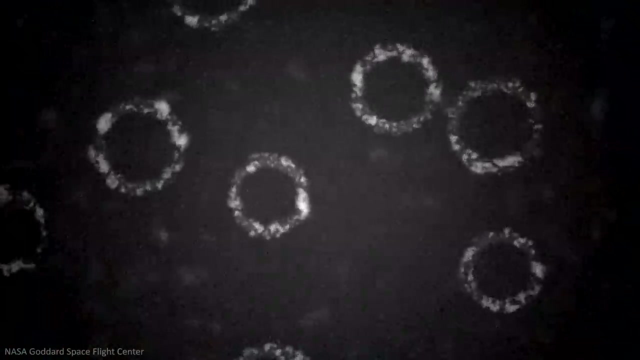 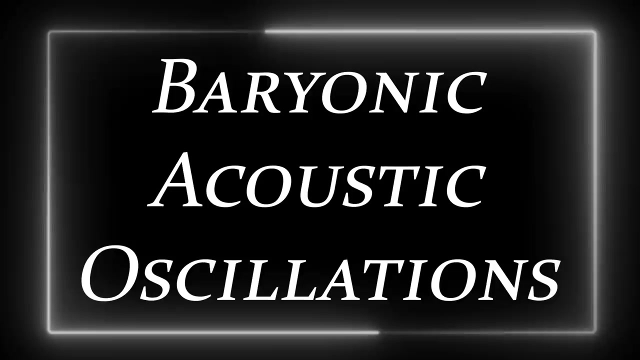 in three dimensions, Creating a complex pattern of concentric ripples, as if from so many raindrops in a pond. In a sense, these compressional waves are sound waves and are therefore known to cosmologists as baryonic acoustic oscillations. 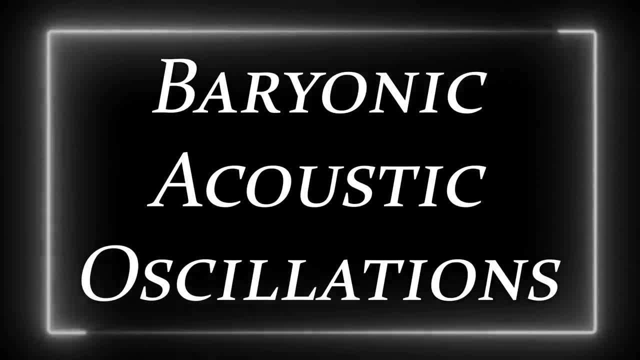 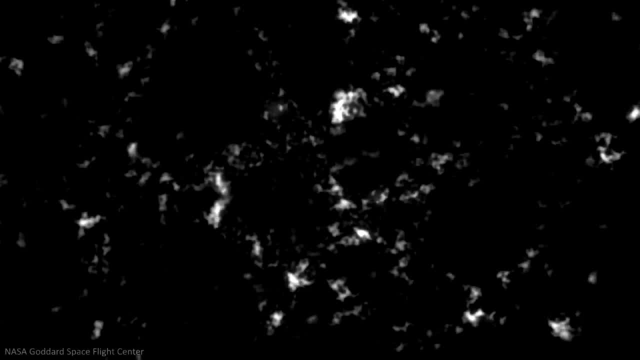 However, this phenomenon did not survive past atomic recombination. Once the universe reached its critical temperature of 3000 Kelvin, allowing electrons to be captured and atoms to form, The expanding ripples were suddenly stopped in place. They were frozen in their tracks as the photons that were carrying the matter outwards could. 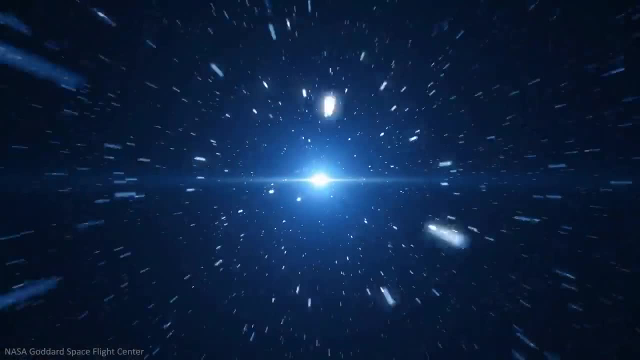 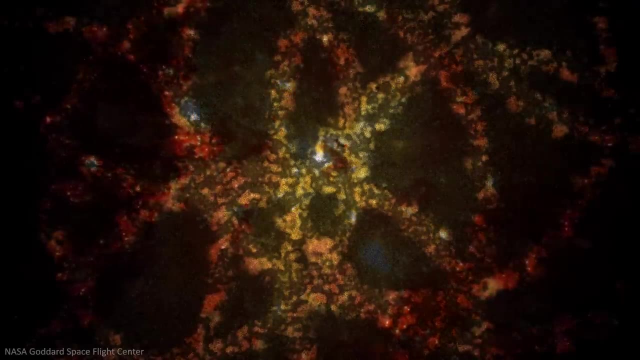 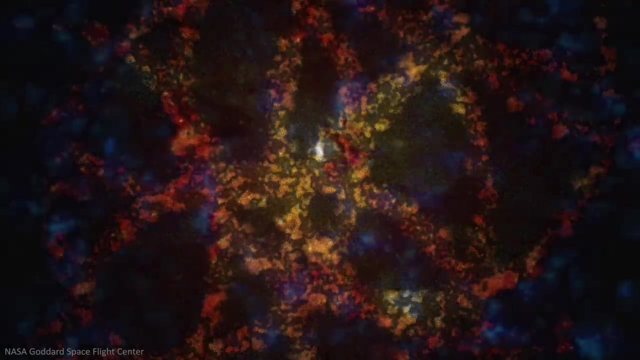 now escape unhindered. The baryonic acoustic oscillations were all frozen in place. They could go no further and the bunched matter at their spherical periphery was left stranded, just as the photons had left it. Now, some 13.5 billion years later, the universe has expanded, but the pattern left behind. 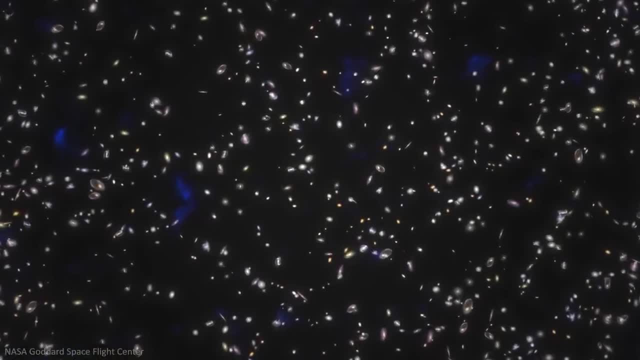 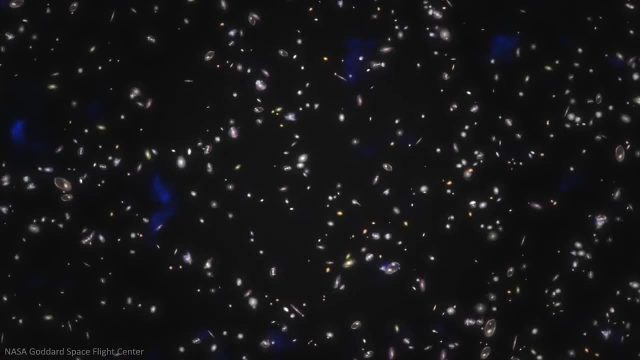 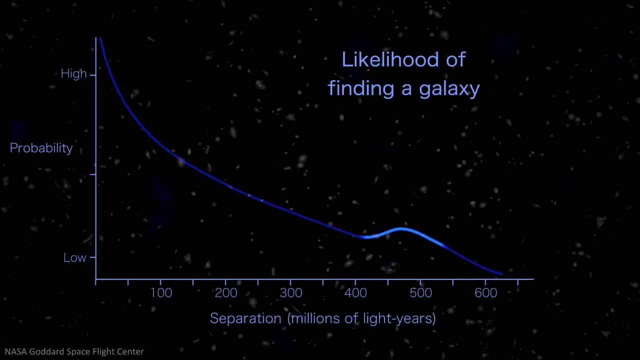 by these frozen ripples can still be discerned In the overall structure of galactic clusters and superclusters. cosmologists find the baryonic acoustic oscillations in the modern universe are now roughly 150 megaparsecs, or nearly 500 million light years across. 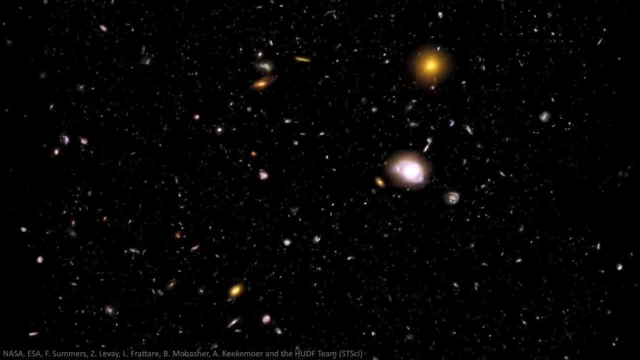 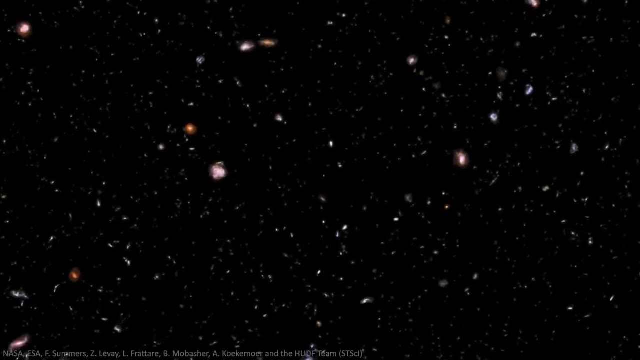 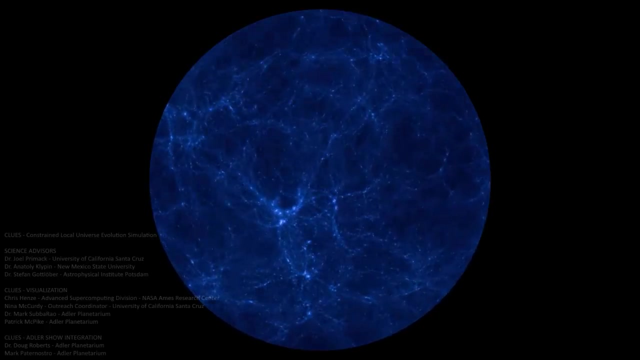 And measurements of their dimensions at greater distances and times within the observable cosmos provide astronomers with a so-called standard ruler with which they can measure the expansion of space. 3. Cosmology: In a universe that is finally rendered visible to our instruments, we can model how things. 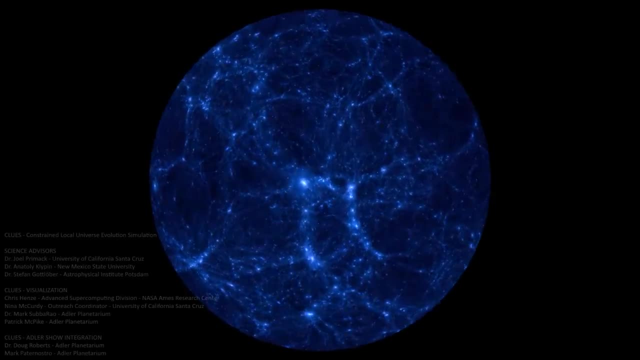 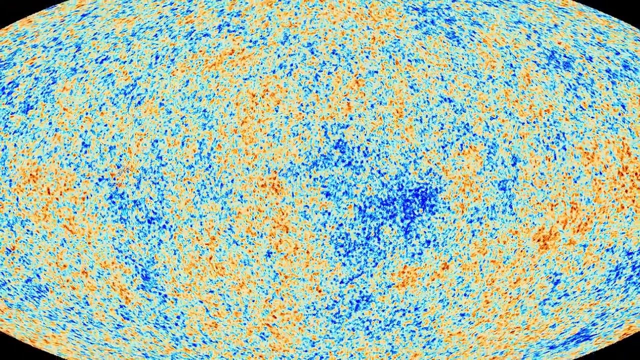 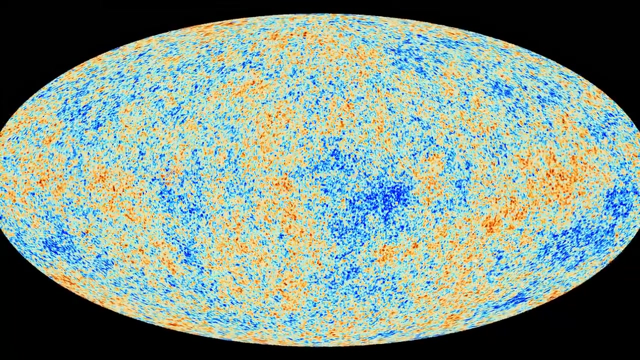 have unfolded and predict how things will unfold in the future. The imprint of the universe's first light may have already stretched and dimmed to a shadow of its former self, but it will be trillions of years yet before it fades completely from our view, giving cosmologists of the future plenty of time yet to decipher its 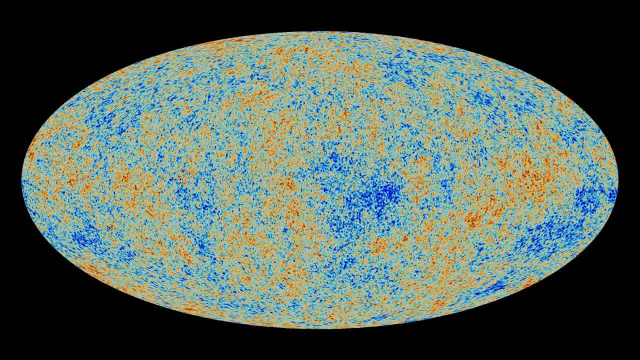 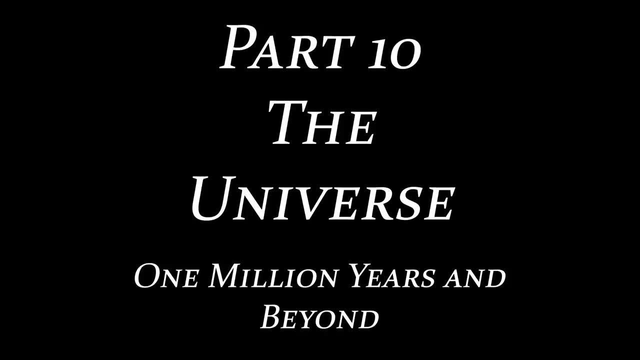 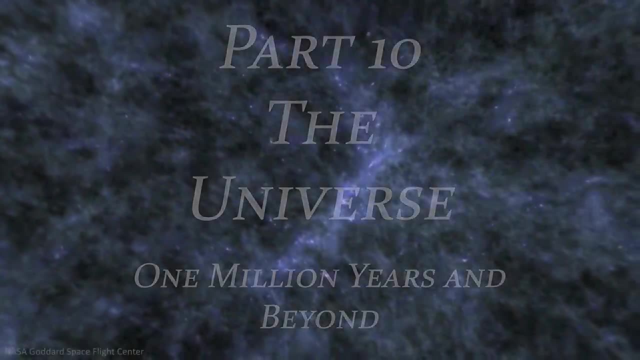 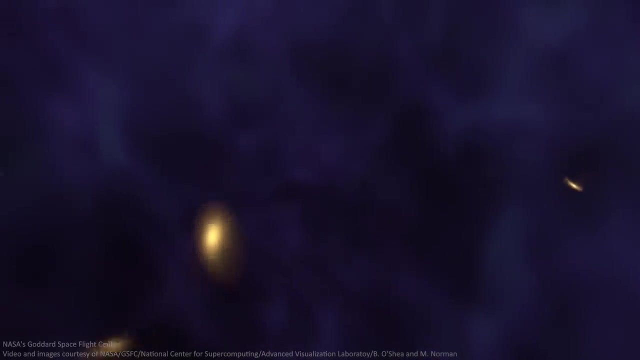 mysteries. A bright twinkle of light ignites in the blackness of space. First one, then another, then a cascade of pinpoints light up. A cluster grows, swelling in size and gradually brightening with the light of even more young stars, and within a few billion years is large enough and massive enough to reach the stars. The universe is now a cluster of stars and the light of the stars is growing and growing in size and gradually brightening with the light of even more young stars and, within a few billion years, is large enough and massive enough to reach the stars. The universe is now a cluster of stars and the light of the stars is growing and growing in size and gradually brightening with the light of even more young stars. The universe is now a cluster of stars and the light of the stars is growing and growing. 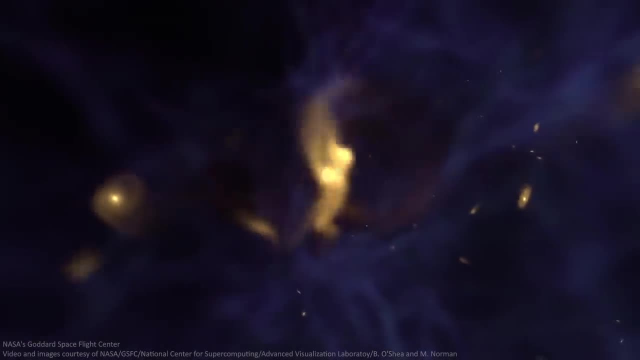 in size and gradually brightening with the light of even more young stars and within a few billion years, is large enough, and massive enough to begin to spin Its own angular momentum is enough to stretch it out at its equator, flattening the cluster. 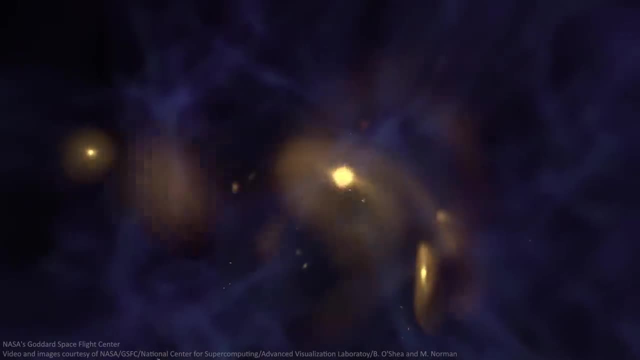 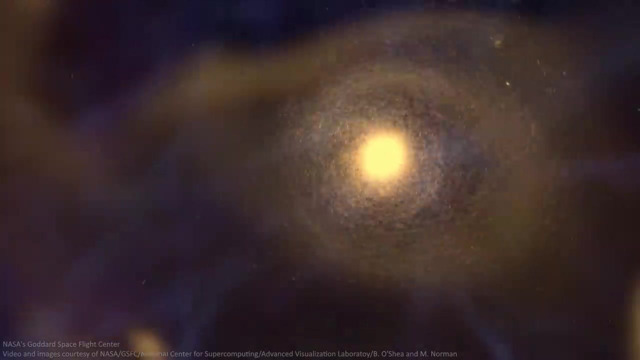 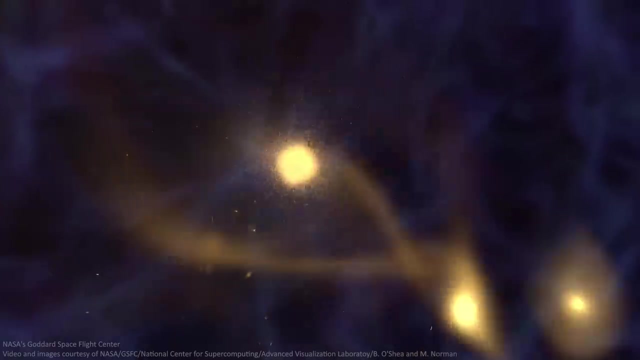 into a disk that whirls at more than 200 kilometers per second, completing a full rotation every 250 million years or so. As this young spiral galaxy wheels through extragalactic space, it captures and absorbs smaller clusters that line its path. Head-on collisions with other spinning galaxies result in mergers which seed the original. 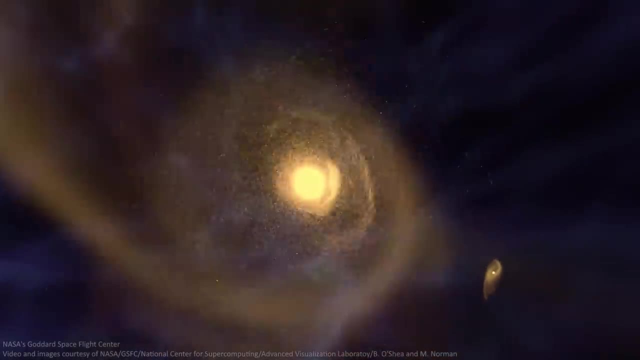 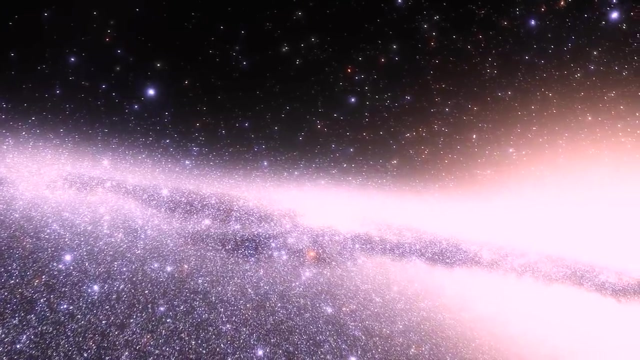 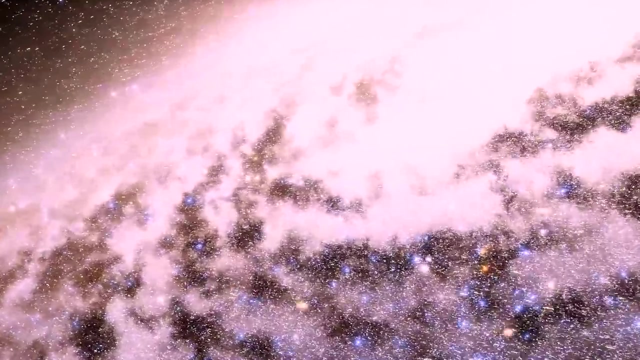 spiral with new material for a frantic burst of star formation. It is some 10 billion years ago and our Milky Way galaxy is in the prime of its life. For a few billion years, within the rippling spiral arms of the Milky Way massive stars. 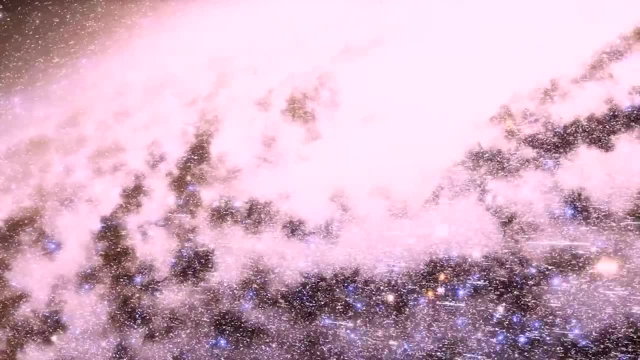 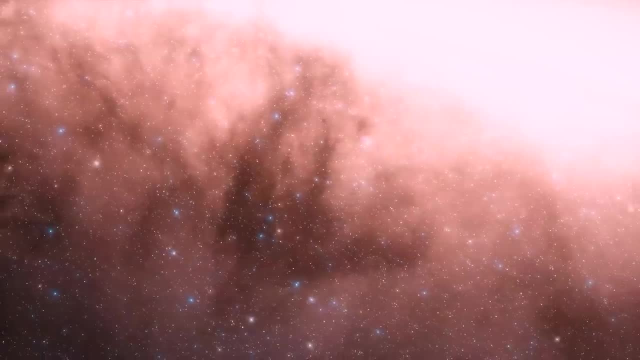 ignite, burn furiously and die dramatically, shedding their spent fusion fuel back into the galactic cloud for recycling. This gas is enriched with the heavier elements that are formed by the fusion of the galaxy during stellar nuclear fusion and provide the foundation for an entirely new generation. 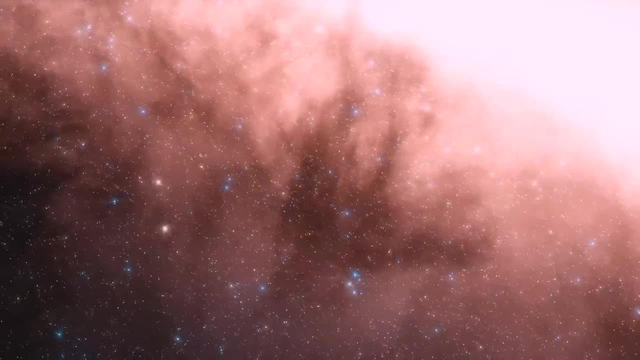 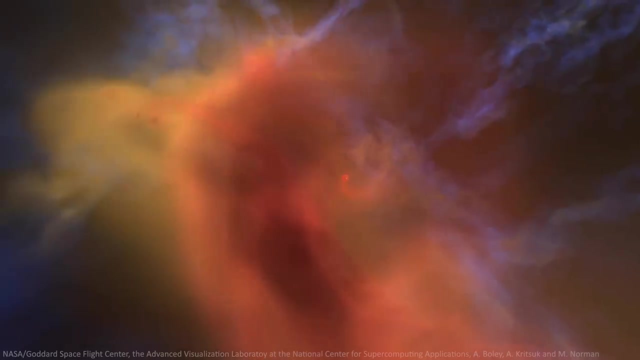 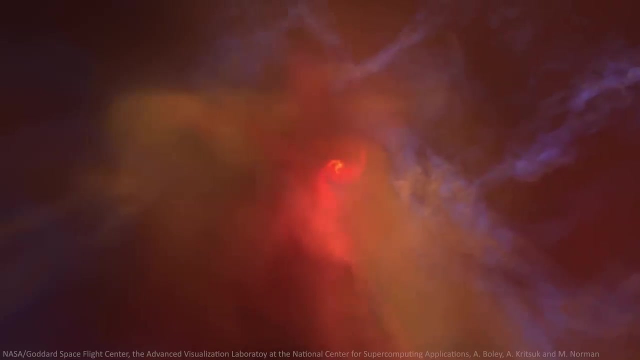 of stars and, for the first time, planetary systems Late to the star-forming party. on a fragmented spiral arm some 25,000 light-years from the galactic center, one such star sputters into existence around 4.6 billion years ago. 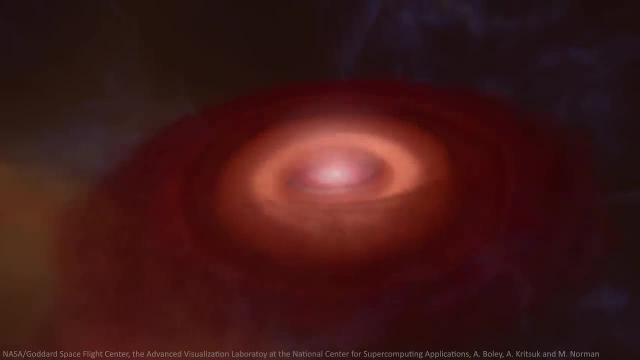 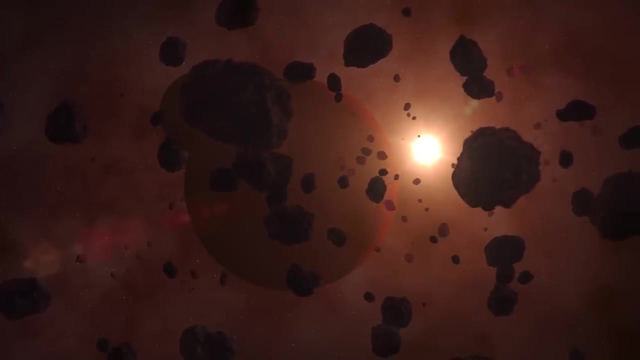 And, like the galaxy itself mirrored on a smaller scale, dust and gas whirl around it in a flattened disk. Dust becomes pebbles, pebbles become boulders and eventually boulders become entire rocky worlds. These rocky worlds jostle for a stable position around the yellow star and, after a few catastrophic 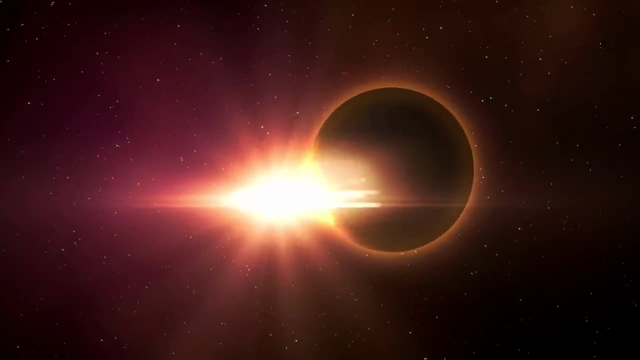 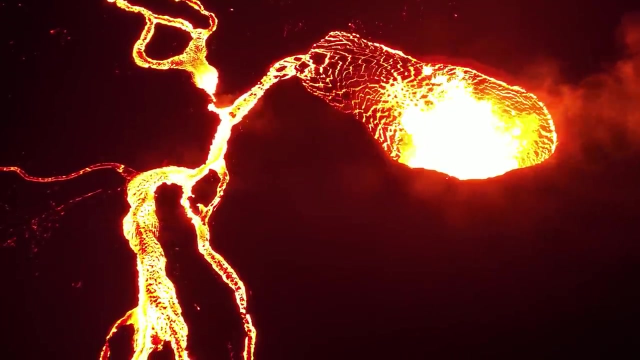 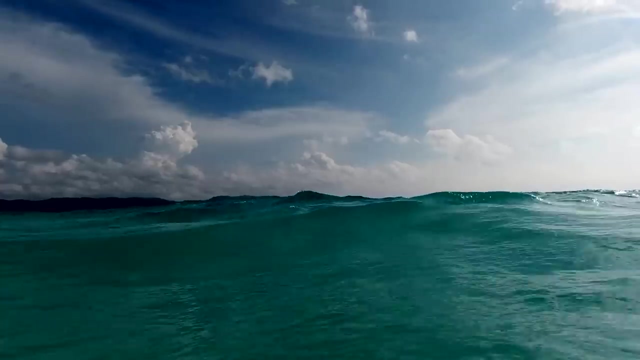 collisions eventually settle into orbits, they will occupy for the next four and a half billion years On the third such rocky world from the sun. as the heat from its violent formation dissipates, water condenses to make oceans and atmospheres and plate tectonics begins the slow recycling. 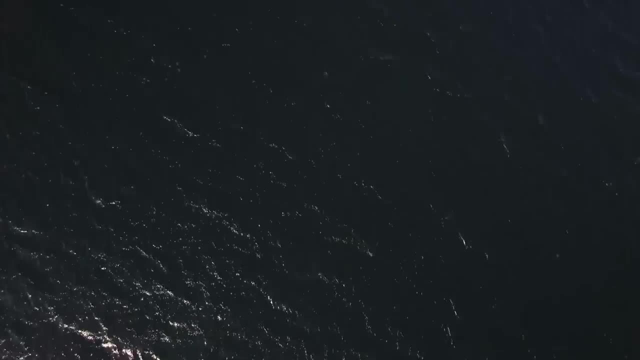 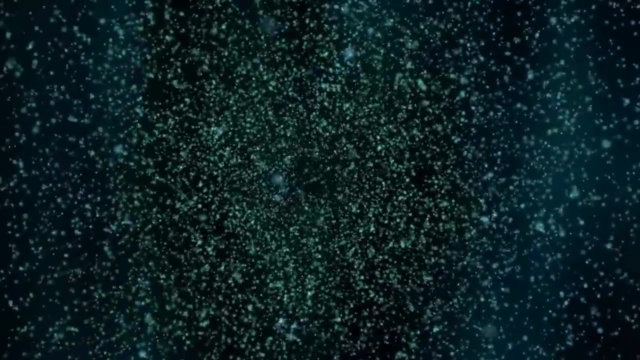 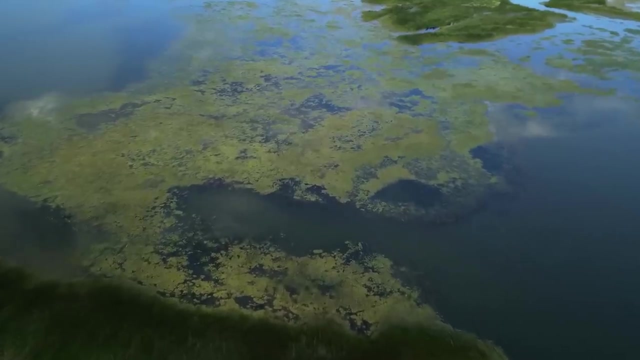 of rock at the planetary surface, Somewhere inside the oceans, somehow a spark of life ignites, finds its feet and adapts and evolves, filling this unique world with an entirely new kind of creation. Chemistry becomes biology, as a multitude of lifeforms swarm the sea, land and sky. 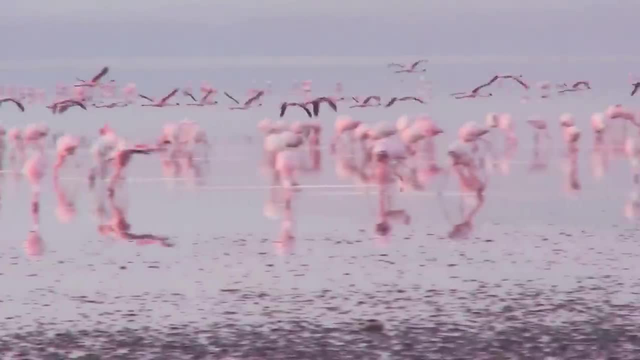 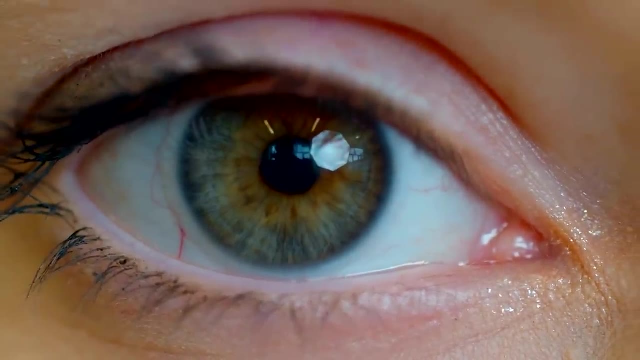 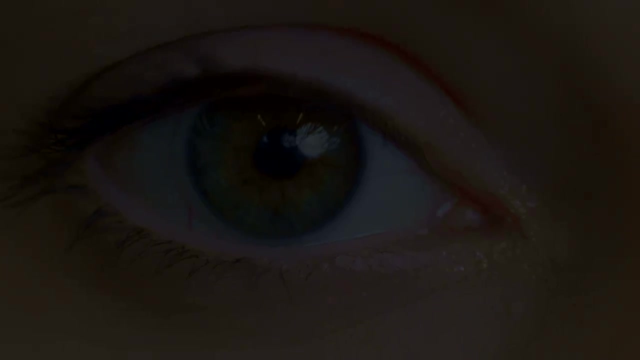 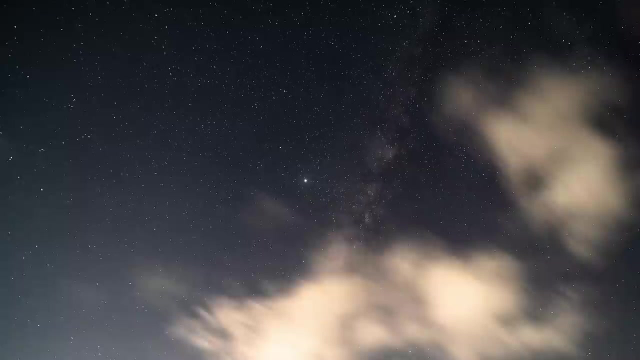 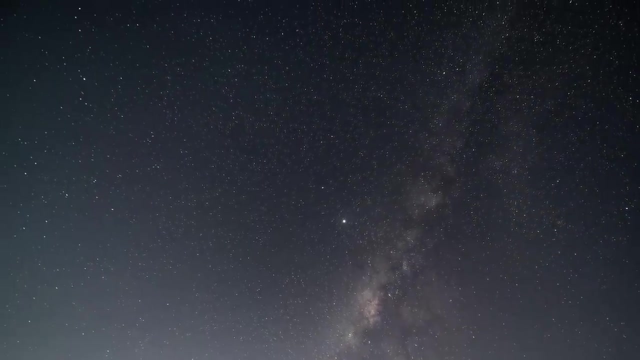 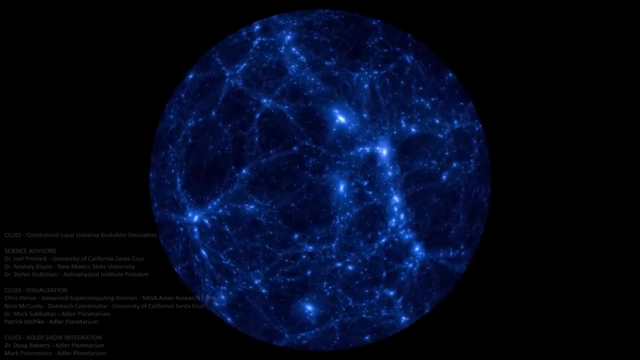 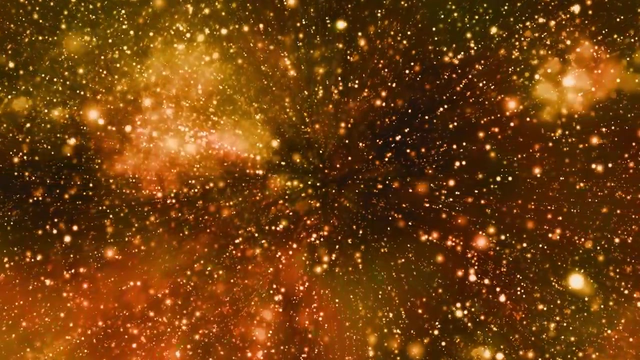 And then, as if from nowhere, a sentient mind appears to contemplate its place in the universe. And then, as if from nowhere, a sentient mind appears to contemplate its place in the universe 380,000 years after the Big Bang light has finally escaped its matter prison. 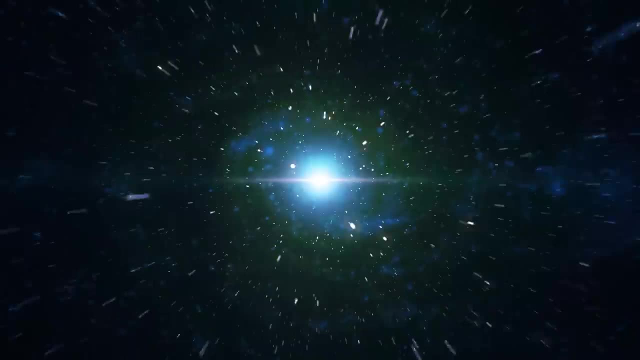 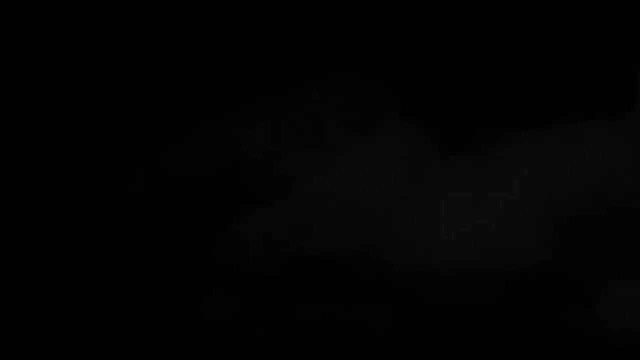 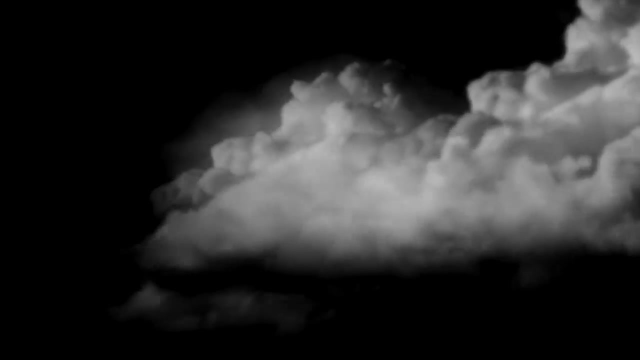 Photons can travel freely through the expanding cosmos, but lose energy as it grows. The universe may no longer be opaque, but it is… dark. The fierce energy of formation has faded, and it will be millions of years yet before a new process, nuclear fusion, comes to concentrate energy once again. 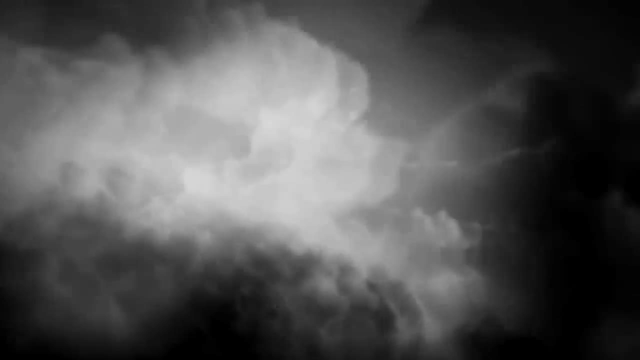 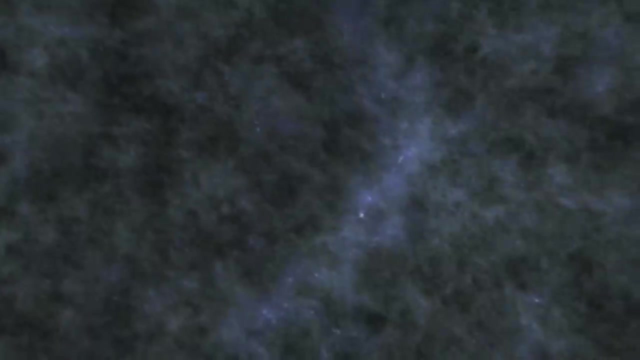 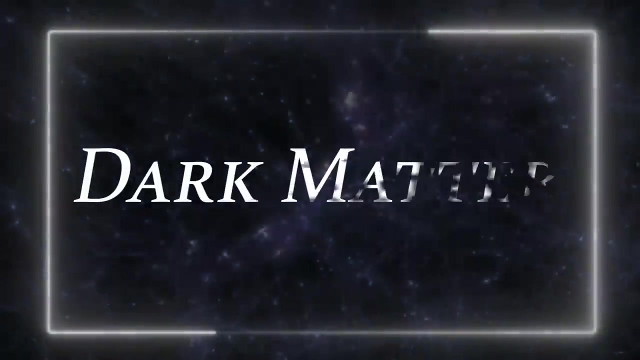 These are the dark ages of the universe, and there may be little to see, but this doesn't mean there is little going on. Indeed, it is during this time, up to and beyond the first million years of cosmological history, that scientists believe dark matter steps up to shape the future of the universe. 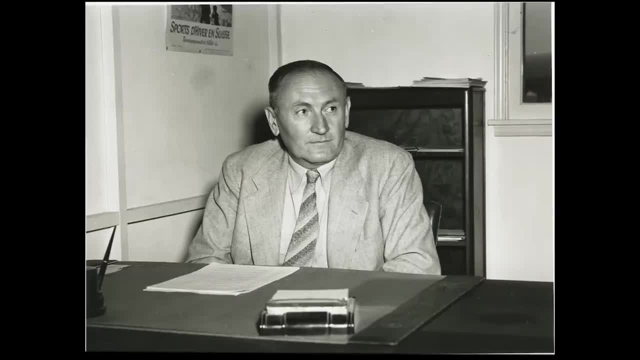 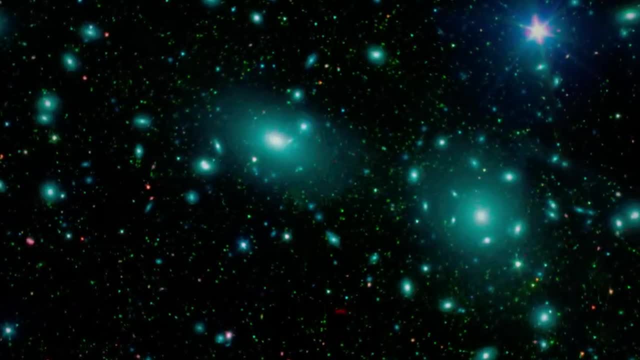 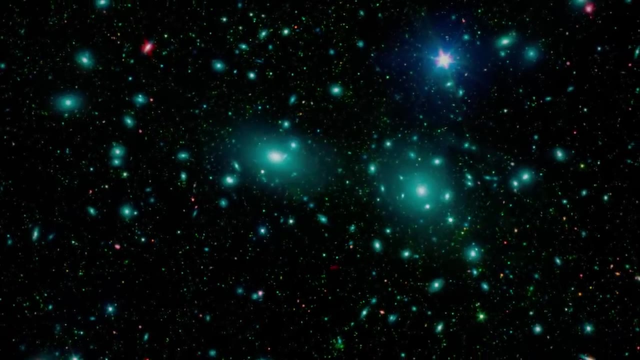 The existence of dark matter was first considered in 1933, when Swiss astronomer Fritz Zwicky was studying the Coma cluster of galaxies, some 320 million light years away from the Earth. These galaxies seemed to be moving too fast for the cluster to remain a cluster. 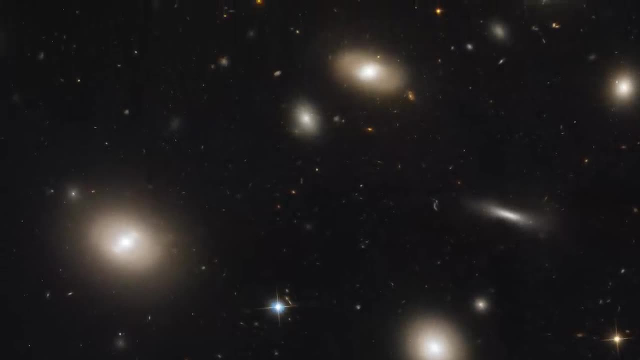 Estimates of the masses of each galaxy in the cluster, based on the luminous stars that could be seen and counted, gave a number that was some ten times less than what would have been needed to keep the group together. The dark matter was first considered in 1933, when Swiss astronomer Fritz Zwicky was studying the Coma cluster of galaxies. 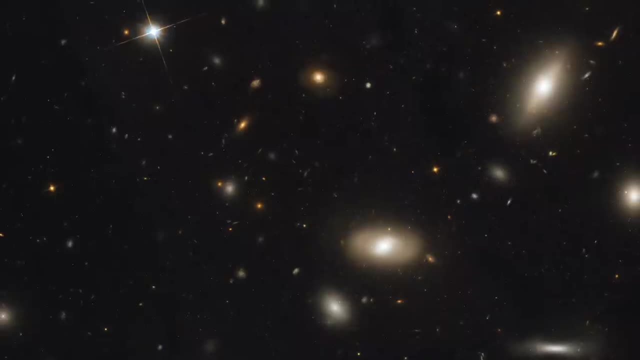 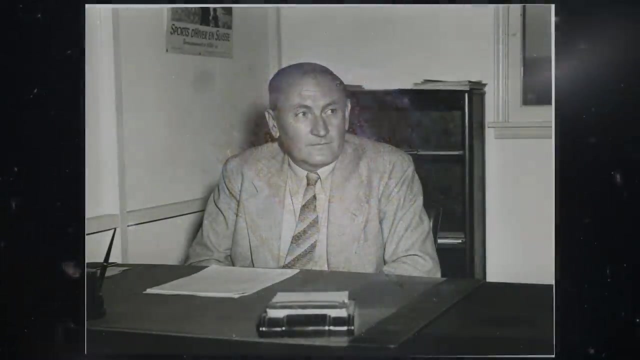 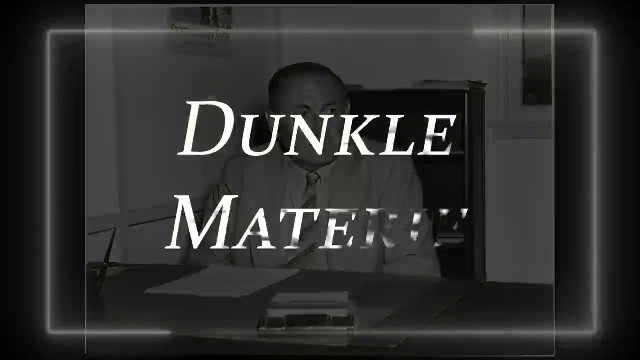 together, given how fast the galaxies were moving. To explain this apparent discrepancy between the two methods of determining mass, Zwicky proposed that there must actually be a lot of unseen mass lurking out there amongst the stars, gas and visible matter. He called it Dunkelmaterie- German for dark matter. 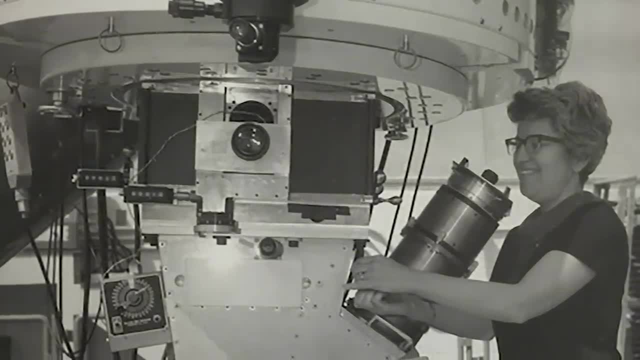 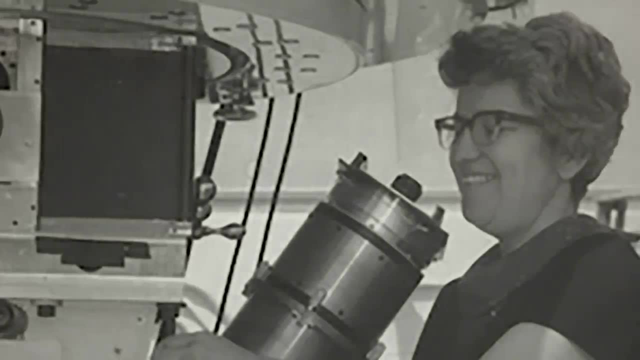 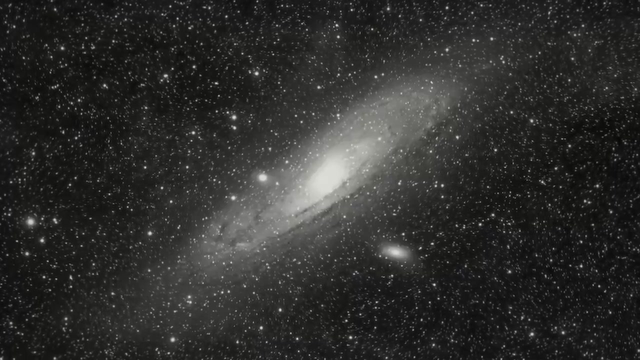 In the late 1970s, pioneering astronomer Vera Rubin was studying the rotation of the Andromeda galaxy, the closest spiral galaxy to our own, when she noticed that something didn't add up in the motions of its stars. At the time, she and her colleagues studied cryptic punch card readouts from their instruments. 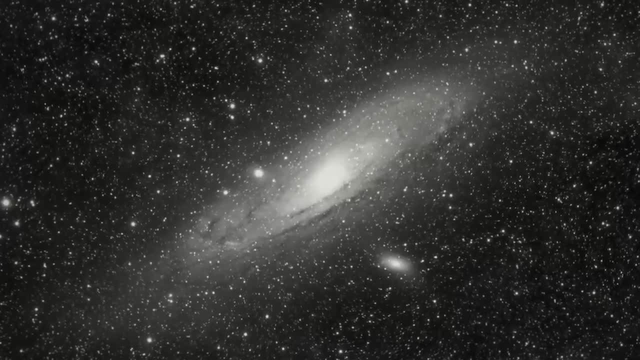 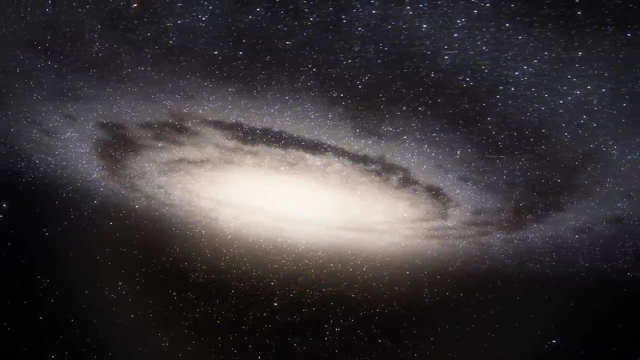 but to this seasoned astronomer the problem was as clear as day. Galaxies were expected to spin fast, close into the centre, while stars at the edges would make a more stately progression. but the punch cards were telling a different story. The stars at Andromeda's outer edge seemed to be 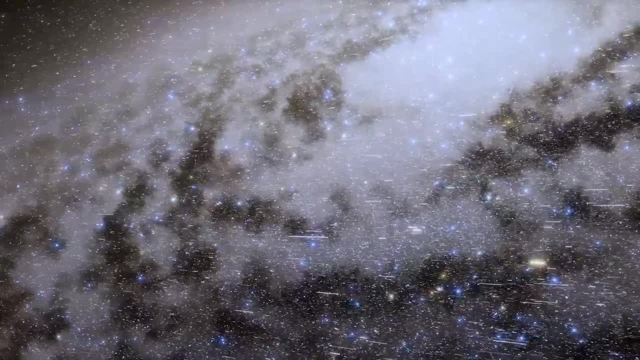 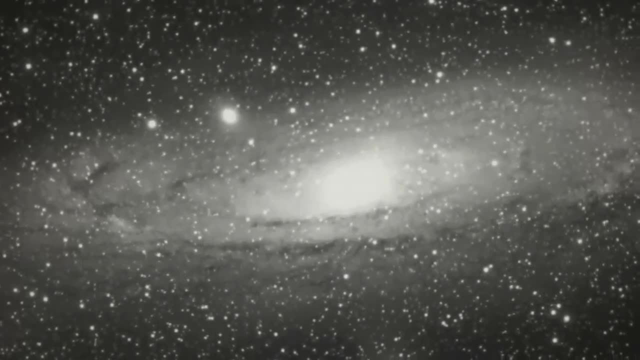 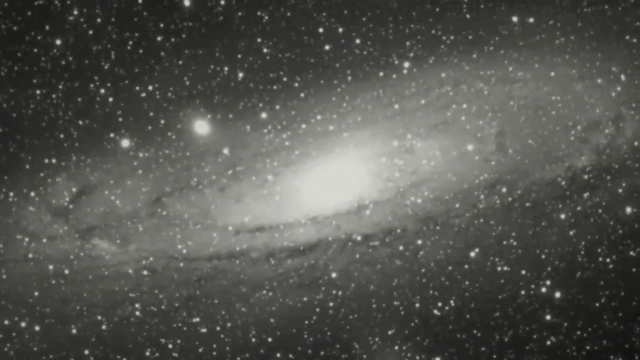 moving just as fast as those in the central bulge, with the tips of its spiral arms whipping around with implausible speed. The only explanation for such a movement, without violating the universe's fundamental laws of motion, was that the stars themselves were only a part of the overall mass of the galaxy. 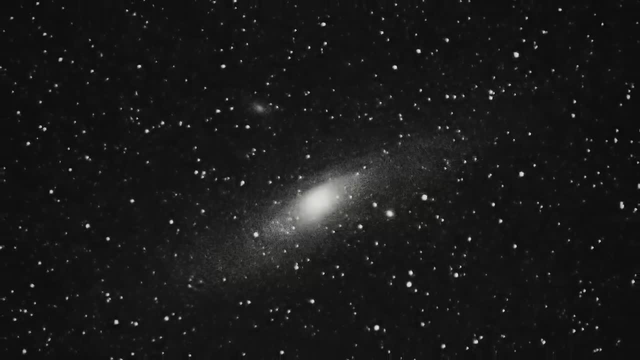 Rubin calculated that the visible matter must represent just 15% of what was really there and that the Andromeda galaxy must be cocooned in a much larger hemisphere. The stars themselves were only a part of the overall mass of the galaxy. 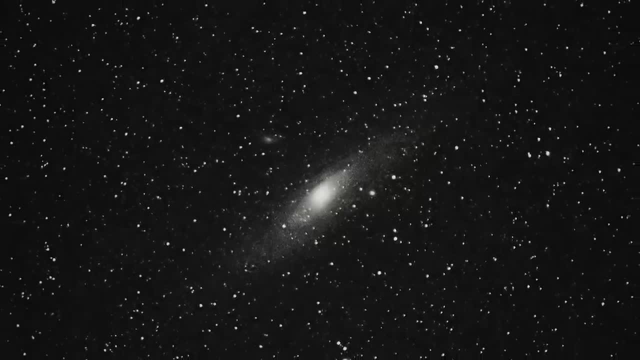 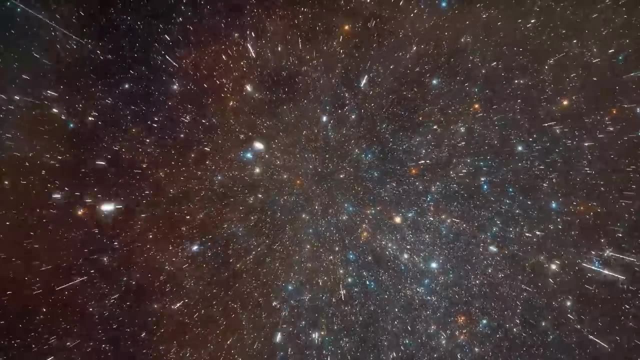 The stars themselves were only a part of the overall mass of the galaxy. The stars themselves were only a part of the overall mass of the galaxy. Subsequent observations revealed that most galaxies are surrounded in this way, including our own. Indeed, current estimates suggest that the Milky Way's dark matter, halo, could be up. 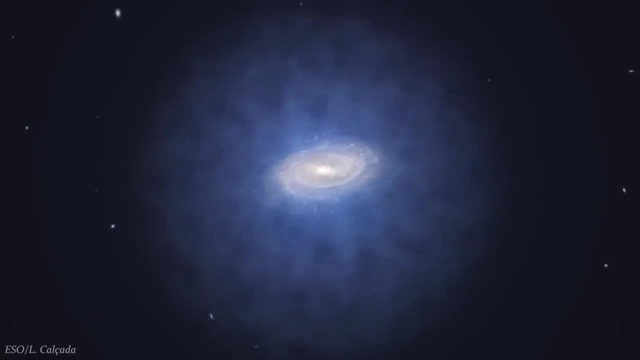 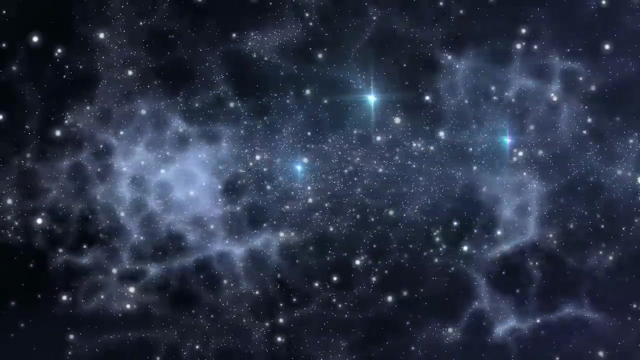 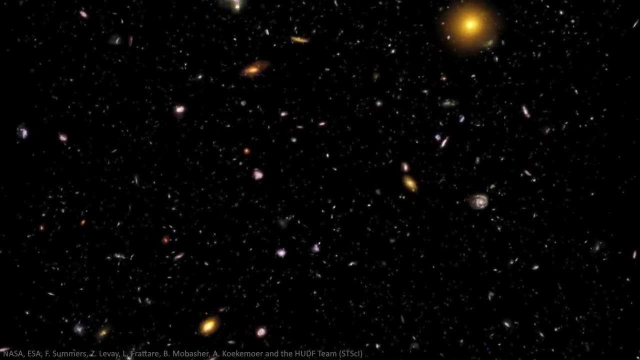 to 15 times larger than the visible extent of its stars, And so astronomers are now convinced of dark matter's significance in shaping the modern universe, despite our continued inability to detect it. Larger scale studies suggest that dark matter outweighs normal matter six to one. 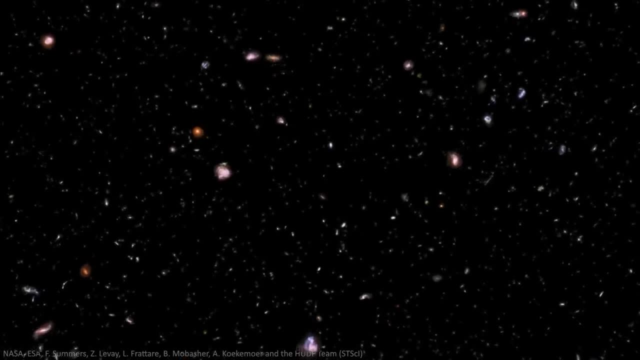 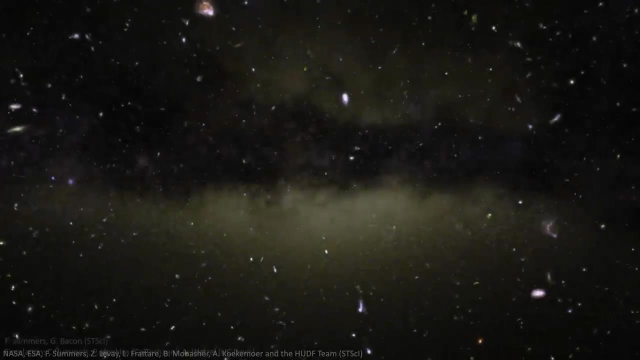 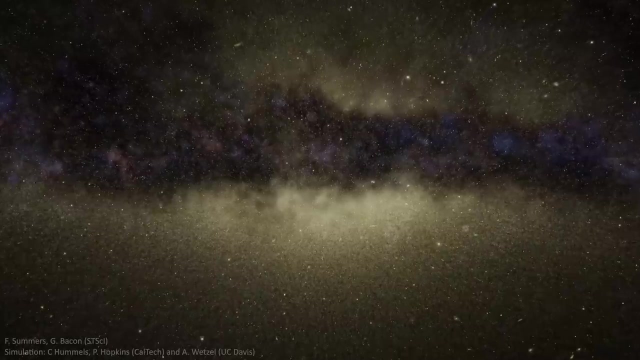 and potentially always has. But what exactly it is remains a mystery even after several decades of concerted study. One possibility is that the dark matter in the universe consists of ordinary objects made up of normal baryonic matter, like quarks and leptons. 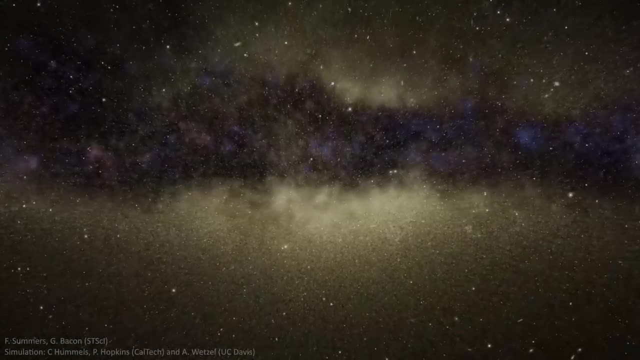 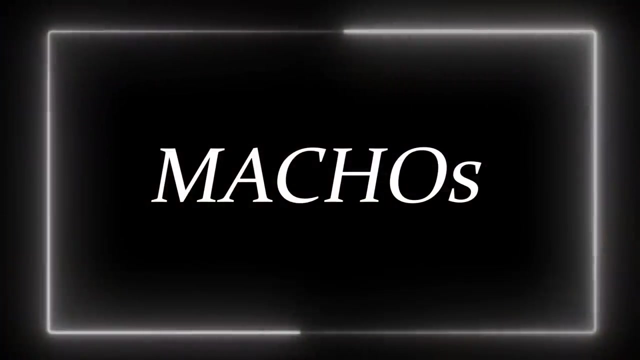 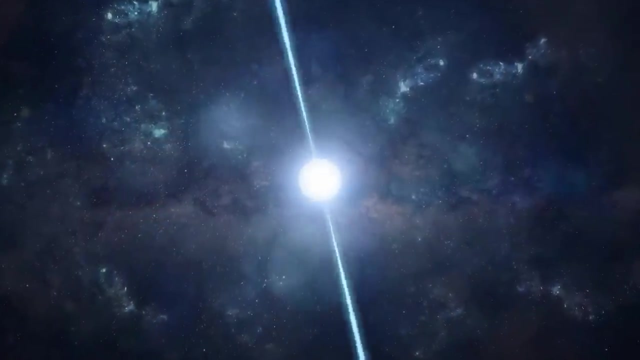 but which are hard for us to detect with our current technologies, Known as Massive Compact Halo Objects. these are more often referred to as Machos. Such objects could be black holes of a wide range of sizes, small but incredibly dense and massive neutron stars created when giant stars collapse at the end of their lives or an extraordinary 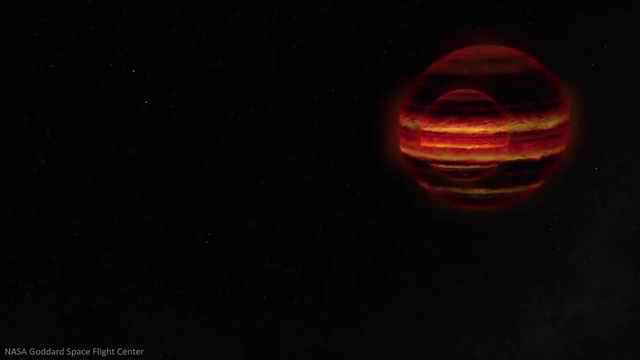 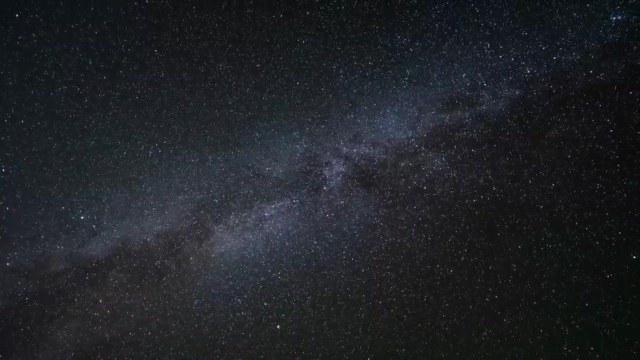 number of brown dwarfs which contain almost as much mass as a star, but not quite enough to ignite fusion. However, as our telescopes and instruments improve and we are able to probe, we are able to detect and we are able to detect, and we are able to detect and we are. 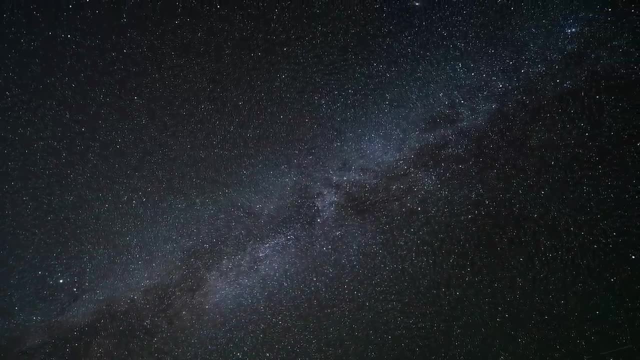 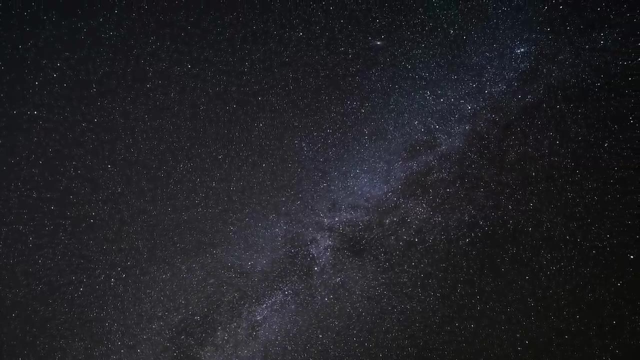 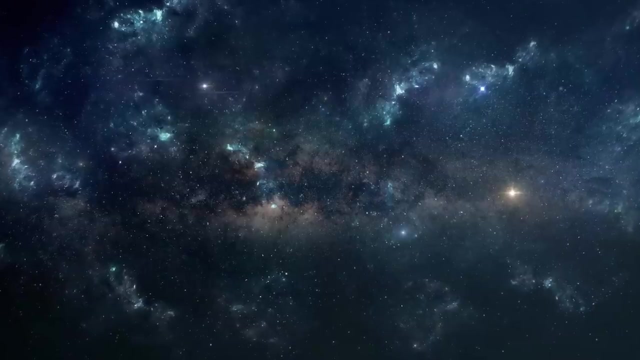 able to probe the depths of intergalactic space in ever more detail. the chances of such objects in sufficient number continuing to escape our notice grow smaller and smaller with every passing year. Because of this continued lack of observational evidence, an alternative possibility is currently favoured among cosmologists that the majority of dark matter 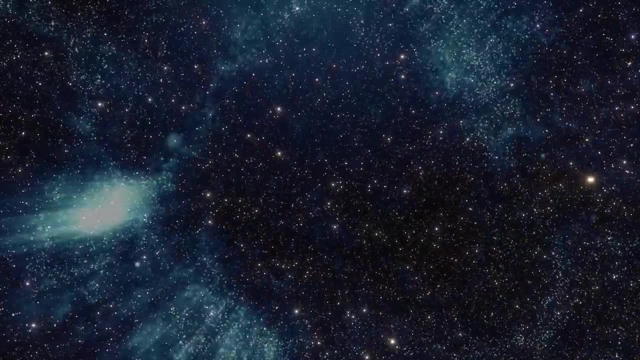 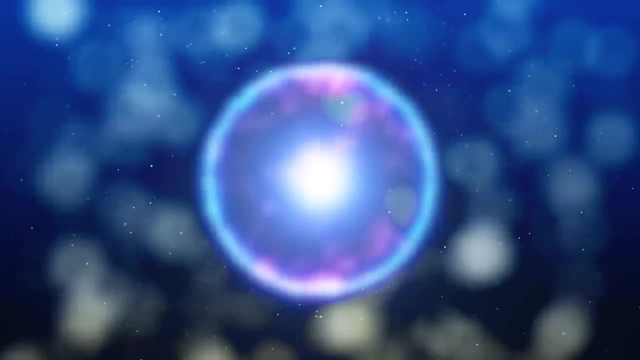 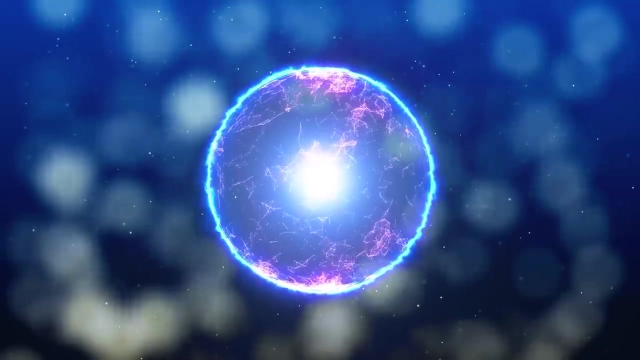 exists as a weakly interacting massive particle correspondingly nicknamed WIMPS. These would be a completely new kind of particle which would sit outside the standard model as we understand it today, but which we have so far failed to detect. They would not interact with. 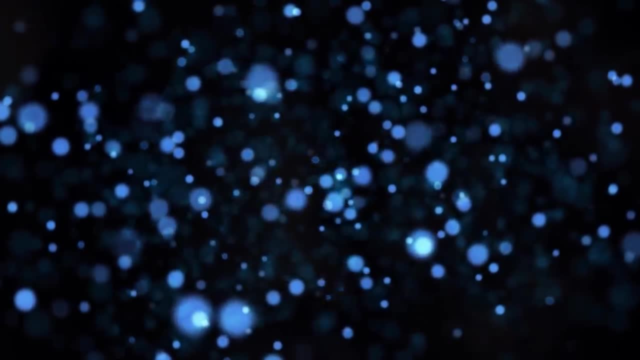 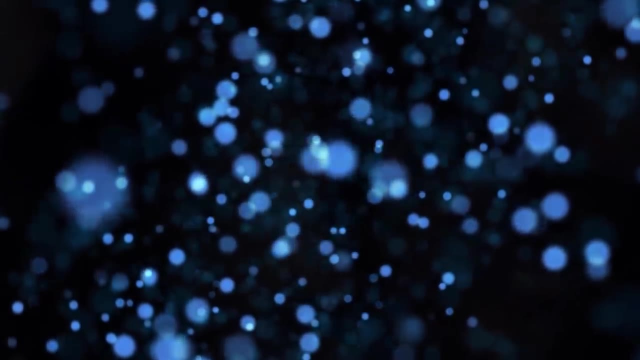 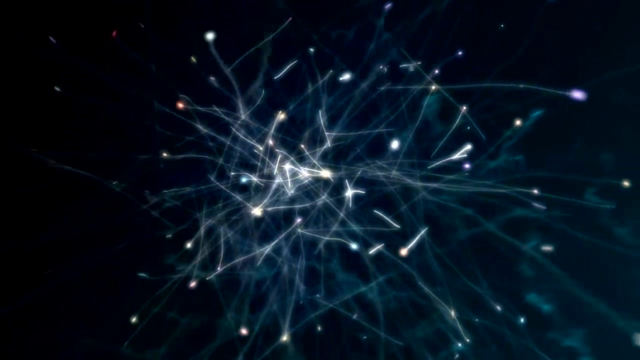 normal matter via any of the known fundamental forces except for gravity, but would nevertheless have a high mass or be present in sufficient numbers to make up for the universe's 85% missing mass. And indeed the search is on in particle accelerators and out in the cosmos, for 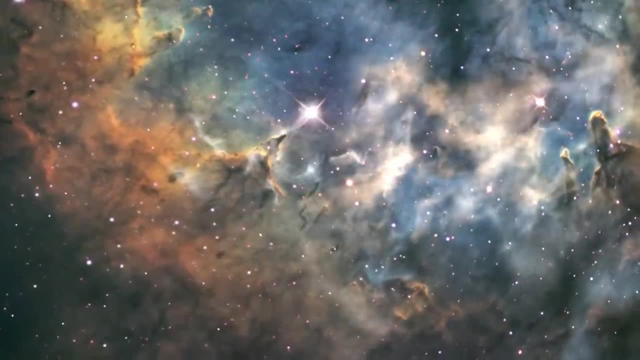 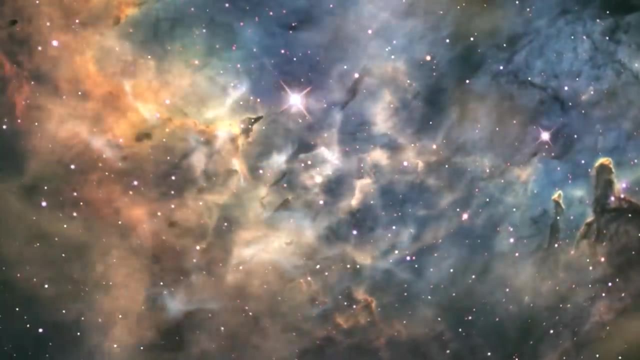 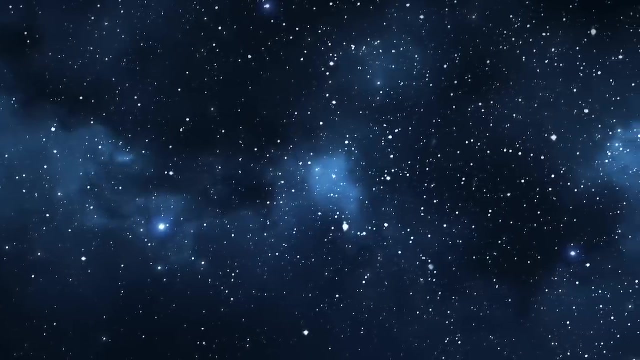 any hint of these heavyweight WIMPS. But with so little to go on, we may have a long road ahead of us. Regardless of whether dark matter is a macho or a WIMP or something else entirely, it is likely that it has always been around sitting in the shadow of tangible matter. 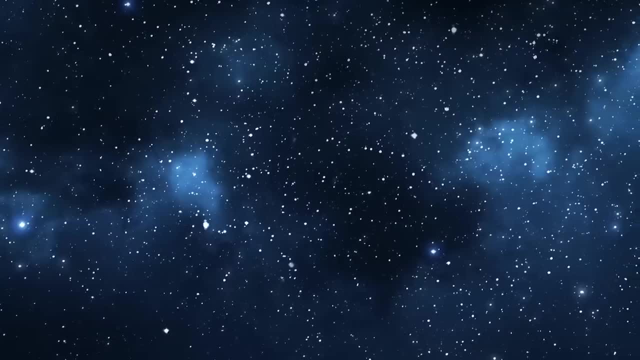 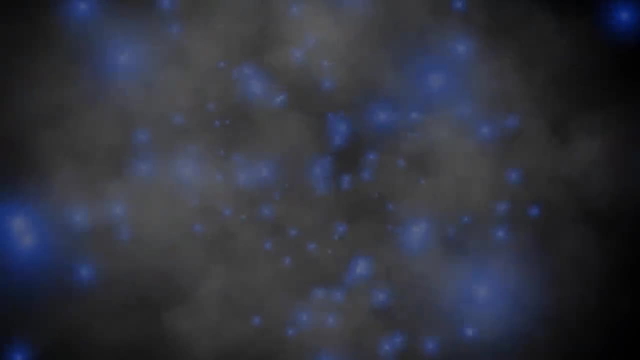 since its creation in the universe's first few fractions of a second, And it was back in the cosmic dark ages, around a million years after the Big Bang, that it began to shape the overall structure of the universe. The cosmic microwave background suggests that 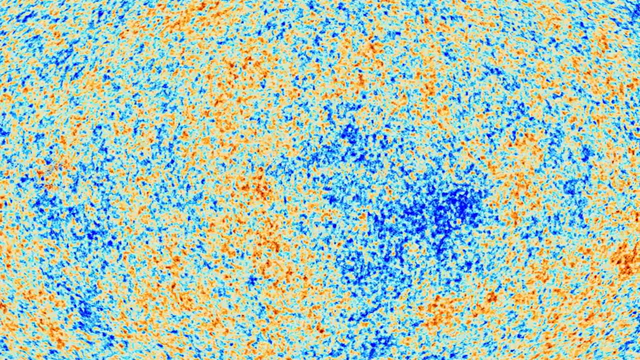 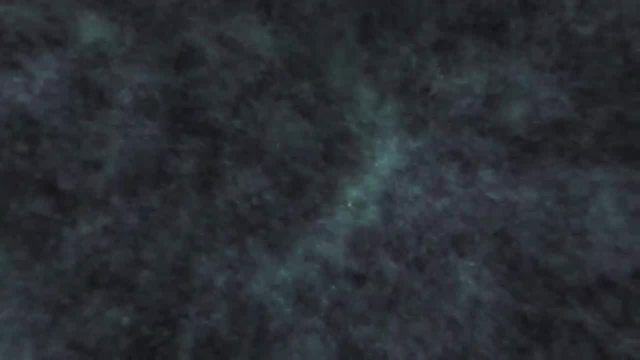 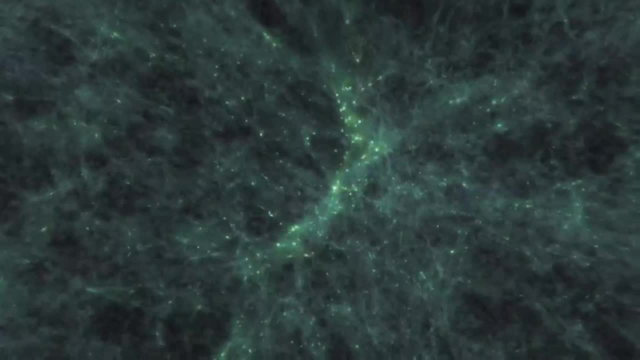 matter and energy were distributed unevenly at the moment of atomic recombination, and so we can expect that dark matter followed suit. But in these darkened millennia, all that mass comes into its own Gravity, pulls the dark matter together, clumping it more quickly, and 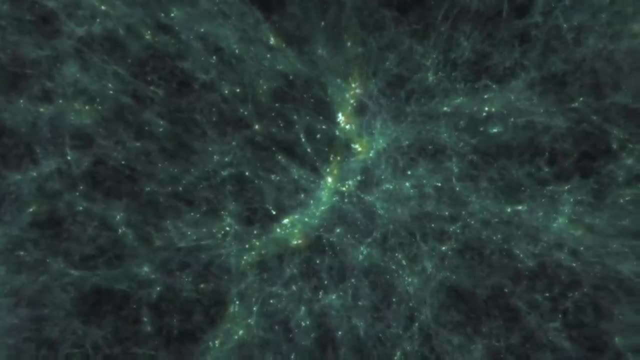 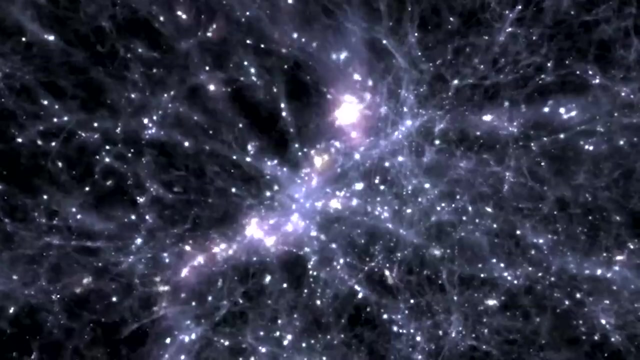 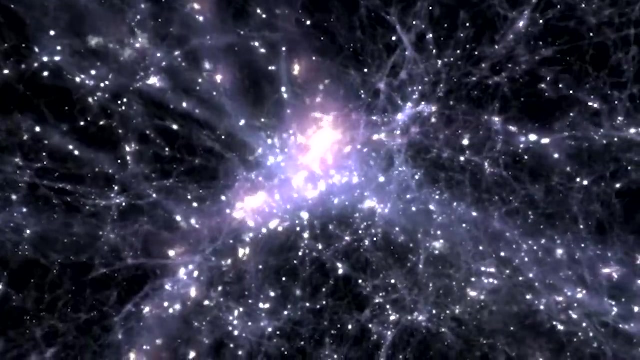 more thickly than we would expect the baryonic matter to collapse by itself. The normal matter then has a dark matter template to follow and is sucked into invisible gravity wells, thus creating cosmos-spanning filaments, nodes and clusters of gas that will become the nurseries. 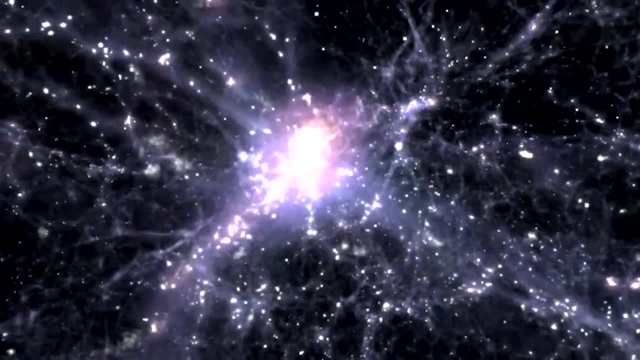 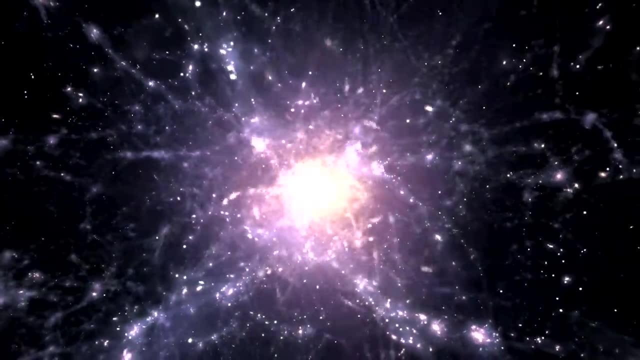 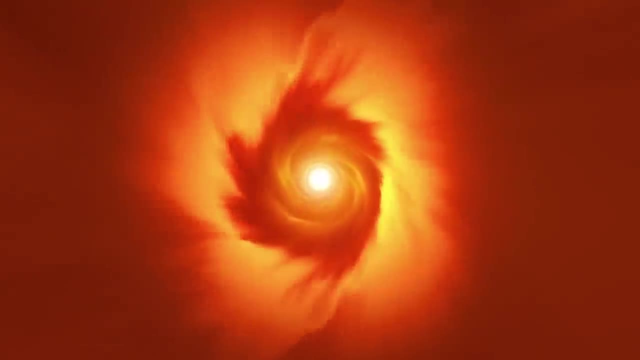 for the first stars and galaxies, And from this point on, the evolution of the universe we see today has become inevitable. Everything that has happened up to this point, spanning the first million years of the cosmic chronology, has set the course of the universe's evolution. 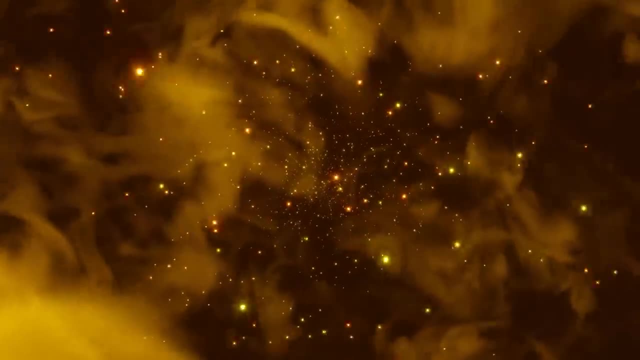 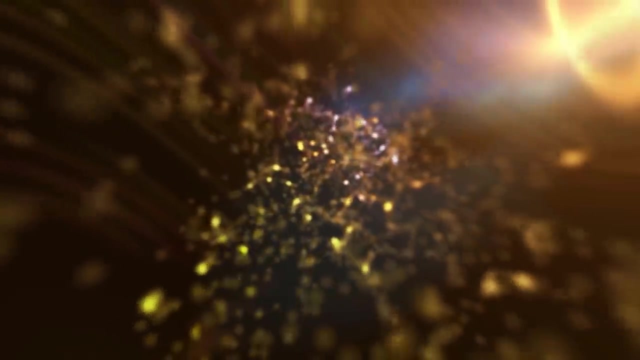 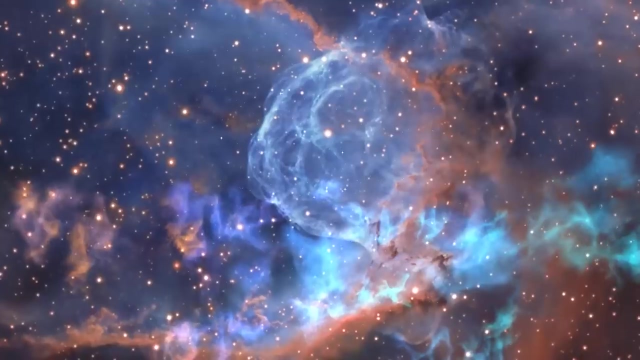 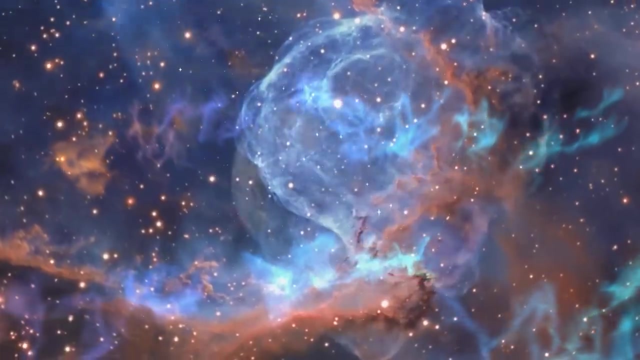 The universe has cooled to a point where comprehensible physics holds sway. The four forces have settled and become distinct, determining all fundamental interactions, And the nature and quantities of matter have settled to provide the ingredients for generations of stars and galaxies, the genesis of chemistry and the ultimate creation of life. 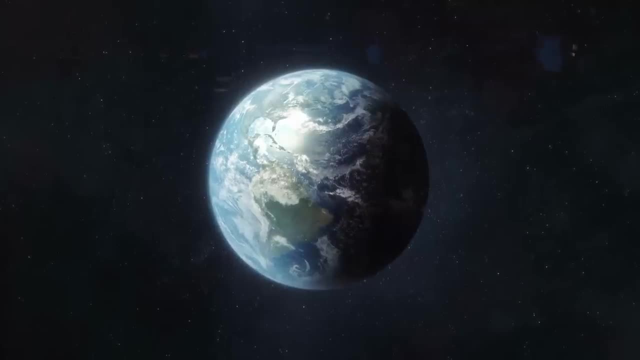 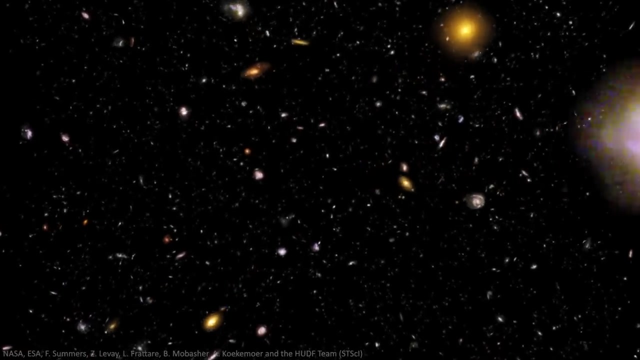 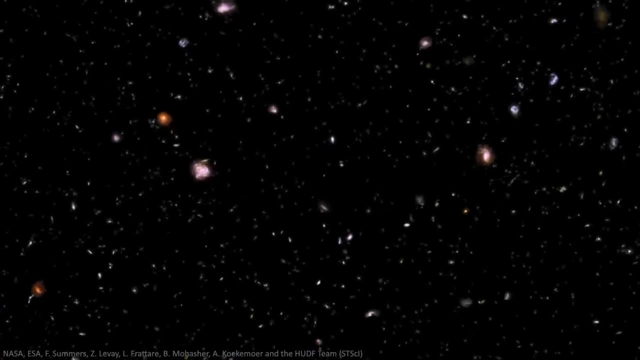 But that is not quite all. For 8 billion years, events in the universe unfolded just as we would expect them to with these basic ingredients. But between 5 and 6 billion years ago, not long before the formation of our solar system within the Milky Way, something changed. 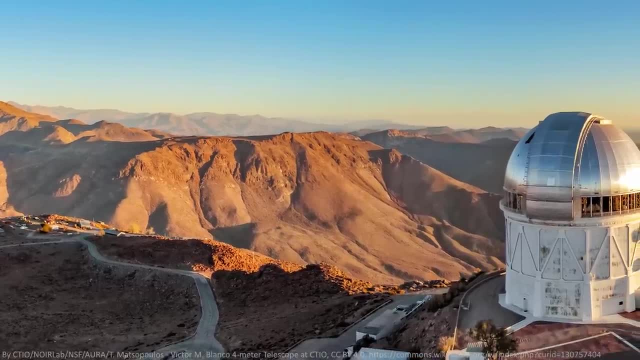 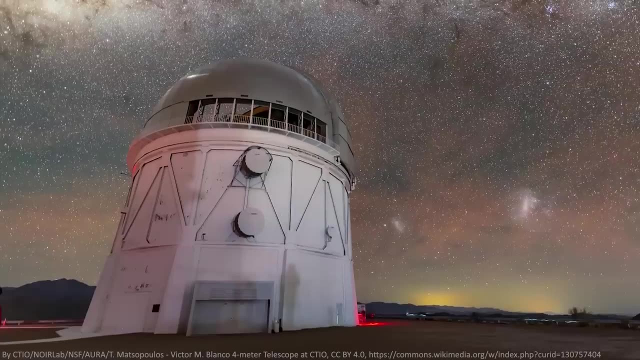 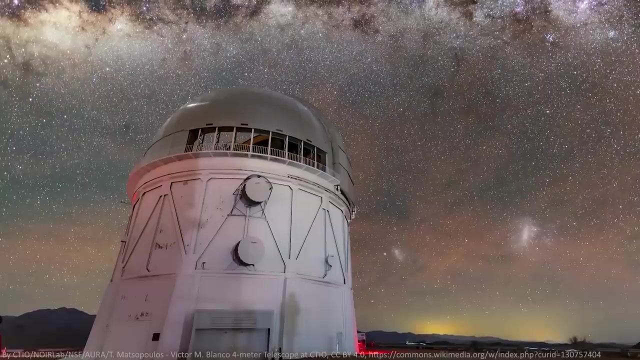 And discovering that something 25 years ago made it clear that we still don't really understand The balance of the universe. This disturbing change in the evolution of the universe was first recognised in 1998, when astronomers were studying supernovae at different points in space and time. 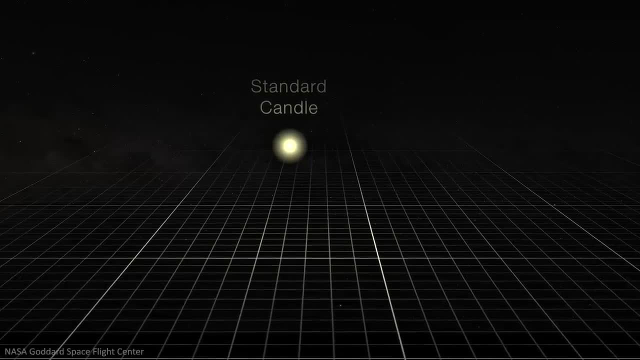 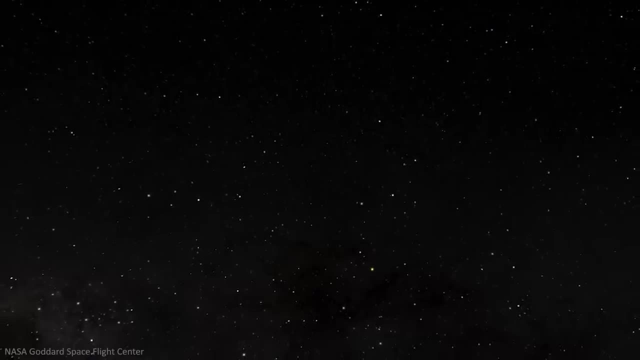 Supernovae of a certain size are sometimes known as standard candles, because they explode with a known and predictable brightness and luminosity. As a result, they have become valuable tools for measuring cosmic expansion, since their light will be stretched into redder wavelengths with the expansion of the 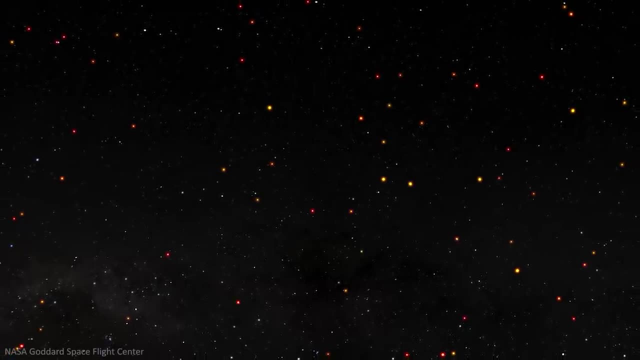 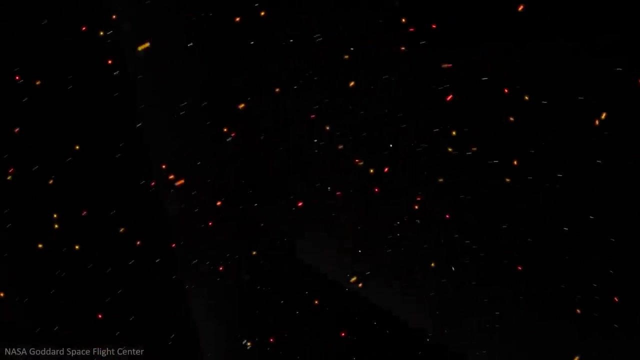 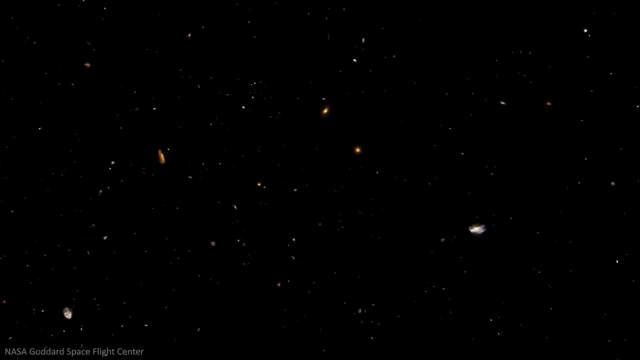 space between them and our instruments, But astronomers noticed that for the last 5 billion years or so, the supernovae are more redshifted than they should be and so have been moving away from us faster than they should, A pattern that can also be seen in measurements of baryonic acoustic. 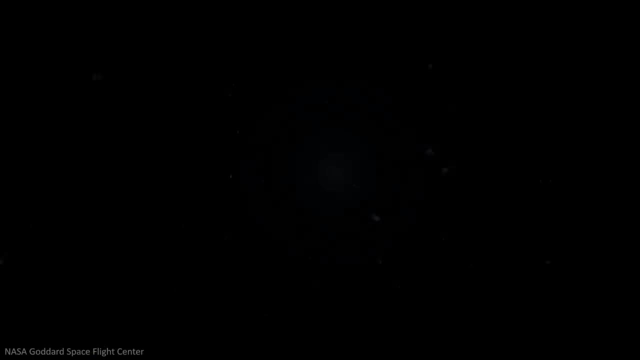 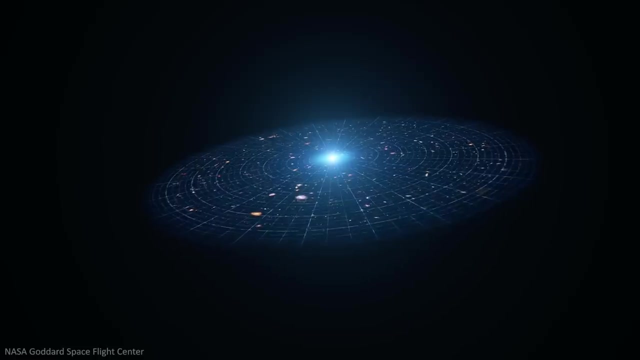 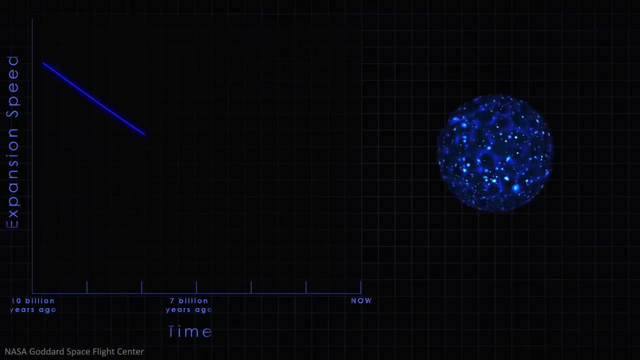 oscillations and galaxy clusters. Not only that, but the accelerated expansion itself seems to be accelerating. Our best explanation for this most recent phase change of the universe is dark energy, And so for the entire history of our solar system, we have been living in a dark energy. 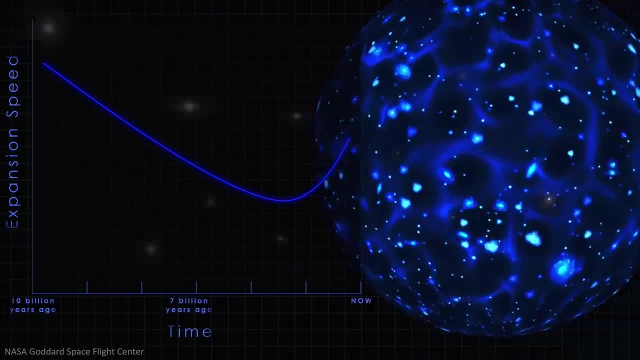 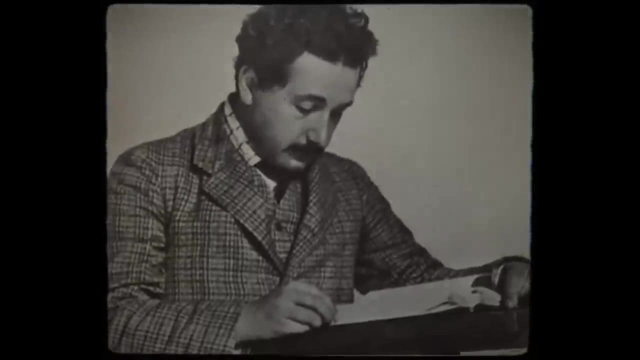 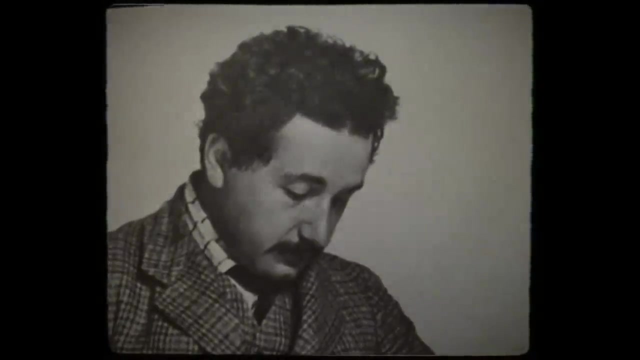 dominated era. As with dark matter, cosmologists still don't have a good idea of what dark energy actually is. When Einstein was formulating his theory of general relativity, he introduced the idea of the cosmological constant representing the intrinsic energy of empty space. 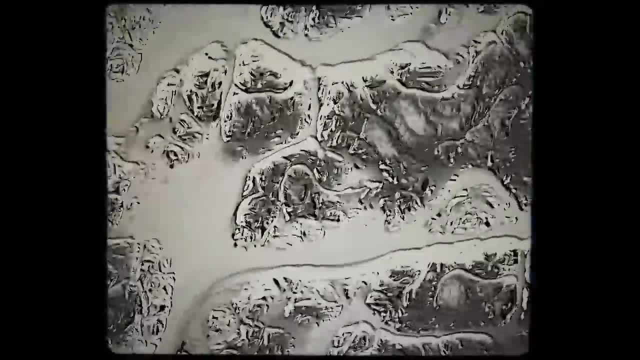 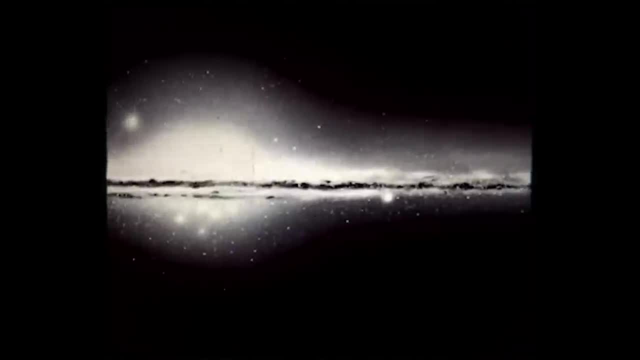 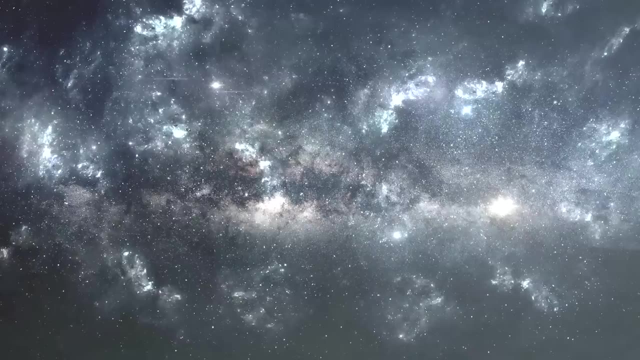 As space expands, there is objectively more of this energy which could serve to drive further expansion. In the end, general relativity didn't need this modifying constant, but the idea has found new life in explaining away dark energy. The problem remains, however, that we do not. 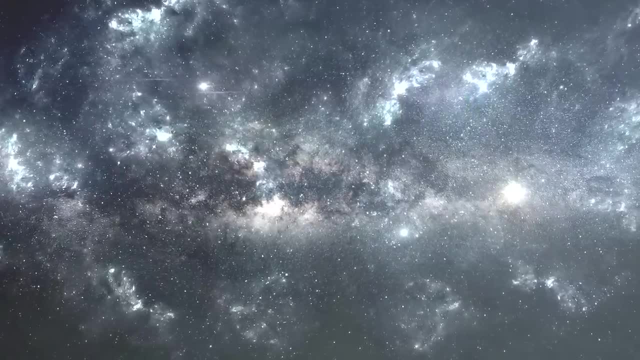 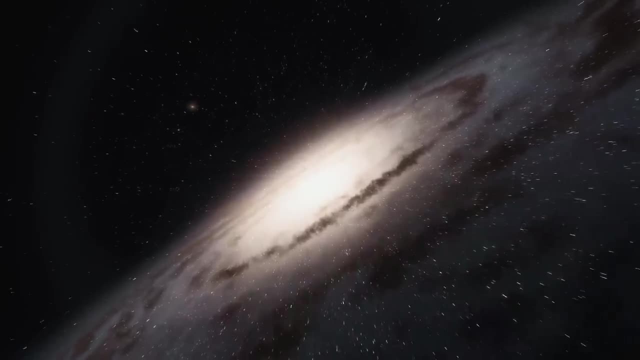 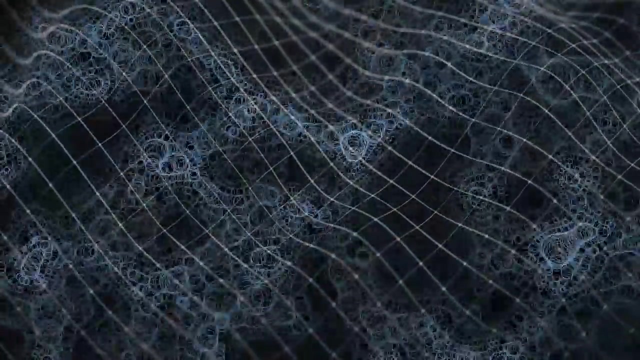 understand why such an intrinsic energy should be present at all. If the explanation cannot be found when searching on cosmic scales, perhaps the physics of the very small holds a clue. Quantum theory predicts a phenomenon known as vacuum energy, in which the virtual particles that spring spontaneously into and out of existence due to random quantum 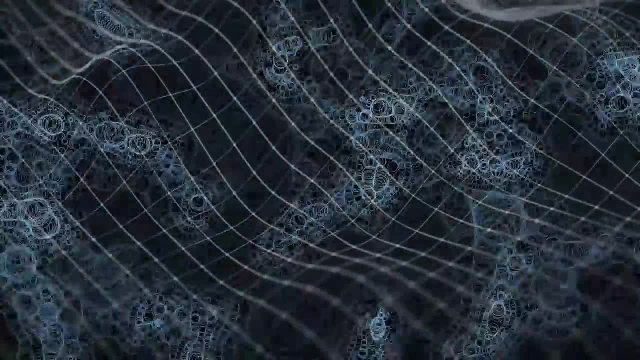 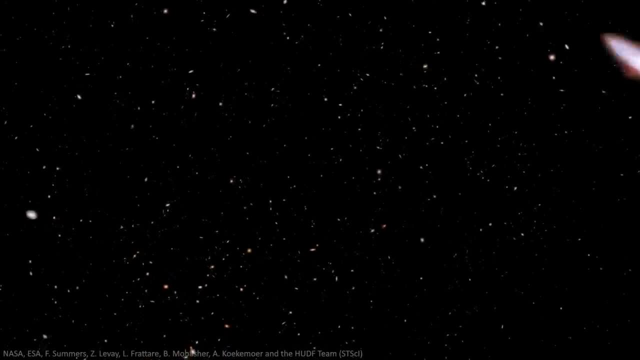 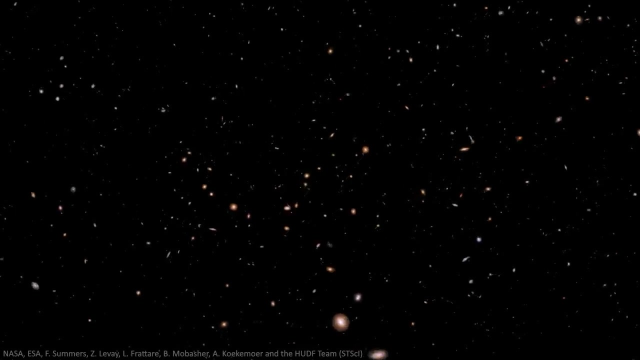 fluctuations exert a pressure causing expansion. It is a promising idea, but calculations that apply this vacuum energy to larger scales come out far too high to properly explain the expansion that we see. Some cosmologists are considering something entirely different, a new kind of energy field called quintessence, which acts in the opposite way to normal matter. 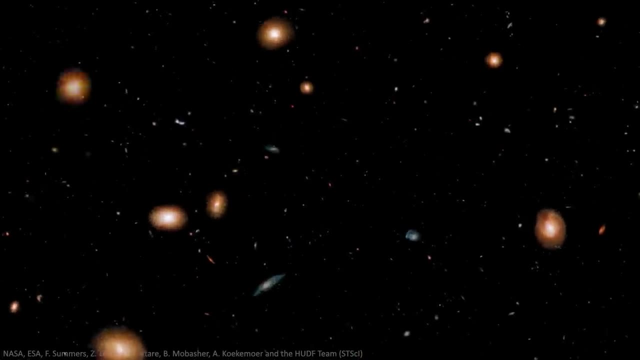 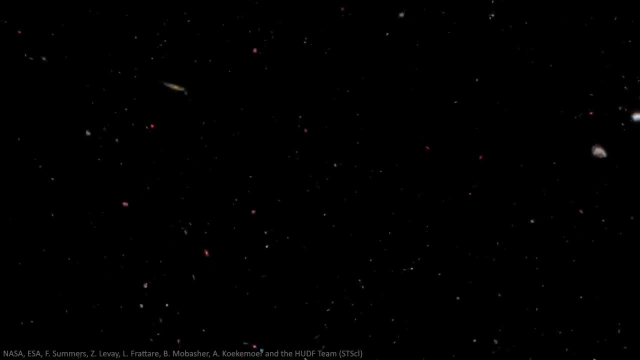 and normal energy can either be attractive or repulsive and can change its behaviour over time. But without experiments or observations that can easily probe that force or even confirm its existence, we are left stranded in the dark as time ticks by and the space surrounding us expands. 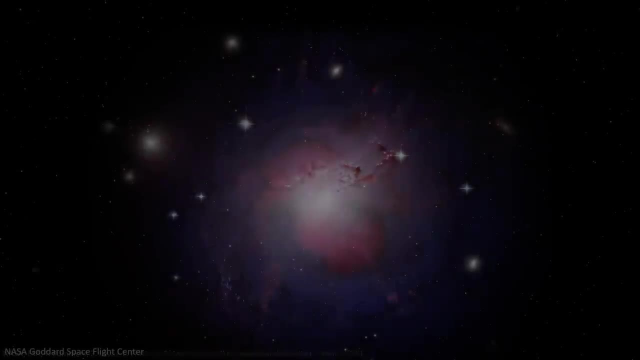 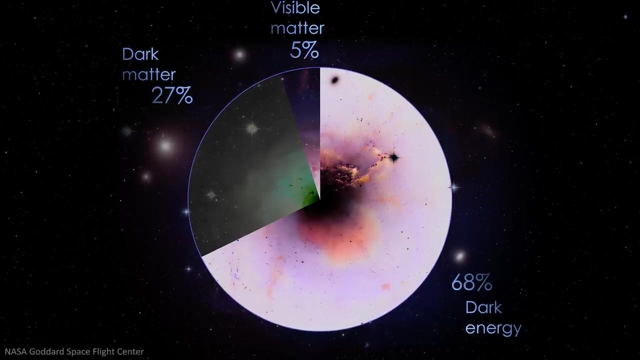 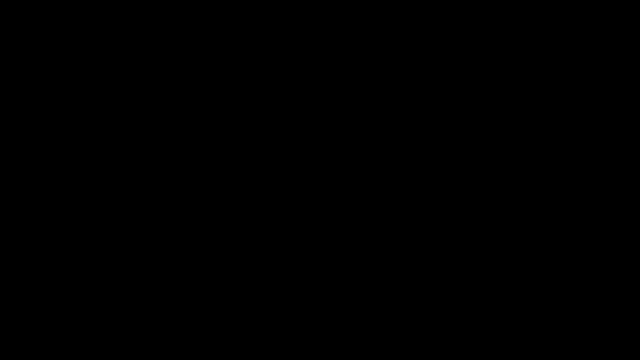 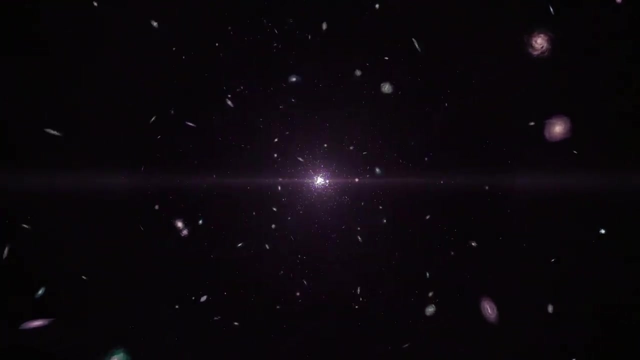 And so, whatever it is, we are left with a universe that is approximately 68% dark energy, 27% dark matter and less than 5% normal matter, And it is from these ingredients that our universe has grown and developed over 13.8 billion years, following the rules and constants that were evident in its very first.